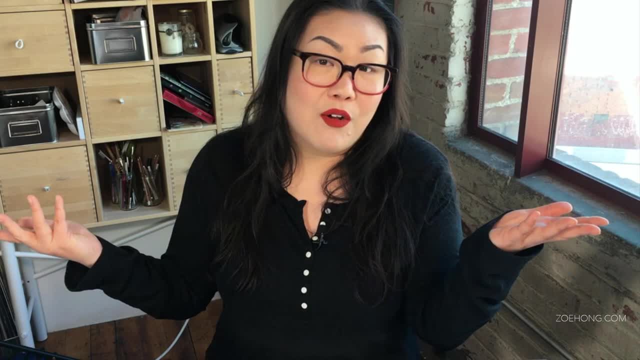 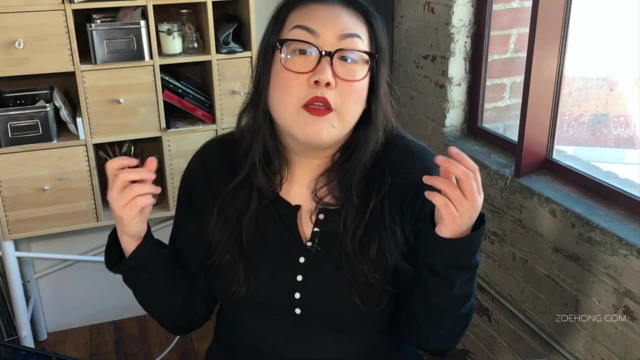 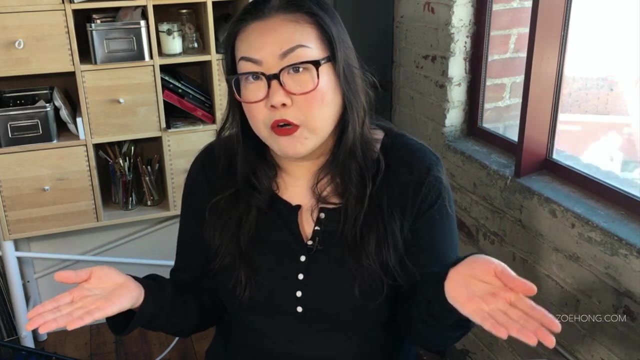 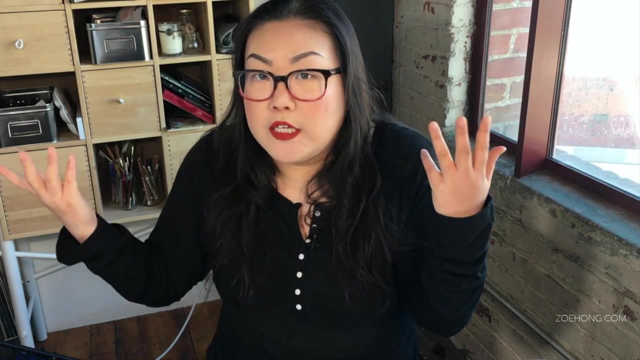 captions for my channel, So that's also helpful. Back to color theory. Okay, the first thing I want to talk about is color modes. You may have seen this in Photoshop, where you know the program asks you what color mode you want to use: CMYK or RGB or grayscale. Okay, number one. I never use grayscale because I like, even if I'm doing a black and white something, I want to be able to choose the undertones for the grays. 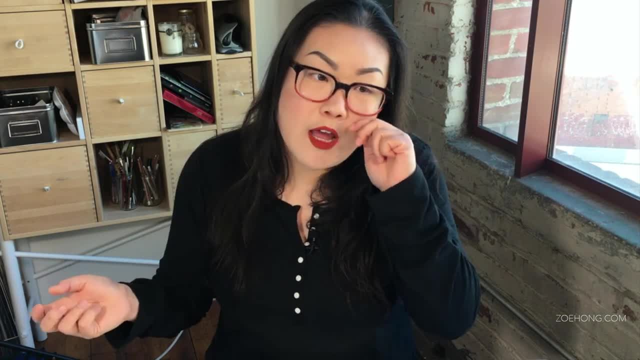 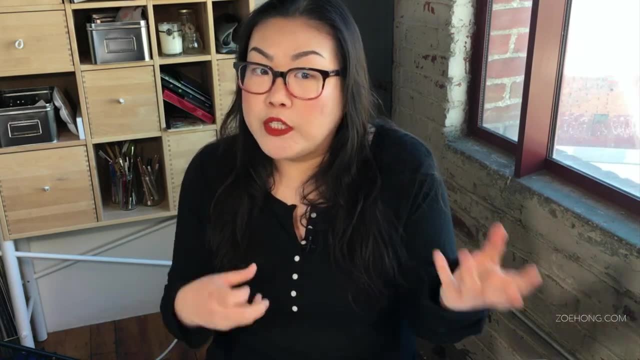 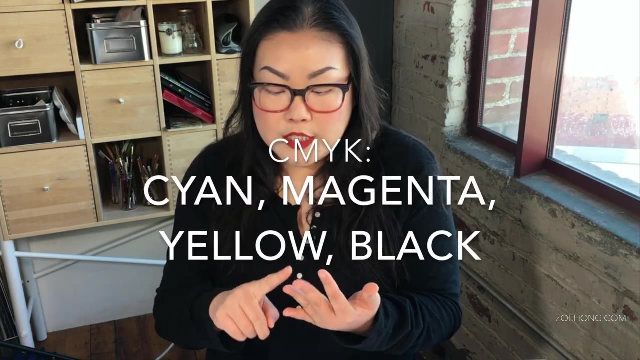 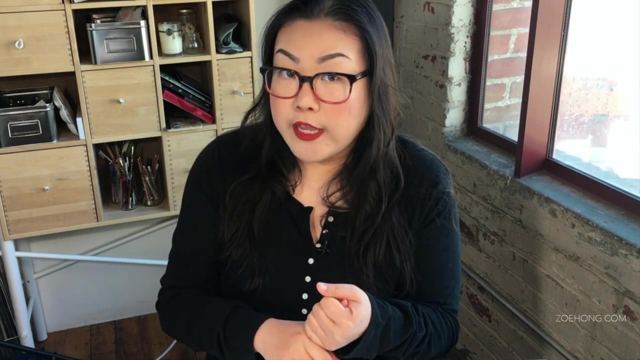 Okay, I like manipulated cool grays and warm grays and things like that, And you can't do that with a completely stripped grayscale document. Number two: CMYK versus RGB. When do you use those? What are those for? What are those letters mean? CMYK stands for cyan, magenta, yellow, black, K is for black And those are the four colors that your printer takes. Okay, if you buy color cartridges for your printer- cyan. 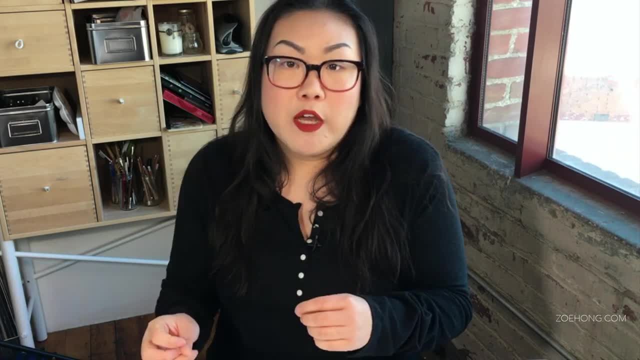 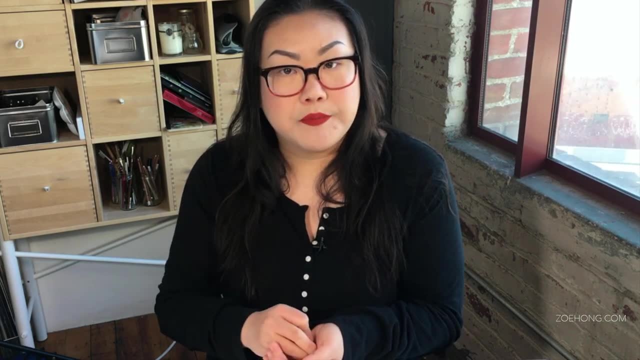 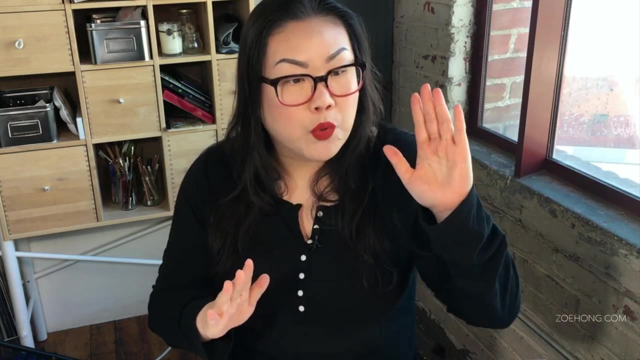 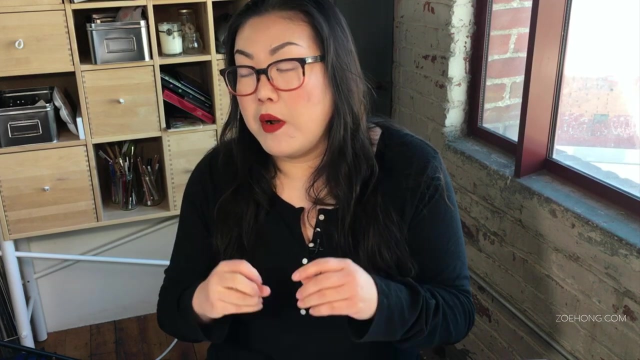 magenta, yellow and black. And CMYK color mode is for anything where it's going to be a physical, tangible thing. Okay, you are photoshopping a photo or illustrations and you're going to print them onto paper. Okay, CMYK color mode is also for mixing paints, because you're mixing pigments and put putting them on paper. So when we 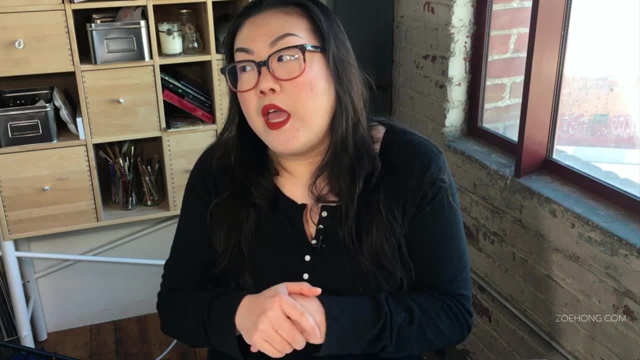 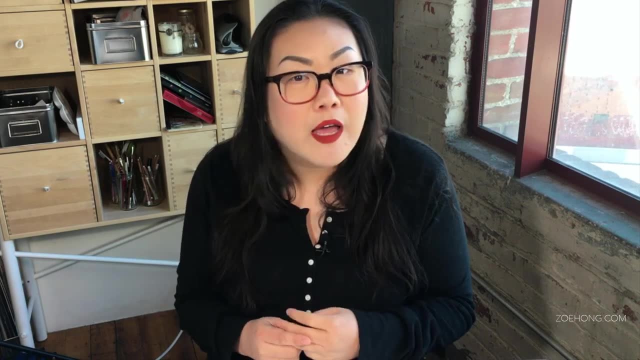 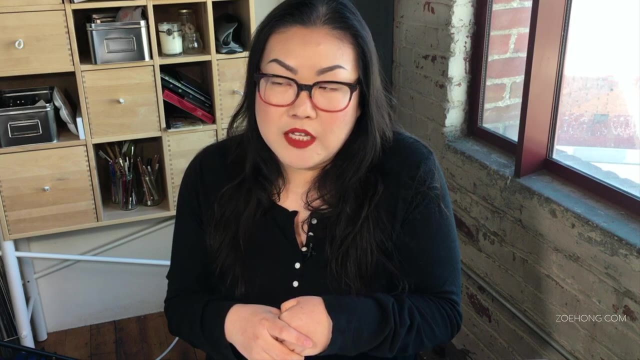 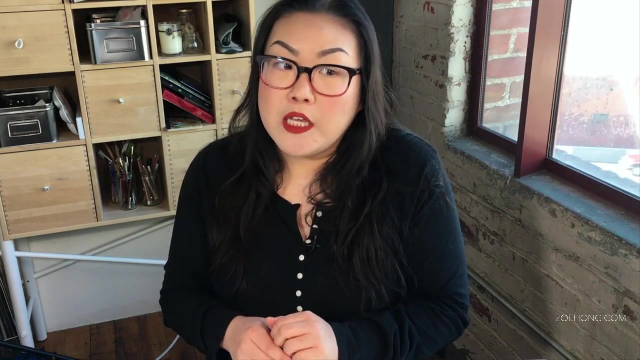 talk about paint mixing. I'm going to show you the CMYK method, And I know a lot of us grew up with the red, yellow, blue. those are primary colors And that's how you mix all the colors. Okay, that is a big fat lie, It is a conspiracy And I'm kidding. It's not a conspiracy, But it is inaccurate and inefficient. I'm gonna show you the CMYK way. in the paint mixing video, RGB is stands for red, green and blue, And that is used for 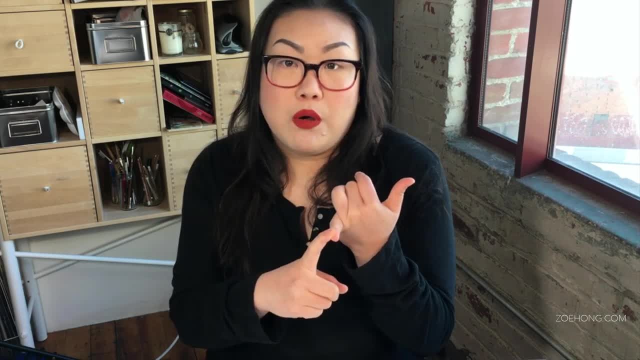 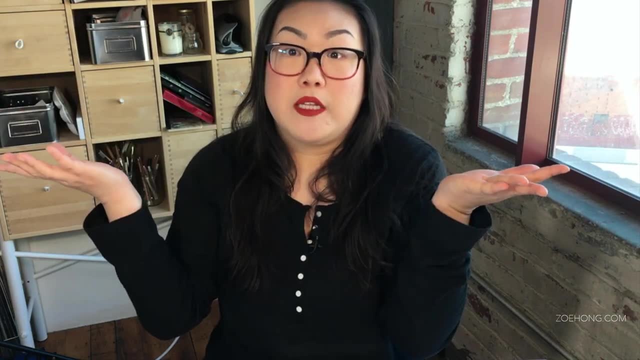 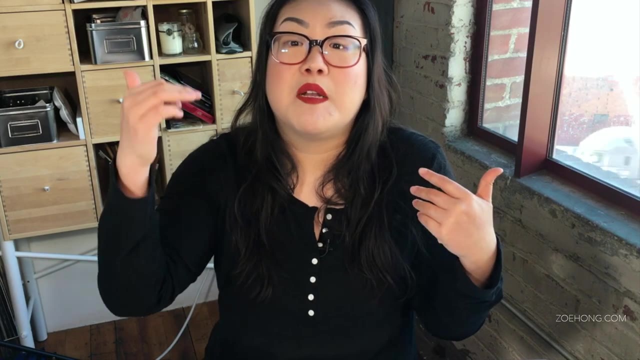 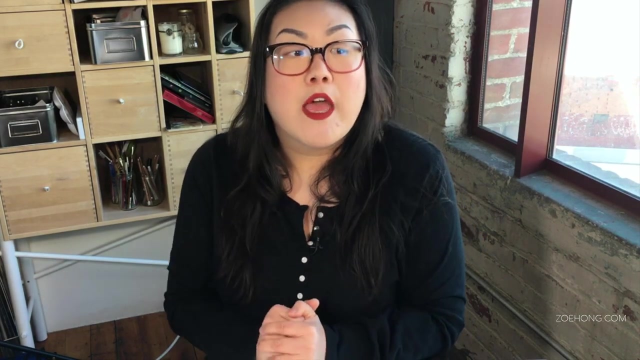 light. Okay so projections that will go, you know, from a projector and projected to a wall or screen. websites predominantly okay. so if you're designing websites, that's all I can think of. Okay so stuff that's light, so that's going to be on a screen, not stuff that's printed, you know, on a piece of paper. Next, every color is defined by these three things: VST. 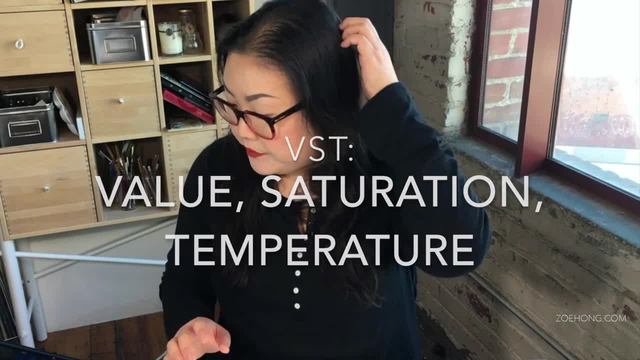 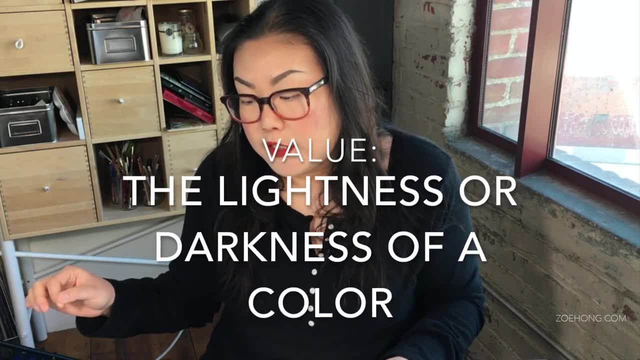 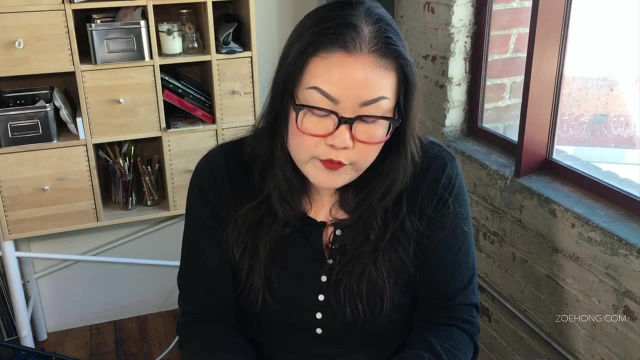 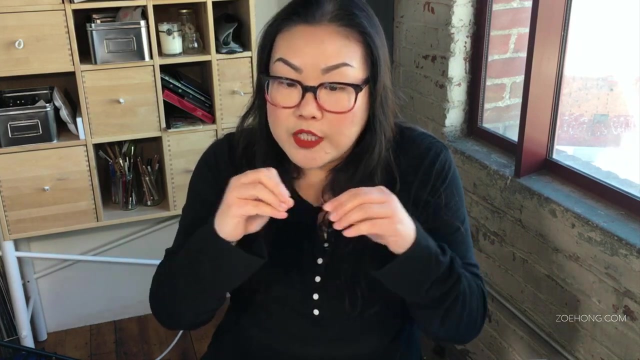 value, saturation and temperature. All right, So first, value. value means the lightness or the darkness of a color, All right, And you know, I have all of these grays, Okay, And have you heard of a gray scale or a value scale? it shows the lightness and the darkness of colors. This is the Prismacolor, warm. 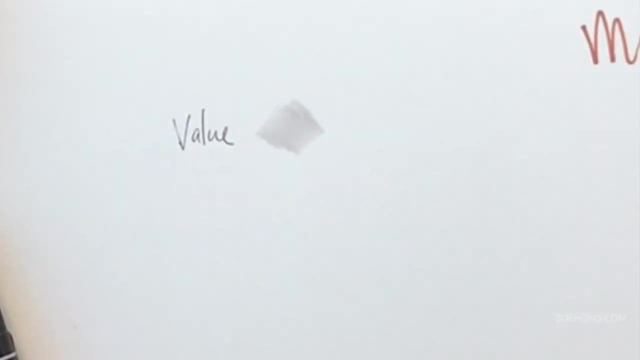 gray set. Here's the 10%, You know, here's the 20%, And it gets darker and darker. These are your values, right? And colors also have values like: why is this marker so dirty? Let's reject that because it's all dirty. I'm gonna put this away because 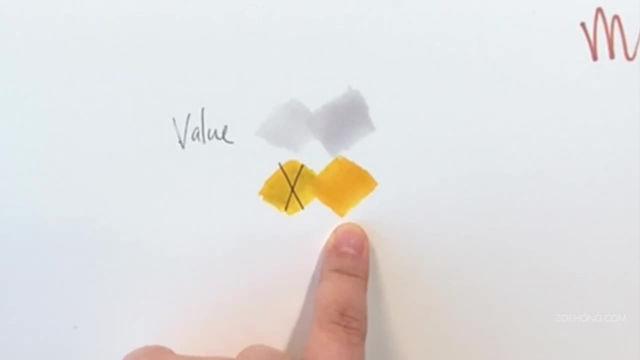 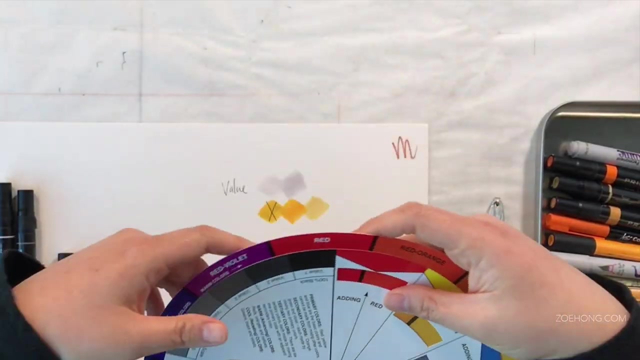 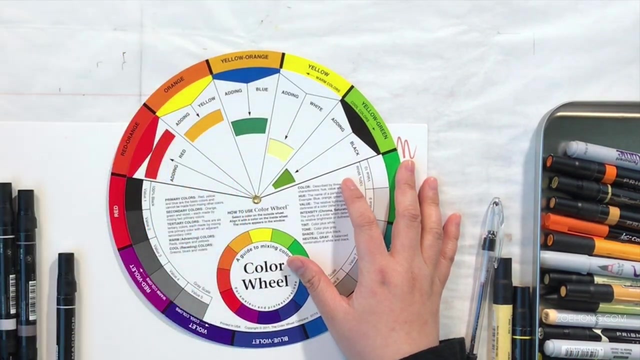 it's all dirty, All right. So we have this value, And then we have, and we have this value, right, It's much lighter. right, It's that same kind of yellow orange color, but it's much lighter. So the lightness or the darkness of a color. Here's a color wheel. I use color wheels in class to teach concepts. I will. I bought these on Amazon, this one and this one, And I'll drop the links If you are interested in. 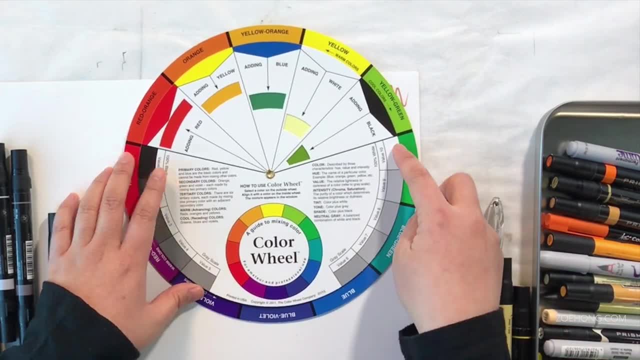 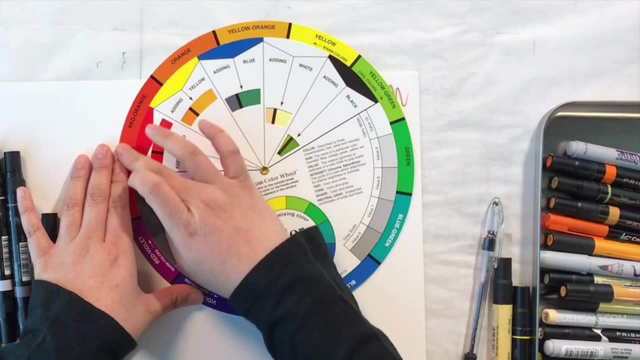 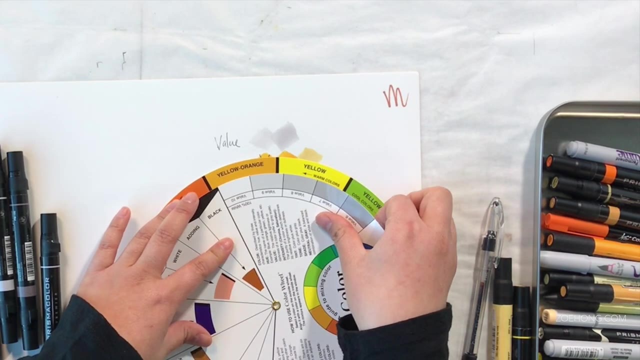 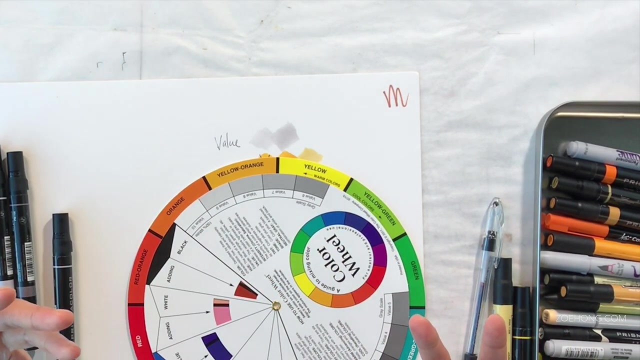 purchasing these for your own education. But you see here where they have the values: okay, 100% white to 100% black, And each color has a value, Okay. when you look at this yellow orange, okay, what value is it? Okay, which percentage gray does it match up with? So the easiest way to do that is to kind of swivel this around. 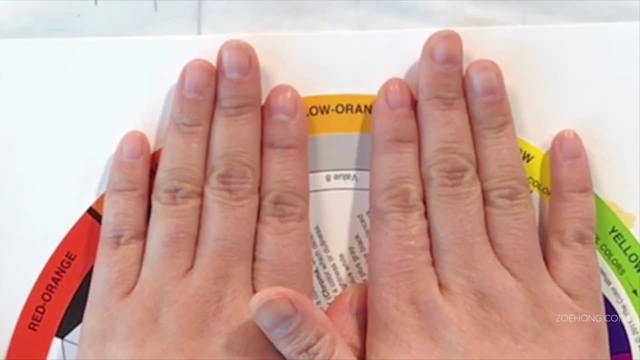 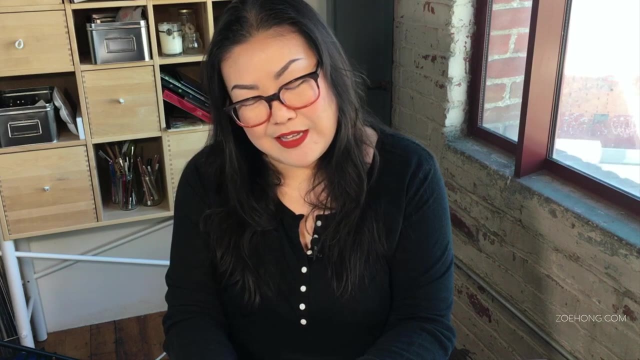 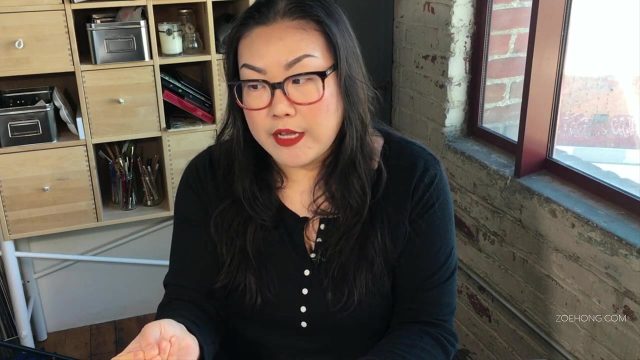 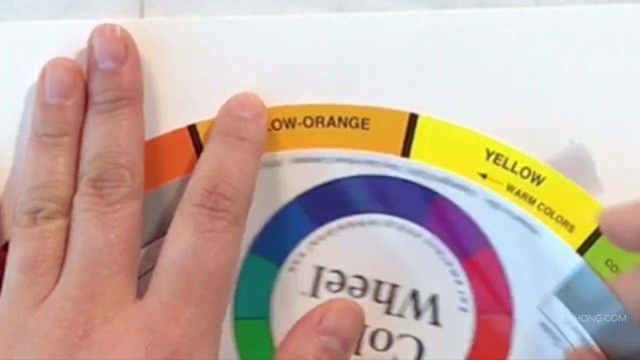 And look down and kind of squint your eyes. Okay, I love teaching this in class because all my students make ridiculous faces- Okay, And if it is a similar value or the correct value match, then this line should start blurring when you start squinting your eyes. See, these two, their values don't match at all. So no matter how much you squint them, 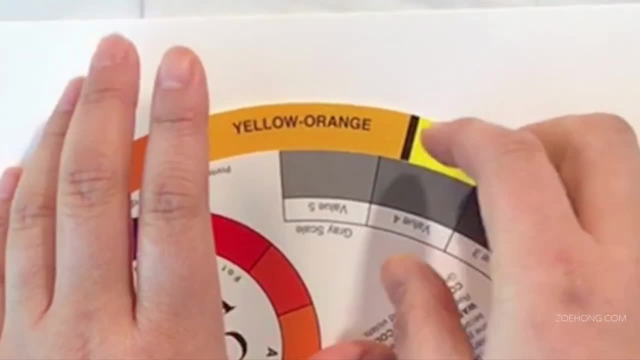 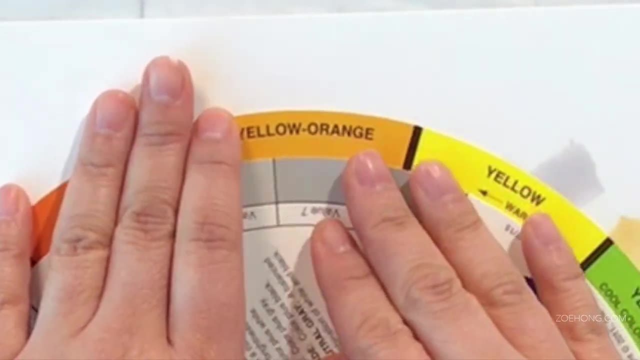 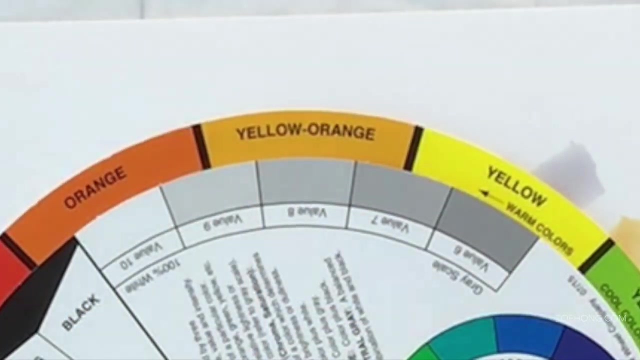 you see that separation between the yellow orange and this gray- but this one, that one- is pretty close, So the line gets a little blurrier. That one is actually a better value match And so that line gets super blurry, right. So every color has a value. It's either a light color, medium color, 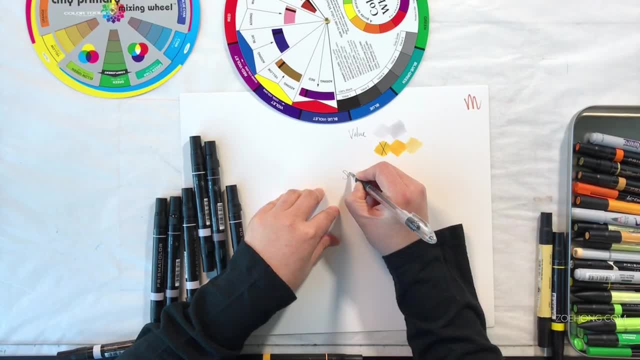 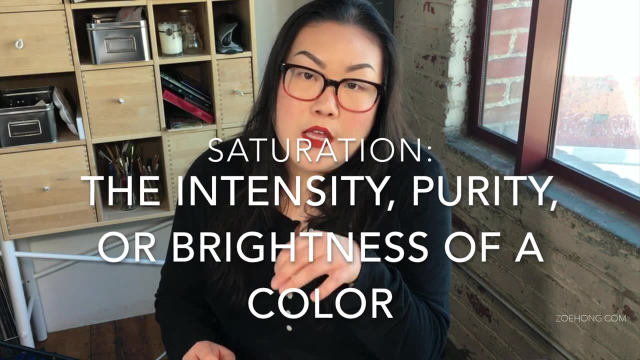 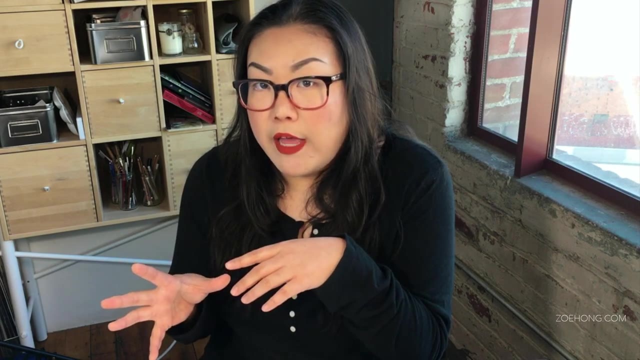 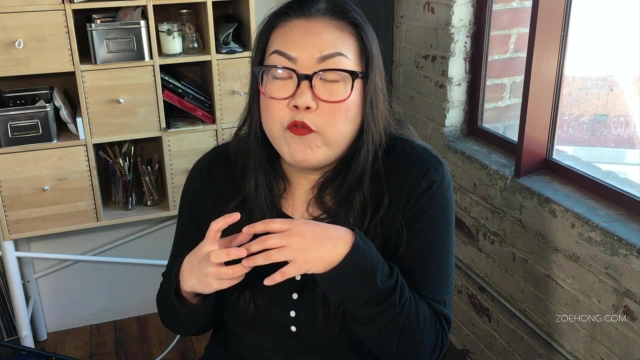 or dark color, right, And then you have saturation. Saturation is the intensity of a color, the brightness of a color, not the lightness. okay, Value is about lightness and darkness. Saturation is about how full of chroma it is, how saturated it is. 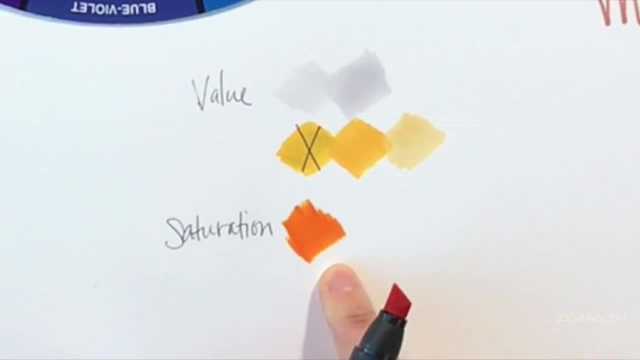 You have a color like this and it is orange. okay, You can keep adding orange to that, It's not going to get much oranger. This is goldenrod. This is a nice color I like to use for kind of dirty blonde looks when I'm illustrating, And if you add more orange to that, it'll get oranger. 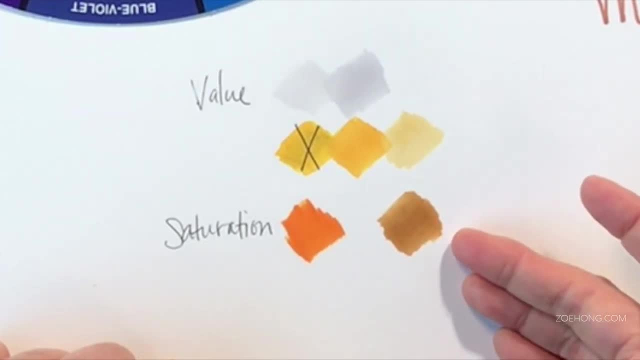 and oranger. okay, It is not very saturated. So you can add more orange and it'll get oranger. See. Okay, And you create a new color. You just add orange to orange, it's just going to stay orange, right? So saturation, brightness, purity, intensity, not lightness, And then 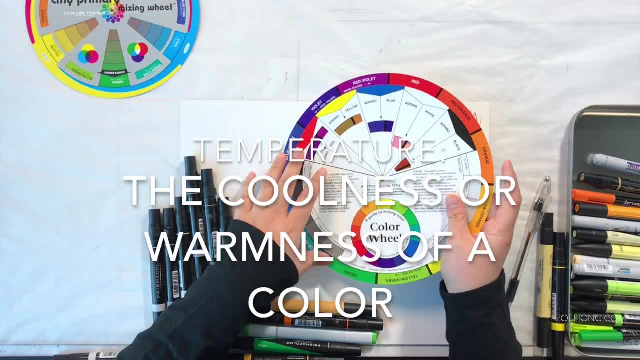 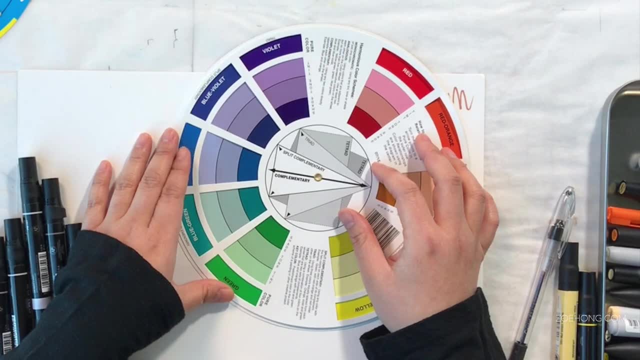 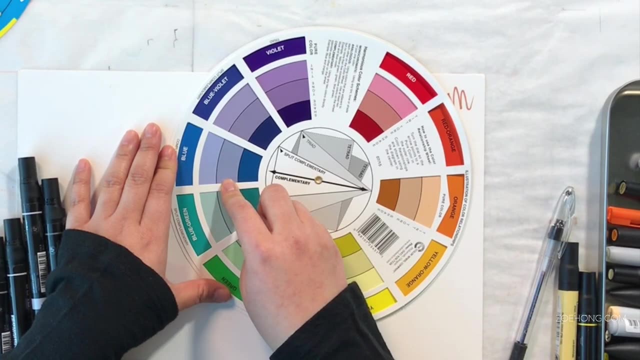 temperature. okay, So we have cool colors and we have warm colors. For those of you following along at home, do you know what the coolest color is? It's the color that you can use to color. is It's blue? okay, Blue is the coolest color because there's nothing you can add to blue. 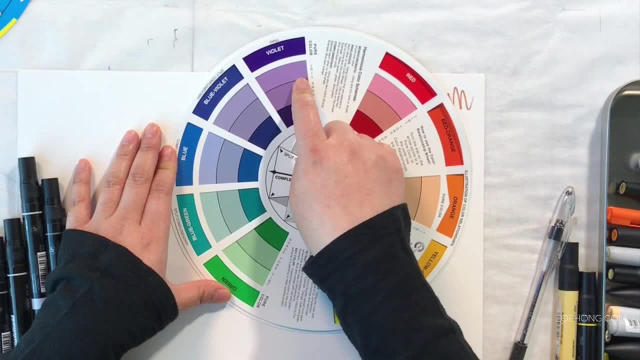 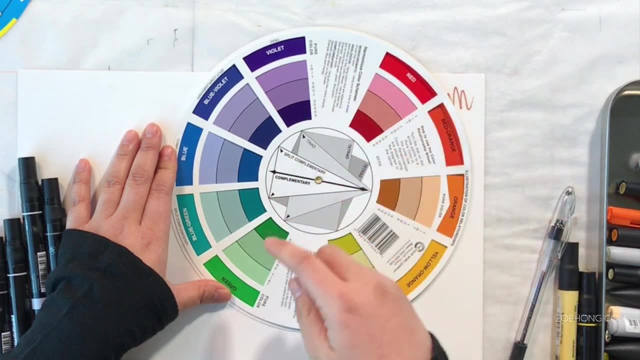 that will make it cooler. okay, If you have violet, you can add blue to it. it'll be cooler. If you add more red to it, it'll become warmer. okay, Green, you can add blue to it and make it. 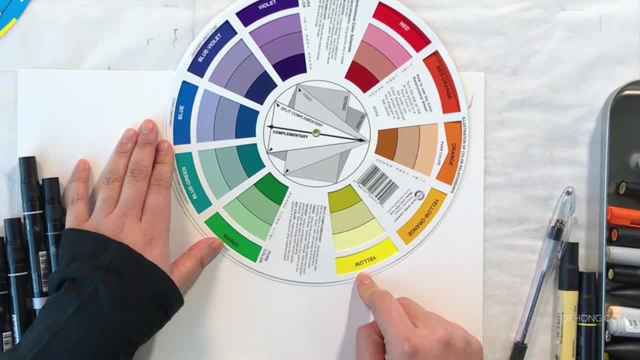 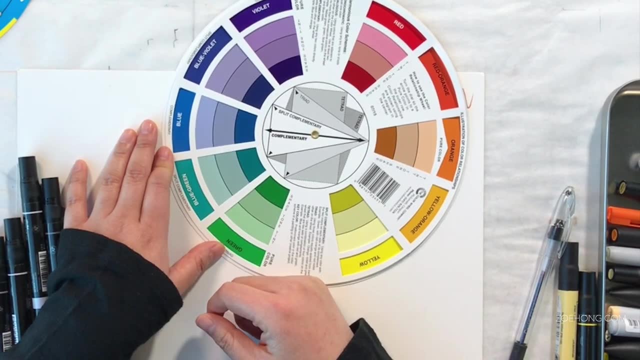 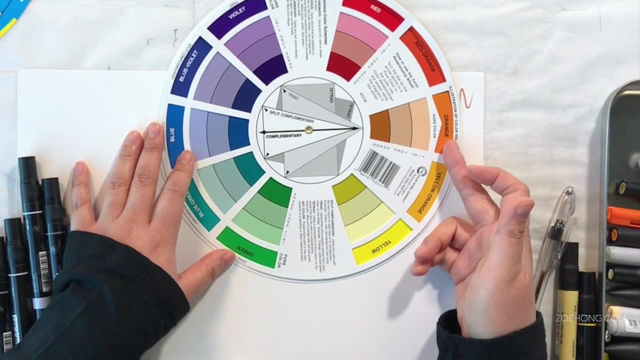 cooler. If you add its next neighbor, yellow, to it, it'll become warmer. And then you can add green to it, it'll be a warmer green. See, that's a blue is the coolest color And the warmest color is orange. okay, And again you can have a cool red. you know cool reds, warm reds, you know. 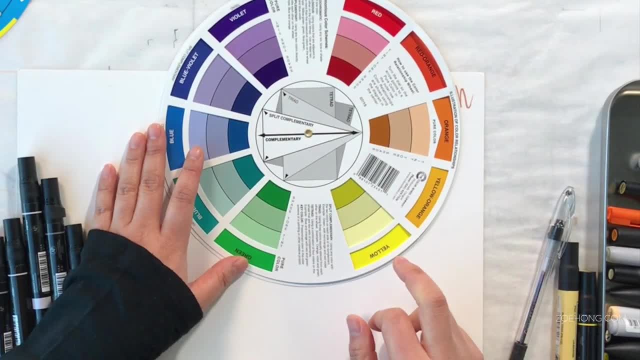 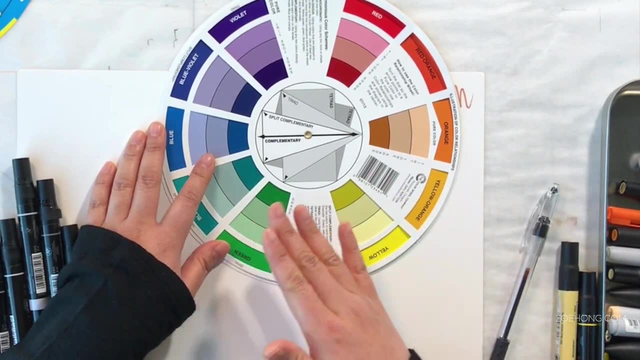 any. anyone who likes wearing lipstick knows what those mean. okay, And you can have a warm goldish yellow or a cool greenish yellow, But orange if you, if you start adding things to it, you kind of get duller oranges, desaturated oranges, but you don't. 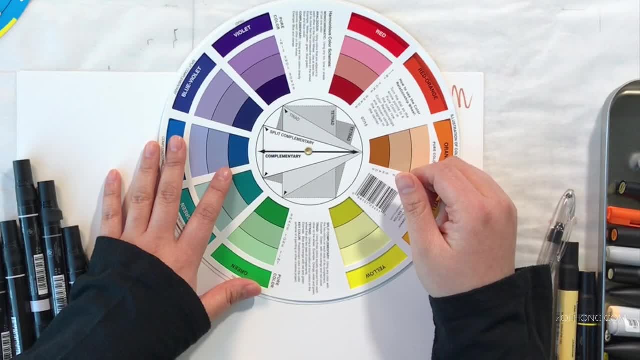 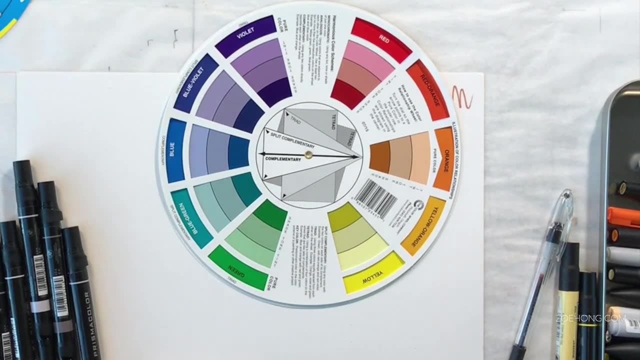 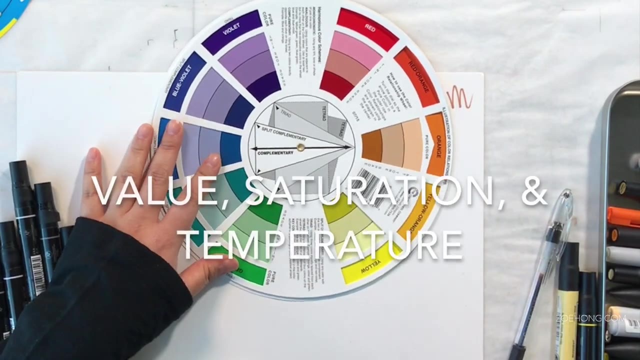 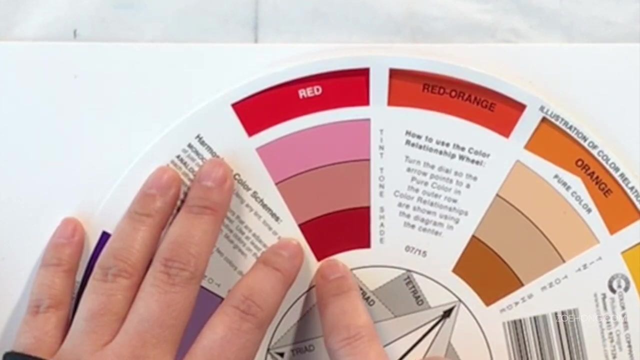 you don't really get a cool orange or a warm blue, you know. So those are your two extremes, And so any color in the world can be figured out, defined, however identified by these three things. okay, Take this red, for example. okay, It is a medium. 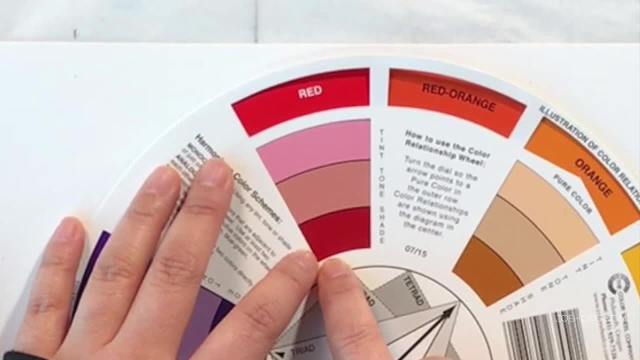 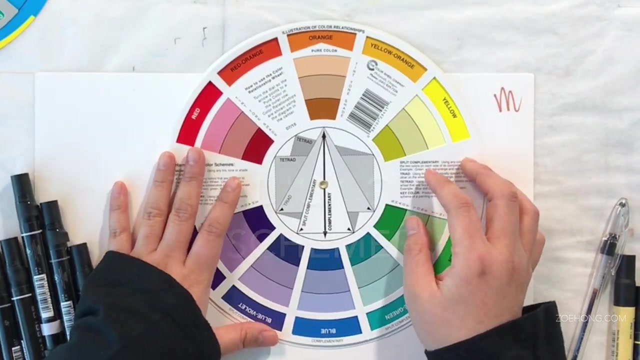 dark value. It is quite saturated, a little bit desaturated. okay, It's still pretty intense. It's not very dull at all And it's warm temperature. okay, It's red, it's pretty warm. So let's talk about color schemes. First, let's talk about triadic color schemes. These are: 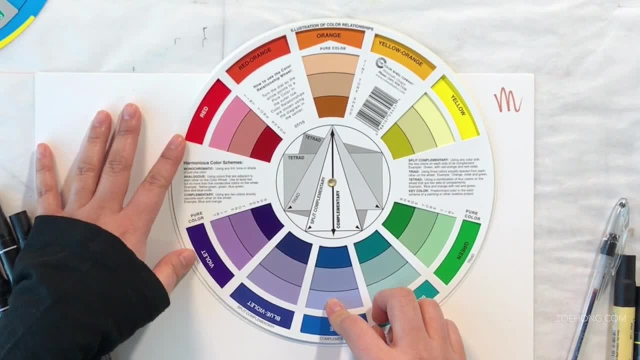 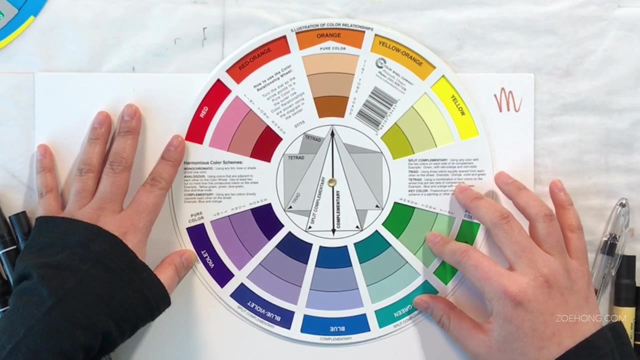 three colors And each color is separated, the equal amounts in between each color. So red, yellow and blue, Three colors in between red and blue, three colors in between red and yellow and three colors in between yellow and blue, Equidistant from each other. okay, Red, yellow, blue, those are your primary colors. 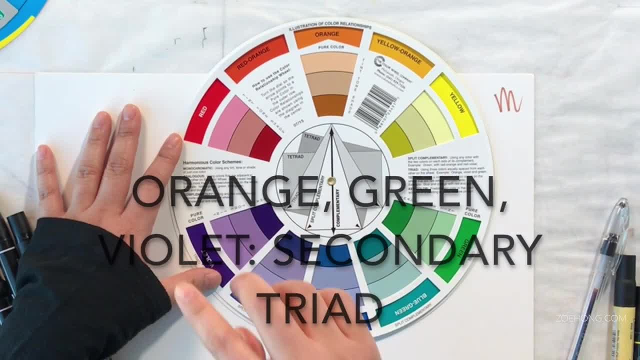 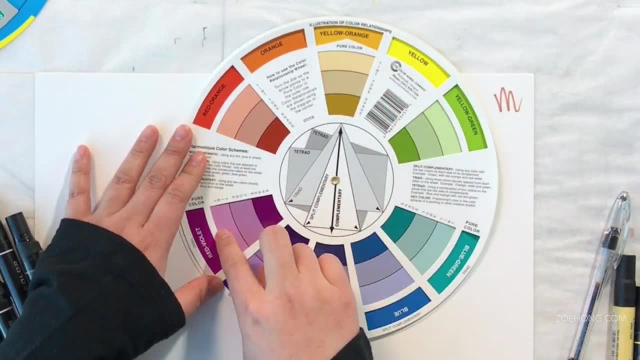 Orange, green and violet are your secondary colors. And then you have two tertiary triads: One of them is yellow, orange, red, violet and blue green, And the other is yellow, green, red orange. 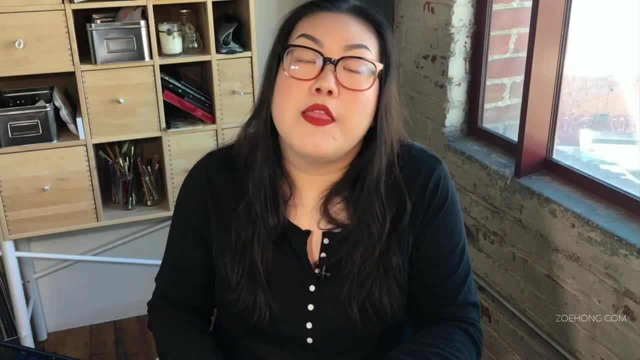 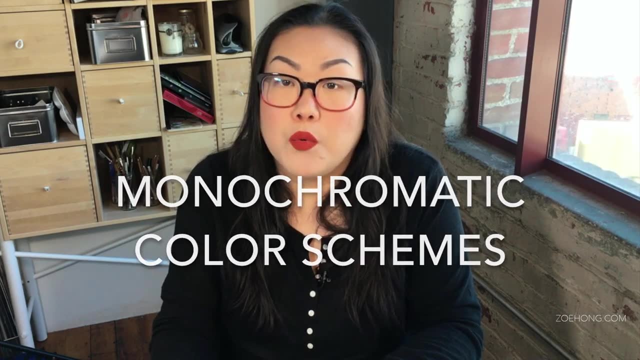 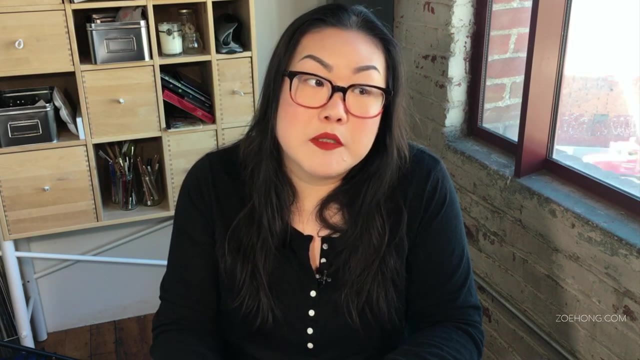 and blue, violet. These are your triadic color schemes. And then you have monochromatic color schemes. Monochromatic it means one color, Mono, equal, one chroma, meaning color monochromatic. And you know people like monochromatic color schemes because, uh, they're easy. 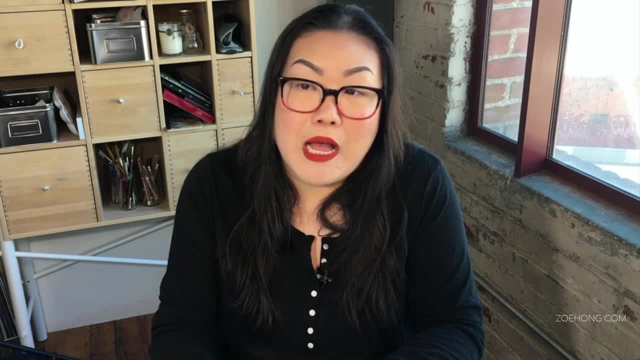 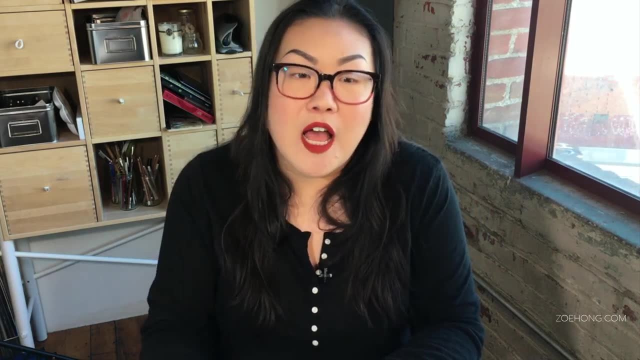 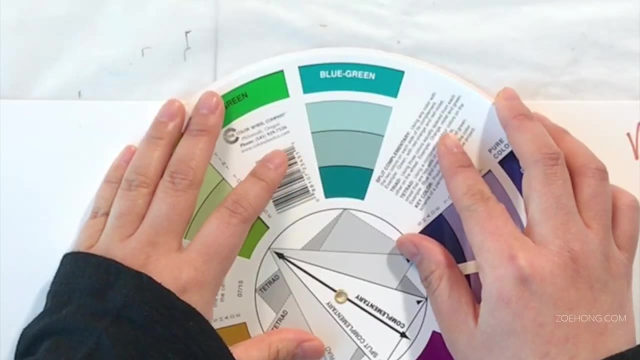 like, if everything is based off of one color, then it's easy to match and coordinate. You don't have to think about matching and what goes with what or whatever right, And it has. it looks very cohesive. Now, when I say monochromatic, I'm not saying that everything is this blue-green. 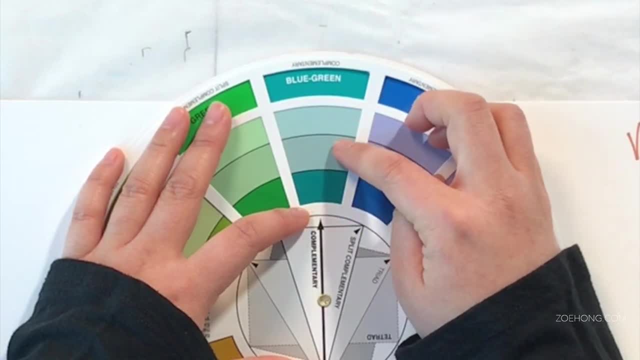 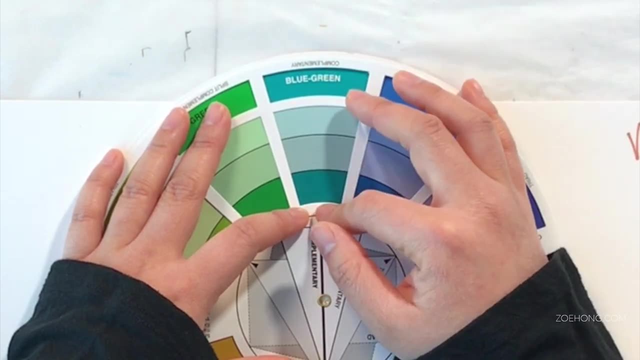 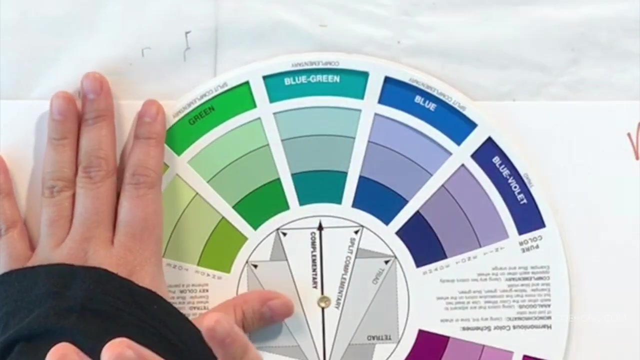 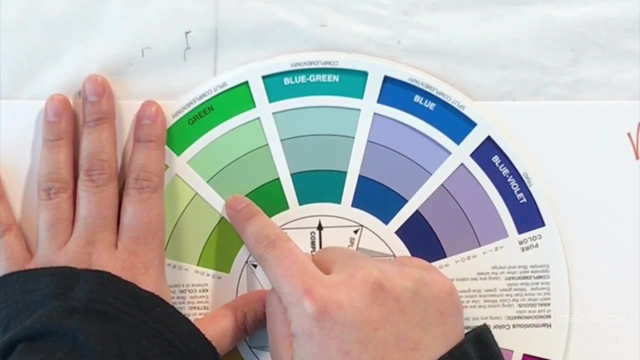 You can also include tints, shades and tones of the blue-green, okay, So you can have variety, different shades of the blue-green, and still be monochromatic- okay. What you can't do is start changing temperature. okay. Changing temperature means moving around the wheel. You can't get. 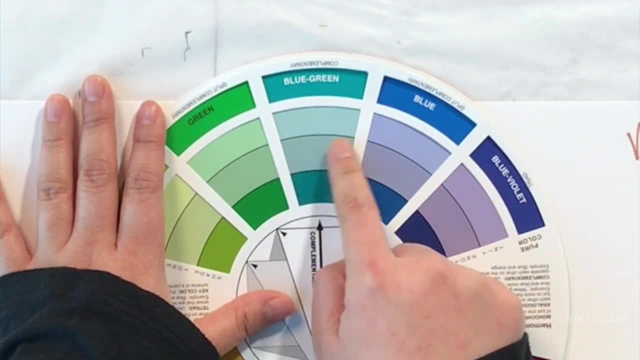 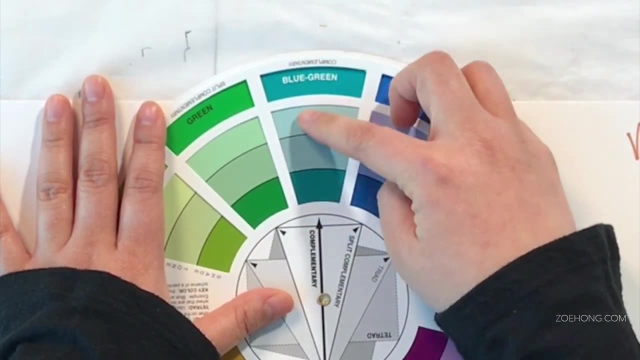 warmer, okay, That's no longer monochromatic. And you can't get any cooler because, again, that's no longer monochromatic, It's something else. We'll get to that in a second. But you could stick to the same blue-green tints and shades and tones in here. 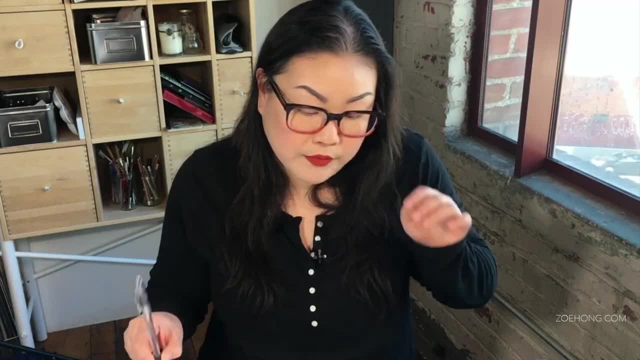 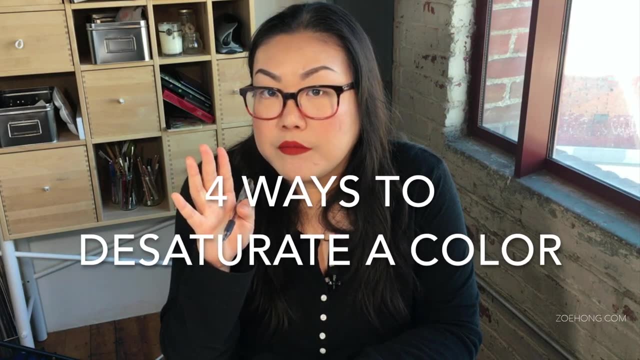 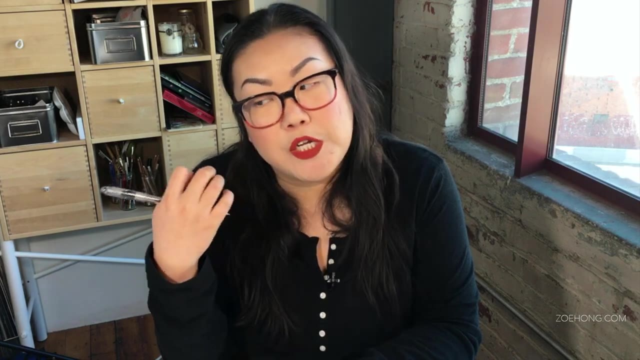 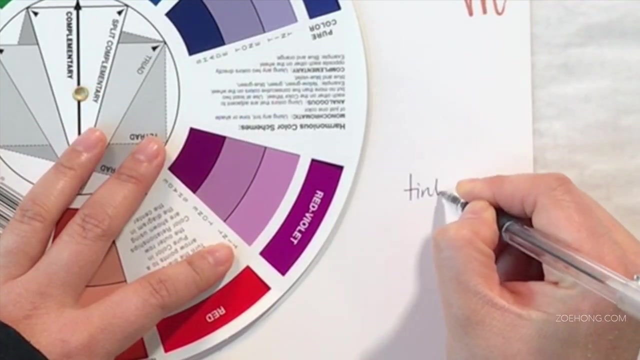 Okay. so, speaking of tints and shades and tones, let me tell you what those are. okay, So there are four ways to desaturate a color: creating softer tones, more muted tones, duller effects, creating neutrals, right, So four ways to desaturate a color. So, number one: we have tints. 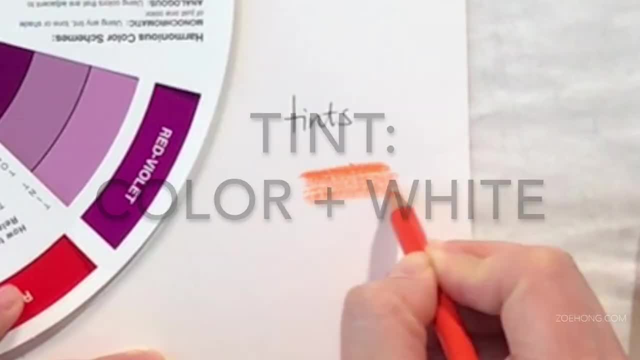 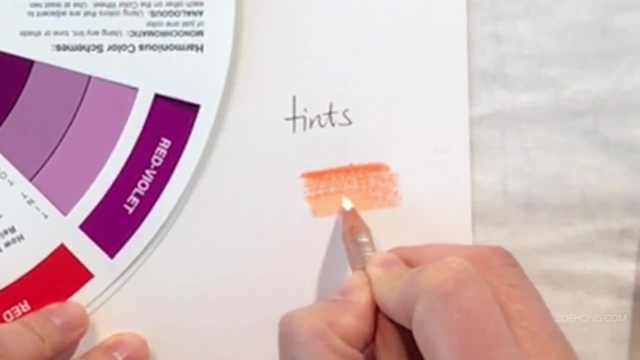 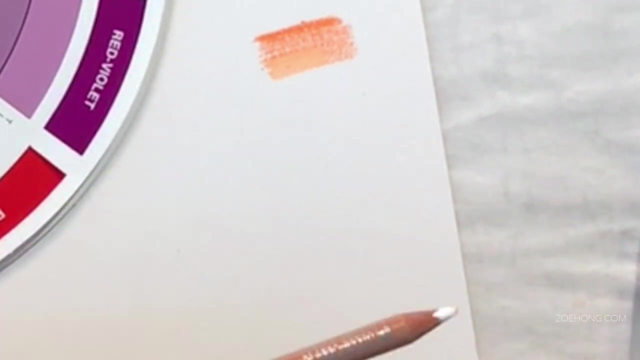 and you can create tints by adding white. We have some tints, We have some orange and you can add some white and you can make a lighter orange. okay, It's still got that pure orange look, but it's lighter. and now I want a creamsicle. 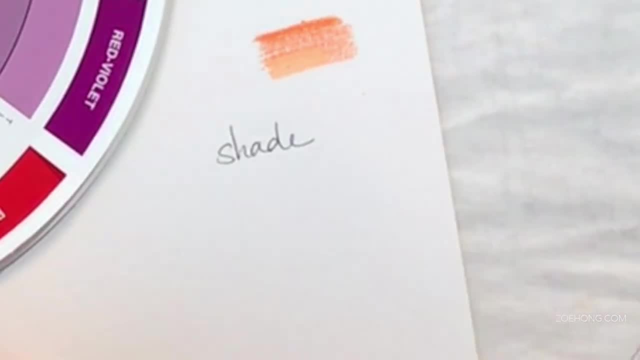 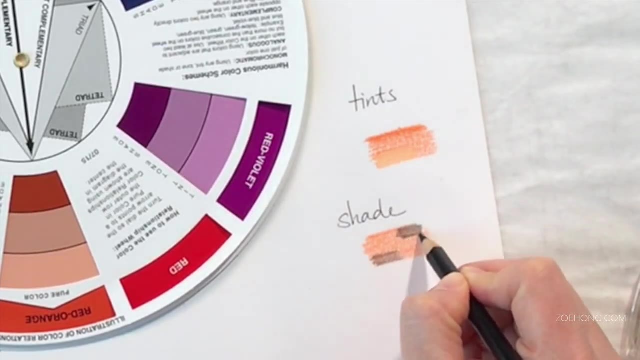 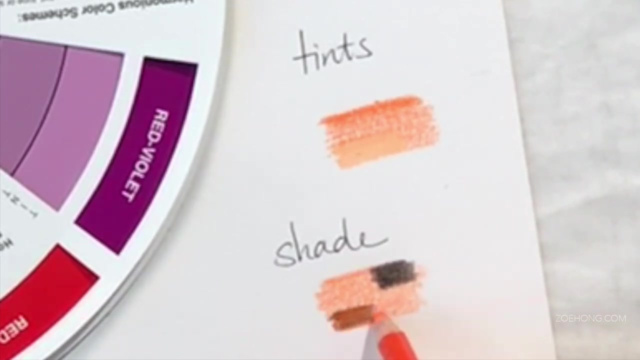 Now the second way is to create a shade, and you create a shade by adding black, And there are so many varieties of tints and shades, depending on how much white and how much black you add. Here's a shade of orange, but it's mostly orange, so it's just a little bit darker. 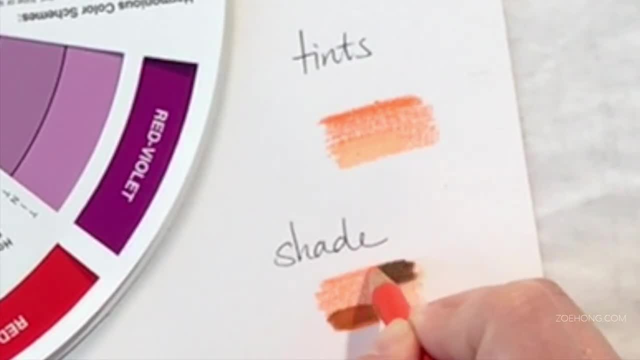 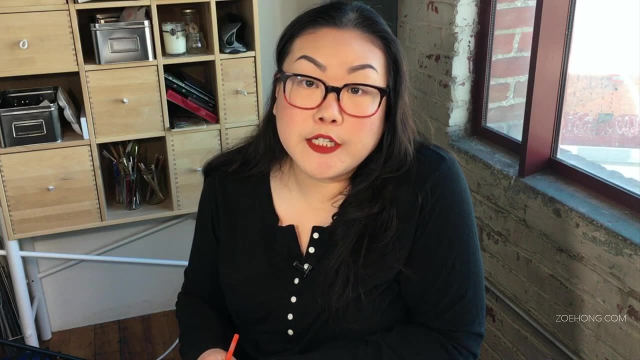 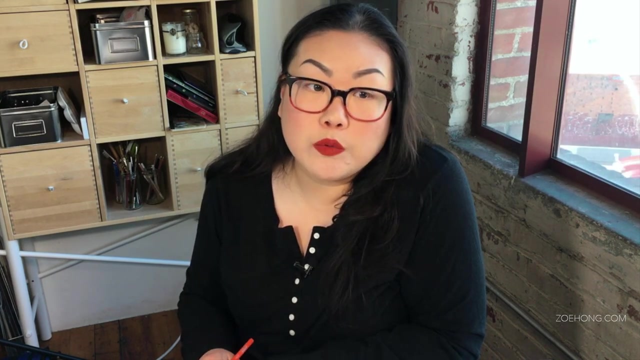 This has a lot of black, so it's a very, very dark orange. And then you have tones. Tones are created by adding grays and again, there's so many different tones you can create by choosing different grays, You know. 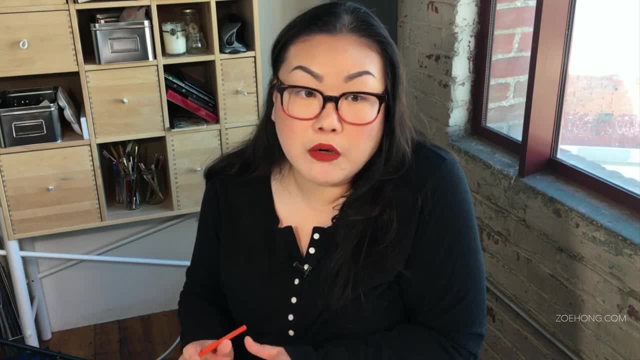 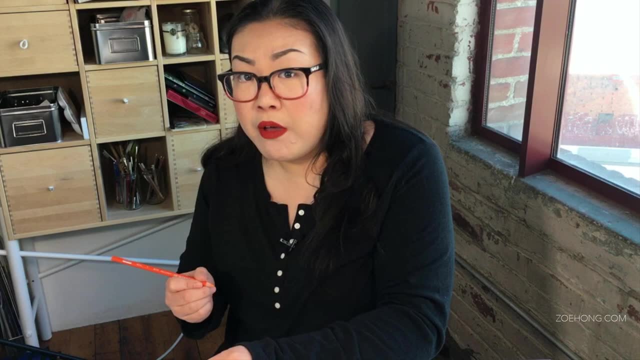 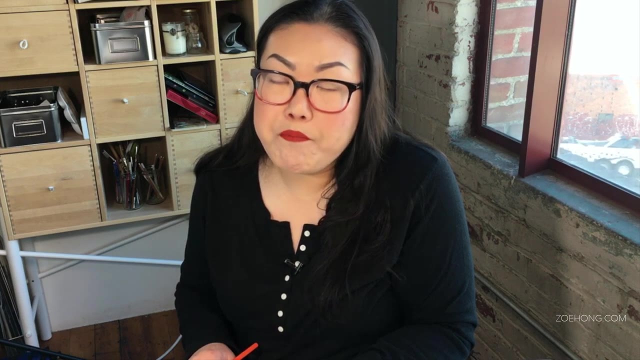 70% gray, 30% gray. you know light grays versus dark grays and also by how much you know orange you have in there compared to how much gray you have in there. Now, when you create tones, what you want to do is to mix the correct gray with your color. okay, 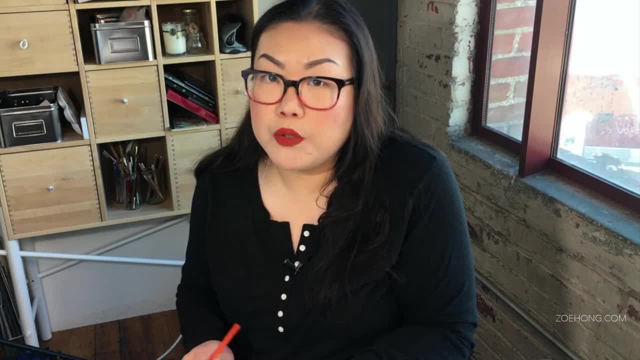 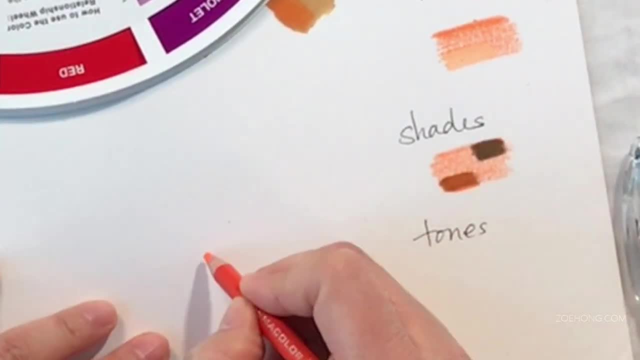 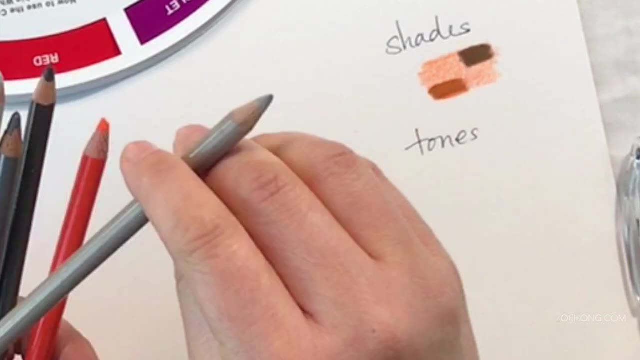 You want to pick the gray that has the same undertone as your original color so that you can get a nice tone. With warm colors like orange, yellow, orange red, orange red, I like to use warm grays. okay, Here's a 50% warm gray. 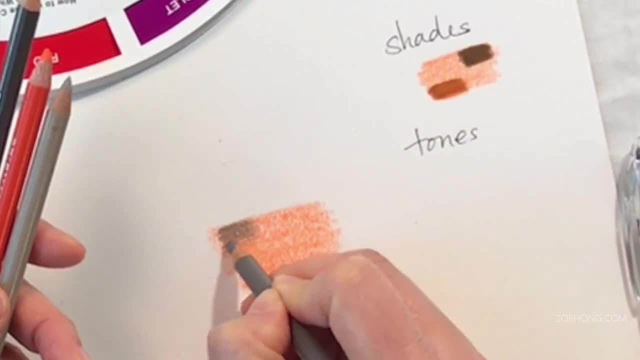 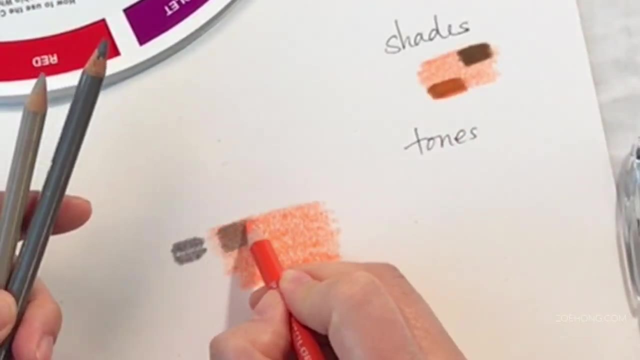 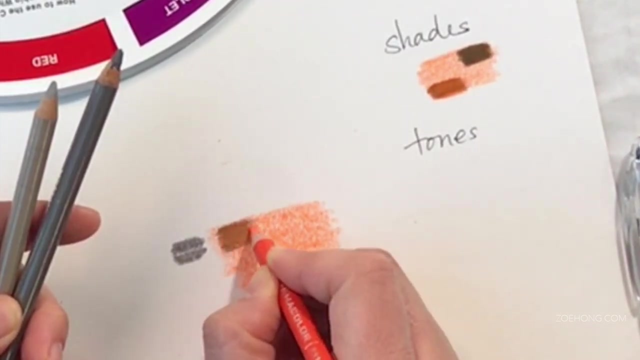 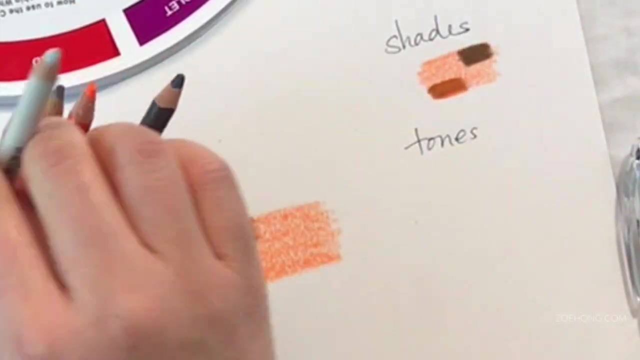 And you know I can add a lot and make it a lot more gray. I mean, here's what the gray looks like by itself And mixing with this orange, you know it starts looking a little bit brownish. Or you could do a really light gray, warm gray. 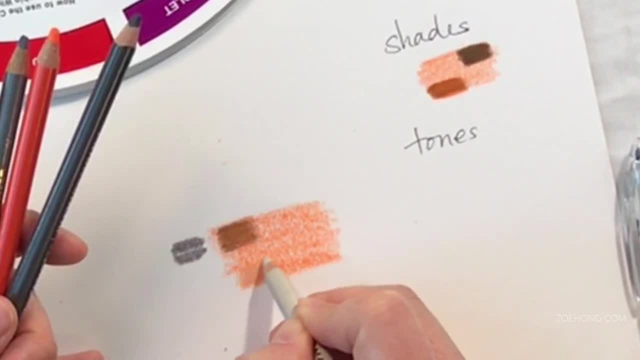 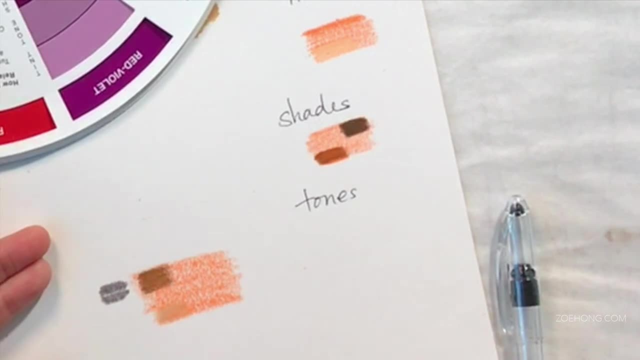 Here's a 10% And you're almost creating a tint, but it's. you see that and that. How this one? you really see a light orange and this is a dulled down Light orange. okay, It's not as bright orange as the tint. 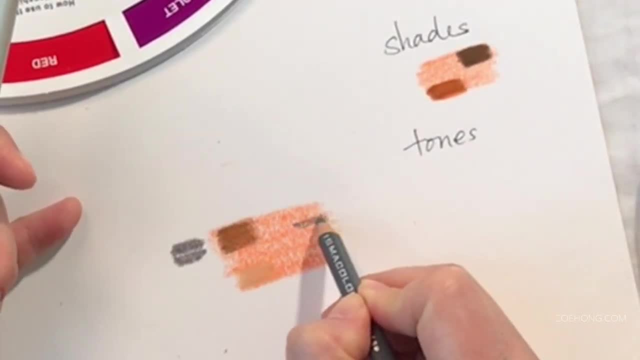 If you have something like this and you start adding a cool gray, okay, The undertones are not the same, So it's like adding gray plus a little bit of blue to it, And so you're getting a completely different color And you're making it a little bit muddier instead of creating true neutrals. 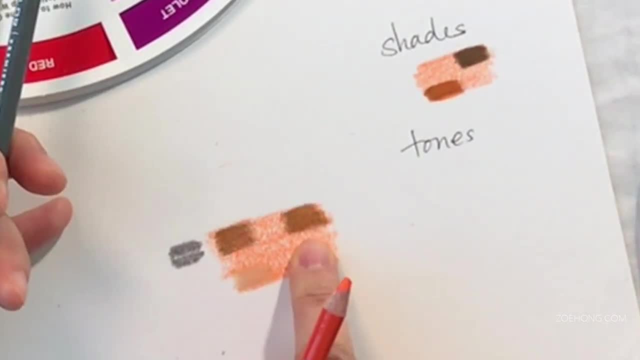 Okay, You know it's starting to look a little bit greenish. You see how it looks greener there because you're adding a little bit of that blue. So instead of it being darker, orange, toned down orange, you know, a little bit brownier with those warm undertones, it's starting to look greenish. 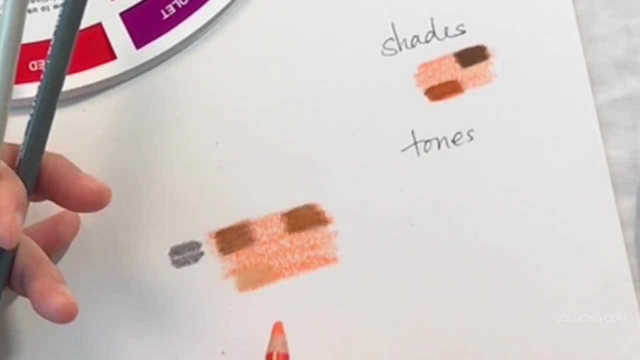 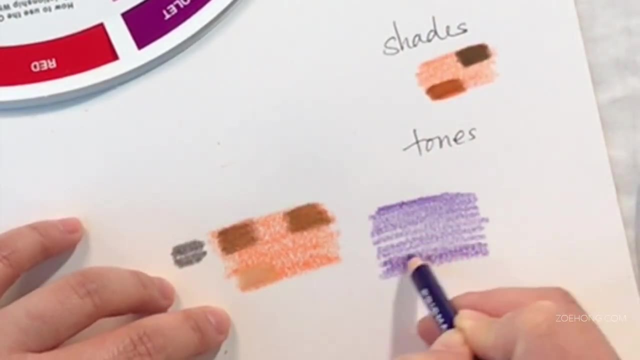 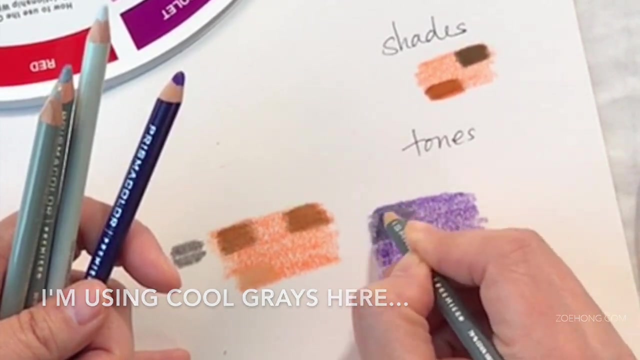 And so I mean you have to decide if that's what you want, Okay. So keep the undertones of your grays in mind. So with colors like blue and violet, you can create duller, less intense violets like that, okay. 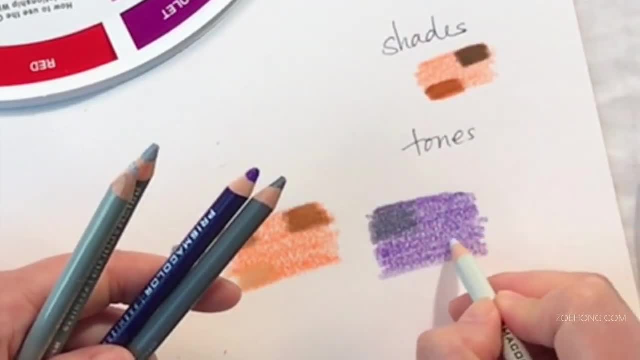 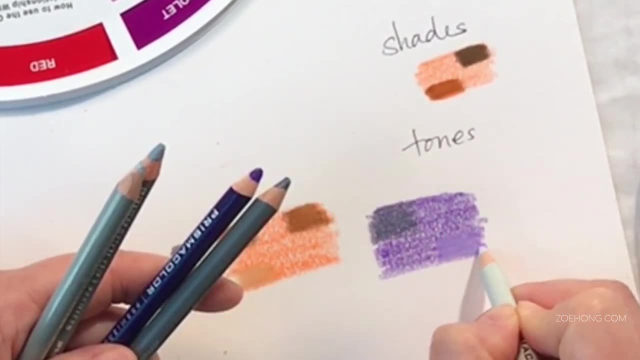 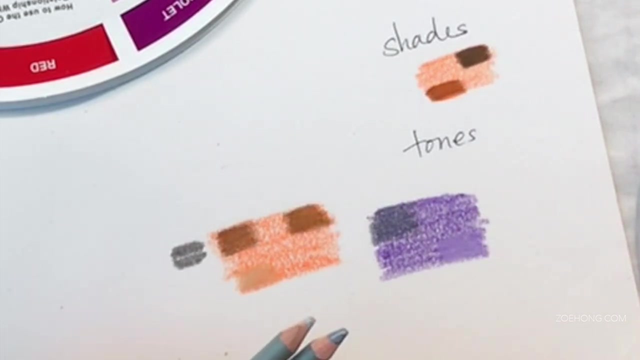 These have the same undertones so they marry well together. Or you can create duller and also lighter purples. So what do you want to do? if you want a duller purple, but the same value? You use the same value gray as the value of the violet. you're mixing it with. 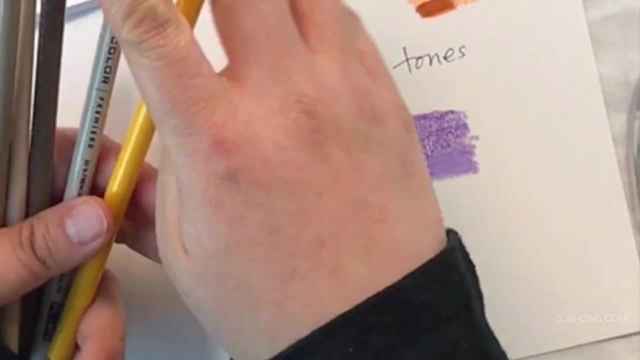 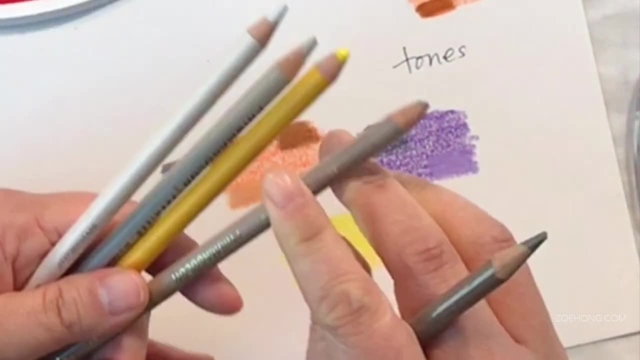 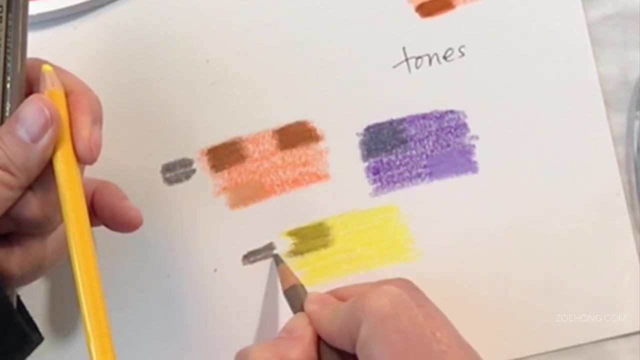 With yellows and greens. I like to use French gray And here's a dark 70% French gray And I'm creating kind of a dark khaki color. That's kind of a really cool neutral in there. That's what the French gray looks like by itself, just warmed up a lot by the yellow. 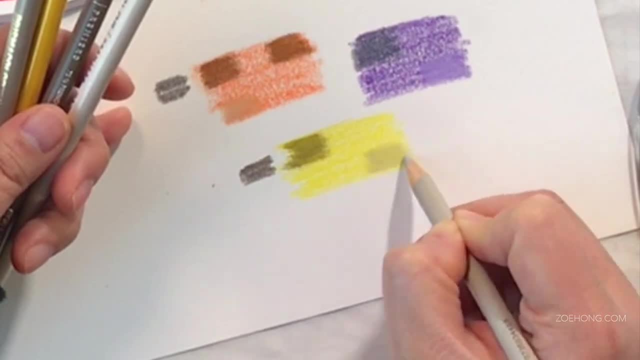 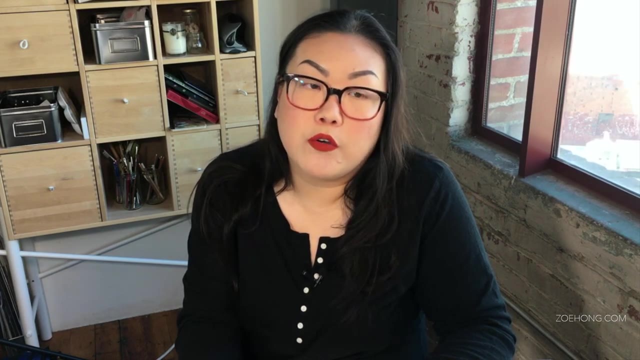 Here's one where the value is a little bit closer, not quite as light as the yellow, but the value is closer. We've done triadic, we've done monochromatic. The next I want to go over is analogous, Analogous, which is related to that word: analogy. 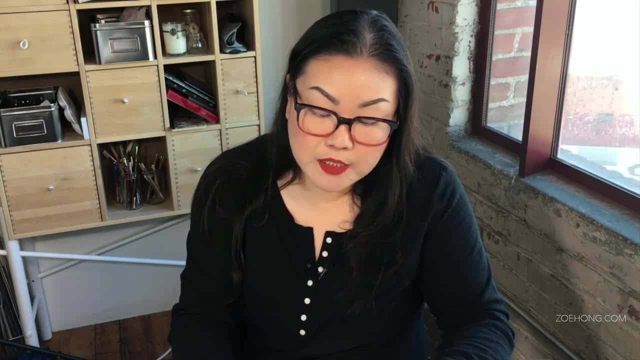 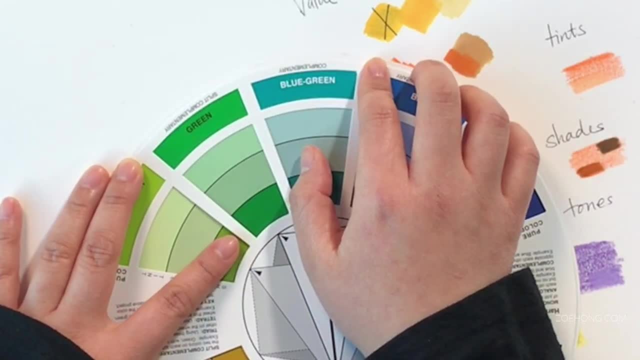 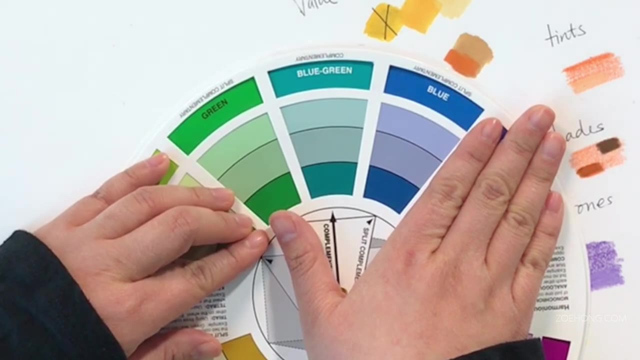 So analogous color schemes are color schemes that include like colors. We're talking about neighbors on the color wheel, So green, blue, green and blue would be an analogous color scheme. So it's similar to monochromatic in that it creates a cohesiveness. 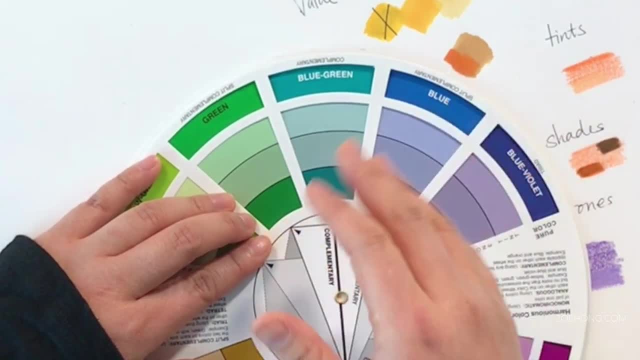 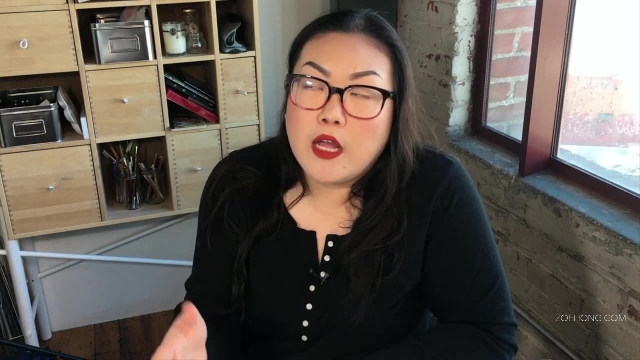 because of all these similar colors, But there's more visual interest, a little bit more variety. The question I get in class a lot is the color wheel. they're all neighbors, They're all next to each other, So how many colors is too many to be in an analogous color scheme? 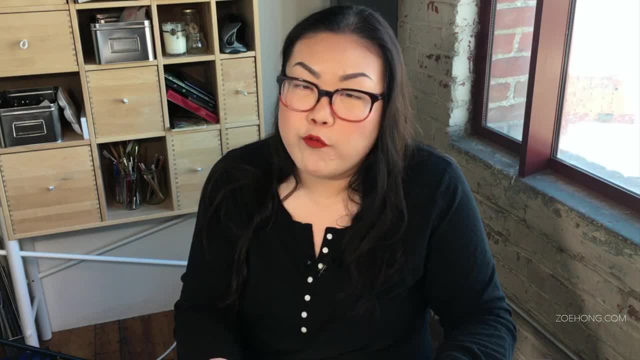 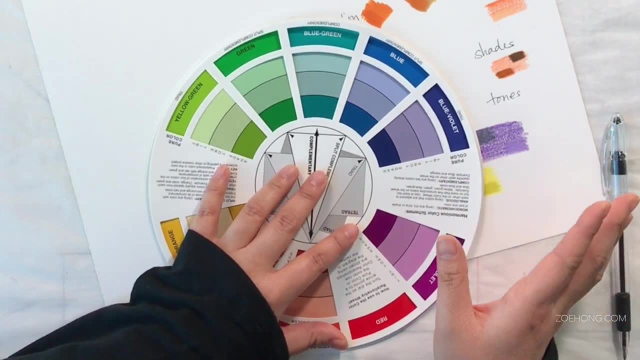 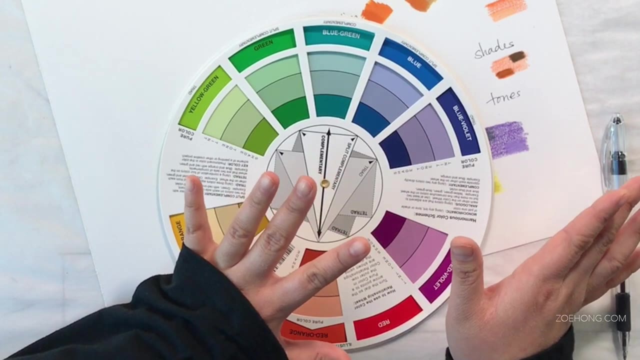 And there's no hard and fast rule. No one says only 4.2 colors. It's kind of a judgment call, depending on the scenario, Like one of the guidelines I use is no more than five colors. If you have half the wheel, that's a lot. 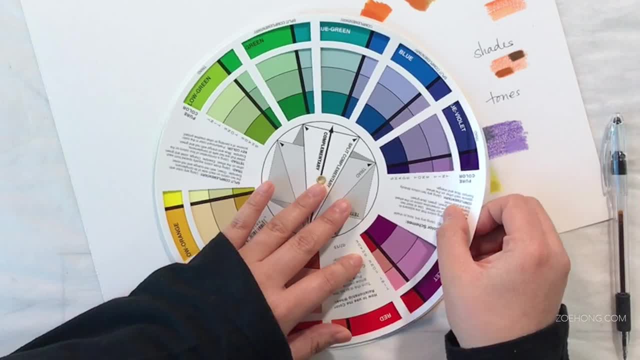 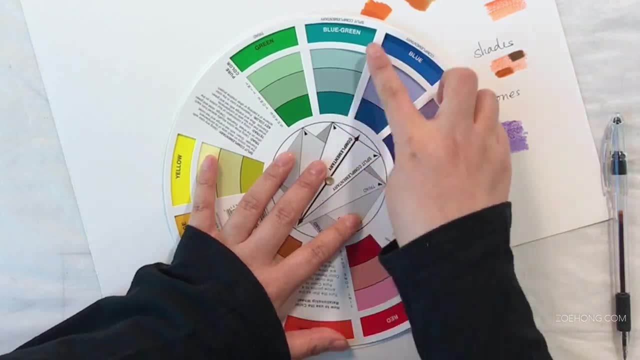 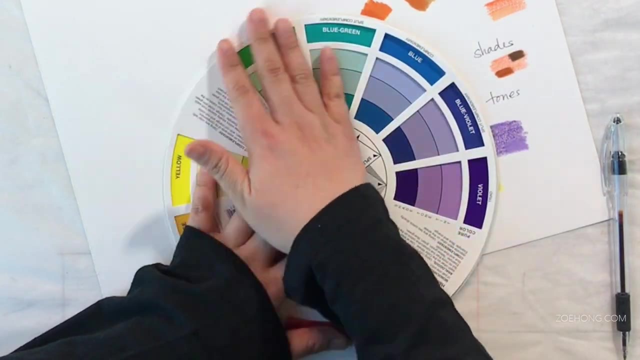 That's not really a color scheme, That's just a bunch of colors. I like to include only one primary color, So this one. it has just the blue and it has a bunch of colors, So there's five of them, but they all look cohesive together. 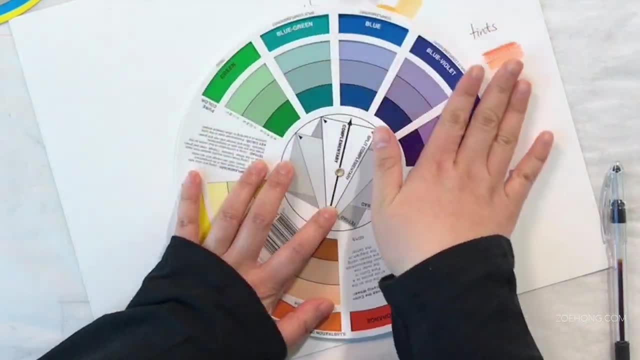 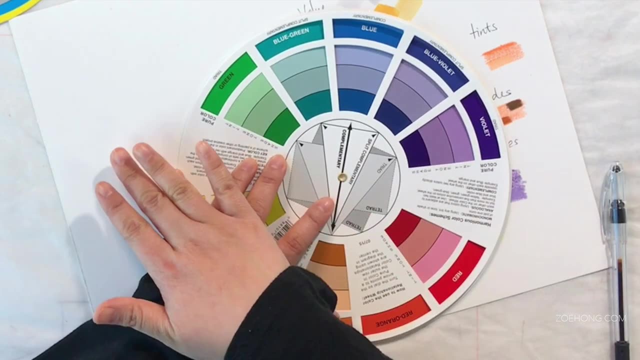 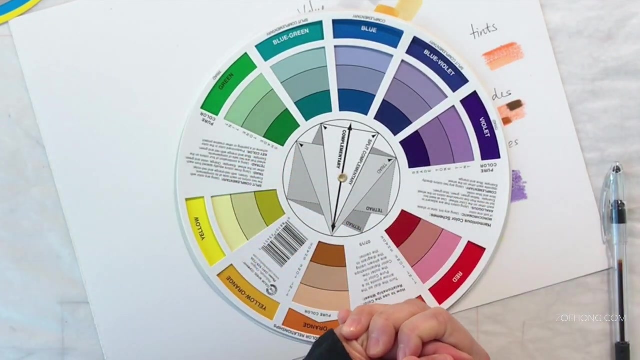 When I'm figuring this out, I like all the analogous colors to have the same undertone. This looks analogous to me because everything has a blue undertone. There's a blue in every color, And so it looks cohesive and they look like they belong together. 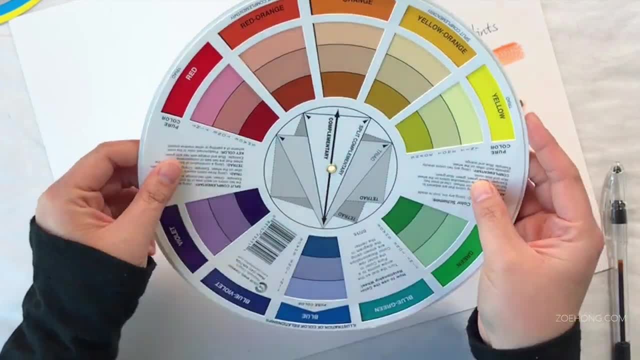 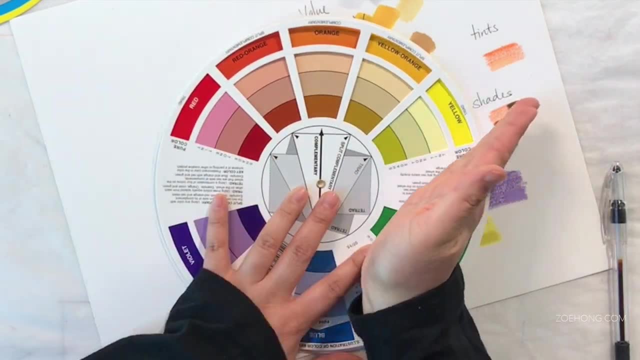 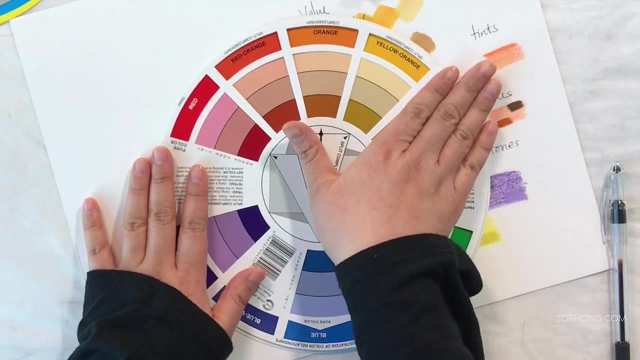 When you start getting more than one primary color. you have red and yellow, So you have some that are red undertone, some that are yellow, And then you have, of course, the middle And it starts getting a bit much. If you take out the yellow, everything has a little bit of red in it. 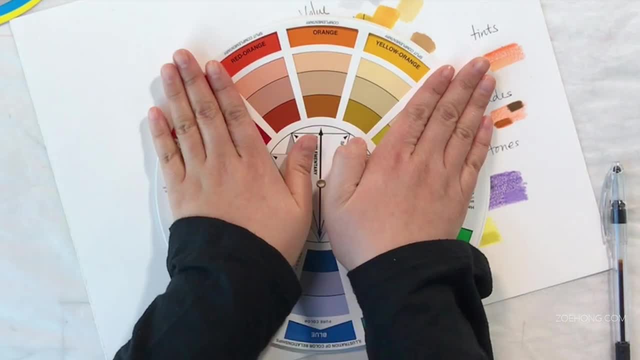 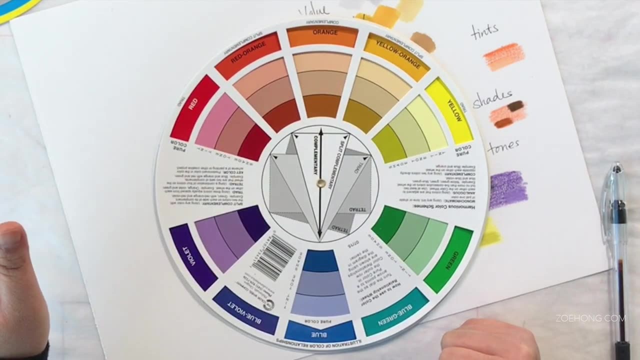 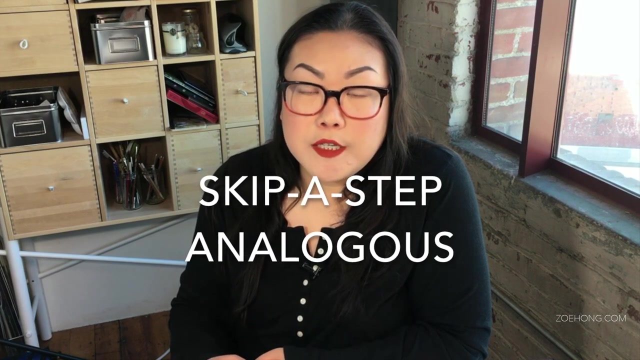 And so this looks cohesive. Here everything has a little bit of yellow in it And this looks cohesive. That looks a bit much. A variation on the analogous color scheme is your skip a step. analogous color scheme: That's when you have a range and you skip one. 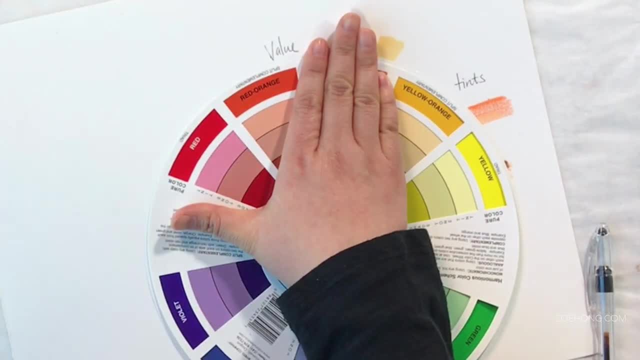 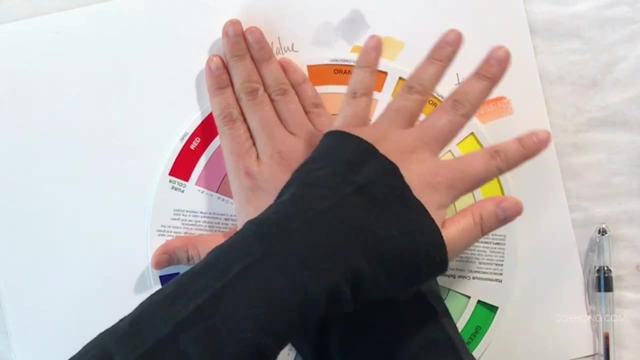 Maybe it's the middle one. You have red, red, orange, yellow, orange yellow, And they all look like everything's on fire. Or maybe you skip this one and you have all these orangey gold colors And then you have pops of red. 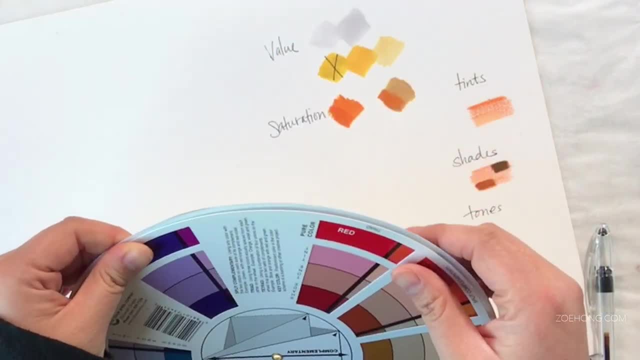 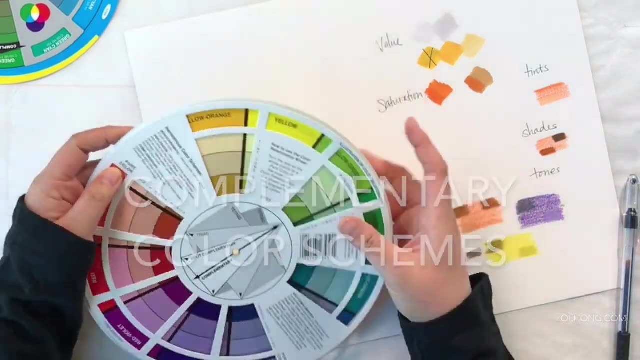 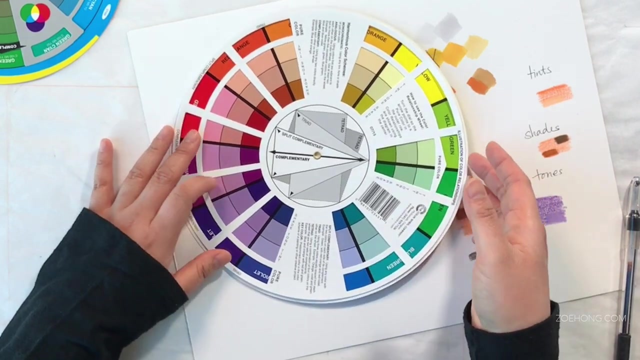 So this is skip a step. analogous color scheme. Next, we have complementary color schemes And this is complementary with an E And not with an I, And complementary color schemes are opposites on the color wheel, So violet and yellow are complements. 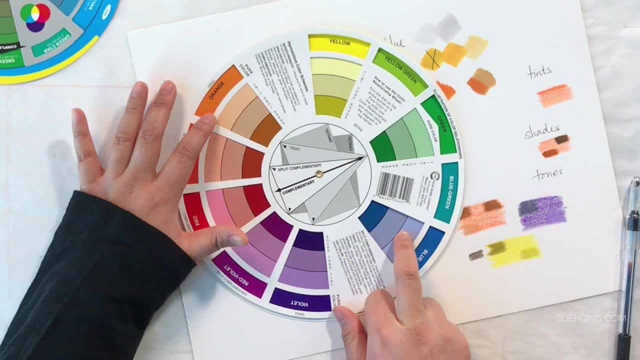 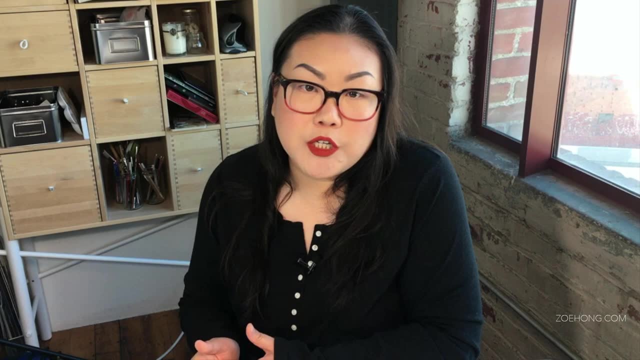 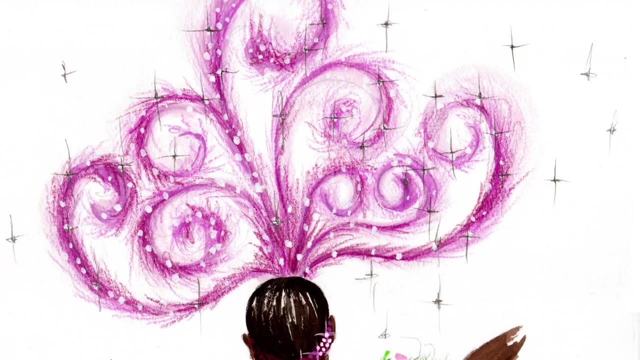 Red and green are complements And orange and blue are complements. When you put two complements together, because they're the furthest thing from each other, they create the highest contrast, So they make each other pop. If you watched the time lapse illustration where I painted the showgirl in gouache and 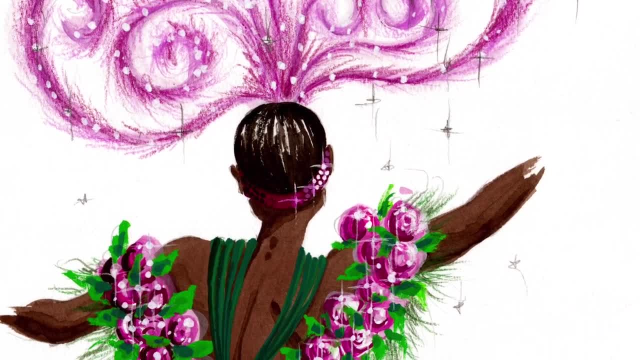 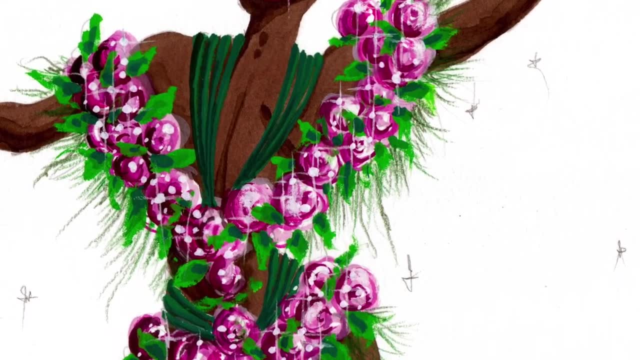 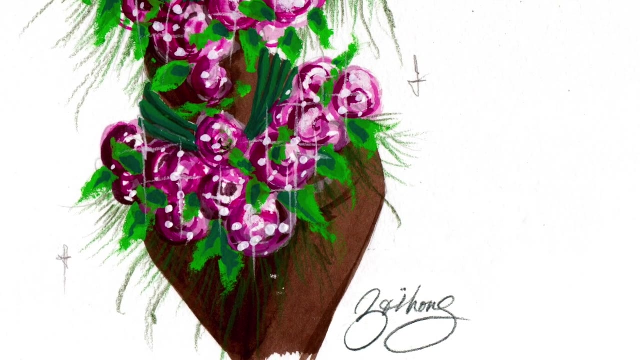 she was covered in flowers and I had the red violet flowers and I was putting a lot of yellow green into the leaves so that the complements working together would really make each other pop, because I really wanted those colors to just stand out very strongly. That's how complements are used. 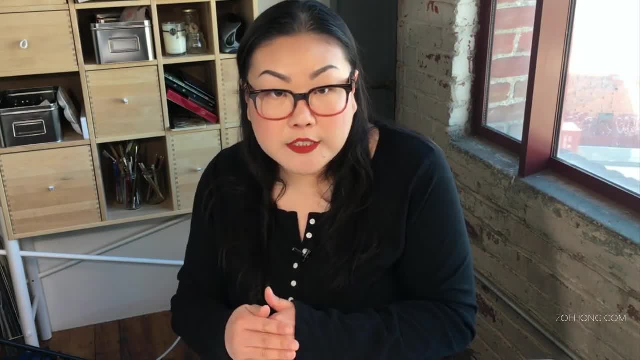 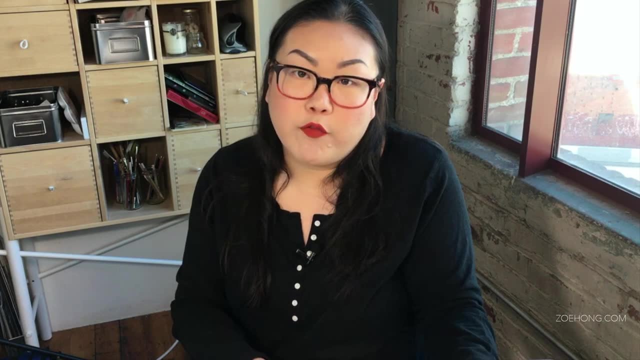 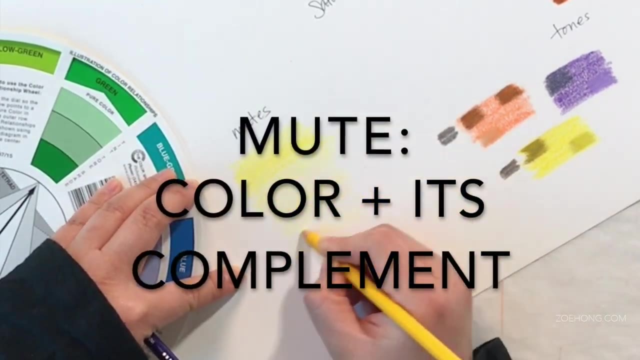 You might be thinking: well then, how do they go? How do they harmonize together? You can harmonize them together by creating mutes with the color. Now, muting is the fourth way to desaturate a color. Muting is when you take your two complements. 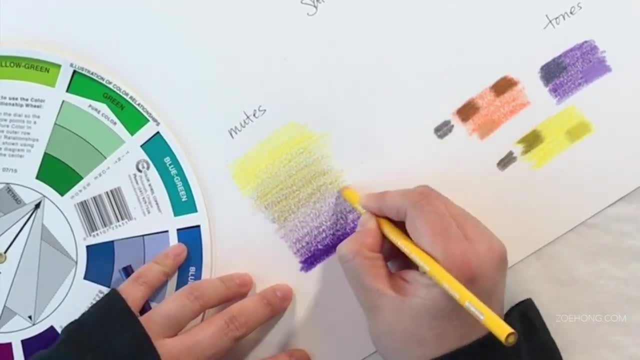 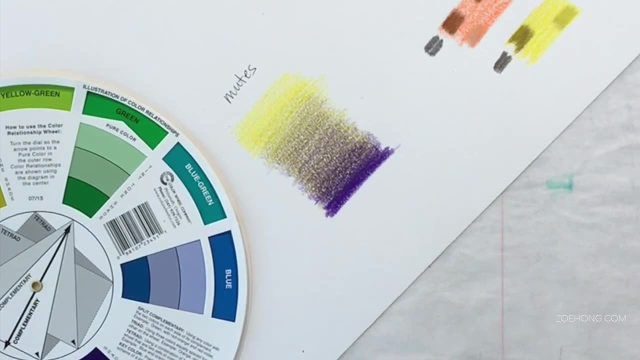 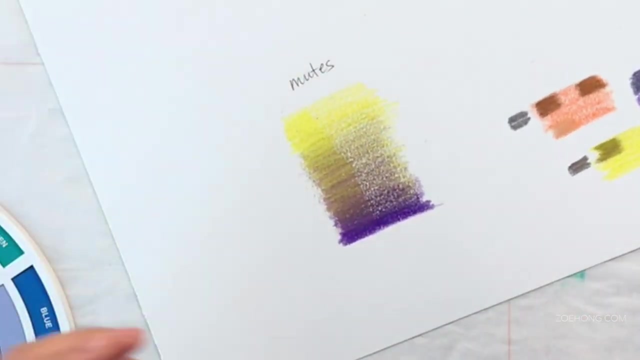 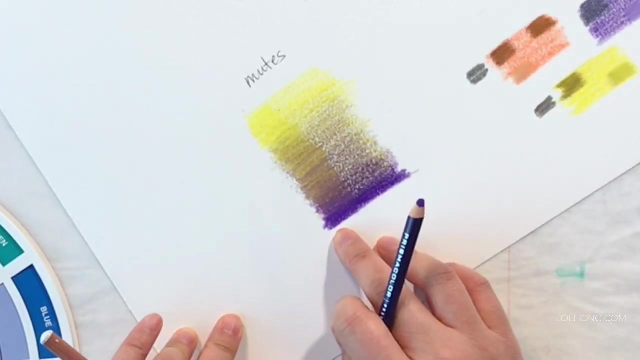 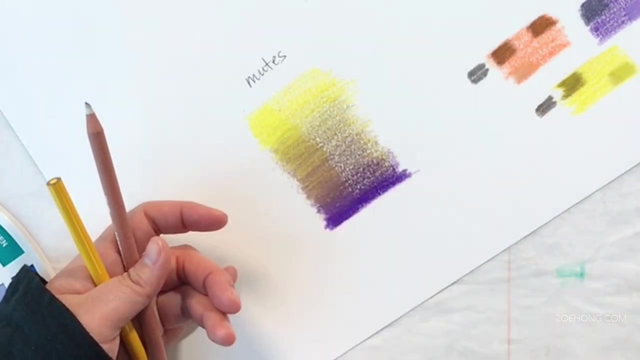 I'm going to use yellow and purple and start mixing them together. Here we go. Alright, So this is not the best blending job I've ever done in my life. Oh my god, I'm trying to move along with this tutorial here. 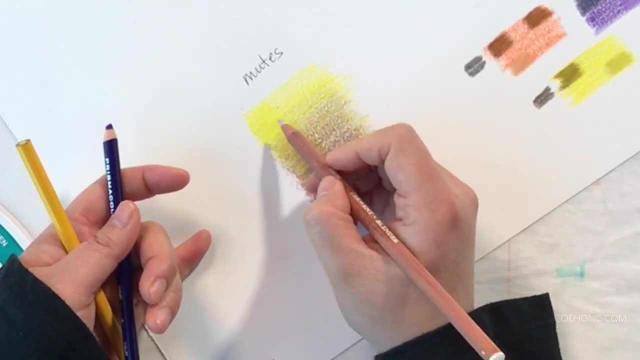 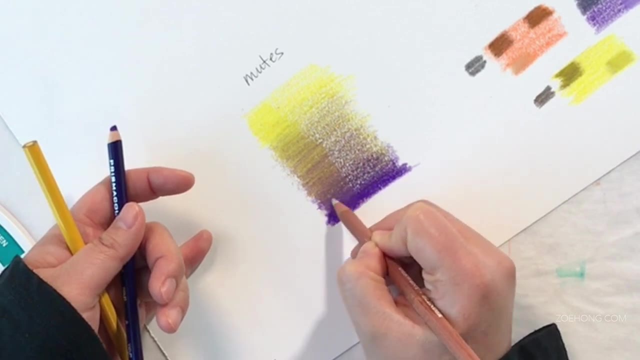 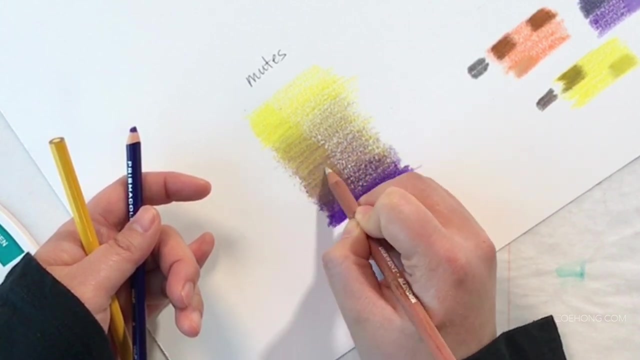 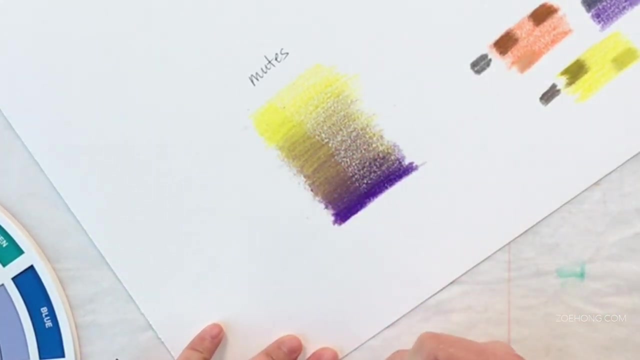 But you can see by mixing different ratios of the complements. You know, here's 100 percent purple mustard territory and here you're getting duller violets, more brownish purples, right, and you're creating all these neutrals in there, okay, and so you can have this bright yellow, you can have this. 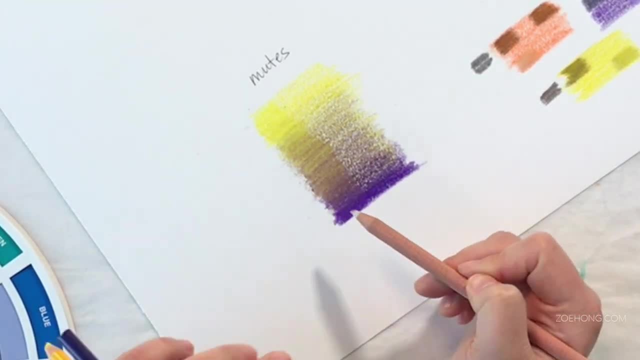 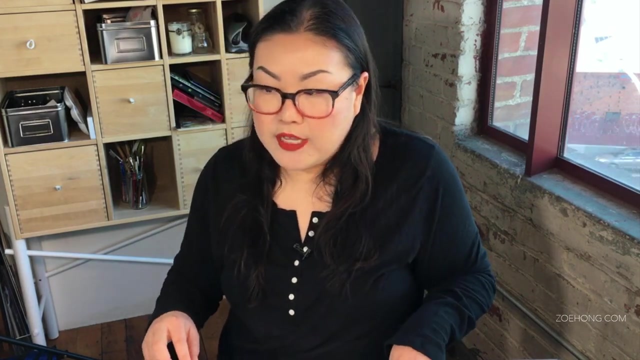 bright purple, and then by incorporating some of these tones in here- i'm sorry, these mutes- incorporating some of these mutes in here, you can start creating a more harmonious color story. the fourth, fifth, seventeenth, whatever uh color scheme i want to talk to you guys about is split. 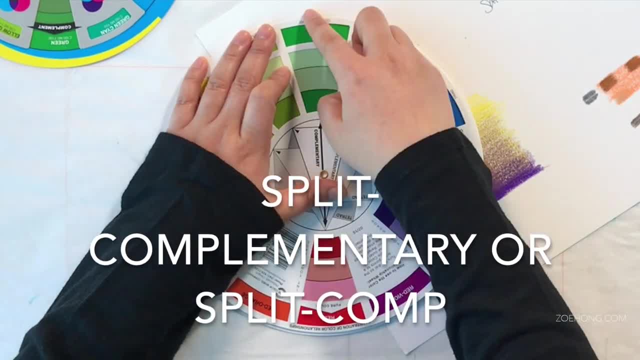 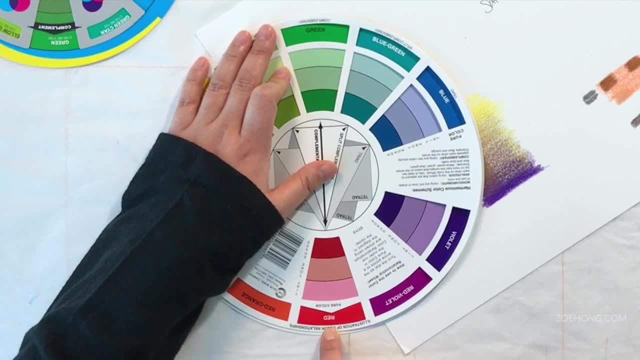 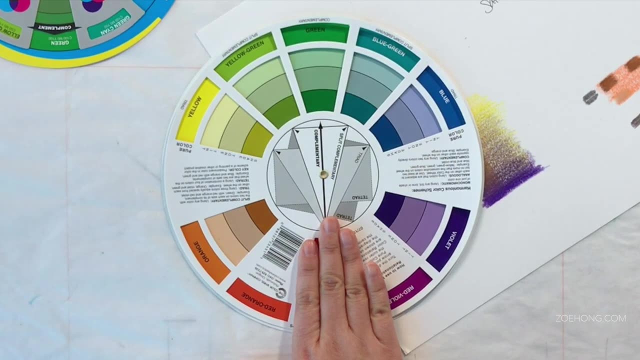 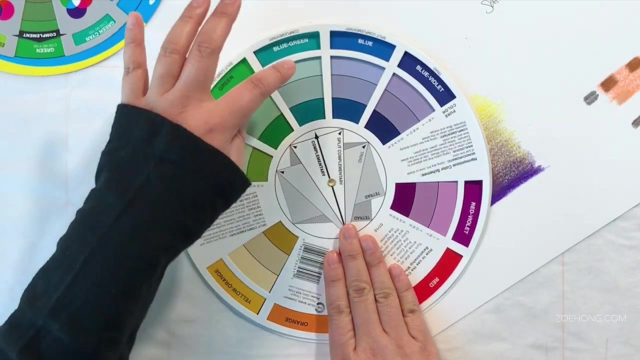 comp: split complementary. split comp is when you have a color, okay, pick green, and instead of the complement your red. you are using the red orange and the red violet. okay, so green, red orange, red violet. that is your split complementary color scheme: blue, green, the complement is red orange, the split comp is blue, green, red and orange and you can do this kind of. 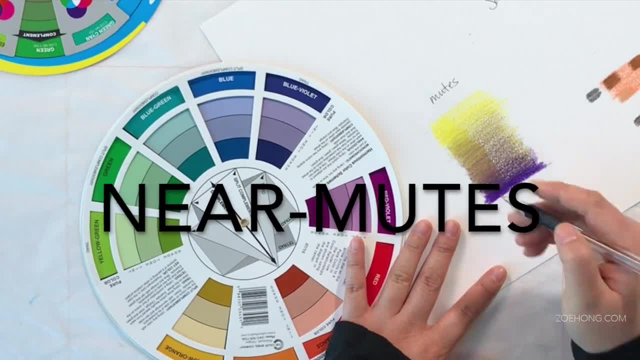 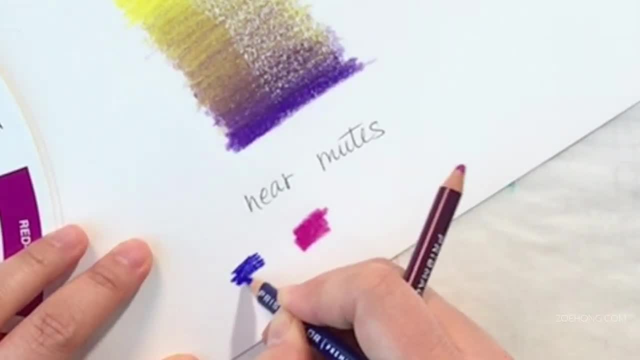 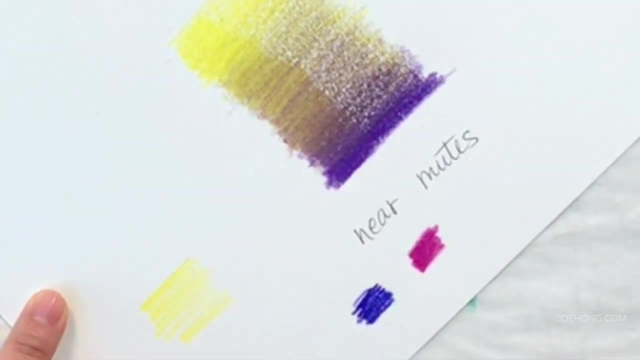 technique to create what are called near mutes. so here is, this is mulberry, which is my red violet, here is my violet blue, which is my blue violet. so, again, you can create near mutes by mixing. there's my split complementary color scheme, here's my yellow and you can create near mutes by, you know, mixing these two colors. 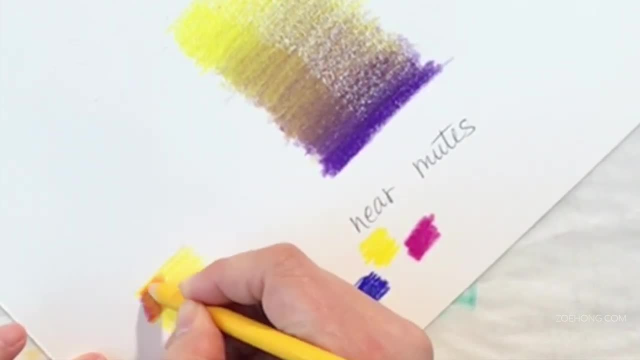 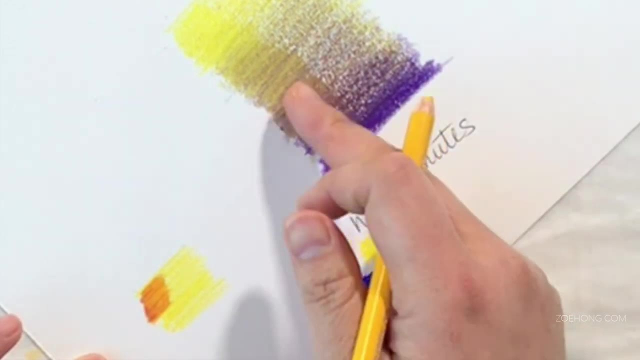 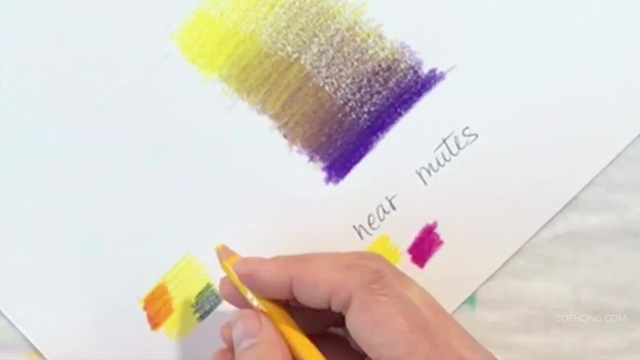 and because the red violet has that more red in it, you're starting to get orangier tones. then what you see here is a little bit more of a red violet, and then you can create near mutes by, and then with the blue violet, because it's so much bluer, you're starting to get greener mutes. 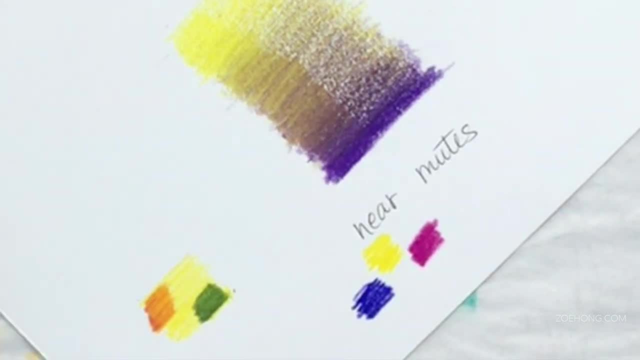 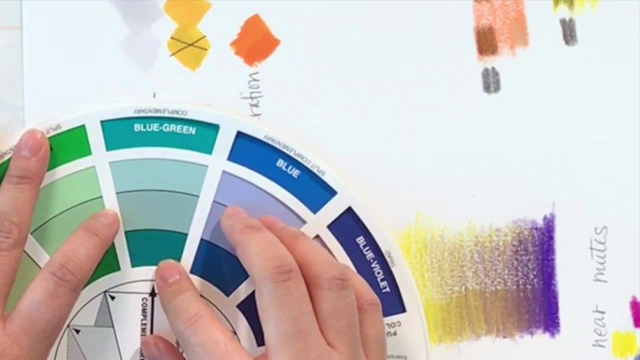 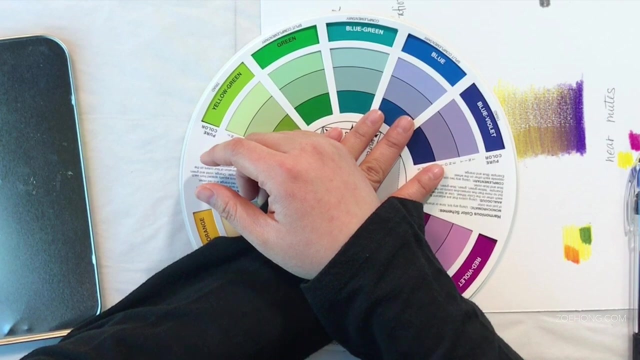 than the full complement. that's how you start figuring out how to create colors. so you know how i said. in monochromatic color stories you have tints and shades and tones, and all that. when you have analogous color schemes, you can have also tints and shades and tones. you can't have. 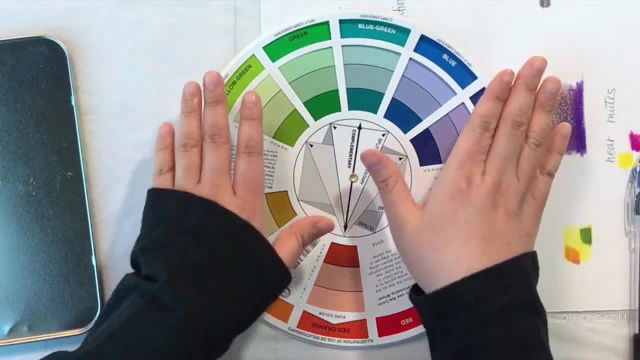 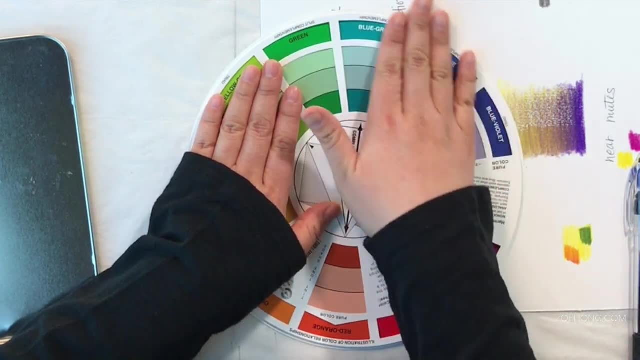 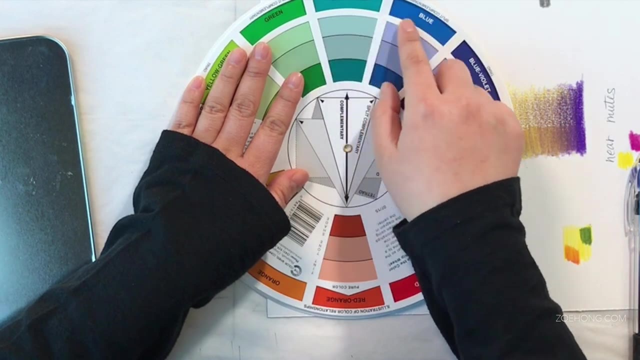 mutes, because now you're introducing a totally different color. so let's say, this is your analogous color story, so you can have tints and shades and tones of these four. but if you start creating mutes or near mutes, you're adding orange and red orange to the equation. you're changing the 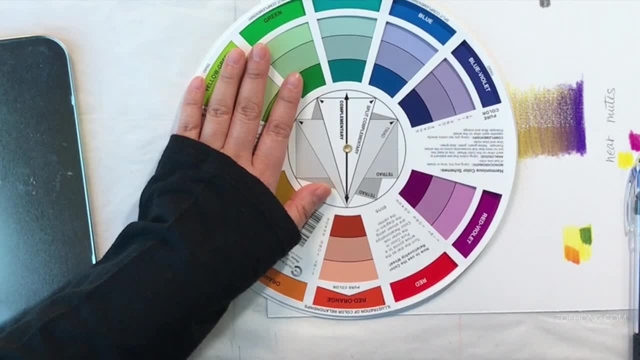 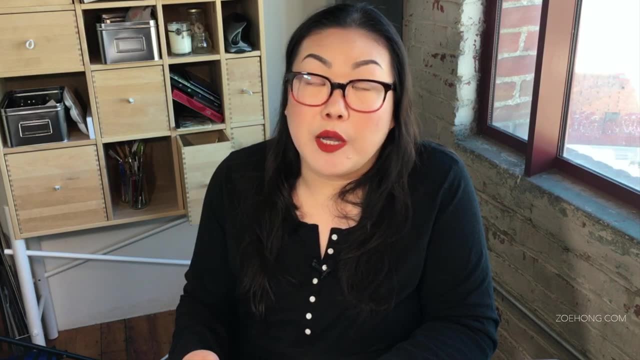 temperature too much and it really ceases to be a true analogous color story. and you're like zoe. do i have to make every color story? and you're like zoe, do i have to make every color story? and you're like zoe story a pure analogous color story, a pure complementary color story? No, that's not what. 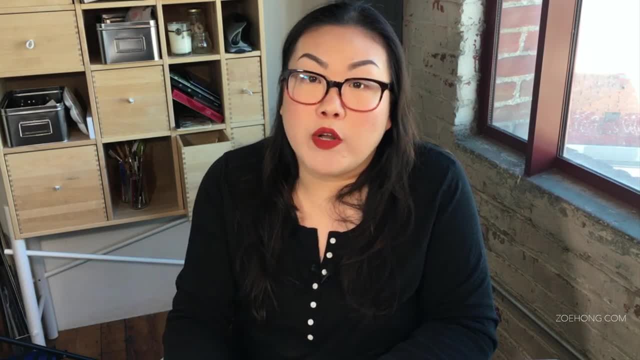 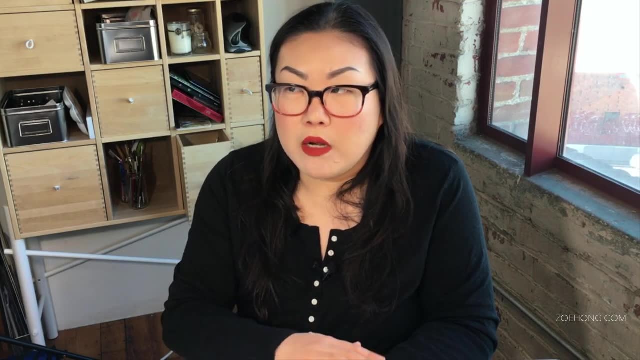 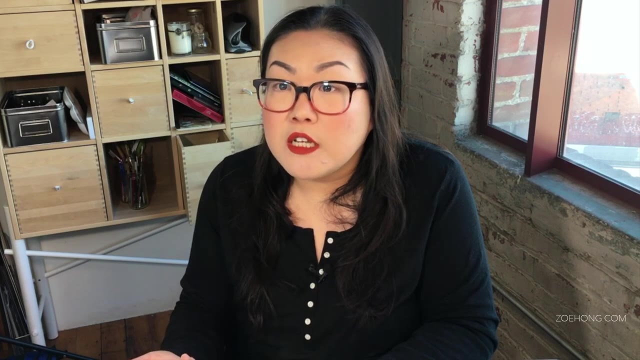 I'm saying, I'm giving you the definitions of what these things mean so that you have a knowledge base. So later on, when you are creating analogous color schemes, if you decide to make a temperature change, it's a deliberate decision and not an accident With complementary color stories. 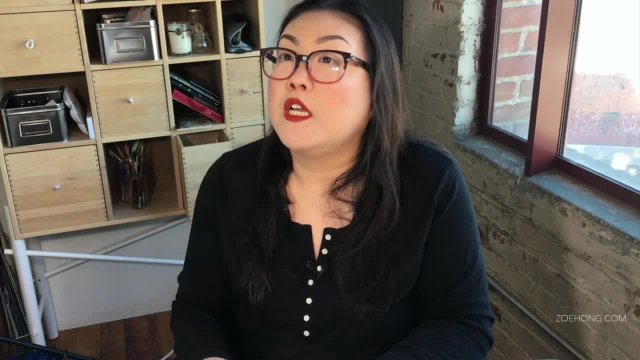 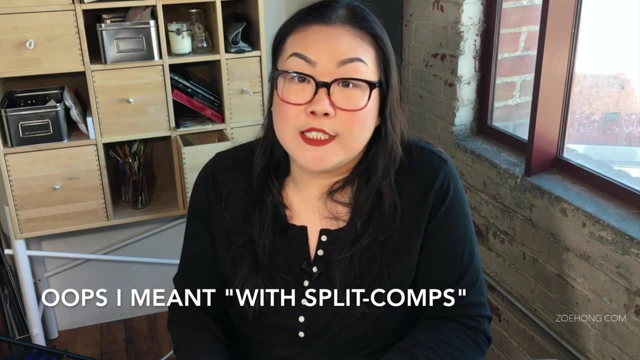 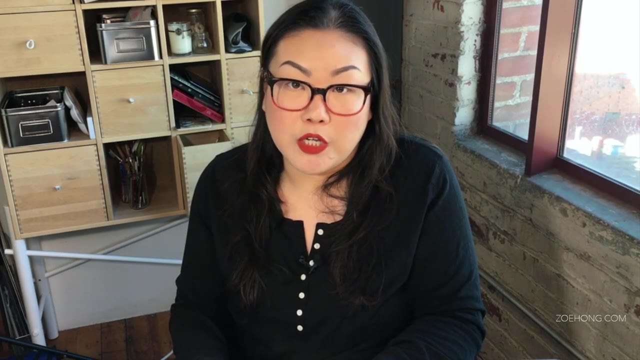 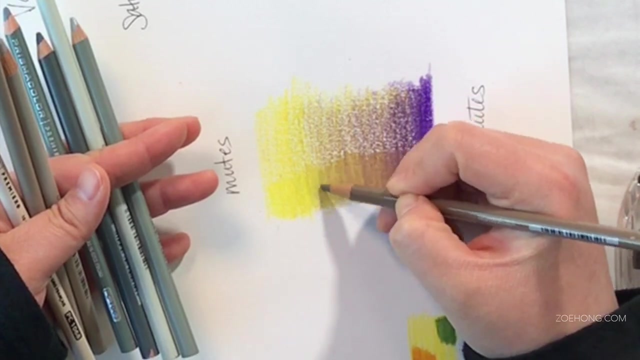 you can tint and shade and tone and mute to your heart's desire And with complements you can tint and shade and tone and near mute and include all the ways of desaturating into your color story. You could have all these colors or you could make this color duller. 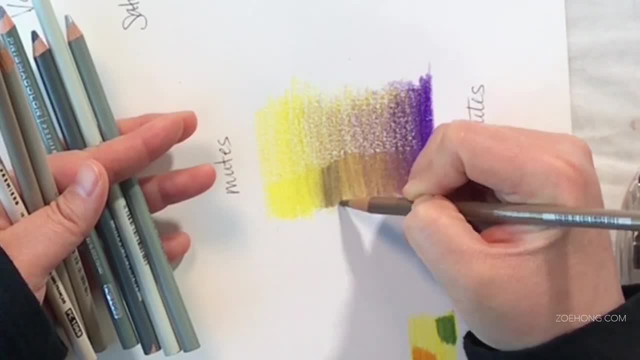 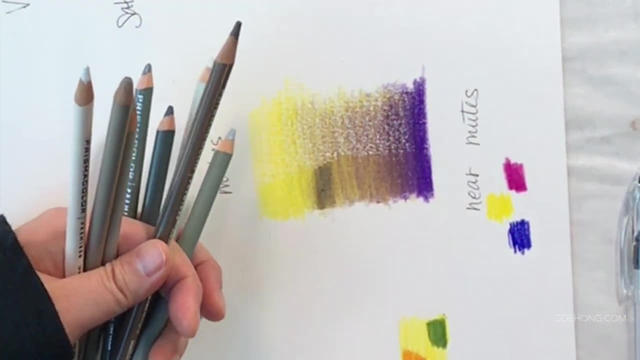 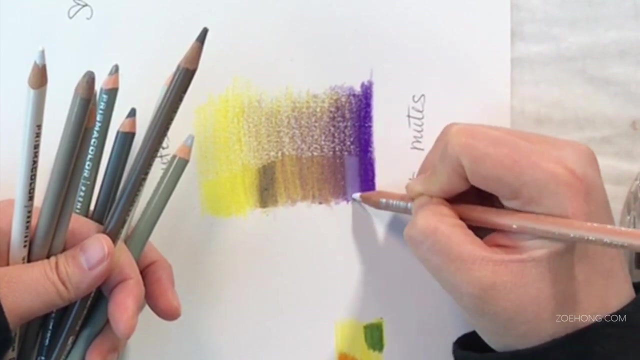 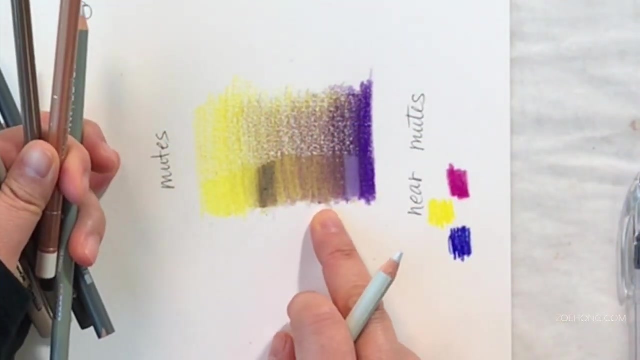 with a lot of French gray, And so you have a tone of this color And maybe you want to include a really light, muted purple in there. Okay, And then you want, I'm using all these grays, I'm using the cool grays for things. 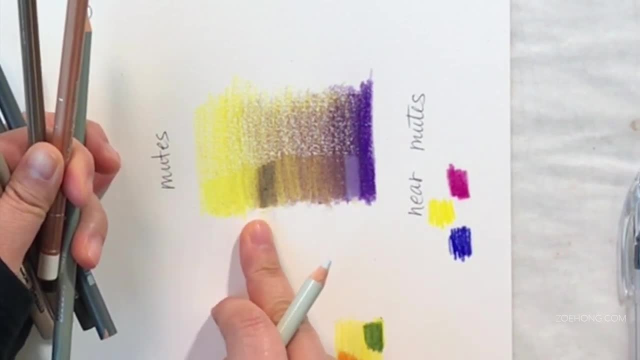 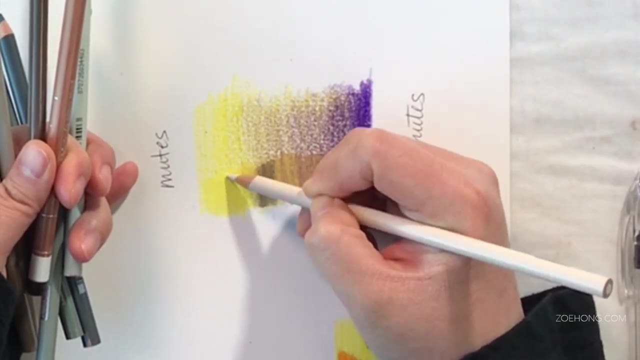 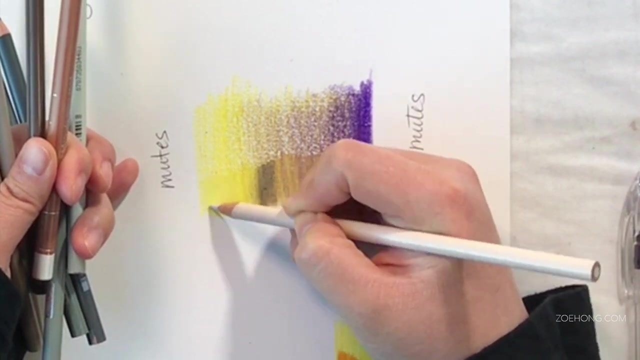 that are more purple and I'm using French grays for things that are more yellow. Okay, And so maybe I want not this bright yellow, but just a slightly more toned down yellow, Cause I don't want super sunshiny business all up in my collection. Okay, And maybe I want to. 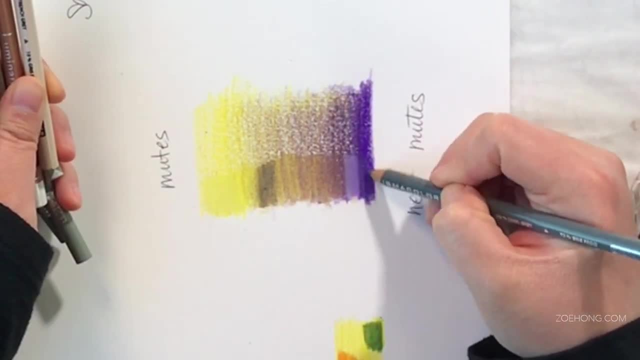 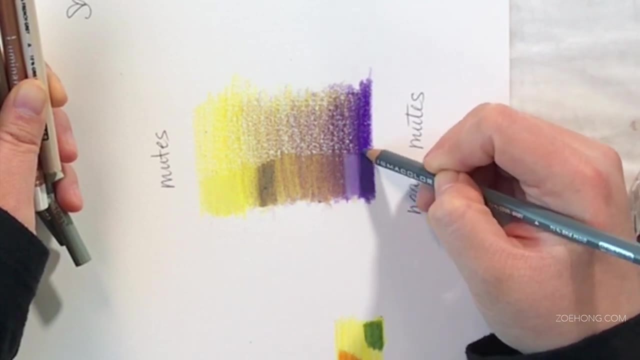 I don't want this vibrant purple. I want to keep that dark value, but I want it a little bit duller. So I'm going to add this 70% cool gray so that it's still purple. You know, the value is not. that great. So I'm going to add this 70% cool gray so that it's still purple. You know the value is not that great. So I'm going to add this 70% cool gray so that it's still purple. You know the value is not that great. 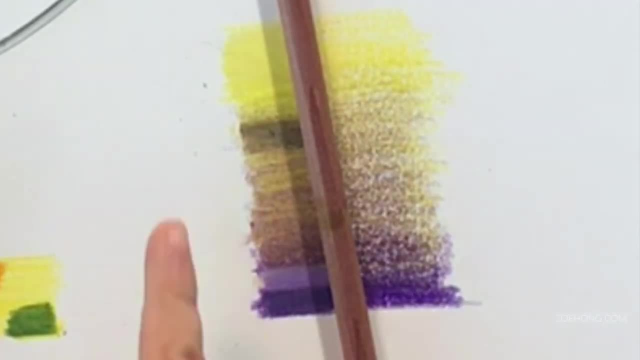 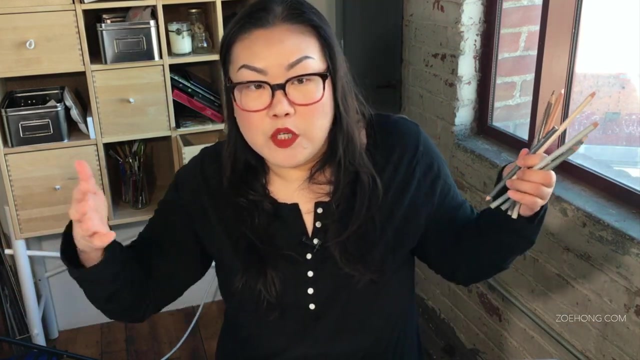 different but it is a little bit duller. And now you're creating this color story with your compliments and creating tones and tints and shades and whatnot of your mutes. Okay, So you can create all kinds of- you know- tints, of tones and mutes of tints and all these things, But as long 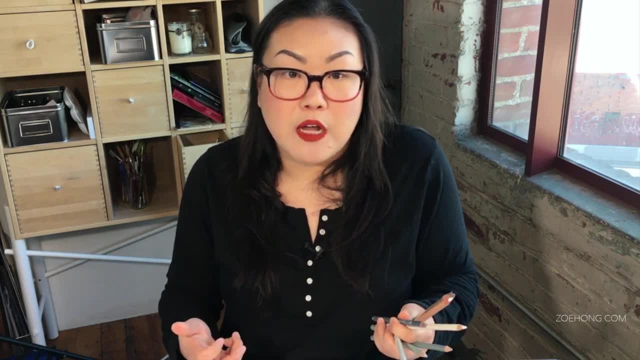 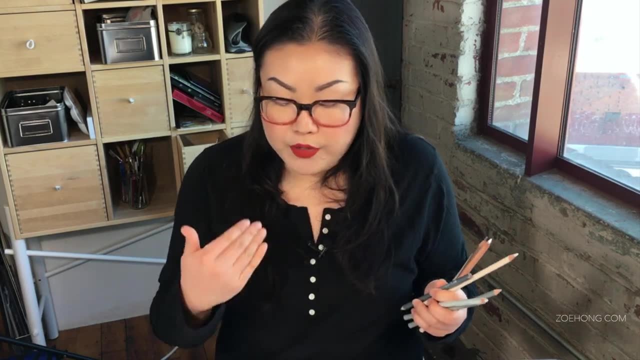 as you know what they are, then you know how to mix them, You know how to create those colors. And when you know how to create those colors, then you understand undertones, tones, And so when you're like, well, I want to add another color in there, then you know. 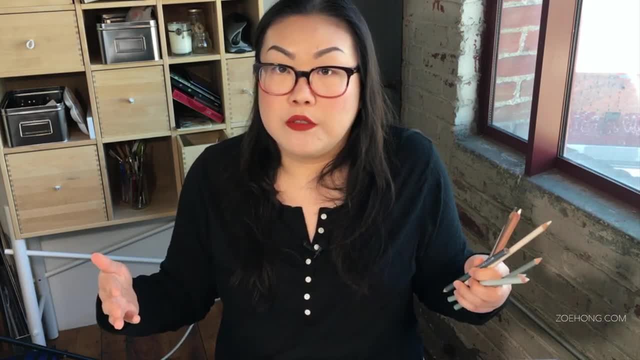 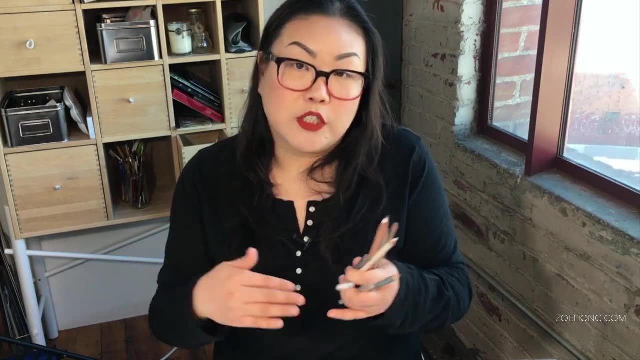 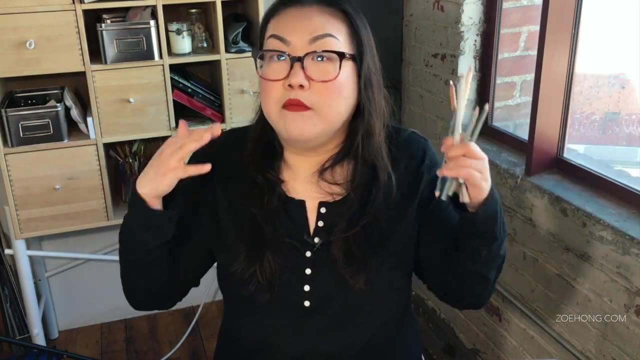 if you pick a color with the right undertone, it will kind of insert itself into this color story easily. Okay, When things share the same undertone, everything works. Okay. You can want things to clash crazily, That's up to you. I'm just saying this is also a way you can do it. 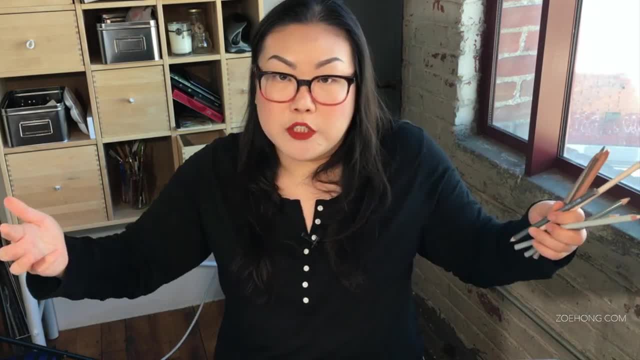 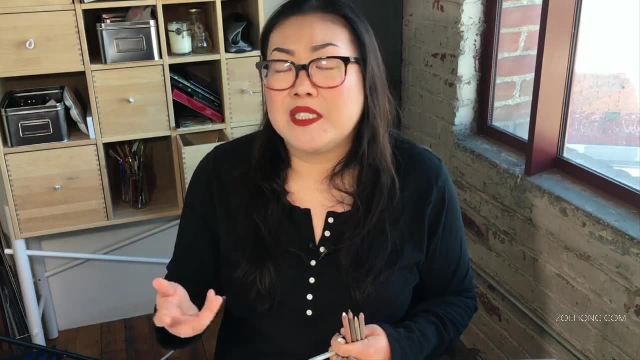 The more you know, the more deliberate decisions you can make. That's pretty much what it is. You know, designers make deliberate decisions on how they want their things to look. I'm not discounting happy accidents. Happy accidents are awesome. I think that was enough for today, right, That was. 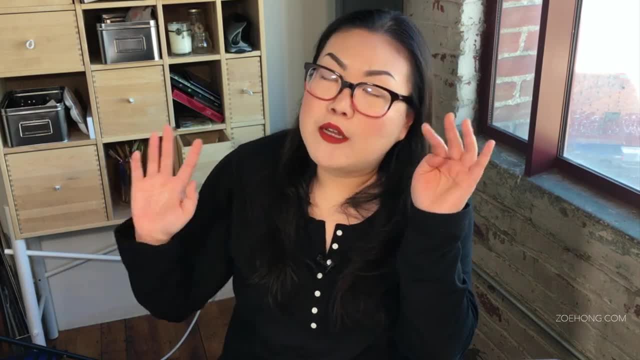 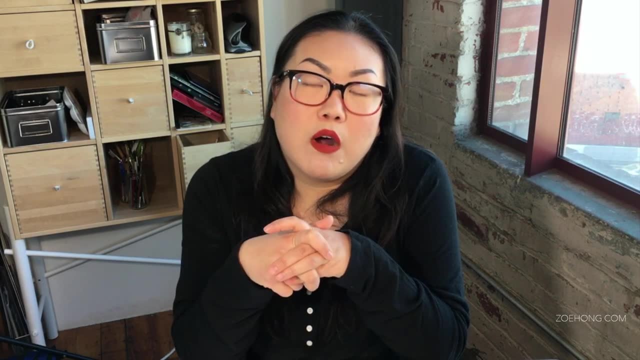 a lot. Okay, I have no idea how long I've been filming, but I feel like that's plenty of information for one day. If you found this video helpful, give me a thumbs up. Uh, if you are burning to have closed captioning available for the rest of the day, I would love to hear from you. 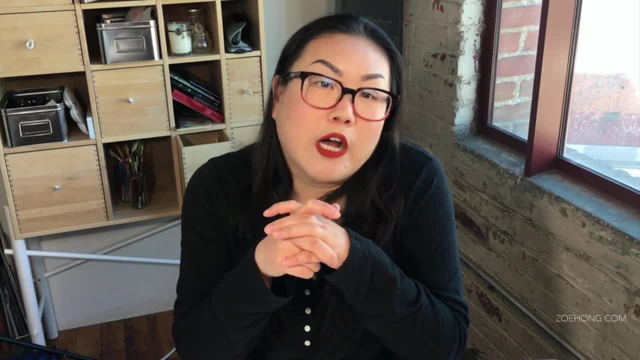 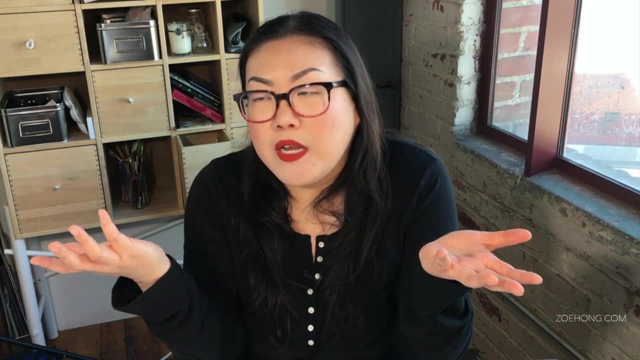 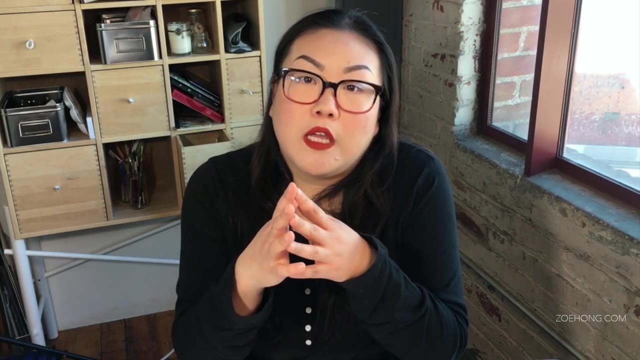 For all my videos on my channel and you've got a dollar or two in your pocket, please consider donating on my channel main page and, uh yeah, share with with anyone. you know these are basic color theory concepts that will help anyone in any art or design field. So you know it really. 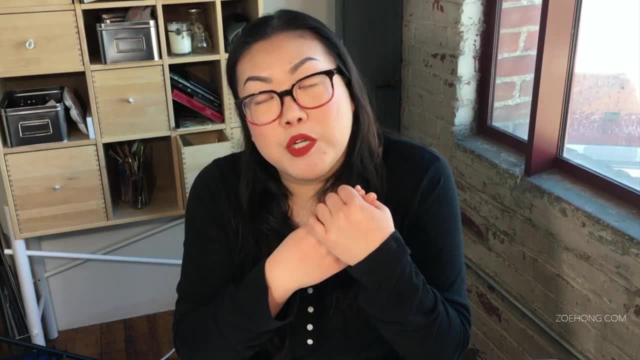 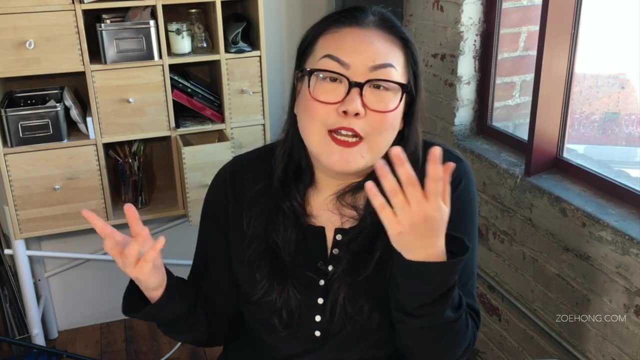 helps me out when you share my videos and subscribe. If you want alerts for when the next in comes out, hashtag, always be practicing And I will see you in the next video. Hey, hey, party people. today I'm going to show you how I painted this color wheel using only 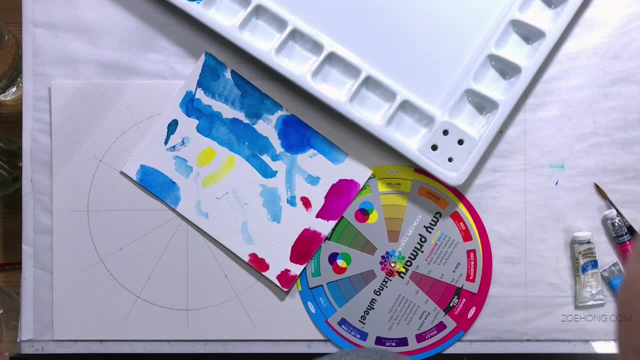 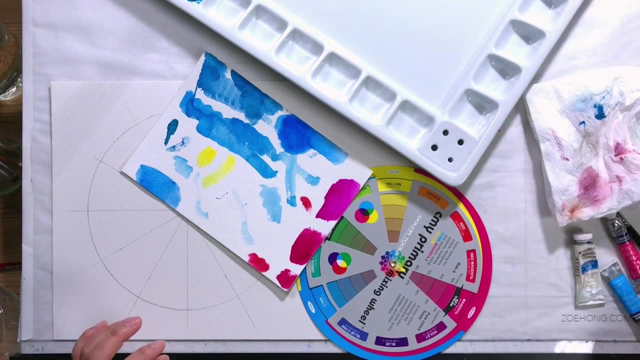 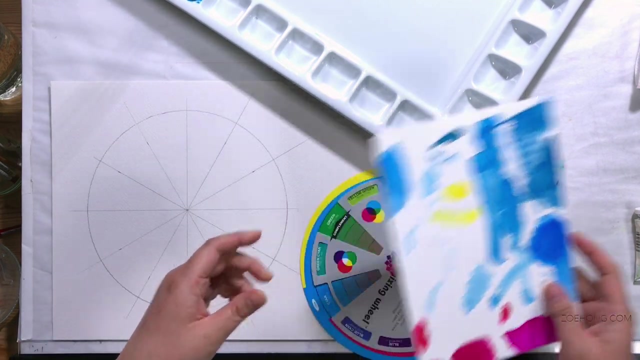 three tubes of paint. Let's get started. I use the CMYK coloring wheel method color system- what have you? to mix paints? Okay, I use the red, yellow, blue kind of standard color wheel color system for designing, But that's what people are used to looking at, And so when I'm designing, I cater to. 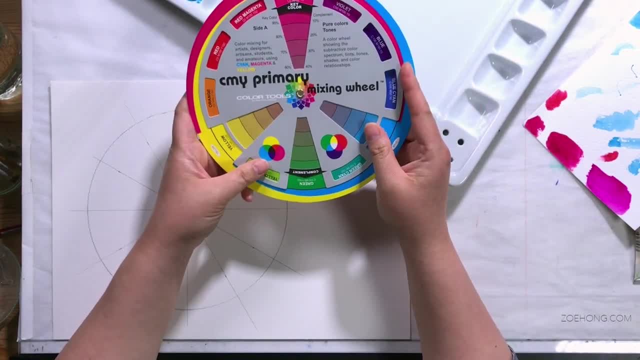 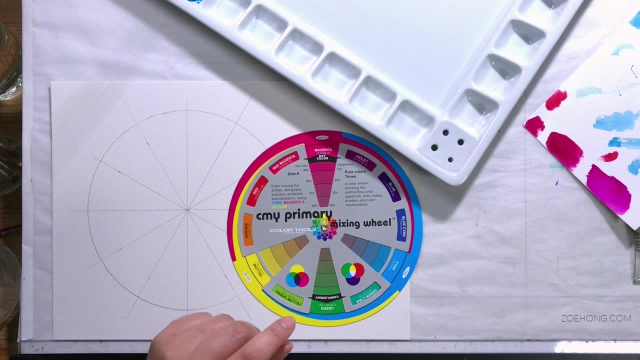 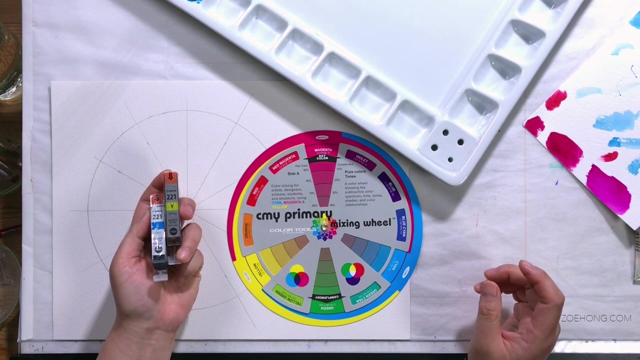 you know what people are used to looking at. but for mixing paints, I find that you get the best methods by using cyan, magenta, yellow and black, and uh, so does your color printer. Okay, That's what your color printer takes. Uh, I don't have my magenta cartridge. 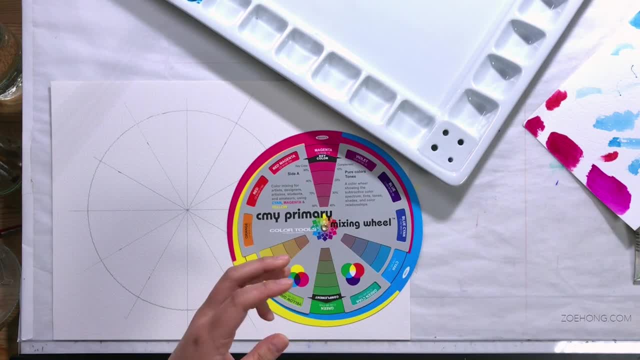 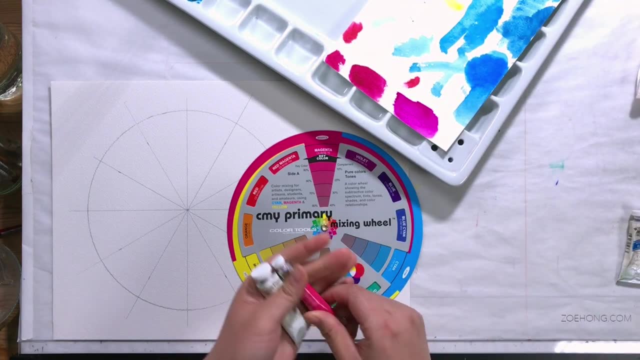 but cyan and yellow and black. That's what your personal printer takes, That's what your professional printer takes. That's why, whenever you want to print something, you want to format the document CMYK. All right. So of course you. 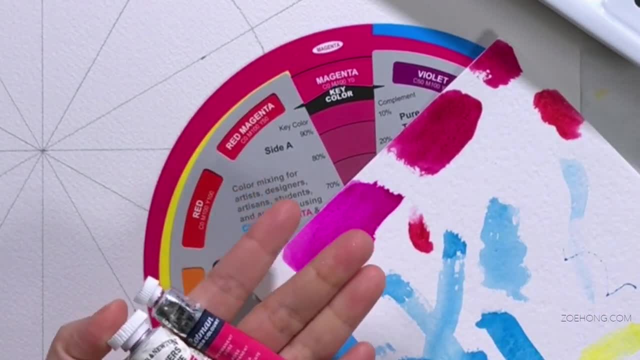 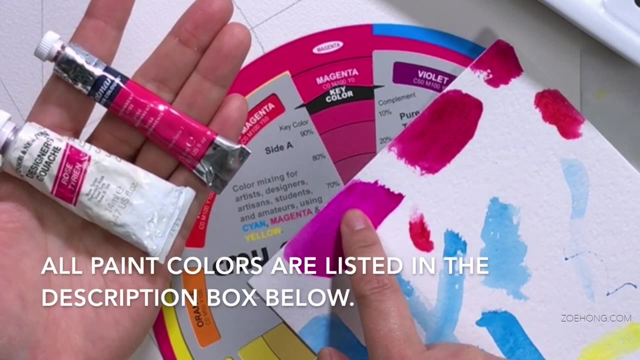 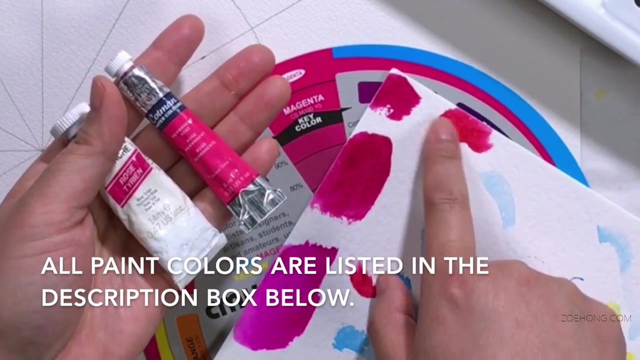 don't have to use the colors- exactly the ones I use, but to help you get started. for magenta, I like the Windsor Newton gouache in Rose Tyrian- It's a little bit blue, Okay. And I also like the Windsor Newton Cotman watercolor in Permanent Rose, which is a tiny bit warm. So sometimes I 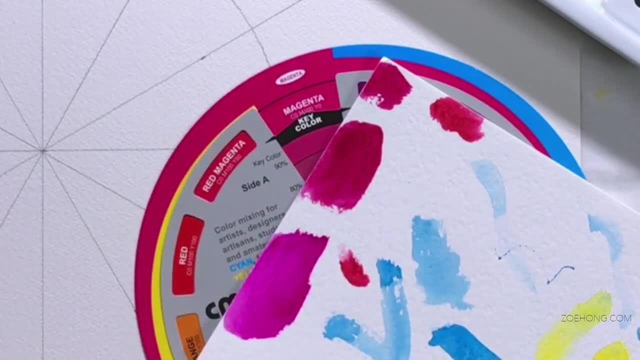 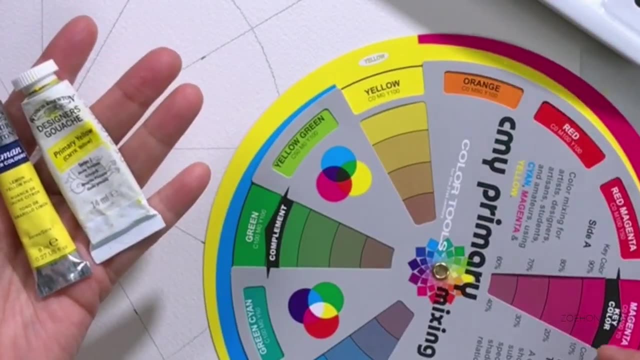 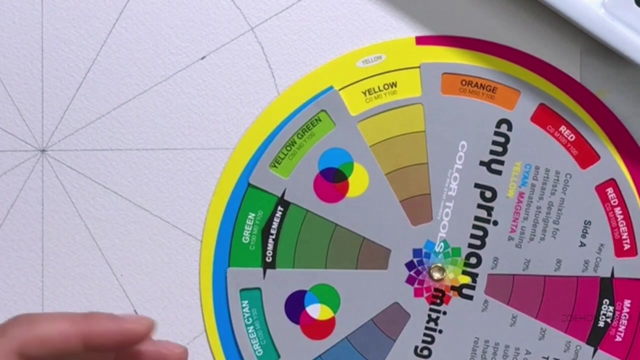 just mix the two. I'm probably going to do that here. I'm going to cheat a little bit For yellow. you know I use the gouache in Primary Yellow, the Cotman watercolor in Lemon. You know yellow subtleties are harder to pick up, So you have a little bit more leeway with what you use. 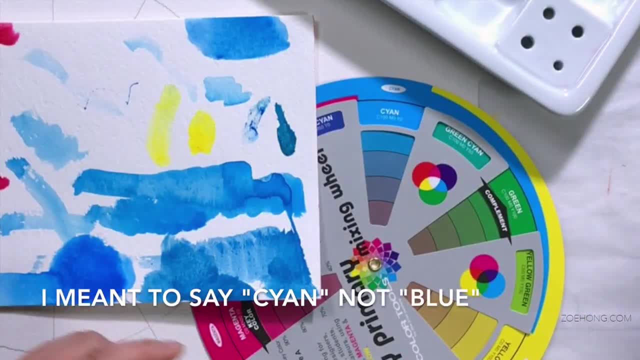 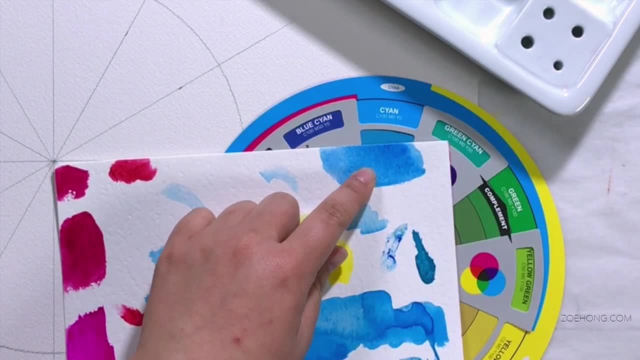 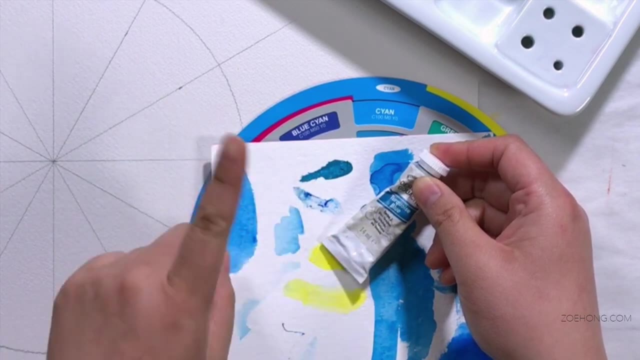 With blue, I use the Cotman- what is this? Cerulean? And for gouache, don't use the turquoise. Turquoise is too turquoisey, you know, because cyan is not actually turquoise. People think it's turquoise. 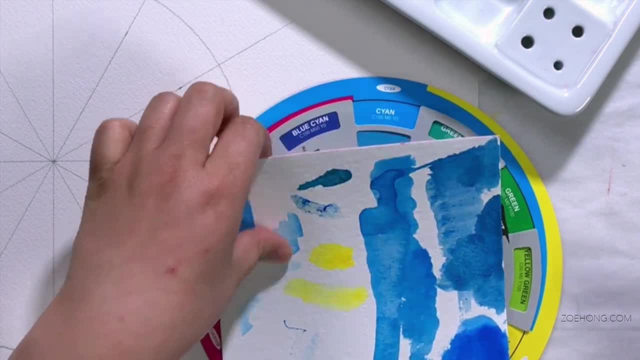 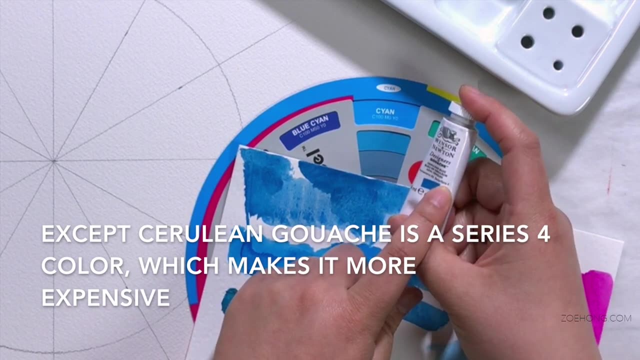 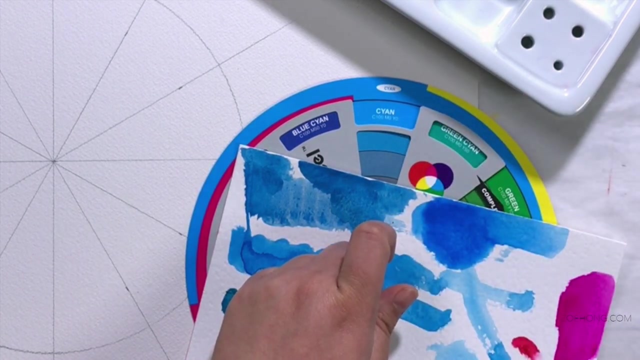 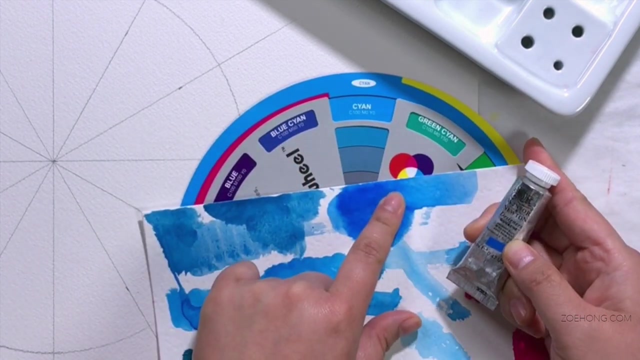 but it's pure, not as dirty, not as muted as turquoise. I like the gouache in Cerulean. The Primary Blue is a little bit too blue- Okay It's. it looks like cyan with a little bit of the magenta in it. Okay, My favorite, and the one I'm using today, is the gouache in Phthalo Blue. 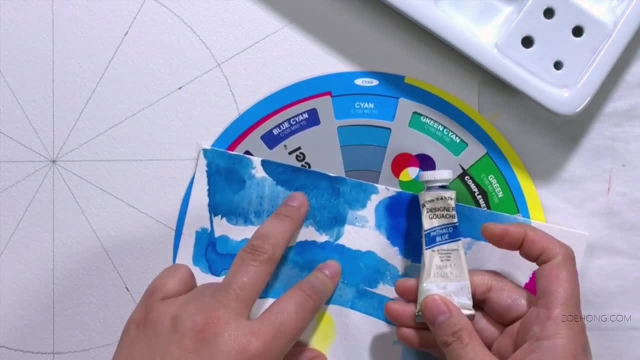 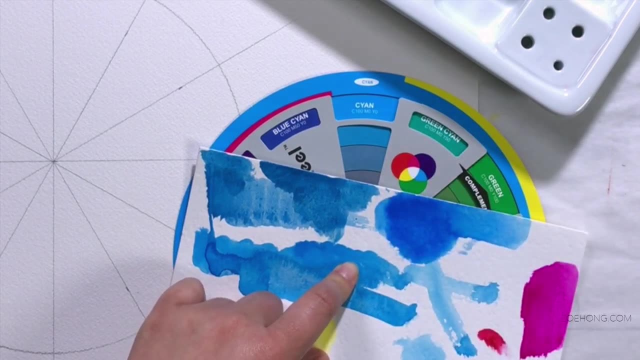 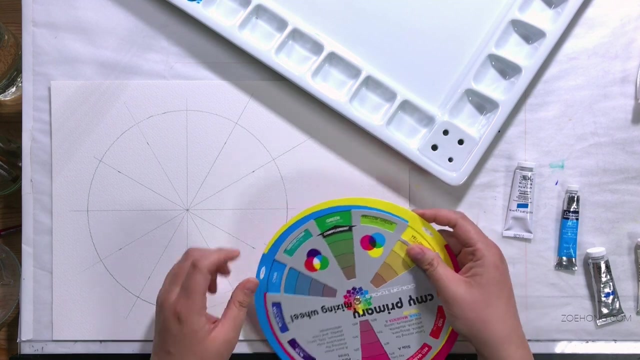 And I think that is the closest to straight up ink cyan that I've seen so far. So again, you don't have to use these, but get something close. I find that using a color wheel to compare Okay, This is a great teaching tool that I love using. 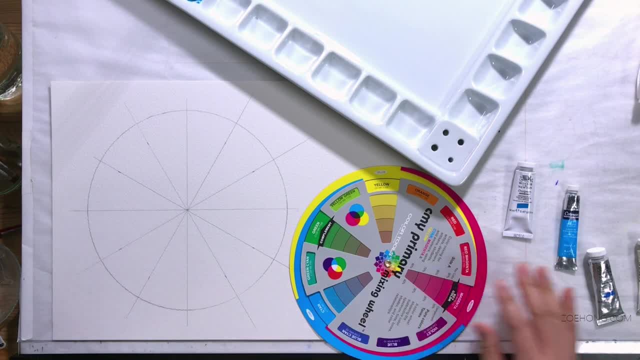 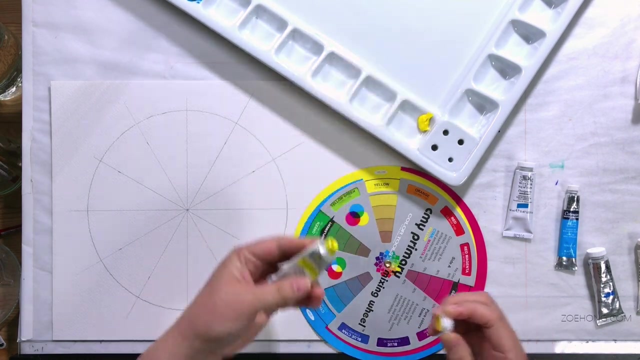 And when you have a hard time mixing a color, I find it really helps to have something next to you to compare it to. So you're going back. Usually, when you're working on a fashion project, that will be your fabric swatch. you know, make sure you're in a well lit space, layer swatch out. 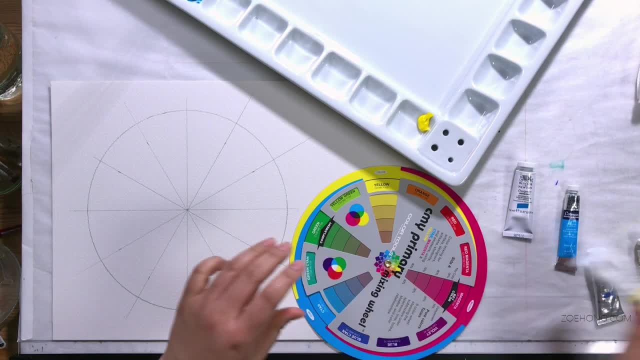 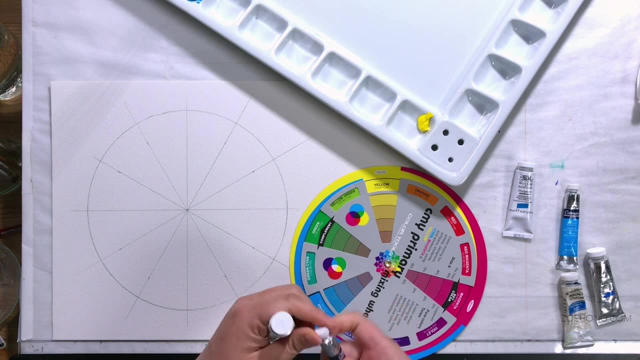 and then take a test, a piece of paper, and mix your colors right next to your fabric. Okay, If your fabric is shiny, make sure that your fabric is not facing the light directly, because that gloss, that shine, is going to affect how you view the color. But other than that, yeah, 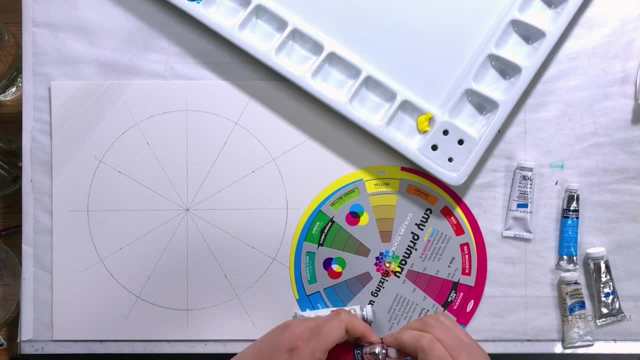 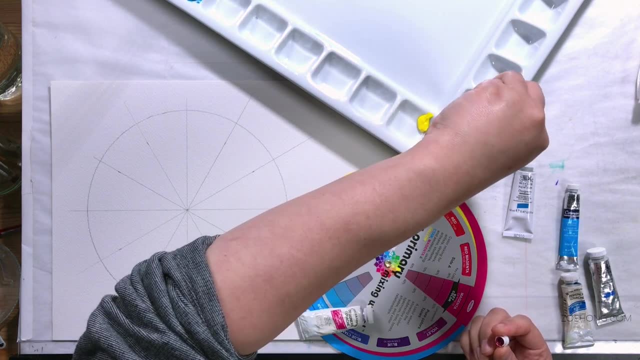 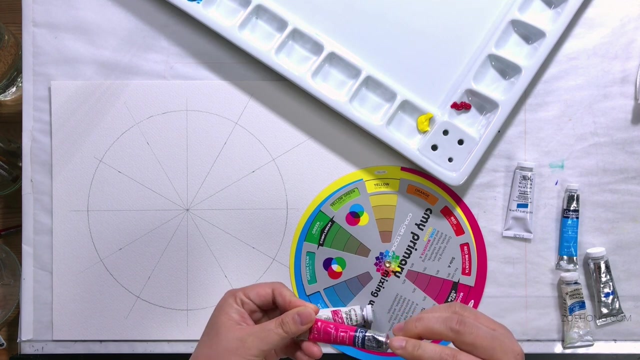 just like put it right next to your fabric. Long time viewers know that I love gouache and I like watercolor and I mix them all up all the time. unless I'm really concentrating on making my paint opaque, Then I you just use a straight up wash If your tubes of paint get a little bit crusty. 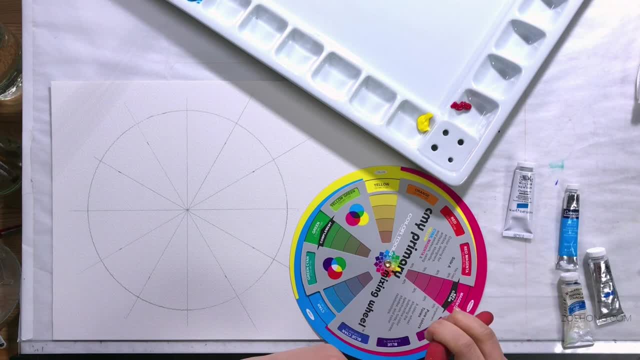 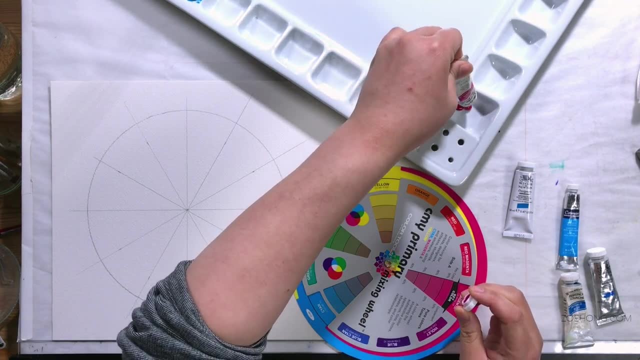 go to the tool store and get some. what am I using? Pliers, Yes, Pliers, All right. I see students using their teeth and I like, I full on- yell at them. I'm like: don't use your teeth. 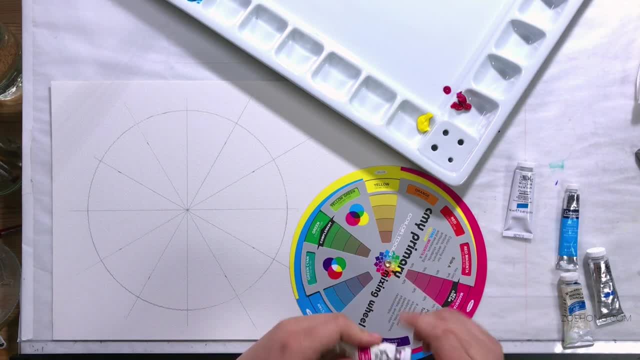 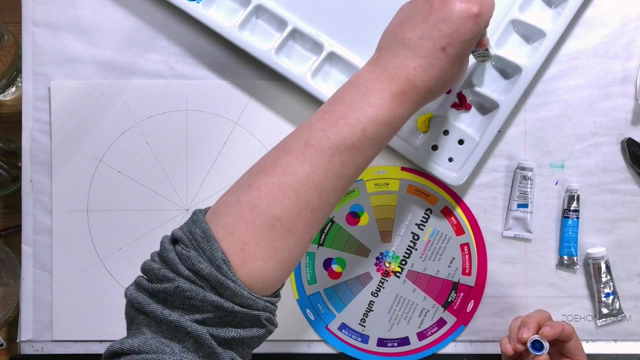 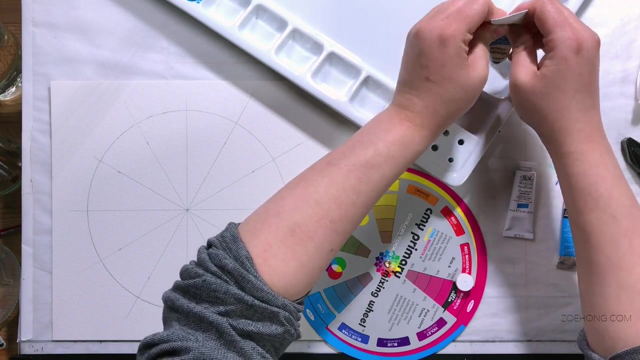 Okay, Do not use your teeth to open tubes of paint. That is so bad for your teeth, Oh my God. All right, So I'm using the primary yellow gouache, I'm using the phthalo blue gouache and I'm mixing up the rose, Tyrian and permanent rose. Uh, cause, I'm a filthy cheater, but again. 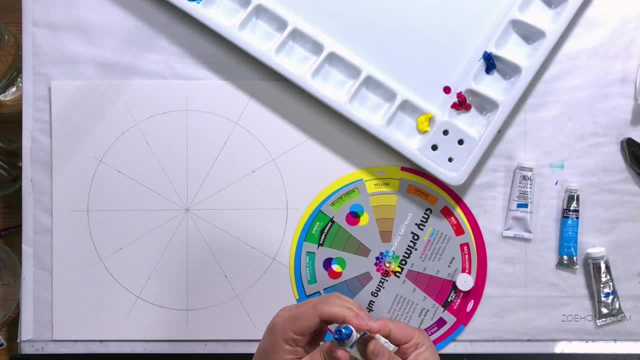 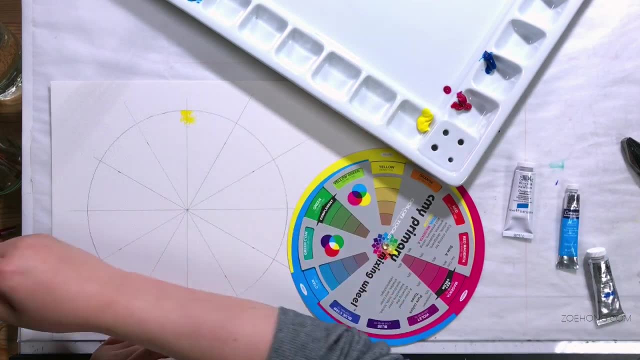 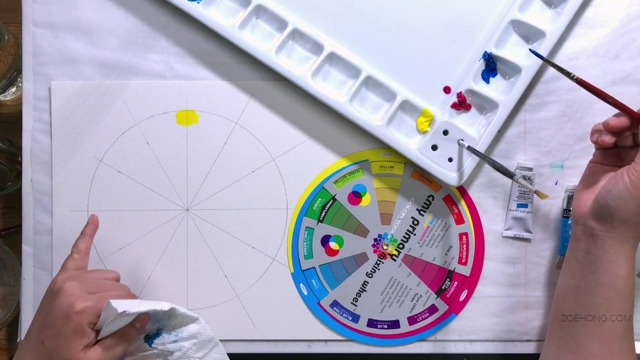 you could use either one, I don't care, And I drew a perfect circle using a compass or protractor- I always get those two words confused. Okay, I used one of those And then I I drew out 12 spaces so I can space out the colors evenly. And I'm just placing the colors. 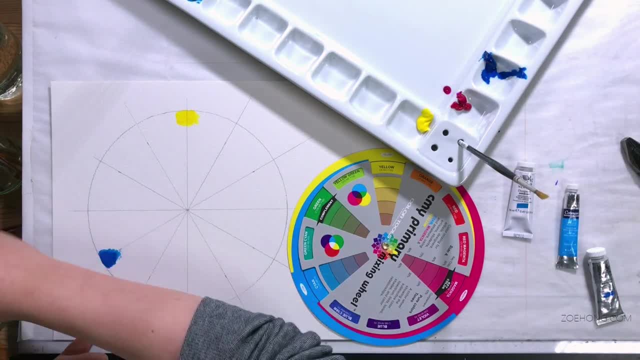 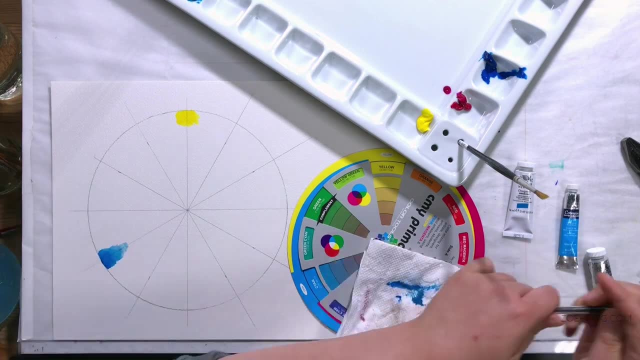 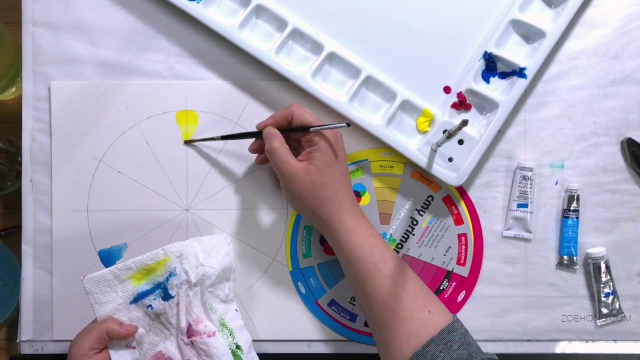 mimicking the color wheel I'm using as a reference. It's not like yellow has to be 12 o'clock all the time, because I want to concentrate on the colors being as pure and intense and concentrated as possible. I'm using several different brushes and several different cups. 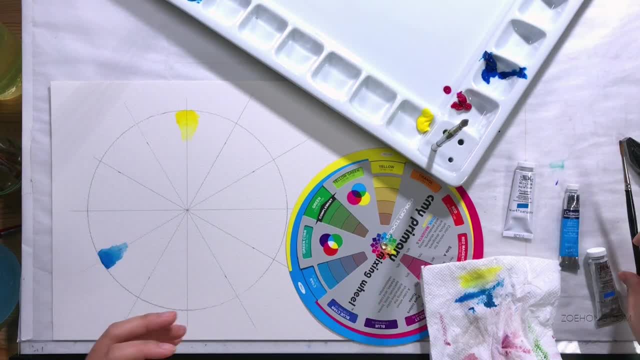 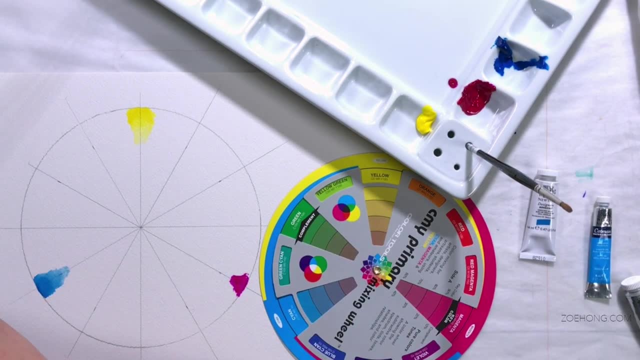 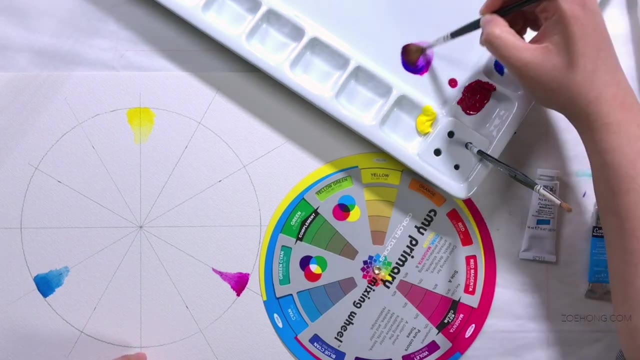 of water If you can see them on the very far left of the screen With watercolor and gouache. if you want to make a lighter color, you typically just add some water. but if you're concentrating on making a color opaque, like if you wanted to put like light, 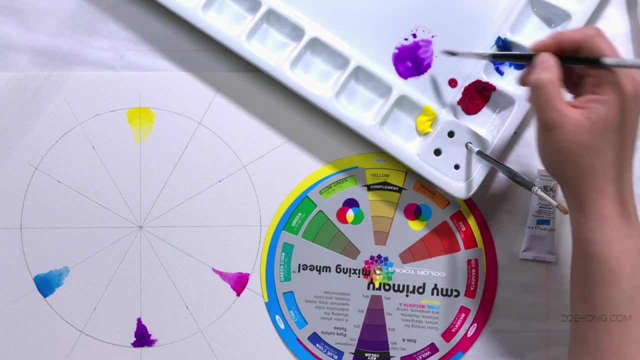 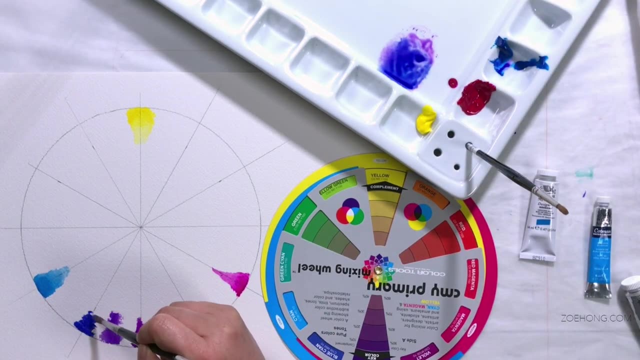 pink flowers on a black background. then you can use white gouache. I'm going to have a whole video dedicated to creating tints and shades and tones and what all those different things look like in the next video. So I'll see you in the next video. Bye. 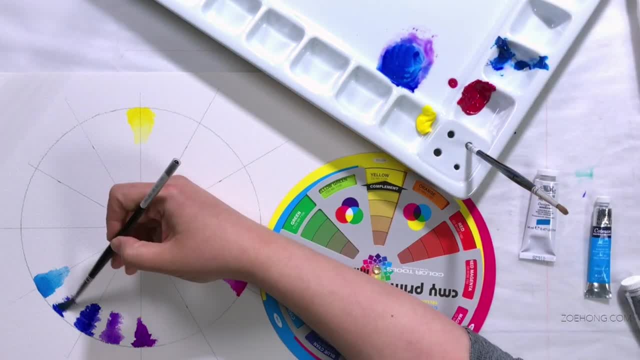 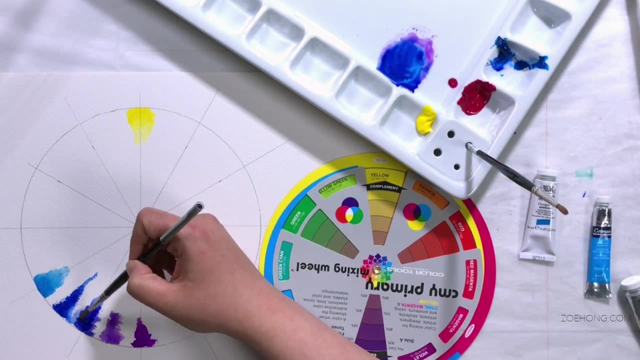 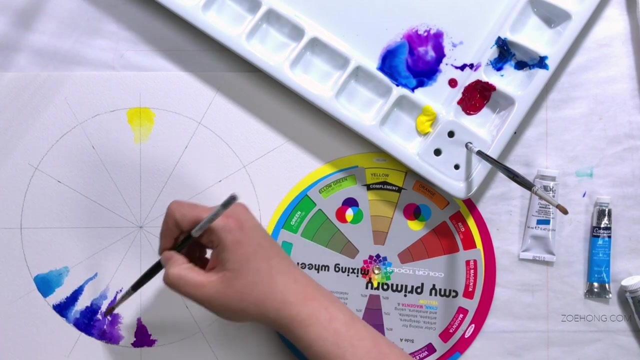 in the color theory series, But right now I am painting up some blues and purples, just mixing cyan and magenta together in different quantities, And the reason I have these like spaced out is it really helps figure out where to place everything, Okay, So 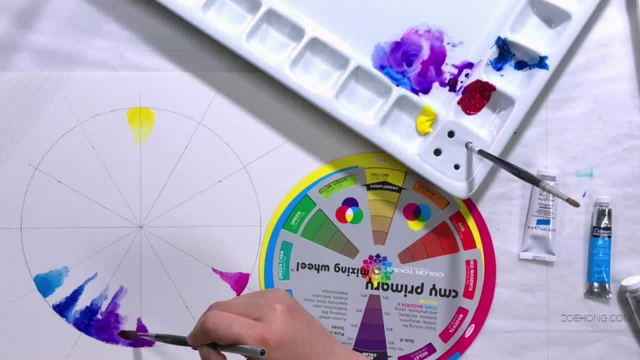 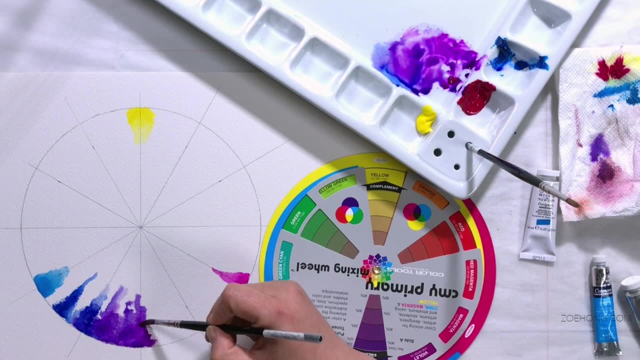 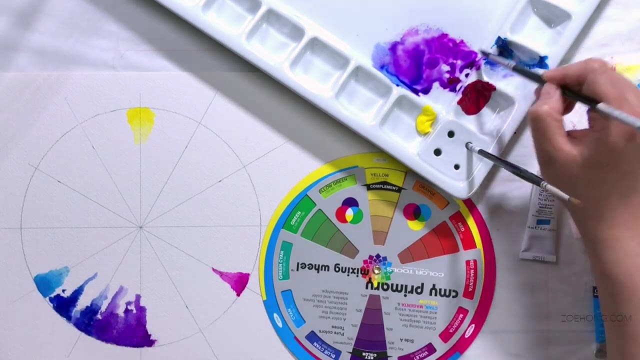 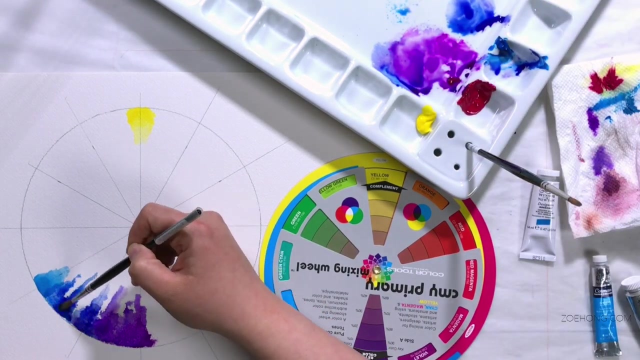 right in the center between magenta and cyan, I have that purple, that violet, and then I get bluer and more cyan as I go to the left And it's going to get more like red violet as I swing to the right. People think that painting is expensive or more expensive than 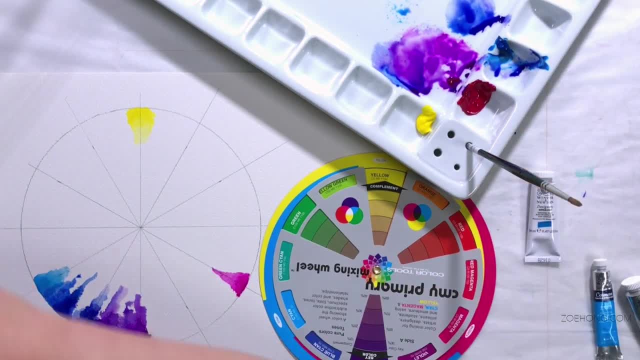 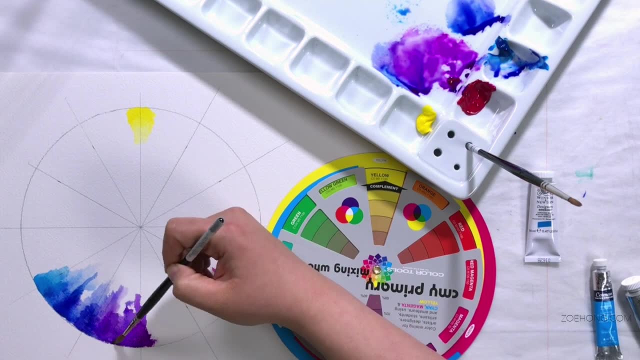 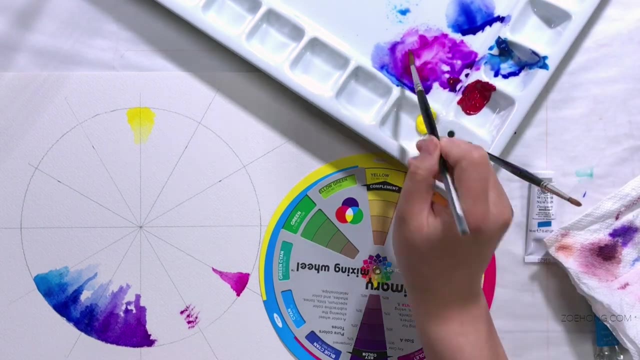 marker renderings. And I don't really think so. You know, I one of the the points of this video is to show you that you don't need a hundred million tubes of paint to mix up your painting A lot of colors with markers. you need a hundred million markers because I mean, there are a few. 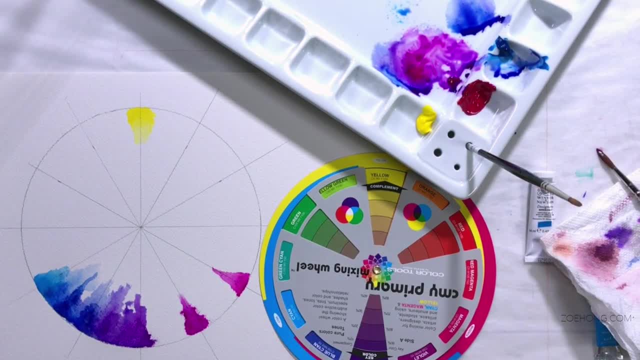 things you can do with layering markers, but I mean not anywhere near with the flexibility of paints. and the initial cost of getting started with painting is higher because I I advocate getting nice high quality brushes to begin with And the papers can be more expensive. 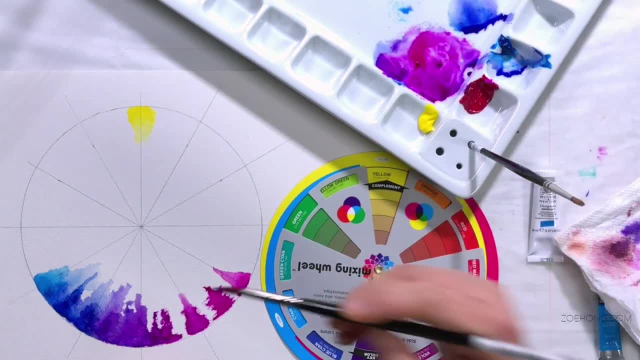 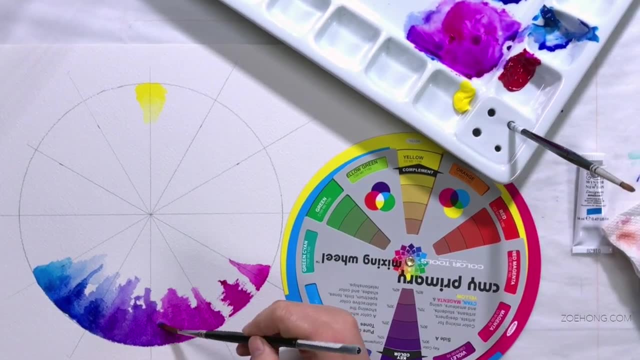 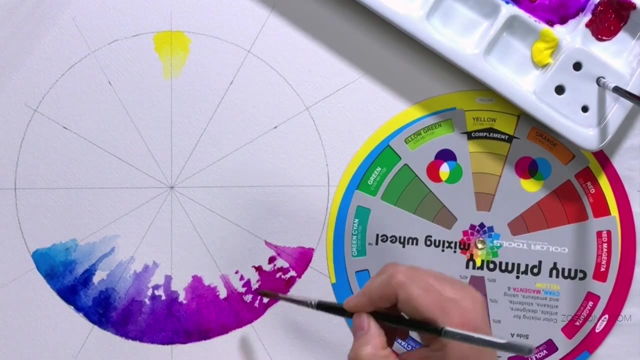 But these tubes of paint last forever and brushes, if you take care of them and you get good ones, they'll last you forever. I've had mine for decades, So in the in the long run, you know, it's not that much more expensive than markers, and markers can be really expensive because you 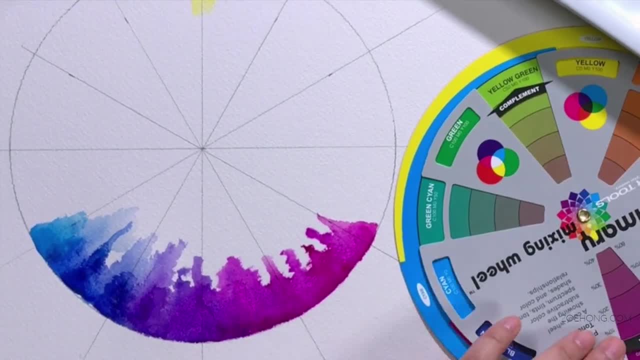 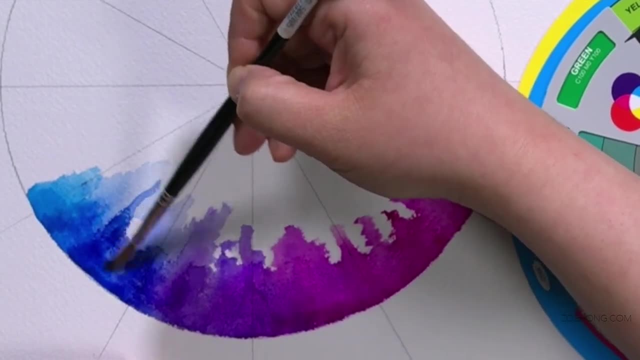 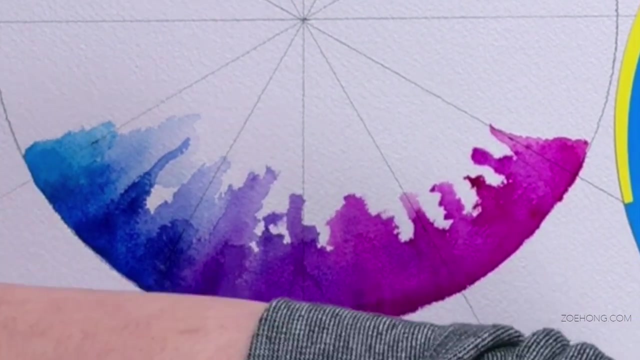 have to keep buying new ones. They dry out or you don't have the right color and an annoying teacher like Zoe comes along and says that marker does not match your fabric. You need to go get another one. So yeah, And you know I am going to continue with the cheap. 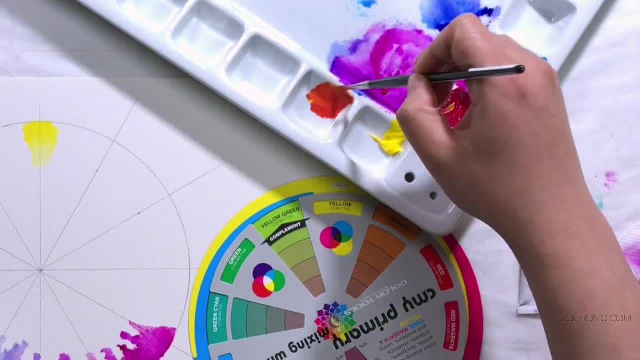 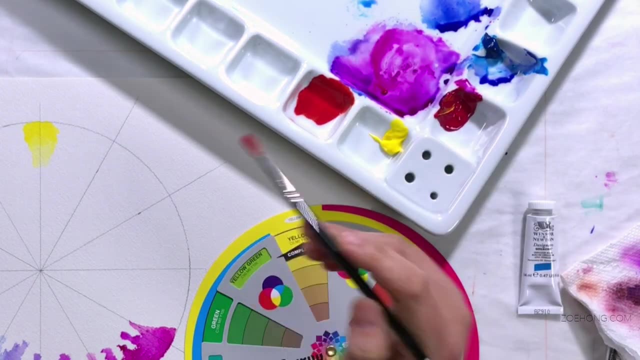 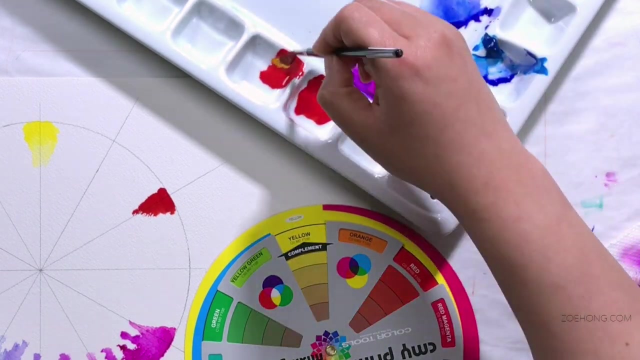 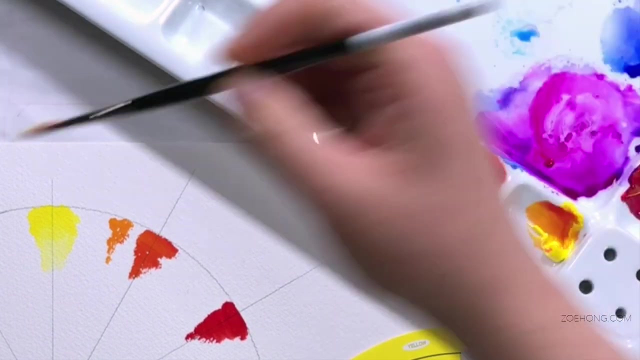 the inexpensive art supply series. I have a bunch of gouaches and watercolors purchased for that video series And, yeah, let's see if we can find some gems in that kit of things that I bought. And again, here I'm doing some reds and oranges just mixing magenta and yellow. It's all there's. 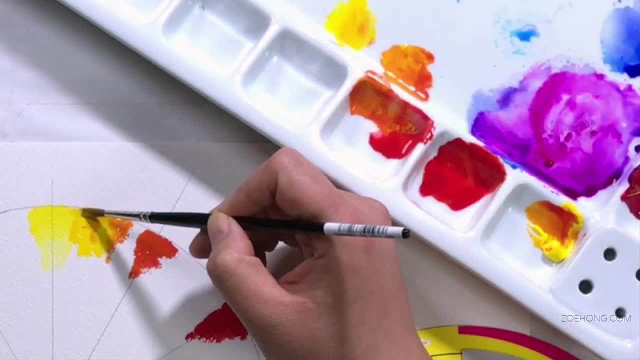 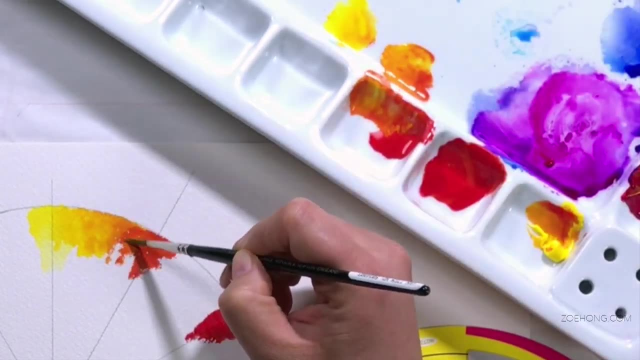 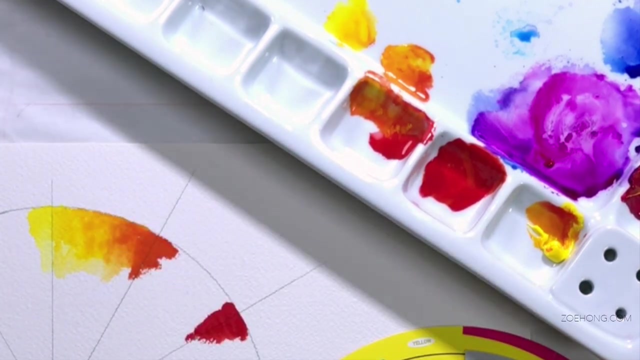 to it And you can see I can get a really awesome intense red. It's right in there in between magenta and yellow. I'm getting some really beautiful oranges and yellows in there. You might be thinking: so, Zoe, does that mean you only have like five tubes of paint? No, Okay. 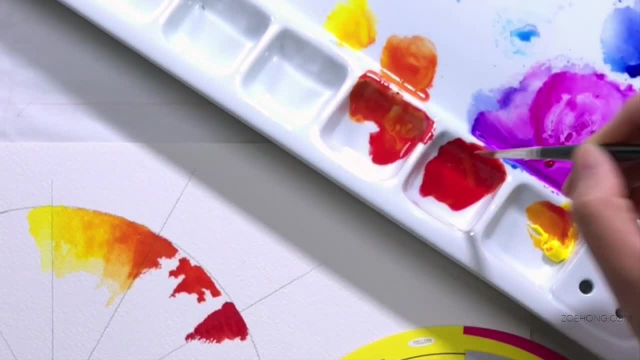 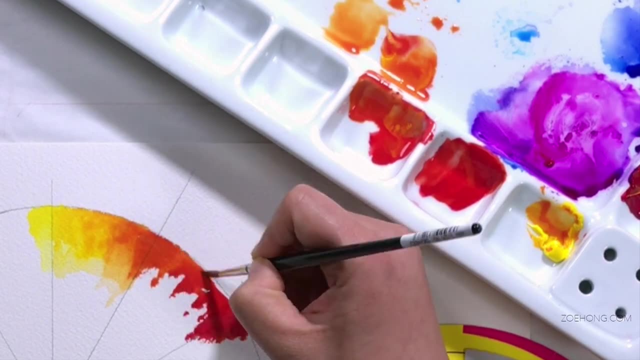 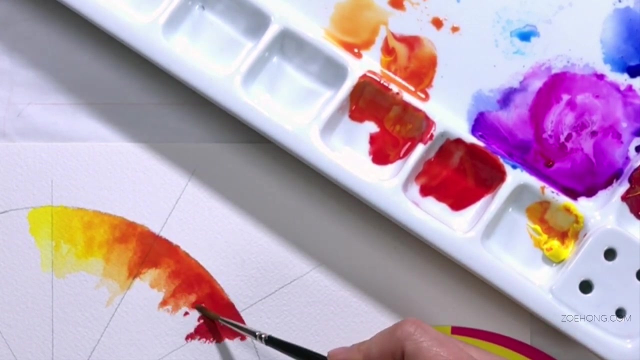 So, yes, I have cyan, magenta, yellow, I have black and white And, yeah, I do have a lot of other colors, because there are colors that I use so frequently that it's a shortcut. You know, I buy tubes of paint as a shortcut. I am going to show you how to make browns, and you know. 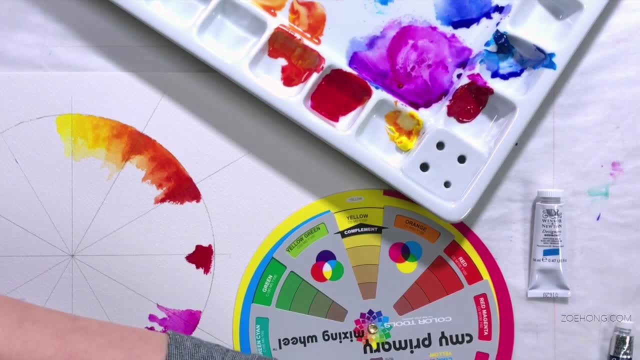 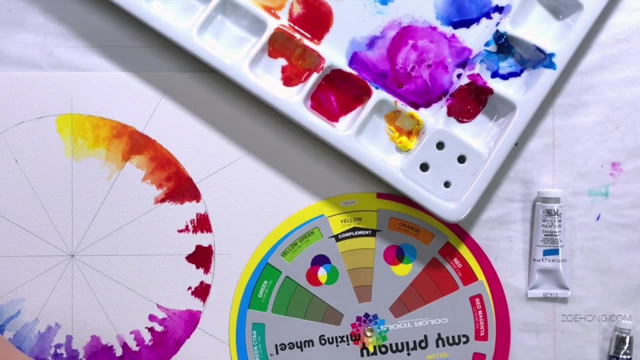 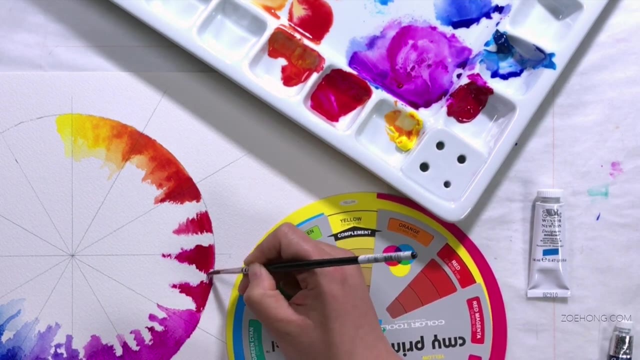 warm neutrals like olive green and stuff in future videos. But you know things like burnt sienna. I use burnt sienna A ton Okay, Because it's the base color for a ton of skin tones And you will see that if you. 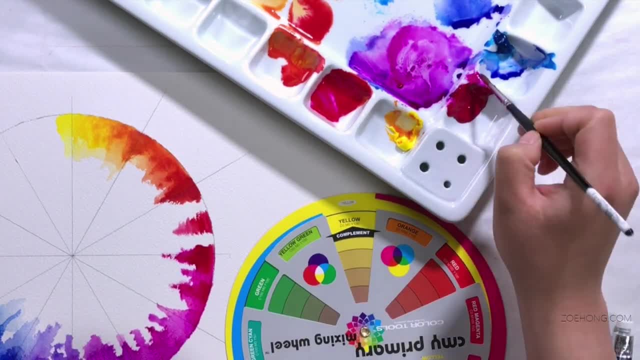 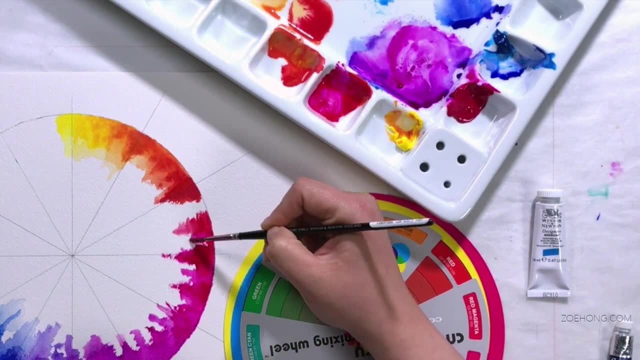 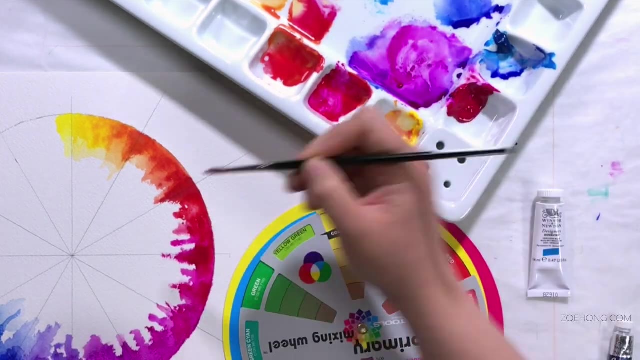 watch my skin tones video. So, because I use it so much, I buy burnt sienna and I use it as my shortcut instead of starting over from scratch. But what I recommend for, especially for those of you beginning painters, is to start with these three, And then you know as you keep painting. 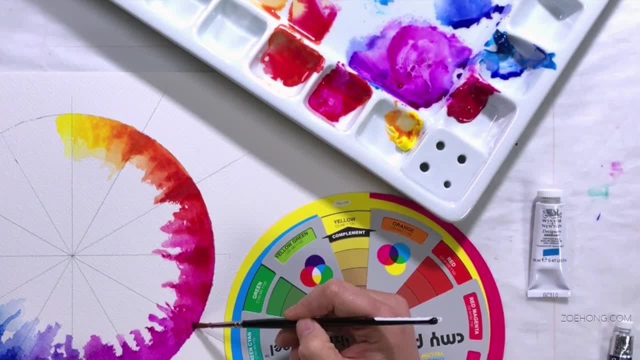 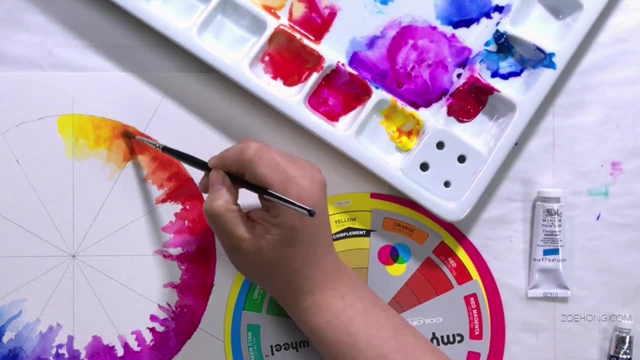 you're going to know what you need in terms of shortcuts. The point of this series is to show you: A- that you don't need all those tubes of paint. B- that you can get a million colors just using a few paints. And. C- most important. 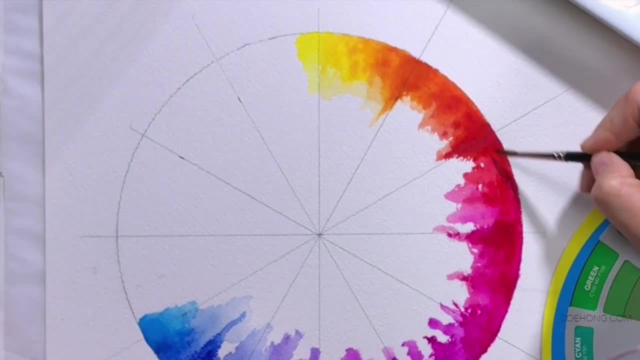 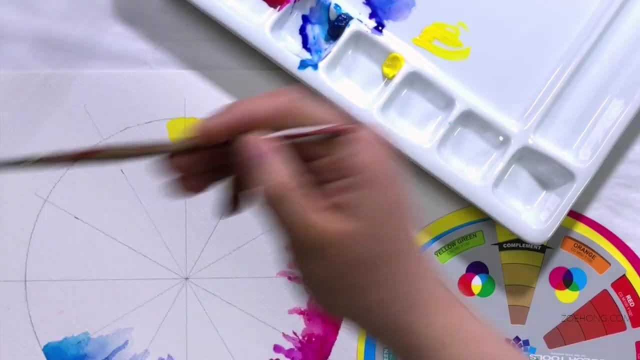 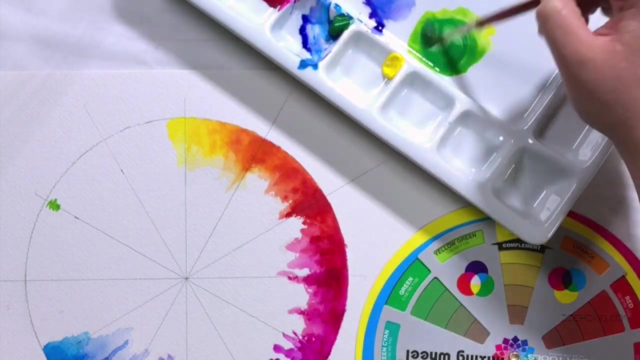 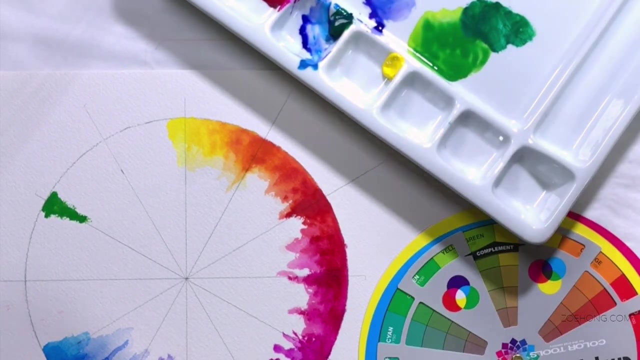 where colors come from, so that you know how to mix different colors to match your fabrics. or what have you, Once you understand the base, okay, like how did I get olive green? Well, I did was mix yellow and cyan And that makes a bright green. Okay, And you have different options. 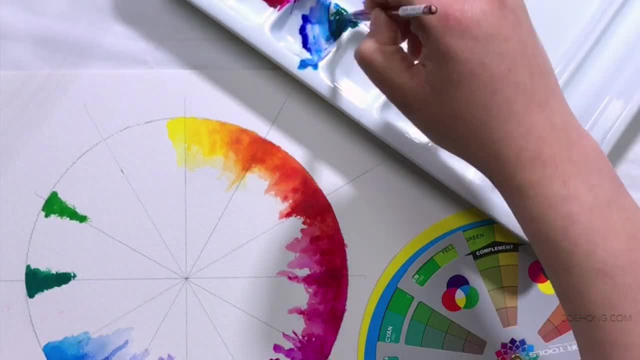 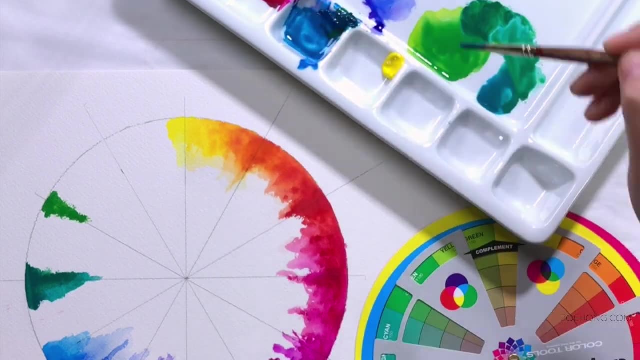 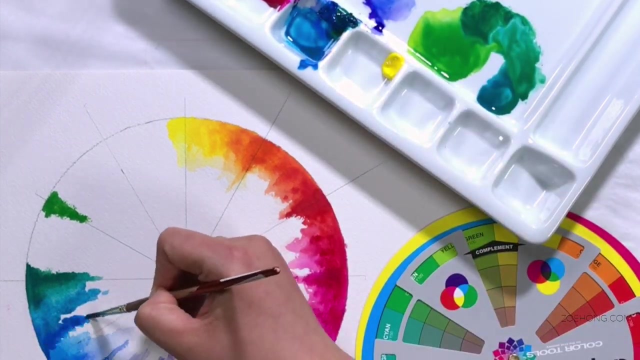 to make duller greens, like adding black, adding gray, Okay, And there are so many grays to choose from right. But I'm going to show you, through these painting videos, what it looks like when you add different grays and blacks to colors, so that you can understand where these colors. 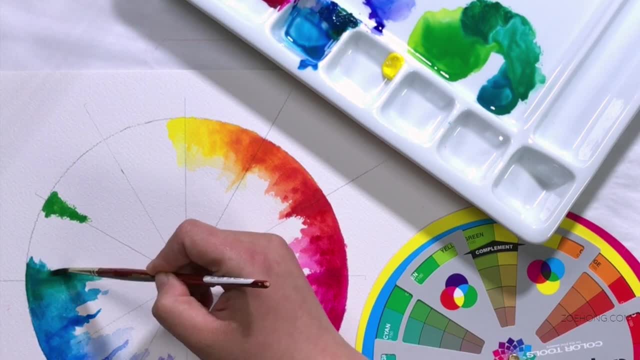 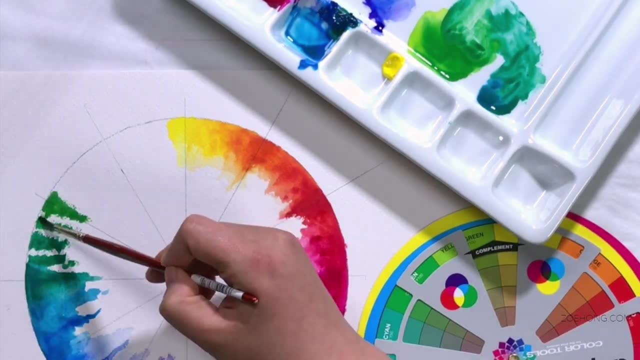 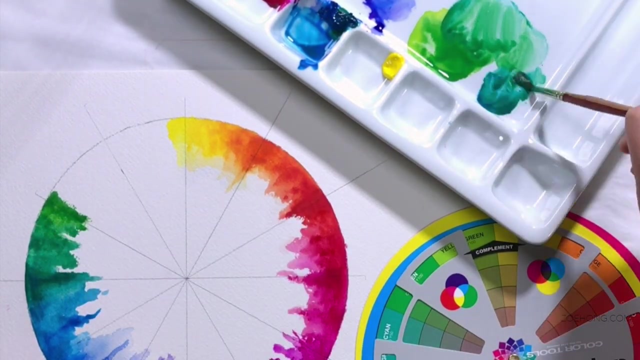 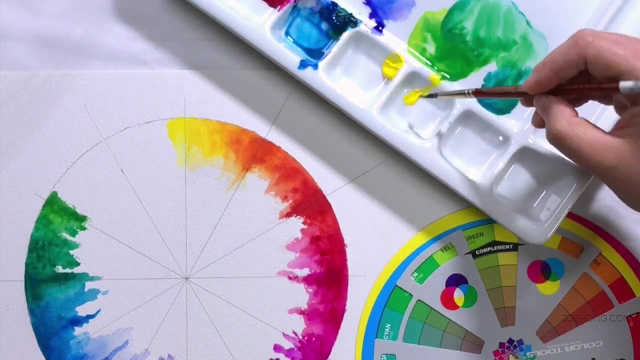 come from. So when you are trying to match that olive gray, olive green wool for your project, you know, oh okay, So I have my green now, And when I add black I get a different green, darker green than when I add gray Or when I add red to it. You're like: why would you add? 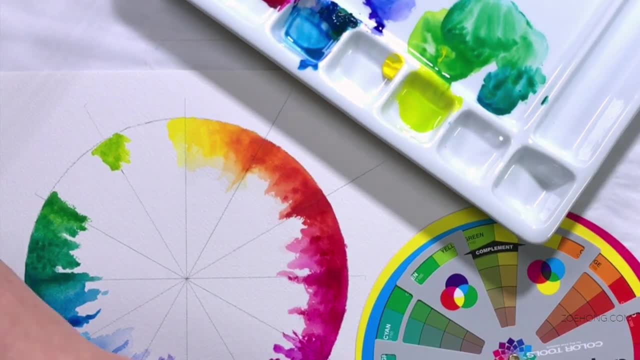 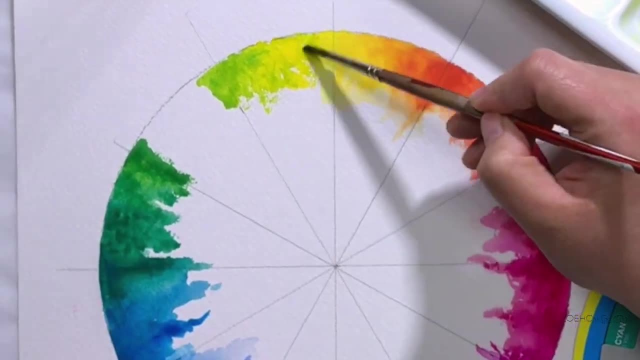 red to green, Because that dulls down the green. Okay, Adding opposites, your complement dulls down the color. I'm going to go over mixing up mutes in another video, But if you watched the first Color Theory Basics video you know. 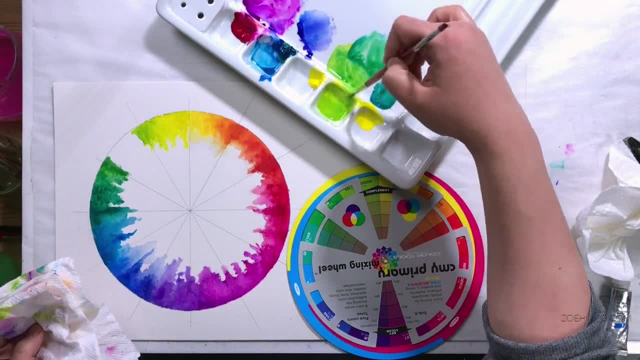 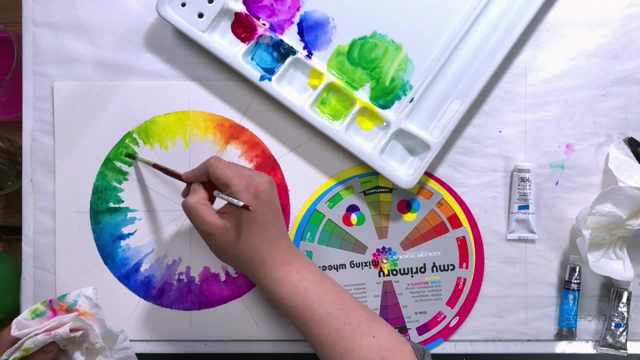 that mutes are when two opposites on the color wheel are mixed together to create browns. How do I get the green I want? Do I want to add black? Do I want to add gray? Do I want to add a little bit of red? Do I want to add gray and red? Okay, So I'm going to go ahead. 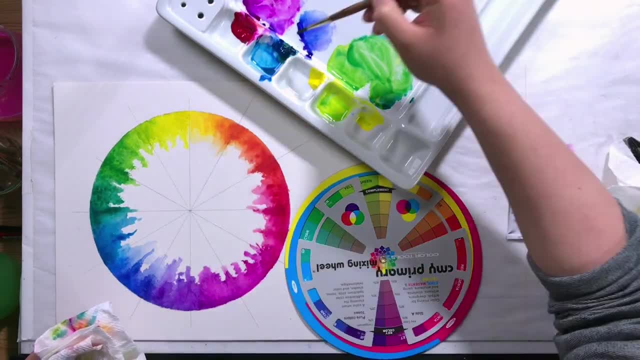 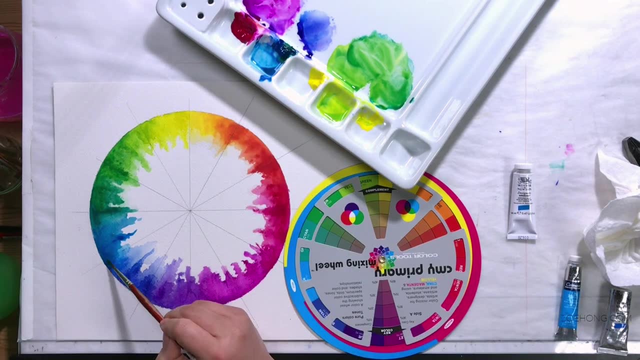 and I want to pick blue for the green, Okay. And then I'm going to grab my palette. I want red, okay. so that's kind of the goal is to like give you all the building blocks for what colors look like when they interact with each other, so that you can. 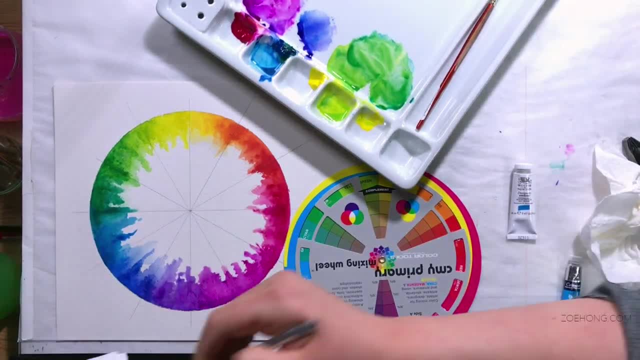 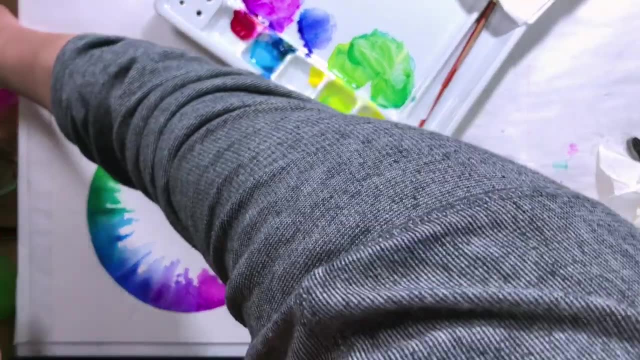 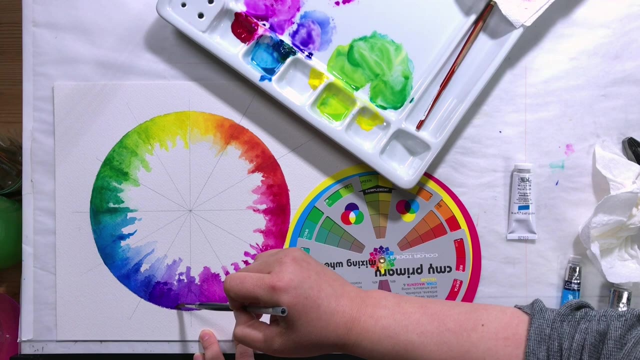 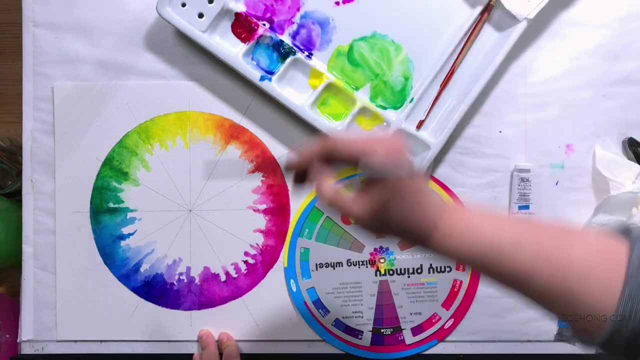 be more efficient at mixing all these colors yourself. now I'm just going in here and I want to show you guys, I want to show y'all like really intense color, so I'm just going in here and just adding more of the same color and making things as intense and vibrant as I can remember- the three elements of every. 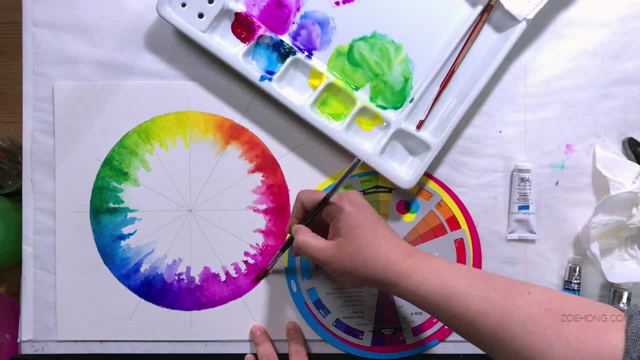 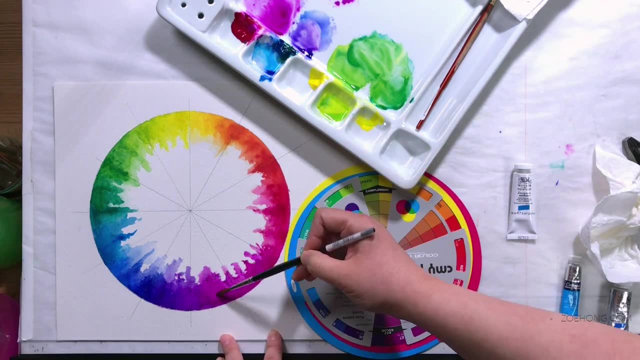 color, value, saturation and temperature. so I'm adding more of the color to make it more saturated, more pure, more intense. okay, as I mentioned before, I'm going to show you guys how to mix all these colors together so that you can see how much of a difference it makes. for temperature: is the warmth or the? 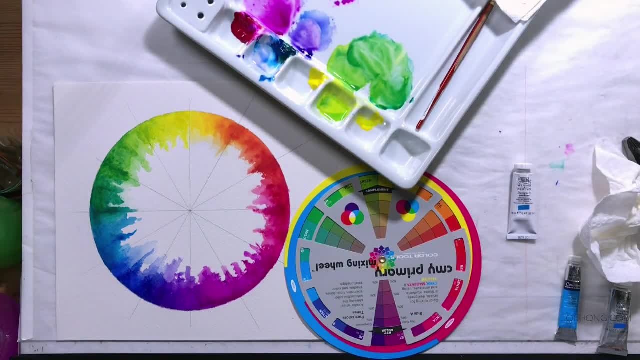 coolness of a color. so our warm colors are the yellows all the way to the red violets, and then our cool colors are from these greens all the way to the violets, and if it looks a little bit weird it's because at this point I'm 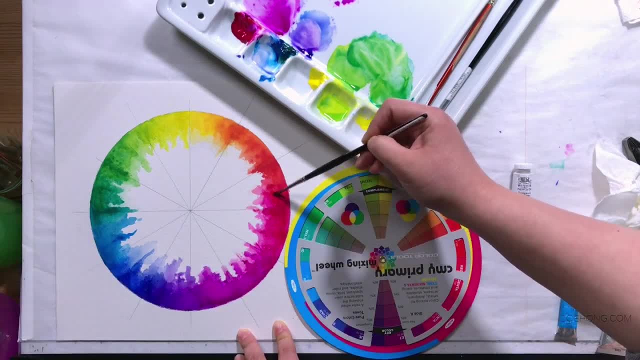 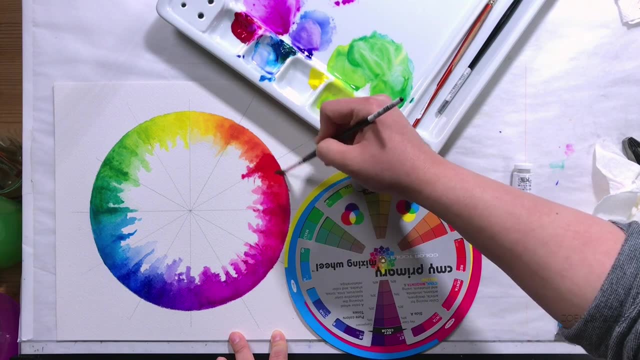 painting standing up so that I could kind of look at it at a different angle than I was before. I do that a lot like as a finishing touch, just to make sure that it looks good from some illustration. I do looks good from all angles. I'll stand up and kind of like tilt my head around, hit the like button. 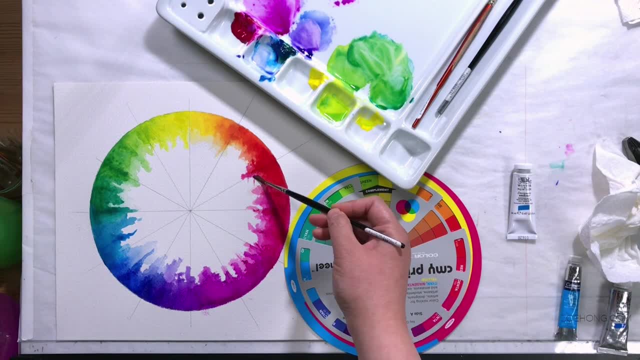 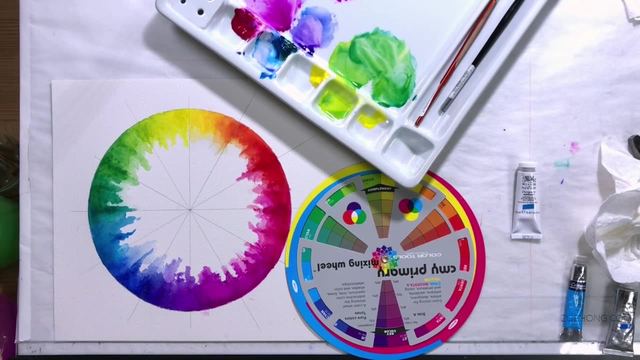 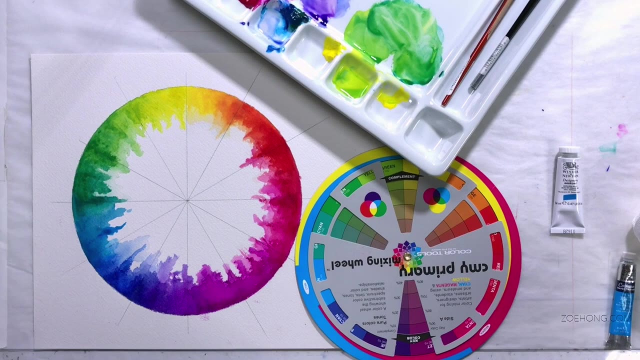 if you found this video helpful and let me know in the comments your questions and what specifically you would like to see in the color theory series if I haven't addressed them already in this video, and subscribe so you can alert for when I post more color theory videos. and yeah, go practice, mix up. some paints have. 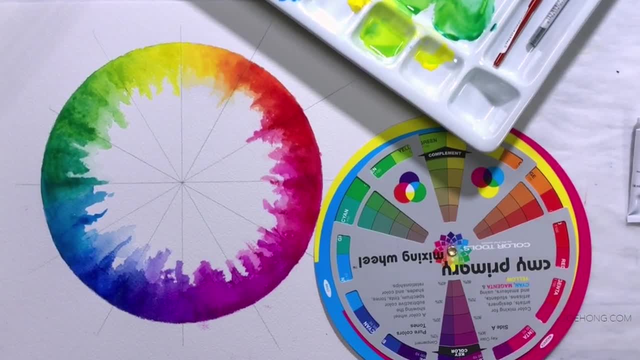 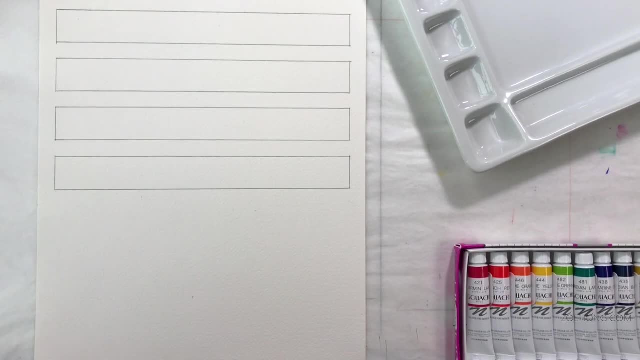 some fun. you meant things how you mix these colors, if that's something that helps you and I will see you in the next video. hey, hey, party people. this video is gonna be a twofer number one. we are going to go deep dive into the world of tints. 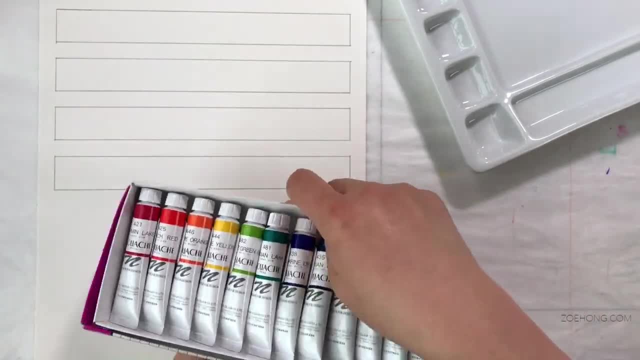 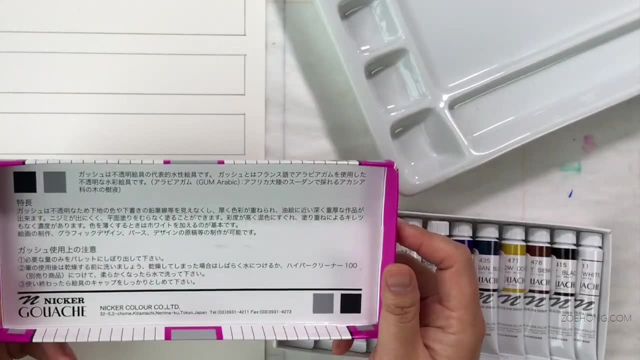 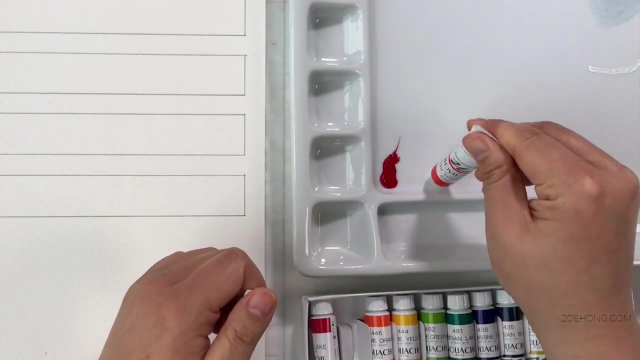 shades and tones. number two: we're gonna test out this new to me brand of gouache called knicker. it's a Japanese brand. as far as I can tell, they're made in Japan- maybe maybe not- and I got this set when I was in Japan last June- May and June- and 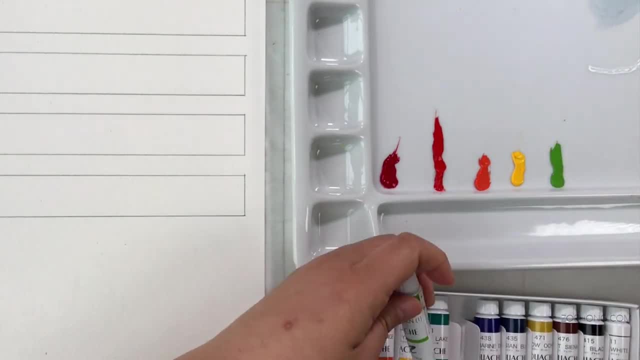 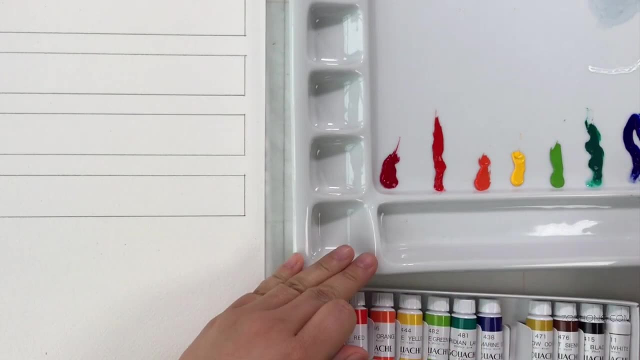 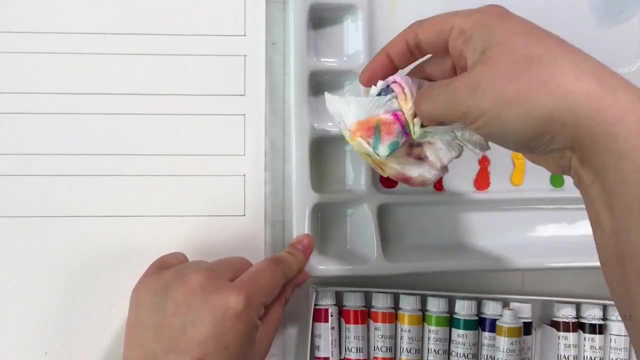 I have yet to test them. I kind of forgot about them. good job, Zoe, good job. and I was cleaning and sorting and stuff and then I found them and I'm like yeah, so anyway, I know I'm the worst. wow, this yellow ochre is like dripping stuff. 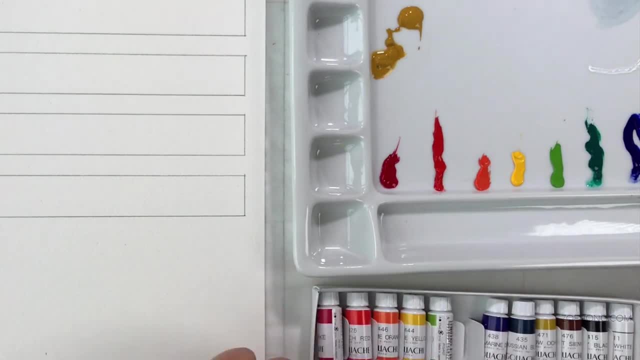 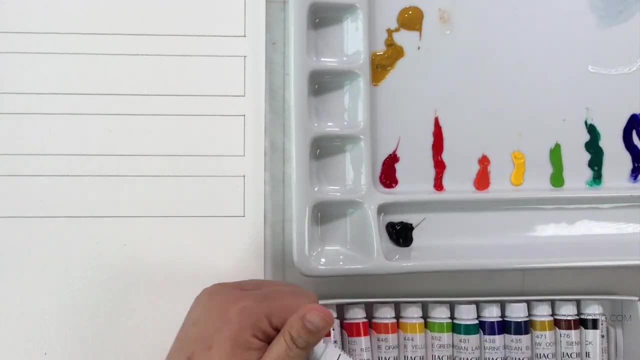 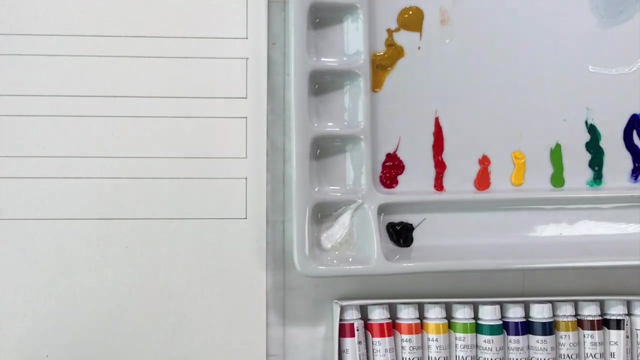 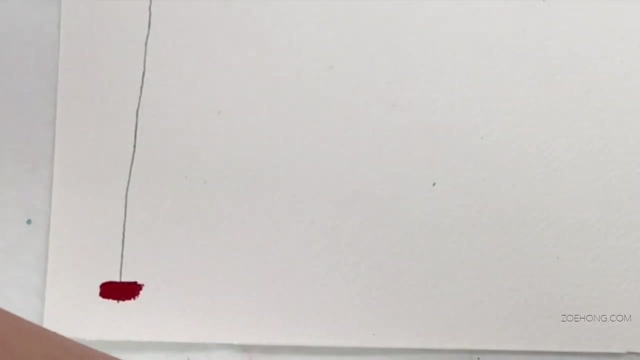 all over the place. that was pleasant anyway. yeah, so we are going to play around with tints, shades and tones and play around with these washes. so this will be a color theory study meets product review video. whoop, whoop, I am using. what am I using? arches watercolor paper. it's my favorite brand of. 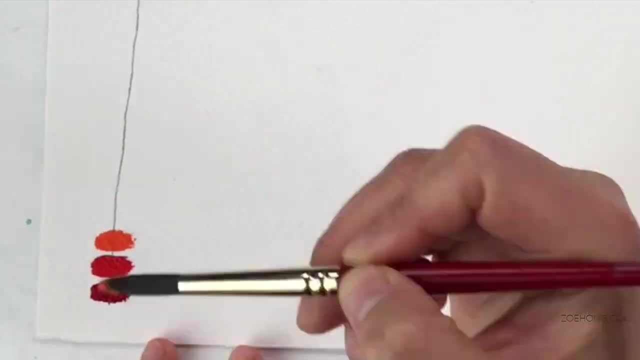 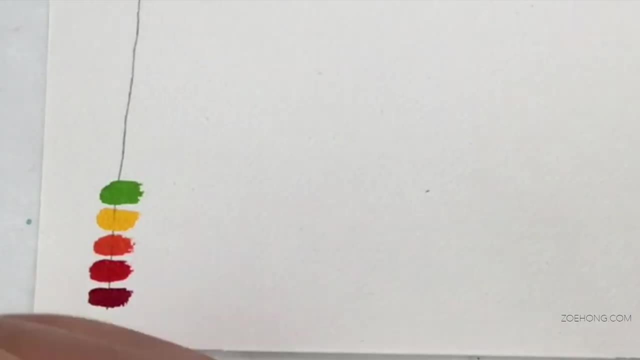 watercolor paper and right now I'm just testing the gouache opacity. I just drew a line with pencil and I'm laying down bits of each color as opaquely as possible and you know, for the most part you're not gonna get it to cover pencil, except for your darkest. 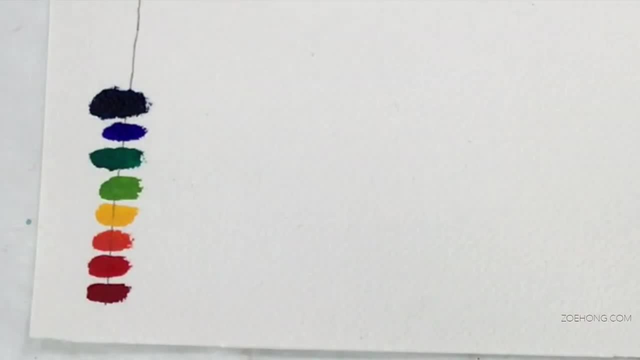 colors like this is Prussian blue I'm using right now. yeah, that'll cover the the lead. but you know I'd be very surprised if the yellow and the orange and similar light colors covered up the pencil. but you can see it covers some of it, So you can kind of see. 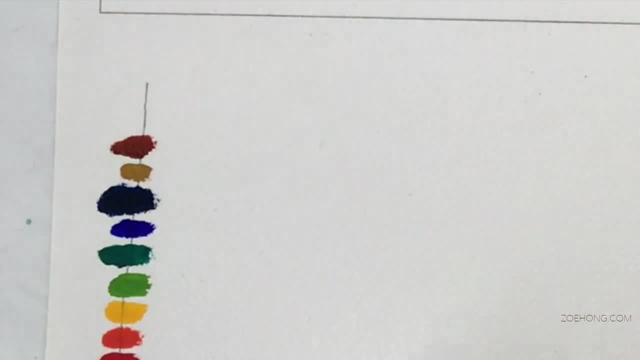 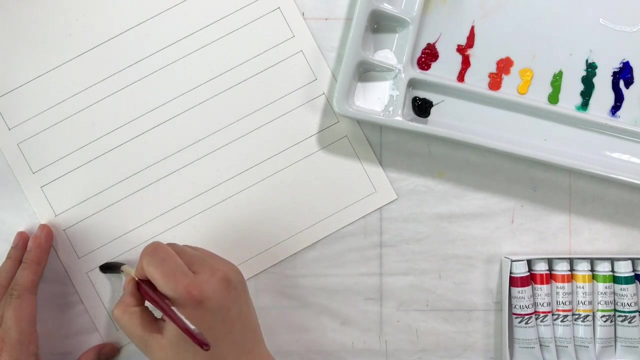 the opacity there And I imagine if I went back and put in a second layer I would be able to cover it. But I always work under the supposition that gouache is not going to cover pencil and I work around that when I'm painting. Tints are color plus white With watercolor there are two. 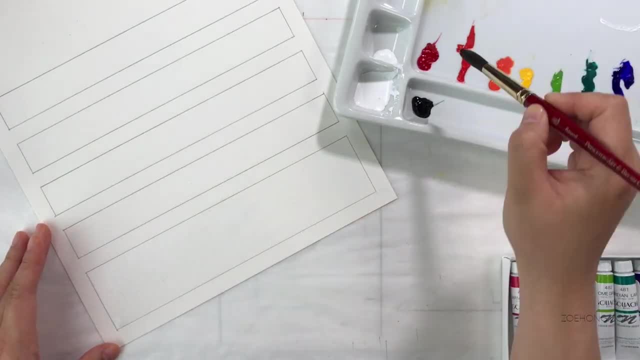 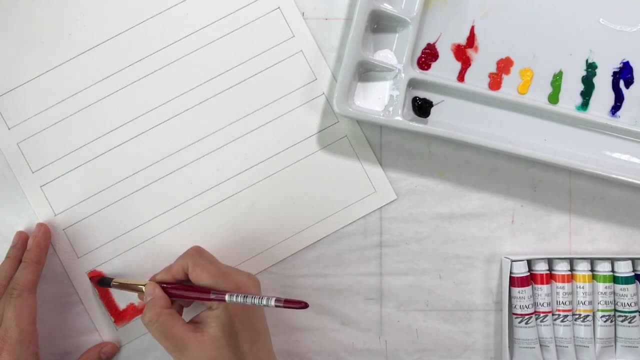 ways that you can create tints. You can add water to your color or you can add white to your color. Right now, I am using the French red, which is a really nice red-orange shade, And I am just using wet-on-wet technique to create tints. Now, wet-on-wet technique is wet. 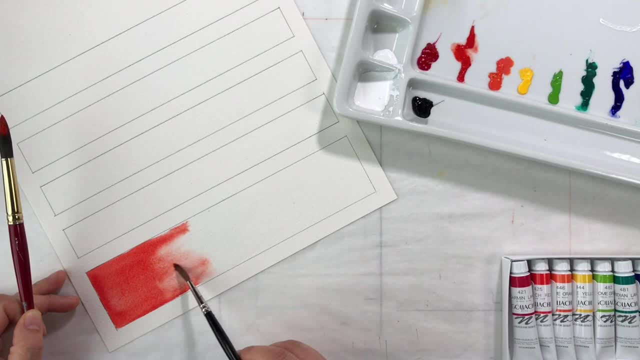 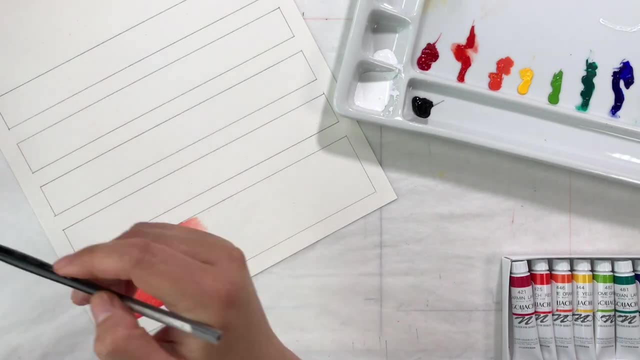 things on top of other wet things. So what I did was I just laid down some water on my paper and then I added the paint before the water dried. The thing with wet-on-wet technique is just because you can't see the initial layer of water doesn't mean you can just put water. 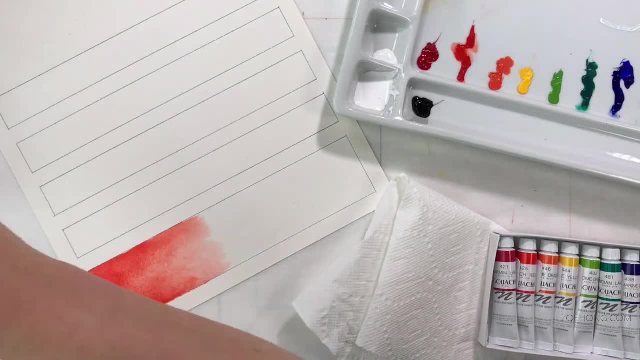 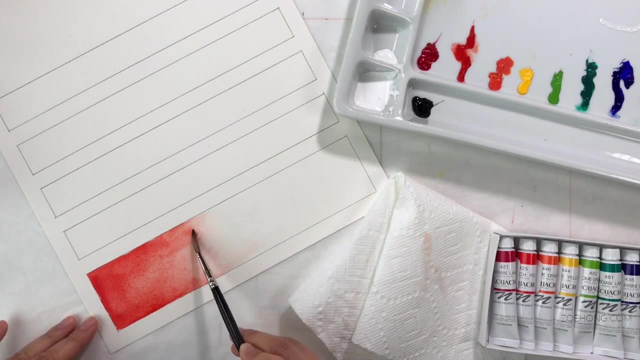 anywhere, Because the paint will go wherever the water was is right, And so you have to limit your water to where you will eventually want color later. Okay, so I limited it to the pencil box that I drew, And then I put my paint, And I'm having a good old time here. These are actually. 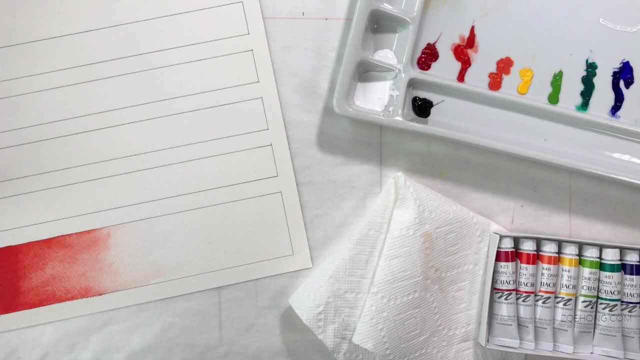 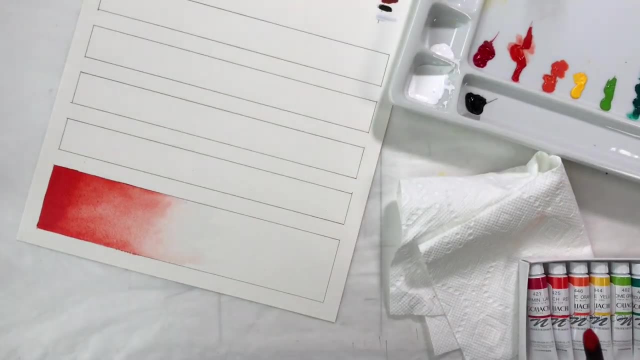 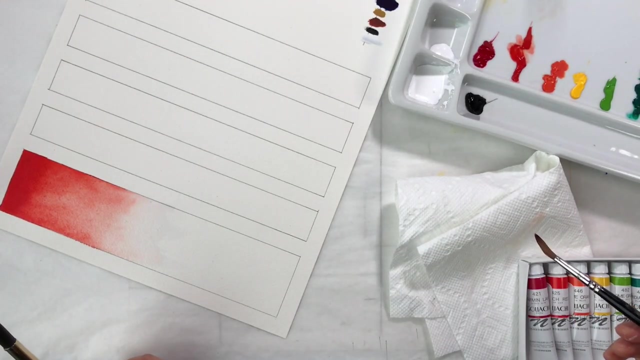 my favorite kind of videos to shoot These sort of like relaxing kind of inconsequential painting things. I have a lot of fun with these. The other way you can create tints with watercolor is to mix the color with white. The tint that. 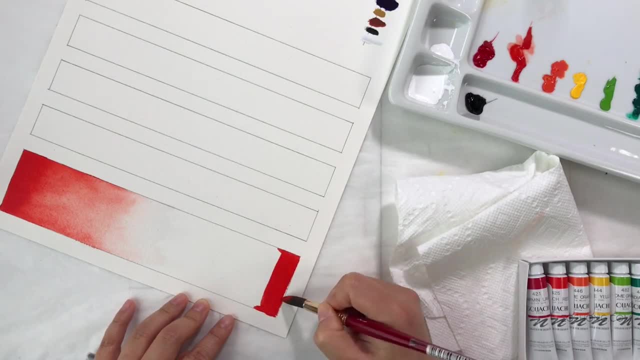 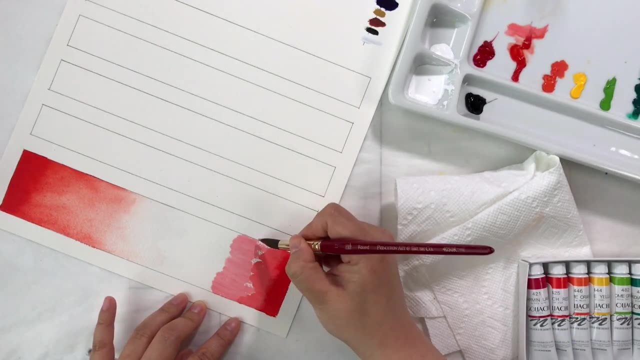 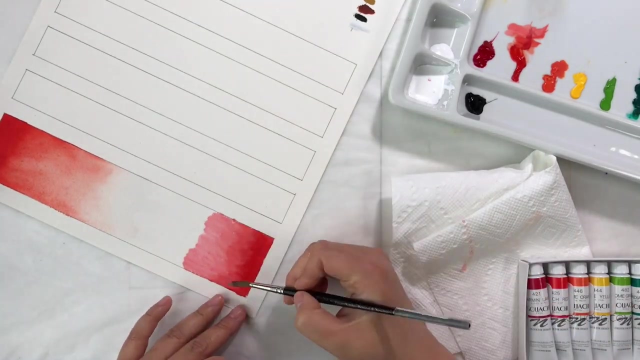 you get. the paint color you end up with will depend also on the kind of white you use. The white that I'm using is this: you know, the white that came in the set, which is zinc white And, as you can see, it is a tiny bit on the cool side. Do you see how? 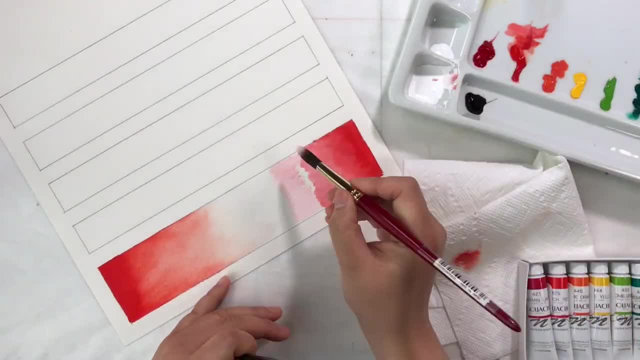 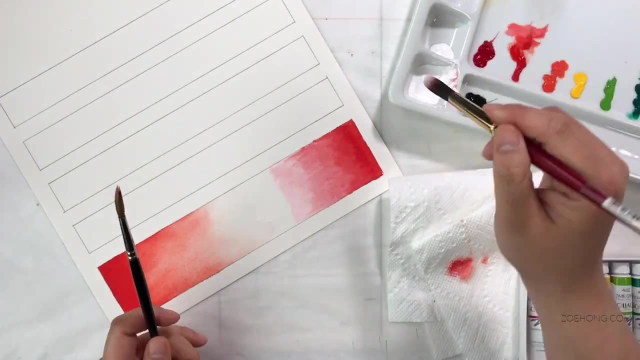 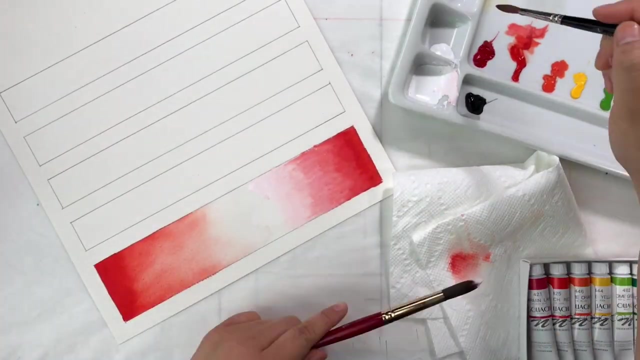 it is making the red orange a little bit cooler tone than when I was just mixing the red orange, the French red, with water And you can see the other half of the bar is a little bit warmer red oranges. You're going to see me do this kind of weird thing where? 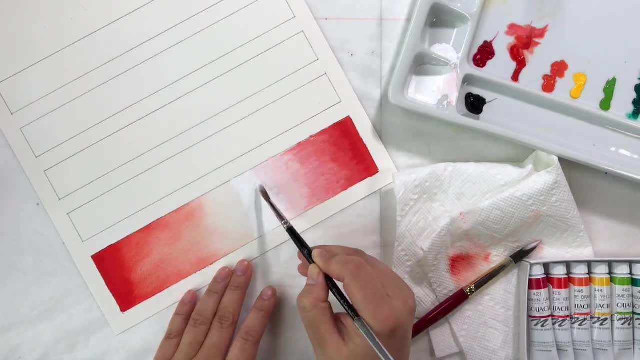 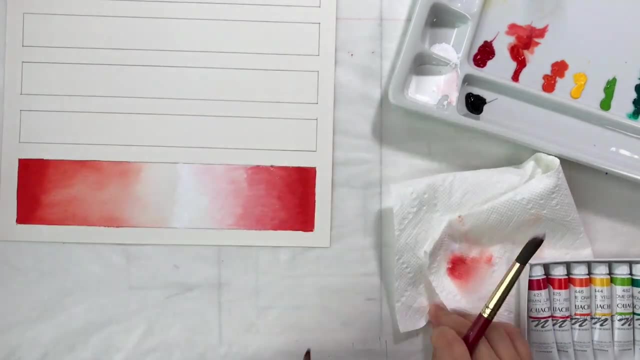 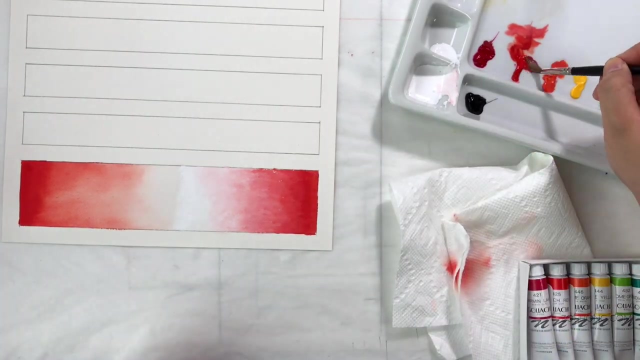 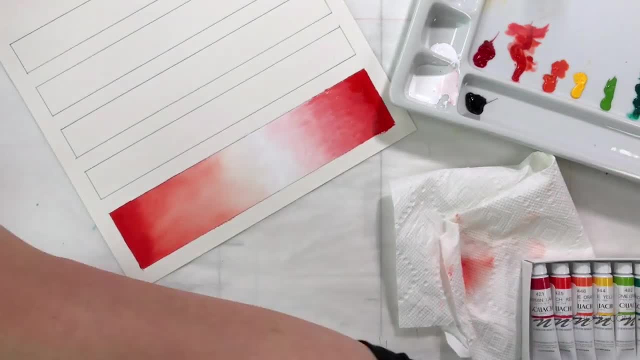 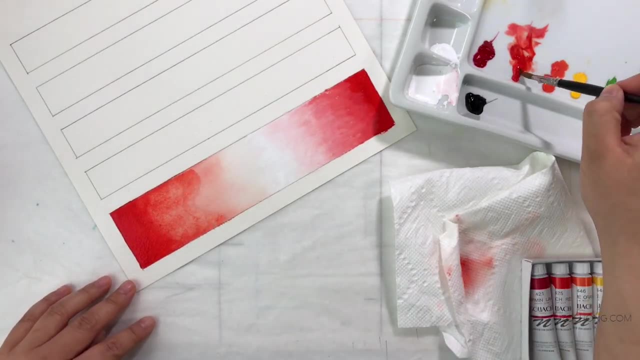 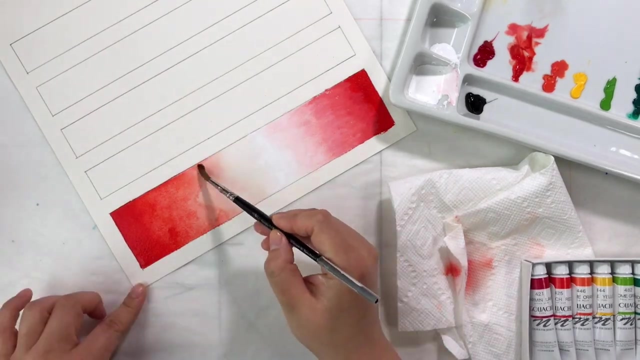 adding paint separately to my paper and then mixing it on the paper. So, yeah, the zinc white that this kit has, it's a little bit on the cool side, which isn't bad. It's just something that you need to be aware of so that when you're working with it you know that helps you. 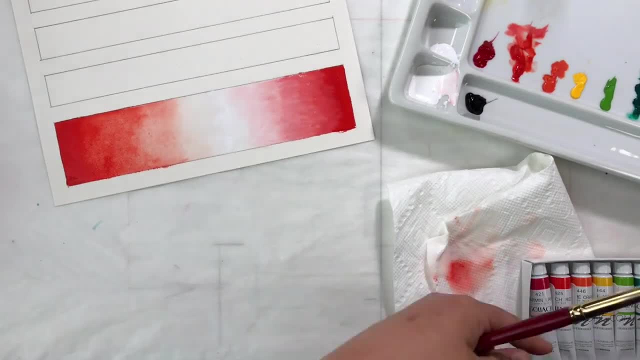 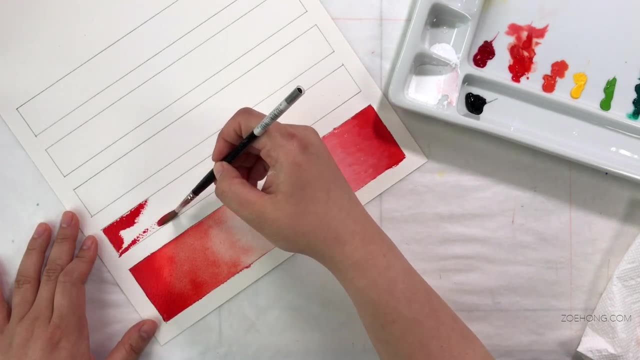 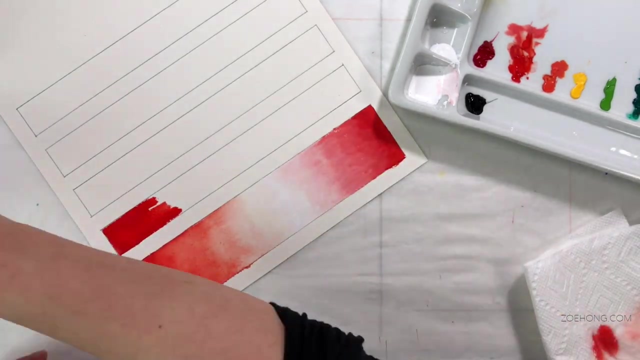 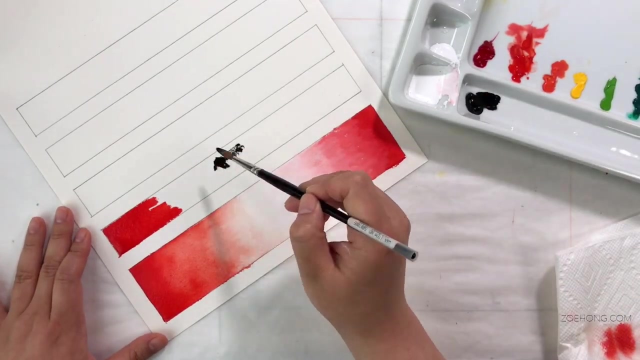 make informed decisions on paint mixing. Now we're going to paint some shades, And shades are color plus black, And the black I have in this set is ivory black And, just like whites, you know, blacks have their own coolness or warmness to it, And you know. 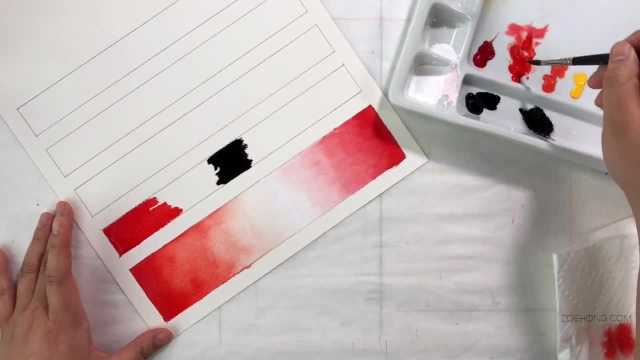 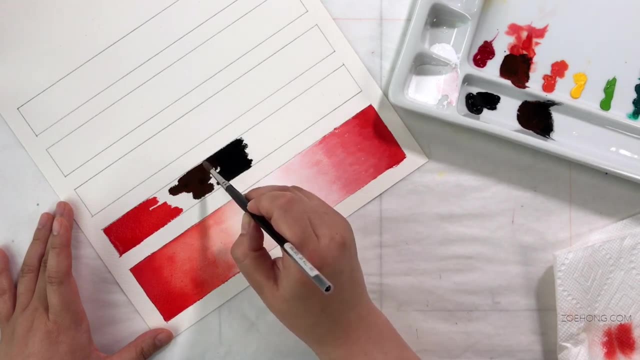 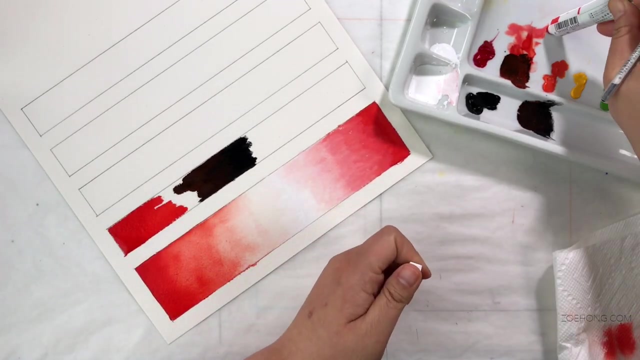 the Winsor & Newton set of gouaches. they have jet black, ivory black, lamp black. And you know every brand has their own way of naming things. You know one brand's ivory black is not the same as another brand's ivory black, So keep that in mind when you're shopping. But color plus black. 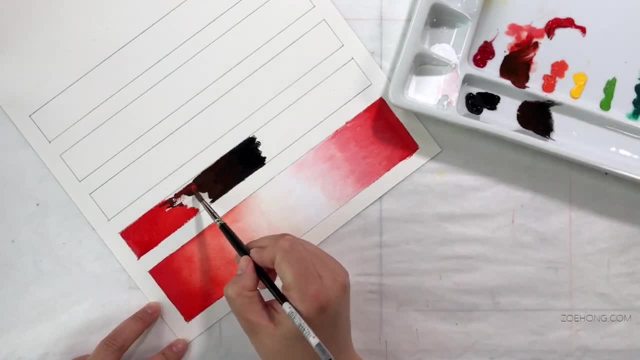 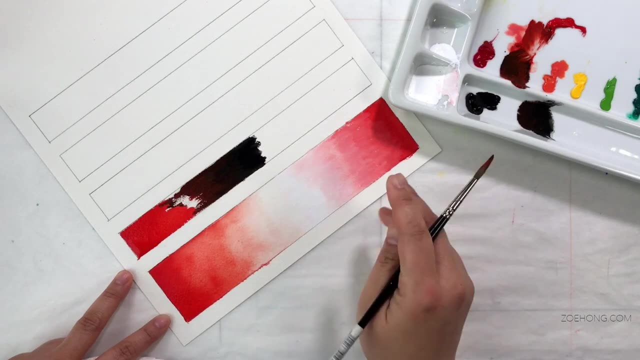 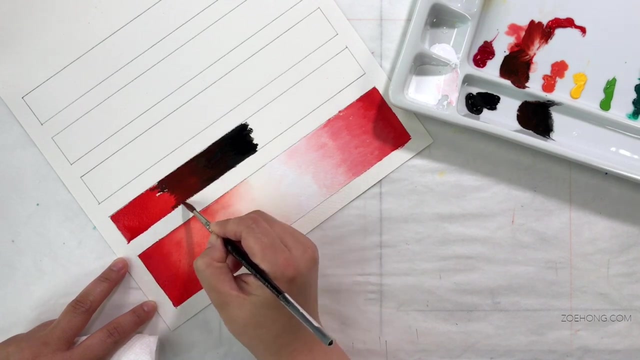 So again, I'm using the French red and mixing it up with black. When I'm reaching to my left on the screen, that means that I'm reaching for my water jars. Normally I would have the water on my right hand side too, but just kind of my studio setup right now kind of makes 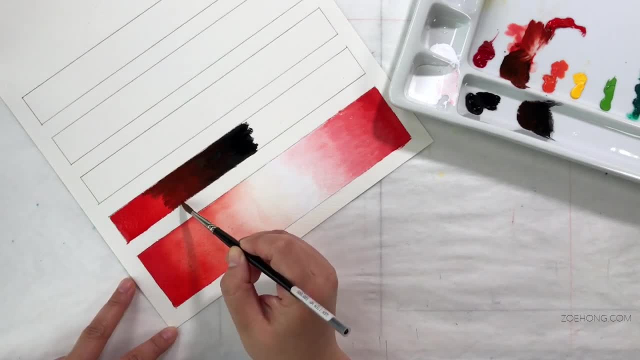 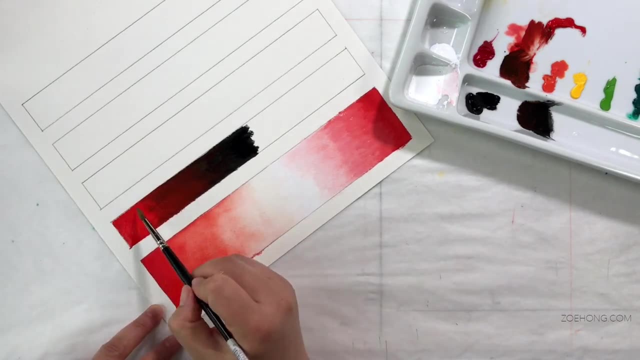 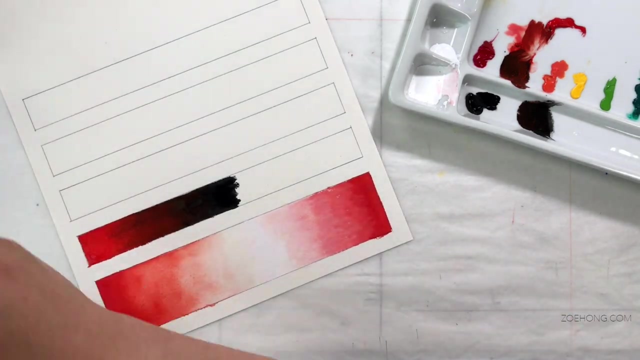 things difficult. Spoiler alert: I am really enjoying these gouaches. At this point, I remember when I was painting, you know, because this is my first time playing with them. I remember at this point I'm like: huh, I think I actually like these better than the Holbeins. So, if you recall, 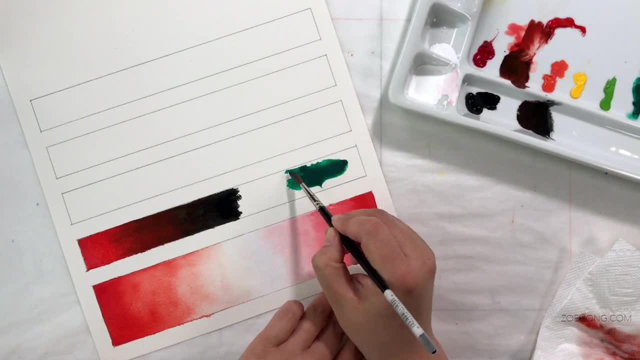 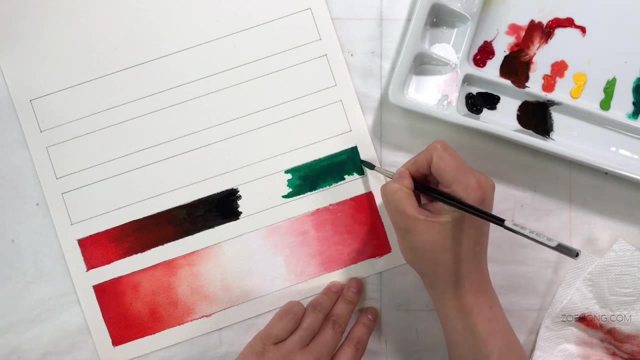 if you watched my Japan haul from last year, I bought several sets of gouache tester sets And I bought the Holbein and I've been testing. I've used them a lot. I really enjoy them. But now that I'm testing out this brand, the Knicker brand, 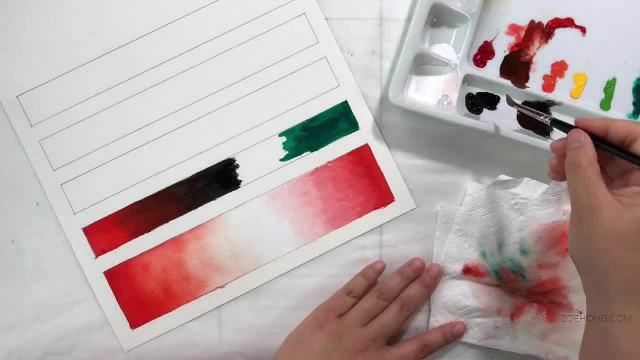 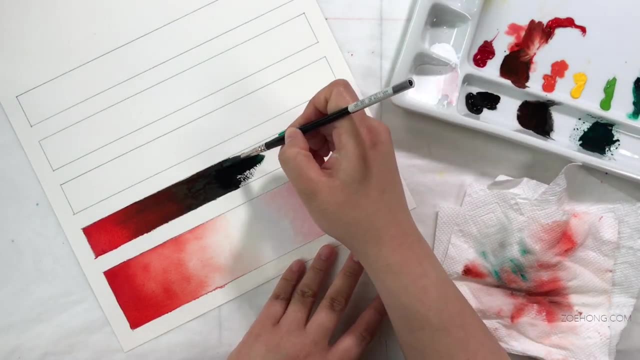 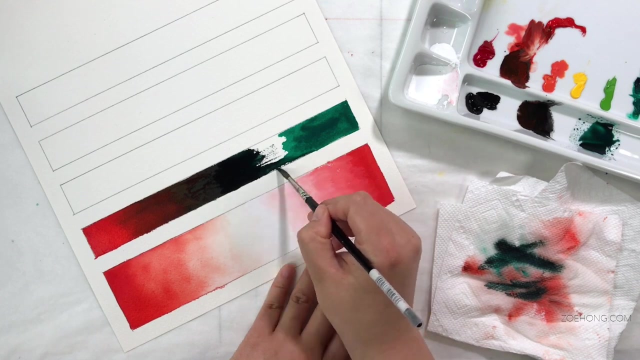 I really like them. I like them better than the Holbein, I think, a little bit Like the Holbein has like a touch of plasticiness to it, whereas this doesn't Okay. This actually feels more like the Winsor and Newton, And I might like that more because I'm just used to the Winsor and Newton. 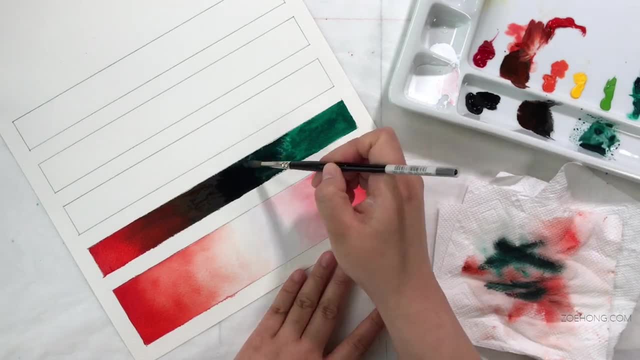 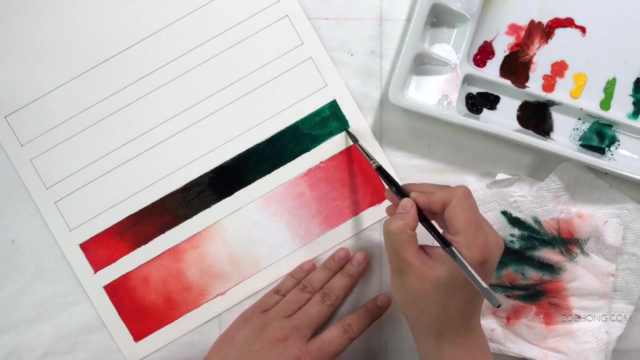 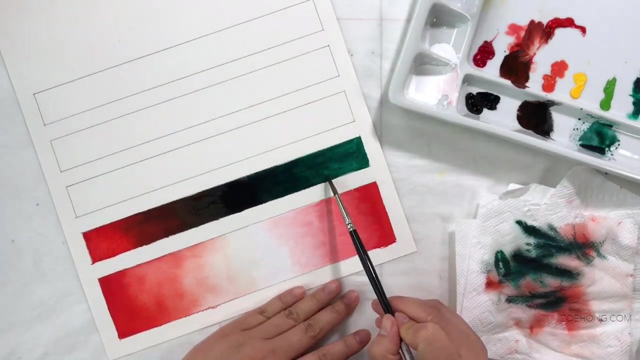 but these work really well. Right now, I am using What am I using? Viridian Lake, which is this nice blue green color, and creating shades with it. I'm doing these examples for you so that you guys can get a starting idea. 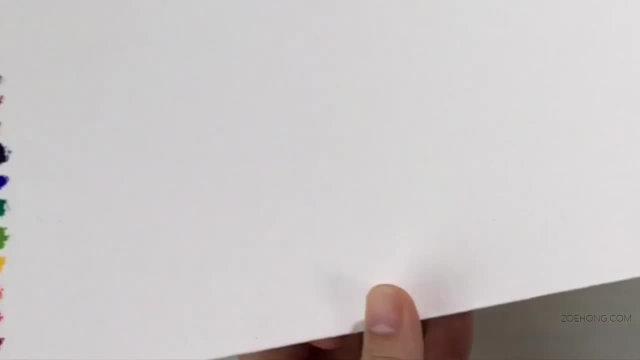 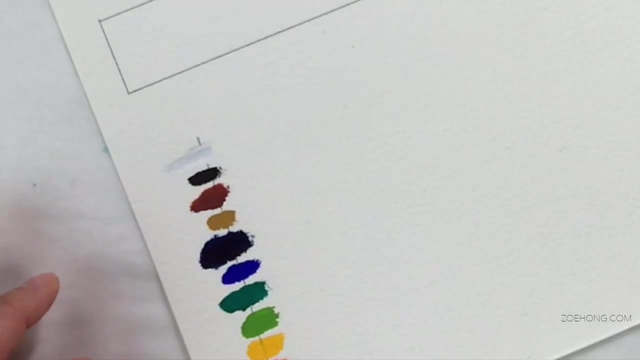 what shades and tints and tones look like and how they compare to each other. but please do go through your own paints and start mixing up your own tints and shades and tones, all right, because you know you have different blacks, you have different whites, you have different colors. 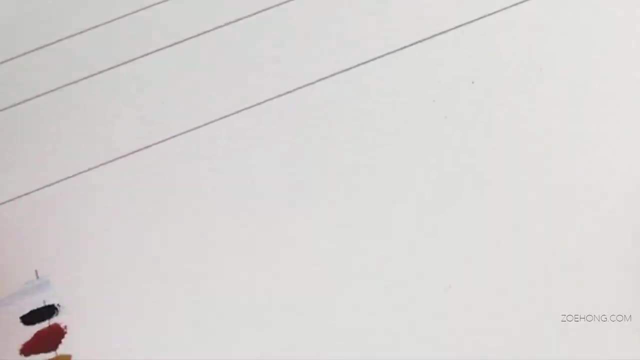 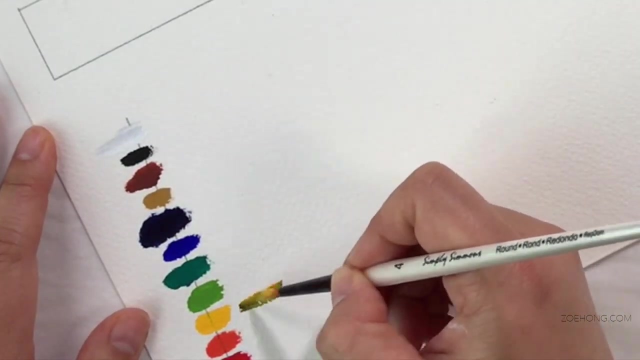 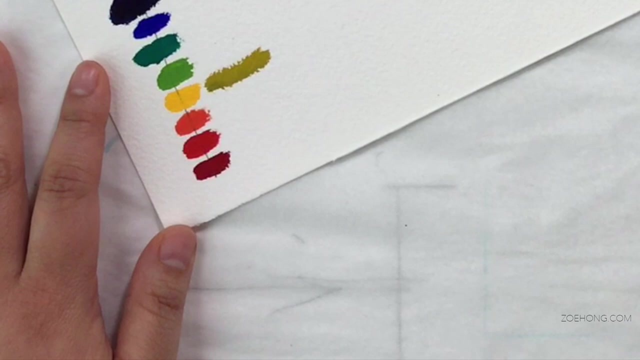 they're all going to look slightly different, but it's up to you to explore and examine what adding different colors do like. this is just a little bit of that yellow, the chrome yellow, with the ivory black, and because the ivory black is a little bit on the cool side, it's starting to 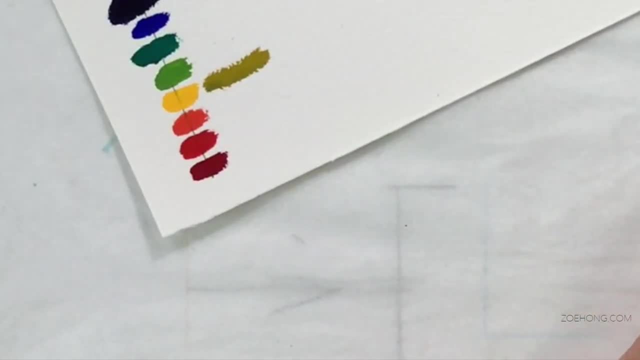 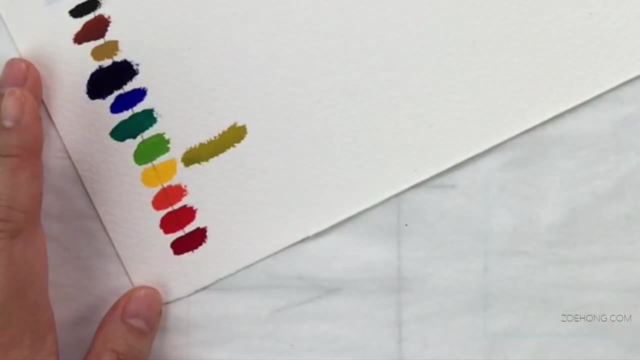 turn my chrome yellow a tiny bit green as I create shades, and these are the kinds of things I want you to see, and I'm going to show you how to do that in just a second. so I'm going to show you how to observe with your own paints. it's like: oh, when I add this black, does it make it cooler, warmer? 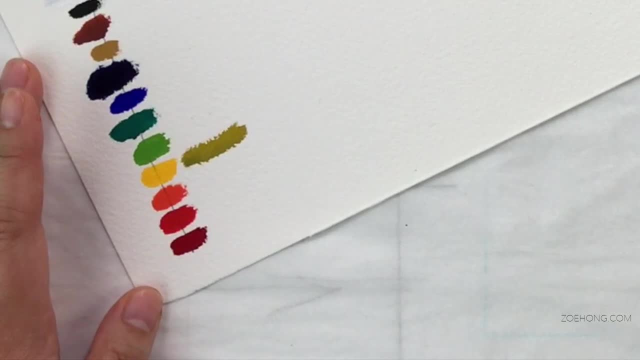 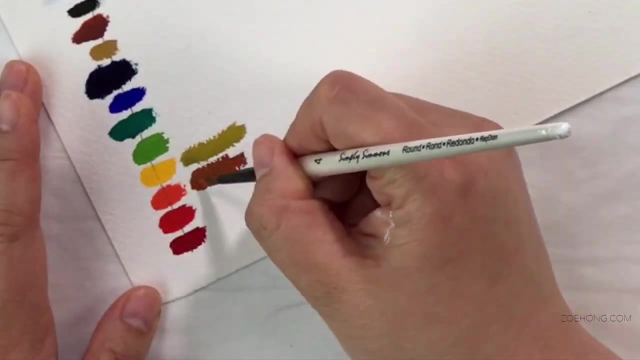 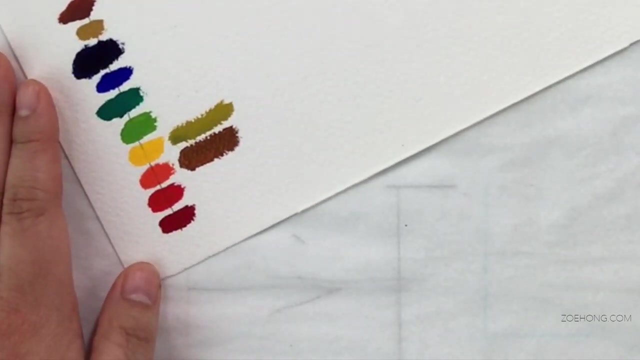 neutral? do I not even notice? do I need more practice looking at colors? probably, and here I am mixing orange and black and it's starting to look brown. yes, that is kind of the basis of: brown is orange and black is a good place to get started. this is the: the knicker chrome orange with the. 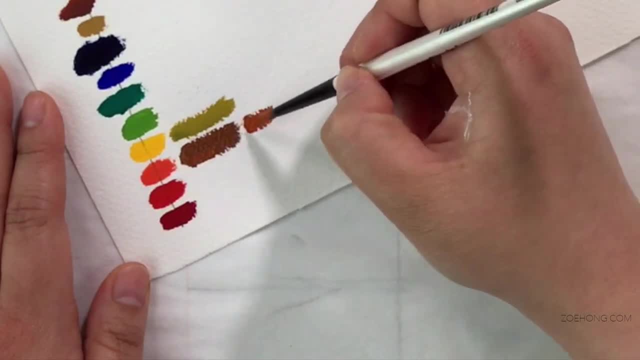 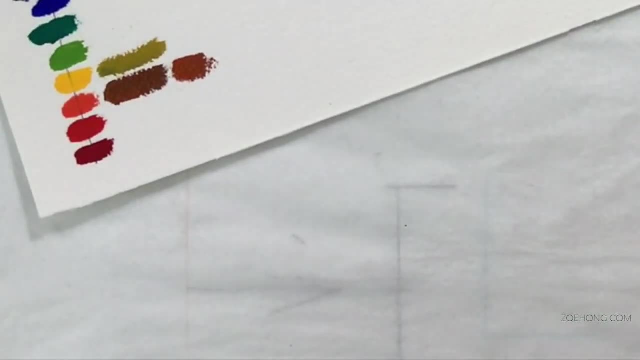 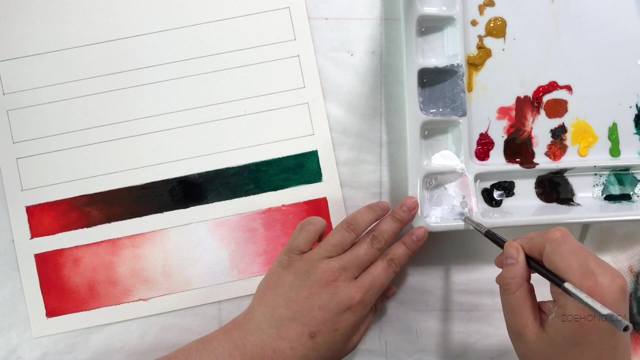 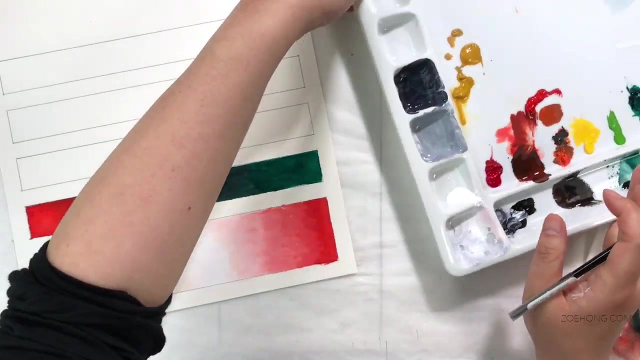 ivory black. here's the same orange with a little bit less black, a little bit more. it's not quite pumpkin pie. pumpkin pie is a little bit more golden right. and now I'm mixing up three different grays to play around with tones. now tone is color plus gray, but that could mean a lot of things you could. 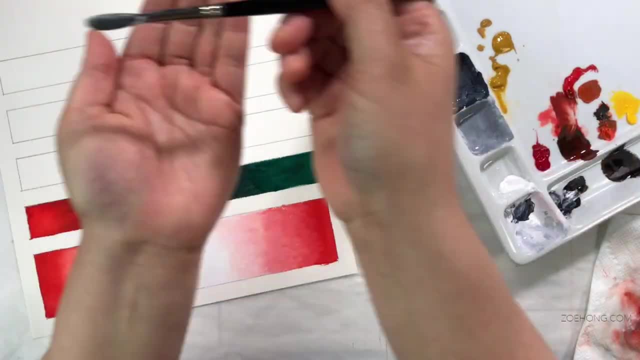 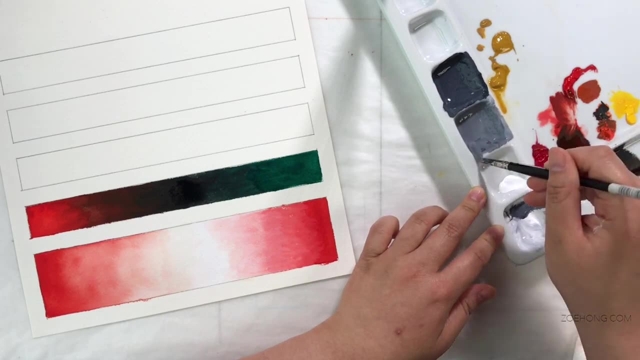 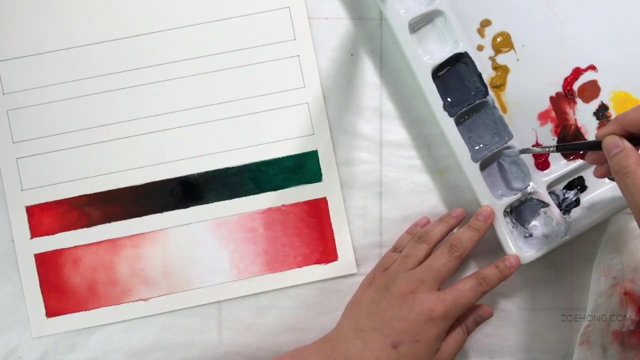 have light grays, dark grays, french grays, neutral grays, cool grays, warm grays. uh yeah, so many grays. right, you've seen those marker brands. every marker brand has multiple sets of different shades of gray. you know, as I mentioned before, I'm 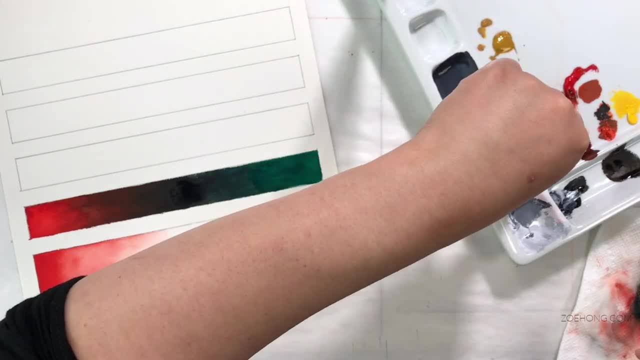 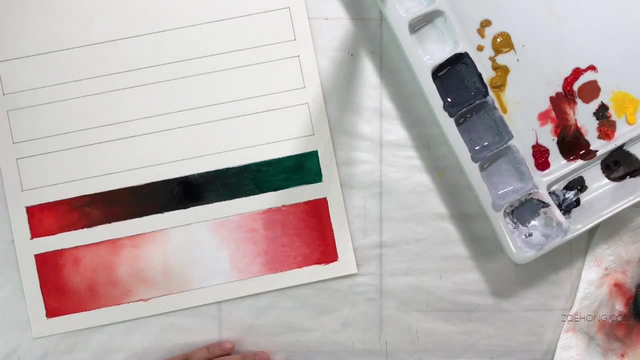 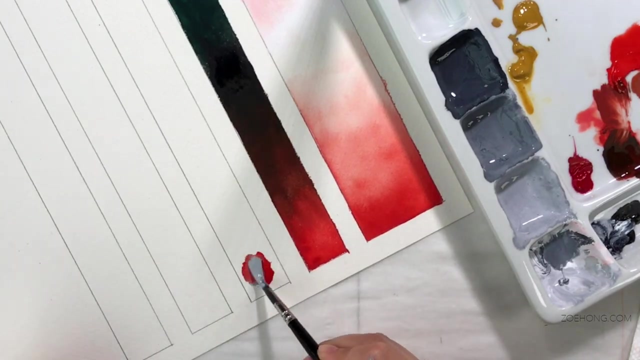 just using the set, and so I'm getting a rather cool gray from this ivory black and zinc white. so I mixed up three, and now I'm gonna keep mixing them up with the french red from before so we can get a true comparison and the colors are going to change. 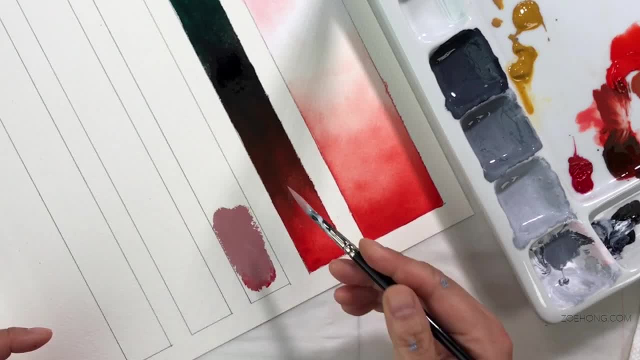 a lot, depending on, of course, what gray you use, which is uh important because it depends on the initial value of the color. this red orange, it's a medium value. it's a medium dark color. remember, value is the lightness or darkness of a color, and this red is a medium value. 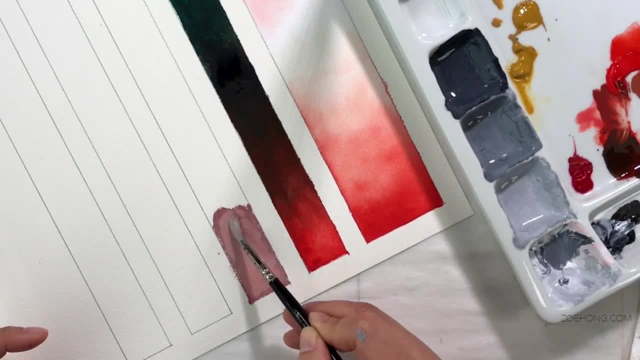 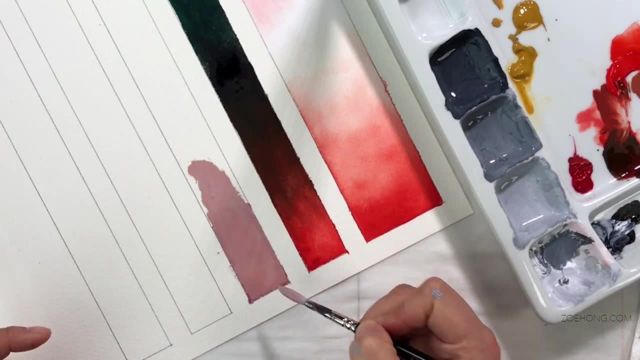 okay, it's not super light like the yellows and it's not super dark like blue. it's a medium value color and so when you add the light cool gray, you're going to end up with a lighter color than before and it's going to be duller and, of course, the more gray you add, the duller and grayer it. 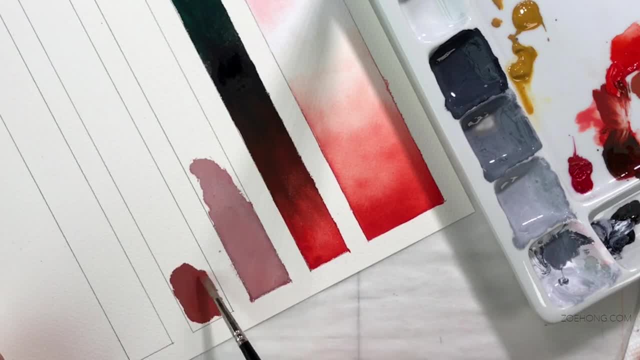 gets. but see, with the red orange and with the light gray you get this sort of wavy color. it's cooler than the original red orange and it's much lighter than the original red orange, this middle one. the second one I'm doing is red orange with the 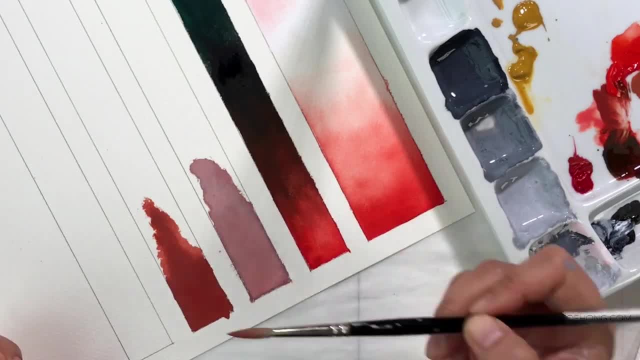 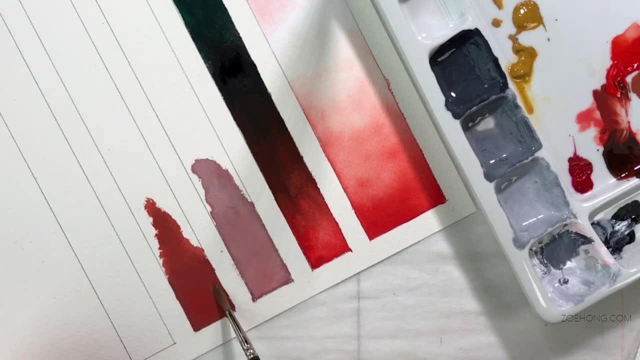 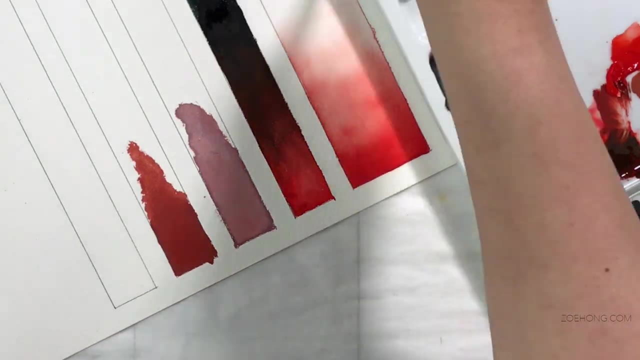 medium gray and because it they're similar in value, the gray is a little bit darker, but they're they're closer in value. the color ends up being more similar. now you see that it's a duller, richer, more brown version of the red orange, but it's closer than the lighter one because the values 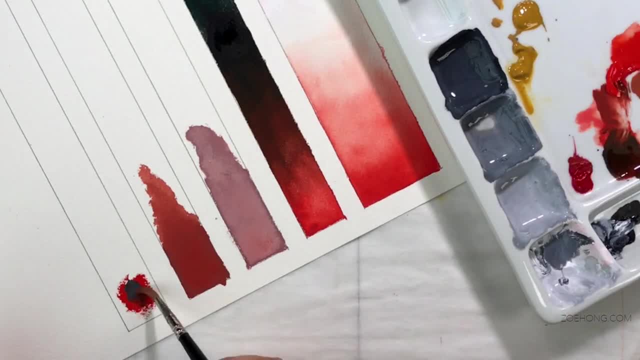 were closer. this third one: I'm using the darkest gray and you will see, as I finish mixing up this bar, the difference between the shades and the tones. even now, when you look at the second one, it is darker than the initial red orange, but it's browner and duller than the shades. the shades give kind of like a rich. 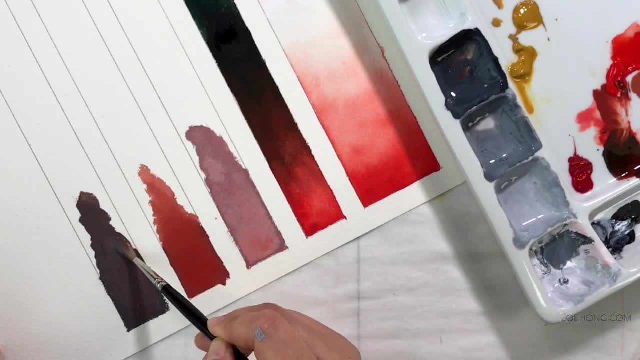 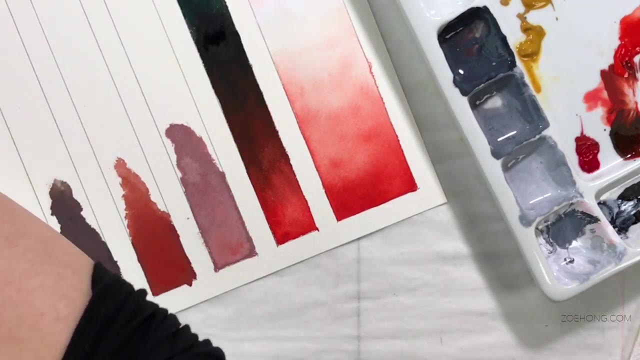 uh, kind of keeping the intensity of the red orange, but the tones tone things down, haha, maybe that's where those words come in handy. see, they tone things down, they dull things down and because of the white in there, it things that look a little bit creamier. 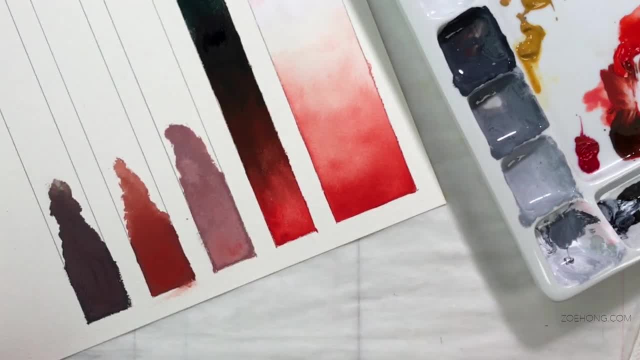 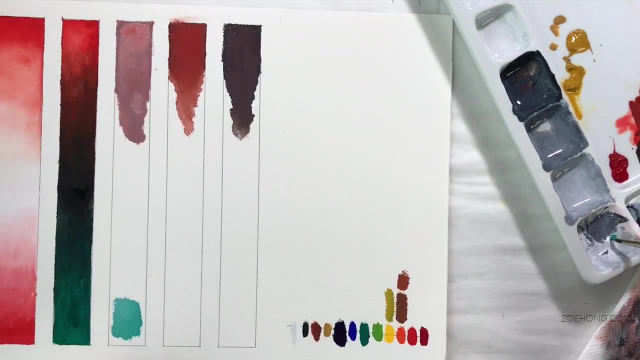 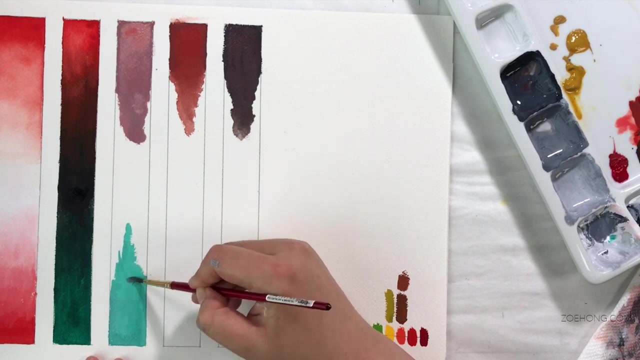 than a straight shade, and now I'm going to do the tones with that blue green, the Viridian Lake color, and again the light gray is much lighter in value than the original blue green color, and so you're, it's going to be very different. I use a little bit less than the red orange experiment. 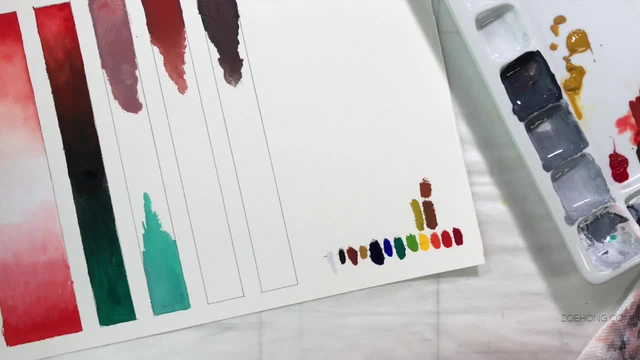 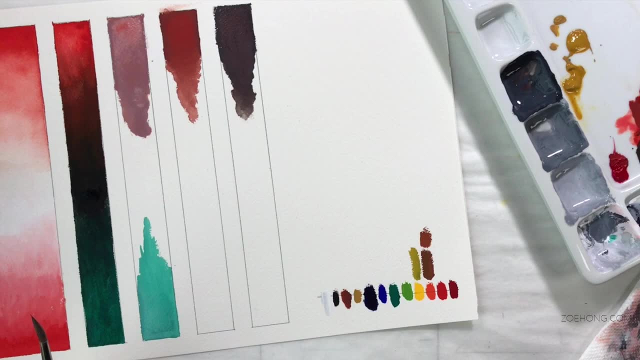 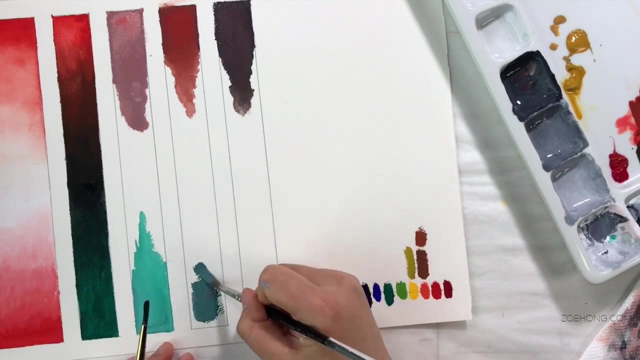 but it's still significantly lightened up the blue green and it's duller. you see that creamy sort of uh overall quality to it. here's the middle one with the middle gray, and again this is. this is a little bit lighter still than the green, but again it is a closer value match, so again, still looks. 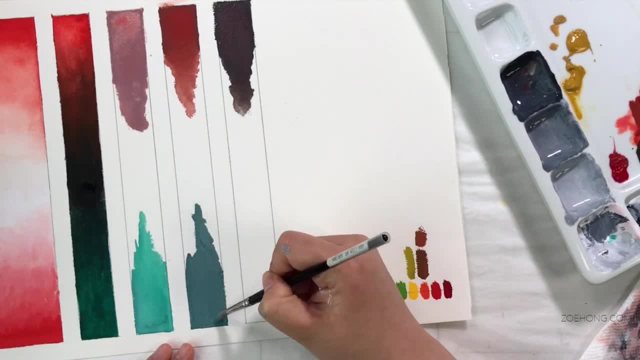 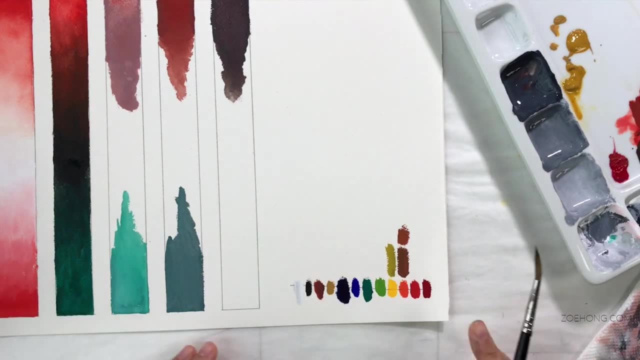 more similar to the original green than the first tone, but again it's got that creamy sort of dulled down. look more neutral. okay, and this is how you start creating more neutral colors. okay, we're gonna keep going with the next video where I deep dive into mutes, but, yeah, this is how you start developing. 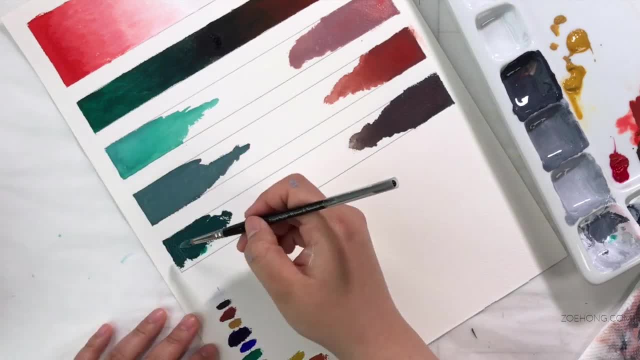 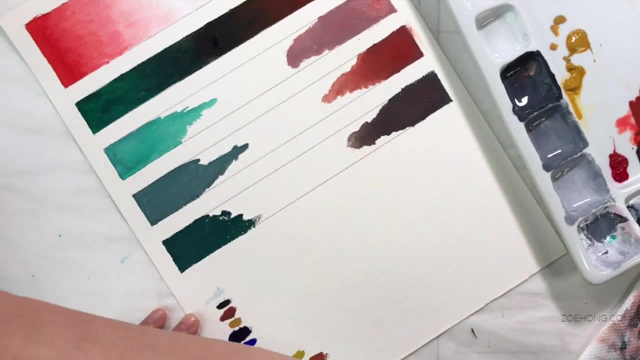 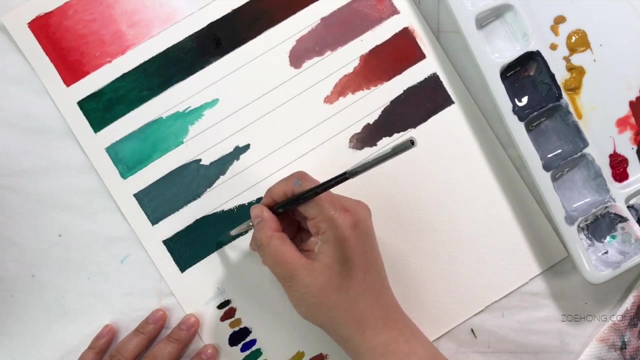 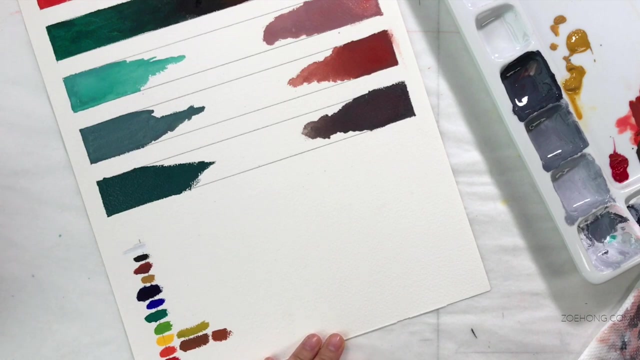 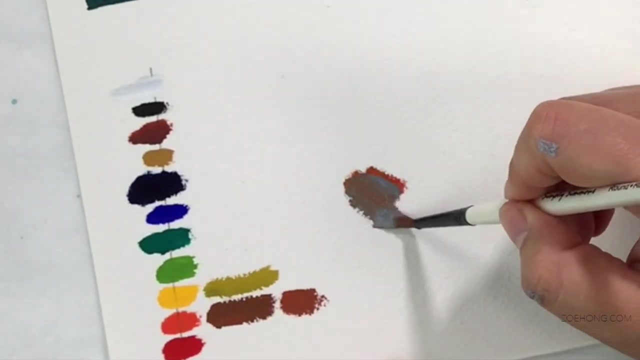 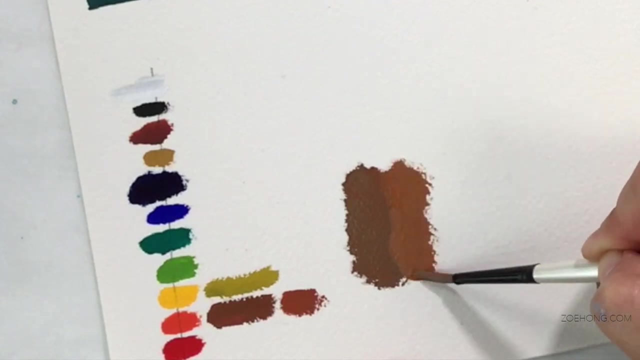 developing softer, duller, more neutral colors. and then this third one is with the dark gray, and it is the closest value match to the green out of the three. so this is the least different, but it's still a little bit darker, a little bit duller. so you know, again, go through your paints, mix up some grays, and here is orange with gray, and here 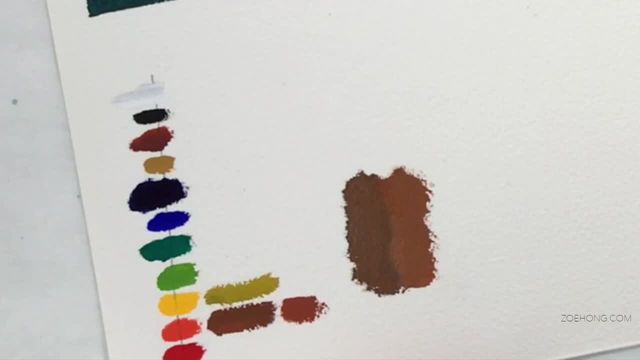 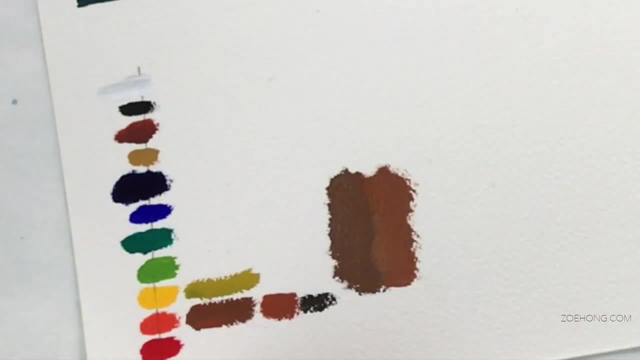 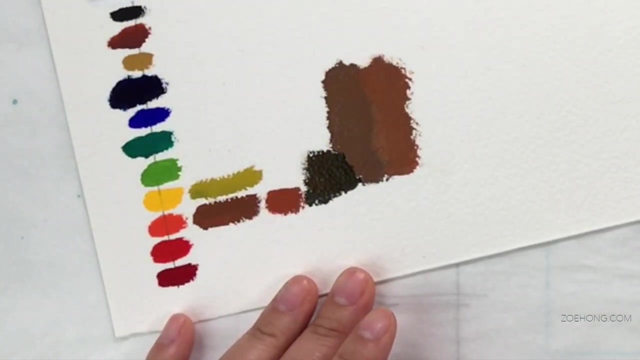 is orange with light gray, and you can see how these colors they ended up looking brown also- are a little bit different than the first two. I painted the little dabs with the black a little bit duller, a little bit creamier, the ones with black. just, they still retain. 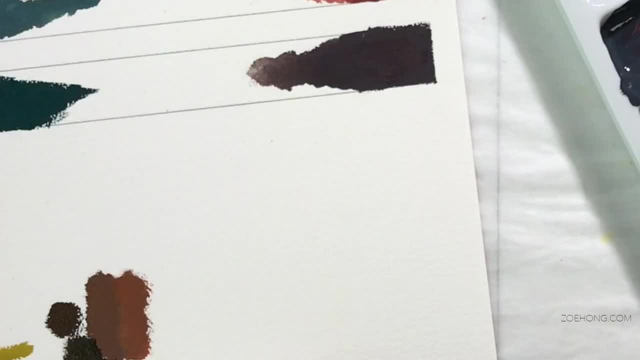 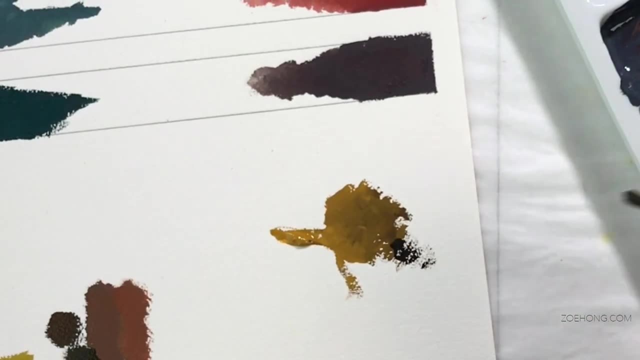 a little bit of color, but they still retain a little bit of color, but they still retain a little more oranginess. now I'm playing around with their yellow ochre. so yeah, all these things that I've been discussing. they also pertain to tubes of paint that started off with more neutral colors. 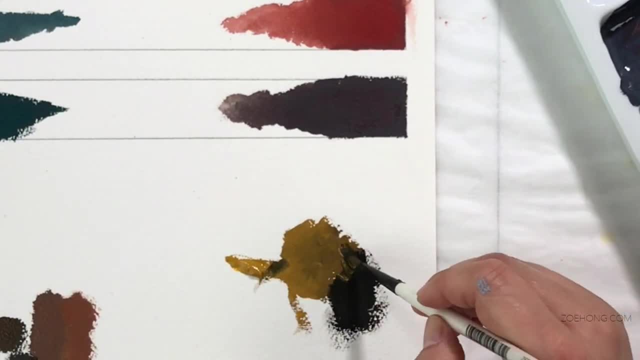 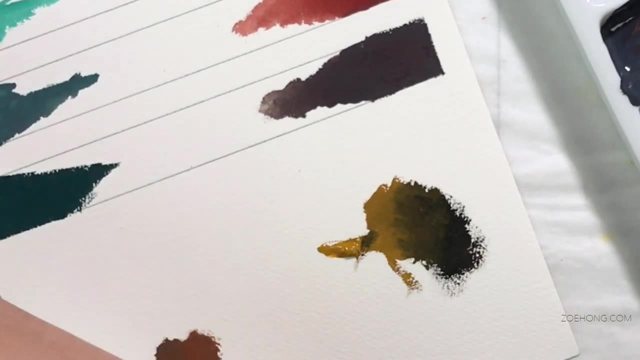 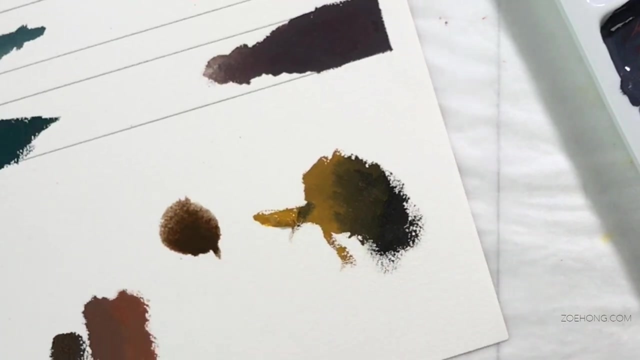 I'm playing with the yellow ochre and now I am creating shades of yellow ochre with the black, and then I'm going to show you tones with the yellow ochre so that you can see the difference. and this is how you're going to in the future. this is how you're going to. 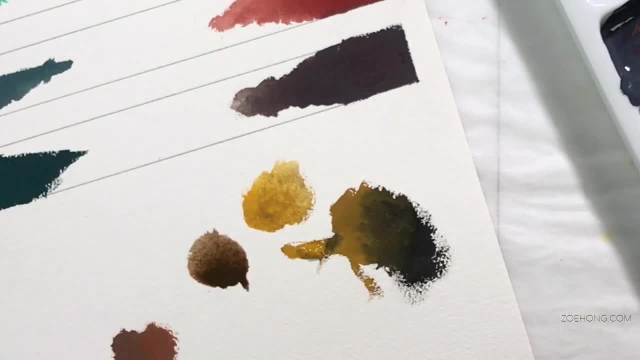 use the information. you know when you need a color. you know you're gonna think back to these experiments you did and was like, oh yeah, you know I need to match this fabric color. it's purple. it's a little bit duller than your standard bright purple. you know I would take this, maybe mix a. 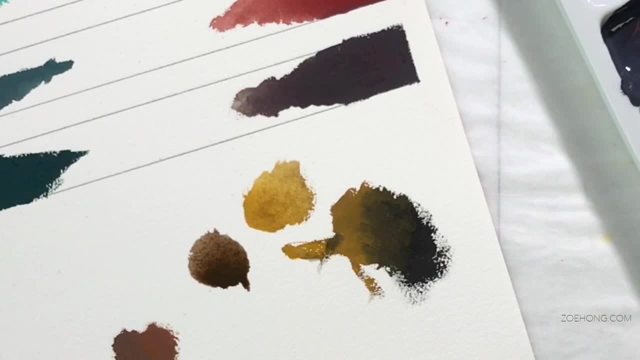 straight purple and be like: uh, all right, this is what I want this color looks like I want it to be. one is a little duller, okay, darker and duller, so maybe i add a dark gray to it. okay, you take these experiments off of this video and apply it to future color mixing experiments. here i am mixing. 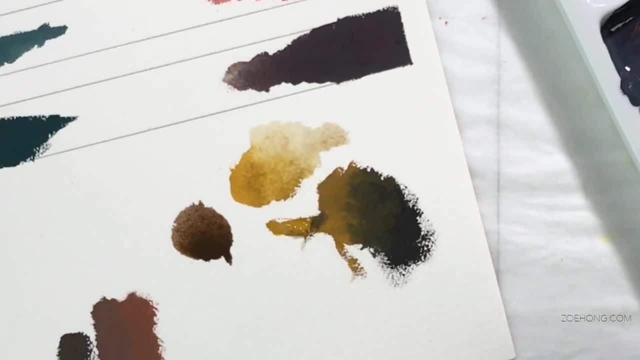 some water with yellow ochre so you get to see what those tints look like and you'll see later on. when you have, you know, an off-white color, beigey colors, and you're like, oh yeah, i've made that color before. oh yeah, it's just yellow ochre and white, and now i'm mixing up yellow ochre with. 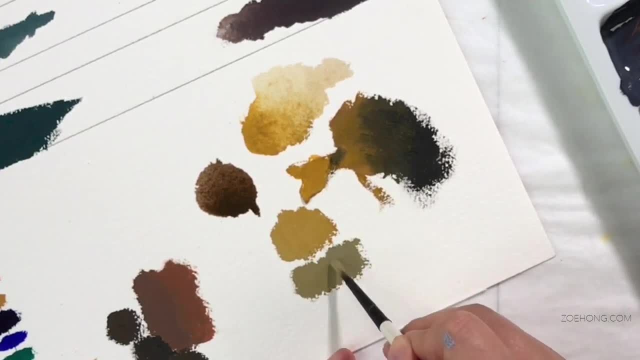 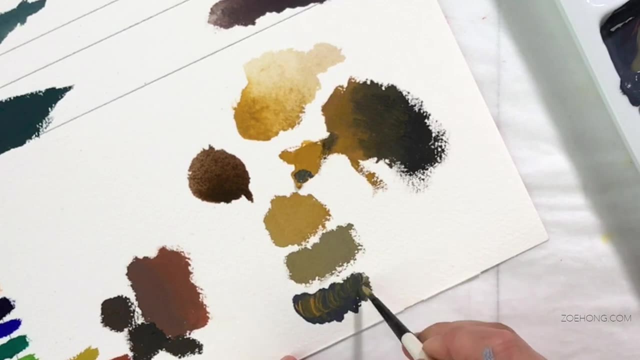 grays and i'm creating these really gorgeous khaki colors, these colors that you couldn't get with the black. the black with the yellow ochre were creating more cool browns, whereas now with the gray, with the cool gray, you're getting things a little bit green. you know you're getting. i'm actually really liking. 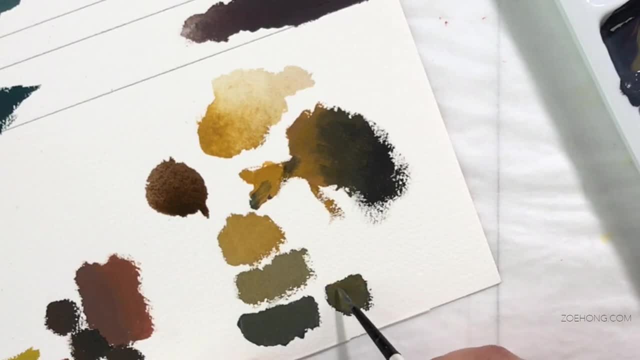 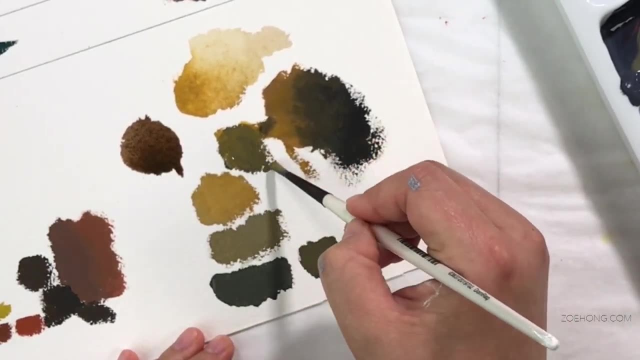 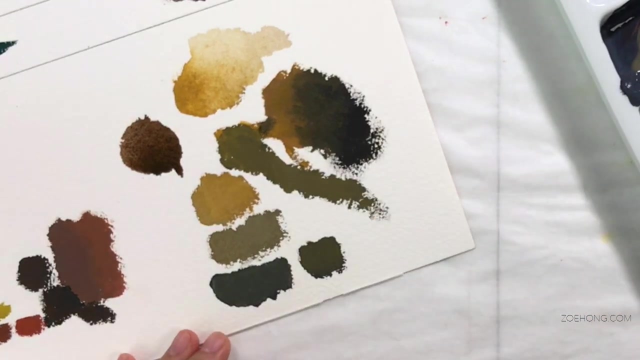 these colors, these kind of dark khakis, medium khakis, with the yellow ochre and the various values of grays that i mixed before. when i'm experimenting i tend to keep things kind of more orderly so that it stays locked in my mind like this is what happens when you add black and 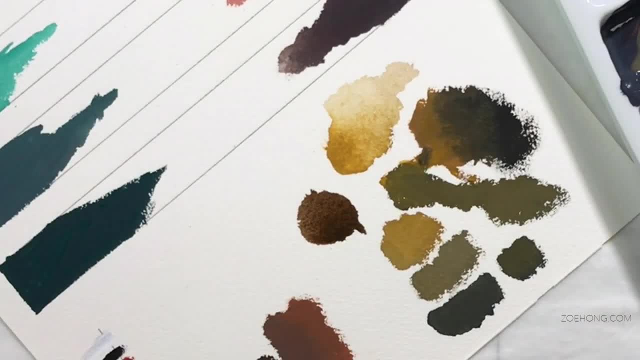 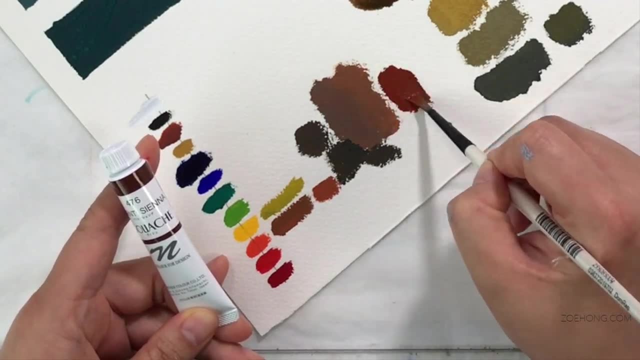 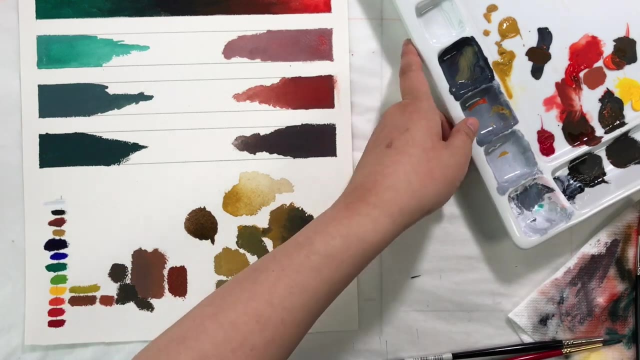 this is what happens when you add water, which is weird. it's like orderly experimentation. that's just straight up burnt sienna from the tube. i just want to show you how you you know now, you know kind of, the origin of burnt sienna. so yeah, final thoughts on that gouache. 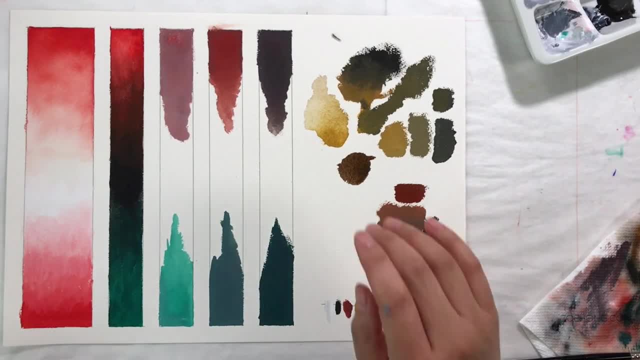 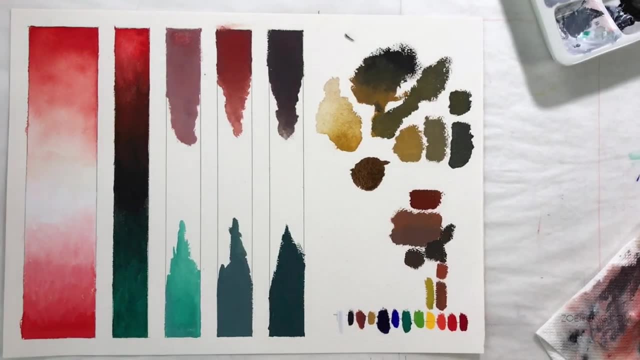 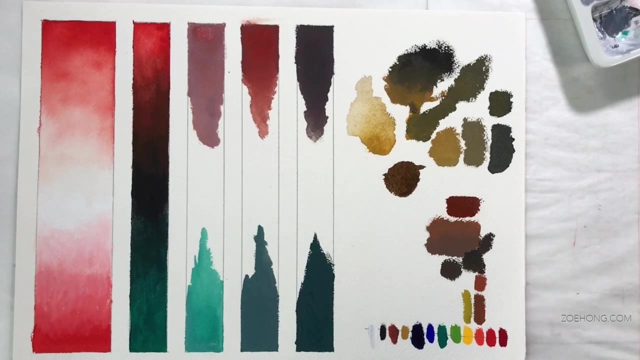 i really like this gouache. i'm going to be painting with these. like in the future, like my next time lapse paintings will probably be using this brand. i am enjoying it a lot. if that changes i will let you know, but for now i'm really digging it. i really encourage you. 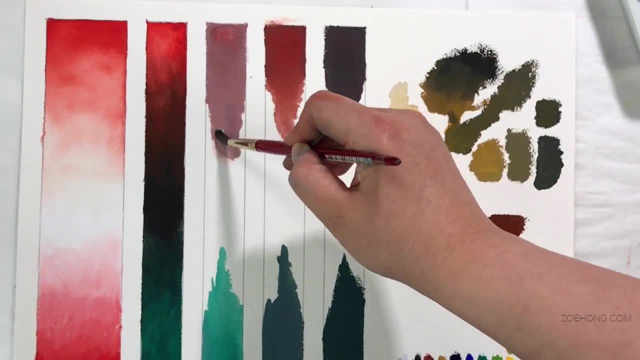 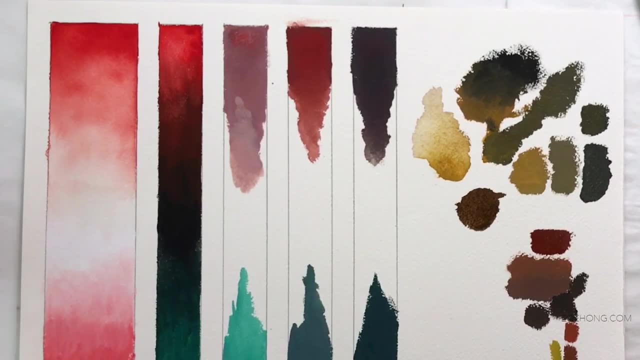 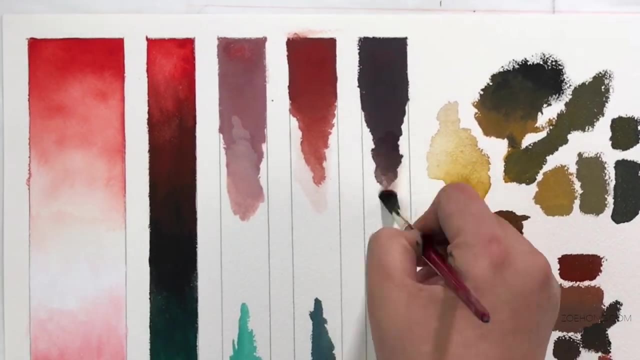 guys to experiment with paints and mix your own colors. and playing with paints and mixing paints and figuring out how these work together will also help you figure out how to get the correct colors when you're working in photoshop and illustrator and also when you're working with. 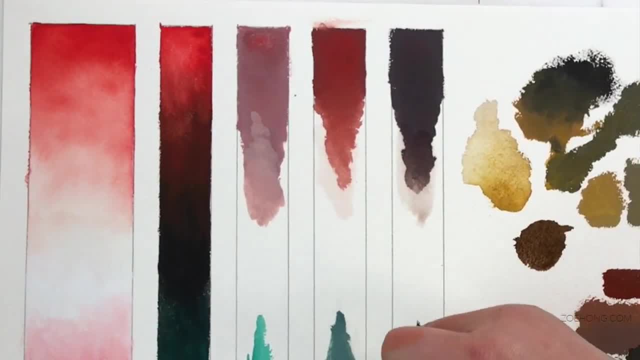 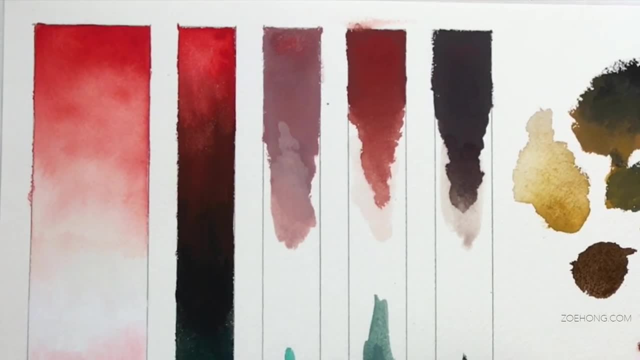 other media. so hashtag always be practical and i will see you in the next video. thanks for watching bye-bye and have a great day. bye-bye. practicing hashtag. practice, not magic. we are not made of magic, we are made of practice. so go practice and, uh, i will see you in the next video. oh yeah, don't forget to like and, you know, share. 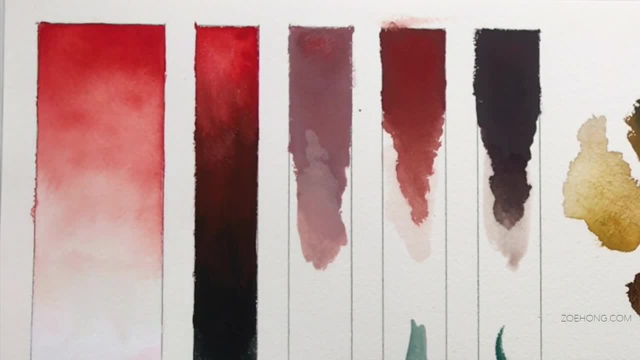 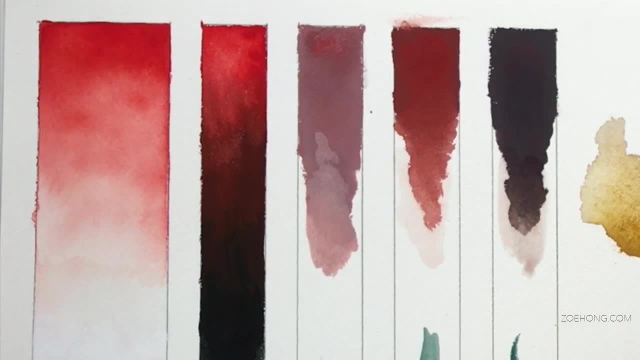 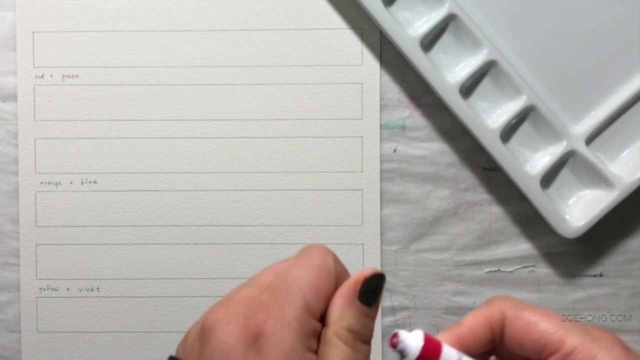 subscribe. oh, you know all that, all that good stuff, the regular sound off stuff. right, have a great time practicing and i will see you in the next video. hey, hey, party people. today we are going to work on mutes. we're going to deep dive into what a mute is and how to create it using paint. 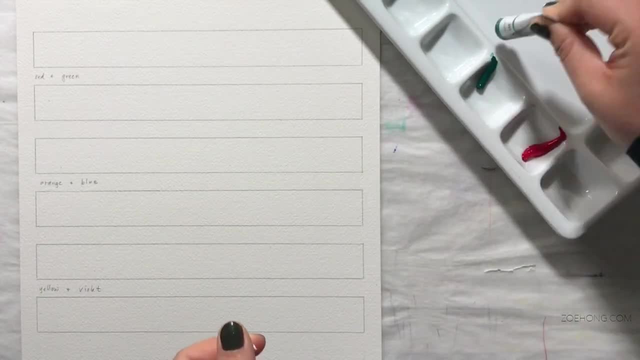 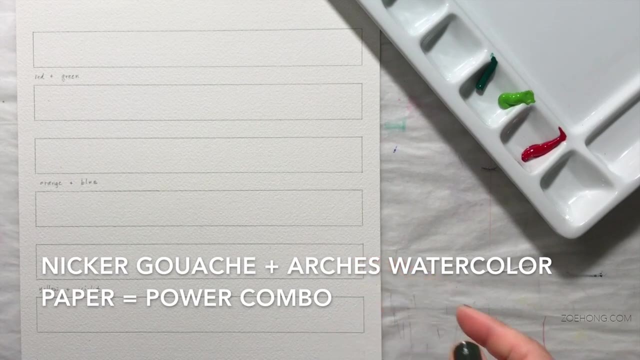 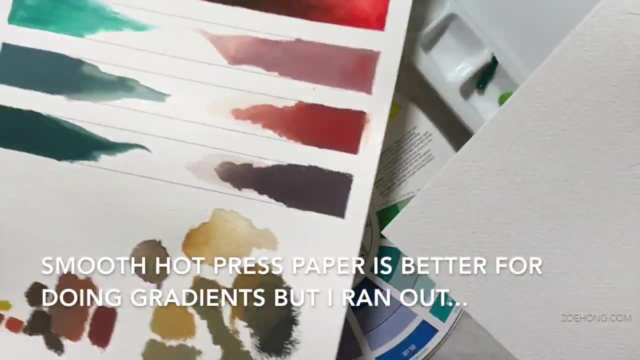 today we are using the knicker brand gouache again. i have basically fallen in love with this gouache. it's really giving windsor and newton a run for its money and kind of leaving the whole vine in the dust. i still have one more gouache brand. 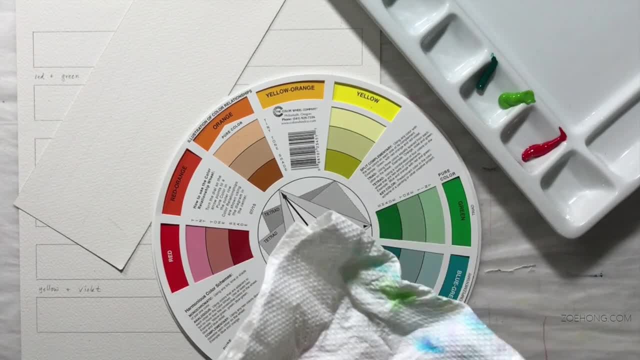 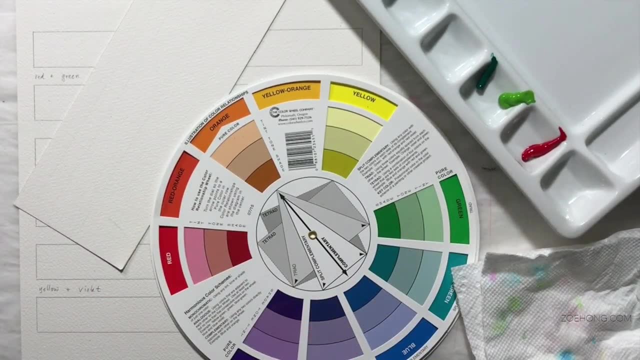 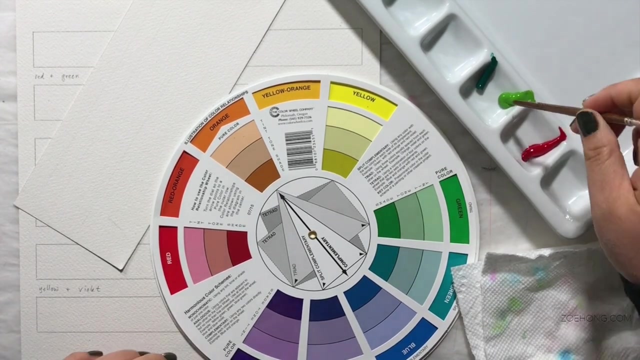 to uh, the pabeo and the talons brand that i still need to really deep dive into, but this knicker brand is just awesome anyway, so this is going to be another deep dive painting sesh. this is going to be the last in the really technical color theory videos for 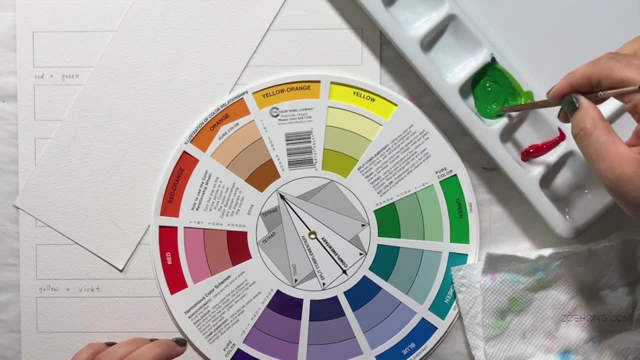 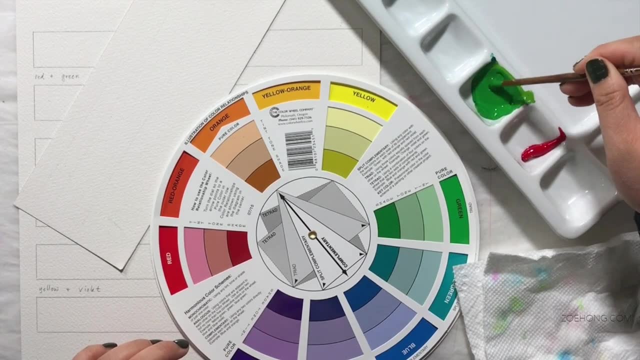 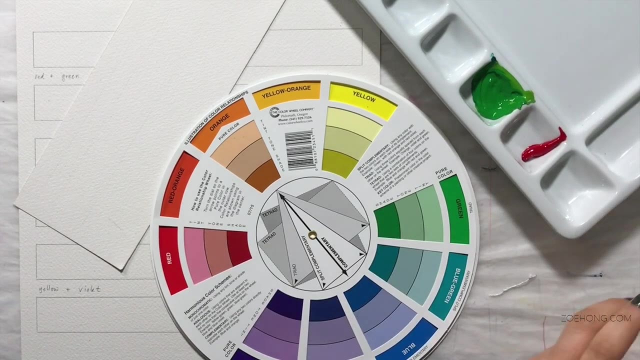 a little, while the next color theory videos are going to be taking all this technical information i have been throwing at y'all and applying it to fashion. are you excited? are you excited? this is what you've been waiting for, right? um, you know, i really felt like i needed to give you all this. 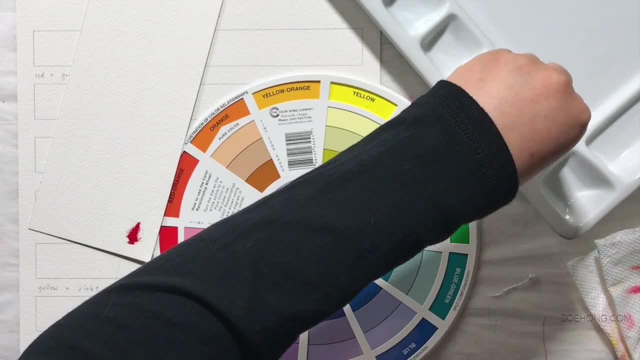 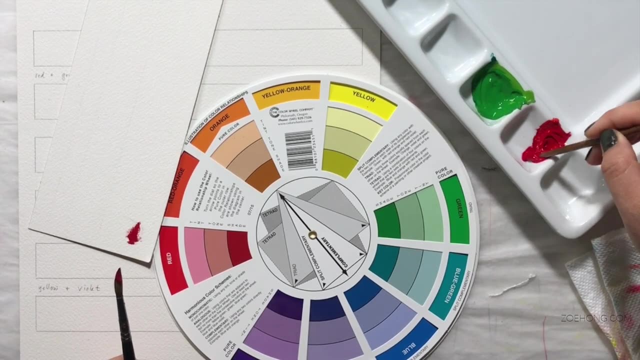 a lot of this background, technical vocabulary, just like. really show you where these colors come from so that i can show you how it applies in picking colors for your collections and how to do color talking and how colors affect the mood of a dress and you know how to make things more figure. 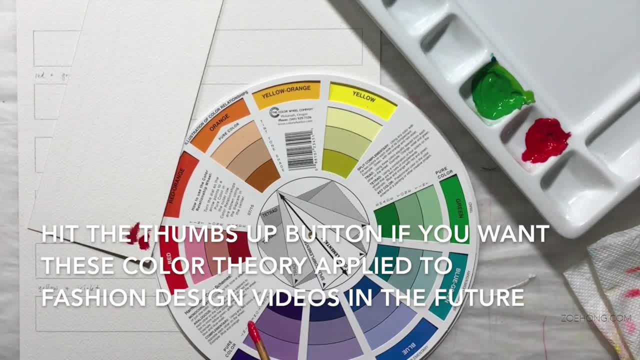 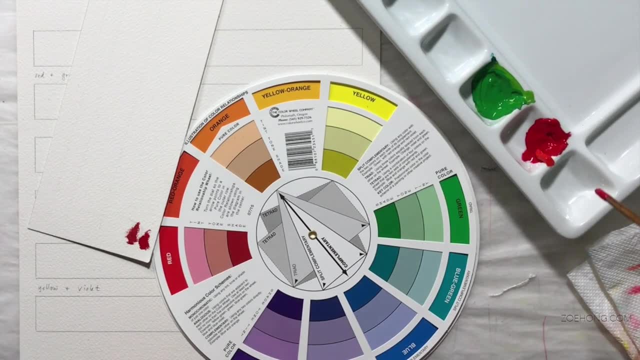 flattering with different colors, and you know, i'm going to talk about all those things in the future videos. now that we've really gone through the technical, okay, uh, this is what i do in class, where, also where i take a concept, i deep dive into the technical before i talk about how it applies. 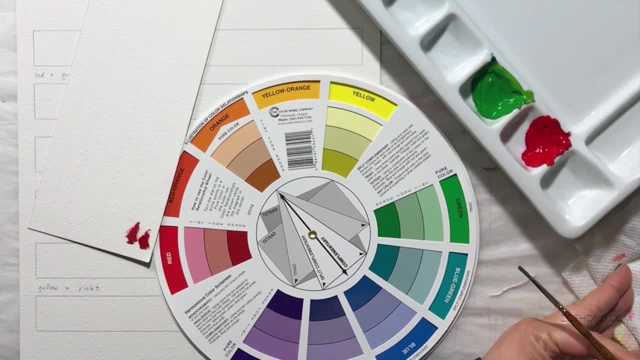 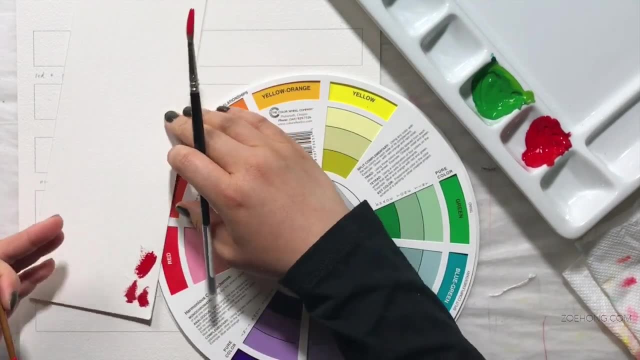 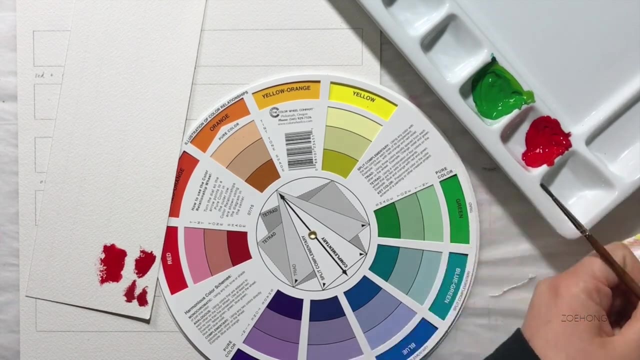 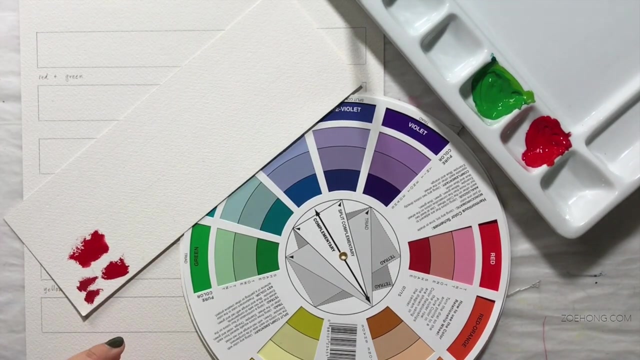 to fashion directly. okay, so that's going to be the next few color theory videos where i talk about how compliments work in fashion and how mutes work in fashion and how monochromatic color schemes work in fashion, etc. etc. all right, and so yeah, all right. so mutes, all right, let's get all technical about. 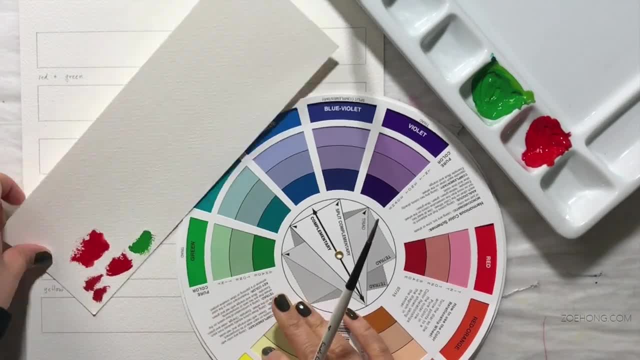 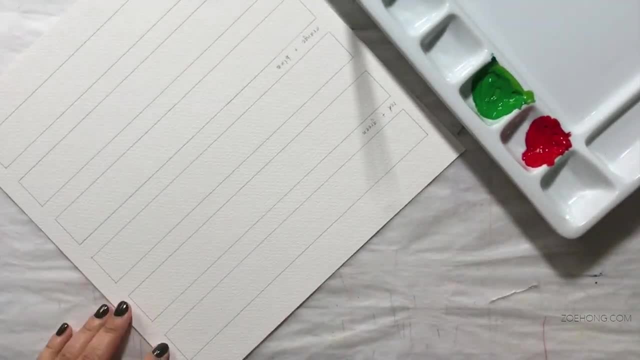 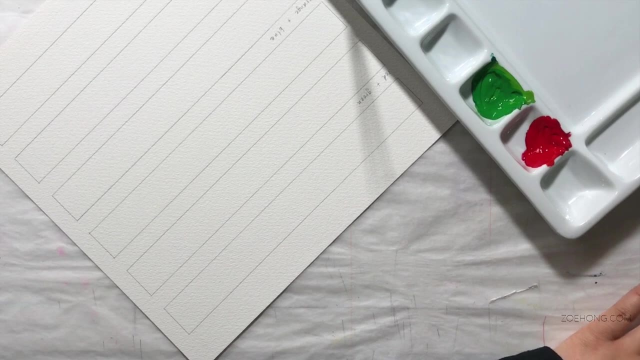 mutes. what are mutes? uh, they are the fourth out of the four ways to desaturate a color. there's tints, shades, tones and mutes, and these four words are very uh specific in the way they're used in color theory. i know people use uh adjectives and verbs toning things down, muting. 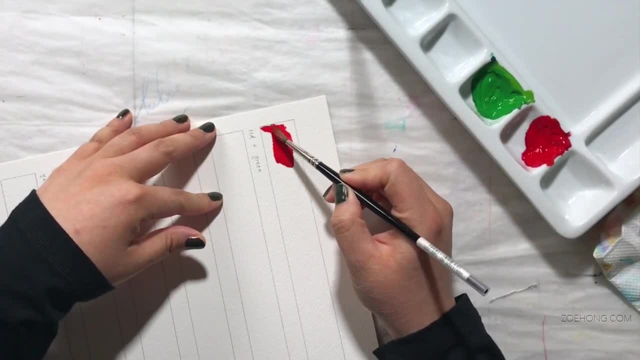 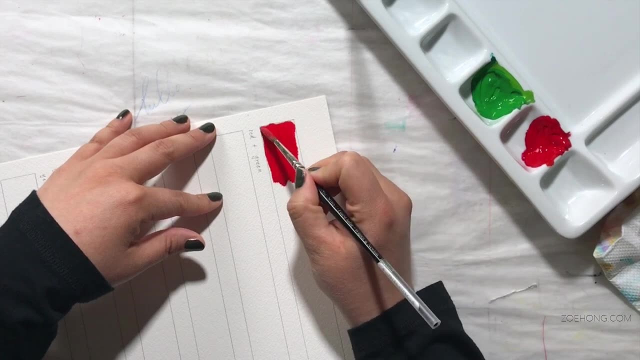 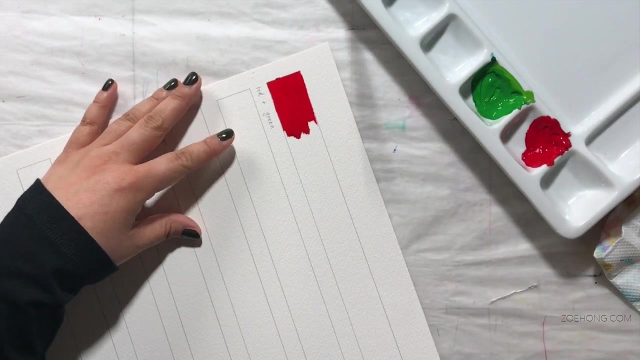 things down, tinting things, shading things much more loosely- and sometimes i do that too- but when we're talking about exact color, mixing these color, these words- tint, shade, tone and mute- are very specific. tint is color plus white, tone is color plus gray, and that could be a light gray, dark gray, warm gray, cool gray, etc. and shade is color. 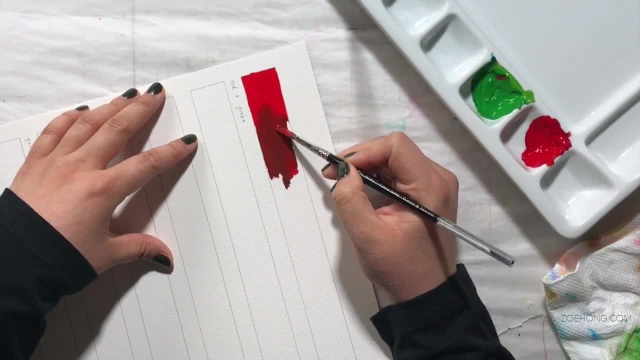 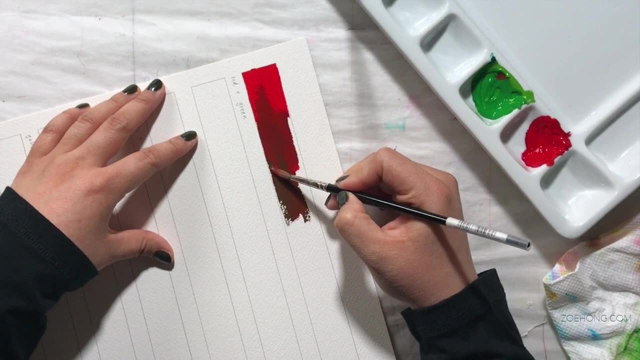 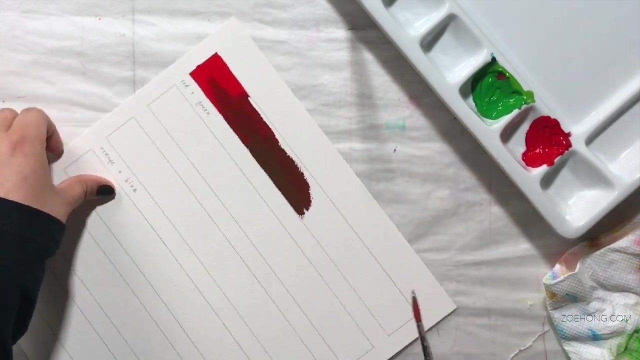 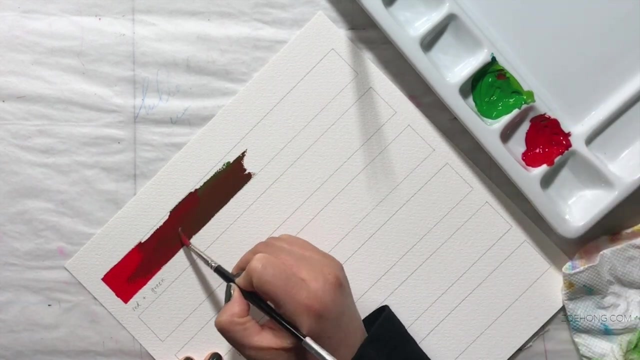 plus black, and mute is color plus its complement, which is its opposite on the color wheel. so red plus green, orange and blue are mutes, yellow and violet are mutes and they're mutes and they're used together to mute the other, as in, you know, when you say mute, you think silence, quieting down, okay. so 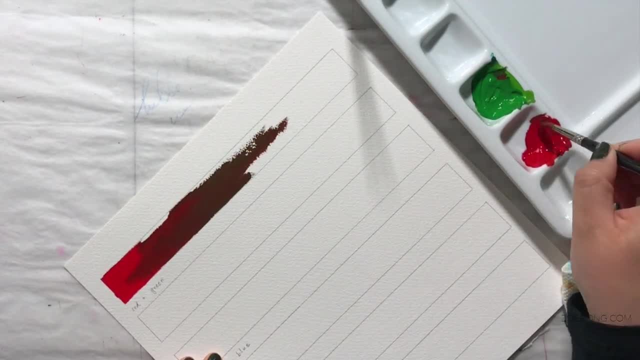 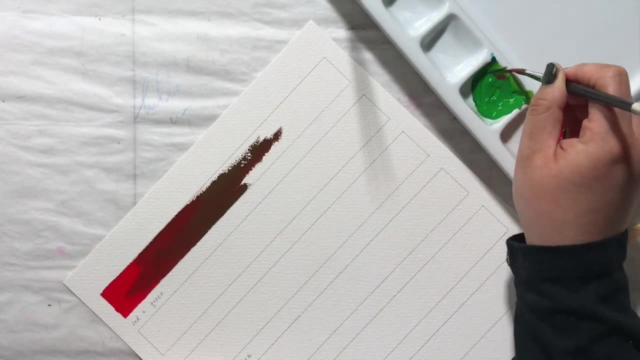 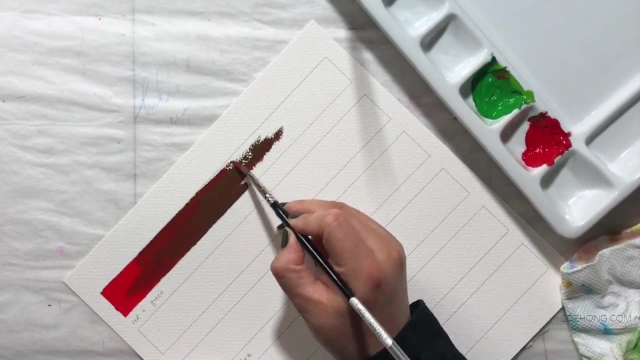 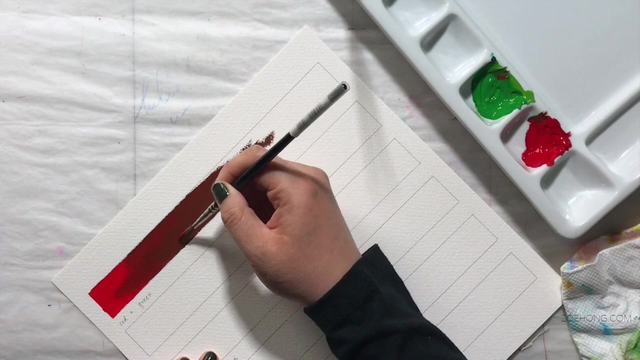 when you add green to red, you're quieting down the intensity of the red, literally what it means red plus orange is red orange, right. and when you add red plus yellow, that's orange. and when you have red plus blue, that's purple. and the red plus purple is red purple, or you're. 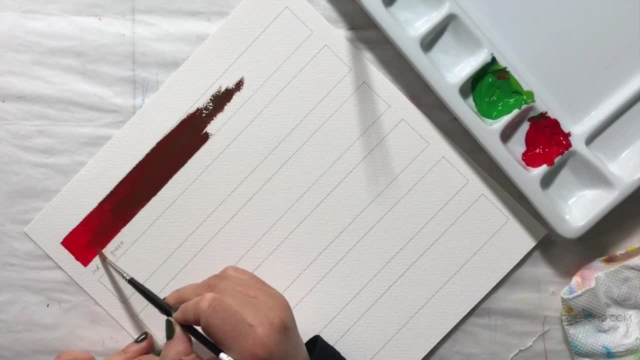 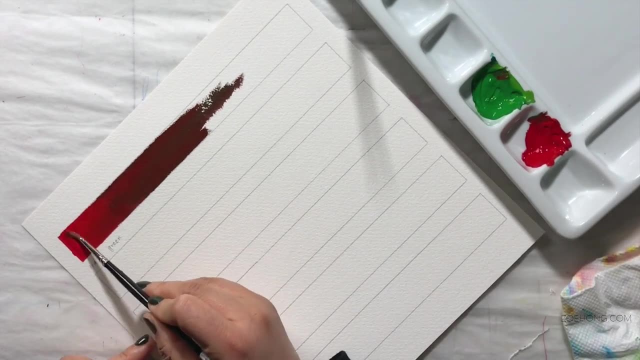 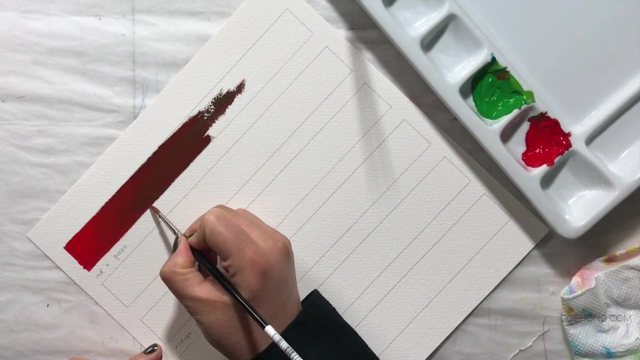 starting to get into, like red, violet, magenta categories. but when you add red and green, that's when you start getting these more neutrally colors And I really like. if you really want to understand colors, I highly recommend that you do similar color mixing experiments. 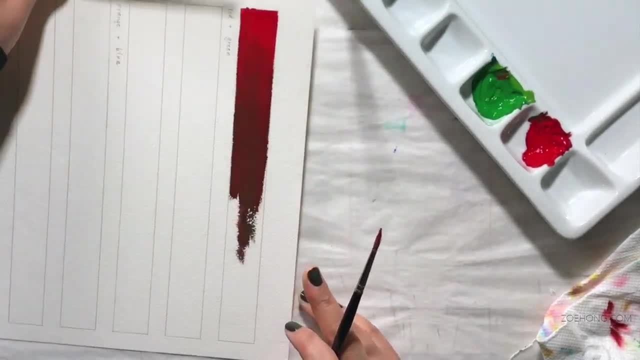 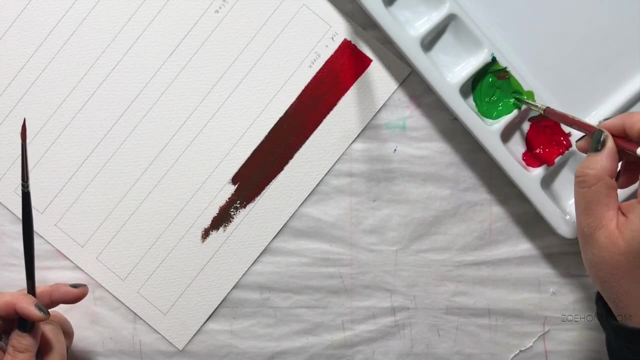 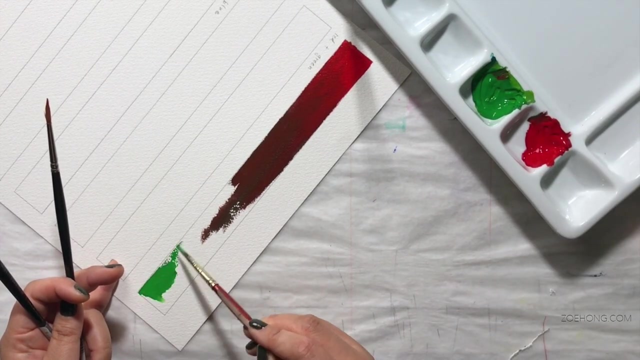 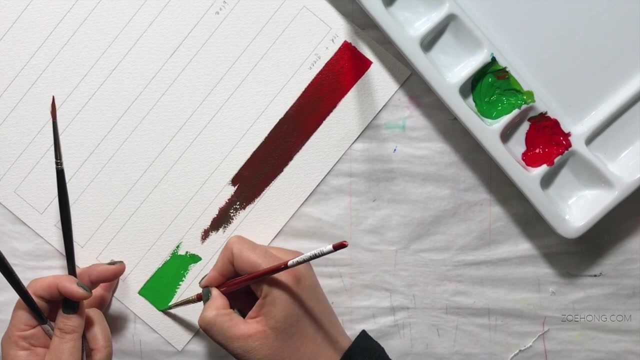 You don't have to work really hard on creating a beautiful gradient like I'm doing right now- Like I like painting gradients and I wanted to make something pretty for y'all to look at while I'm talking- But just simply try mixing a red plus a green to see how that red looks compared to red plus black or red plus gray. okay, 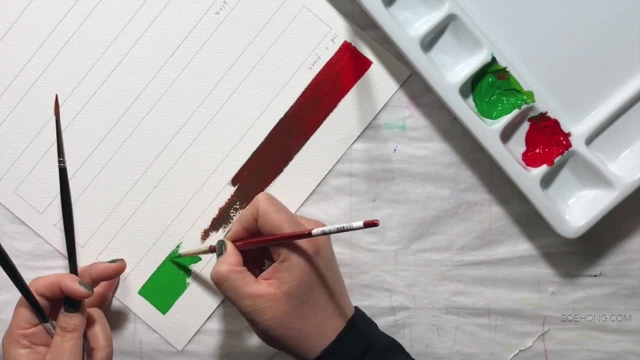 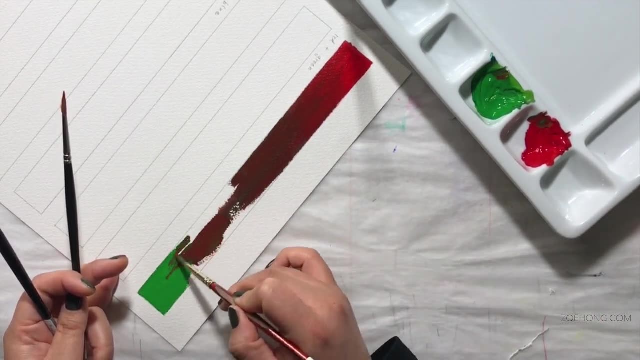 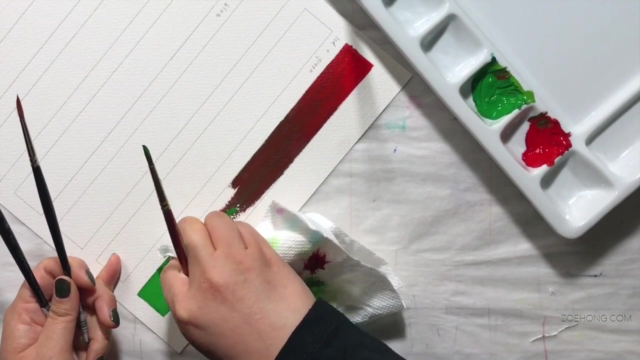 Because those are all different ways of desaturating the red, but they're completely different. You know the warmth of the green. you know green has a lot of yellow in it. the warmth of the green And the warmth of the red is going to make the red more brown. okay. 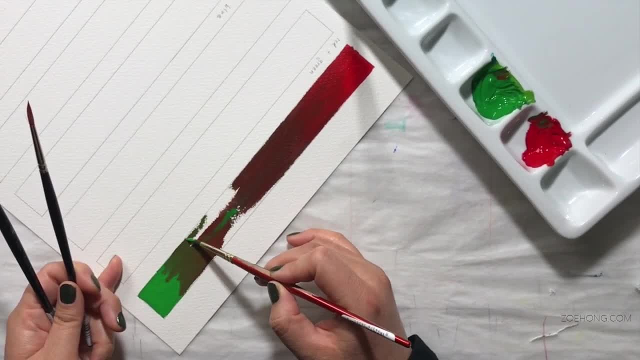 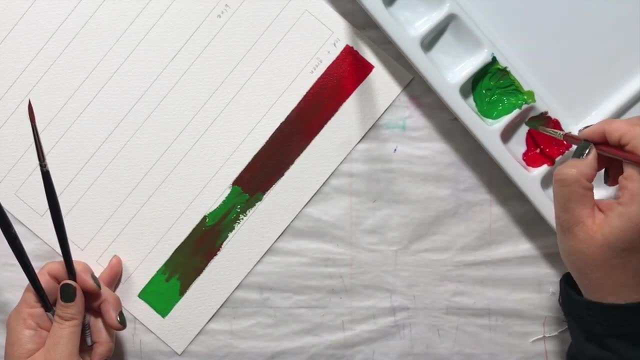 Like gray plus red, depending on how warm or cold the gray is, it's going to keep red pretty cool, Like red is a cool. it's a warm color but it's on the cool side of warm, if that makes sense to you. 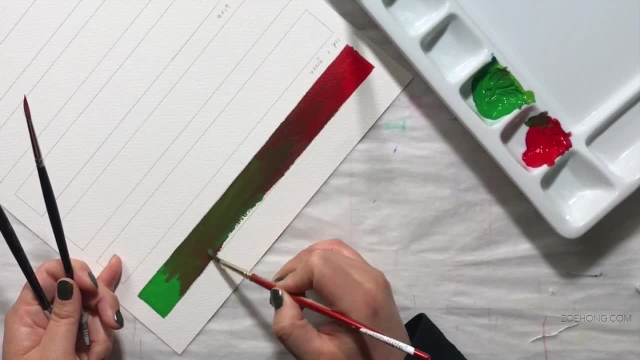 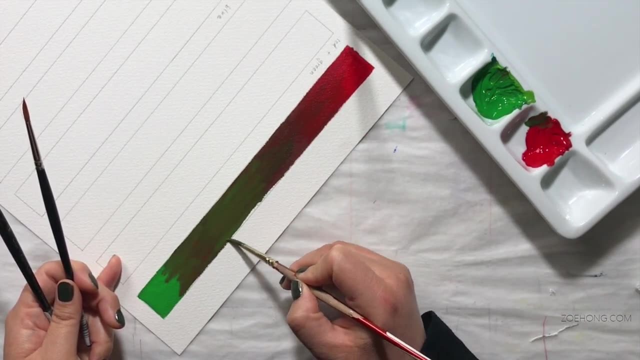 And so red is one of those colors. if you tip it in one direction, it could get really cool, like burgundy, or it can get really warm, like poppy red orange. you know, Anyone who wears a lot of red lipstick knows what I'm talking about. 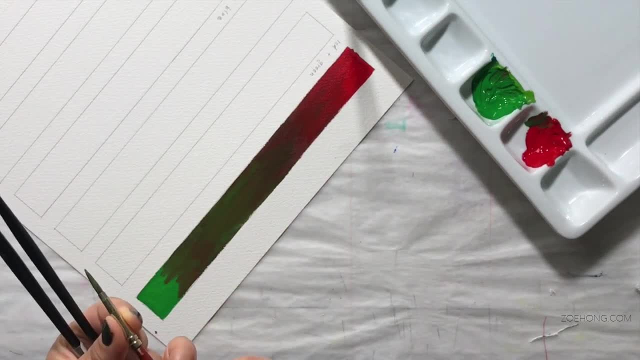 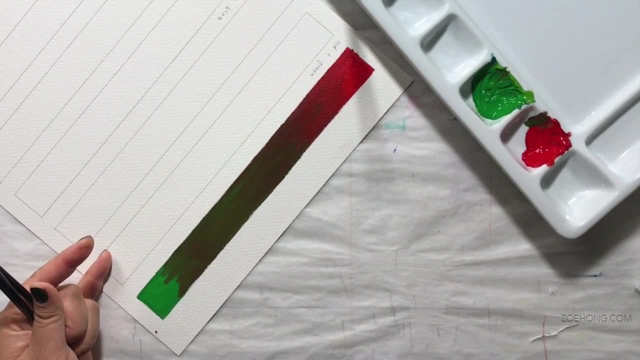 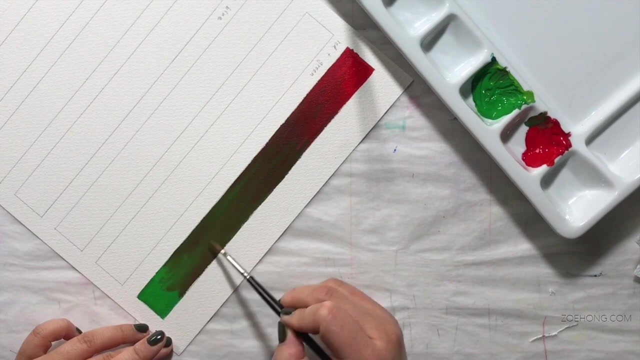 So when you add the green, the warmth of the green, and then toning it down because it's the opposite, you know you get these warmer browns and you also get these duller greens, And again those greens are going to be really different from when you have green plus black. 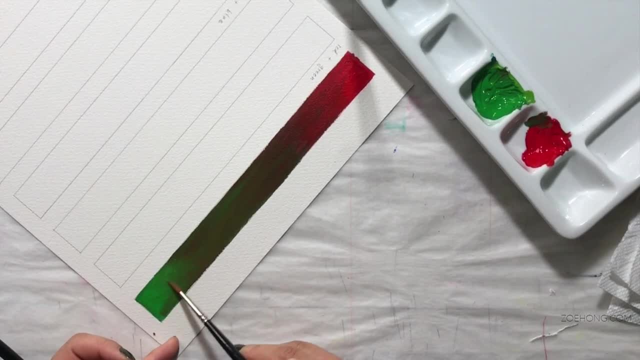 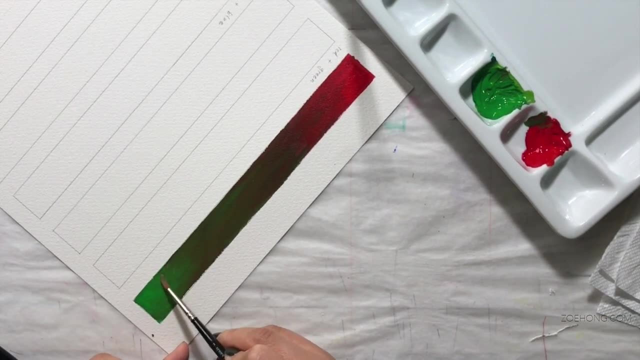 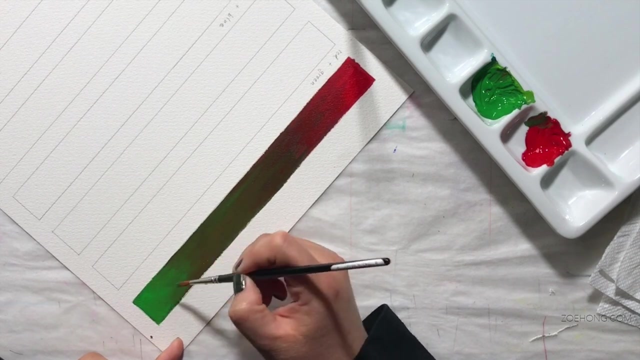 versus green plus black, Green plus gray versus green plus red. And again, I really encourage you to mix those colors yourselves with the paint that you have Now, just like in the previous video where I was talking about, especially with the grays, with tones. 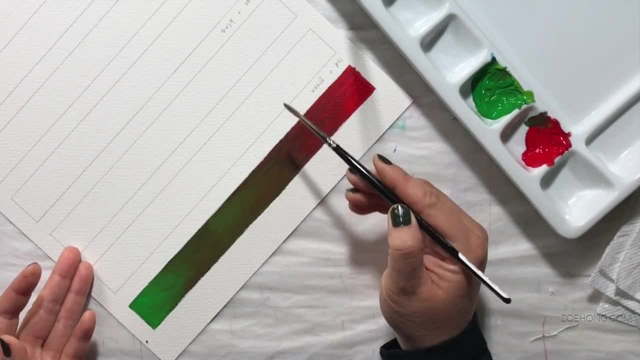 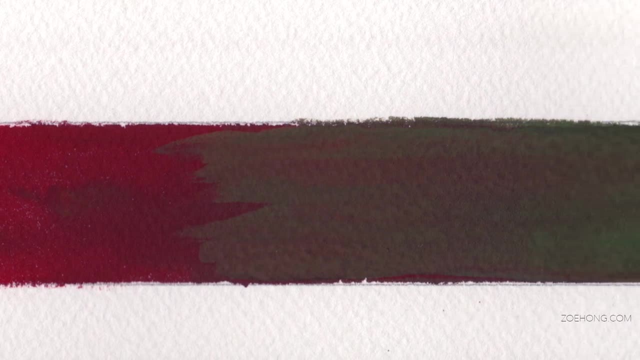 how you can really change the color, depending on whether you add color plus dark gray color, plus medium gray Color plus light gray. you're getting lots of different colors And then colors versus plus warm gray, plus French gray, plus cool gray. you know. 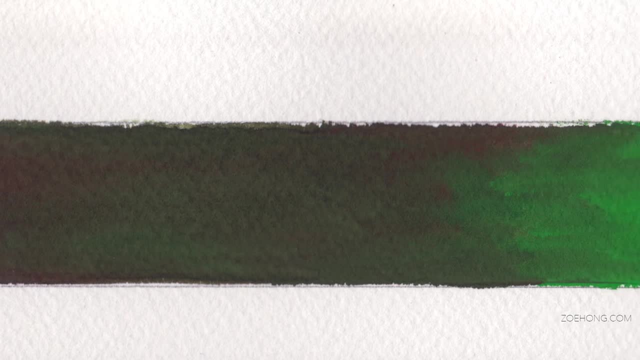 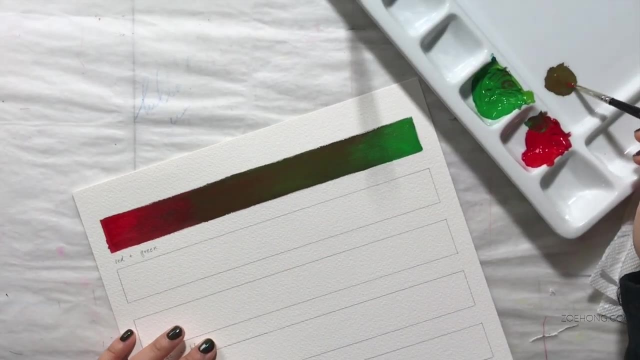 all these different things that you could do. the same is true of mutes. It's not just full-on red plus full-on green. I mean, those colors are awesome, but you can also again add in a black so you have a shade of a mute. 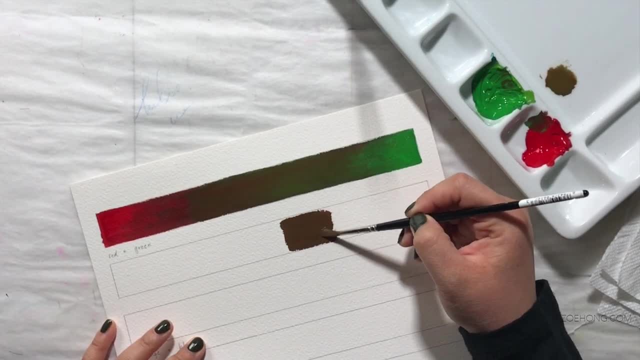 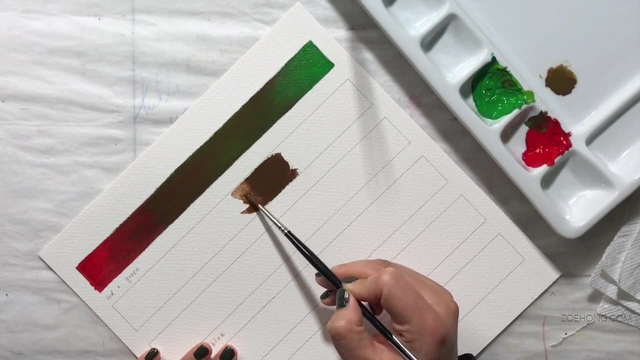 And you can get some really dark dull. You can get some really dark dull greens, beautiful olives, or you can add some white And see how here I'm adding some water to the brown that I created with the red and green. 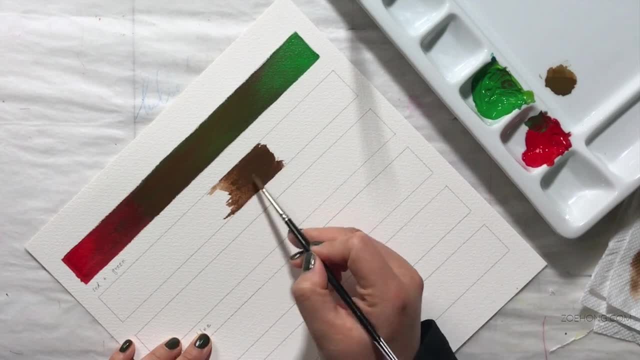 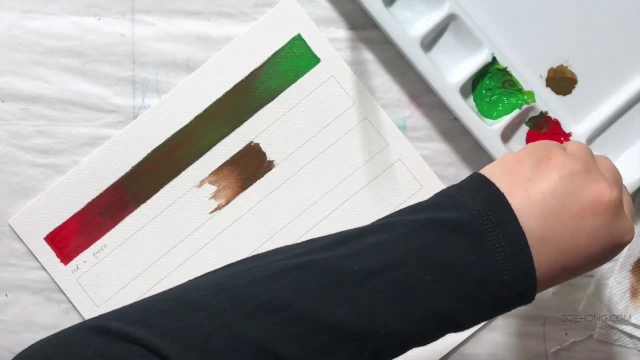 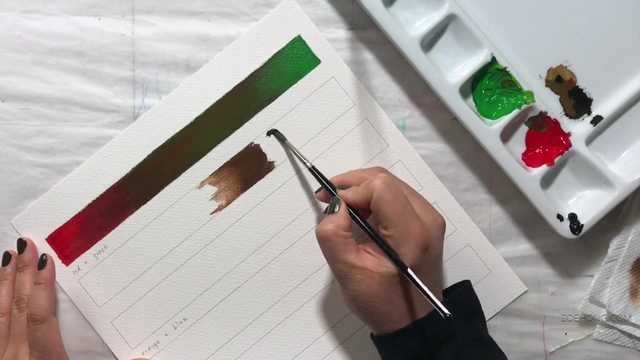 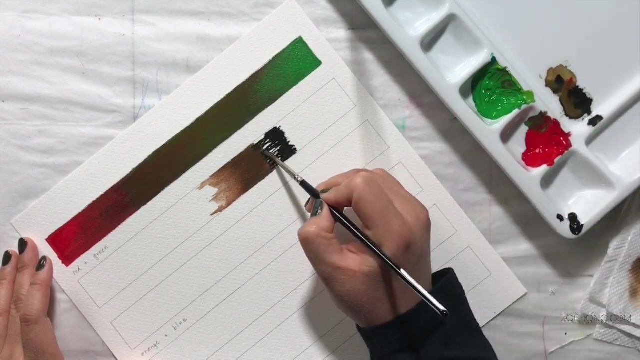 And so you're getting lighter and lighter browns. Okay, So that's a tint of a mute, Like in class when I'm lecturing I get all tongue twisted and I'm like there's no editing in class, Anyway. so, yeah, you add black to it. you start getting super dark, like dark umber, like black brown colors. 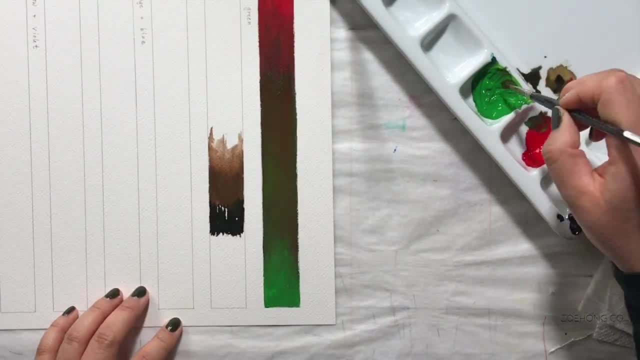 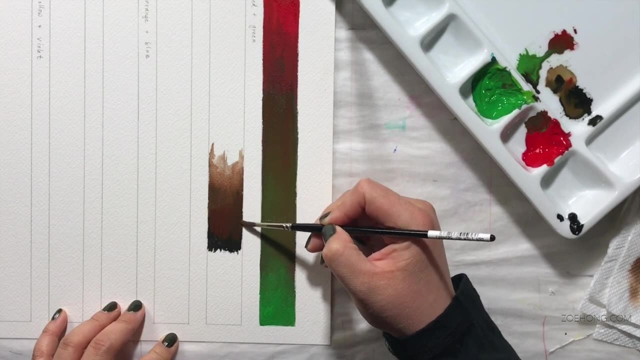 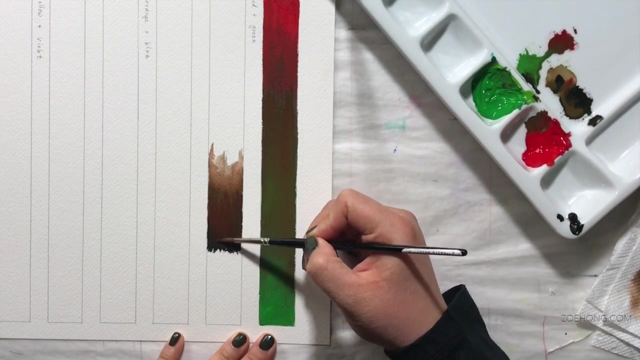 And then you add white and you get the lighter browns and you have the full range. and you can play with that too, And you can also make a tone of a mute or whatever you want. but understanding, you know the base of a mute will really help you. 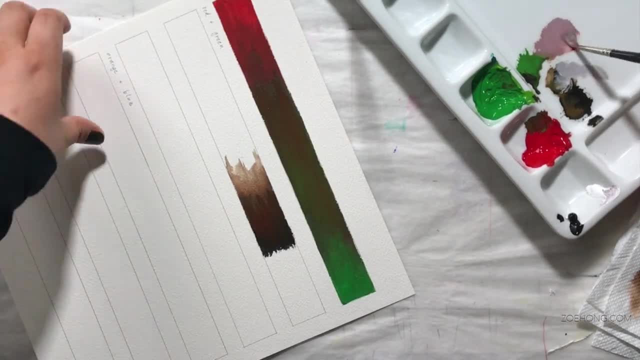 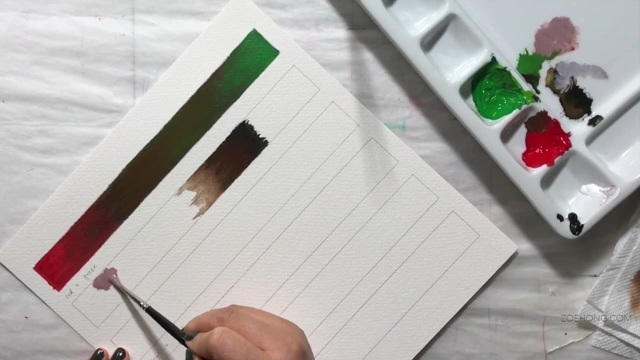 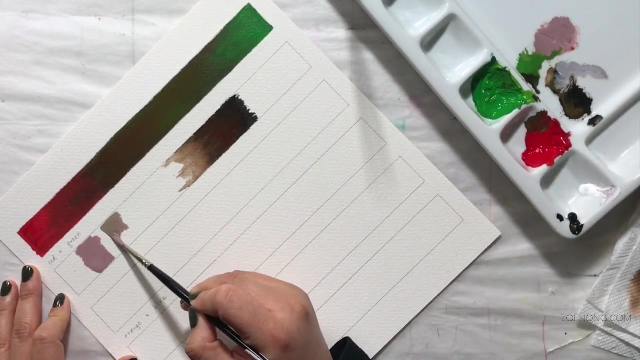 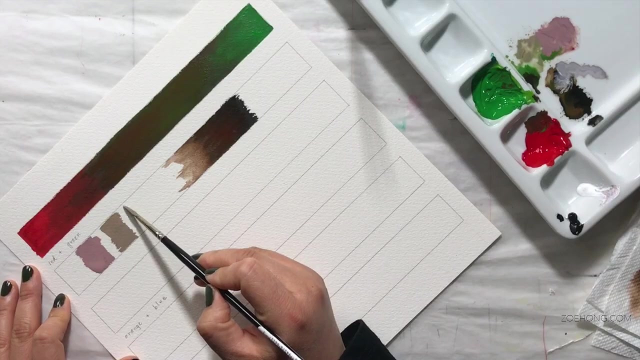 So here I am mixing white and black, So I have a bit of a cool gray, because the permanent white and the ivory black tend to make a coolish gray- not super cool, but coolish. And then adding red with a touch of green is now creating these tones and they're very, they're like white. 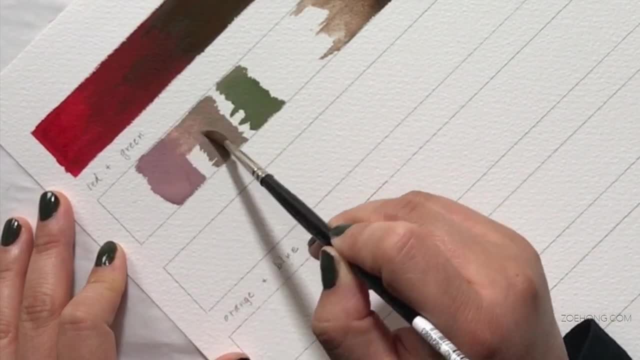 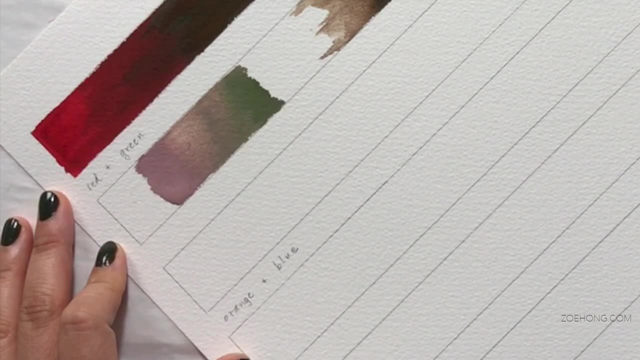 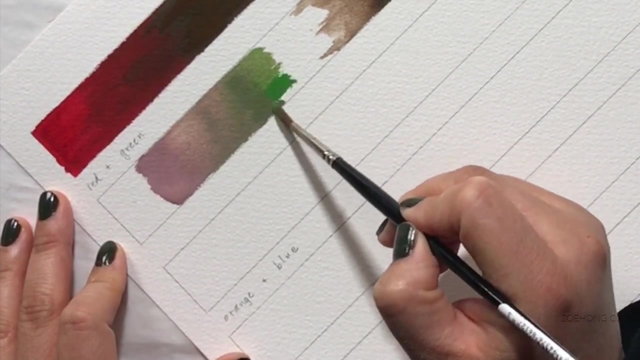 neutral. Neutral but not bright enough to be pastelly, Like we associate pastels that are very bright, not dulled down, with a lot of the gray, Same, but now I'm creating these like dusty roses and these muted celadon jade colors, which I really like. 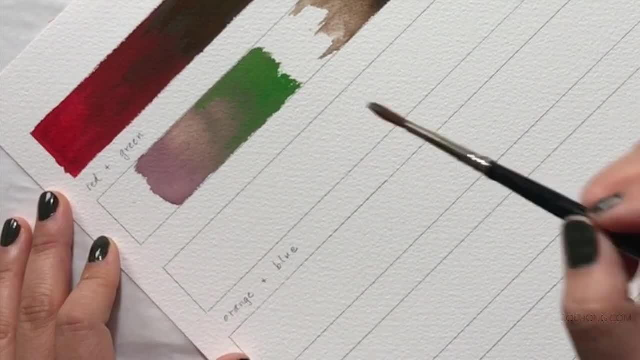 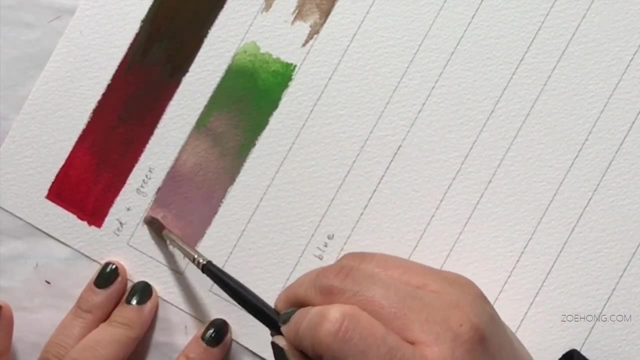 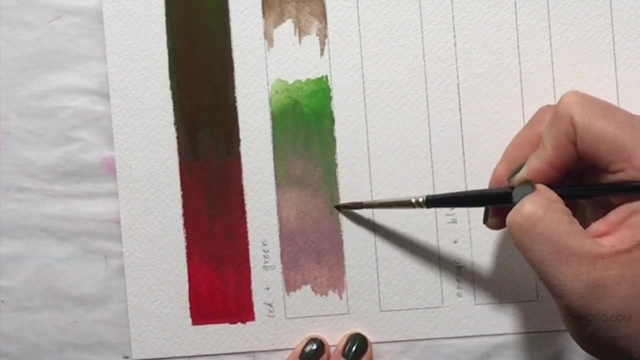 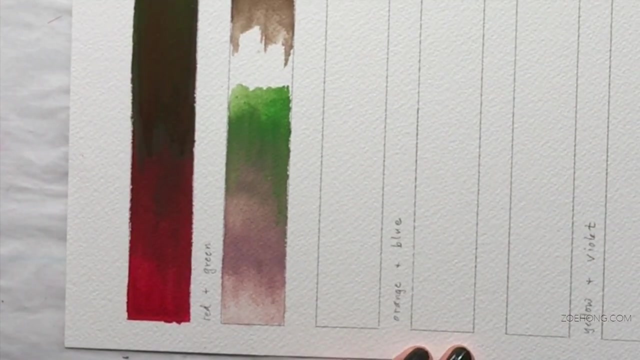 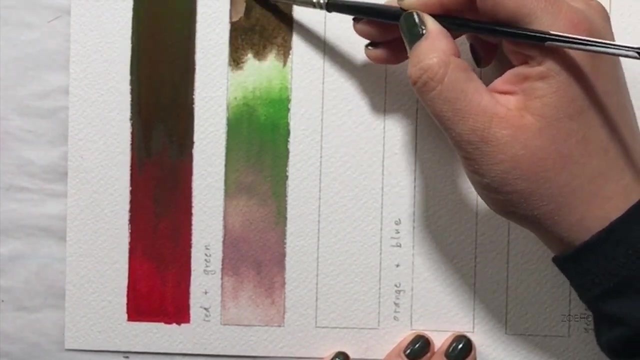 And again, it all depends on how much gray you know. you can have something that's a lot of gray, something that's a lot more green, So that it's just lightly dulled down or borderline. So this bar, I'm showing you just just a tiny percentage of the colors that you could create by using red and green and white and black. essentially, 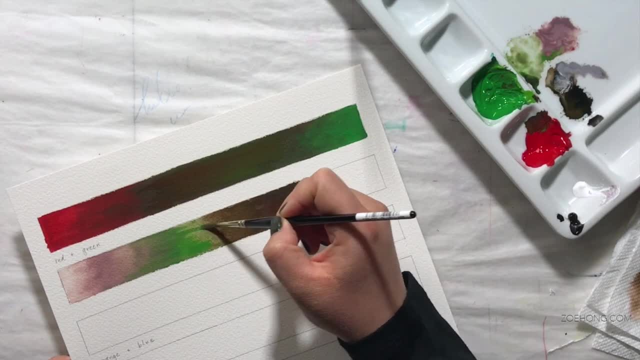 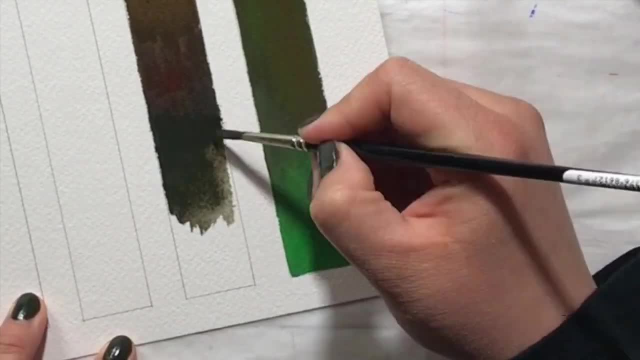 And then kind of lines up with these, these nails here, the strokes that you might need to put in the background, that you want to avoid being cute, So you might not have to be over very dark default. but then you'll have this. today will continue to foundation or contrast these colors. 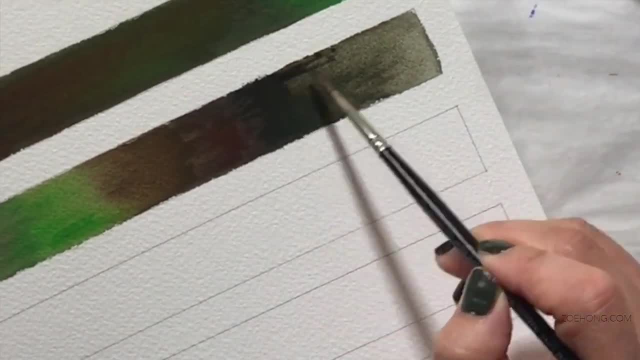 Great. I will tell you about it in a minute, but it's worth coming back to and passing through, Thank you. So here's another setting And we'll give you a Berger Terrence, which is perfect. Maybe it's not too light. 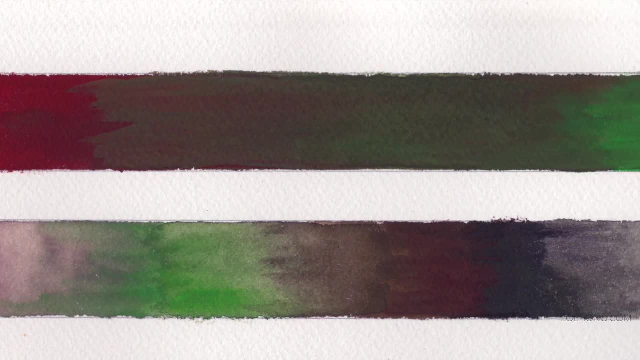 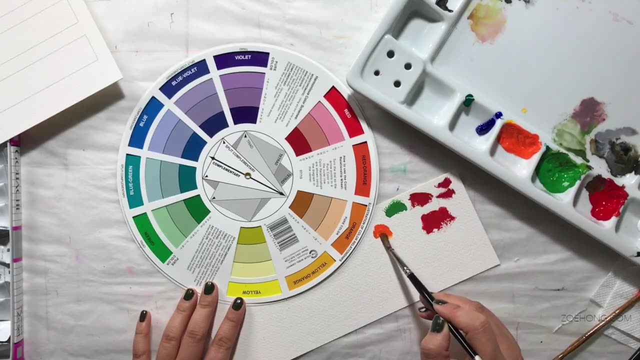 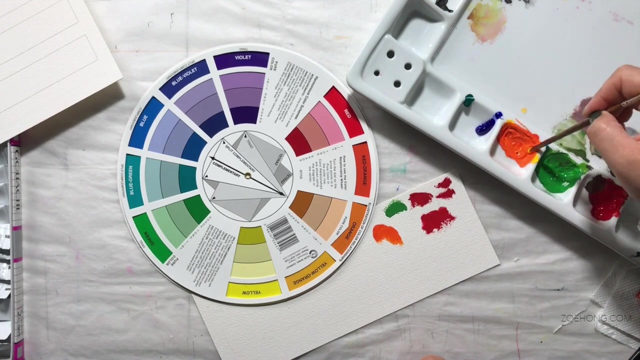 This was the hands. Okay, We'll stop there a minute, Tim. Sorry, I'll just jump back in, Tim. Thanks, Thank you. you too, get back to doing that one at a time. Before I paint each of these mute bars, I mix the colors to match the color wheel that. 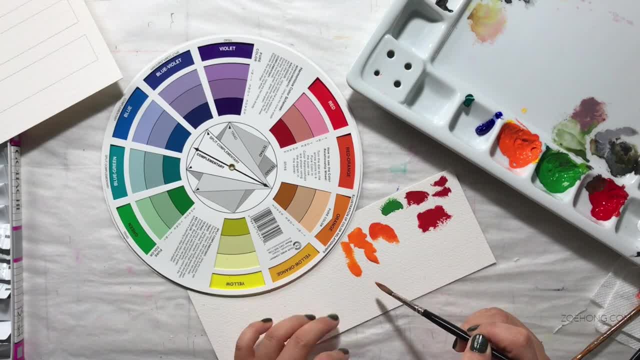 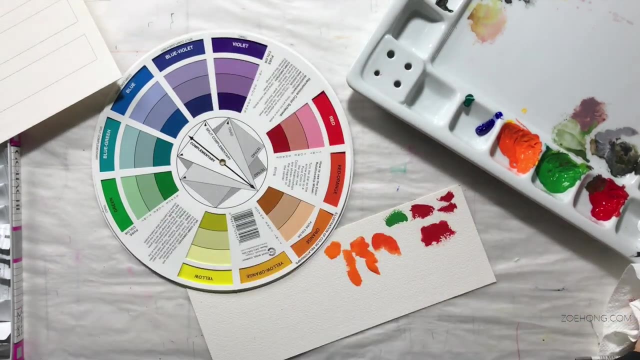 I'm using just so you all are seeing some kind of consistency. So of course I have orange and blue tubes of paint, but they're not the oranges and blues on the color wheel. So I'm just, you know, I'm throwing in a yellow into this orange so that I'm getting a closer. 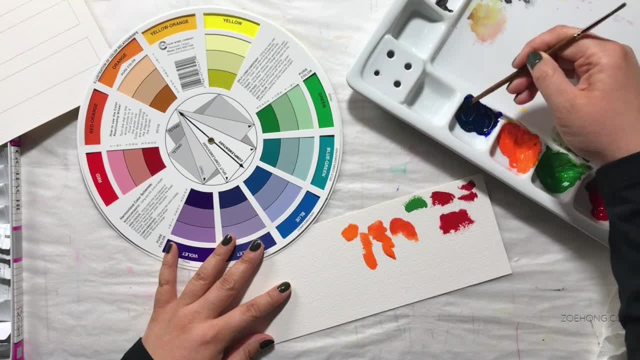 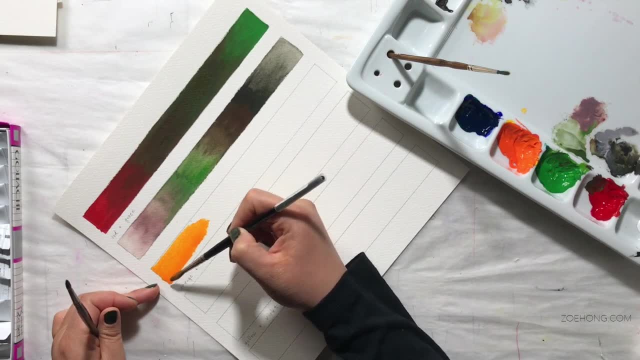 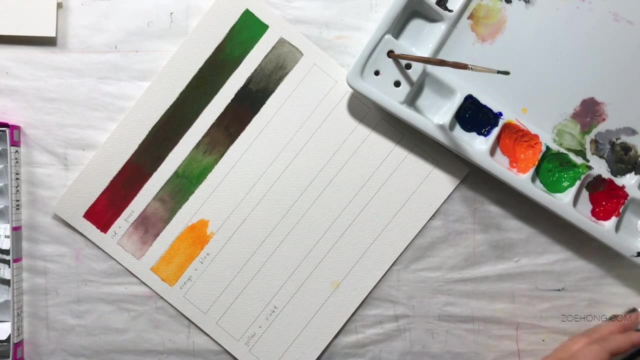 match to the color wheel and then I'm going to try to get the right blue. Now I am doing the orange and blue mutes color bar, mute bar, gradient bar, bar, bar bar, And again adding a little bit of the blue is going to mute down that orange. 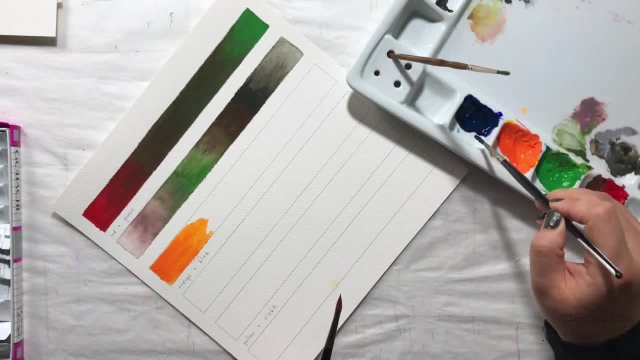 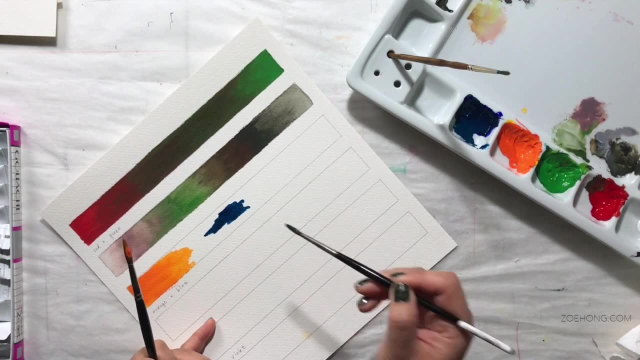 And adding a bit of the orange will mute down the blue And when you get to the middle, okay, you're going to end up with a different, warm, neutral than you did with the red and green, because you know some people think like well, when 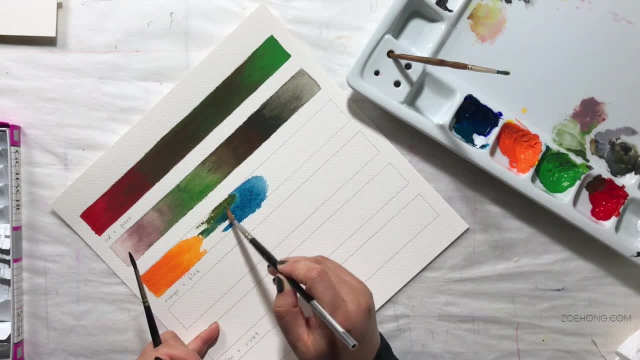 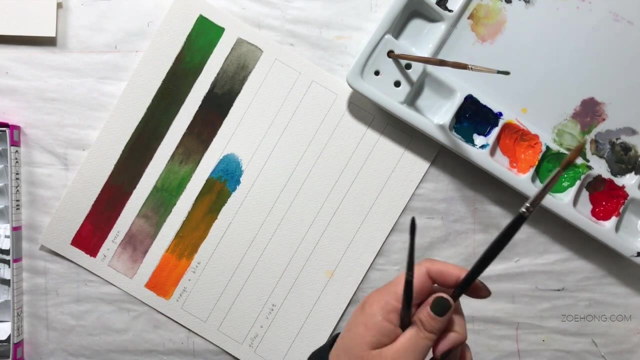 you get to the middle, you're basically have red, yellow and blue all up in there, Because when you have red and green, you have red and green is yellow and blue right, And then you have orange and blue, Which is orange is red and yellow and then blue. but it's the different quantities and 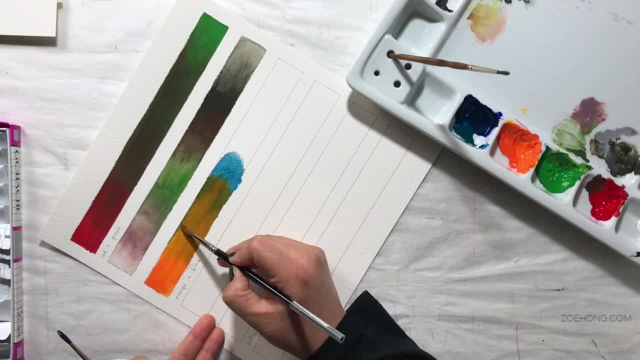 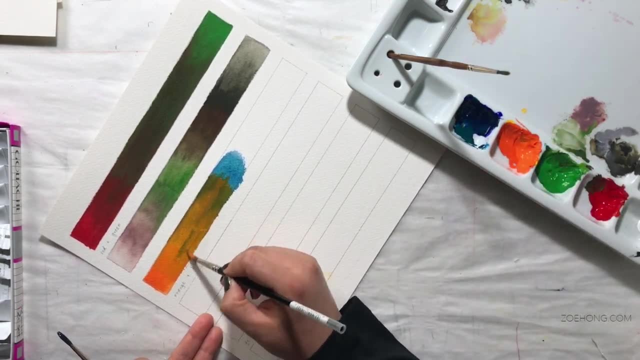 ratios of the colors that create the different warm neutrals, different browns. So when you mix orange and blue, you're going to get a slightly different brown than you would mixing red and green. Also, it's nice to have options And so when you are trying to get a nice brown that goes well with orange. 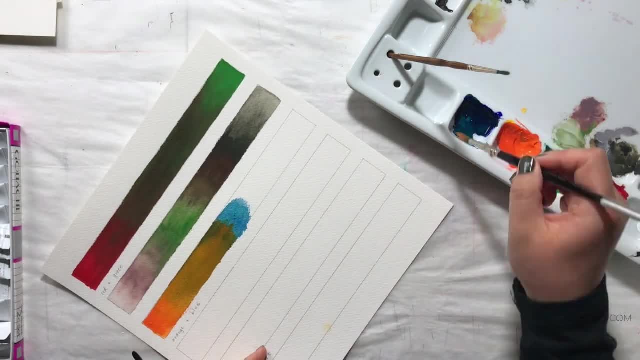 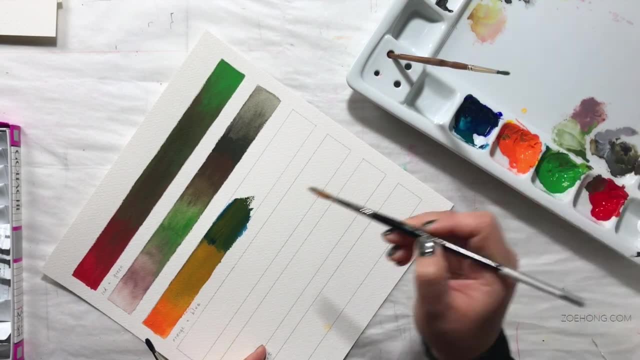 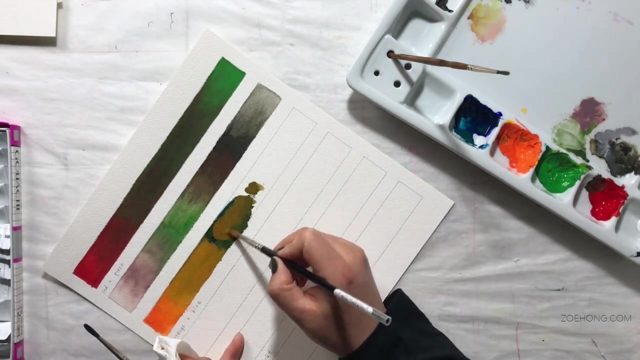 And you want your undertone family to be all the same, I would recommend that you create a brown using orange, with blue And again with the green. if you want a brown and a bunch of warm neutrals that all share a greenish undertone, then I would suggest that you start with the green and start adding. 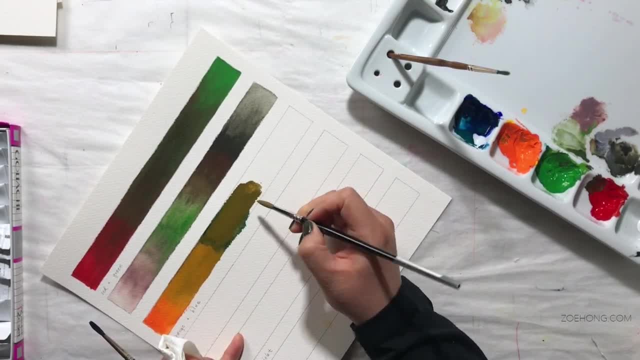 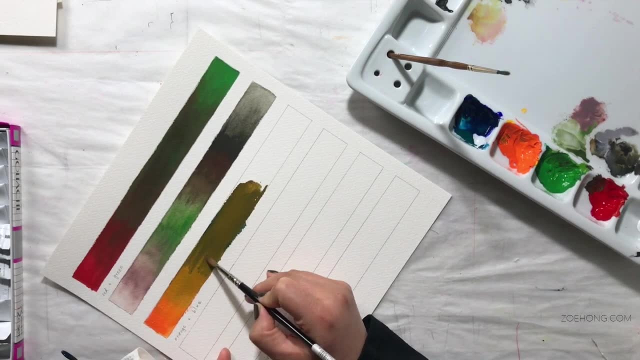 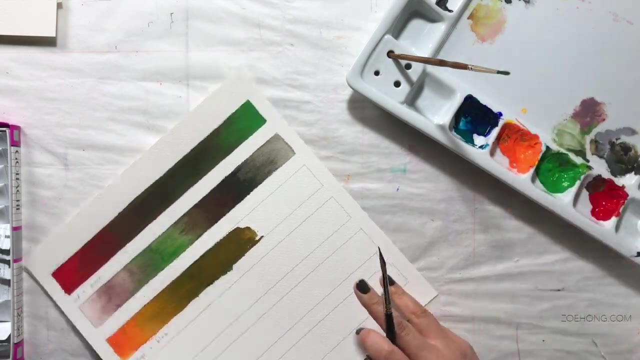 bits of red and, you know, maybe a little bit of black, as needed. Now, a thing that's very different from the orange and blue mutes, To the red and green mutes, is values. Remember, value is the lightness or darkness of a color. 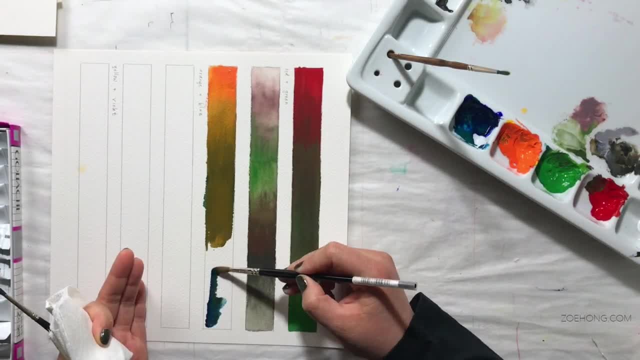 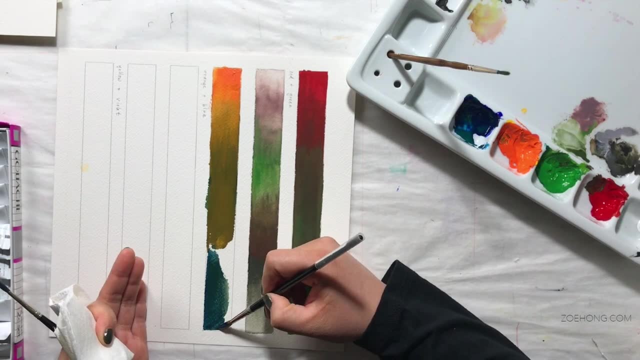 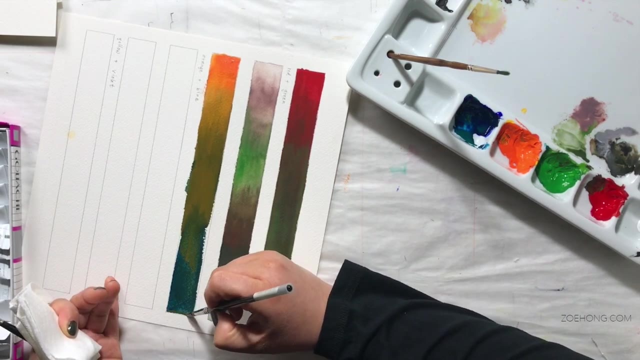 And so when you're mixing these colors, the value becomes very important. Blue is a very dark color, So adding a little bit of blue, this very dark color, dark value color, to orange is going to impact the orange a lot, Because the orange 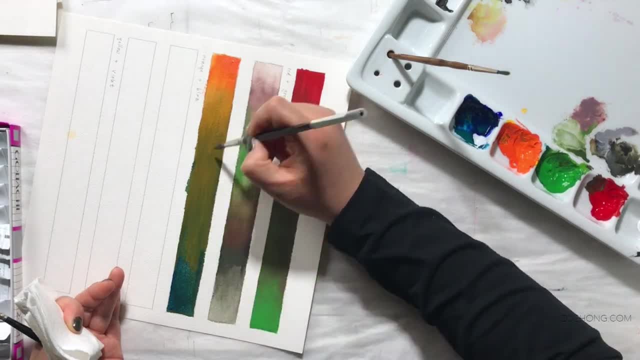 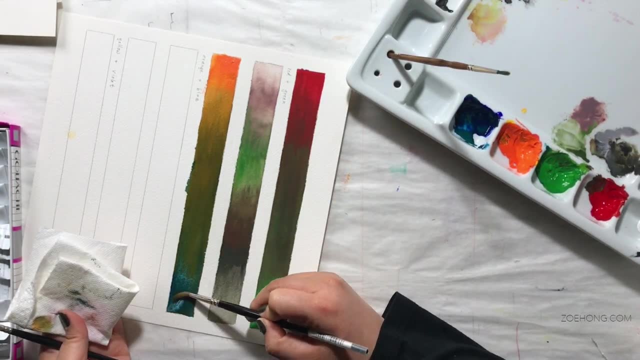 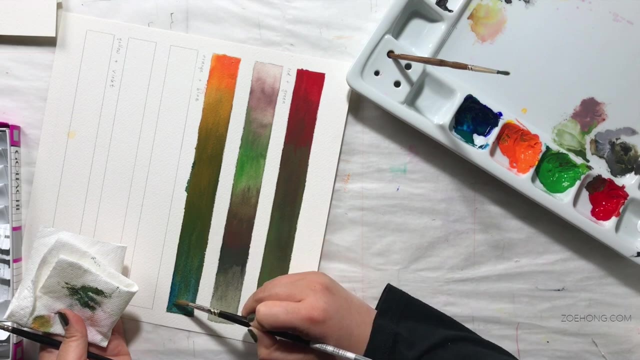 Orange is only at like 40% And this kind of straight up blue is more like 70, 80% right, Whereas the red and green they're pretty similar in value, Like when you look at the straight up green and the straight up red, one is not significantly. 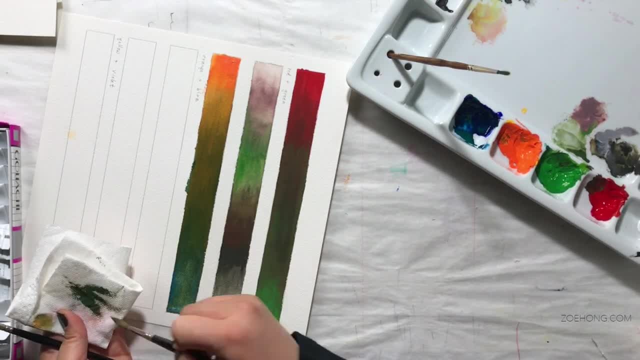 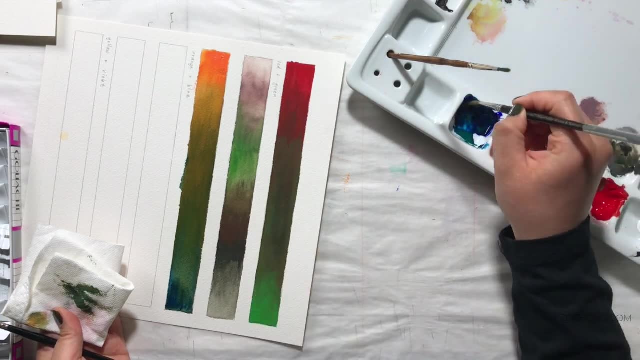 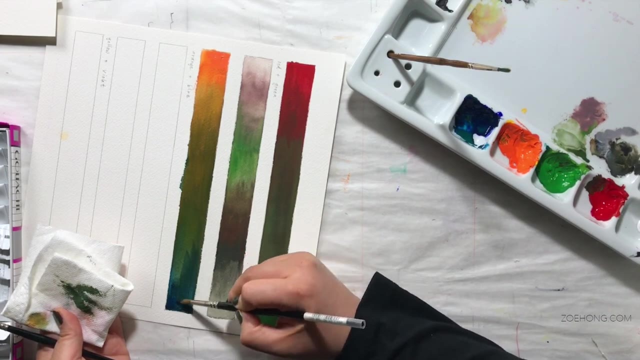 darker than the other right, Whereas with the orange and blue the blue is significantly darker than the orange. So when you are mixing your oranges and your blues, remember to chill out on that blue. Keep a conservative hand on that blue, because it will really overpower the orange very quickly. 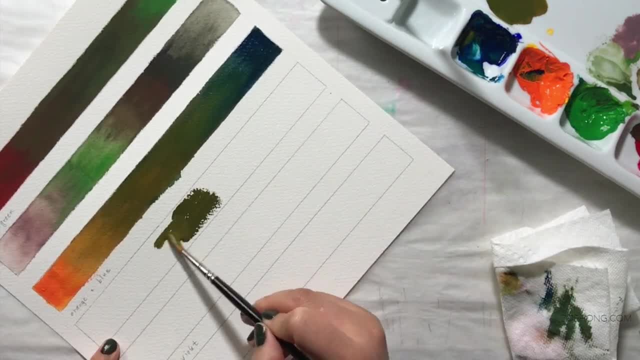 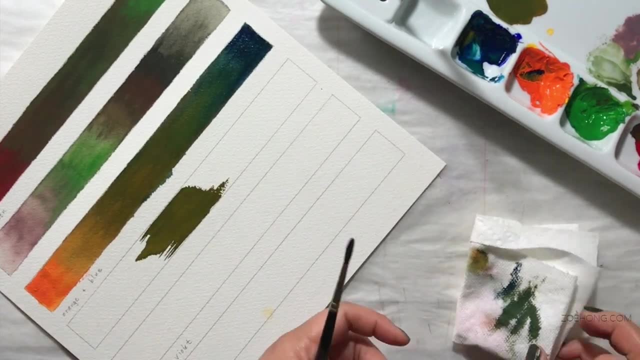 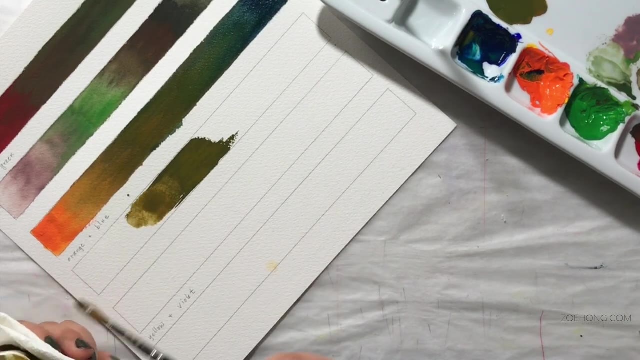 And here again I am mixing mutes and also tints and shades and tones of mutes so that you can get another few ideas on how to create these colors. So I've taken the mute and I am adding more and more water to create tints of mutes. 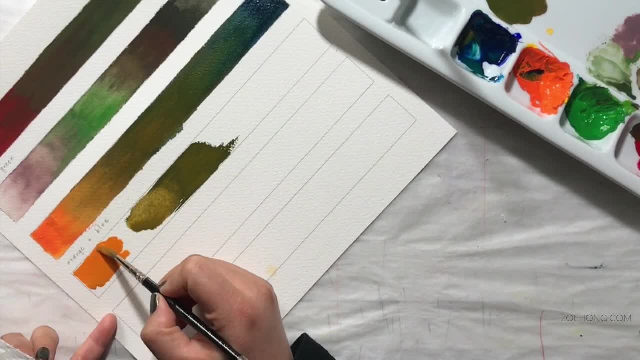 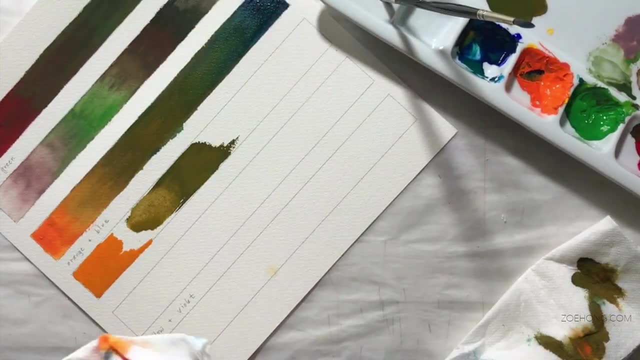 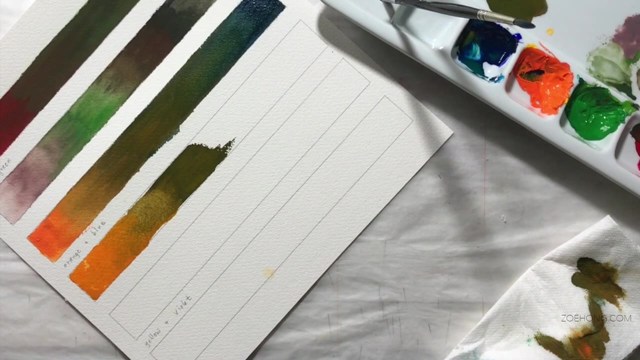 And you can see how these colors lightened up. Like You can see the differences in the browns and the undertones a little bit more clearly. Yes, No, Hopefully It's okay, It doesn't come overnight. You know, you have to kind of increase your eye sensitivity by practicing looking at colors. 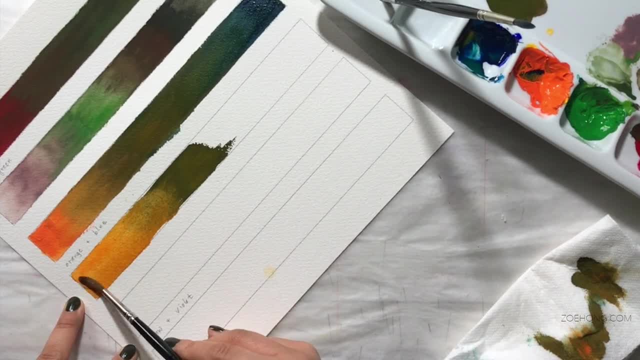 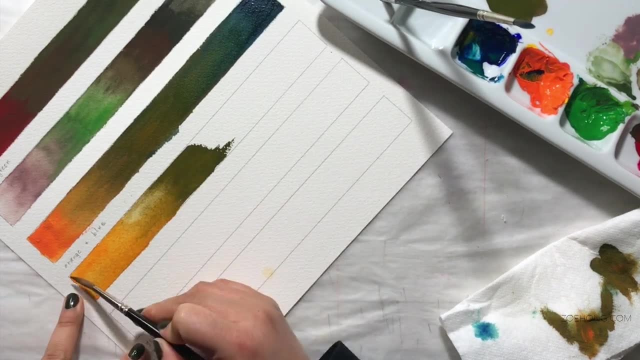 Okay, That's what I do a lot in my color classes: Make my students practice looking at colors. And so here we are with the orange. I'm adding a lot of water, So you're getting a tint of orange. Okay, A lot of orange going into tints of mutes. 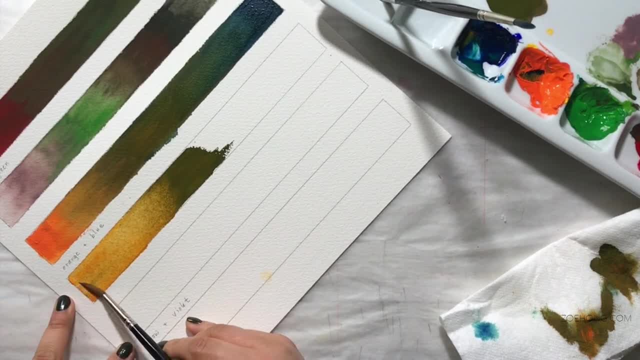 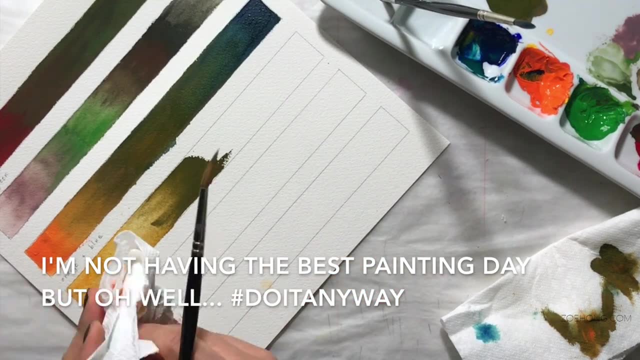 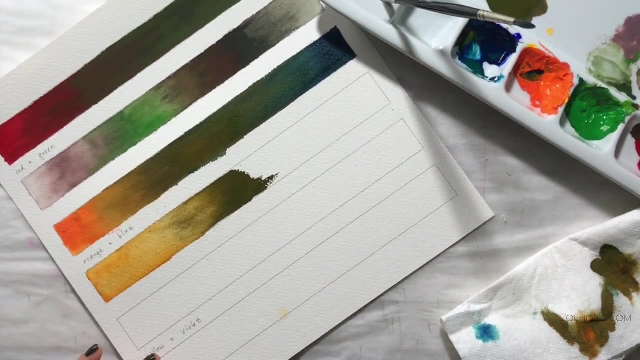 And now you're seeing these. they're greenish because they're more orange than they are blue. But again you get these like khaki, olive-y colors that are again really different from the mutes of greens mixed in with the red. 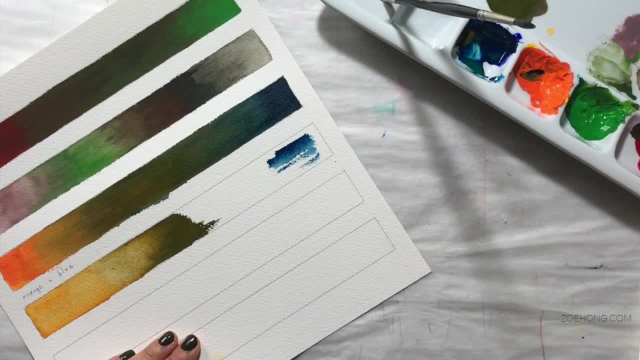 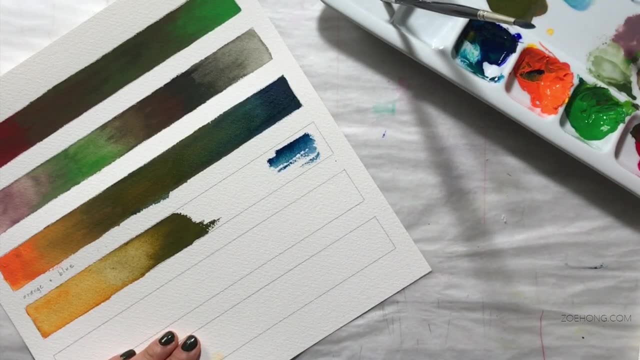 And now, on this side, we are doing. what am I doing? Oh, I'm adding in some gray with my blue to create tones of mutes. Tones of mutes, of shits and tints. Did I say shits and tints? 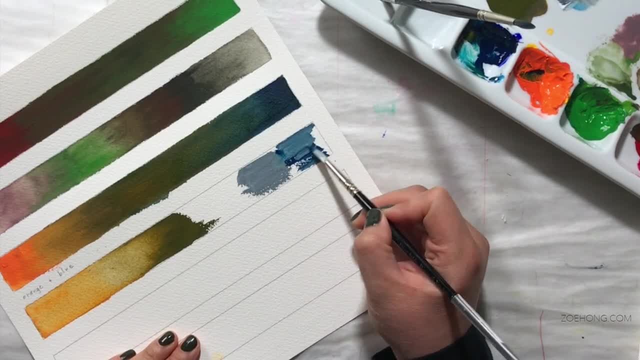 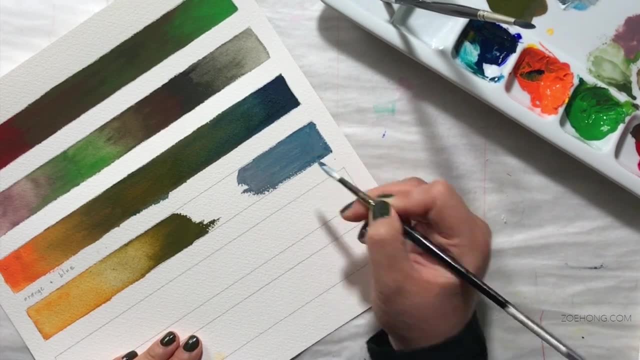 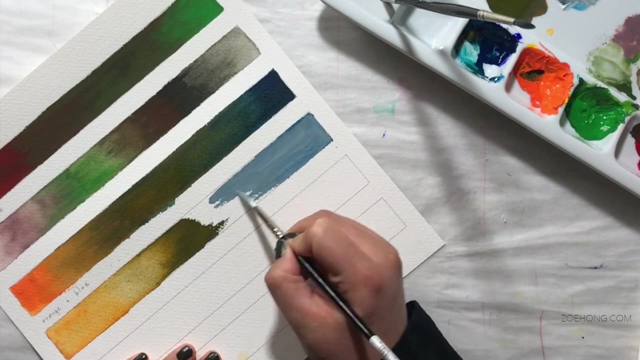 Good job, Zoe. Oh my God, My boss one time asked me if I wanted to teach a high school class And I was just thinking to me they're thinking like, oh, Even my husband was like I don't think that's a good idea. 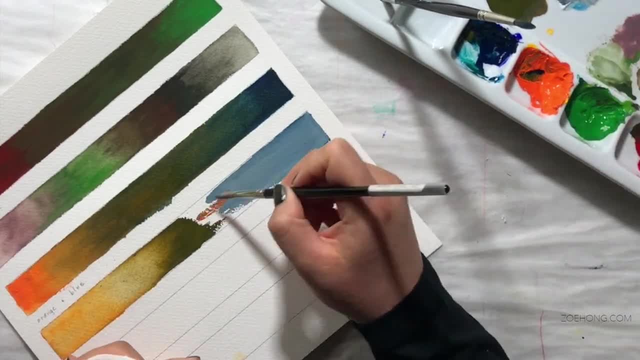 Like you with anyone that's young, I mean even 18 year olds- That's just. I don't think that's a good idea. Like you with anyone that's young, I mean even 18 year olds, That's just. 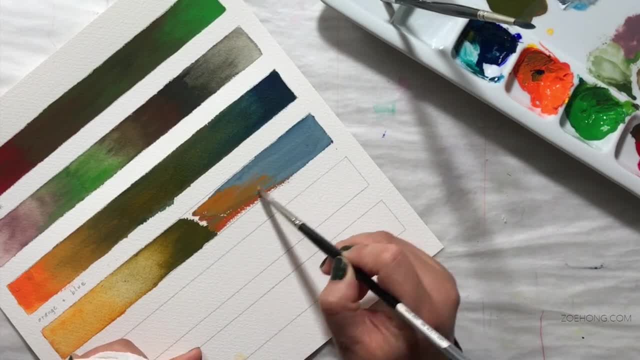 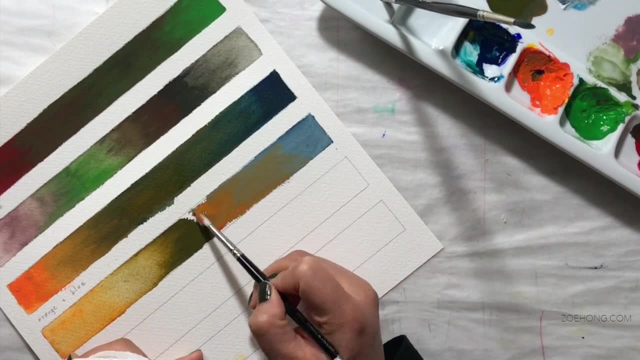 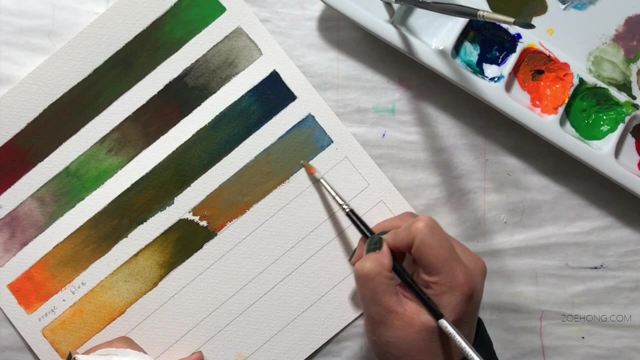 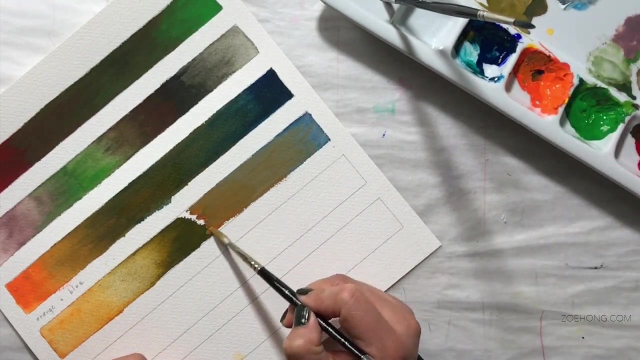 Because, again, you can't edit in person. Anyways, here we go. We have created mutes, but with a white gray, And so I've lightened the blue a lot. The value of the orange is a little bit darker because the gray is kind of close to the value. 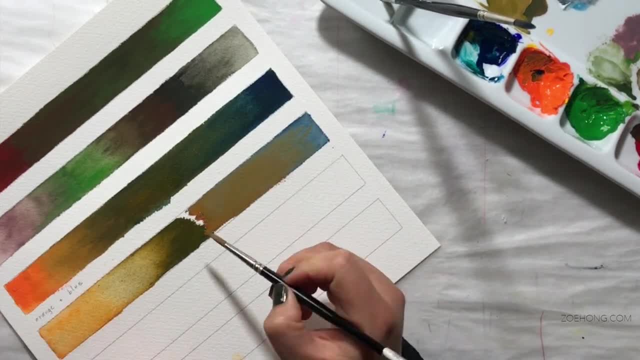 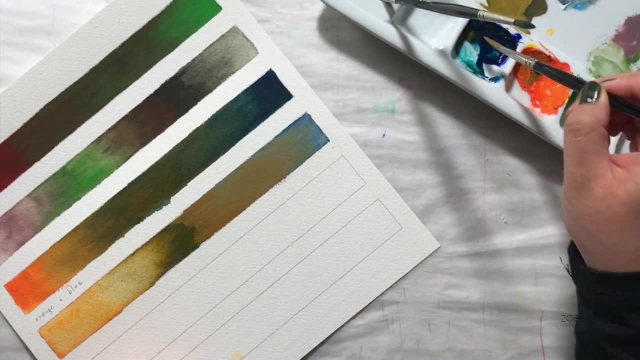 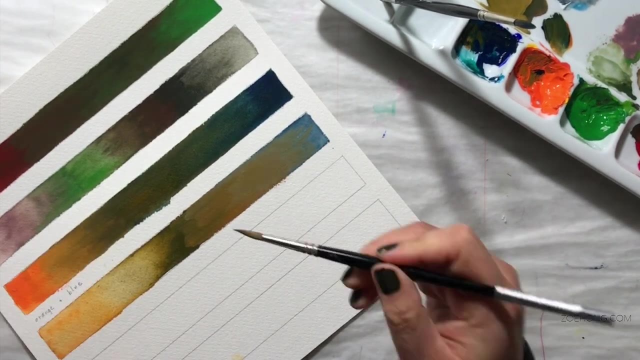 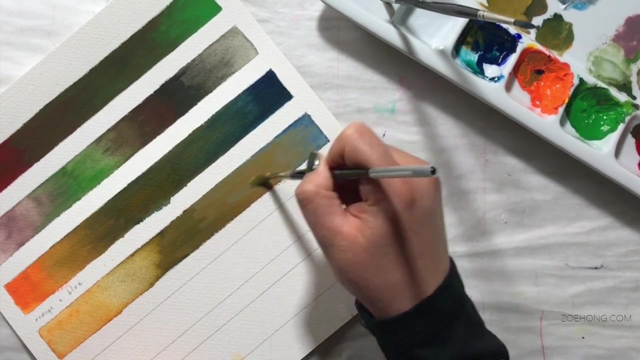 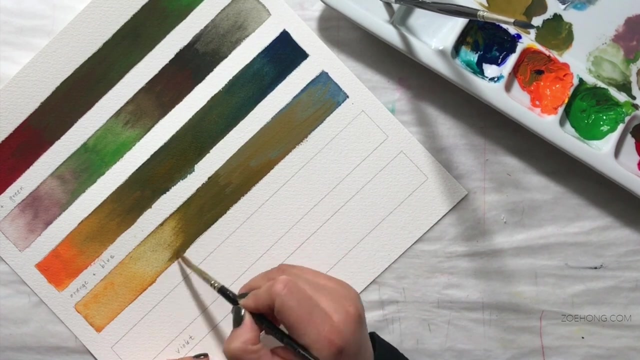 of the orange, And now you're seeing these tints. Oh wow of a mute. Now you've got these awesome dull blues and cool browns, One of the umber sepia kind of family. I don't know, I'm not great with those words. 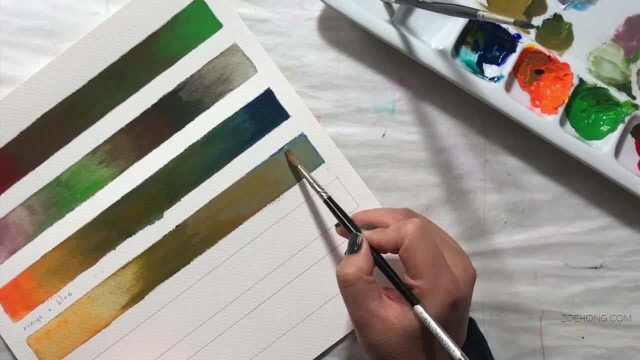 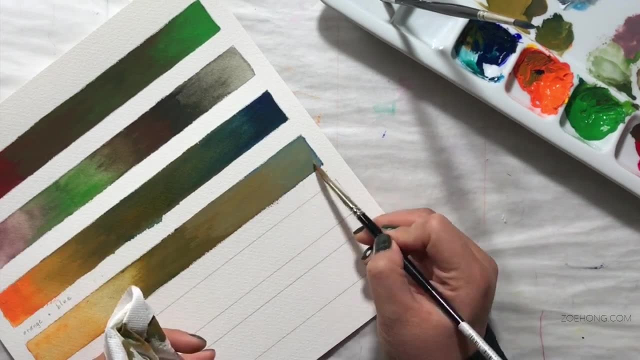 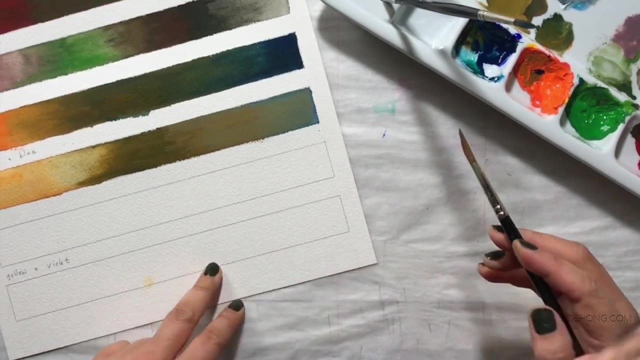 I just like when I talk about color, I like being very explicit and saying: cool brown, warm brown, cool gray. Those things make more sense to me than trying to use branded names. I used to have this job and we did a lot of leather. and people don't get super adventurous. It's not like I blame them. Leather is typically an investment piece. You'll buy a leather jacket and wear it for many years, or hope to wear it for many years. Not a lot of people will buy. 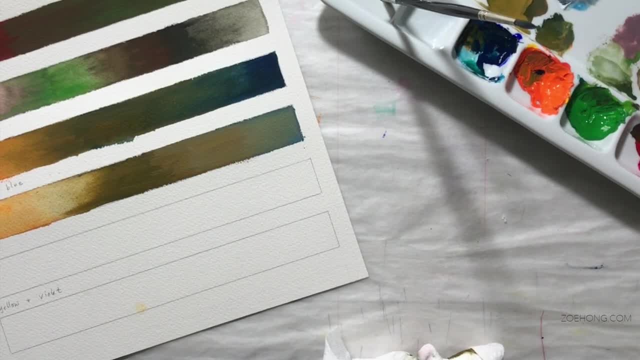 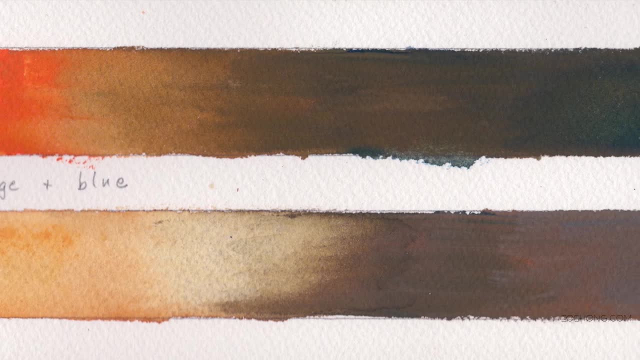 a raspberry pink leather jacket, but they tend to stick to browns and blacks Every season. you have to make it new and exciting. We would have to sit there and come up with new and exciting ways to tell people: this is our new dark brown and this is our new light brown. 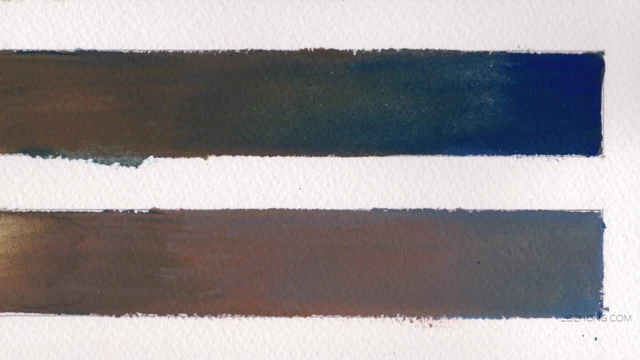 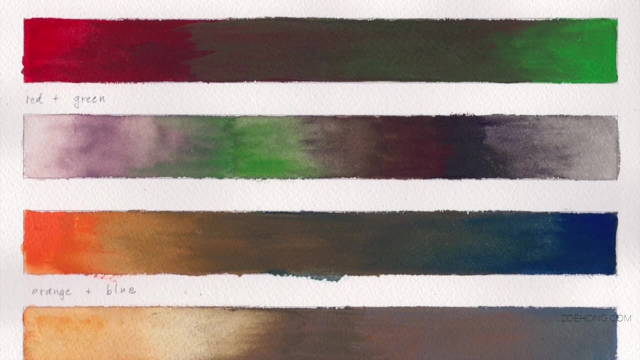 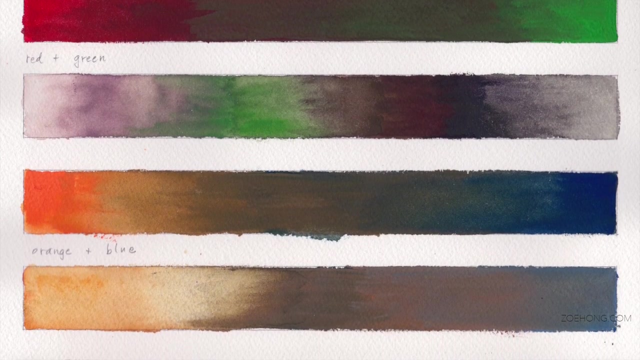 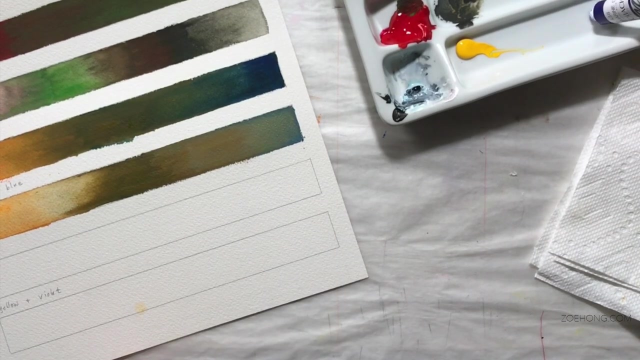 We would sit around and think of ways. different words for brown. We resorted to a lot of really just smoking and drinking things. We had tobacco, we had whiskey, scotch amaretto, coffee, espresso. A lot of these are great. 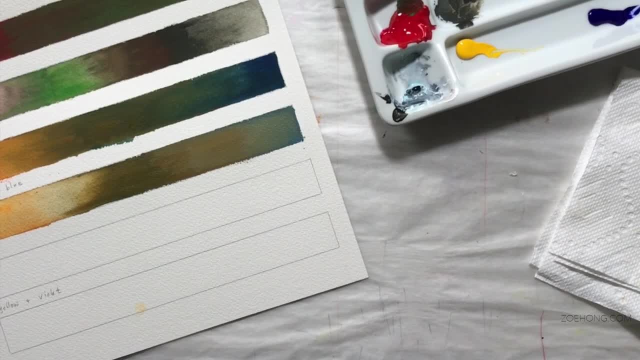 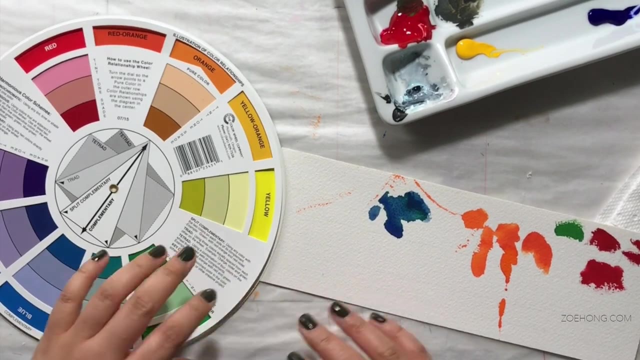 brown descriptives: Espresso being like your darkest brown Coffee being just like slightly under that, Amaretto having a little bit more red in it. Whiskey getting like a little bit light with gold undertones. So many browns, So many colors of brown. 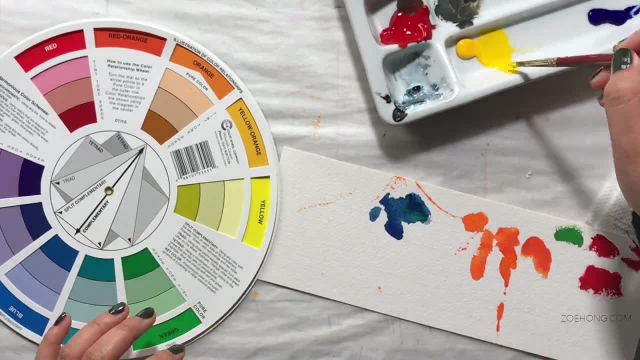 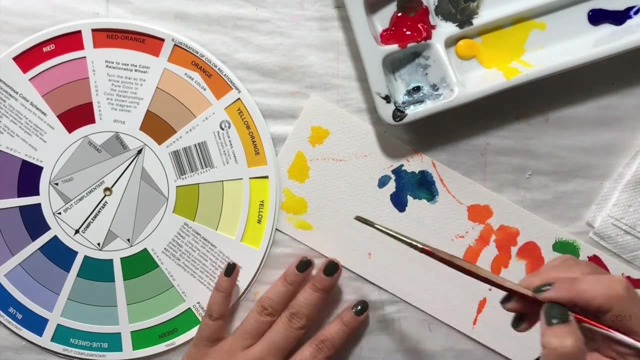 Then you get more caramel, cognac, butterscotch. Then you start getting hungry. You want a candy. You're in this meeting listing browns and you're like, okay, let's take a break, and everyone goes back to do their own thing. 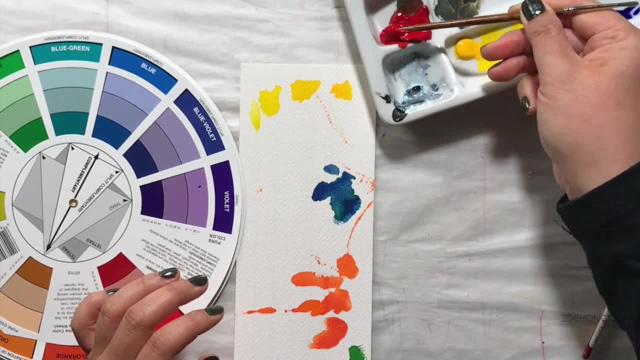 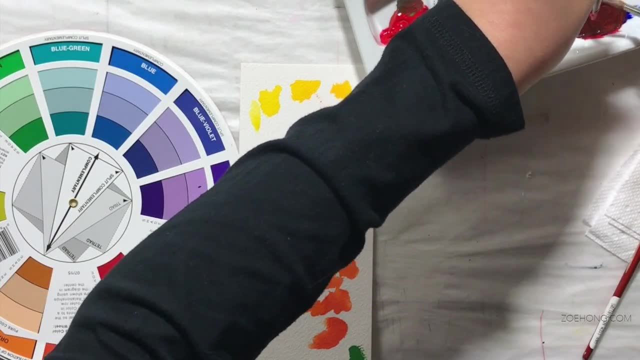 Then someone hops into your office and is like: oh, I thought of another one, Browns. So many words for brown Brown, brown brown In color class, in design class. I like to talk to my students as, hey, let's do a more. 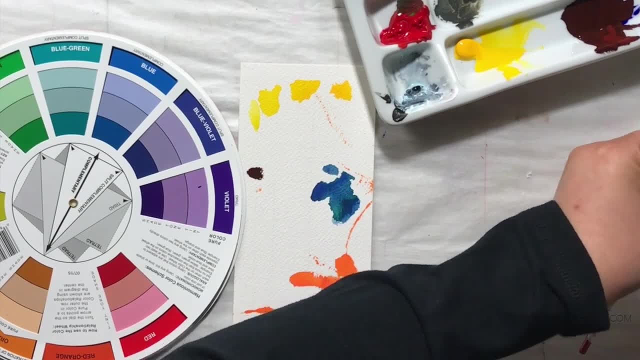 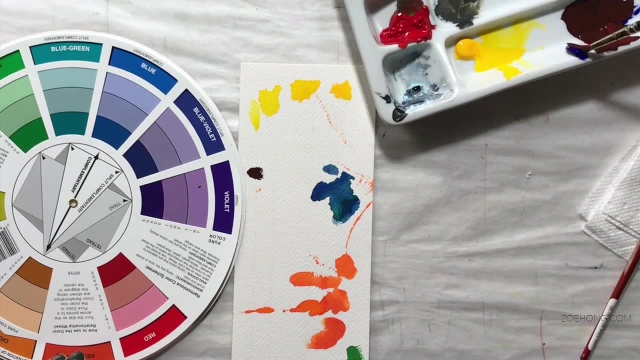 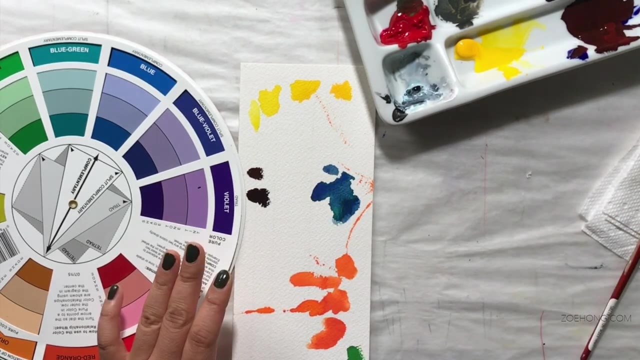 reddish brown, Let's do a more dark brown. I think that actually is more helpful. But you know marketing, branding, making things exciting and stuff. Now we are doing the yellow and violet. This mutes and again I am adjusting my paint colors to. 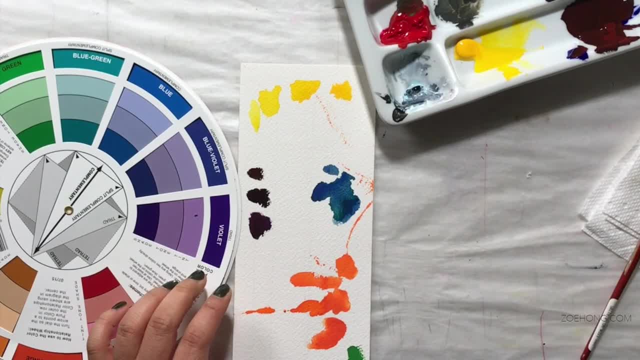 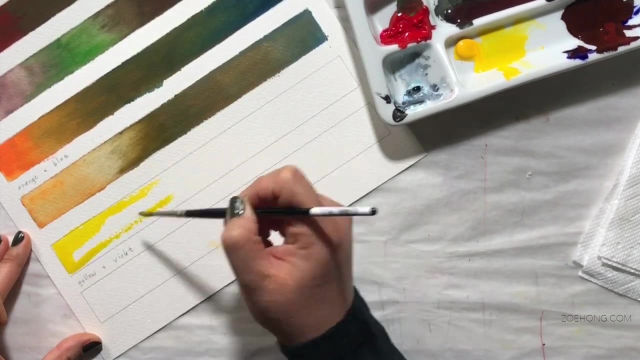 match up with my color wheel. and yeah, I think I kind of really struggled with the violet because it was very, very different from the color wheel violet. Not to say that my paints are wrong, That's just the cream I had And the violet and the. 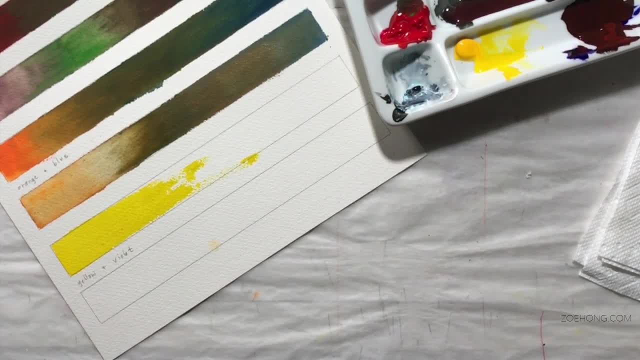 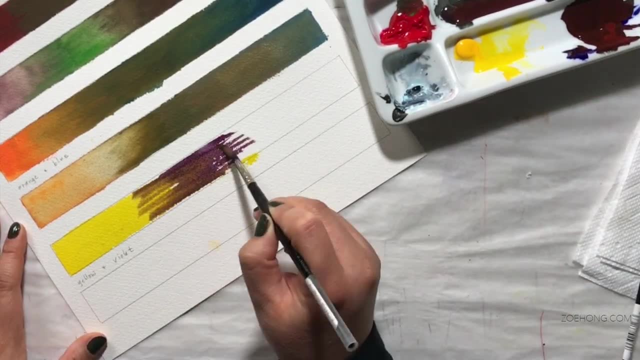 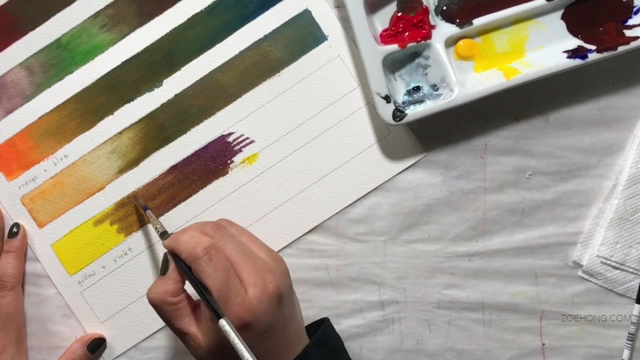 yellow. their values are even more extremely different than the orange and the blue. Okay, Yellow tends to be like a 10-20% value and the violet is your darkest on the color wheel, which is at like 80-90 give or take. 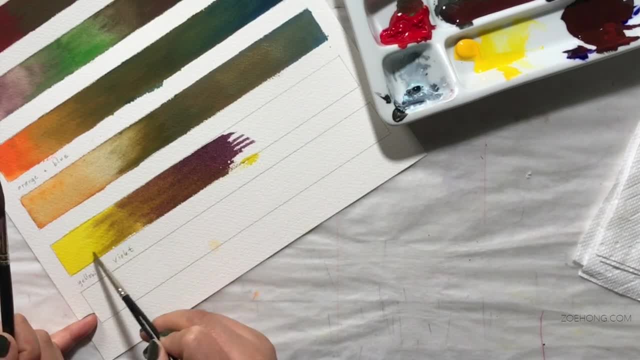 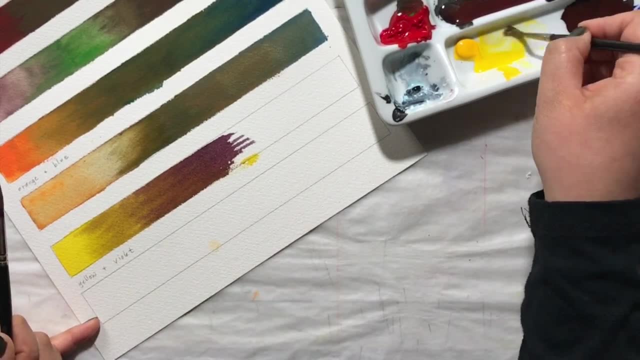 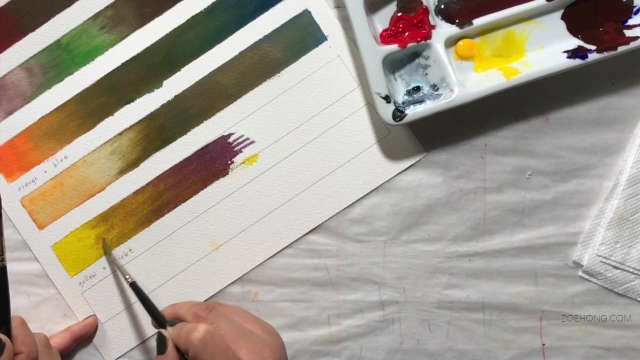 As I was saying before, be careful when you start adding violet to yellow, because the violet can be overwhelming really quickly if you add too much. So keep a light touch on that violet. So to review one of the reasons why people like compliments so much: 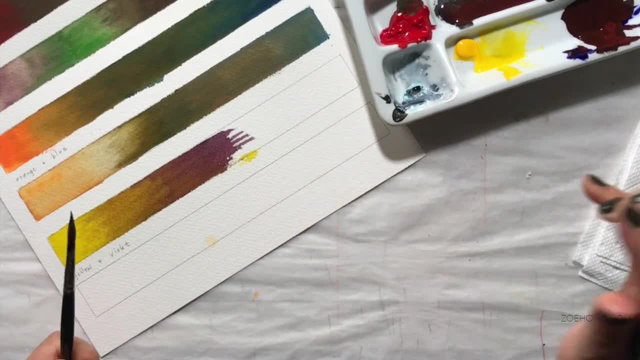 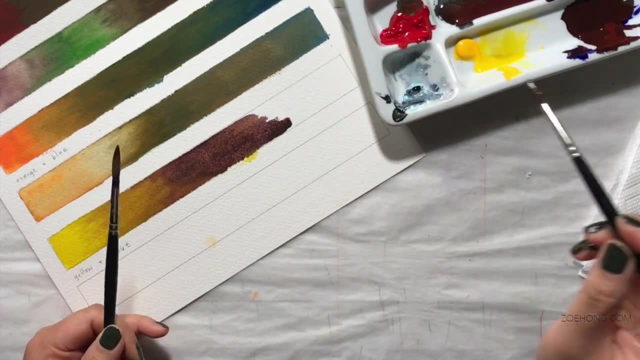 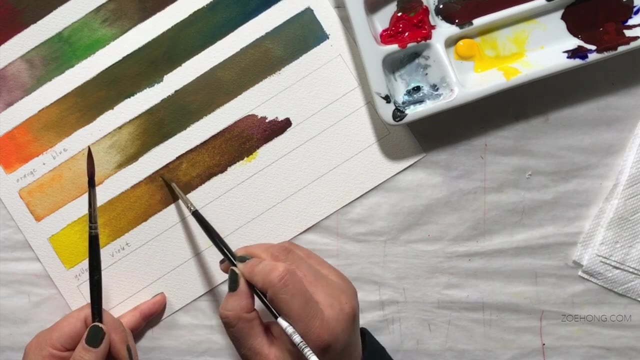 is because they're opposites on the color wheel. They offer the most contrast to each other, which makes the contrast pop more, And so when you put blue and orange together, the blue looks bluer and the orange looks oranger. Someone asked me. 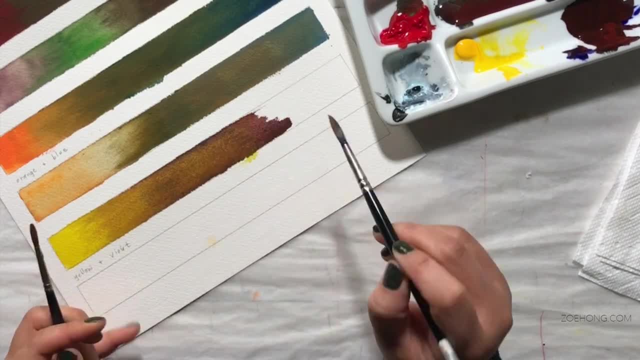 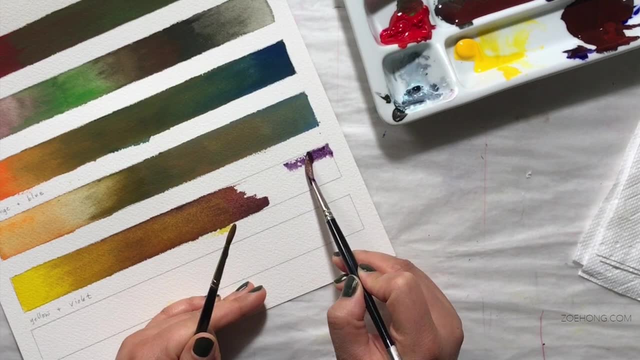 to sum up color theory in one concept Like: what's the point of understanding color theory? It's just colors. It's like: well, the whole point of color theory is to see how different colors go with different colors, because when you put certain 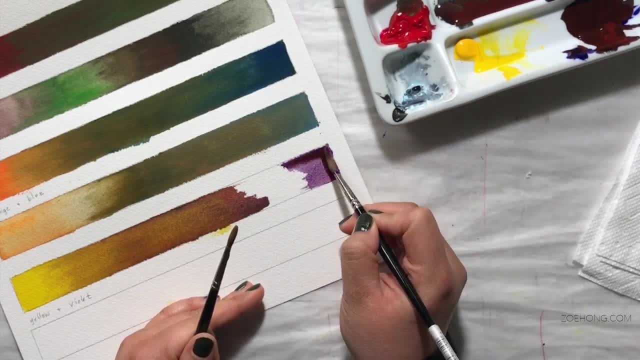 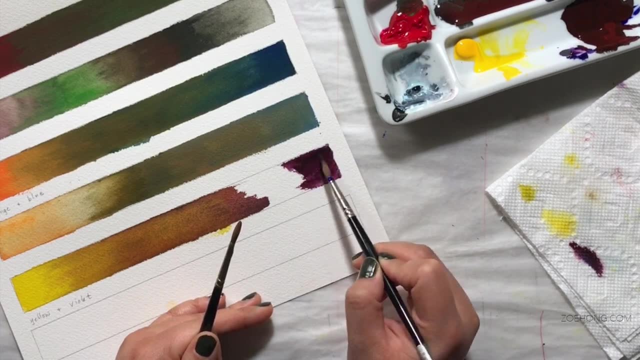 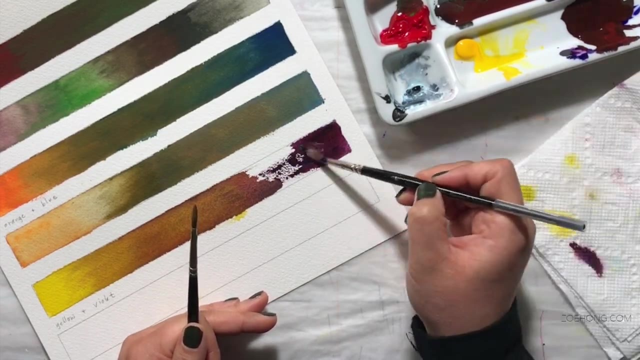 colors. with different colors, the color itself looks different. For example, when you put orange next to blue, the orange really pops and the blue really pops because they're opposites. The contrast really makes them pop. Okay, When you put blue next to green, 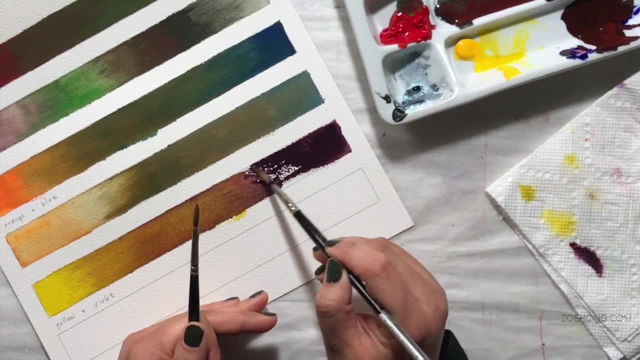 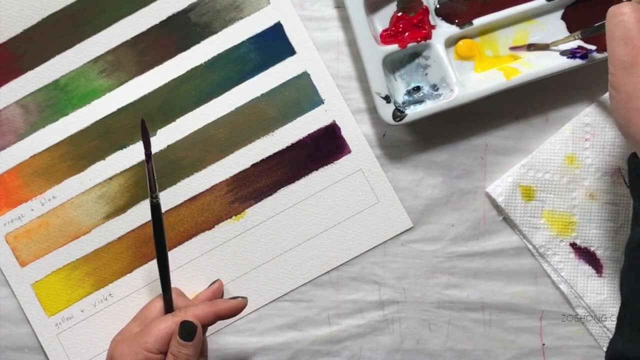 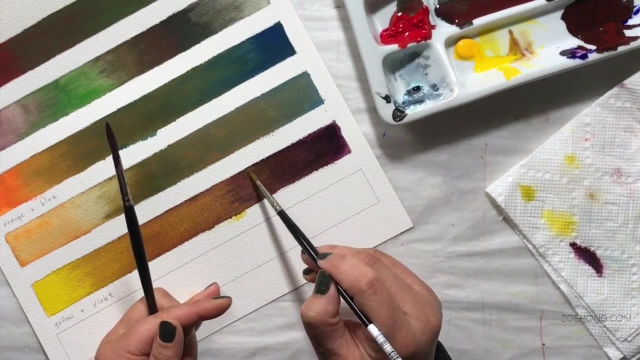 they look harmonious and they start blending in together. Neither of them really pop. When you look at a lot of movie posters, their whole goal is to be eye-catching and so they will employ compliments a lot so that the color contrast and the pops really catch your eye. 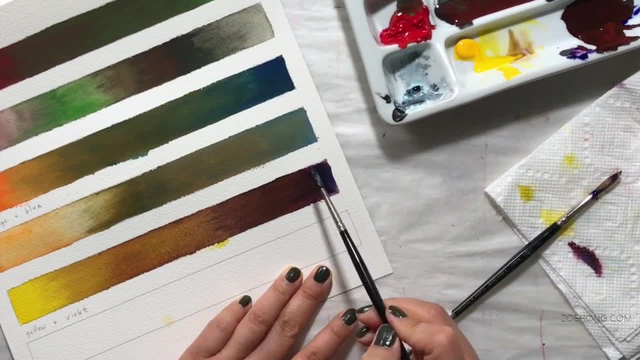 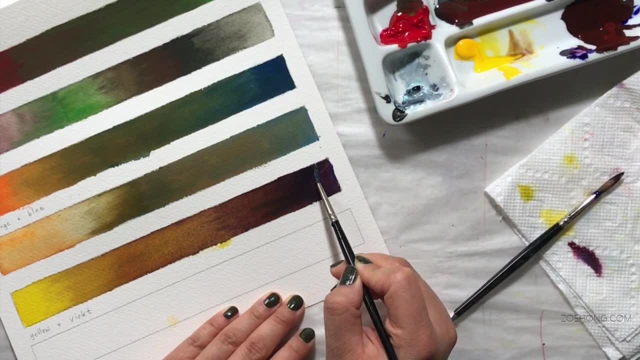 Okay, Next time you go to the movie theater or a mall where there's a bunch of movie theaters, look at some posters and see if you can spot the color schemes that they're using and why they're using them If they want like. 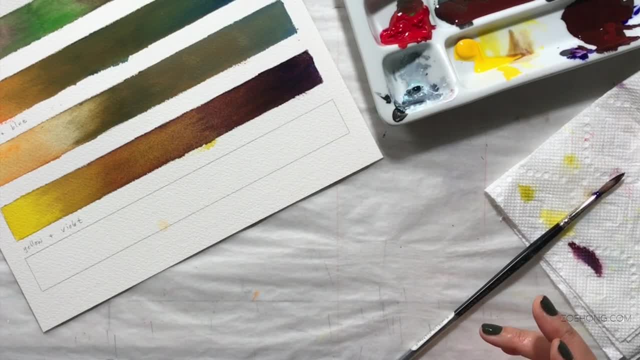 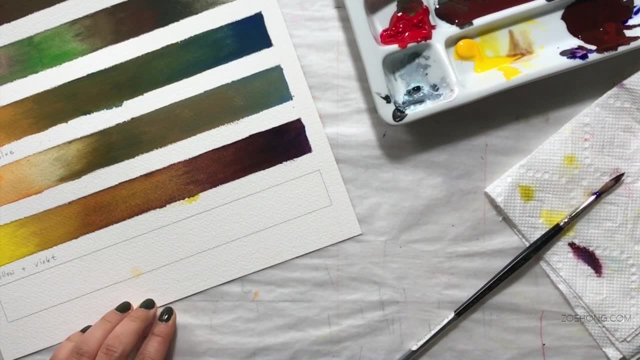 a lot of the time when they want something that's more like this is going to be a slow, winding drama. they'll use more colors that are harmonious and closer together on the color wheel, And when they want something that's going to be more, 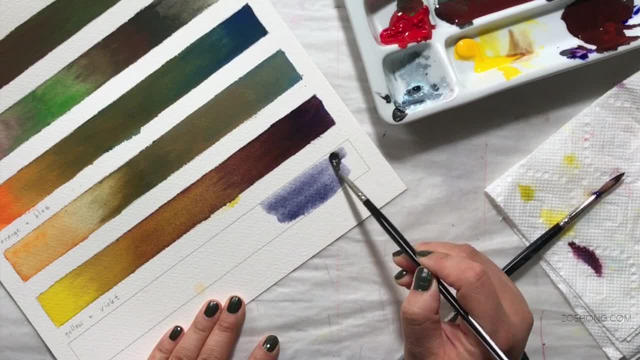 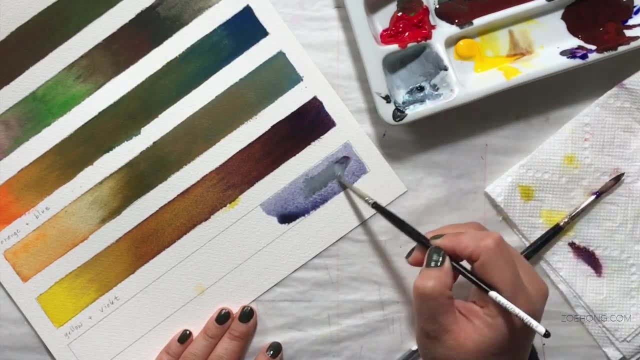 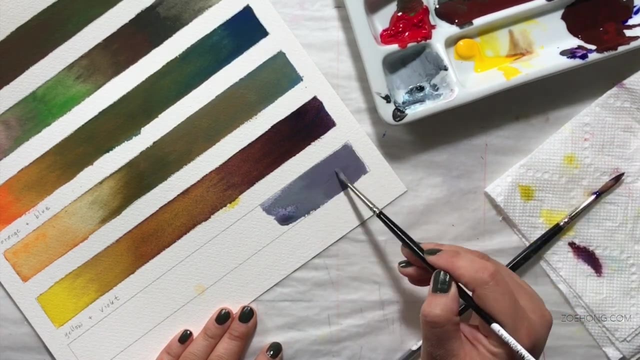 action, drama, things exploding. you're going to see a lot of orange red fire with a lot of this blue green kind of background landscape, A lot of blue glass skyscrapers exploding with like orange flames shooting out. you know, like that. 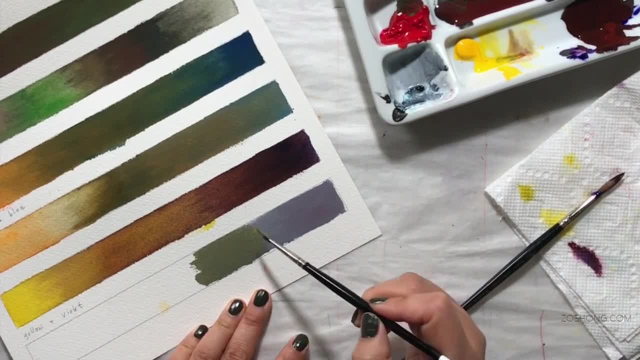 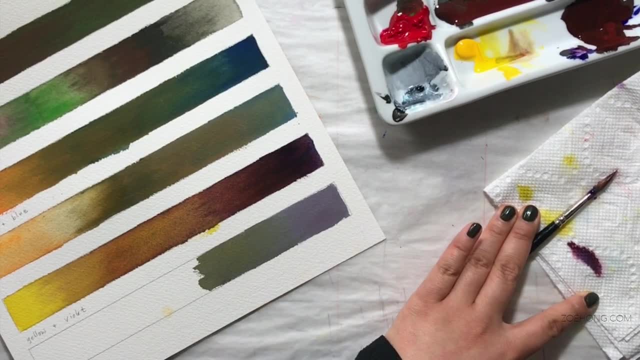 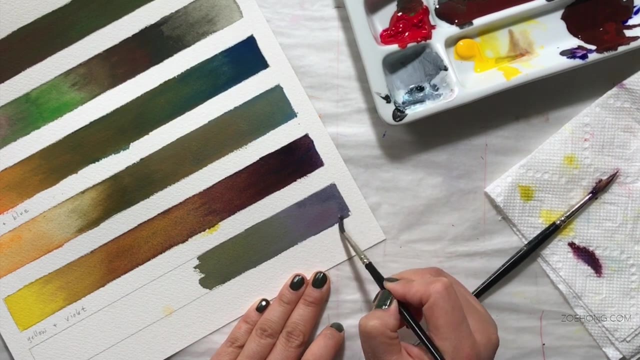 kind of thing. So compliments make things pop. but there is a harmony to that, because they're exact opposites. opposites attract something, something, And so when you start muting them- okay, when you have an orange and a blue, and then you have like 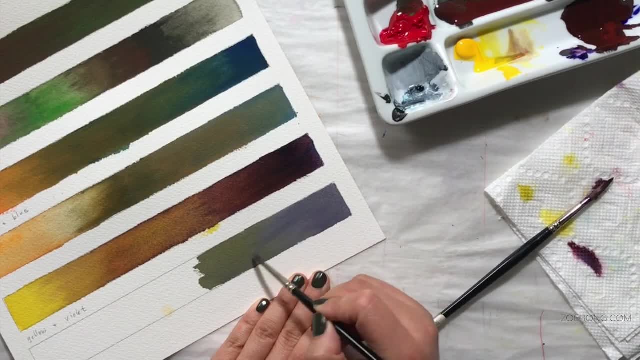 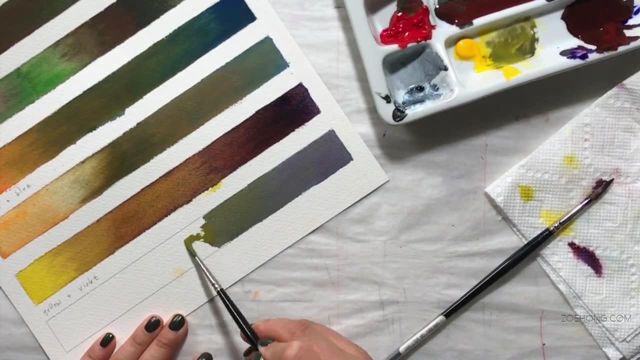 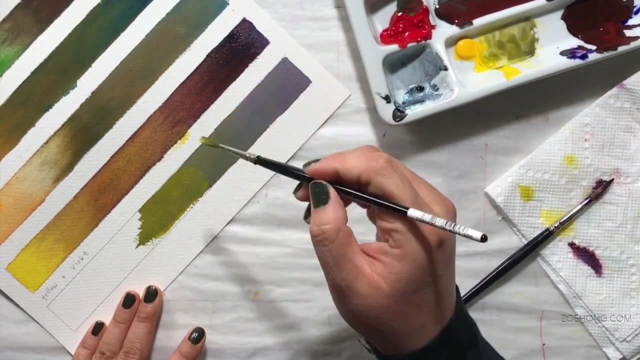 a muted orange and then some browns that have orange and blue in them. then you're starting to get similar undertones And you're starting to create a family of colors that work well together despite the fact that they're so different. And again, in future videos we're going to 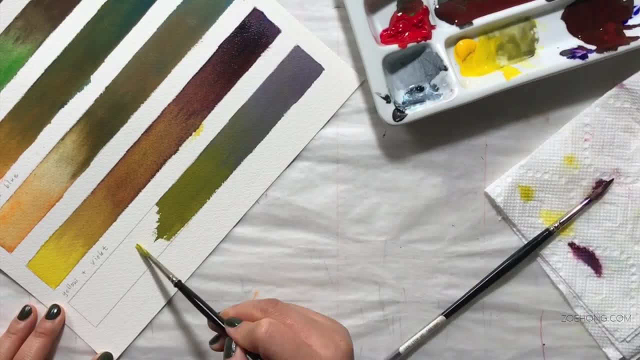 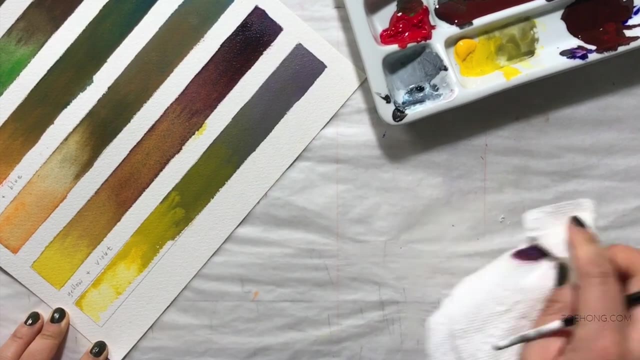 we're going to talk more. We're going to, like I could talk about color theory until forever. So I mean, as long as y'all are continued to be interested in studying color theory, I will keep making videos going into color theory. I think color 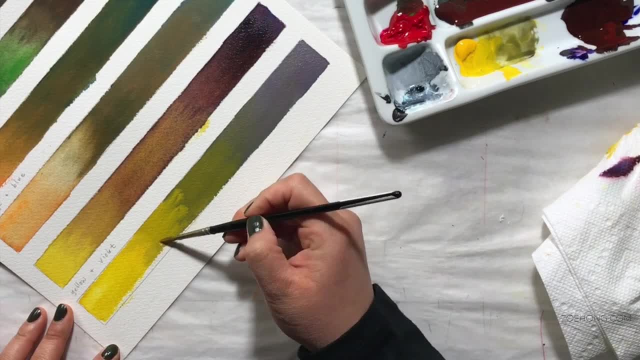 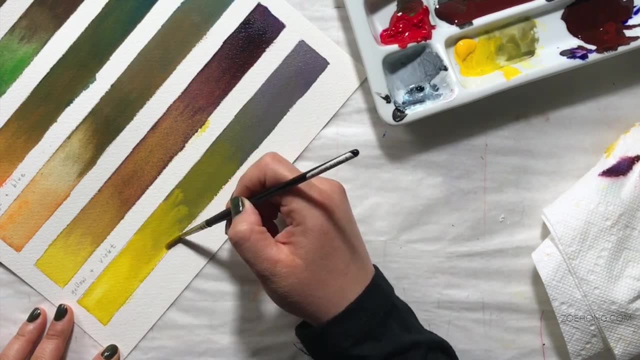 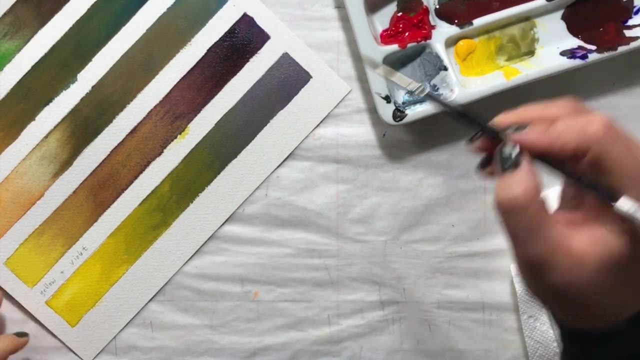 and understanding color is so important, not just to fashion design, but to any kind of visual art or design: product design, graphic design- because color is number one thing we notice about any product, whether it's a wearable or not, When you walk into a store. 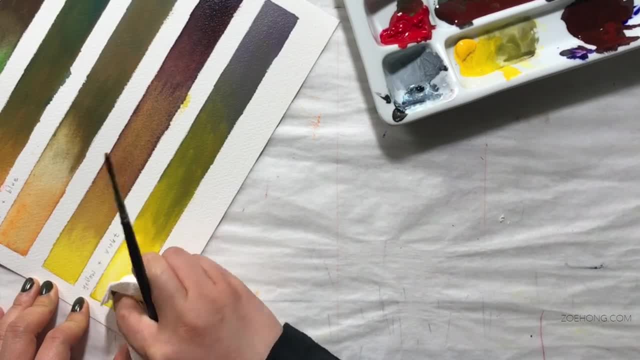 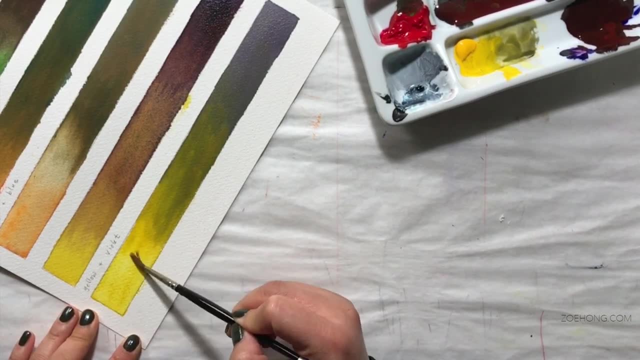 and you're looking at a bunch of clothes. what is the thing that makes you gravitate towards something Nine times out of ten? it's going to be the color. You don't know if it fits you right, yet You don't know how the 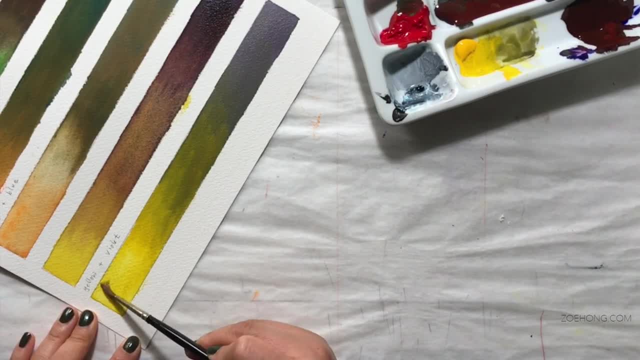 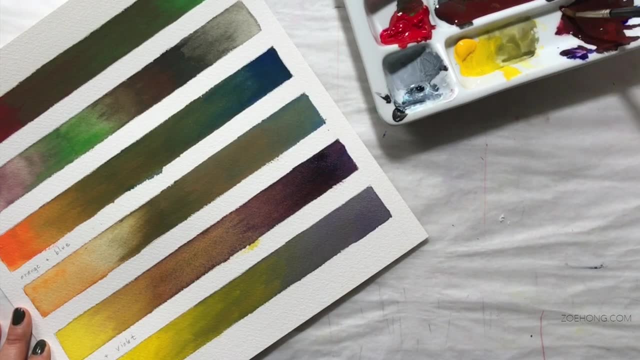 fabric feels, yet You haven't even been over there to touch it. You don't know if it's going to make your butt look good. You don't know if it feels really great against the skin. You don't know. you know unless. 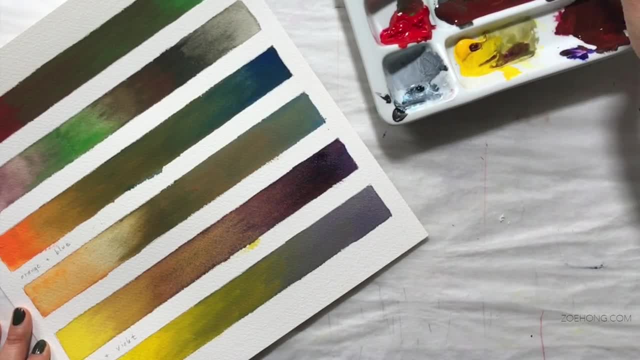 you go to a designer specific store. you probably don't know who made it, but that color is going to attract you. It's a color that you love. It's a color that you hate and you're just looking at it because you're like: why would? 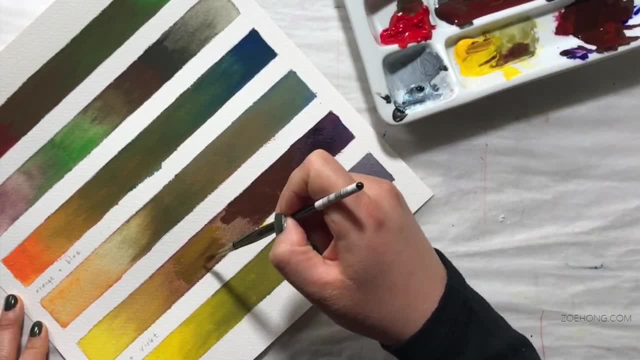 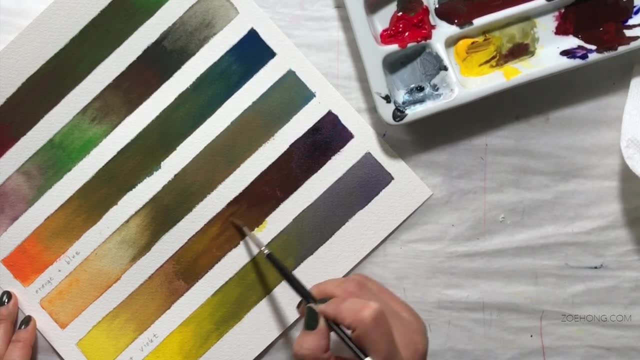 anyone make that color, But the color will attract you. You're going to look at it and be like, oh, that color is great. Or oh, that color always looks awesome on me, I want it. Or oh, it's black, I love it already. Okay, that's. 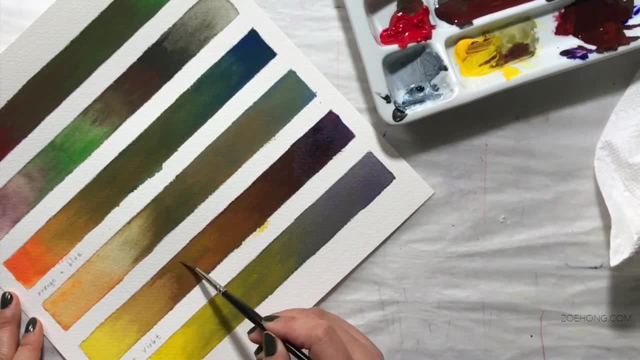 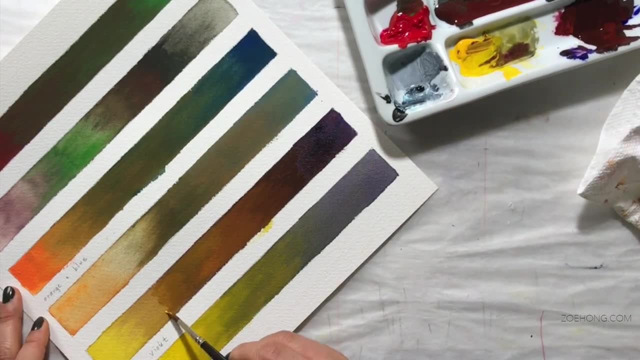 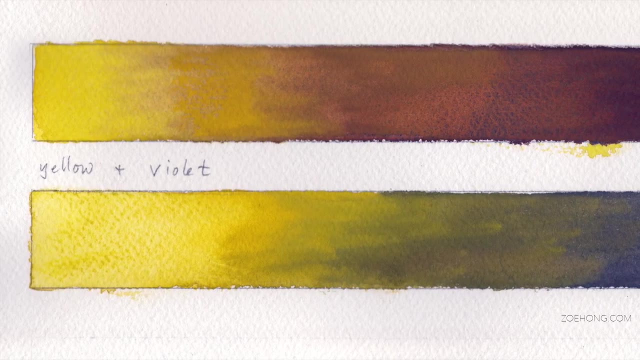 just me. So getting the color right in clothes and collecting clothes and collections in your products, Really important. So again I can talk about color theory for 800 years. Yeah, So again this last bar. it is what was I doing. I was adding. 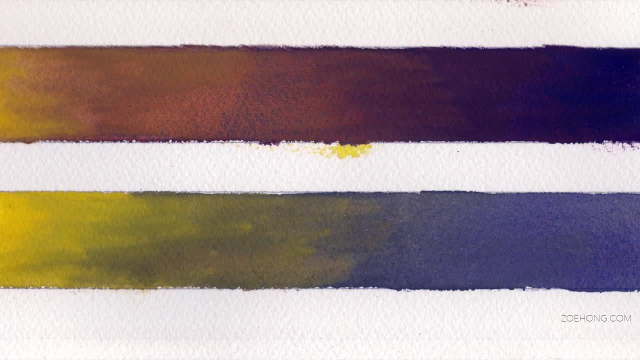 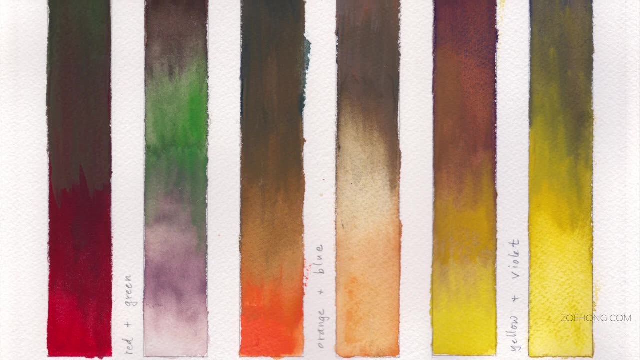 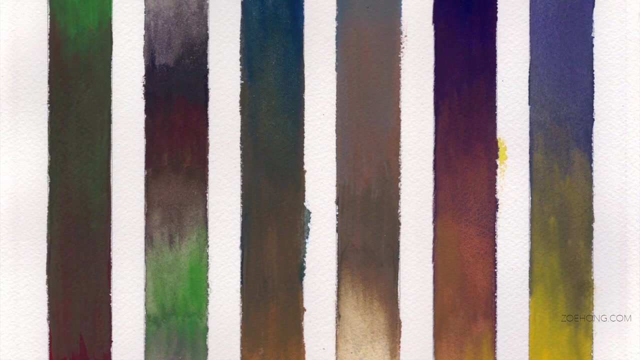 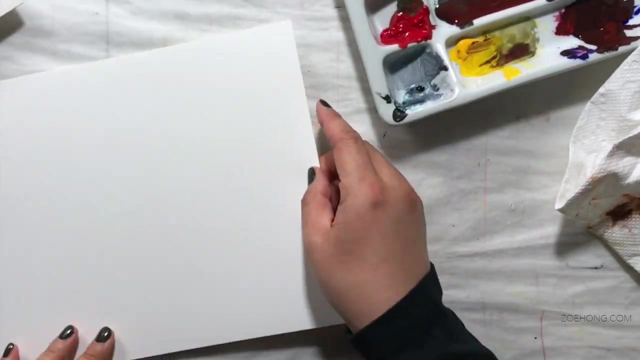 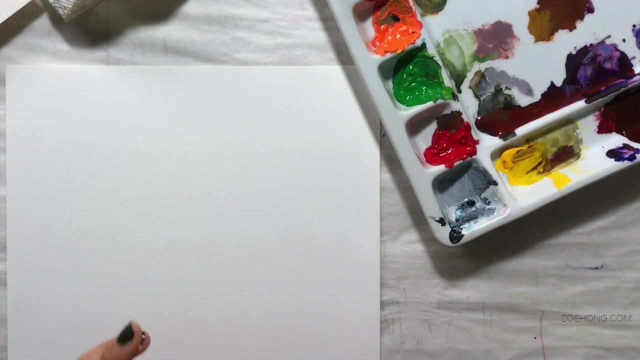 tints and shades and making tints and shades and tones of tints and shades and tones. So I'm just testing out a little scrap piece of the Fabriano paper that I bought in LA. It's really cheap paper. It's super, super smooth, Not the cold press paper I was using. 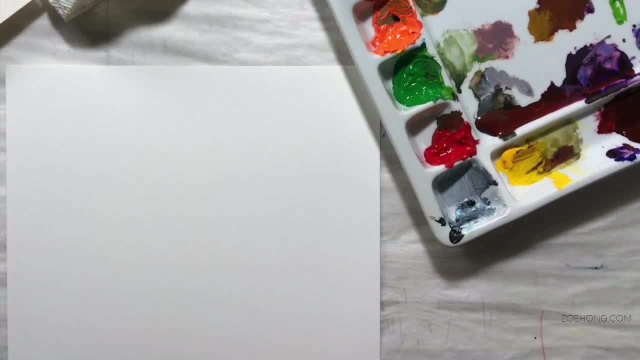 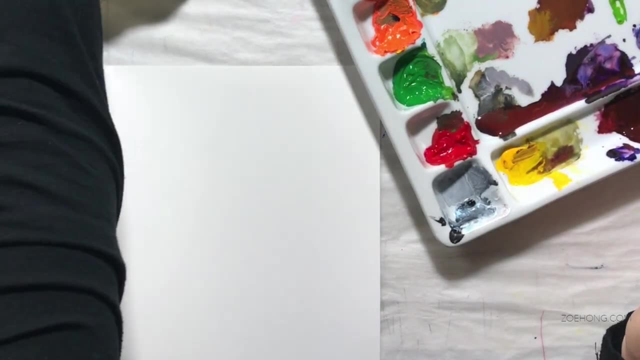 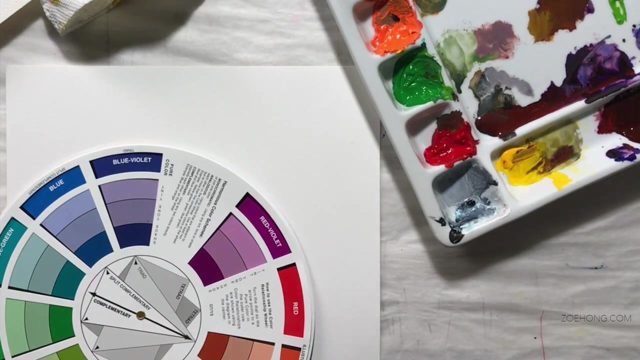 earlier I was demoing on the Arches cold press 140 pound watercolor paper for the mute bars And I was like, okay, I'm going to do this And that is my holy grail watercolor paper. It's my favorite. It's also as expensive as shit. So yeah, I'm. 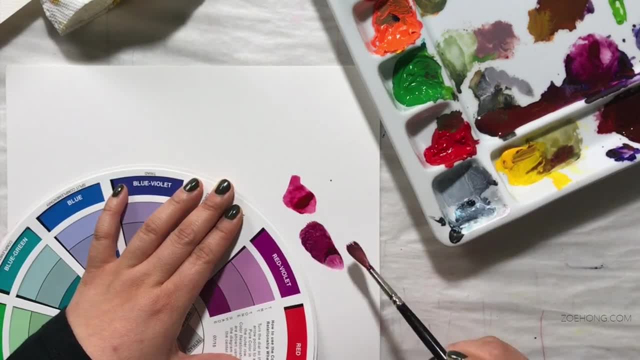 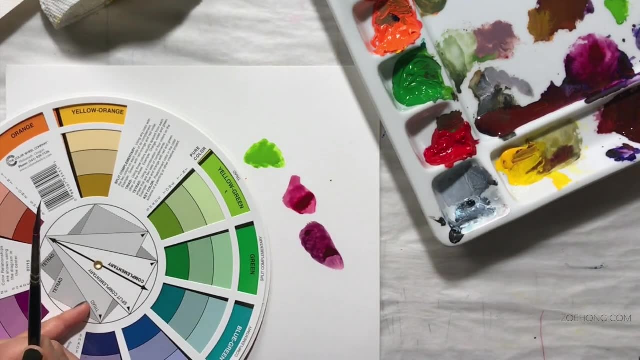 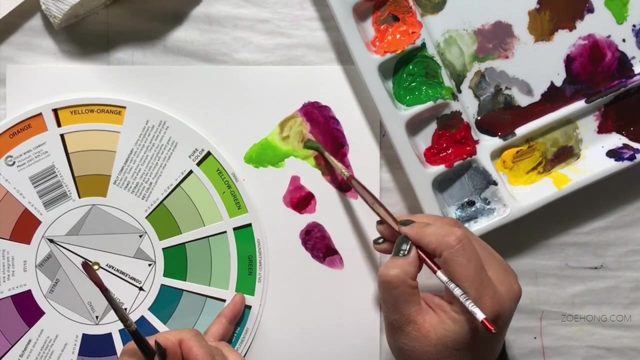 testing out all these other papers. I'm not going to go as in depth with the tertiary mutes as I did the primary and secondary mutes, But I did want to show you again that you can use tertiary compliments to create mutes and tints and shades. 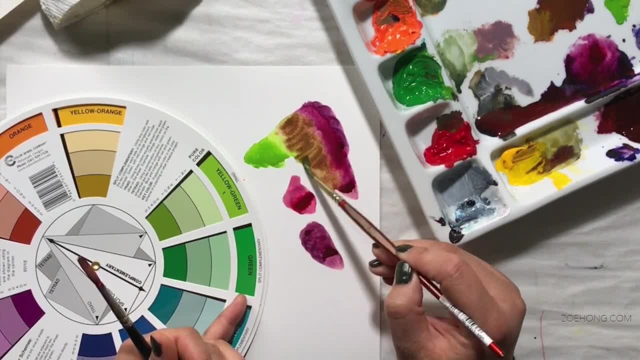 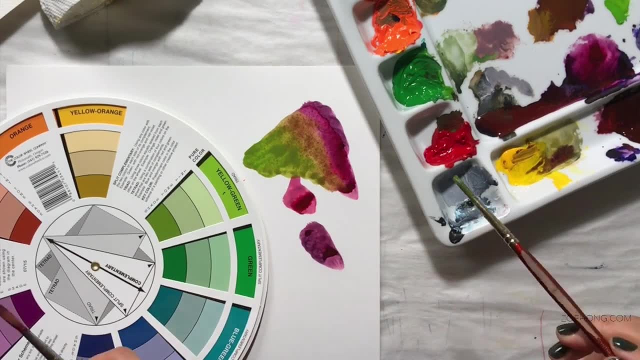 and tones of mutes. Well, and let me tell you, when I was doing, when I was shooting this, I remember distinctly I was like, wow, this paper is terrible. Okay, that was like the first impression. And then, as 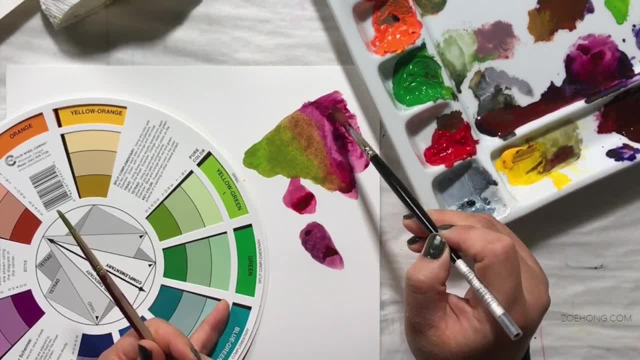 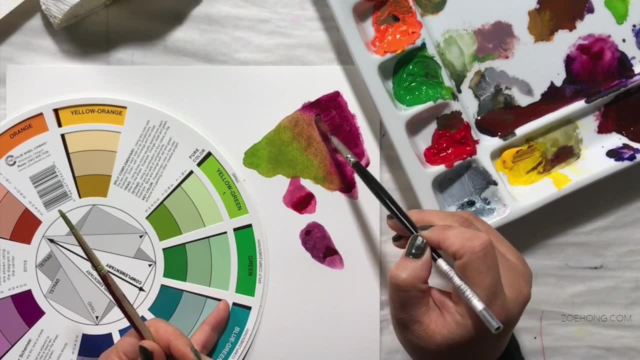 I kept painting, I got more of the hang of it. So I really do have to test this paper out more before I can really slam it. But I did not have a great first impression, But it was just barely good enough where I'm like: all right, let's try it. 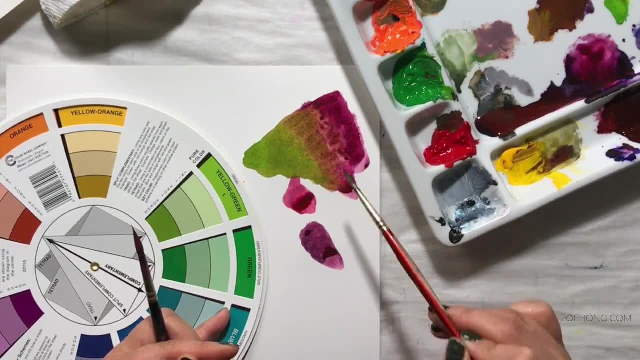 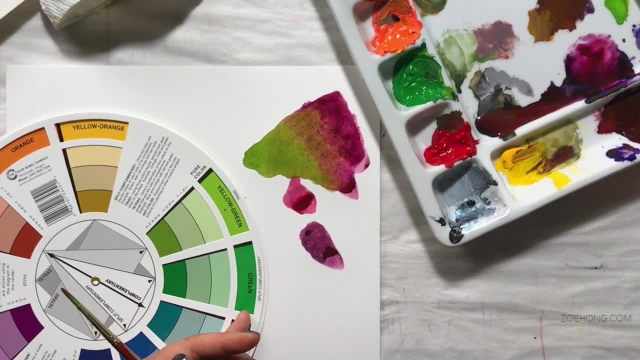 again later. Yeah, so here's a yellow, green and red, And I'm going to use yellow, green, red, purple, red, red, violet. So what are tertiary colors? Okay, so primary colors are red, yellow, blue. secondary colors are orange, green, purple or 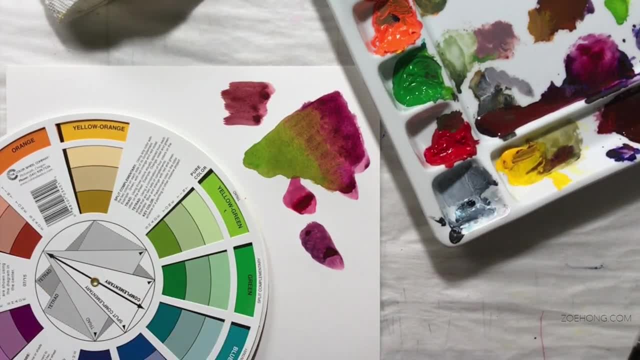 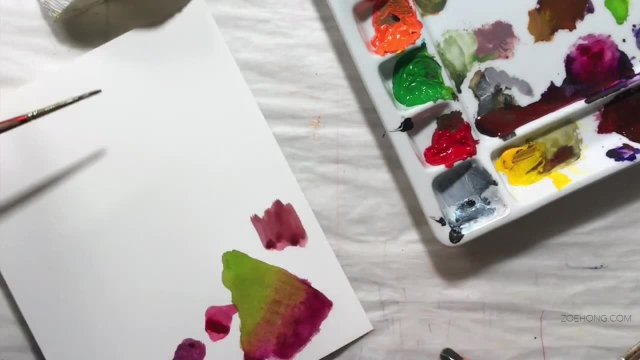 violet, And your tertiary colors are the inbetweens your yellow greens and your red oranges, etc. etc. And again, you can use your tertiary compliments opposites on the color wheel to create mutes, like I did with the yellow, green and the red. 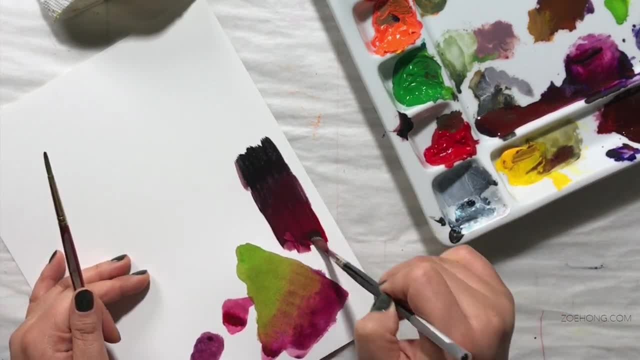 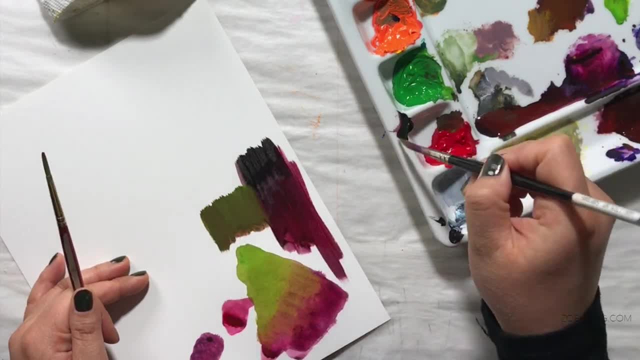 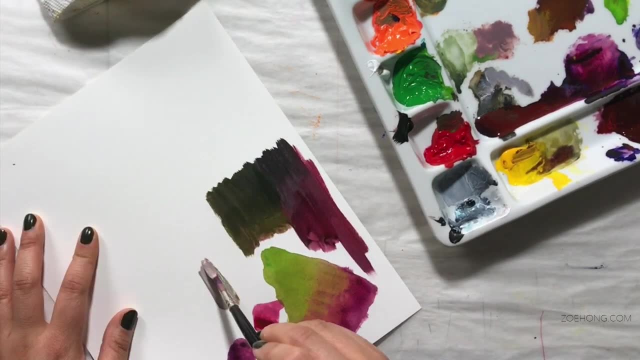 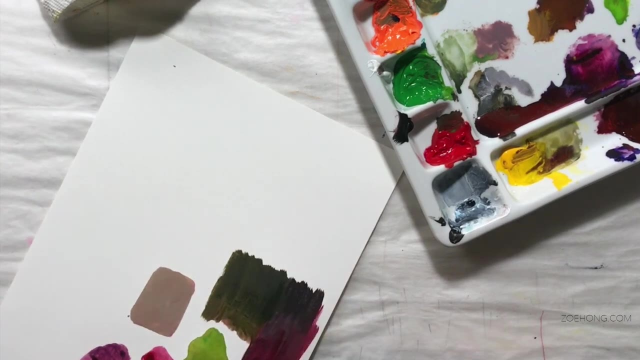 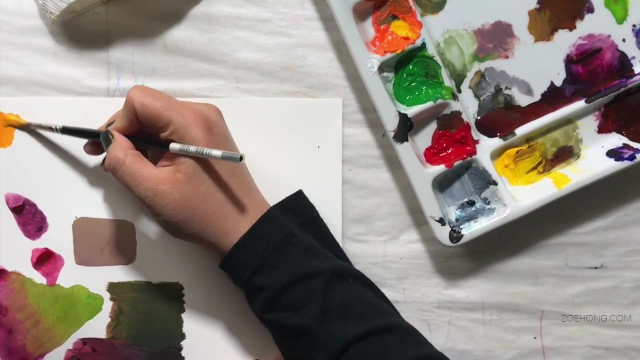 and et cetera, et cetera, et cetera. And again, you know, using these express colors are going to create slightly different neutrals. So here I created a light tone of a mute and I kind of love that weird wobby clay color. I love that. Here we are with a little bit of 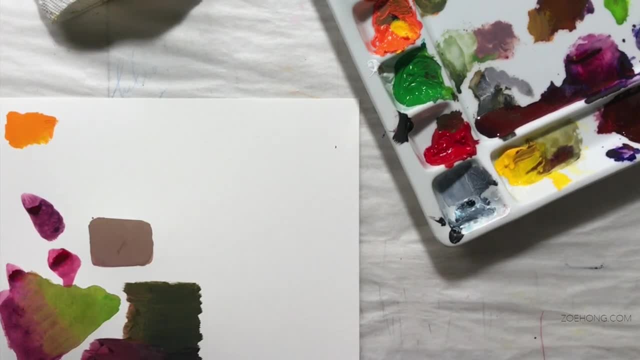 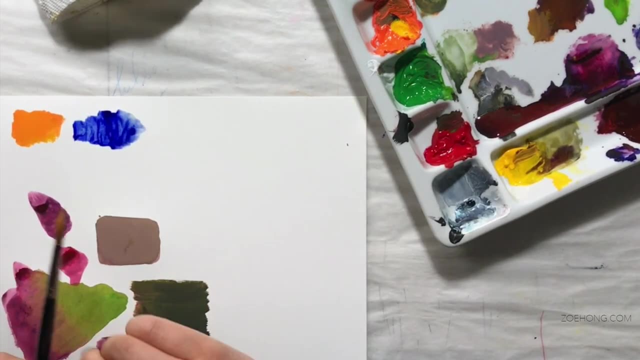 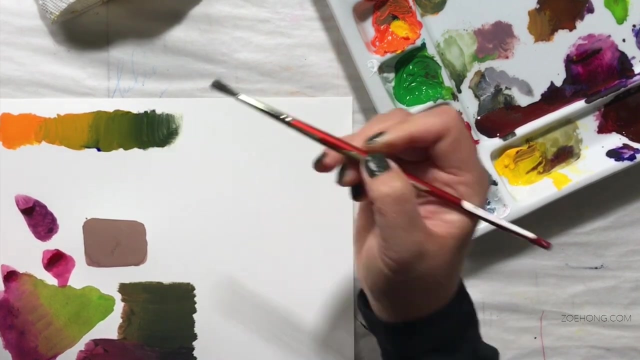 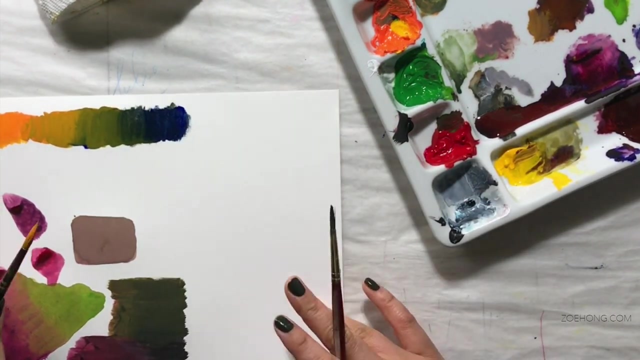 a yellow orange and a little bit of the blue violet. another pair of tertiary compliments, And we're just going to mix those up, And we get a bit more greeny browns in here. The nice thing about this paper, though, is it's so smooth. 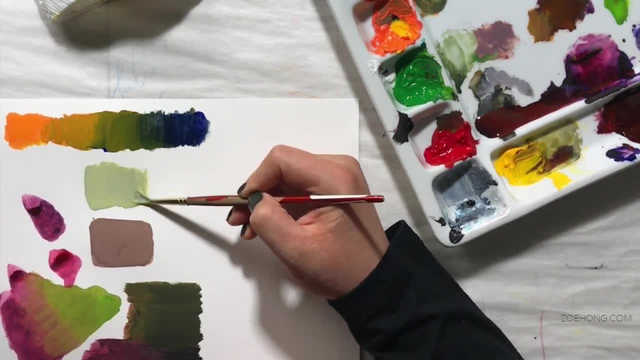 that it's not going to get bushed up so much. So I'm going to use a little bit of greenish brown here And I'm going to mix those up a little bit and it's going to look more green, creating that gradient with a really thick gouache, just so. here's another. 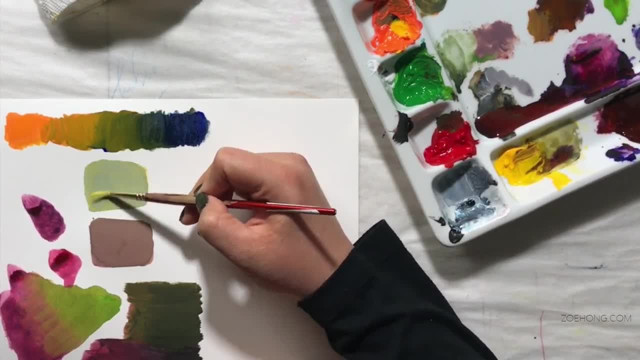 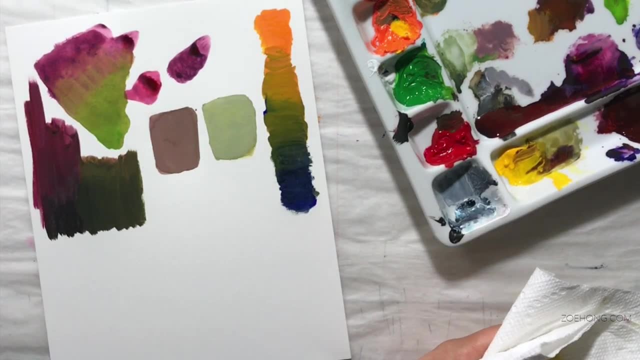 light gray mixed in with the mute, and now you have this like a beautiful celery. it's like a really light celadon pottery color. i love that and, yeah, you really should be doing exactly what i'm doing, which is like playing around and kind of cataloging the colors that you 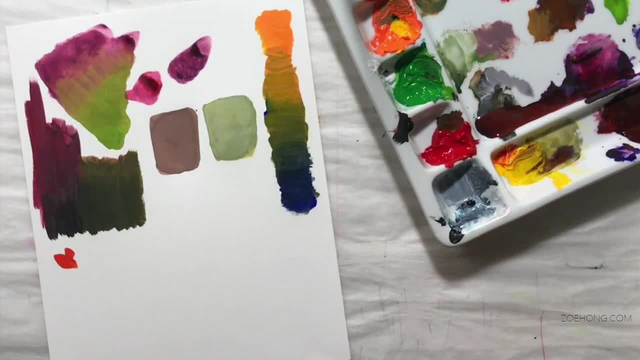 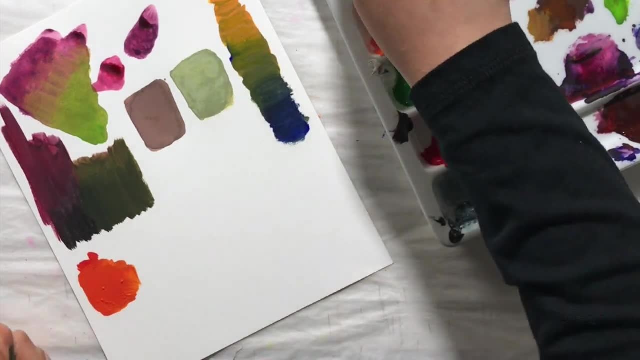 use to create different colors, and even if you don't make your own youtube videos, i mean, why not record yourself doing mixing exercises so you can go back and see how do i mix that color again? oh yeah, how's these colors, you know, is? it's really a nice reference. 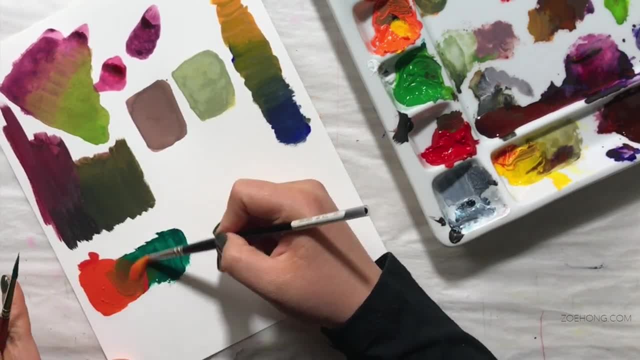 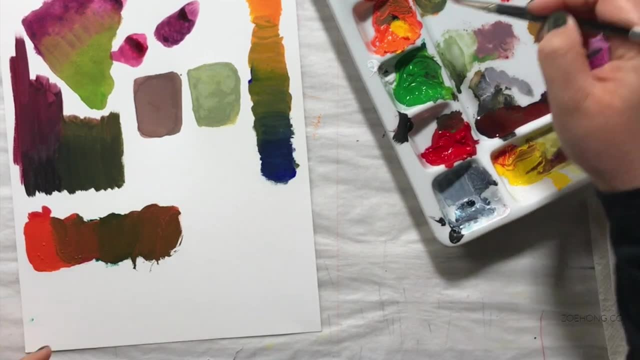 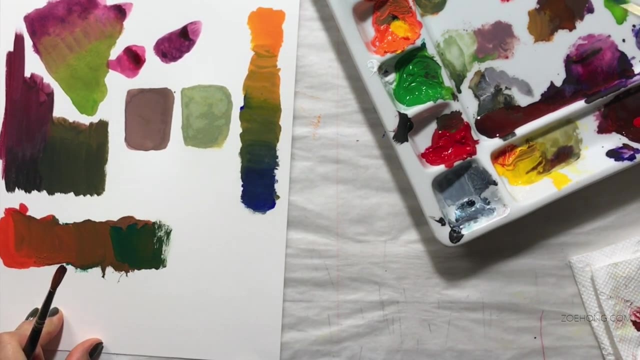 here is, uh, red orange with blue- uh, blue green. excuse me, i really hope that this video was helpful for you in understanding color theory more thoroughly and i'll see you in the next video. please give this video a thumbs up if it helped you and that if you would like me to continue the 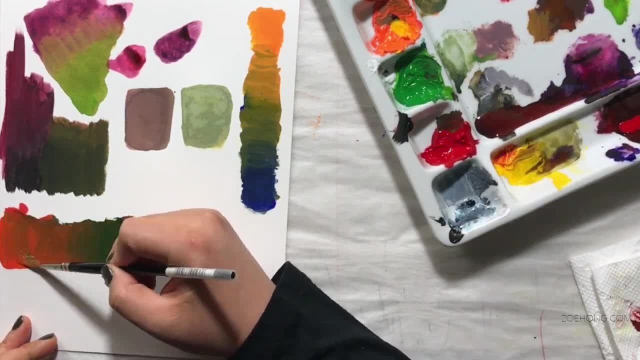 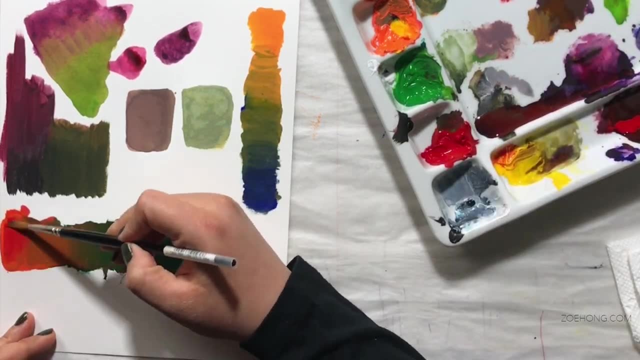 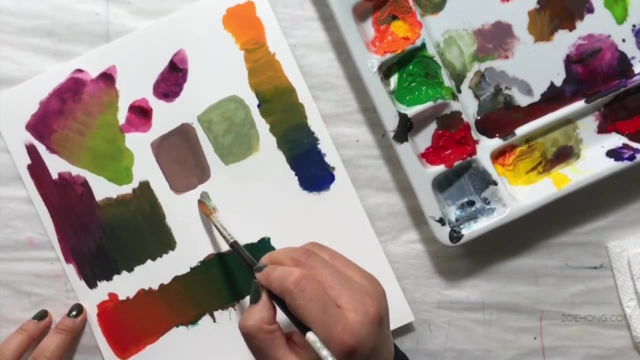 color theory series and, uh, if you want me to continue by applying these color concepts to fashion my lesson, my tentative lesson plan right now is to just straight up draw some croquis and slap some colors down and we can study how different colors affect the designs of dresses. 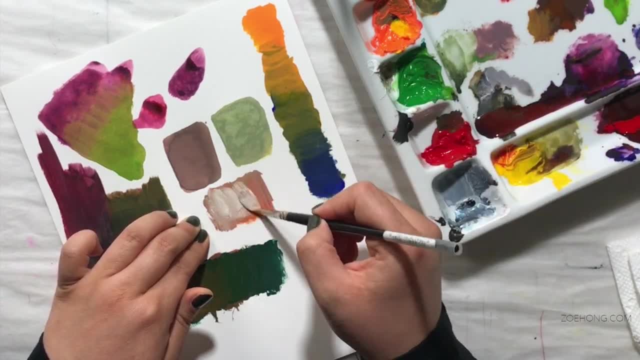 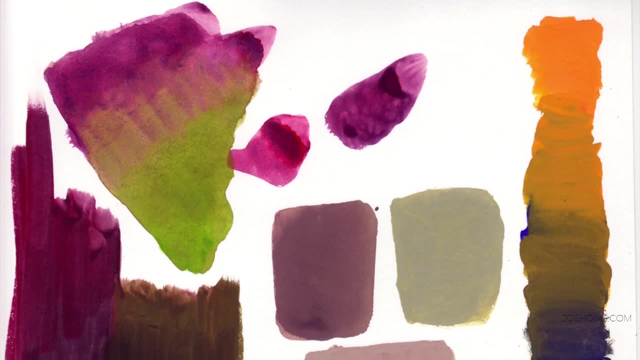 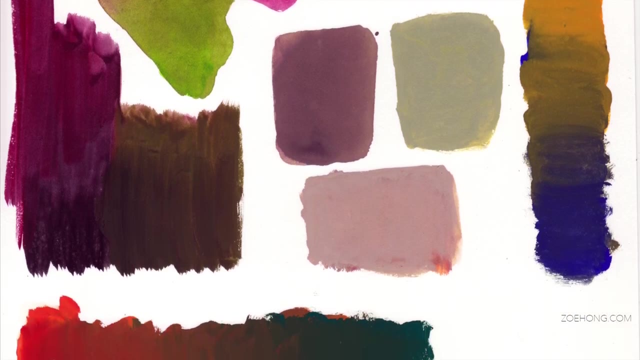 and that's really the most direct way to study it and also another reason why i push people to learn basic drawing skills. you don't have to be a brilliant illustrator, but to have basic drawing skills so you can test colors in the way that i plan on showing you in future videos. 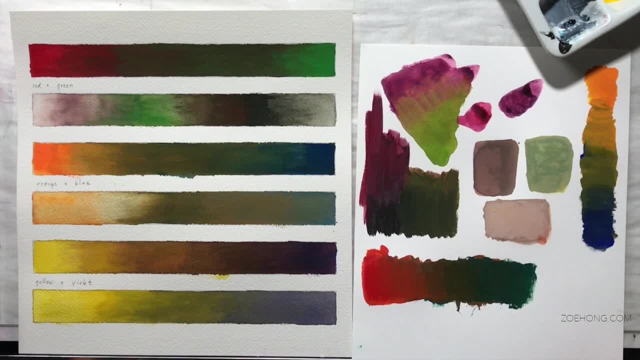 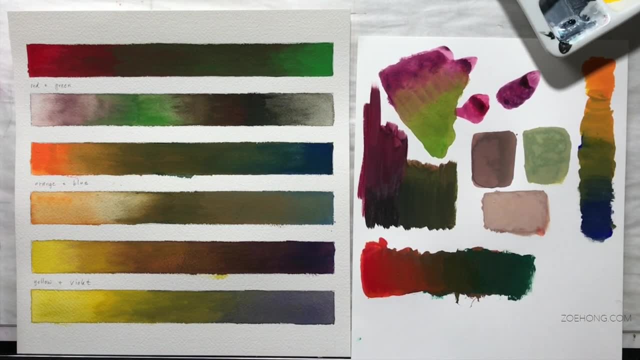 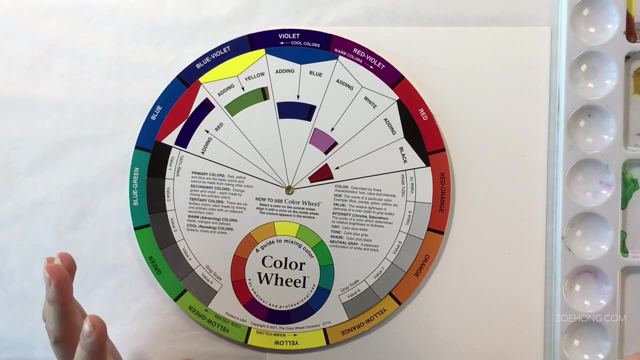 go mix up some paints, Go, have fun. go practice. subscribe, if you haven't already. drop me all your questions in the comment section below and I will see you in the next video. Hey, hey, party people. Today we're going to talk about split complementary color schemes and how to use them in fashion. 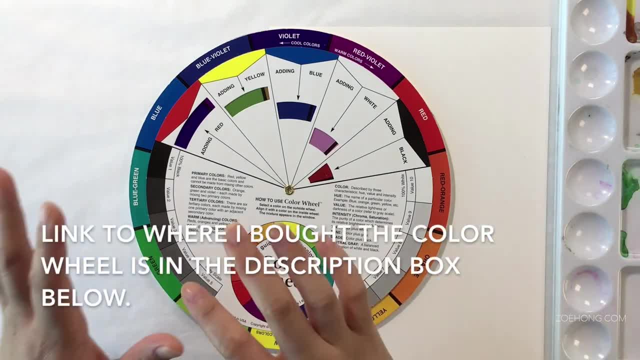 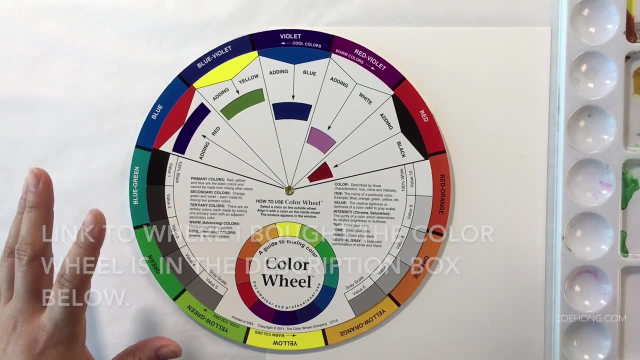 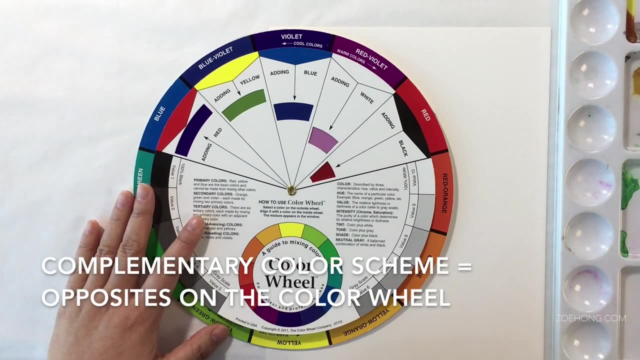 design and illustration. So let's go over some vocabulary and then we're going to get into application later in this video. First of all, what is split complement? So rewind a tiny bit. what is a complementary color scheme? Complementary color schemes are opposites on the color wheel. 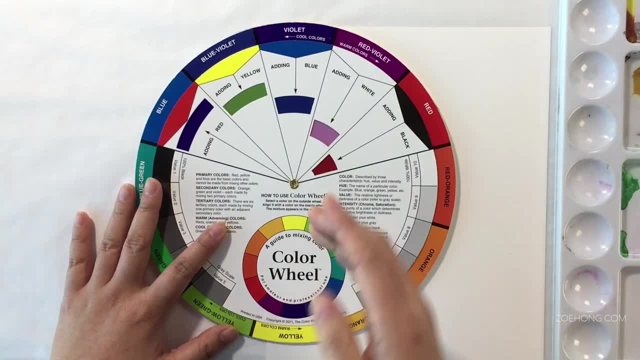 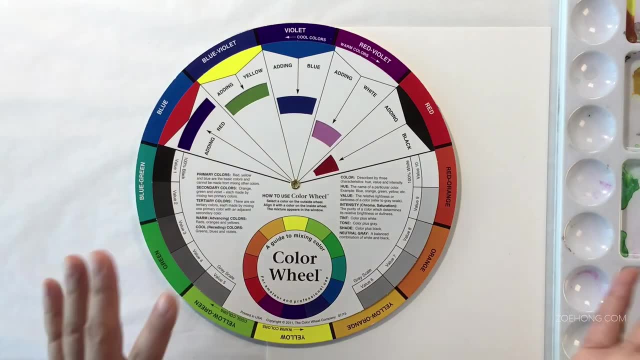 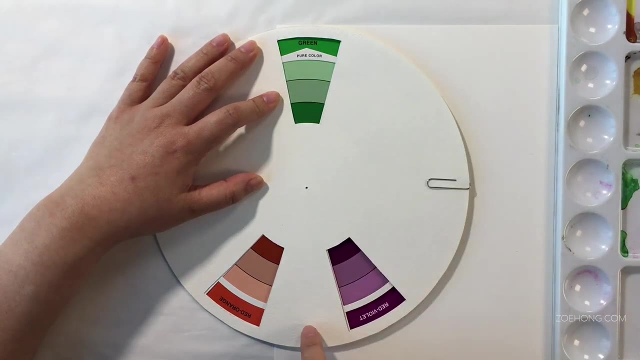 Violet's complement is yellow. opposite of the color wheel Red. violet's opposite is yellow, green, et cetera, et cetera, Split complements. take your first color, green, for example. The opposite of green is yellow, Green is red. 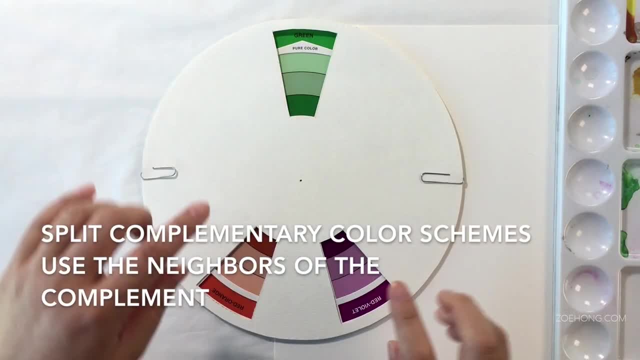 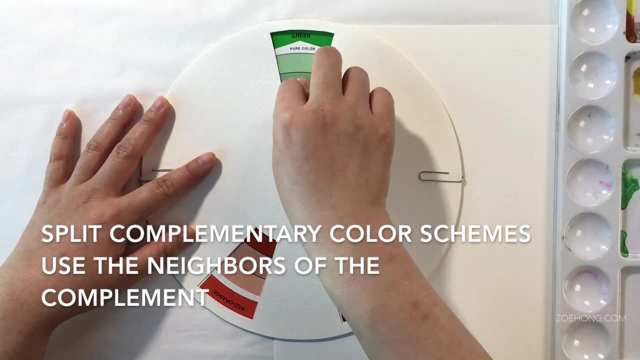 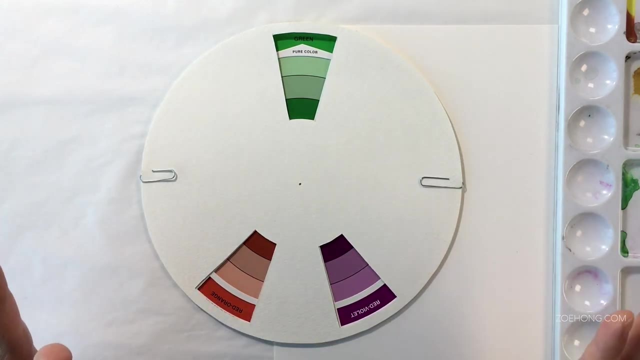 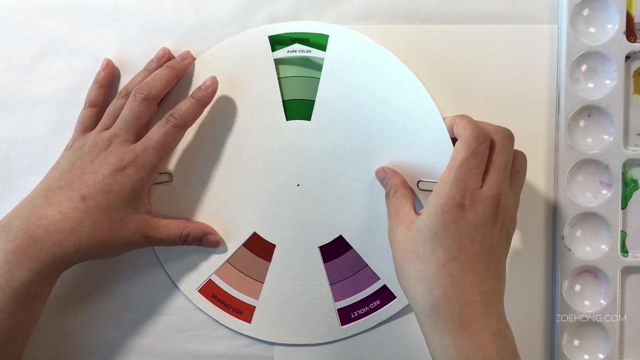 The complement of green is red, But split complementary color schemes use the neighbors of the complement. So green's split complements are red, violet and red orange And these three together make up a split complementary color scheme. Because of their uneven positions on the color wheel, each color has their own split complements. 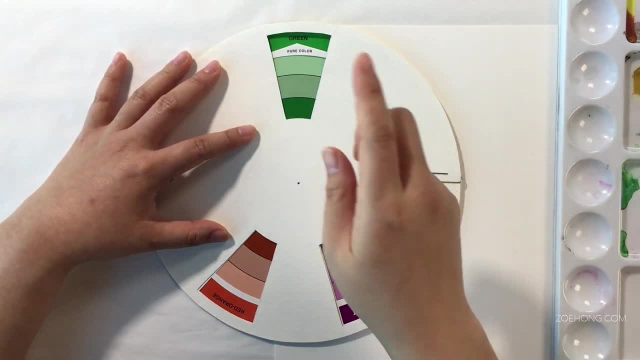 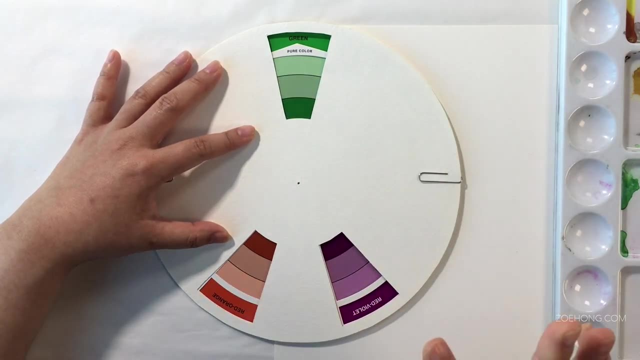 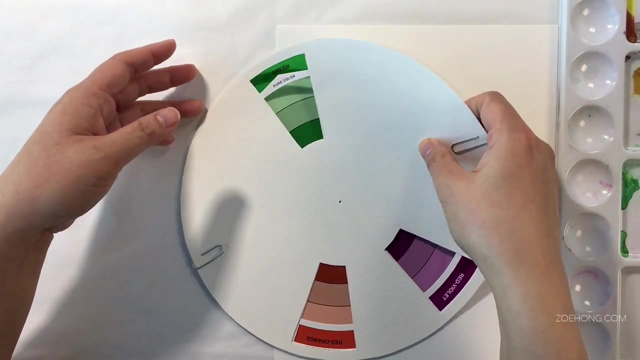 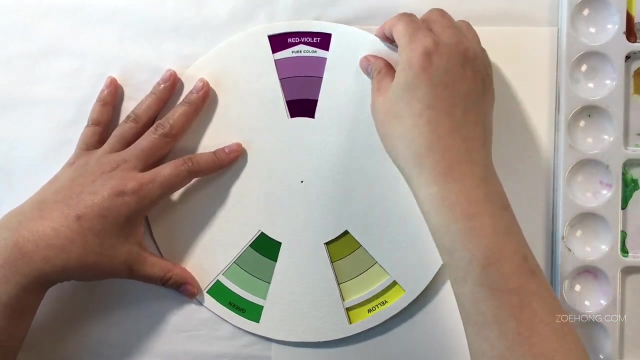 So what I mean by that is, green's split complements are red, violet and red orange, But that doesn't mean that red violet's split complements are green and red orange. If you use my kind of messy but effective cutout, if you start with red, violet, red, 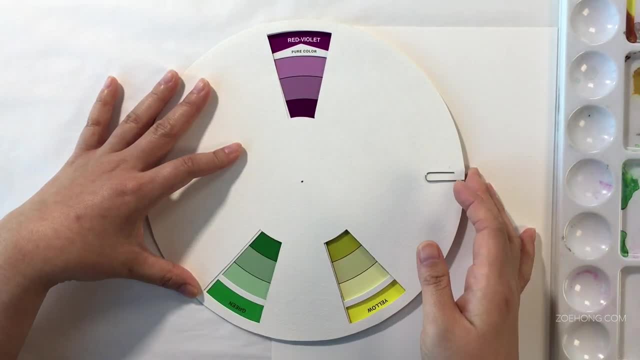 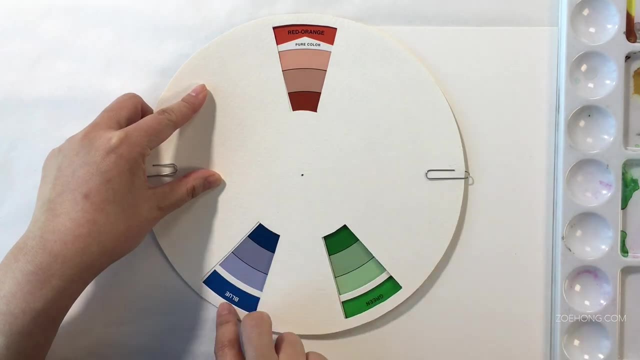 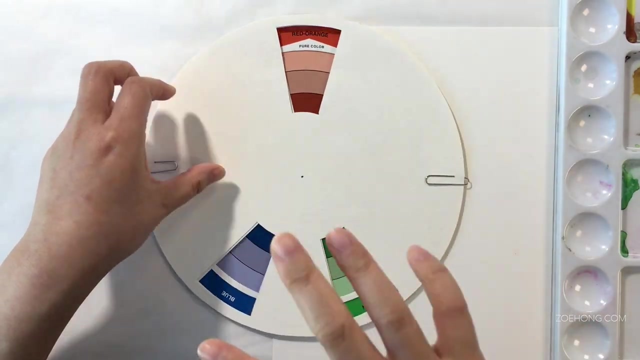 violet's split complements are green and yellow. Okay, And then red orange's complements are green and blue. So yeah, they share that green, but the trio is different. And the trio, you know, the mood, the vibe, the scheme, everything is different because 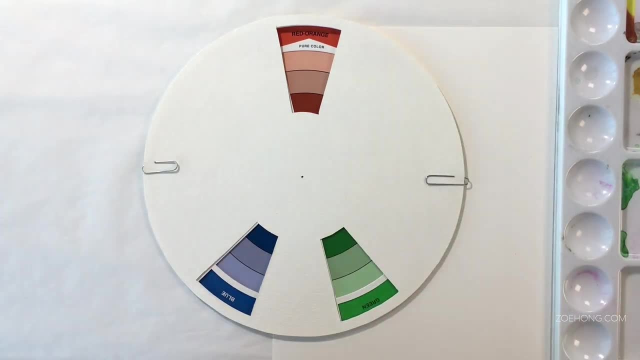 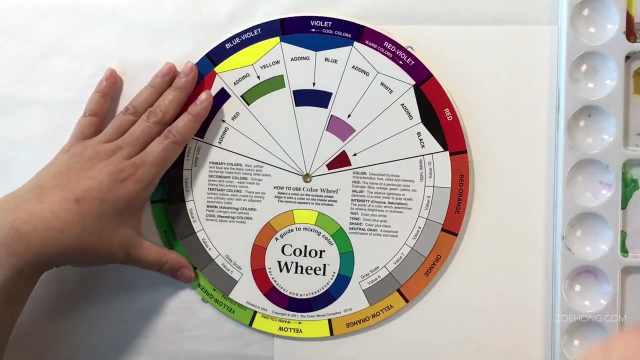 that third color is different. Okay, So every color has their own two distinct split complements. Previously, when we had discussed complements, This time I wanted to do a video where you guys talk aboutIGS, which is okay. I wanted to do a video where I talked about thelasher, which is that. this is the beauty. 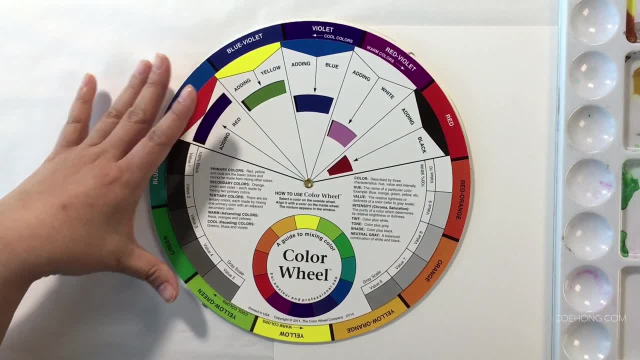 of this project- Thelasher's white color, the green color, And in this video I talk about how to make colors with complementary colors. Okay, And there's a whole video on muting. Okay, I'll post a link in the description. 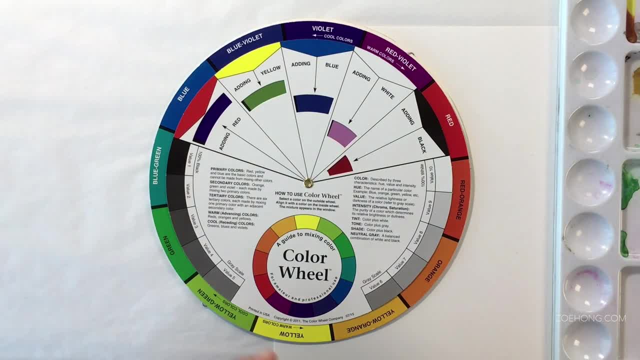 I watch, I listen to so many podcasts. I keep wanting to call them the show notes, Because that's how podcasters say it. They're like, and we're going to leave you a link in the show notes. So I keep saying in my head: 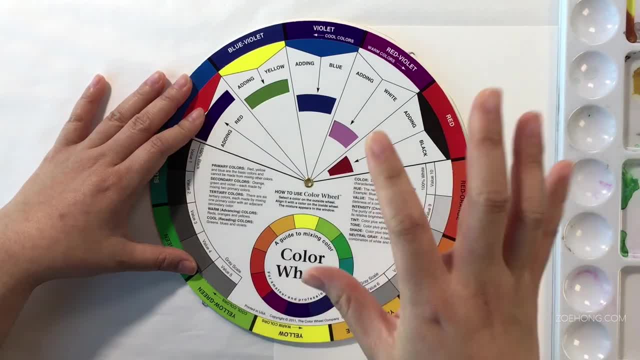 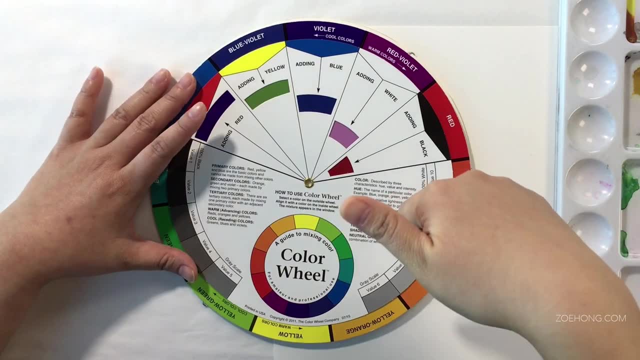 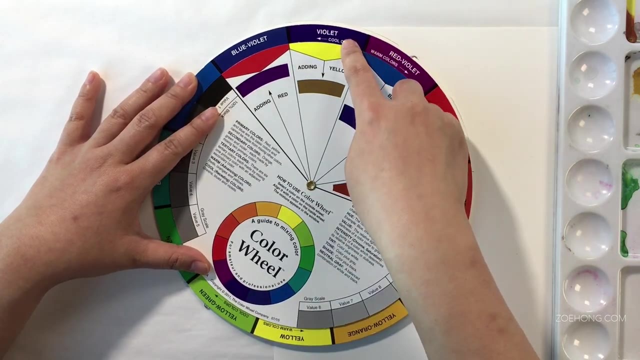 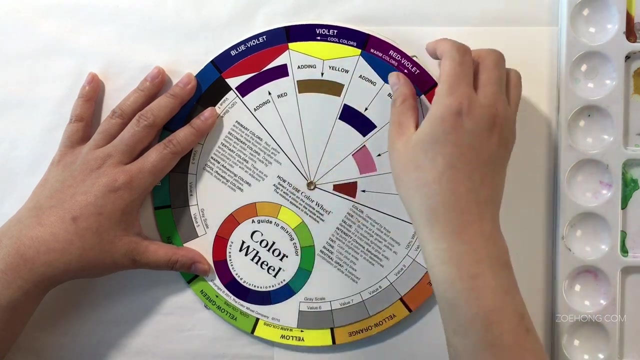 I keep thinking I'm going to drop a link for you in the show notes, Anyway. So I'm going to drop a link to the muting color schemes video in the show notes. but basically, when you add the opposite- violet and yellow are opposites, they're complements- you get muted colors And similar to this with. 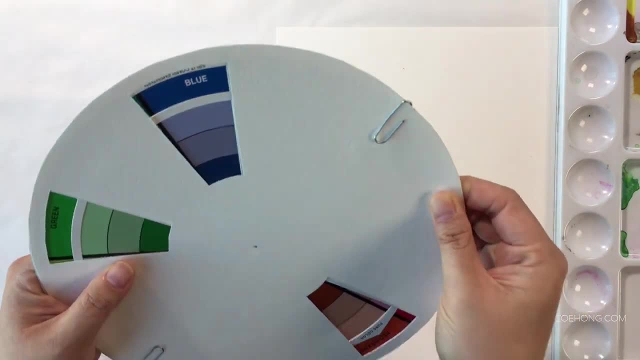 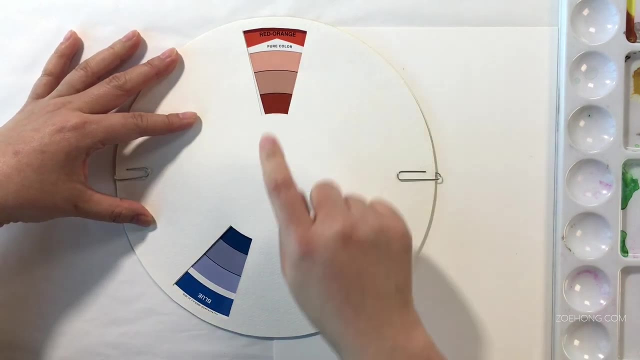 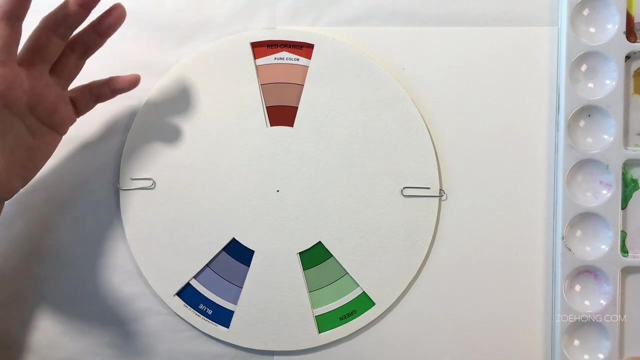 split complements. you can create what are called near mutes with split complementary colors. So I can mix a red orange with a blue to create a near mute which is going to start giving you those you know, toned down neutrally colors. And if you go this direction, 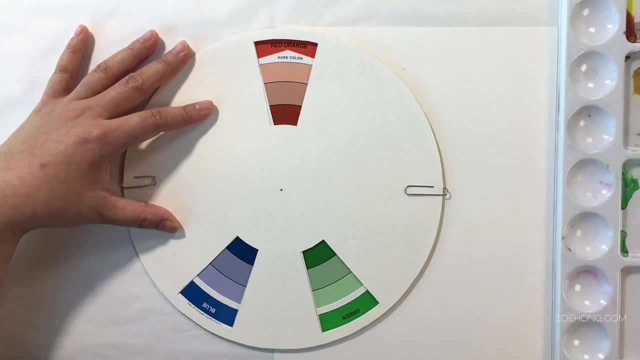 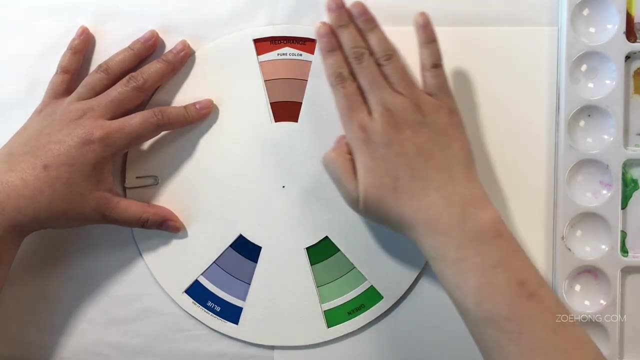 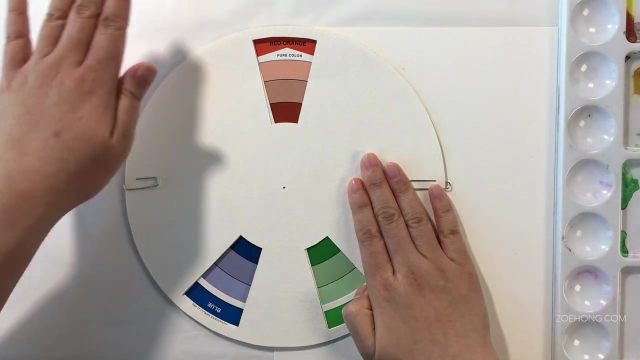 your neutral colors are going to start looking a little bit warmer because both these colors have yellow in them, And so you have like a more warmer vibe over here. If you start muting with the blue, you're going to get a slightly cooler vibe with your neutrals. 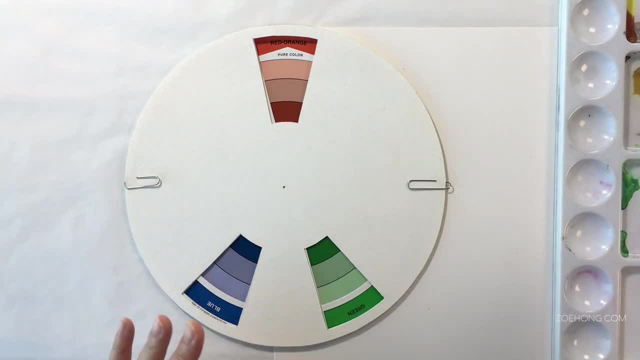 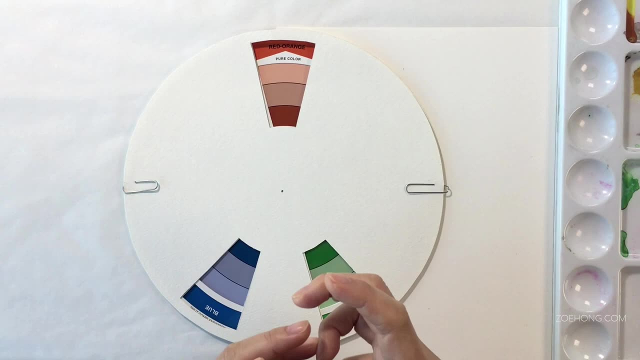 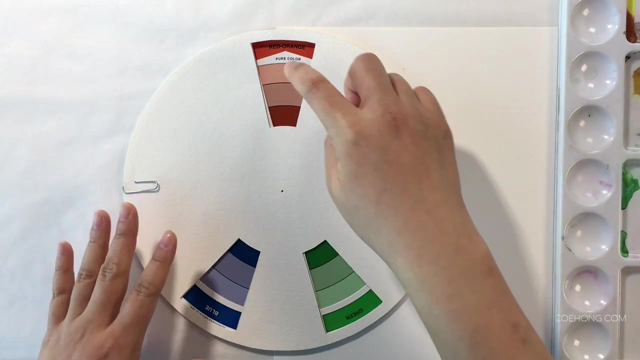 just like any other color scheme, A split, complementary color scheme is not just these three pure colors but any variation and combination of tints, shades, tones and mutes of each of these colors. So if you have a tint of a red orange, 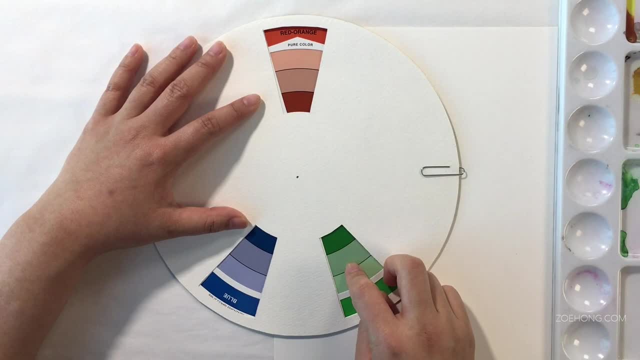 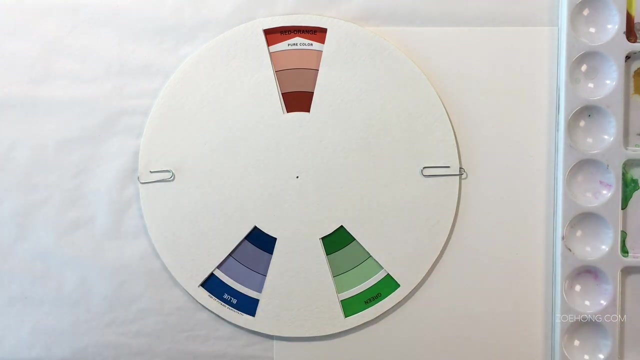 which is red, orange plus white, and if you have a shade of a green, which is green plus black, and if you have a tone of a blue which is blue plus gray, that's still a split complementary color scheme. Okay, When you say split comp, you mean the base of each color. 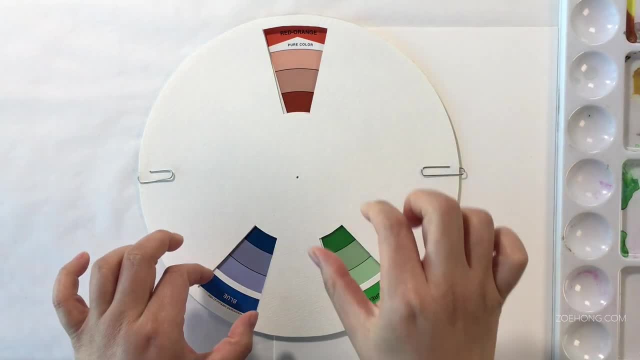 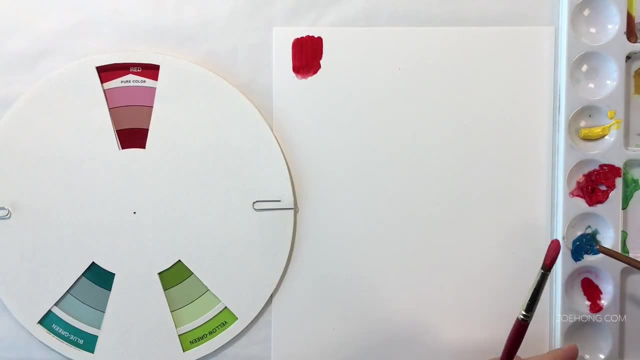 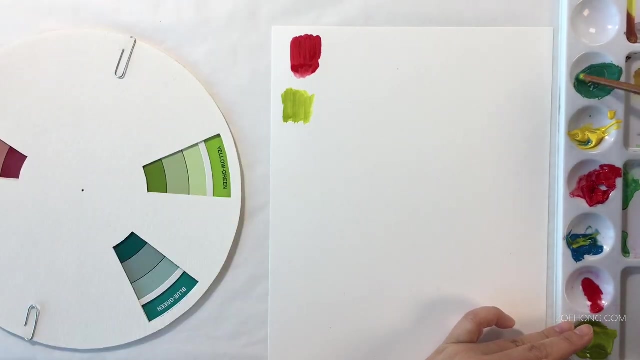 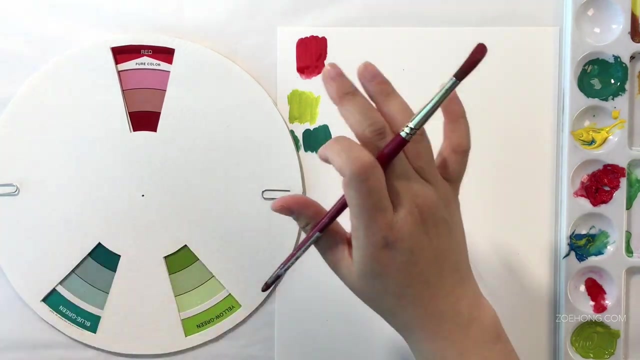 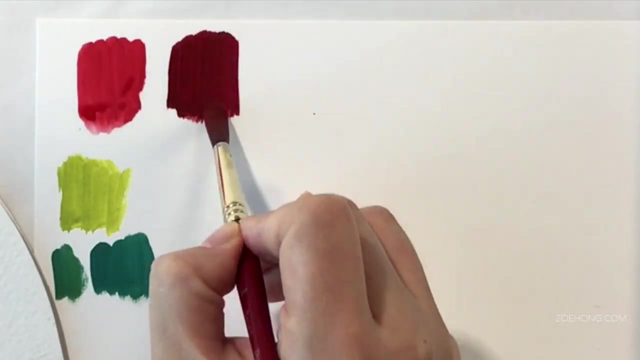 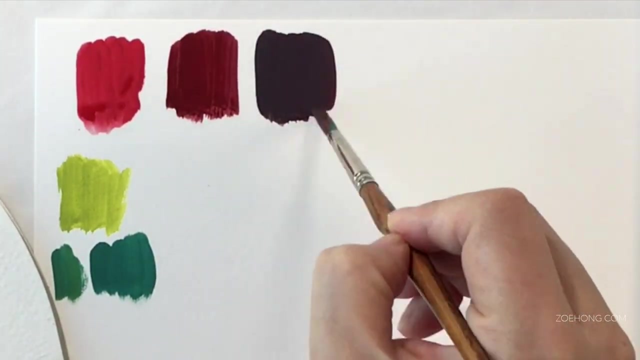 is a split complementary color scheme, not just the pure color. So remember when I said we could create near mutes with these three colors. So here is the red with some of the blue green, And here's more of the blue green, And here's even more of the blue green. 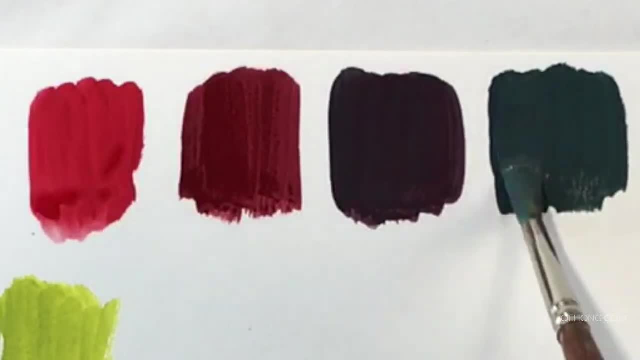 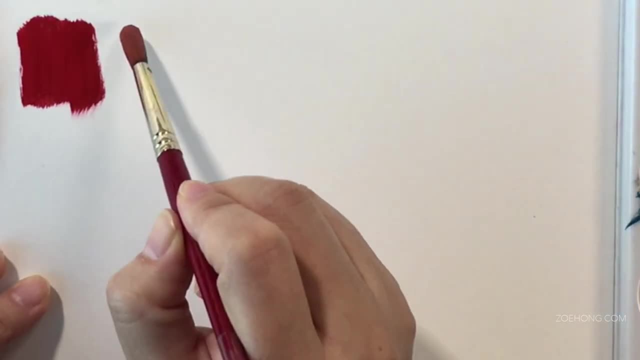 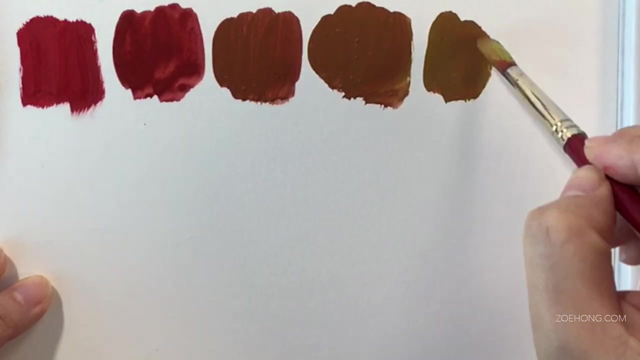 So you're seeing some of the transition. You see how the colors are working together And let's try creating near mutes with the green. So that's red with yellow green, That's red with more yellow green, and some more and some more. 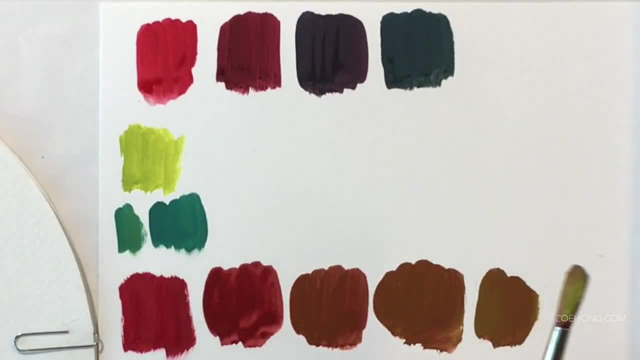 So you're seeing the transitioning of the colors becoming more neutral And, as I mentioned before, because there's so much, there's warmer tones in here. The neutrals are warmer. they're mustardy, mustardy, yes, approaching mustardy colors, greenish, 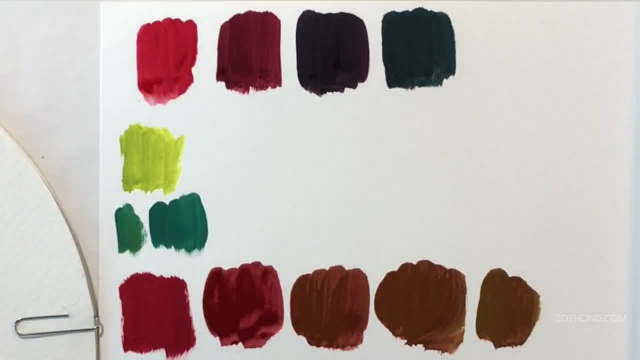 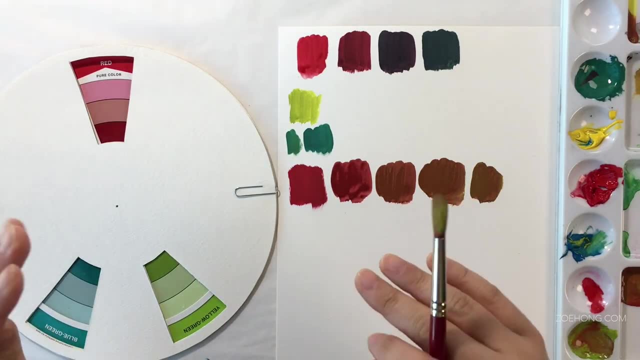 And then in here, because the blue green is so close to blue, you're starting to see more violety, especially in here. So depending on how you want to mute the colors down, what kind of more neutral colors you're going for, you can mix them appropriately. 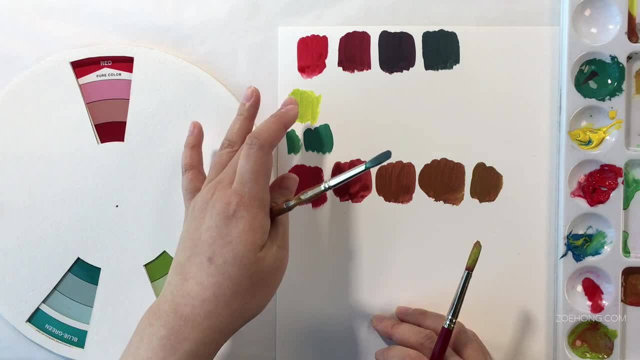 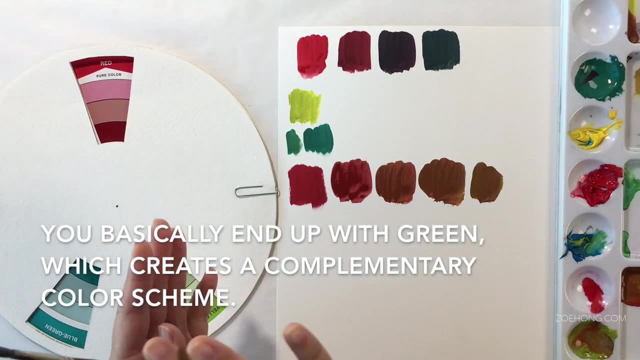 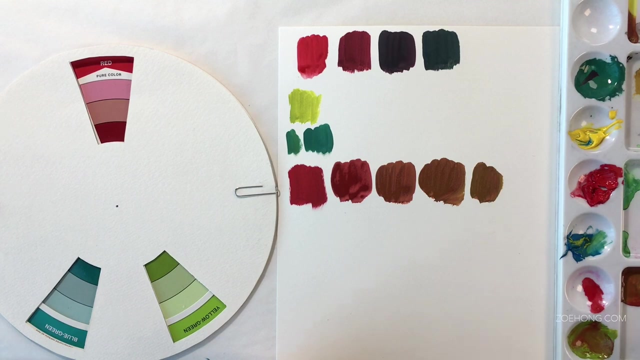 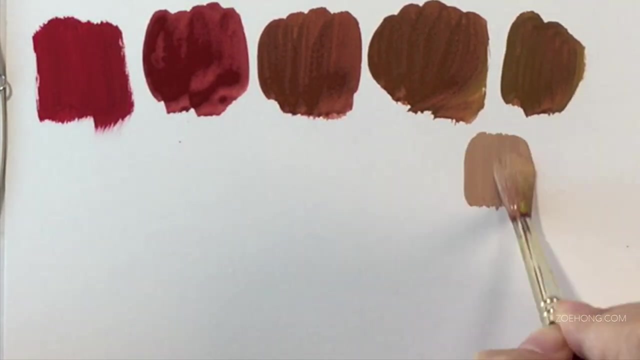 Now mixing the yellow green and the blue green, you end up getting a completely different color And so it kind of veers off the split complementary course. I think at this point you all know what tints and shades And tones look like. If you don't, I have so many videos. but here is white with this. 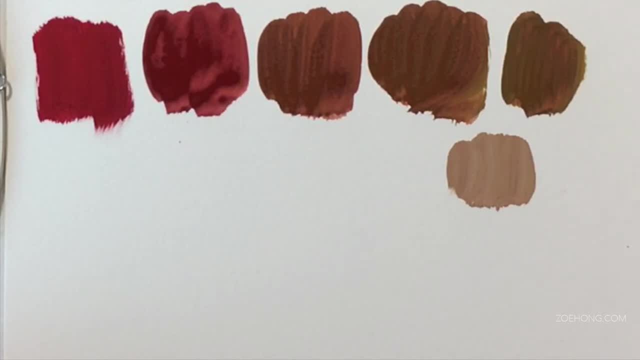 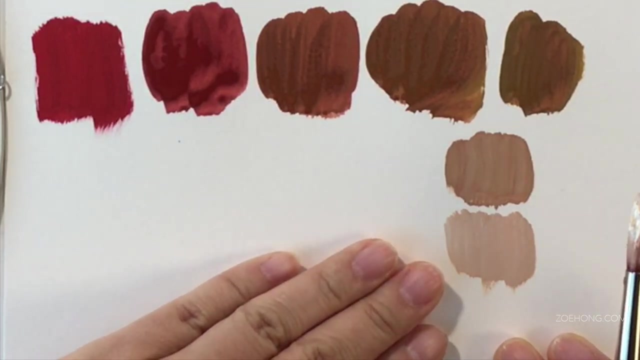 Okay, so you can just start making so many colors. Here's more white And you're starting to get these browns, And then, uh, I mean we're getting kind of close to flesh tone territory right At this point. you may be thinking, but Zoe, 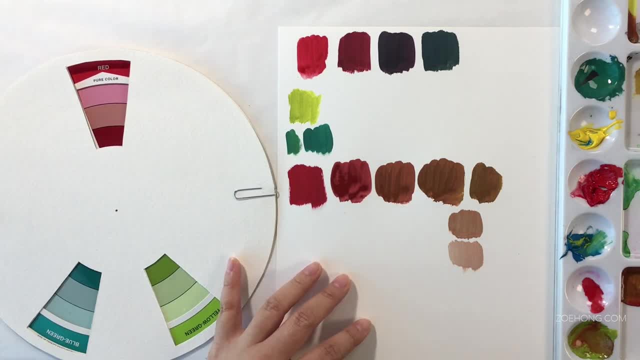 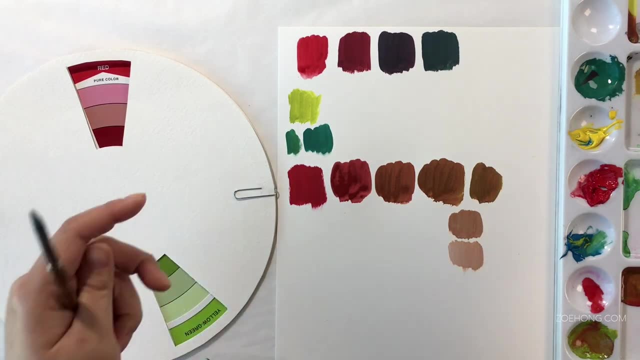 I've seen your skin tones videos and any video where you start talking about skin tones and you usually start with burnt sienna or burnt umber. Well, yeah, I mean, you only need magenta, yellow, cyan and black to make any color. 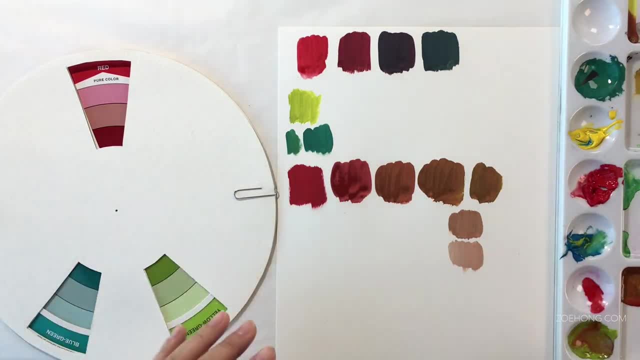 Okay, if you need proof of that, just look in your printer. Your color printer has cartridges for cyan, magenta, yellow and black and they print out every single color. And I know some color printers have a grid gray cartridge and that helps with subtleties. But what is gray? It's like black. Okay, Now when. 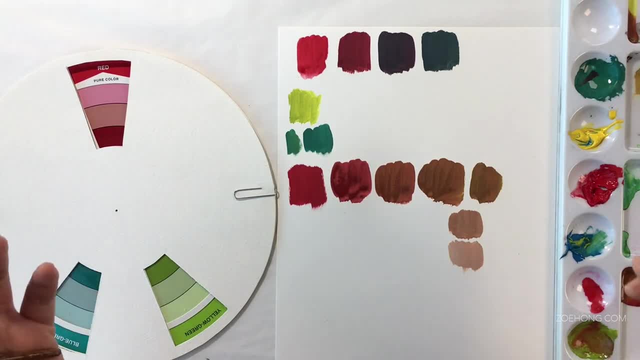 I buy colors like burnt sienna and burnt umber. they're shortcuts, because burnt sienna and burnt umber are basically shades of orange. If I'm going to use a shortcut a lot like burnt sienna, it is worth it to me to buy the tube of burnt sienna. Okay, But if you want to start painting, 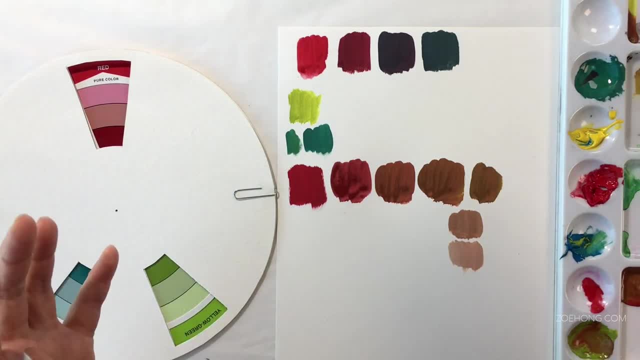 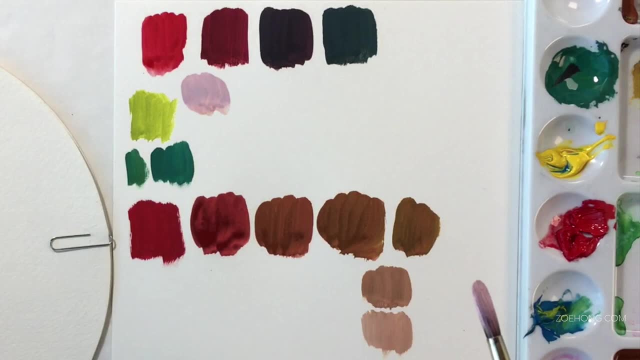 and you don't have that much money or you don't want to invest a lot of money yet, yeah, just get the four: magenta, cyan, yellow and black. And here's some white. with these near mutes, And because of the blue tones, you're creating a pink with more of like a lilac tone. 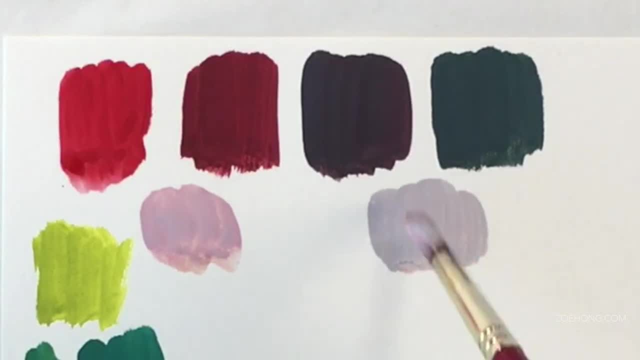 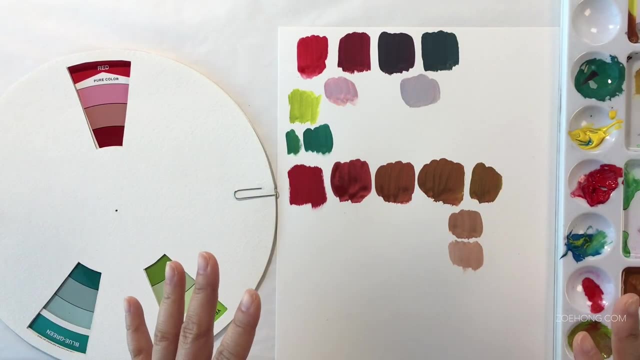 because you've got so much blue in there And then over here you're getting this dusky blue gray. So I could do this all day because I love fixing colors and I love making color swatches. However, we don't have all day. 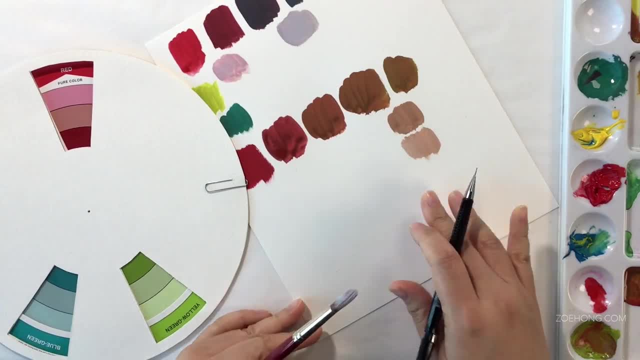 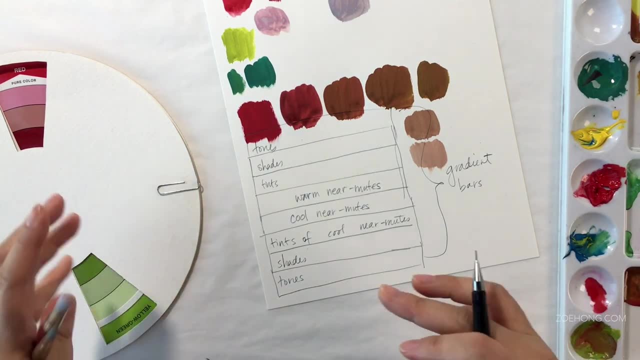 If you want a homework assignment from me to explore split complementary color schemes, here's what I would do. If you really want to study color mixing, the only way to do that is to literally mix your colors. Okay, So what I would do is I would take 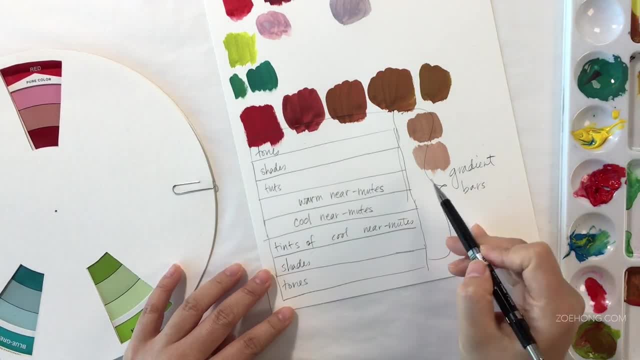 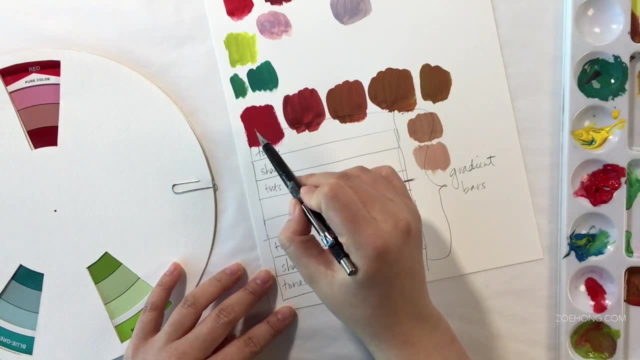 you know a set of split compliments that you like. So start with your purely saturated warm near mutes. In this case it would be the red plus the yellow green, And then I would do a gradient bar of the cool near mutes. In this case it would be the red. 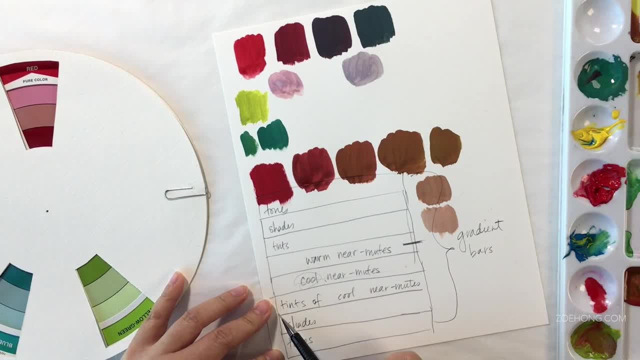 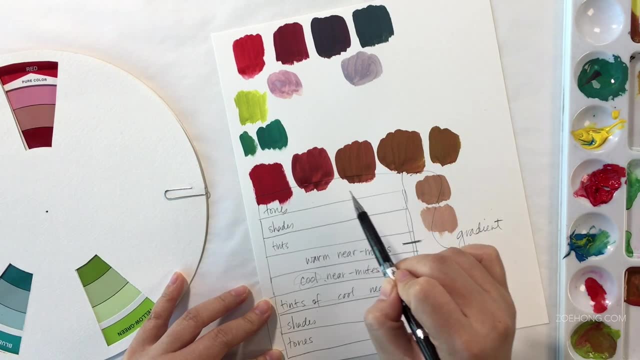 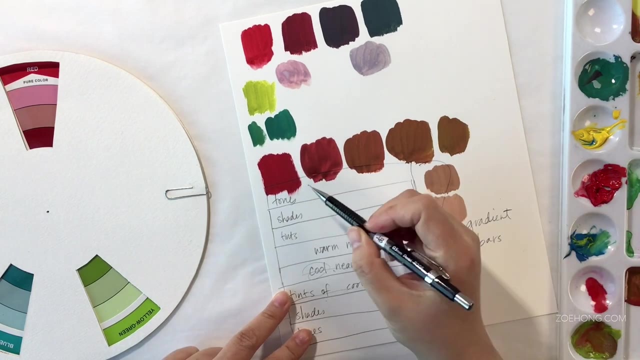 plus the blue green, And then I would do tints of those, shades of those and tones of those. tints of the warm near mutes, shades of the warm near mutes and tones of the warm near mutes. Okay, And really understand how I mean you're going to really get where these colors are coming. 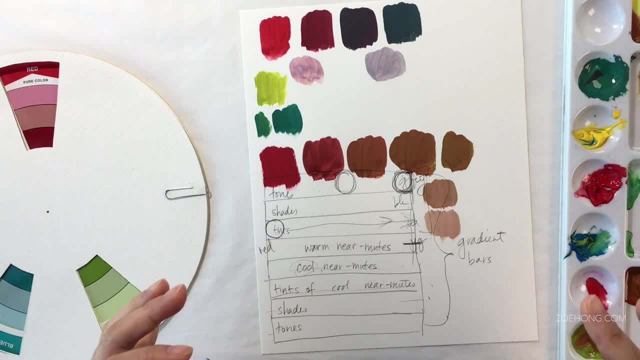 from. You're not going to be able to create every single color variation- impossible with this chart- but you're going to start getting an idea as to the realm of possibility And the more you mix your colors and play around and document what colors you mixed in. 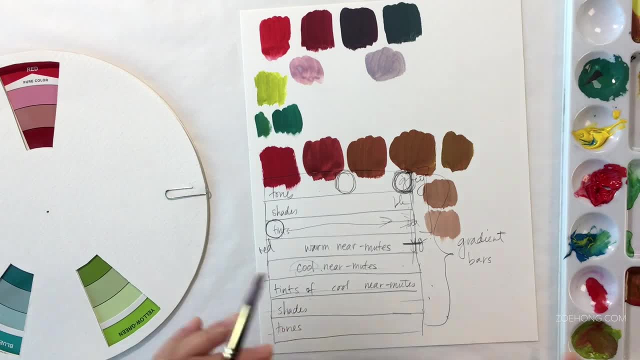 order to get specific colors, the better you're going to have an understanding, the better painter you're going to be and the better you are going to be at selecting colors and color stories for future design projects. Now I designed these three dresses. 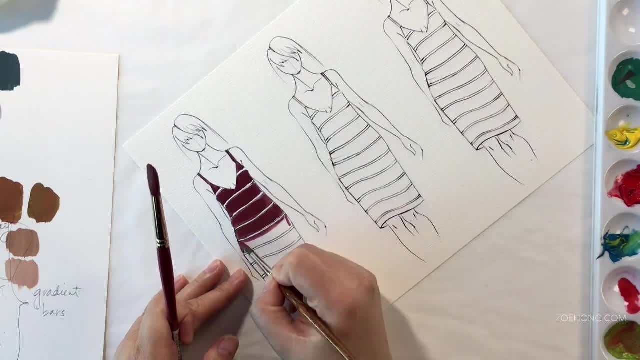 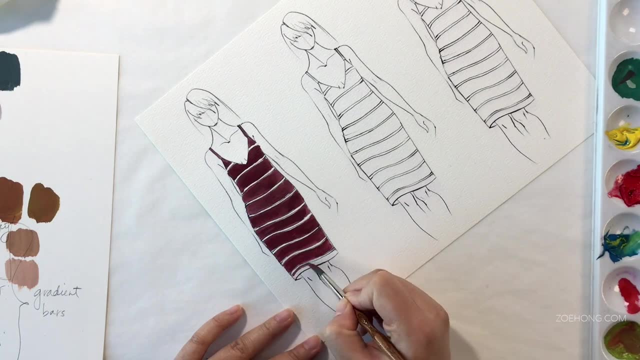 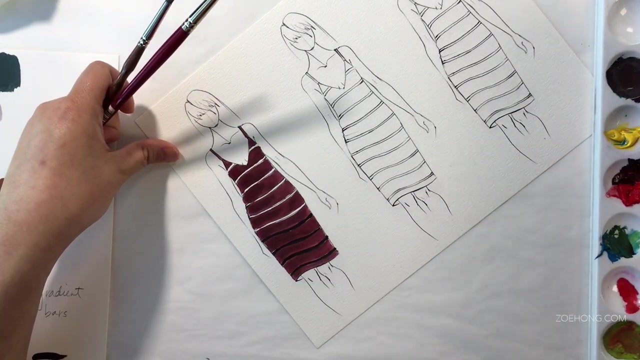 or this one dress, and I deliberately chose a skinny stripe and a broad stripe so we could play with color proportion, Because it's not even so much what colors you pick, but how, in what quantities, you use the colors to get the effect that you want. Like, if you use a lot of 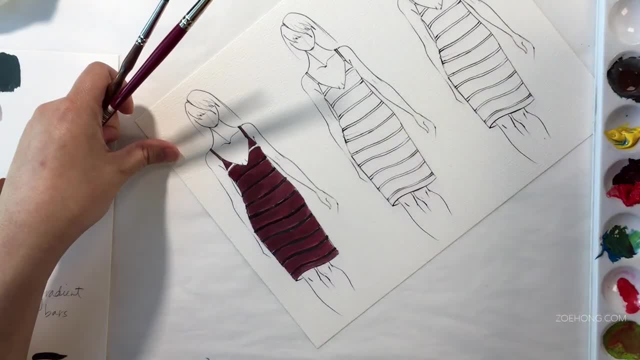 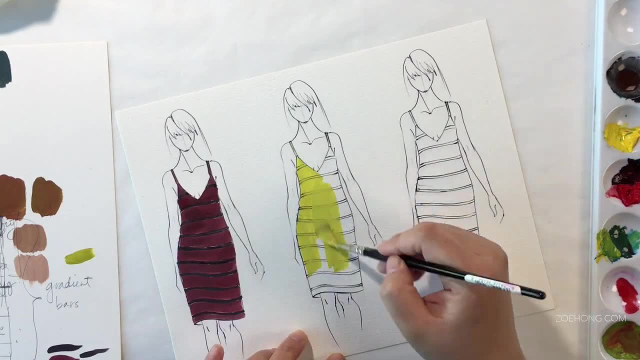 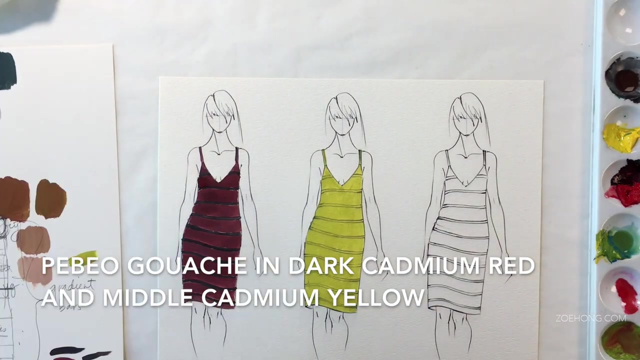 warm colors. what is that? you know? what effect does that give versus if you use a lot of cool colors? Okay, really quick, because you guys always ask me what I'm using. I'm using Pabeo gouache's in dark, cadmium red, and then the middle cadmium yellow, and Winsor & 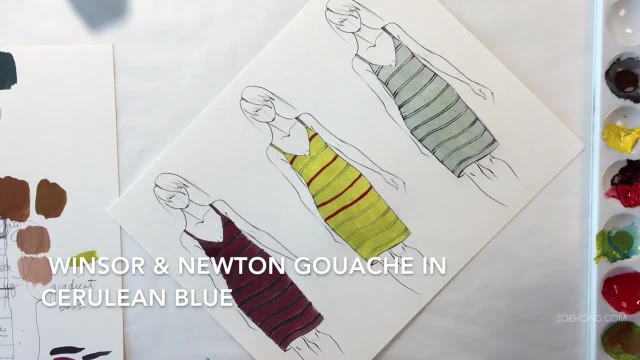 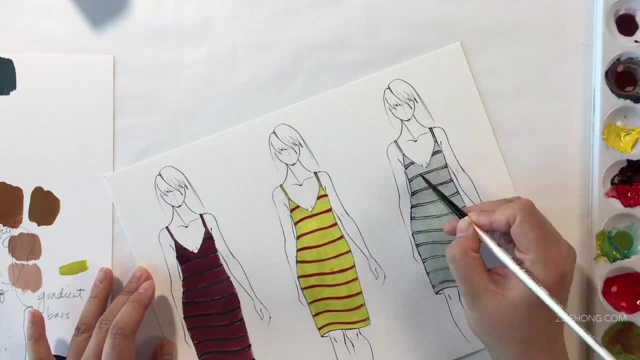 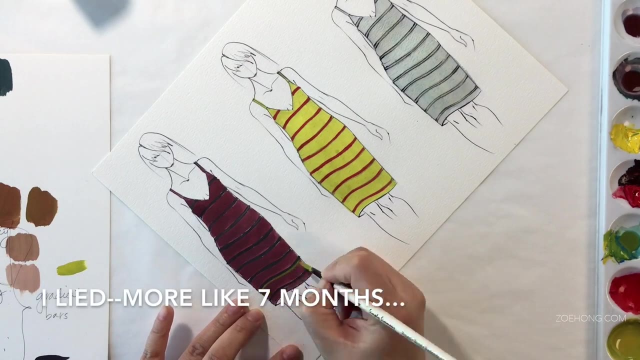 Newton cerulean blue. I've been using the Winsor & Newton for a long time and I enjoy them a ton. I have a bunch of these. They're great Pabeo's I've only been using in the past year maybe. 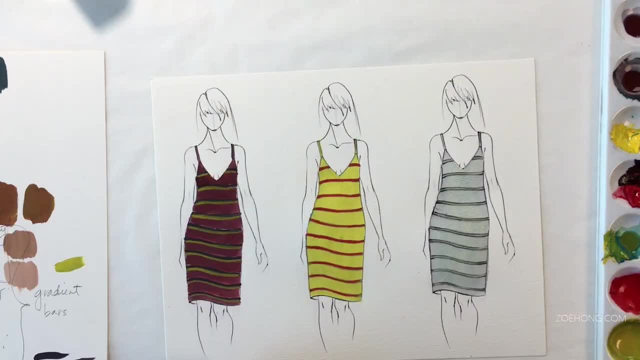 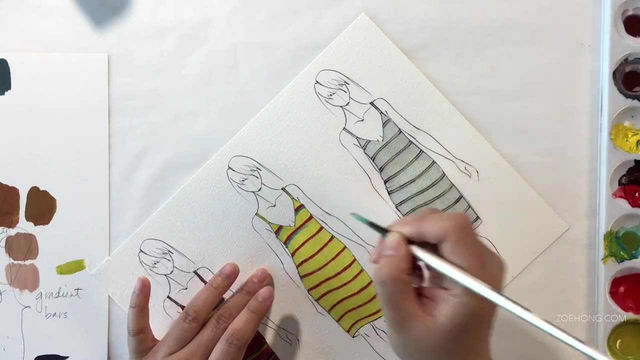 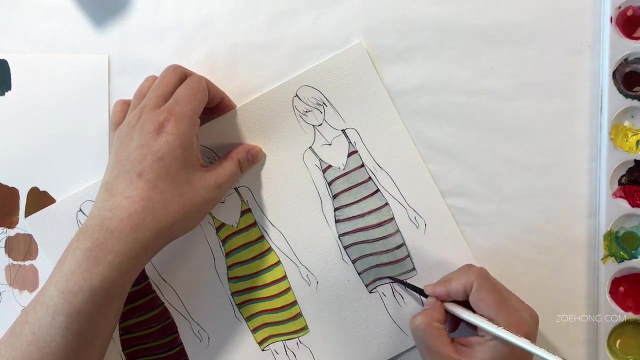 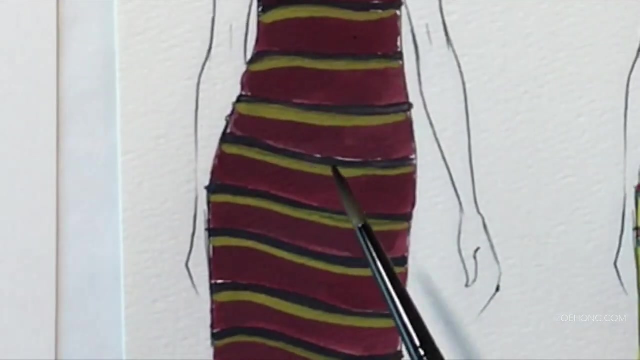 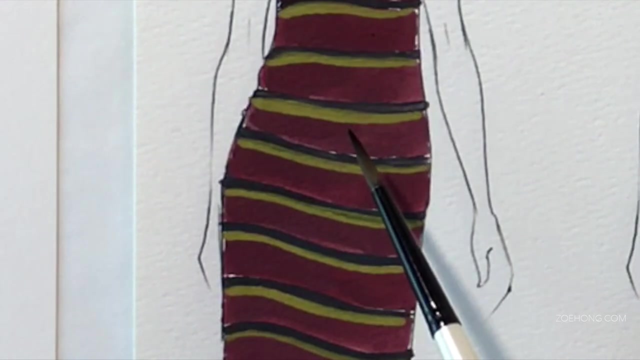 And I've been enjoying them, but they're still new-ish to me. Alright, so these three dresses- clearly not the most amazing painting jobs I've ever done, but not the point, right, Alright. this is a tone of red, this blue is a shade of a near-mute and this green is a light shade, just like a little bit of black in there. 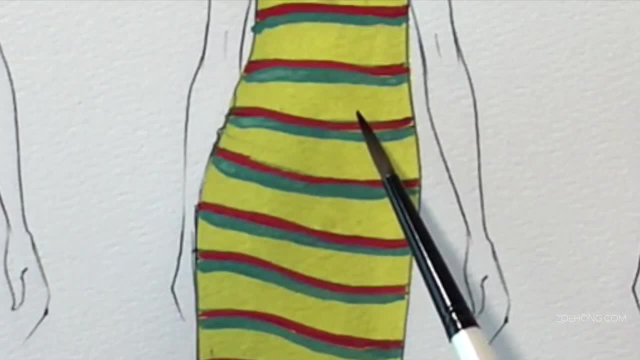 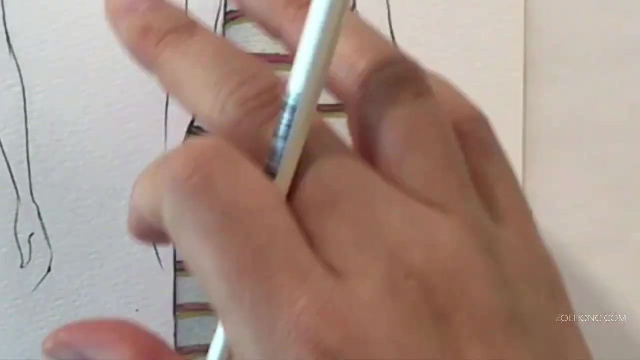 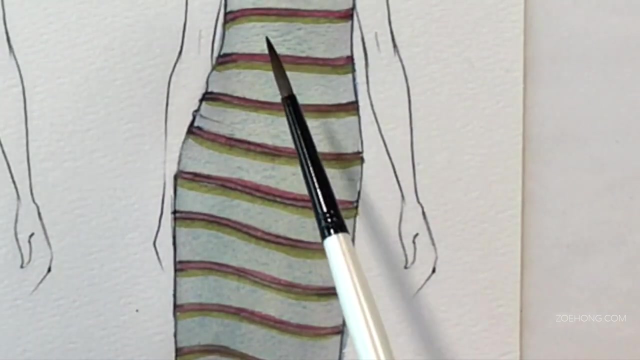 This is a tint of a yellow-green. this is pretty close to just straight-up red. and then we have this blue-green. has like a touch of red and a touch of white in it. okay, To harmonize back with the red And this is a very like tons of water added to create this very tint of a blue-green. so this is a tint of a near-mute of red and a tone of the yellow-green. 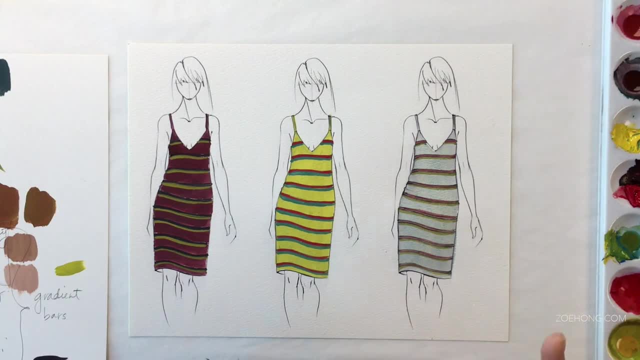 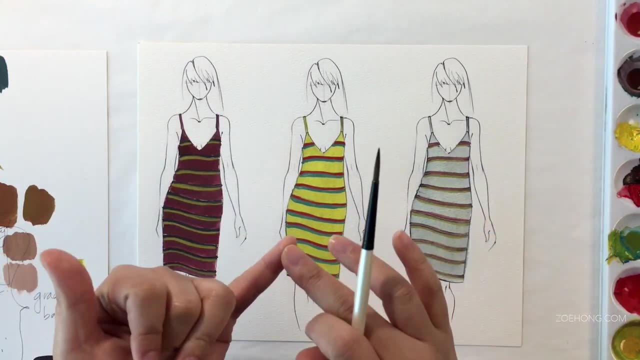 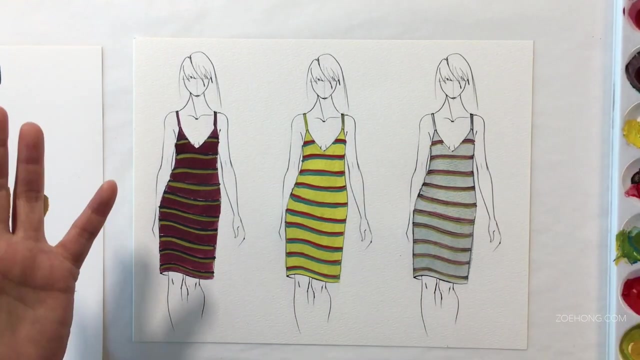 So I use these words so that you understand what colors I mix together. but essentially, every single one of these colors was painted using red, Yellow, Yellow-green, blue-green, white and black, And varying degrees of water, of course, right. 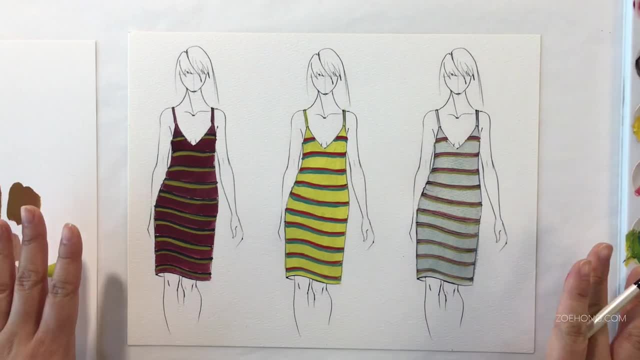 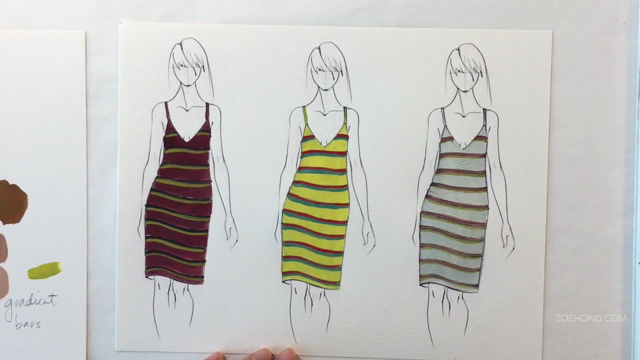 Now, which of these is your favorite? Which of these do you think is the best one? I would love to know your thoughts in the comments and think about it like this too. It's like which of these is right for your customer. 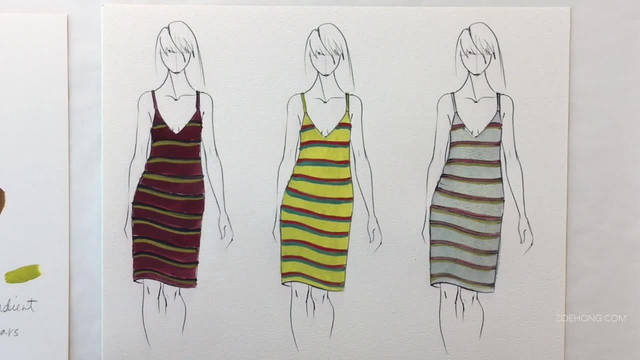 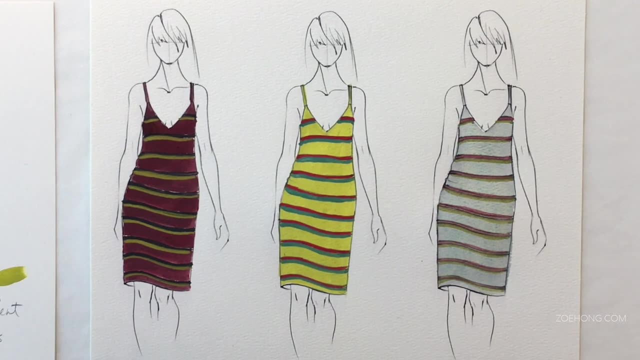 Oh, my customer is young. they like bright colors, they like something. They like something that looks fresh and vibrant. or my customer is a little bit more conservative. they don't really do loud colors, they like things looking a little bit more subtle. okay, 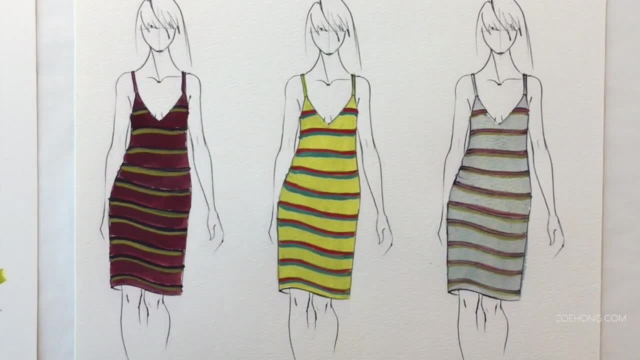 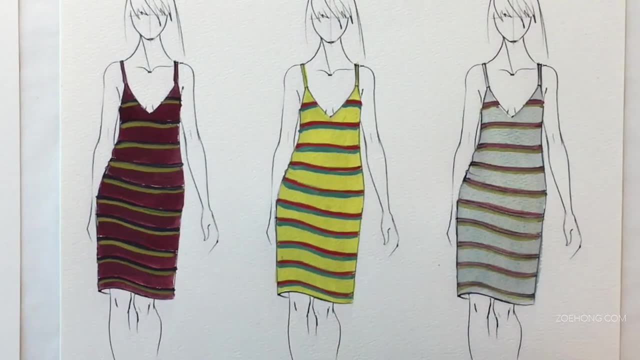 So which one is your customer? Also, what season are you designing for Which of these three colorways? Okay, so, maybe for winter you put a sleeve on it, and maybe for summer you make it a little shorter. But just the colorways. which one works for fall? 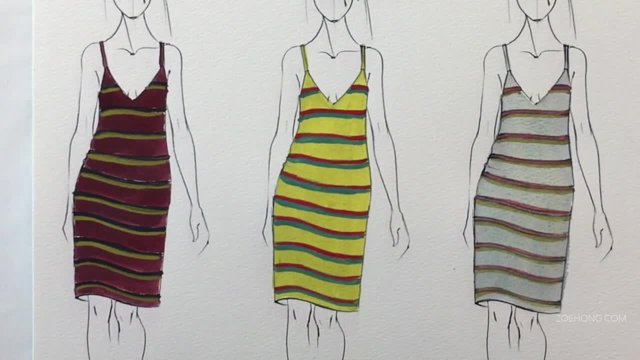 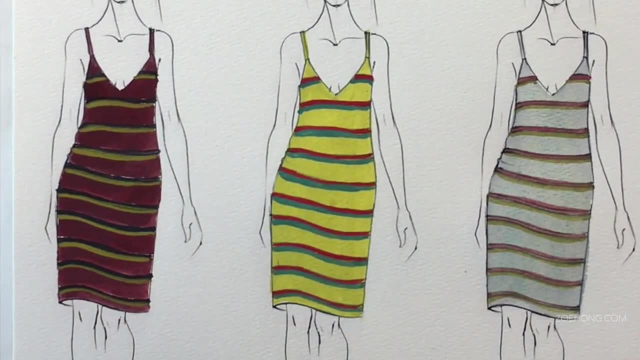 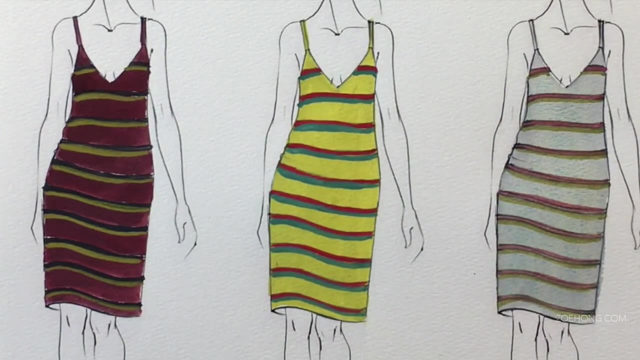 Which one? Which one works for spring or resort? okay, So you have to think about it in those terms, because when it comes to color stories, it's not usually about ugly and beautiful. It's about what's right for the customer, what's right for the age, what's right for the season. 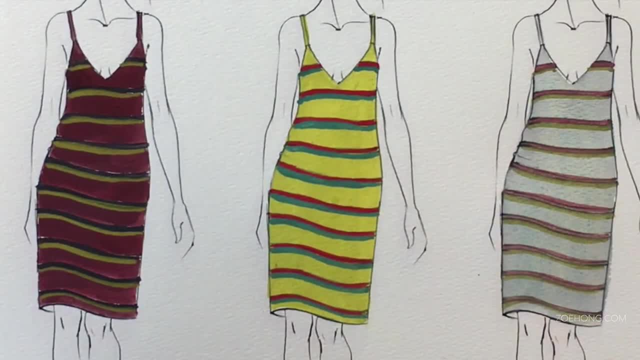 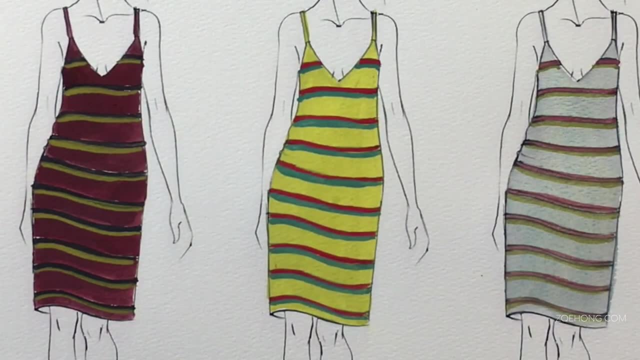 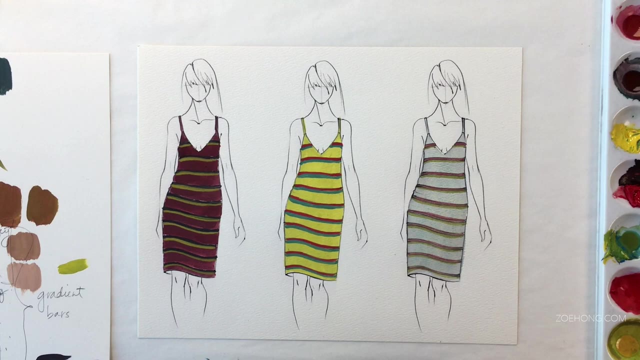 What looks right with the base fabric you put on it, Which of these fabrics would look cool on a shiny fabric And which of these would look cool on something nubbly and fuzzy? And then, in terms of illustration, okay, when I am, if you watch my painting, my football padding collection thing, videos. 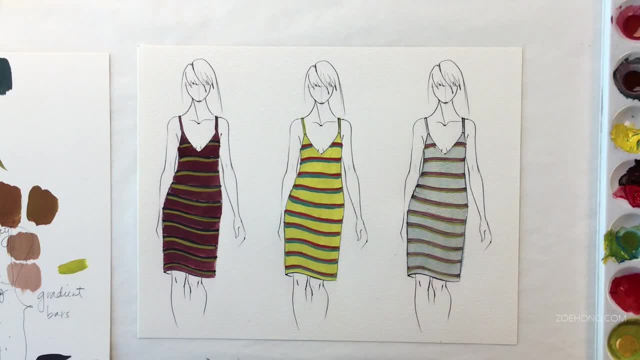 then you will have heard me say that I'm going to paint the hair at the very end, Because hair to me is like, okay, what's going to make the rest of this look good? I never start by saying: oh yeah, you know, I'm going to draw this blonde girl. 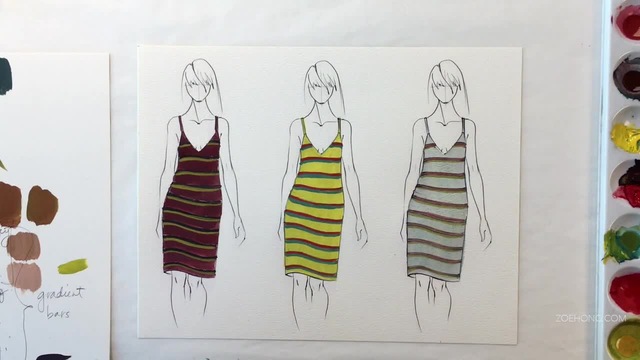 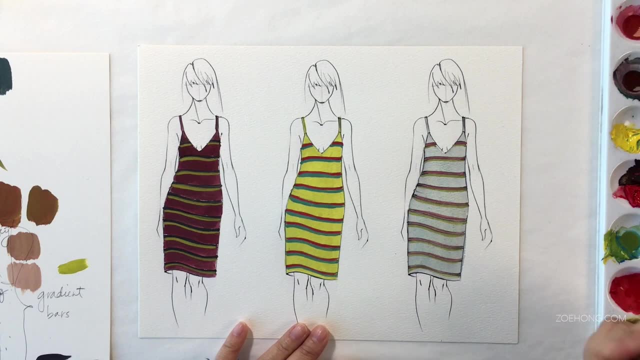 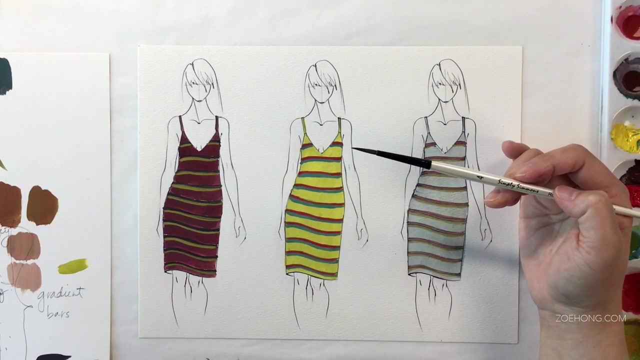 It's very rare that I do an illustration project like that. It's really like: okay, this is the fabric swatch I was given, or this is the design that I'm painting. What's going to look good with this? What hair color is going to make this dress really pop out? 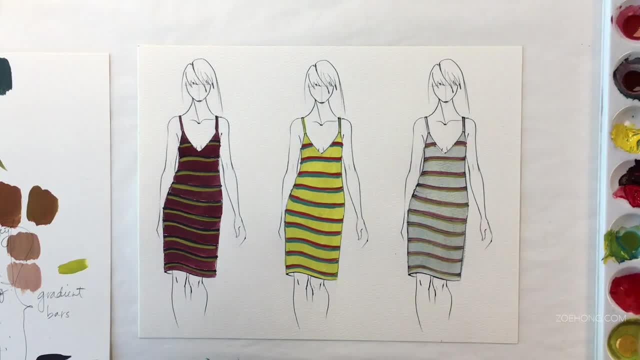 Why don't you answer me in the comments section and you give me why you think so? It's like Zoe, I think that a platinum blonde would look great on the blue dress. because, Okay, I'd love to hear your thoughts. 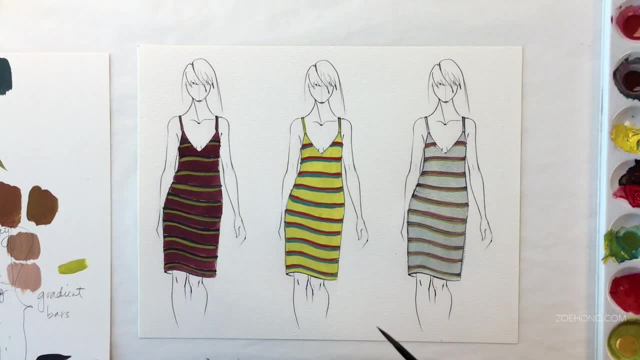 Because color theory is really about getting base information like hey, this is a split complementary color scheme, Taking that base information and analyzing it for your needs. Please do hit the thumbs up button if you found this video helpful and if you would like more color theory videos in the future. 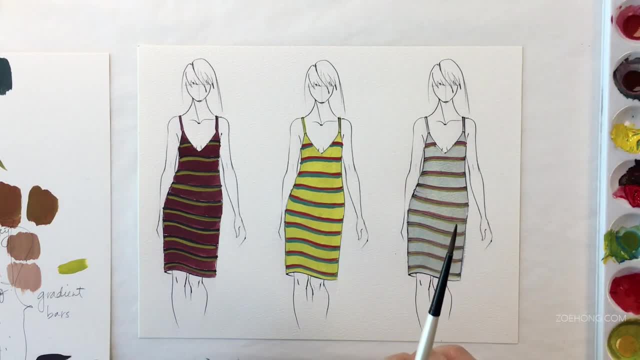 And share: subscribe. Oh, don't forget to hit the gray notification bell, because apparently you don't actually get notifications if you don't hit the bell, Even if you subscribe. That's how it works, apparently. Go paint some swatches, go mix some colors, practice hashtag. always be practicing, and I will see you in the next video. 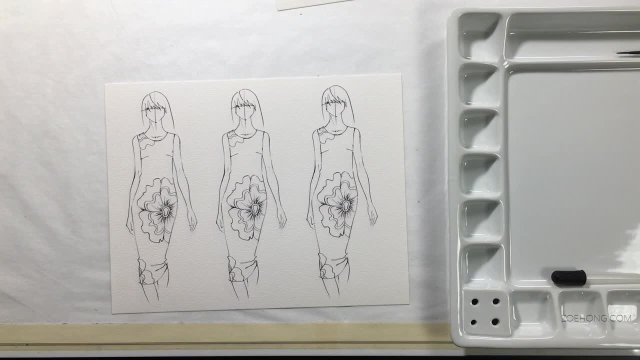 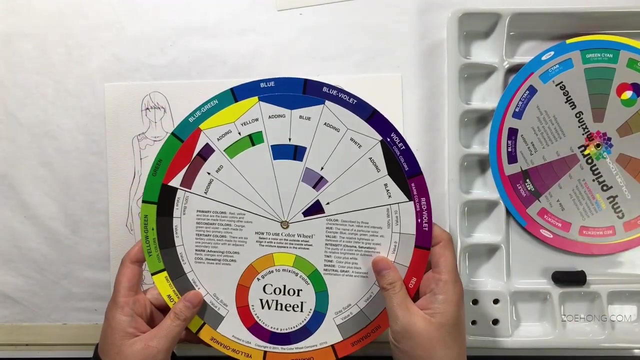 Hey, hey party people. In this video I want to show you how color theory concepts translate in practical application to fashion design. I have mentioned this before, but I use two different color wheels. I use your standard red, yellow and blue color wheel. 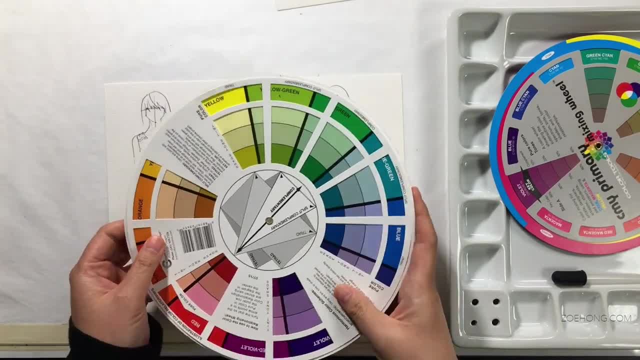 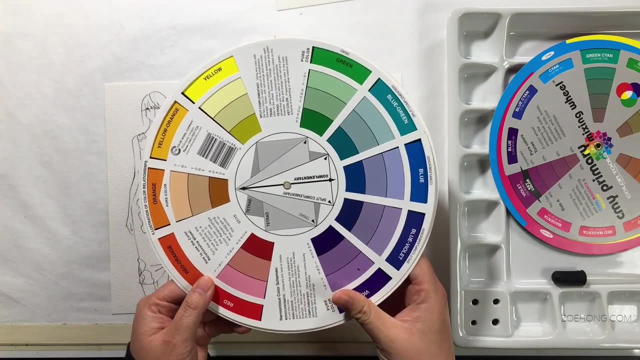 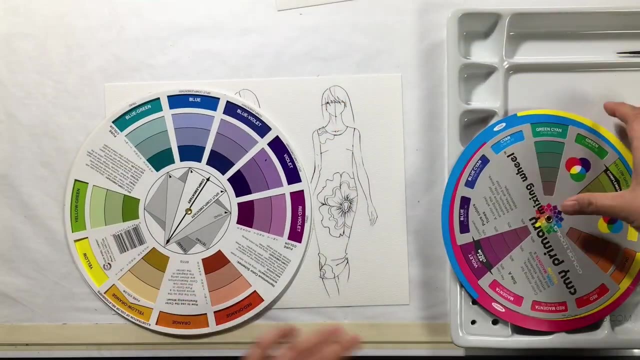 For design purposes, for matching colors, for figuring out what goes with what, figuring out color schemes. and then I use a cyan, magenta, yellow, black color wheel for the actual mechanics of color mixing. And today I'm going to paint using inks. 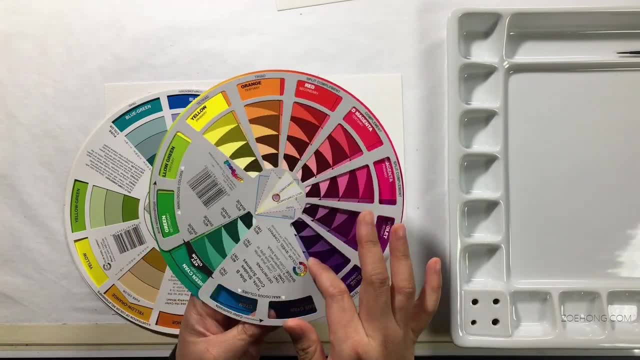 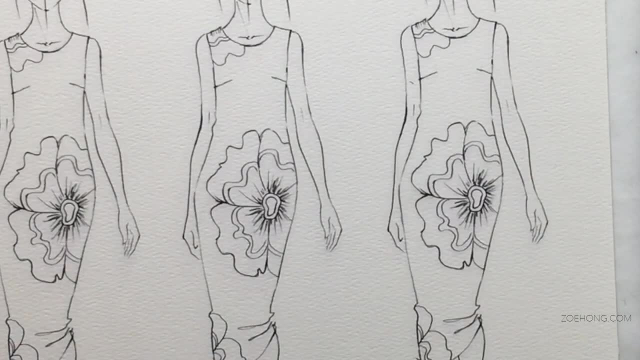 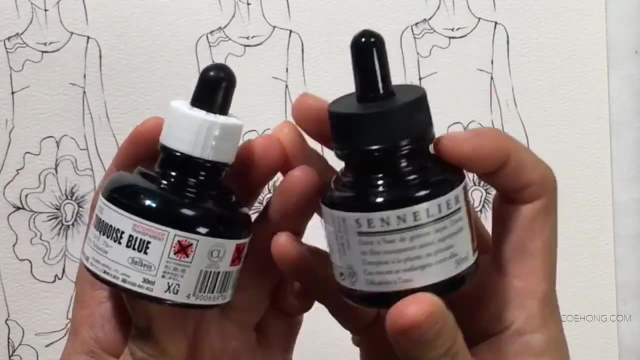 You all always like to know what materials I'm using, So briefly I will show you. today I'm going to experiment with Holbein inks and liquid watercolors, basically, and the Sennelier inks I'm using Bien Fang watercolor paper cold press 140 pound, et cetera, et cetera. 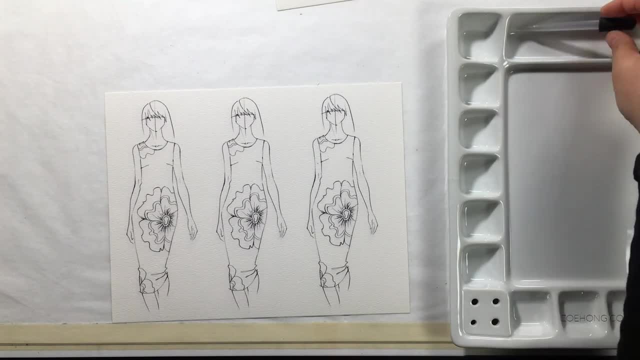 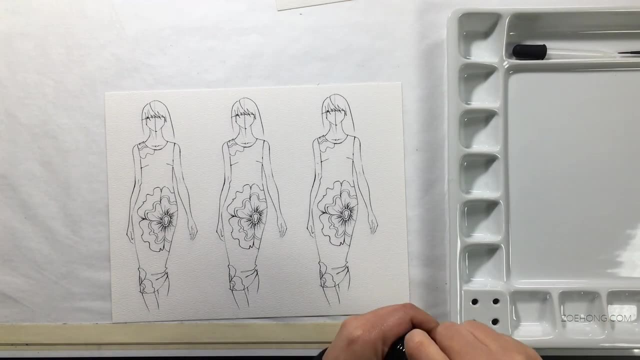 And I'll put all the colors and you know the specifics in the description box below. But just know that with the inks I'm still experimenting. I don't have an opinion on these inks yet. I'm going to experiment with them. 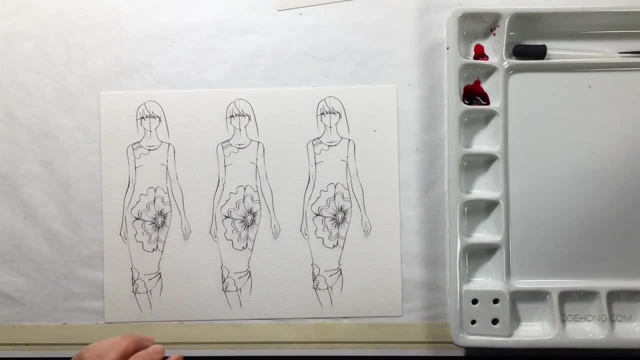 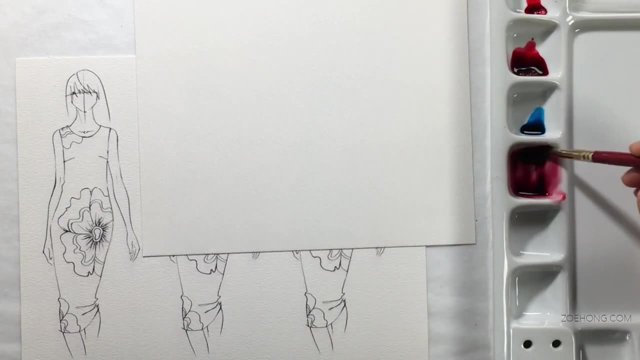 I'm going to experiment with them. I'm trying to use them more so that I can give you a proper product review later on. So first I'm just mixing up some colors. So I have these three dresses here. They're identical in design. 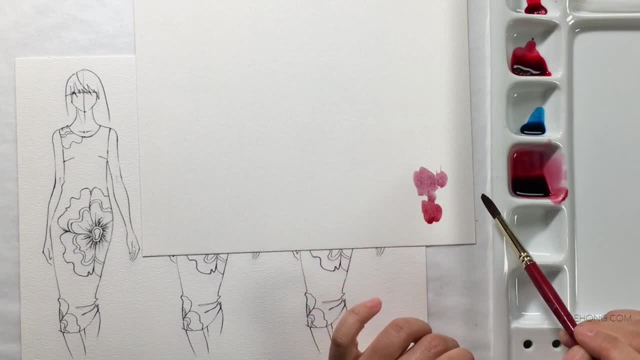 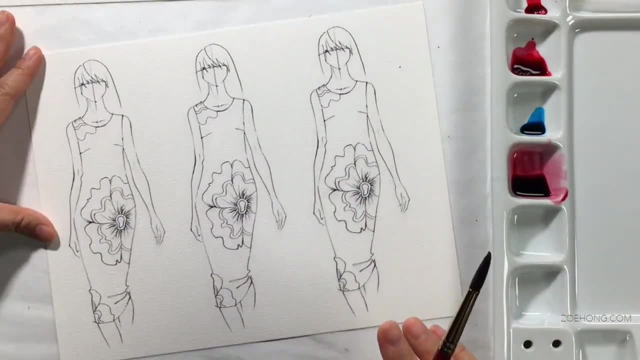 And I'm going to paint the flowers in the same red color. It's a cool red, you know more, a little bit tinged with a little bit of blue, As opposed to a warm red which is tinged with a little bit of yellow. 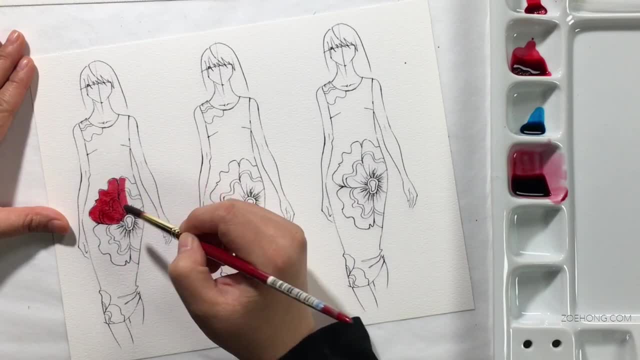 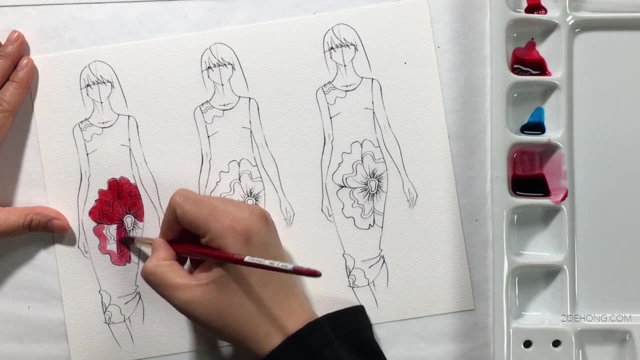 And it's got a tiny bit of black in it, So it's a shade of a cool red. Remember, shade is color plus black, Tint is color plus white Or, in our case, color plus water, Because water is how we lighten watercolors typically. 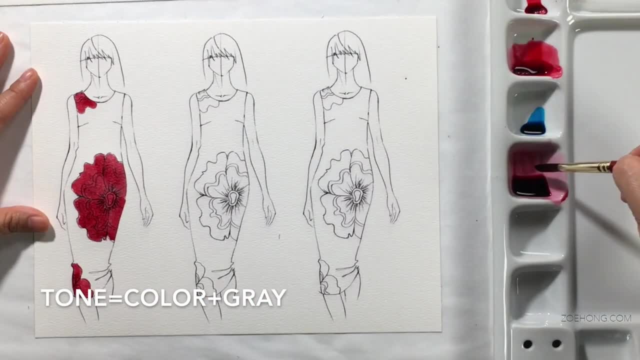 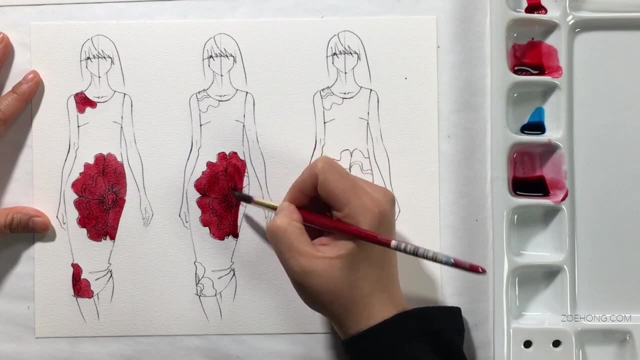 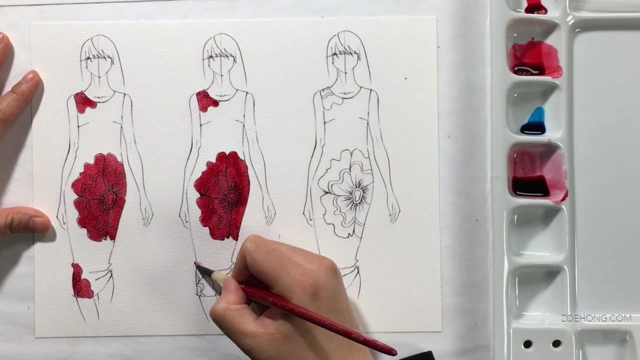 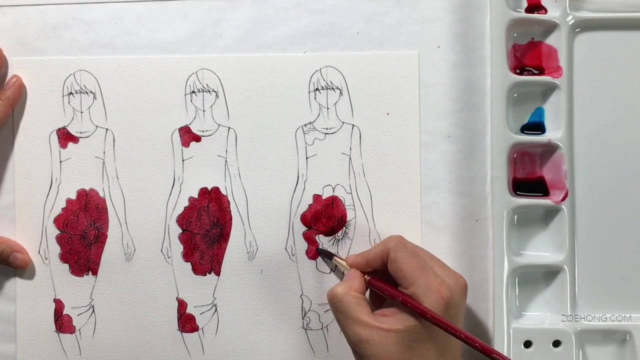 And tone is Tone is color plus gray, And so I'm going to do the flowers of this print on all three dresses the same, And I'm going to paint the background fabric color in different colors so that we can discuss how to choose the right color for your design. 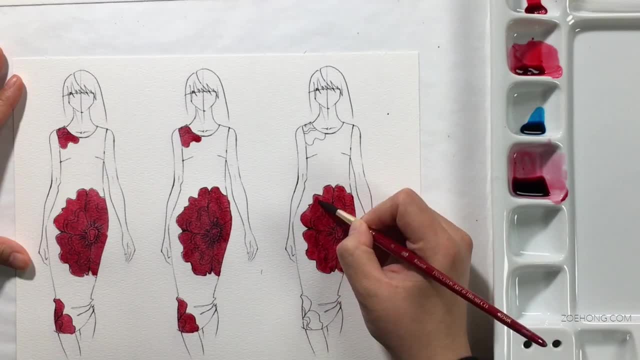 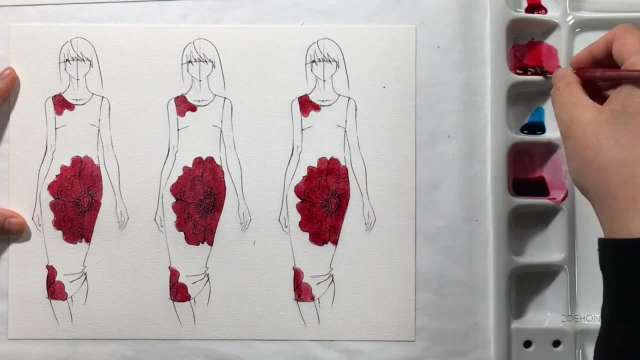 Because you know, color theory is not like math, where there's so much color, There's so much color, There's so many clear-cut. yes, no, right, wrong answers. In math, 4 plus 2 is 6.. 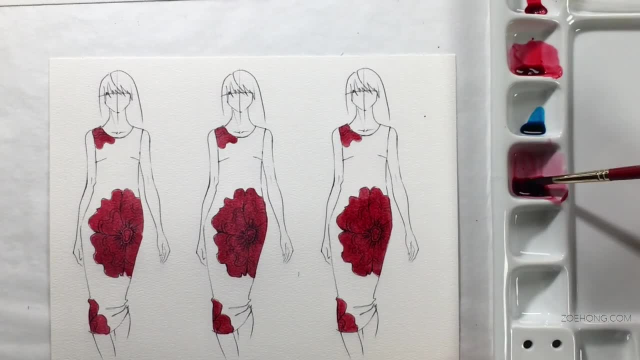 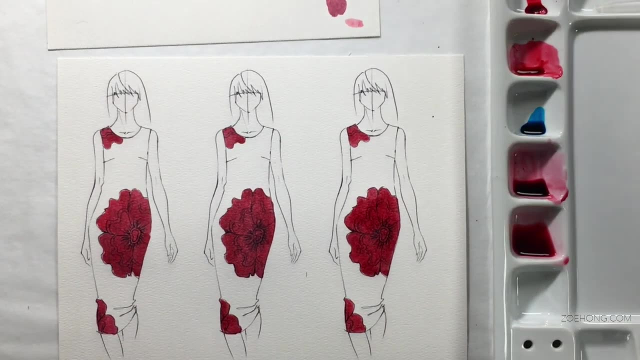 That is it The end. Have a nice day. That's not how color theory works. Okay, Color theory is more like: okay, what is the message you're trying to give your customer? What kind of look are you going for? 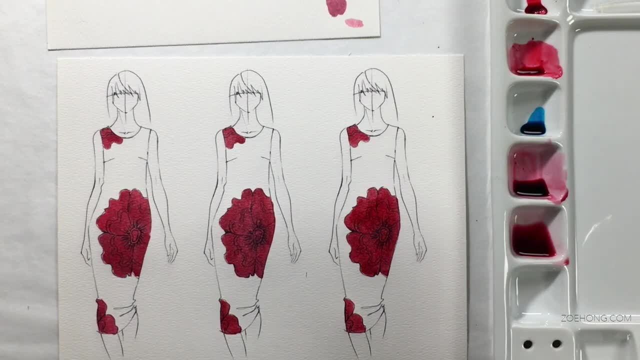 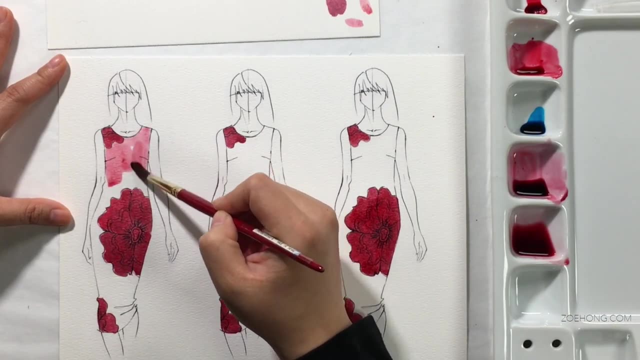 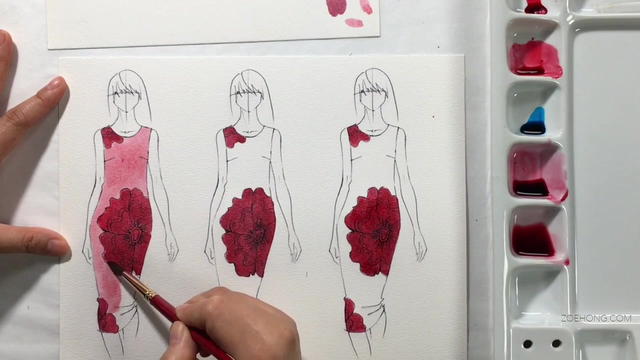 What kind of mood are you trying to convey with The color palette that you've put together? okay, Are you going for, you know, aggressive, assertive, strong. Are you going for soft, muted? Are you going for melodramatic? 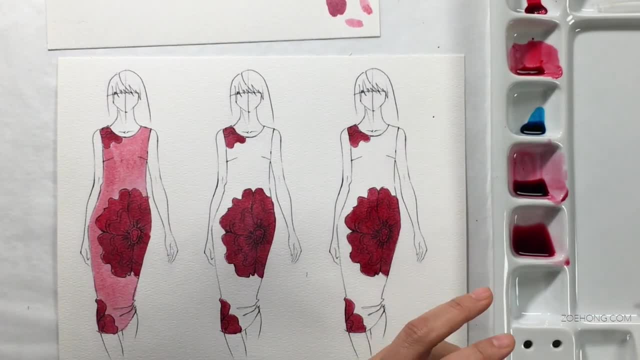 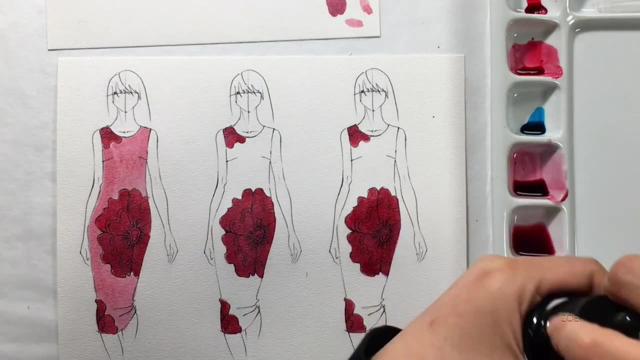 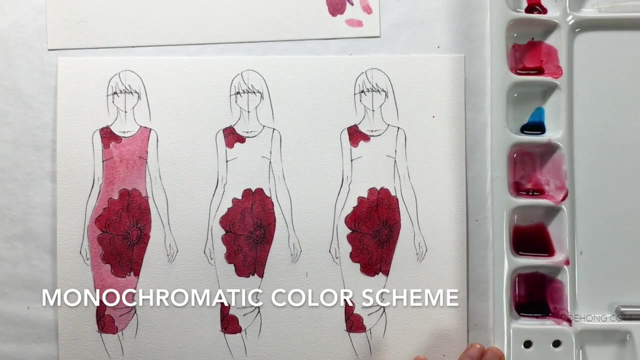 Like what do you? you know you find the color story that matches your collection. Now this first dress. I am using a monochromatic color, So I took that first cool red, added a ton of water to it and now I have this. it's. 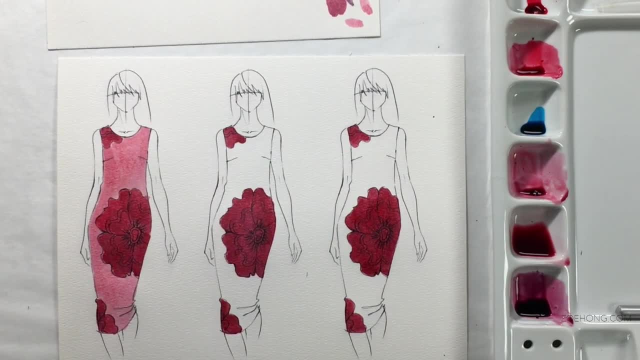 not, it's like I wouldn't even call it pink, It's like a soft red, okay. But when you have a monochromatic color scheme, you know it's an easy harmony because the color base is the same okay. 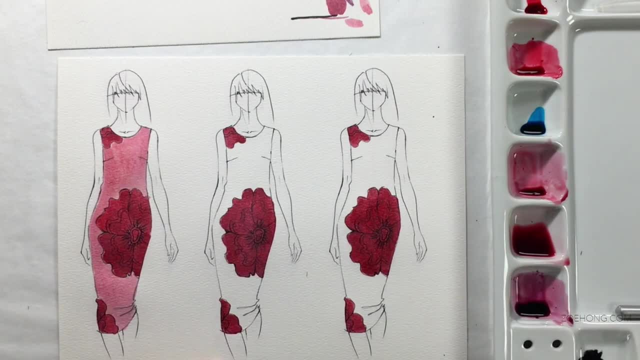 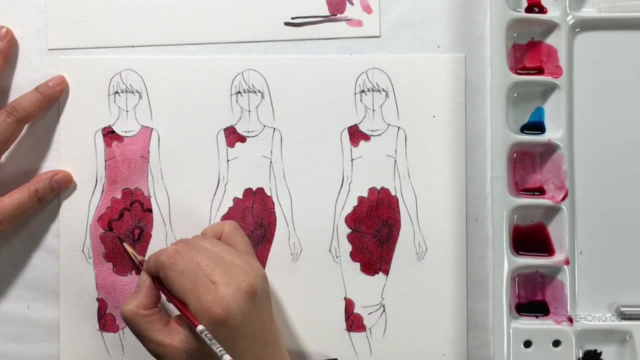 Remember, monochromatic color schemes doesn't mean that all the colors are the same. It means that you have a color and you use tints, shades and tones, Tints, shades and tones of that color to create the color story. 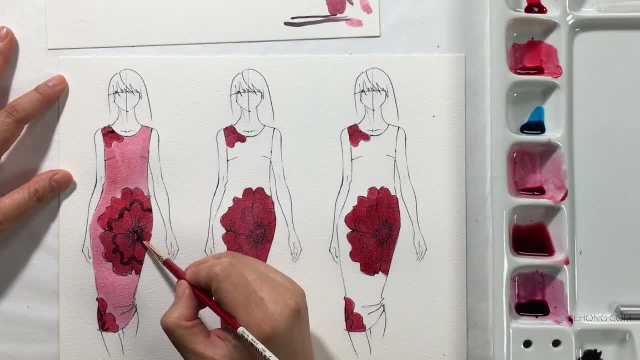 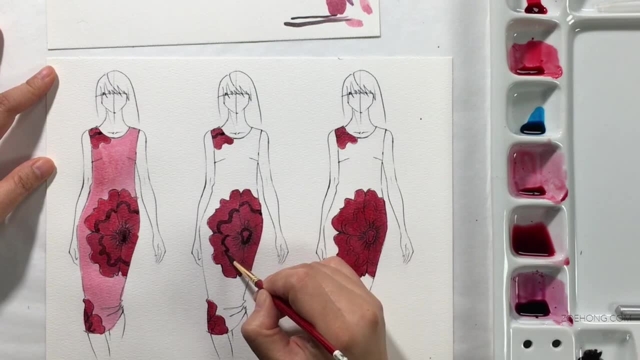 So this first dress is monochromatic color story. okay, And you have a very strong red. you know they're desaturated reds. There's not a red, that's like a very bright poppy stop sign red, But it's a red color story. 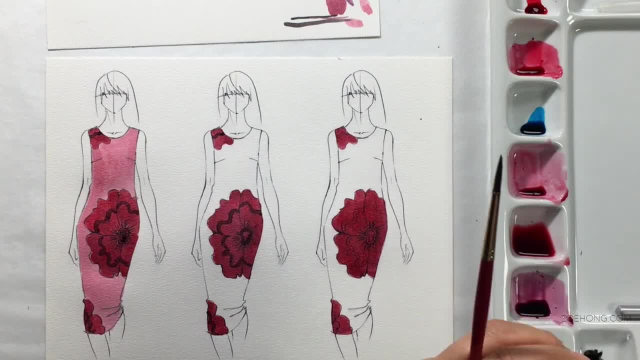 You're kind of giving that message. This is a message. It's very feminine, okay, because of so much red. That's also looking on the pink side. It's got flowers, so it's already got more of a feminine look and you're really pushing. 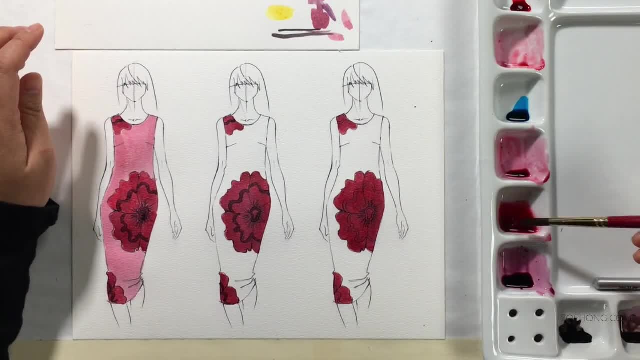 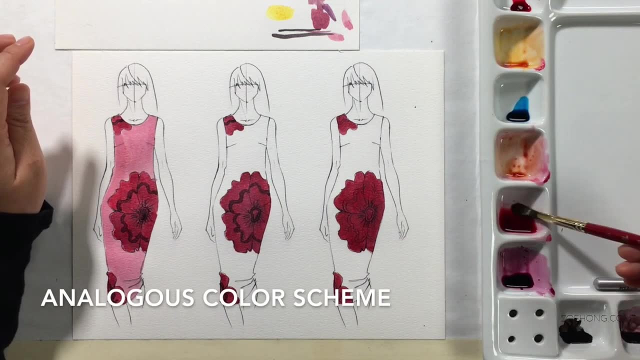 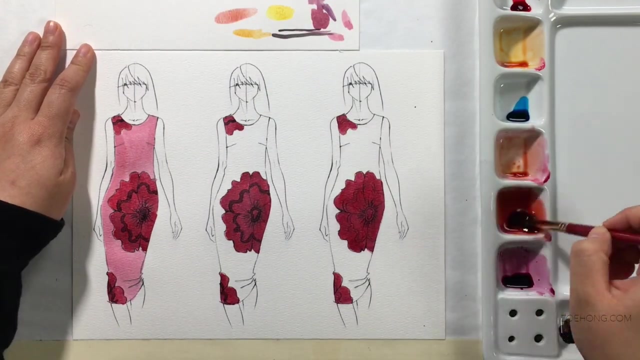 that. Now the second one, I'm going to use an analogous color scheme. An analogous is: if you recall and if at some point you get lost, go watch that first video in the color lessons playlist that goes over all these vocabulary words in depth. 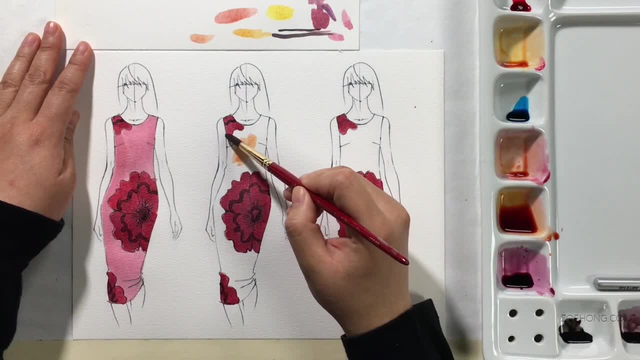 Analogous color scheme basically is using colors that are neighbors. It's on the color wheel, So if I'm using a red, what are its neighbors? You can go warm side and go red, orange, orange, yellow, orange, yellow. 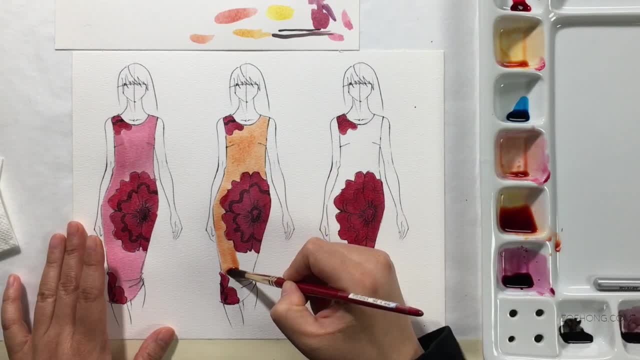 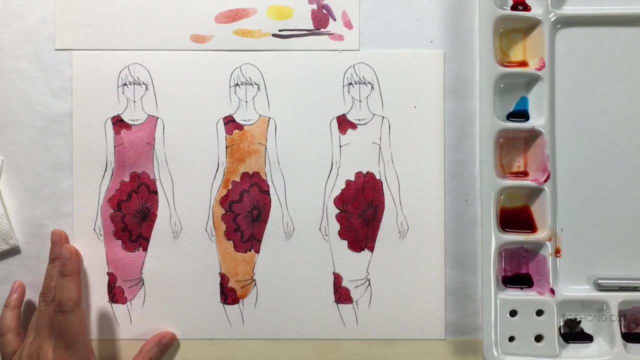 Or you can go cool side and go red, red, violet, violet, violet, blue, like in that direction. Or you could do a little bit above. You could do like a little red, red orange and a little red red violet, that kind of. 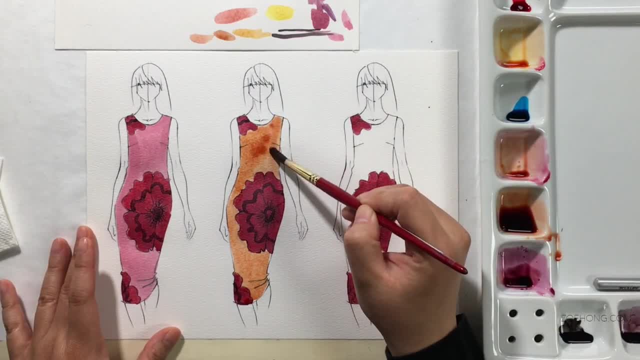 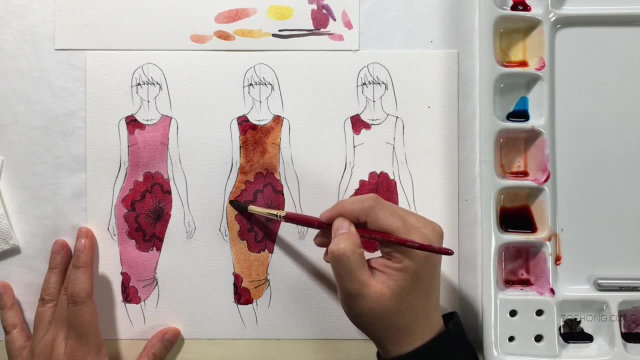 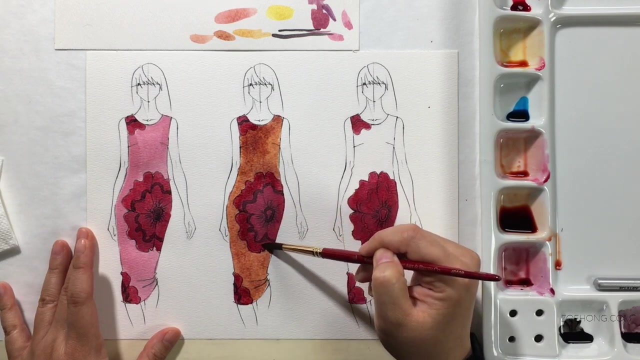 color family And in this one, So that I can have a distinct difference between the first one and this one. I'm going for a desaturated red orange And I am purposefully using not the perfectly saturated colors that you see on the color. 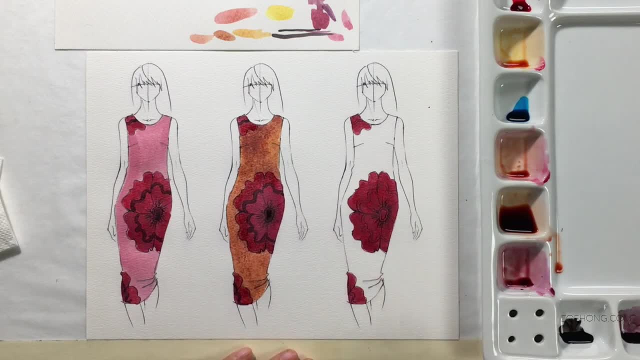 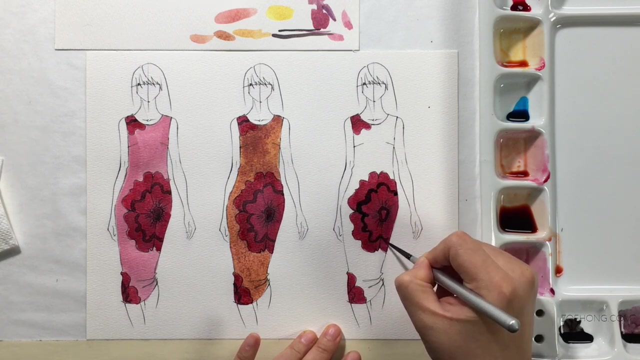 wheel, because we often do not design with those colors. So I'm using the red orange. I've desaturated it a lot. It's a shade. I added a tiny bit of the Higgins Black India ink and I've turned it almost brown. but 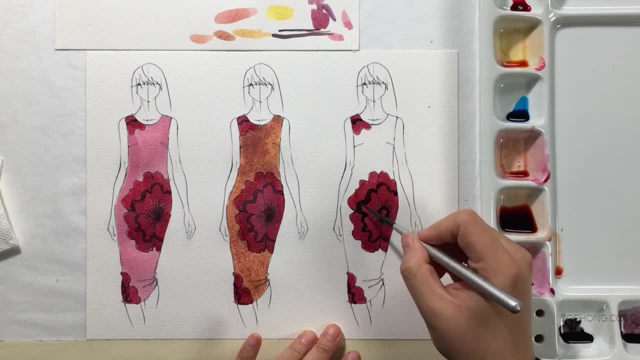 it gives an overall earthy look. Now, when you look at the first two dresses to me, I look at the first one and I think spring, This would be appropriate for a spring collection with the lightness of the pink, pink, soft red. 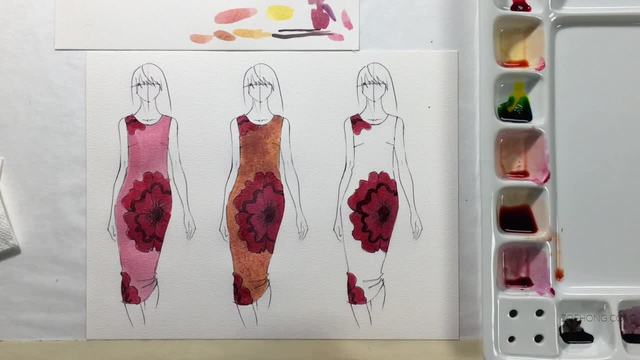 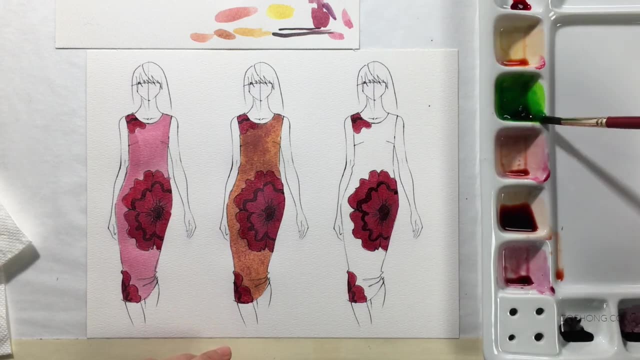 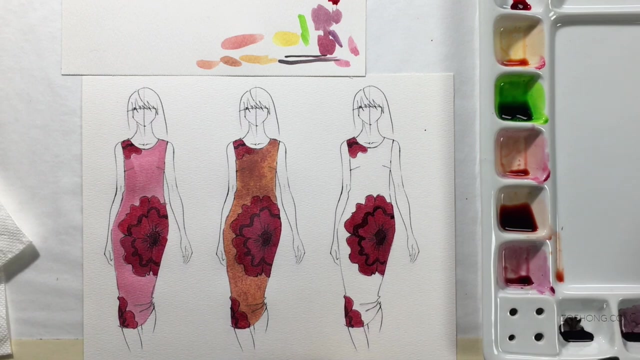 And the second one: because of the warmth of the red orange shade It looks more appropriate for fall. I deliberately tried to choose very kind of like neutral silhouettes so that that wouldn't make you think one way or the other but really give the message with the color. 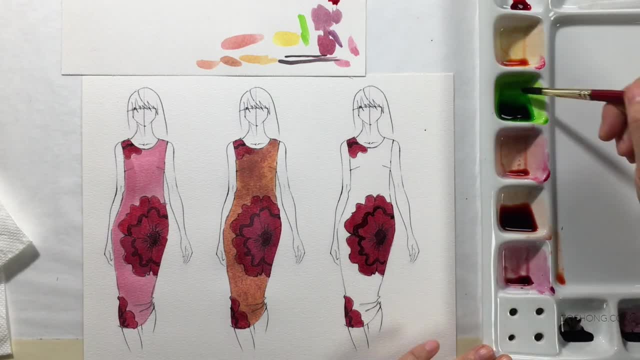 And I think that warmth, with the brown and the dark red coming in together, that gives more of a fall look, that gives a little bit older, slightly more sophisticated look as opposed to the monochromatic shade, So I'm going to go with that. 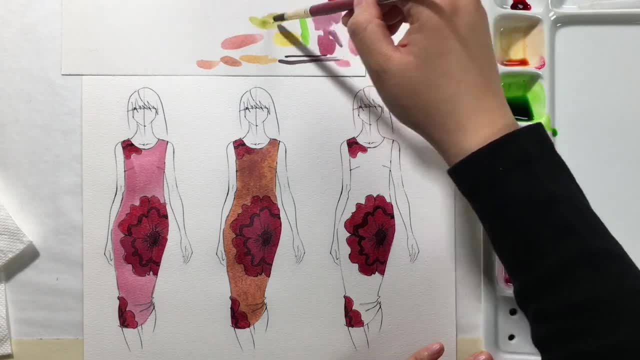 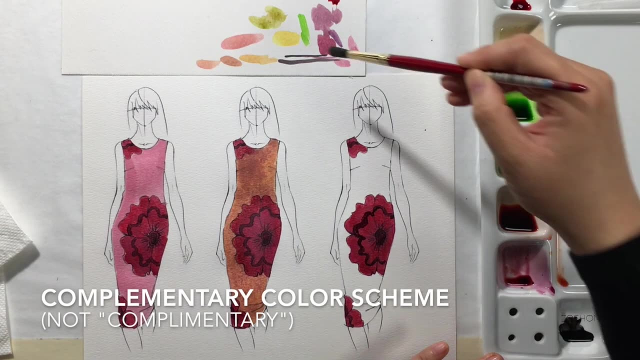 I'm going to go with that. I'm going to go with that. So the second color scheme. what do you think? Now this third one. I am applying a complimentary color scheme, So complimentary colors are opposites on the color wheel. 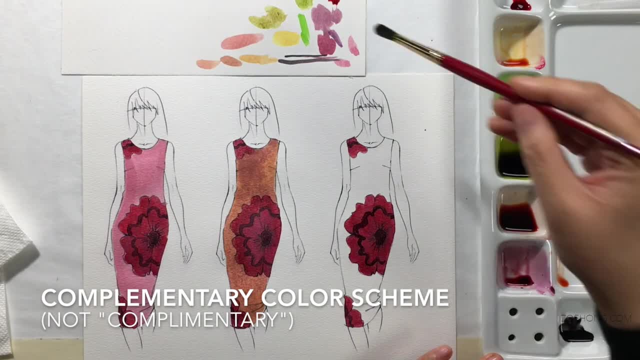 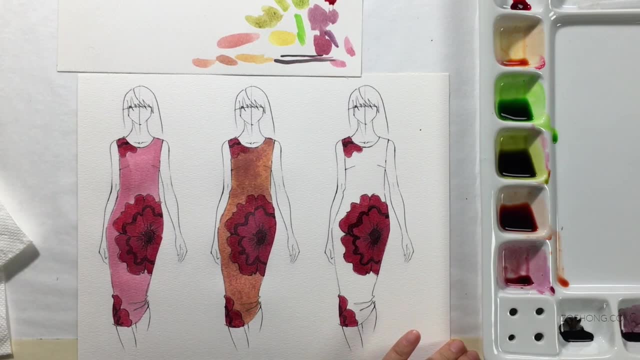 Reds complement is green, So I'm doing the background in green, but I don't want it to look like Christmasy. Okay, That's the thing with red and green is, if you're not careful it looks Christmasy. but 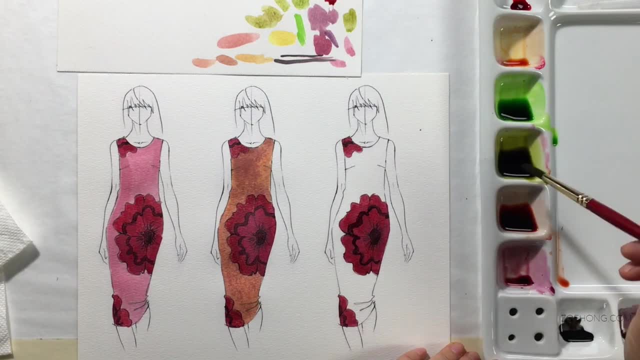 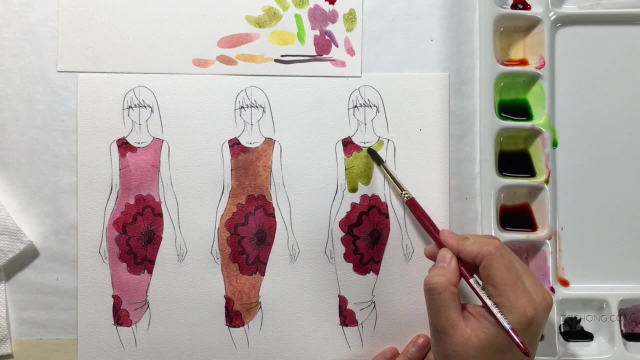 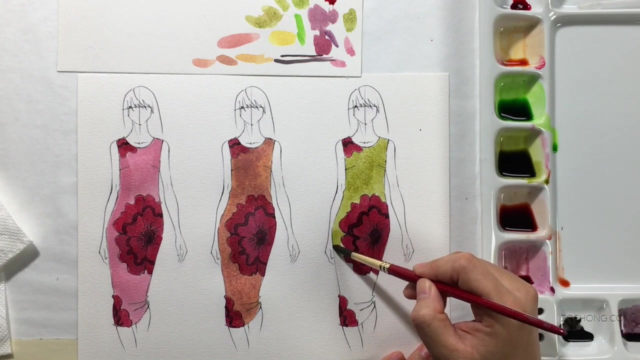 one. I created a muted green. Mutes are color plus complement to create a more neutral color, and so I've got a tiny bit of that reddish undertone to the green so that it harmonizes back to the red and you create this red and green color. 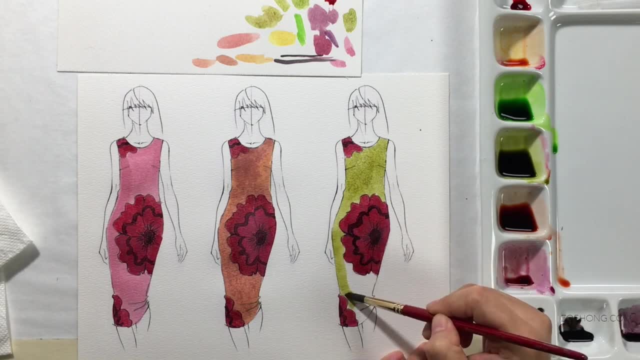 palette that doesn't look Christmassy, But because the colors are complements, the number one thing they do is make the other color pop while still harmonizing together, and so the green looks more fresh and vibrant and the red looks brighter, because the fact that they're 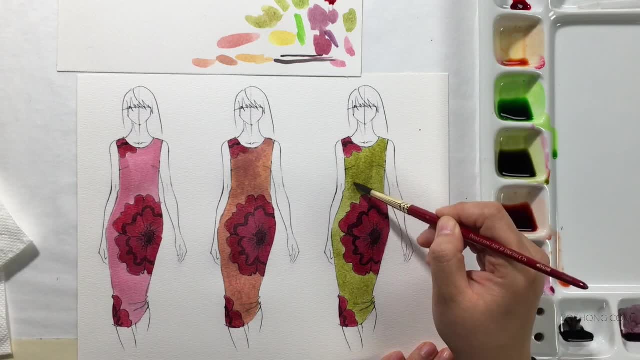 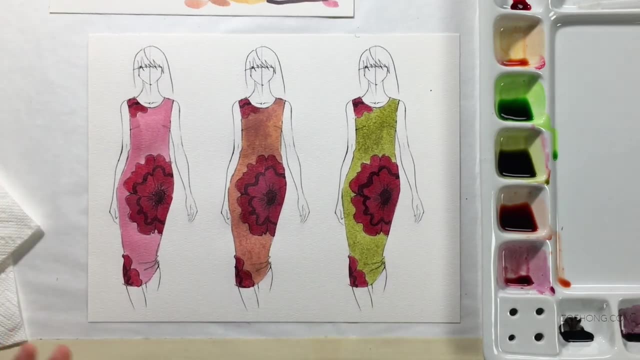 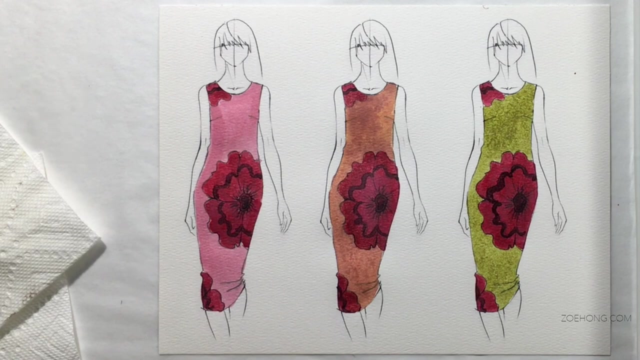 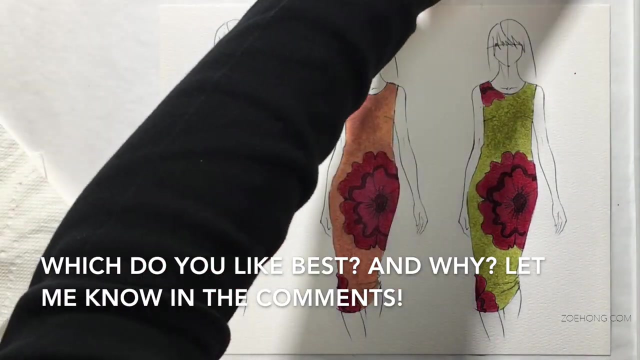 sitting next to each other. Remember the whole thing about color theory is the whole point of color theory is that colors don't matter by themselves. Colors always look different depending on what color you put it next to, and figuring that out you know, figuring how colors work together and how they look together. 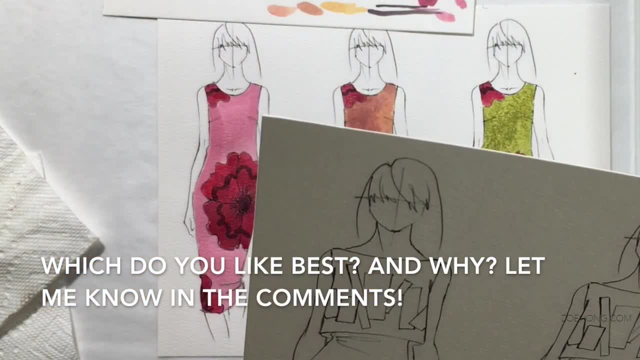 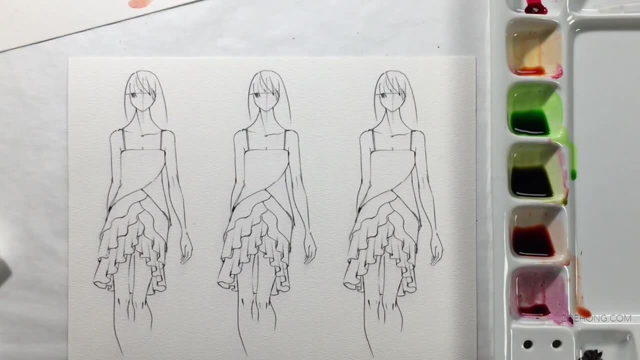 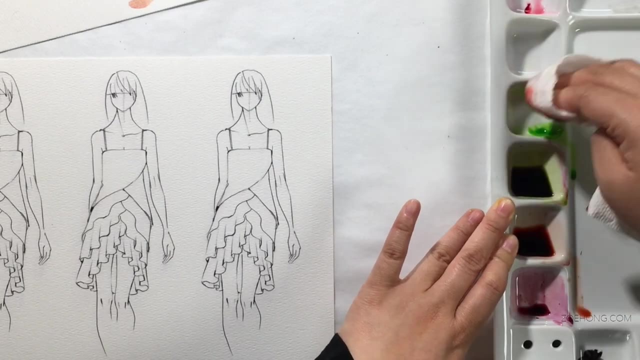 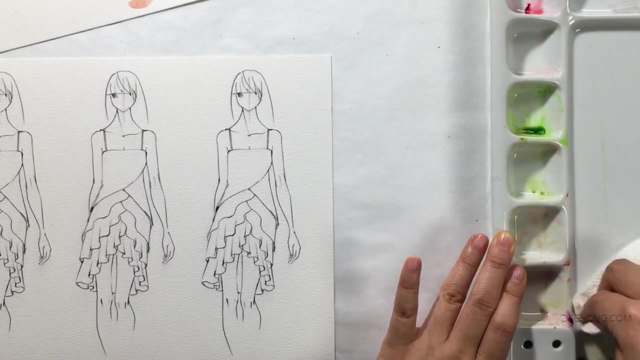 is what is going to help you be a better designer. The next concept I want to discuss is value: value usage and value placement. Value is the lightness or the darkness of a color. Okay, so in a previous video I talked about high key. 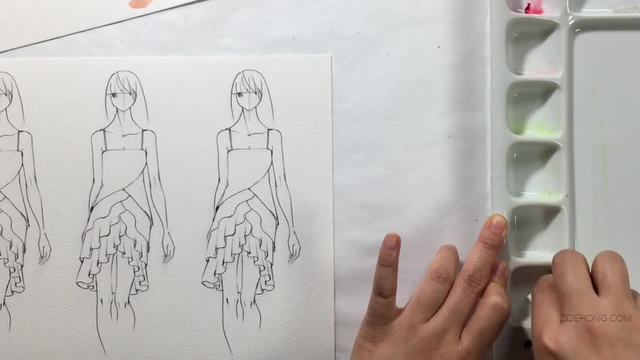 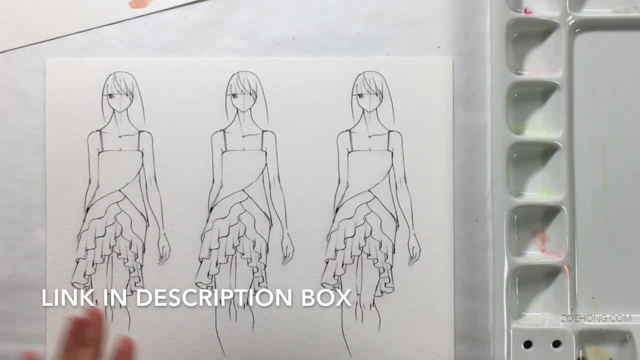 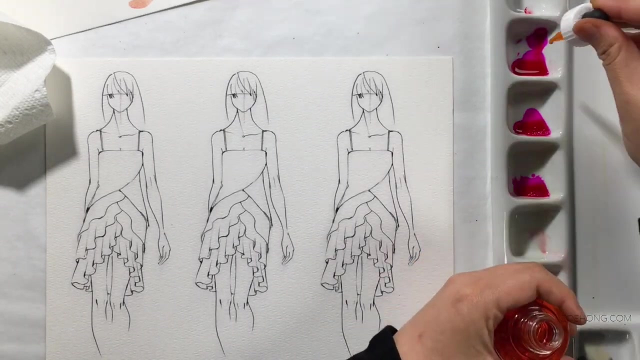 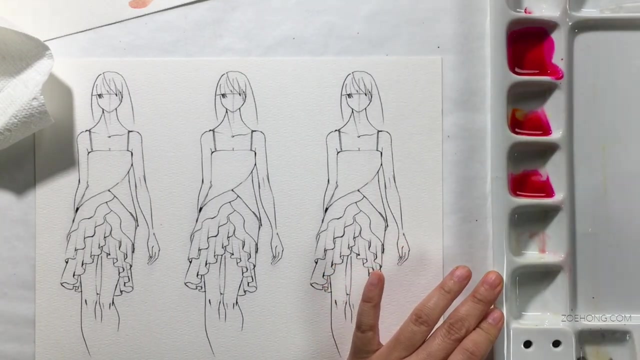 middle key, low key. I think that was in the multi-figure composition video, where I talked about how value creates mood and how it creates composition, and- and I mean that one- it focuses more on the multi-figure composition, but the concepts are still the same for a singular dress, and so where you place, 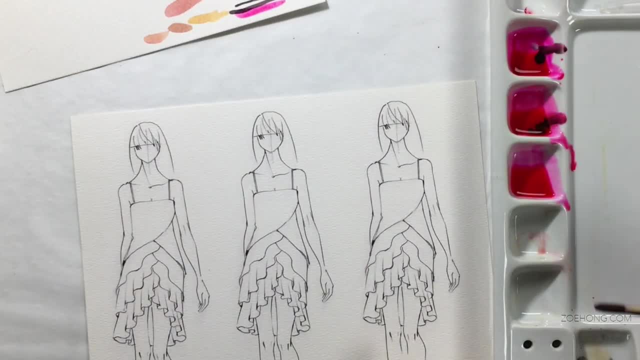 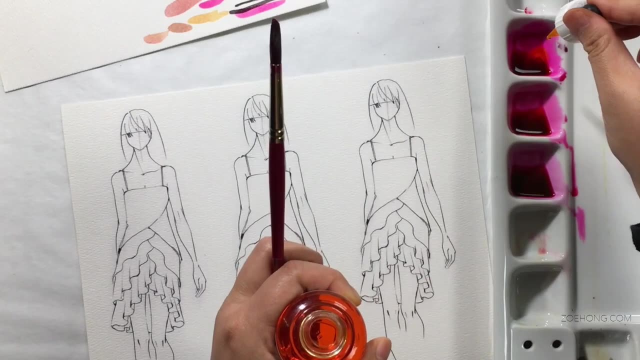 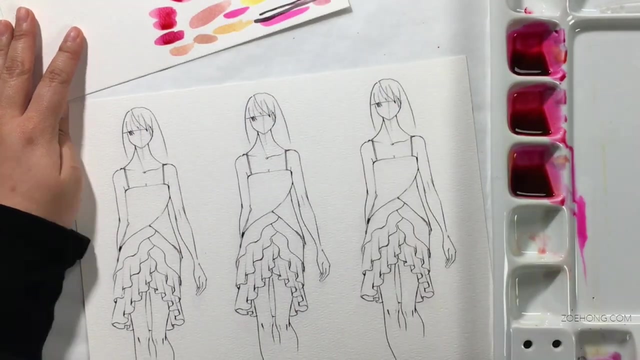 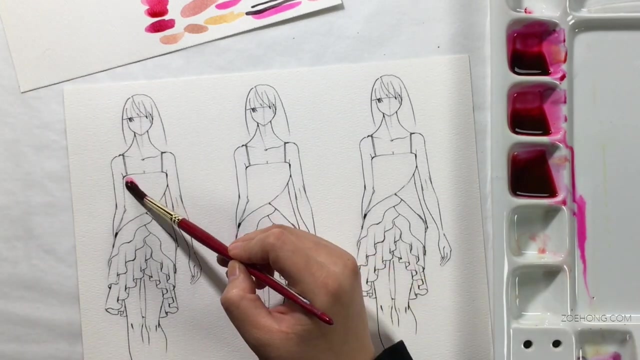 your light colors, where you place your dark colors in your middle colors and how you use dark colors and all that. all those things add to the design, add to the effect, the overall effect, and so that's something I want to show you in these three dresses. in this first dress, I'm keeping things fairly middle-key and 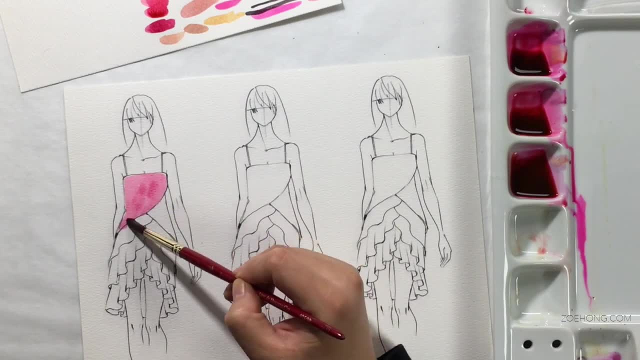 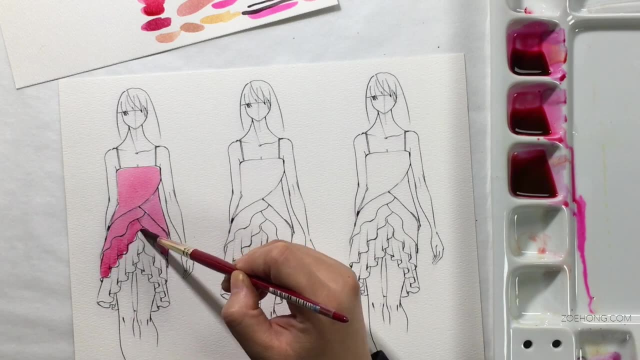 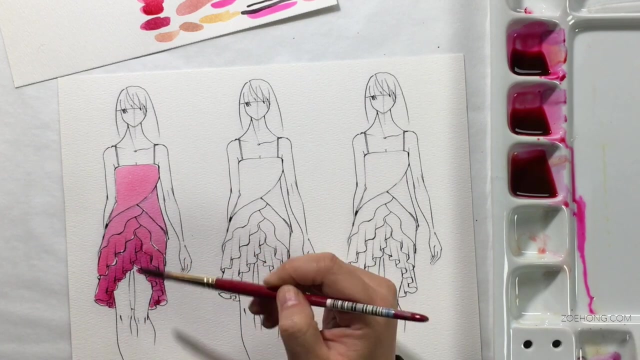 I am going to create a gradient where the ruffles towards the hem get darker, but I'm still keeping the value range fairly narrow. okay, I'm not creating a lot of contrast. okay, I want, in this particular instance, I want something that's a little bit darker and I want something that's a little bit. 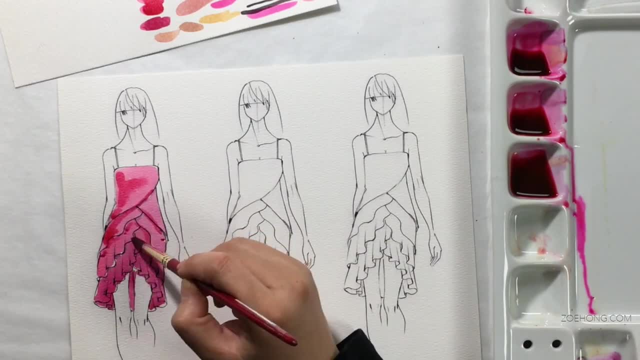 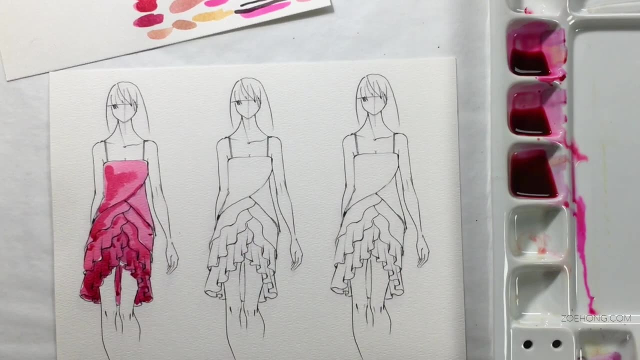 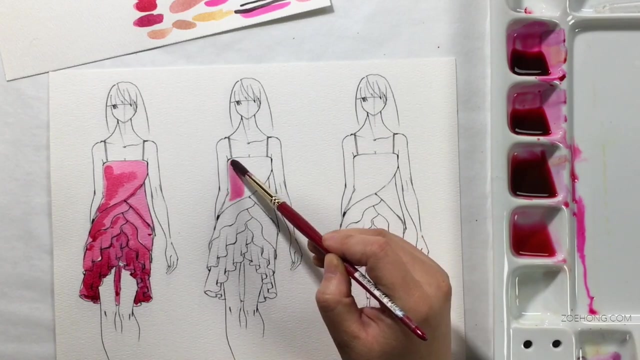 softer transitions. okay, I still want the gradient. I want the visual interest of the gradient, but I want to keep it kind of a narrow focus. side note: this ink dries so fast I had no time to blend my shadows, oh my god, so that painting doesn't look great. right in this middle dress, I am creating the gradients again. I'm creating the gradients again. I'm creating the gradients again. I'm 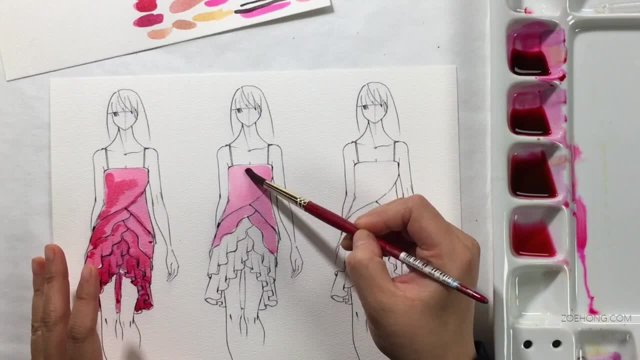 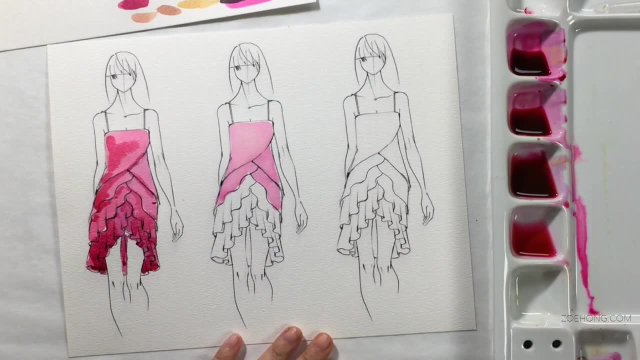 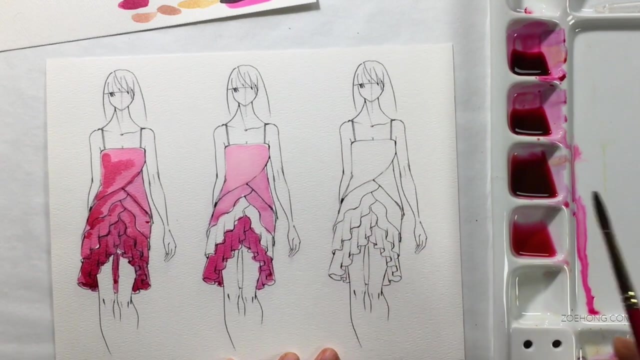 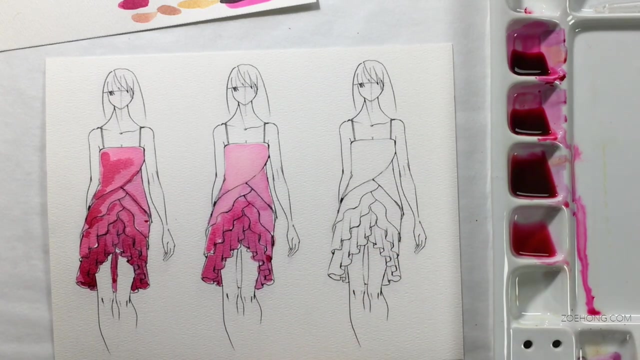 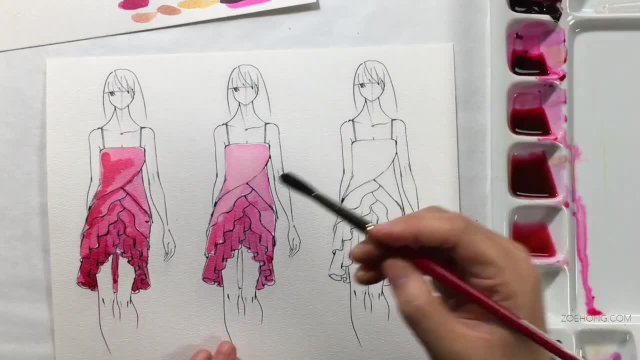 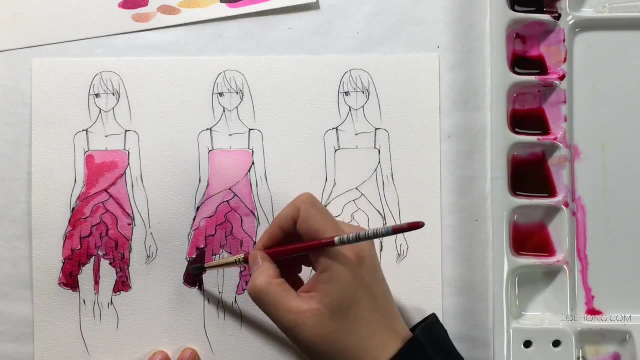 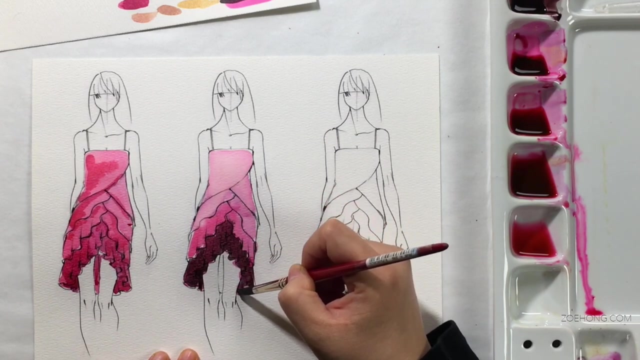 this burgundy color for the bottom ruffles and then so you have the full range. which do you prefer? do you like the narrow middle key color range or do you like the extreme pale pink to the burgundy? there is no right answer. this is your preference, this is the design, this is the process. 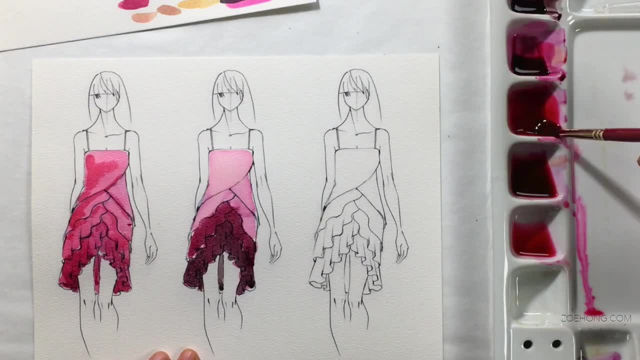 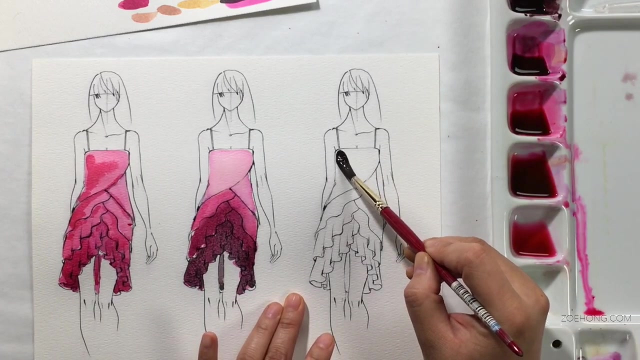 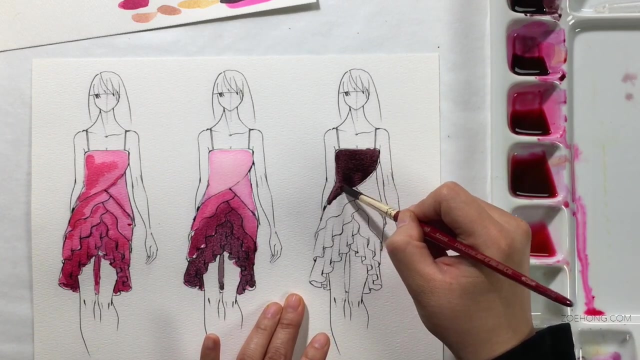 because the thing is honestly like: i can think something is ugly and you can think it's beautiful, or vice versa. what i'm trying to push onto you as designers is make deliberate, educated decisions on how to use color. okay, you'll get to a point where things come naturally. 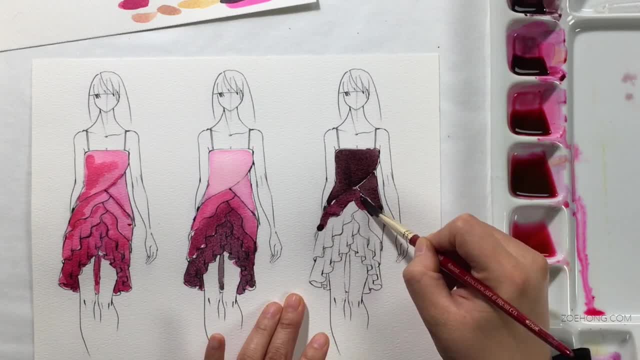 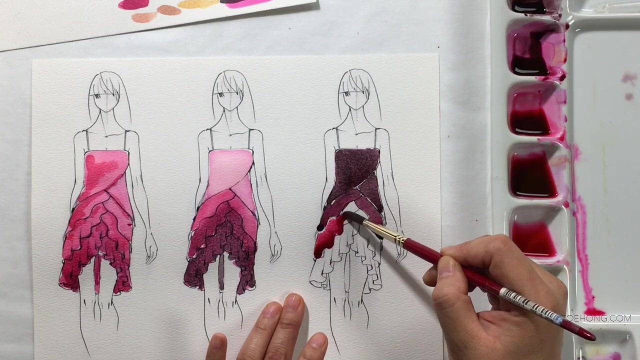 and you're not thinking in terms of color schemes and how to do this and how to figure things out in the most academic way. it'll become more of a natural instinct, but that requires time and practice. In this last dress, I am putting the darkest values on the top and putting the lightest. 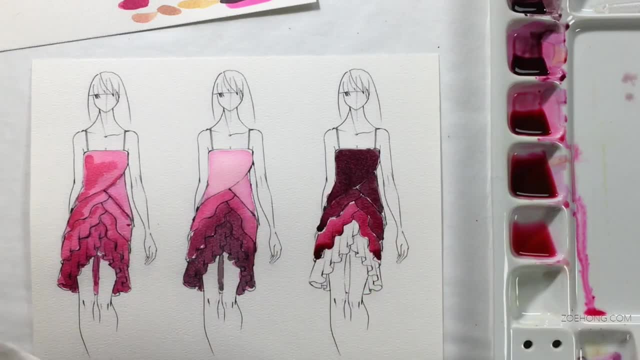 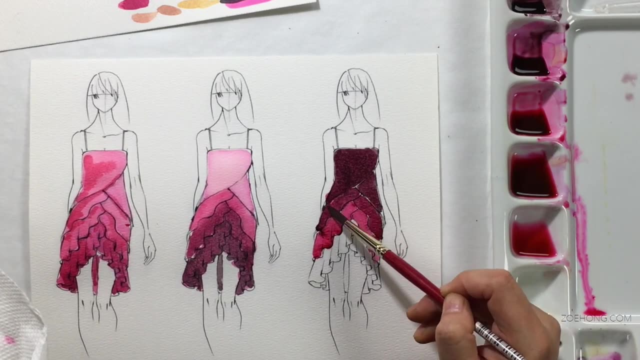 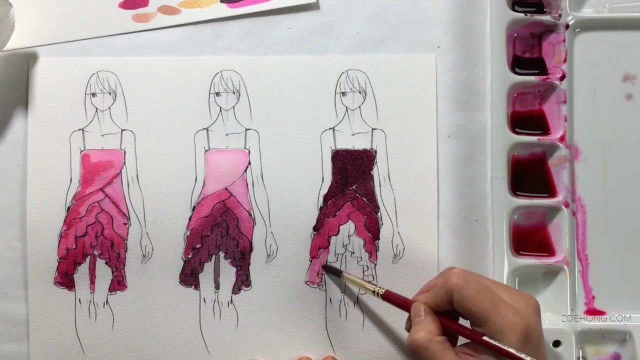 colors on the bottom, And when I'm done painting this one, pay attention to how it changes the proportions, or perceived proportions, of the dress, because dark colors tend to make things look smaller and light colors tend to make things look bigger, And so when you have these extreme 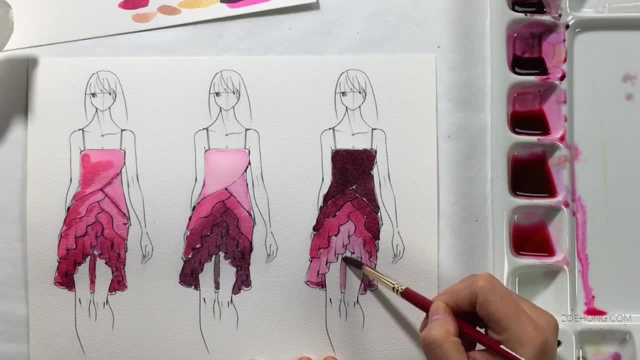 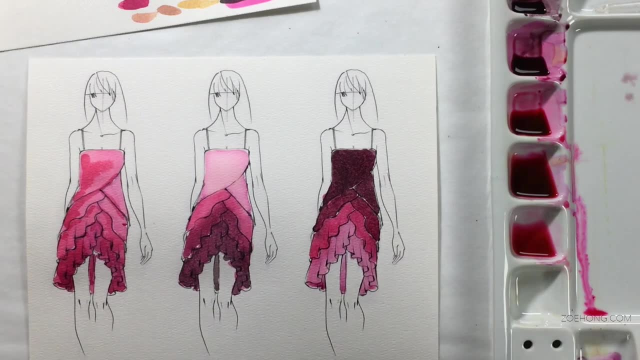 value changes, it is going to change what the proportions kind of look like. You know where the points of emphasis are. the overall effect. Okay, let me know in the comments what you like, what you think you know. is this a desired effect? 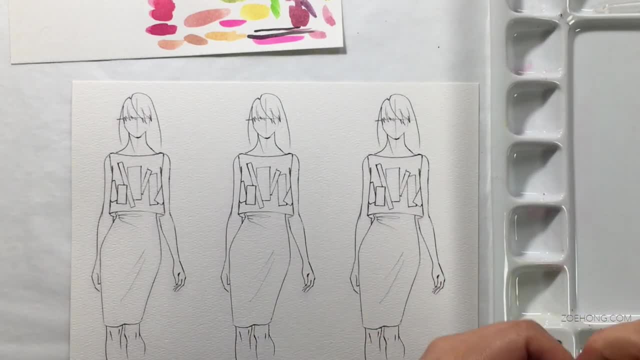 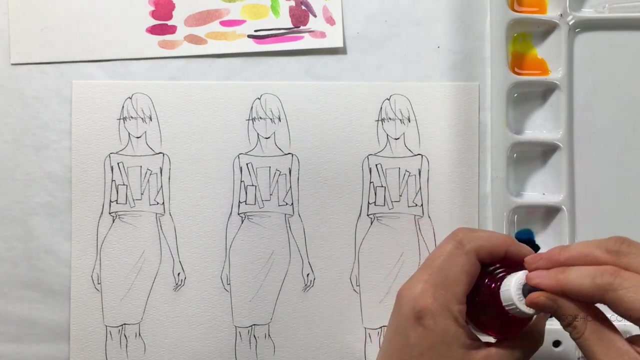 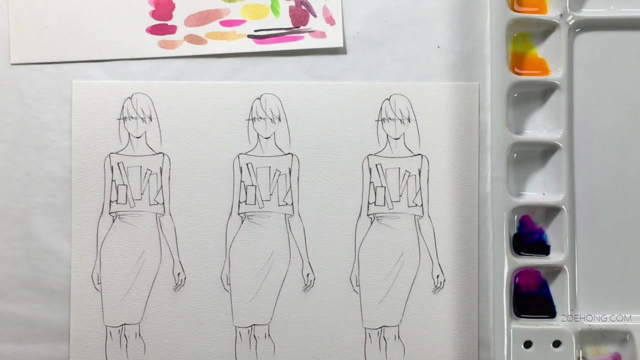 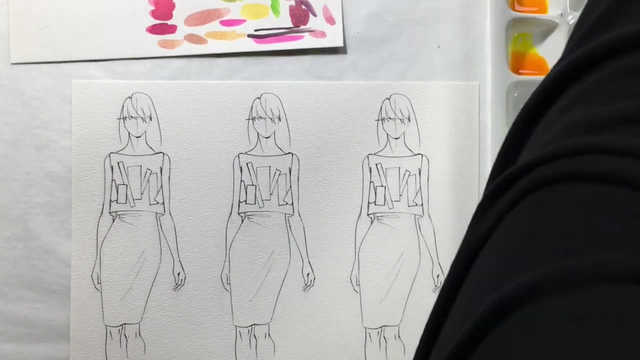 This set of three dresses. I want to talk about complementary color schemes more in depth, because I want to talk about how we use the complement to create more neutral tones and how certain neutrals go with other neutrals because of the undertone of the color. Okay, when we discuss complementary colors, some people just assume. 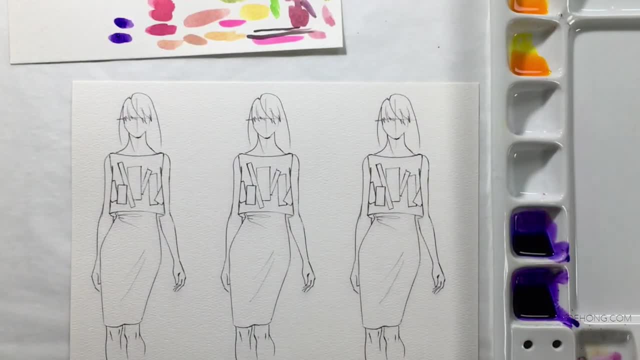 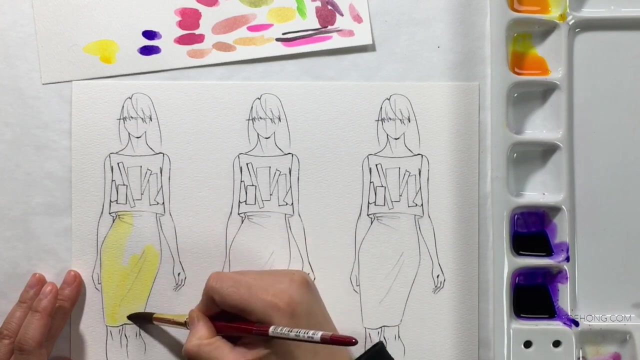 oh, yellow and purple, and we use the bright colors and you look at that and usually you know they don't look great. Okay, they're pure saturated form, Okay. And so you might be thinking, well, I'm not going to use. 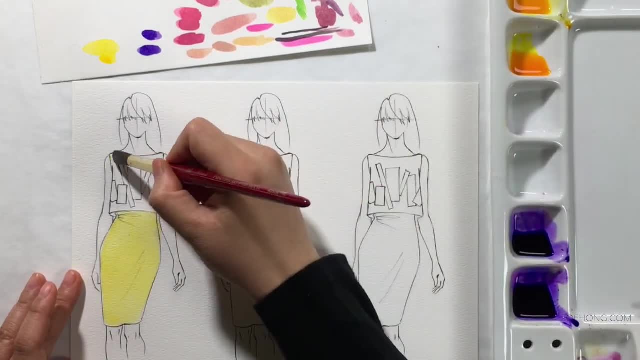 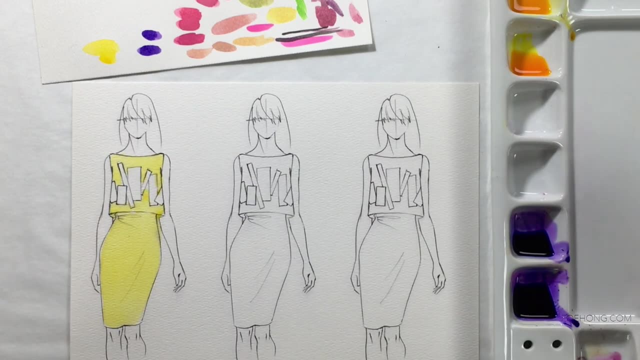 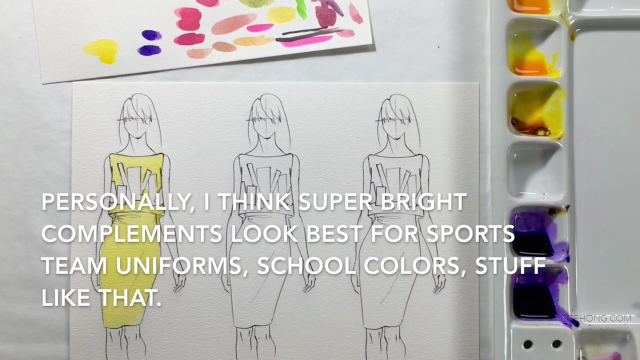 that Zoe, because it's too bright, It's too different And I don't really get how they harmonize. and yellow and purple- Does anybody really wear that? I get that response a lot And I get it. I don't particularly like yellow and purple in their purely saturated form. 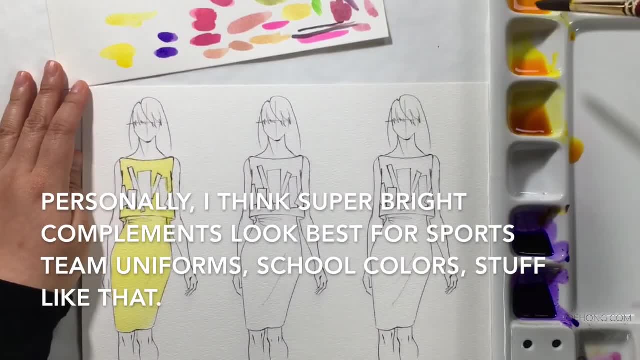 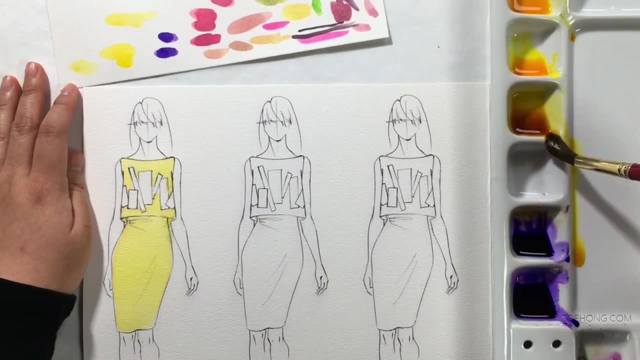 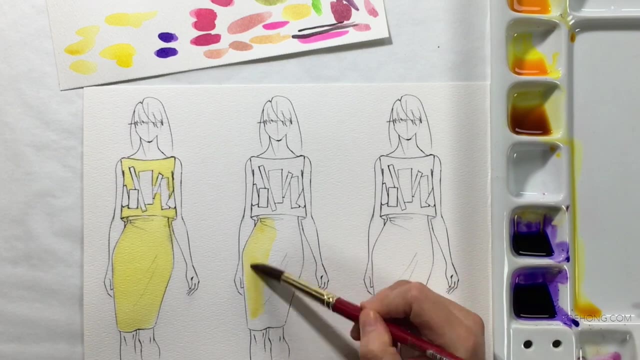 much either, Not together, anyway, Like I like, and wear a lot of yellow. actually, You're like Zoe: you wear something other than black. I do when I'm not teaching. In this second dress I have a yellow, but I have muted it with some of the violet, So you're. 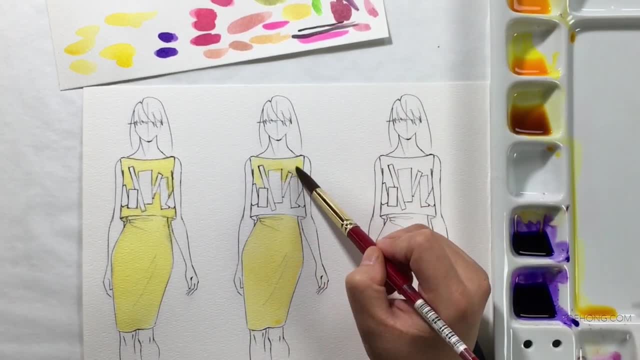 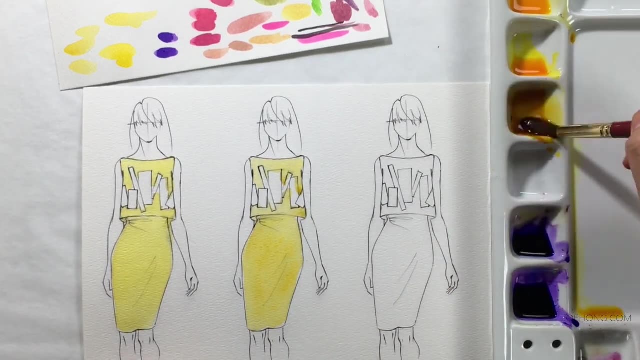 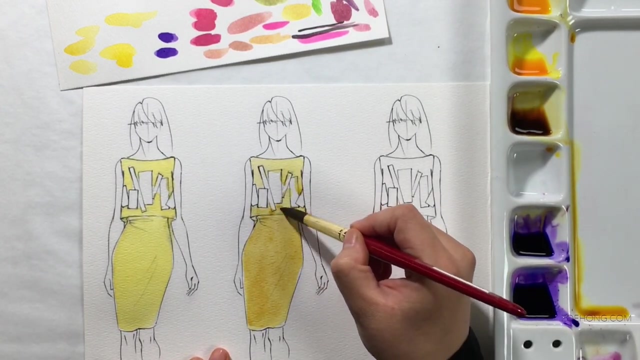 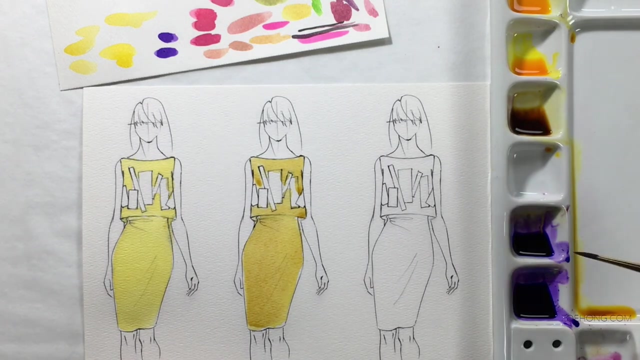 getting a softer yellow. It's definitely distinctly yellow, but it's creamier, It's more neutral, It's a little bit more sophisticated. It's going toward the light, warm, creamy, neutral territory. In leather speak we would call this kind of like a blondie, cashmere chamois. 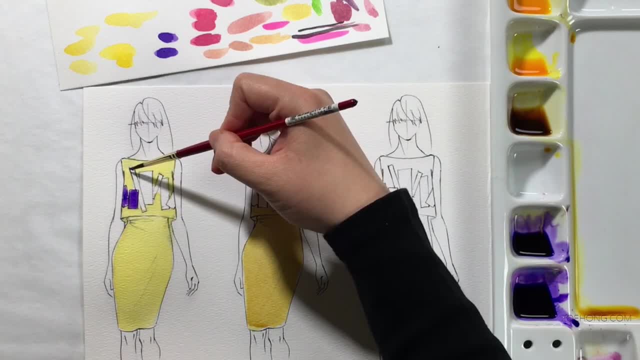 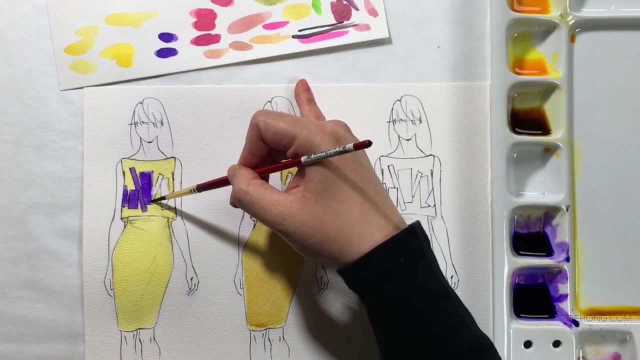 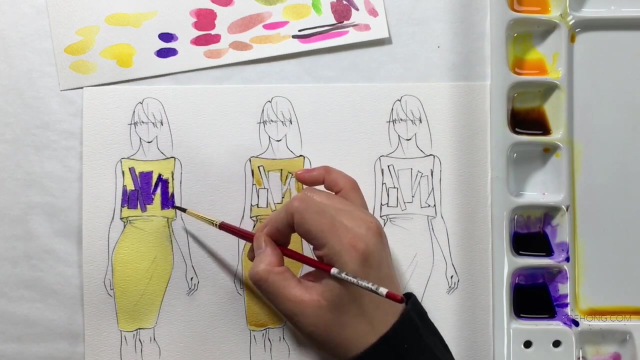 sort of color. So you see how those two yellows are very different. And now I'm applying that bright purple to the design of that first dress And you see those two colors and it's like it's very bright and compliments. Yeah, They really push the other color They make. 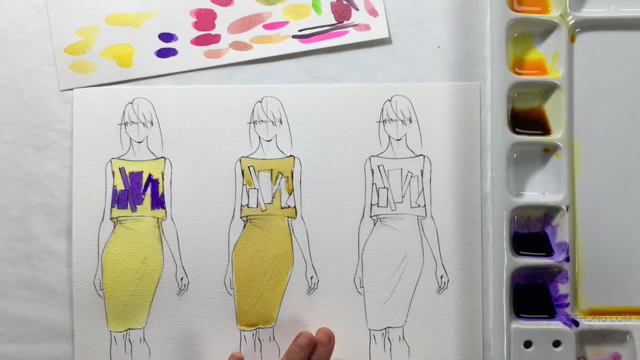 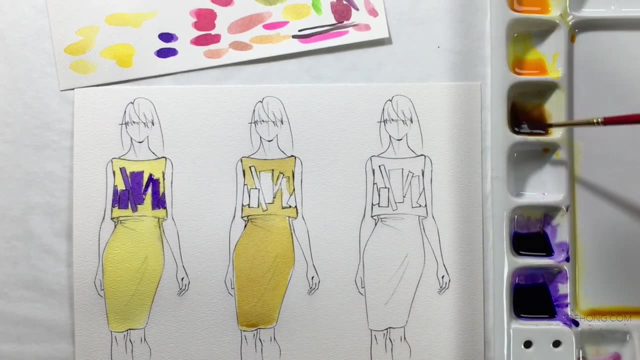 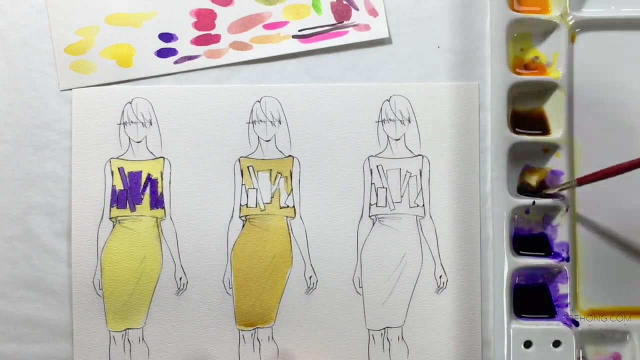 the other color pop, And I mean, this is why redheads look so great in green. Let's think about this for a second. Yes, So yeah. but then here I took the purple and I muted it down with quite a bit of yellow, and you see how the colors are more neutral. but because 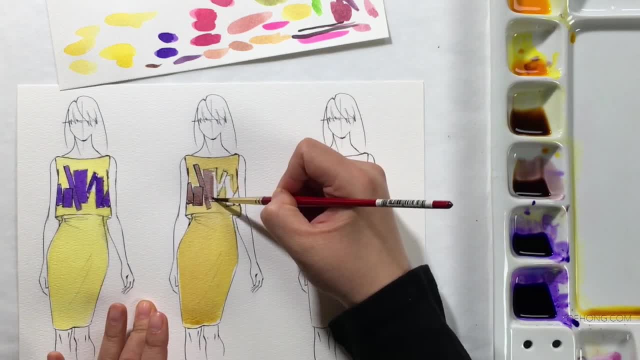 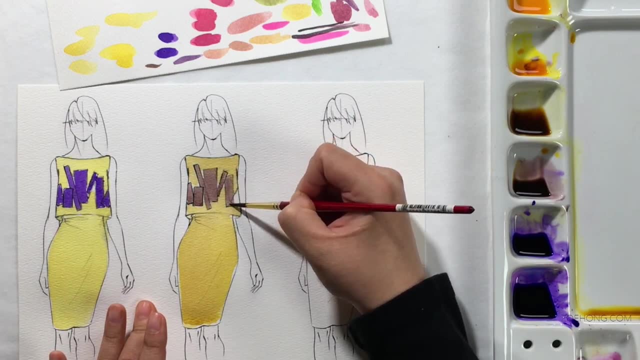 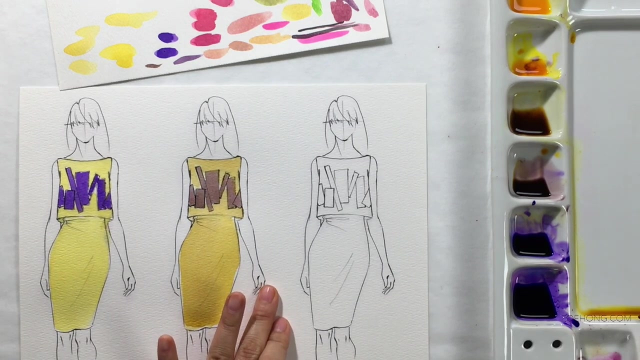 they're both Both comprised of the same two colors just in different quantities. you're still getting a harmonized. look like the colors go together because they're essentially the same color. It's a mixture of purple and yellow in different ratios. They're both the same, And then in 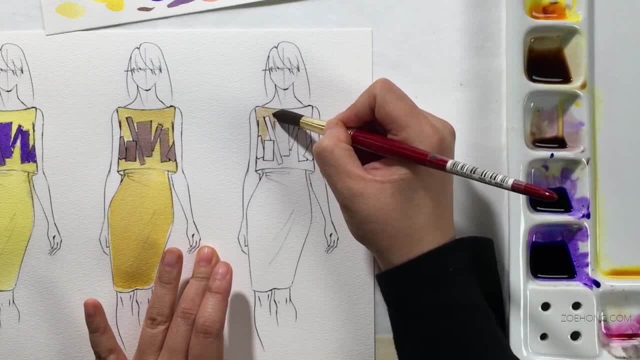 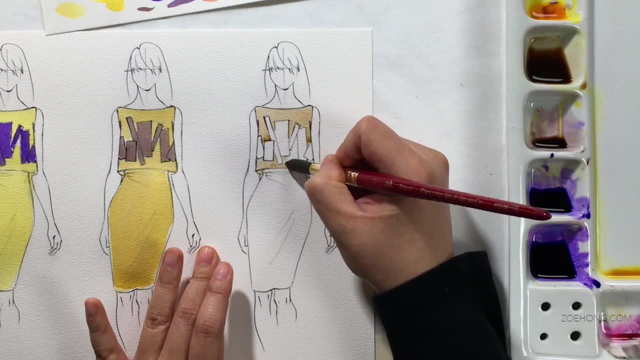 this third dress. I'm playing and pushing the compliments more. Yeah, And these are all compliments. These are all. three of these are compliments. These are complimentary color schemes. Complimentary color schemes are not always just like bright red and bright green, bright. 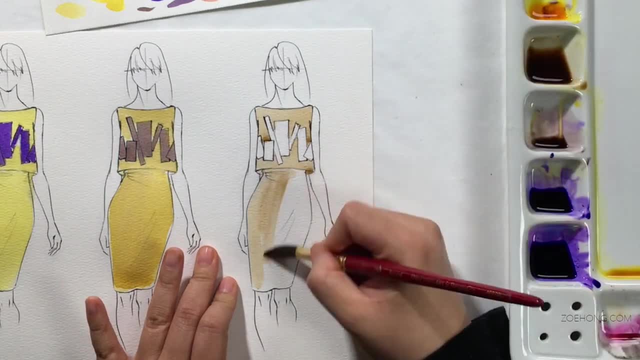 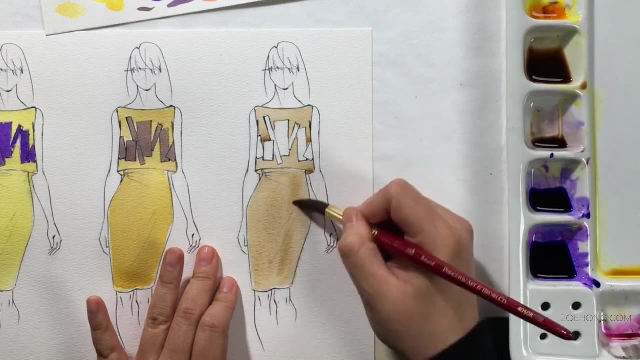 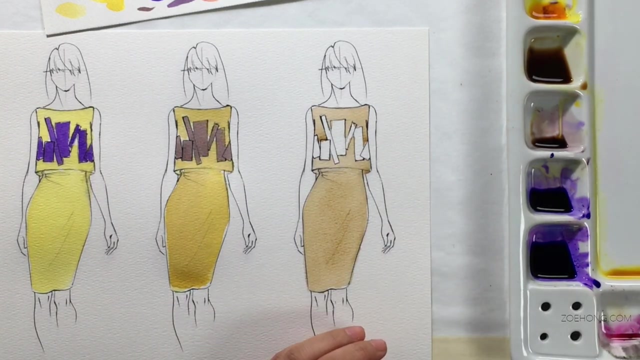 orange and bright blue. I hope you all watched my video on muting and neutrals and how to mix neutrals with pink colors And that's in the color lessons playlist. And this is the best way to figure out neutrals is to use compliments of the colors that already. 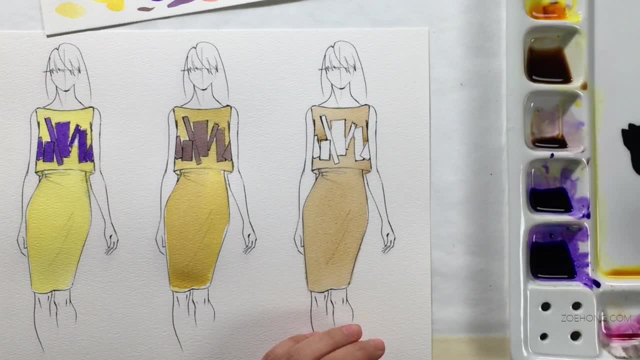 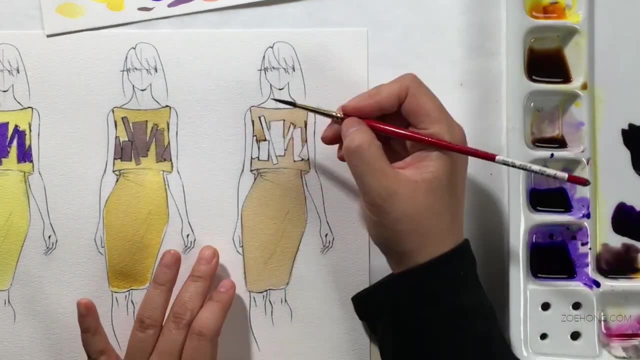 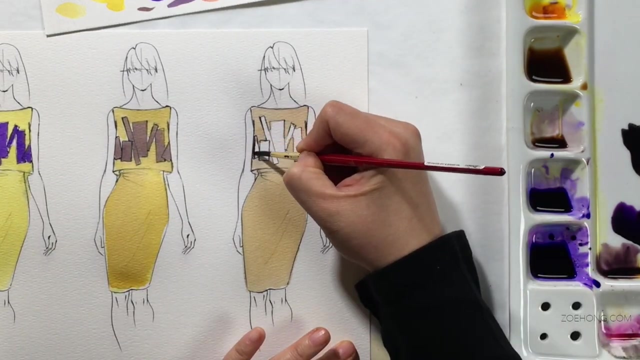 exist in your color palette and you know you can do a thing where, when you're picking out fabrics, you can. you know, maybe you decide you want yellow and purple in your collection and you want a neutral that goes with both. maybe you mix up a few paint swatches of yellow and purple. 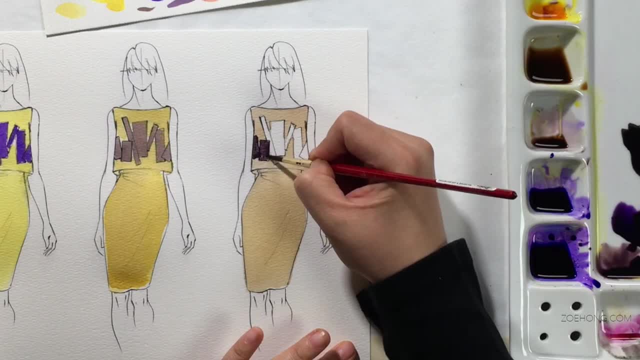 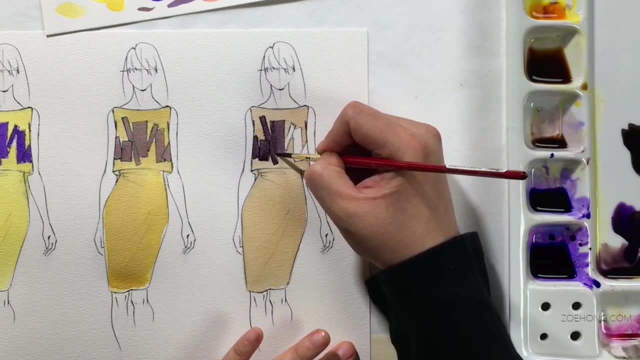 the yellow you want and the purple you want, and then you'll get some different uh gradations of the neutrals that you want and then you can take those to your fabric sales rep and be like: these are the neutrals i'm looking for, because i think these are going to. 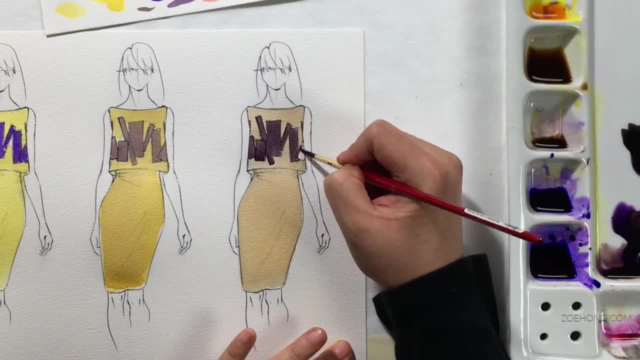 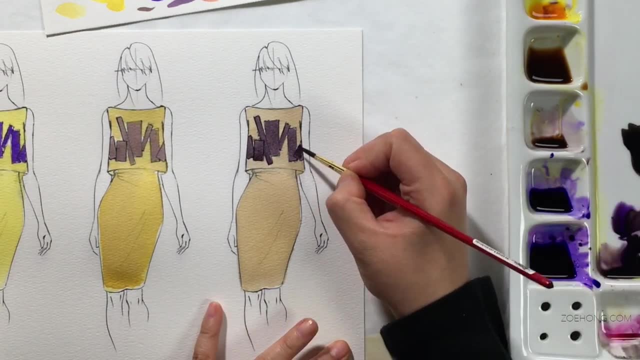 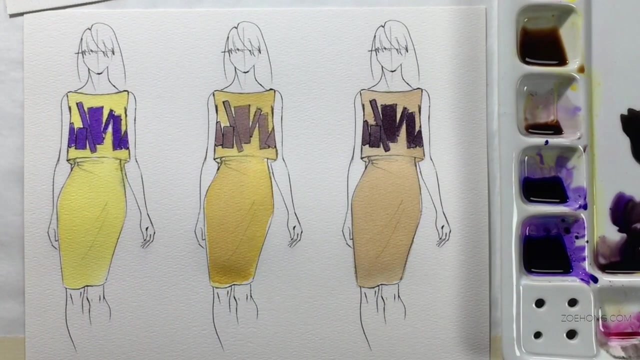 harmonize well with the pop colors that i've already selected. okay, so these are just a few lessons on practical applications of color theory and fashion design. please hit the like button, the thumbs up button, if you want me to continue this series. if you found this video helpful for your design purposes, share, subscribe. 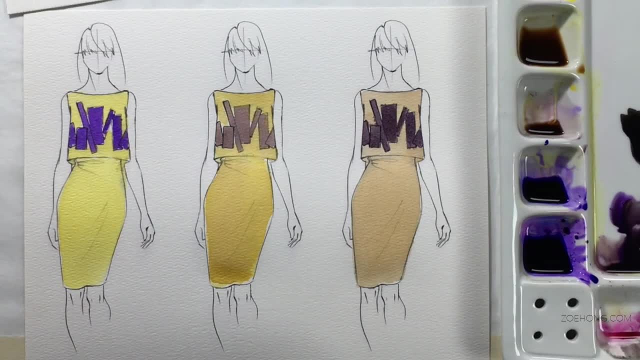 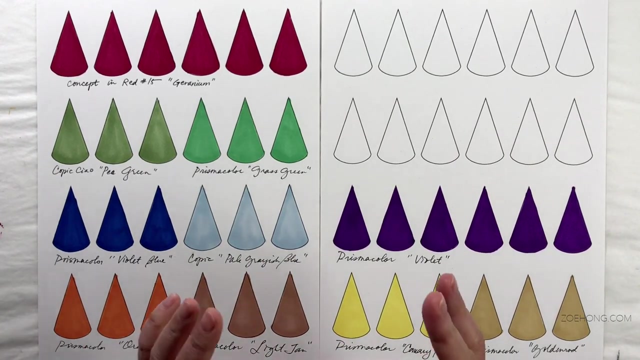 you comment, let me know which ones were your favorite iterations of these dresses. ask me all your color theory questions and i will see you in the next video. hey, hey, party people. in this video i want to talk about color theory as it applies to working with markers. my previous 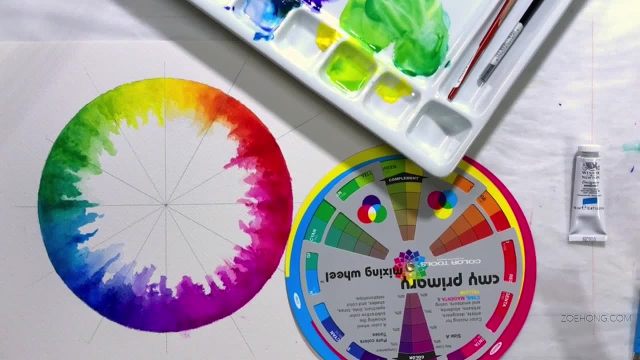 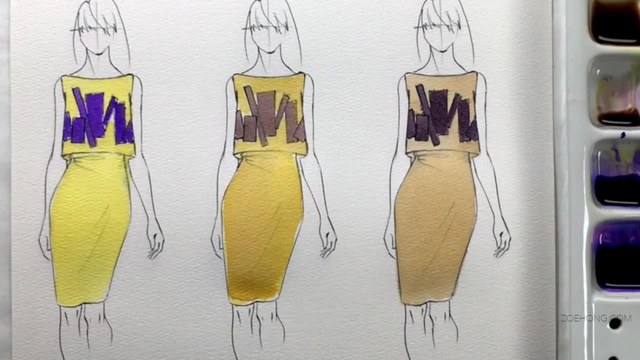 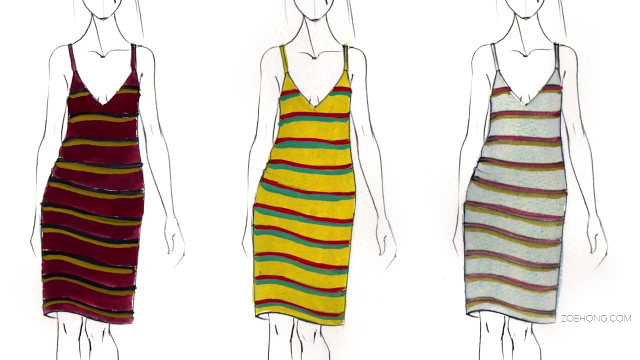 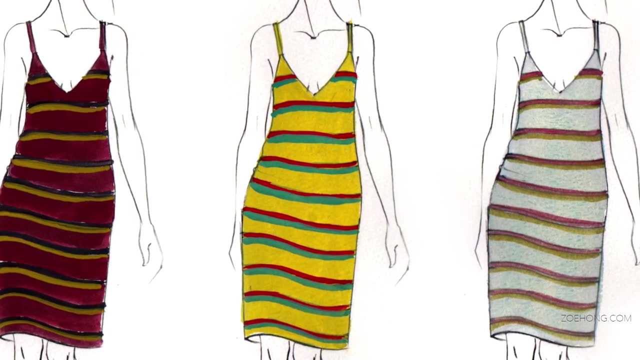 color theory videos. they were deep dives into terminology and color mixing and working with paint, but i know that many of us work with marker a huge chunk of the time, if not a majority of the time, and i wanted to take those same concepts and show how they can or cannot be applied to working. 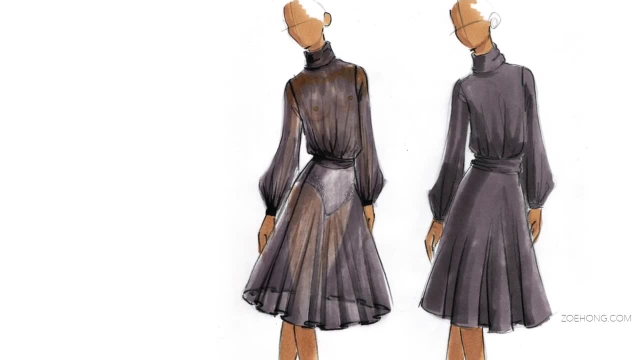 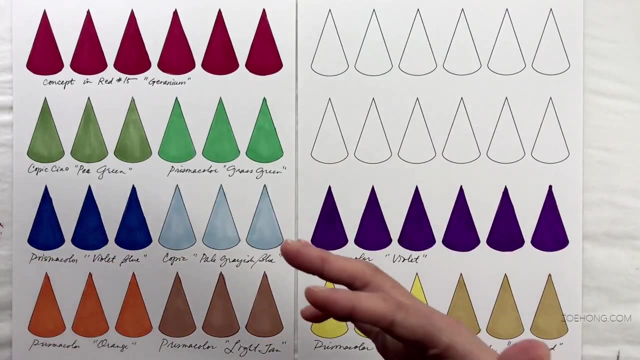 with markers. first up, when you are working with markers, you can layer them to create new shades. you don't want to layer a lot. it's not like paint and watercolor or oils, where you can layer a whole lot. there's only so much layering you can. 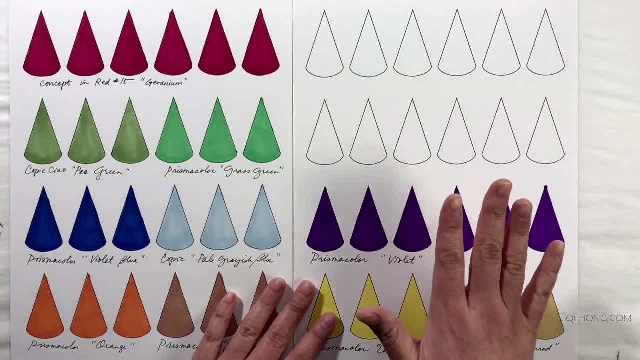 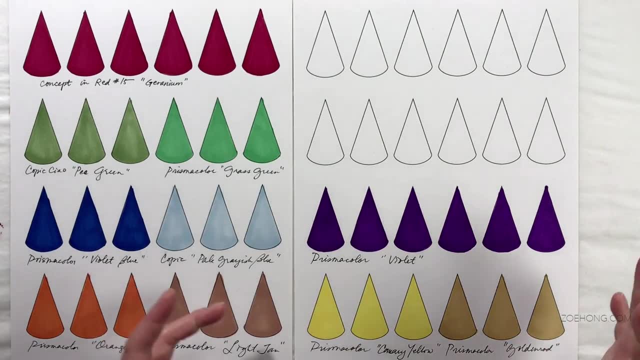 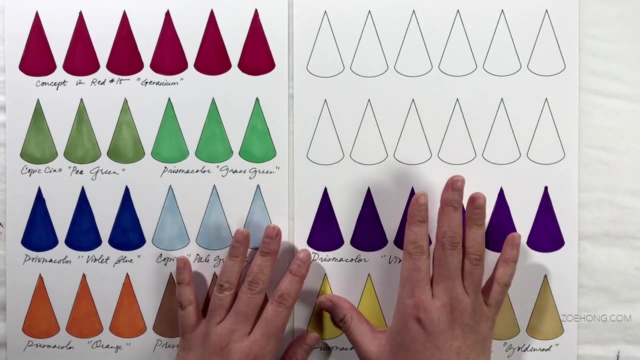 do with marker, but you can layer a little bit. make sure that the paper you are using can take that much ink, though. all right, there's a lot of different kinds of papers you can use free ink. today i'm demoing on simple cardstock. it's pretty inexpensive, just whatever stuff at the office. 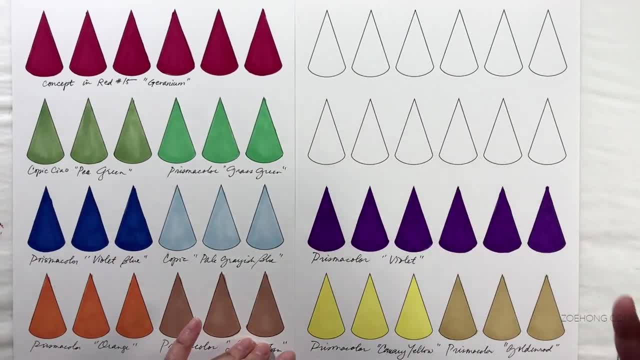 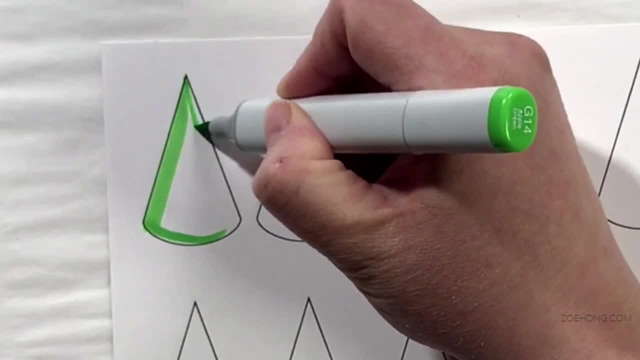 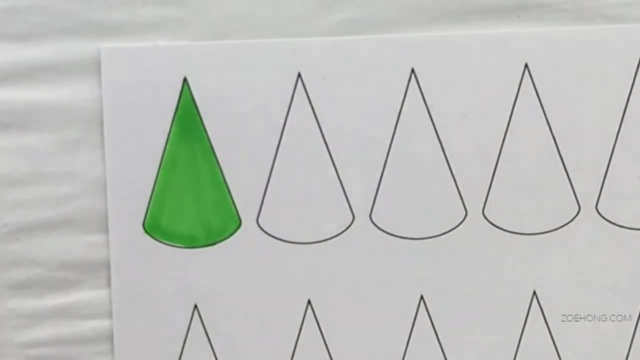 supply store. okay, they take marker pretty well. i like to use marker paper. i don't really love bristol for marker work. okay, this is not going to be the most beautiful marker rendering video you've ever seen in your life. that's really not the point of this video today, so just roll with my messy cones here. 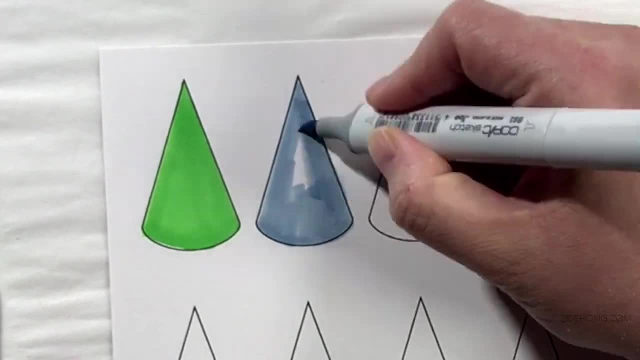 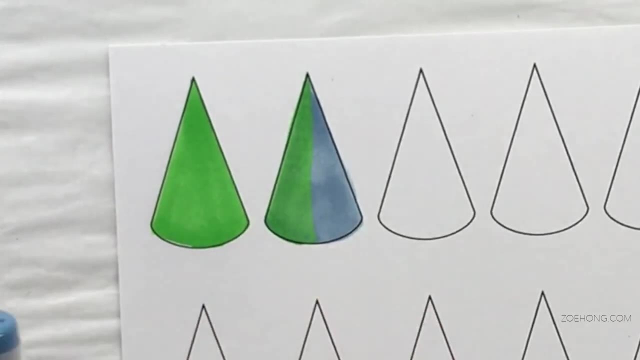 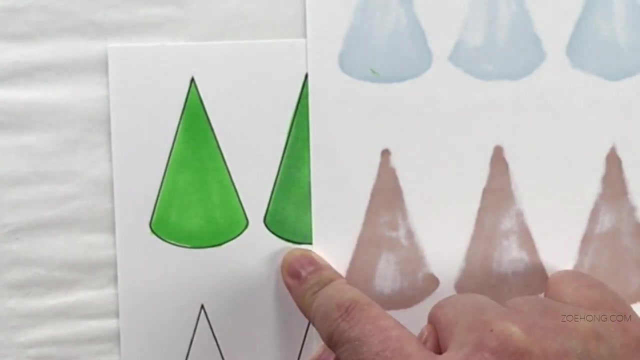 it's a funny sentence i never thought i'd say: just roll with my messy cones here. can you tell the difference between the green by itself and the green layered on top? it's a little bit darker and cooler. okay, so if you wanted to just make a real subtle change to the color without having to run out and get a new marker, 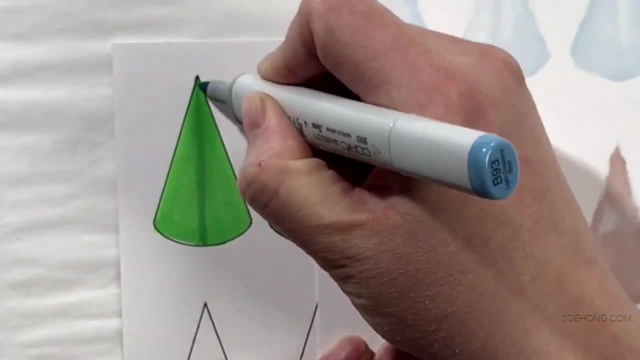 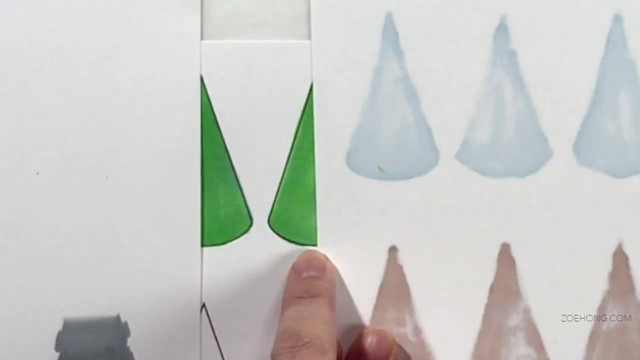 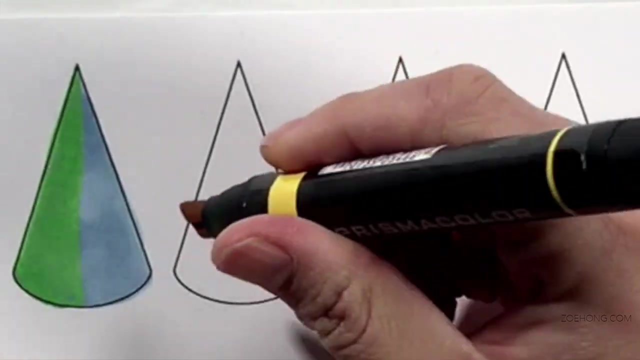 you can layer. now, the order in which you layer your markers also makes a difference. do you see how this one is slightly darker than this one? it's because of the way it's layered. i'm going to show you a more drastic example. okay, so this is prismacolor yellow ochre and this is 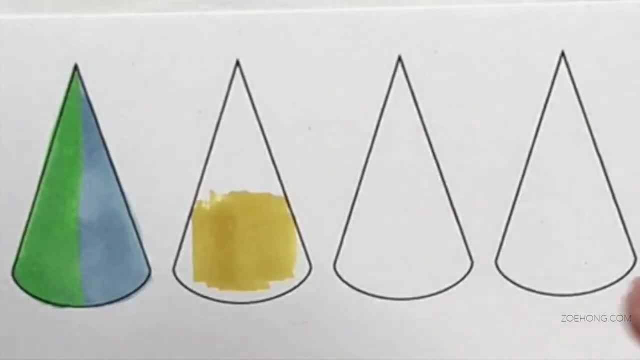 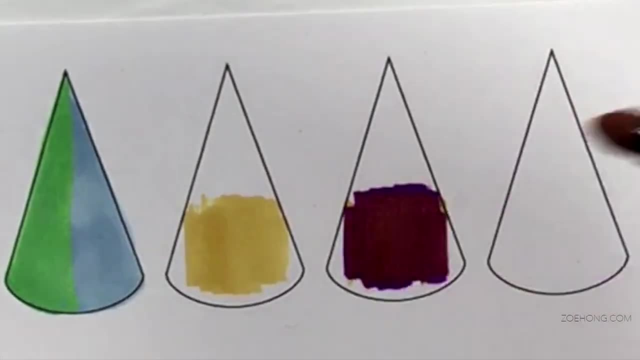 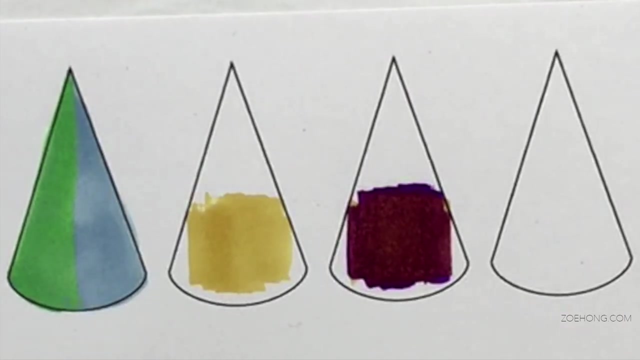 prismacolor dark purple. i lied, i don't want this one. i want this one: prismacolor violet. now, if you put the yellow ochre on top of the purple, it looks like this and, as you know, if you watch my previous color theory videos, and you know that when you mix two opposites on the color wheel, 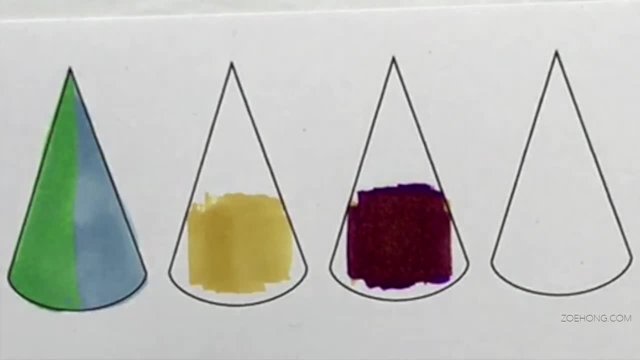 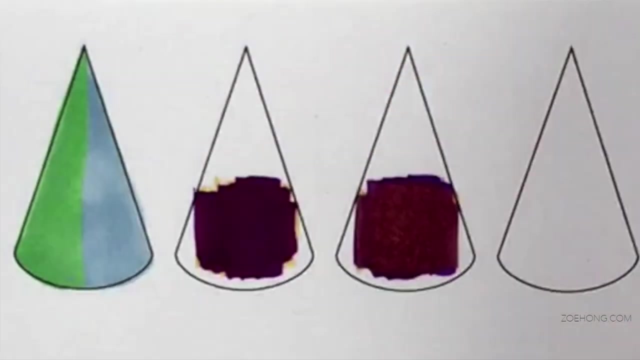 together. you're mixing complementary colors together, which creates a lot of color, and you're a mute, a much more neutral color. Okay, I've muted that purple down so that it's looking more brownish. Okay, Putting that violet on top of the yellow ochre. Here's the purple by itself. 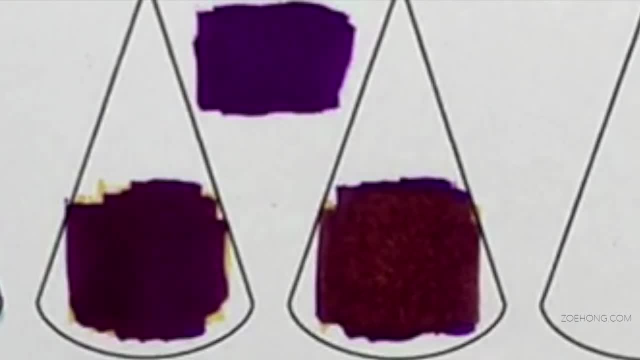 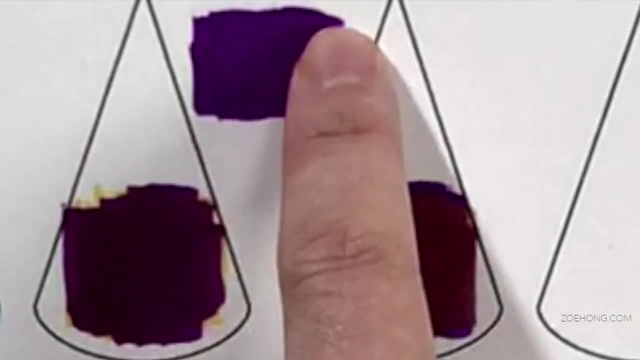 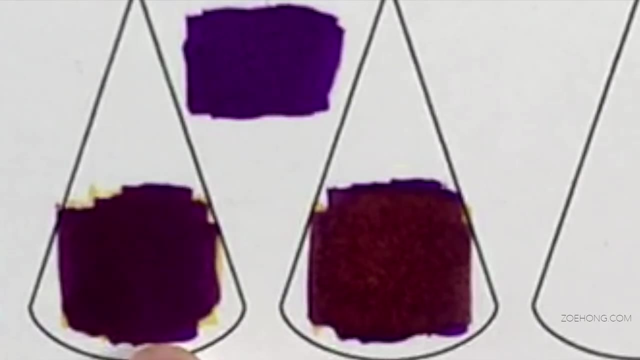 The yellow, because it's such a light color. it affects the purple less. It still mutes it a little bit. It does warm up the purple, You see that. So this is the violet by itself, This is violet on top of yellow ochre, and this is yellow ochre on top of violet. Okay, And you see. 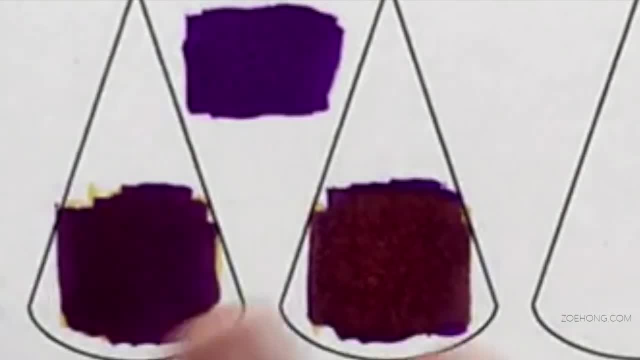 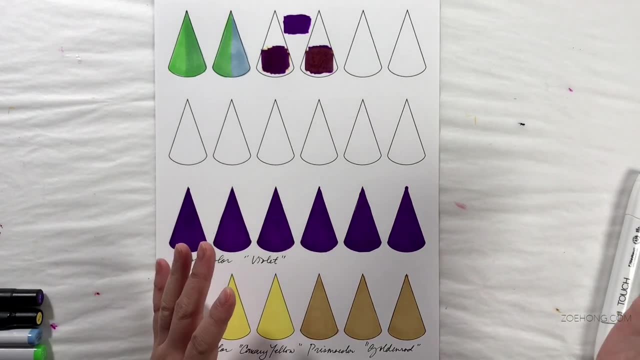 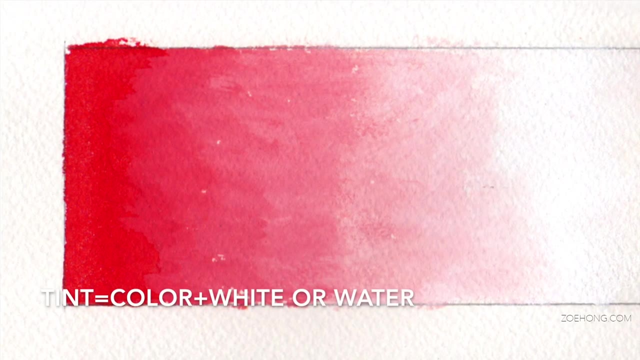 this muting effect going on by layering them in a specific order. So another big thing that we discussed in the color theory videos was the four ways to desaturate a color: Tinting, shading, toning and muting. Now, tinting with paint was color plus white or color plus water to make it. 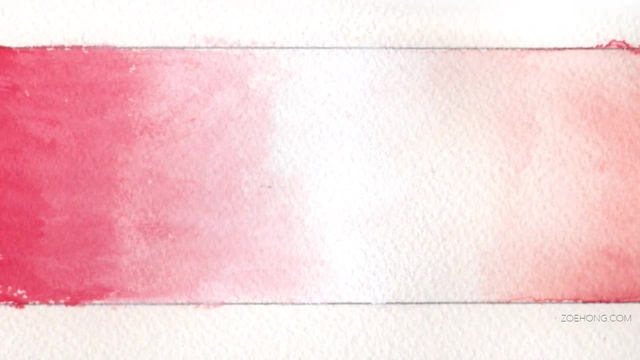 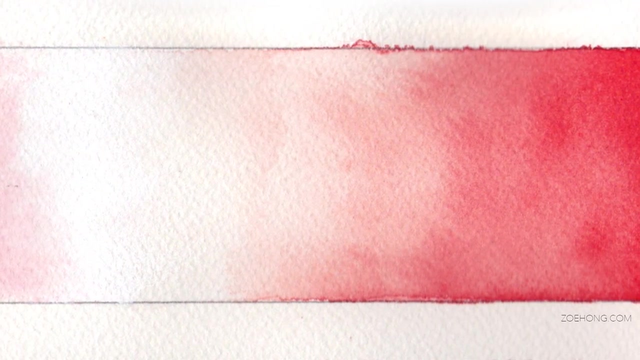 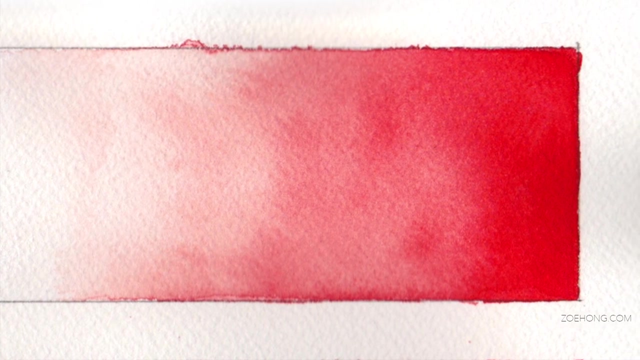 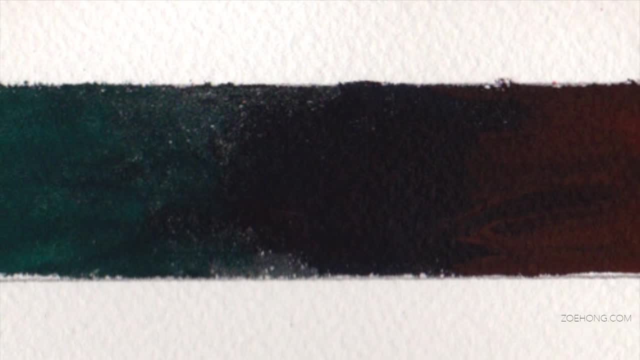 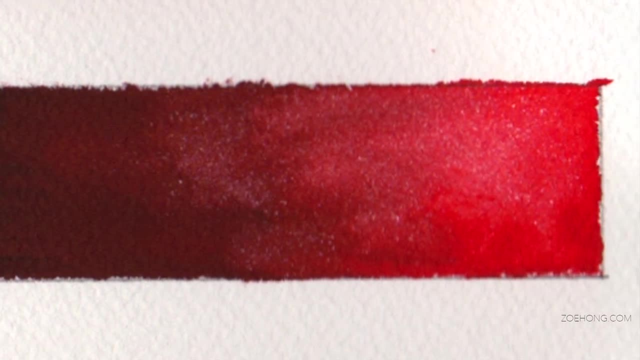 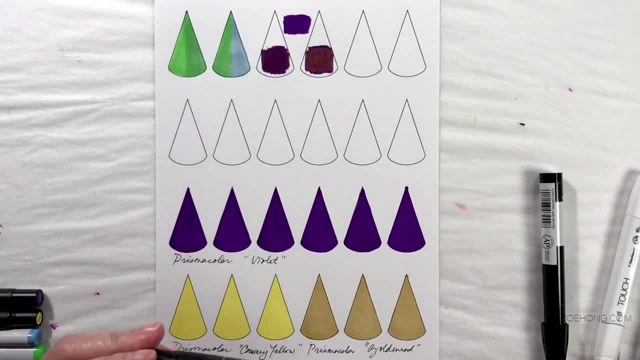 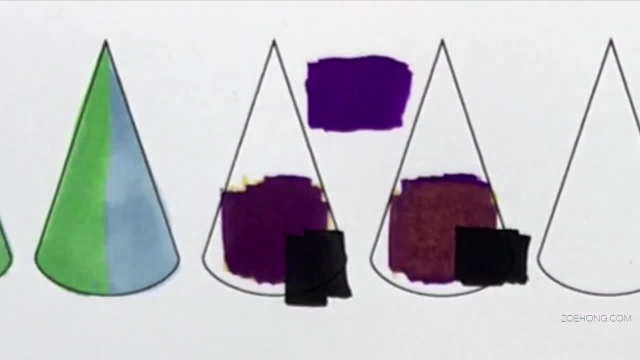 jet black and black. This is black and this is one of the weakest black markers that I've ever used. It's the weakest black and it still will cover it. So no matter how light of a touch you use with black, it's gonna be black. So you can't really mix black with. 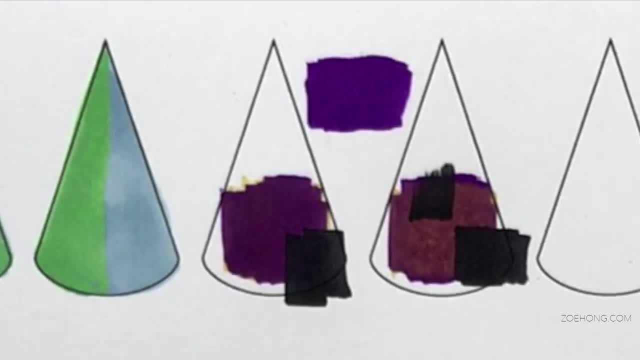 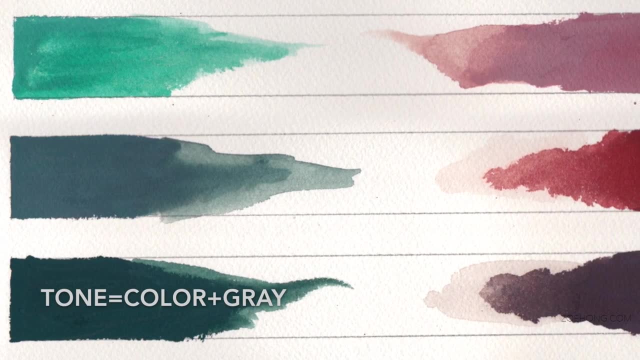 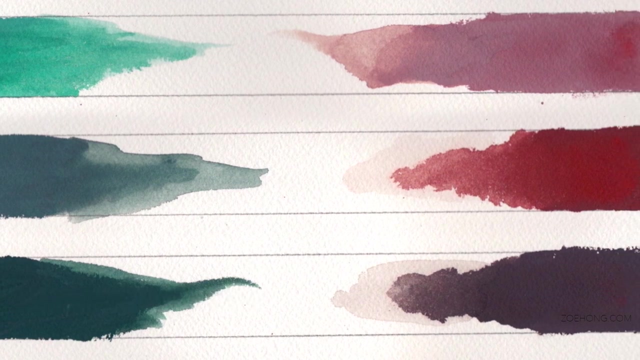 markers, You are gonna have to get a darker marker color With tones. tones is color plus gray, And in this area you actually do have some wiggle room. So when you're layering grays with marker colors, you have to consider a few different things. Number one: 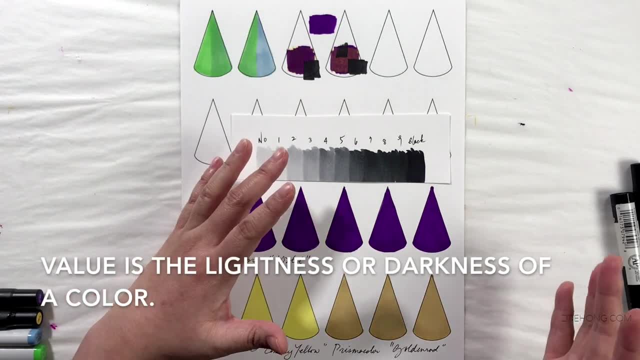 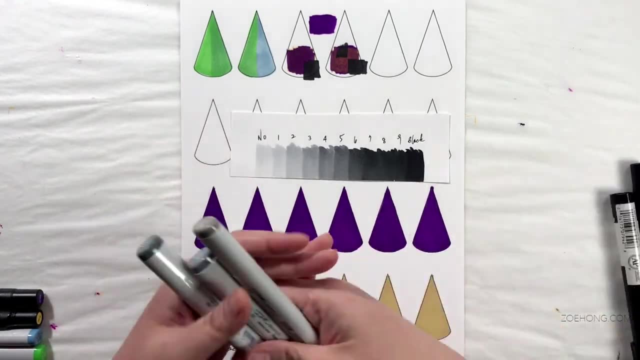 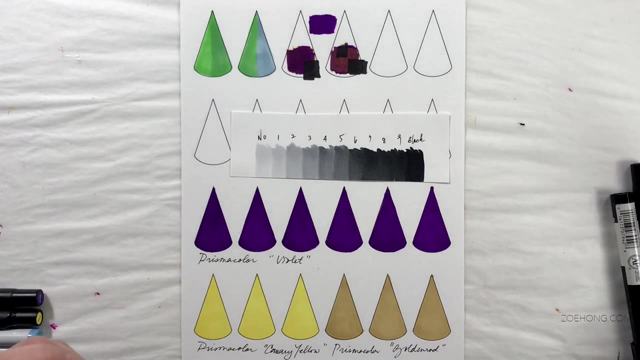 the value. Value in color theory means the lightness or darkness of a color. And so when you look at these gray markers, from any brand, you know Copic, they name theirs. you know one, two, three, four, five Prismacolors: they call them 10%, 30%, 70%, But you know. 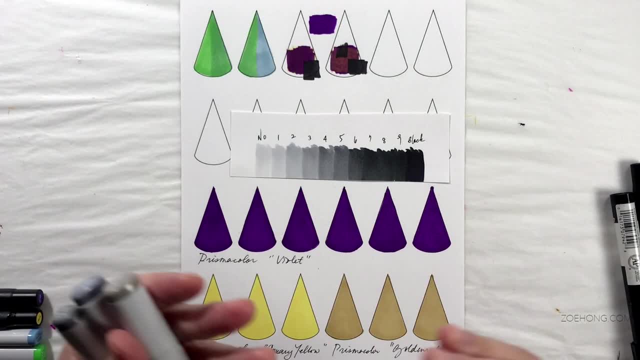 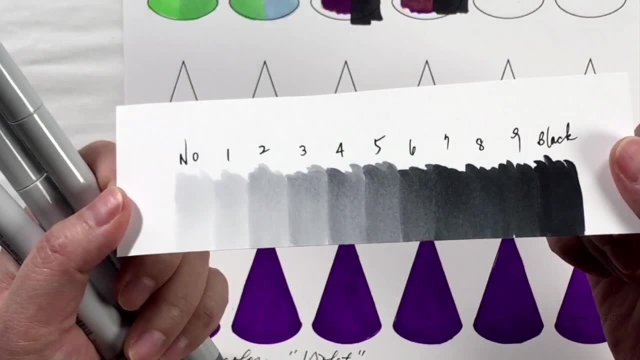 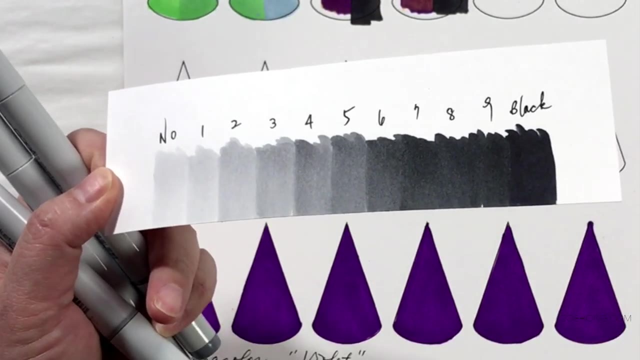 all these brands. they have that scale, okay the value scale, for their grays. I did this grayscale using the Copic neutral gray series And so they have from zero to nine, and then this is the Copic black. I know they have a neutral gray 10, but mine dried out and 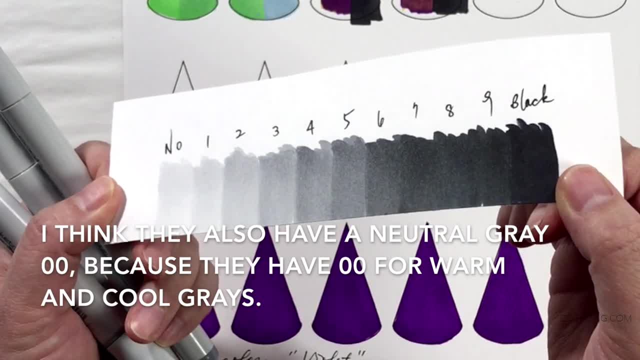 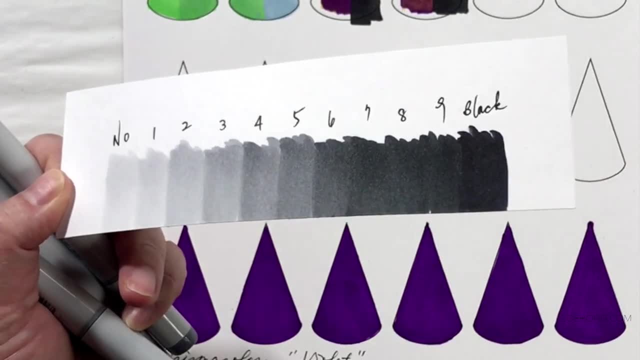 I need to get a new one. But now that I've made this grayscale I'm kind of wondering if I really do need one, Because the Copic black isn't that strong. Copic has a special black, their 110.. Their black is color number 100.. Their special black is 110.. 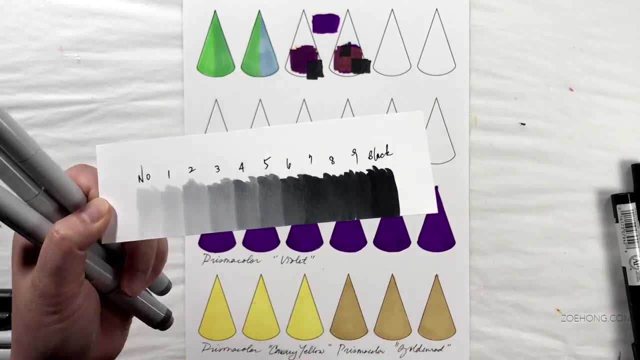 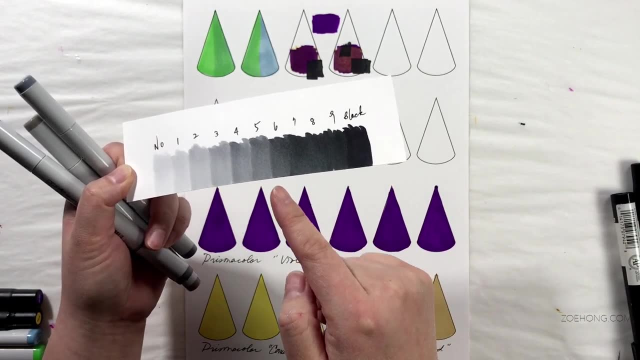 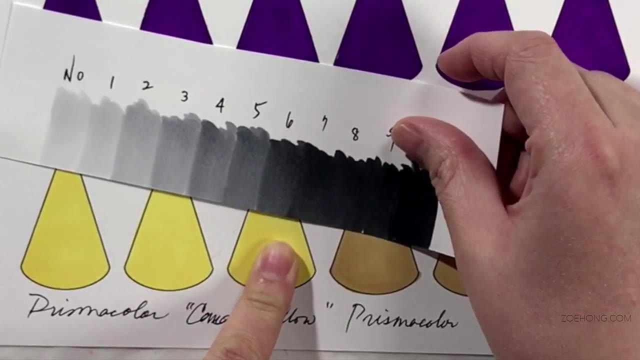 And that one is a more intense black. So when you're layering, consider your value that you're adding. okay, If you use a dark six or seven on top of this light yellow, what is going to happen compared to if you did an actual value match which is closer to two? You may be at this point. 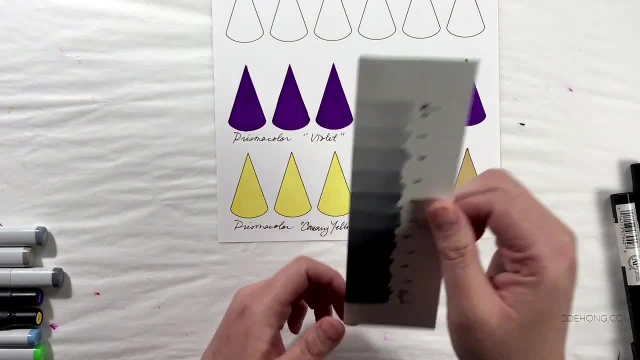 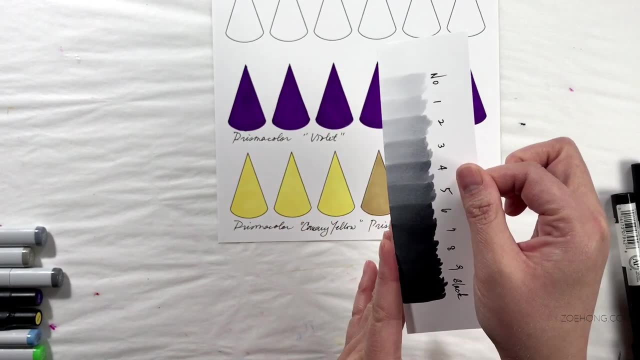 thinking: uh, how do you tell it's a value match? Okay, What you want to do is make yourself a value match. So if you're layering a dark six or seven on top of this light yellow value scale, like this, and bring your marker all the way to the edge, So you can do it edge to edge. 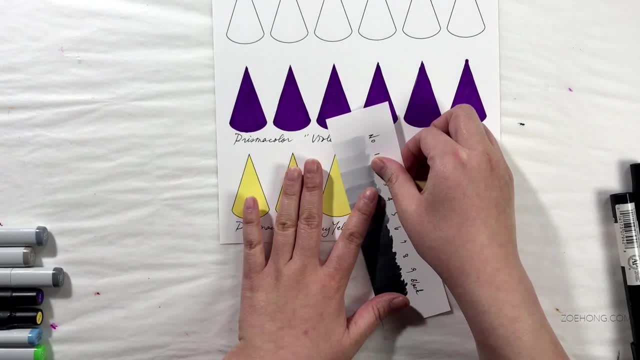 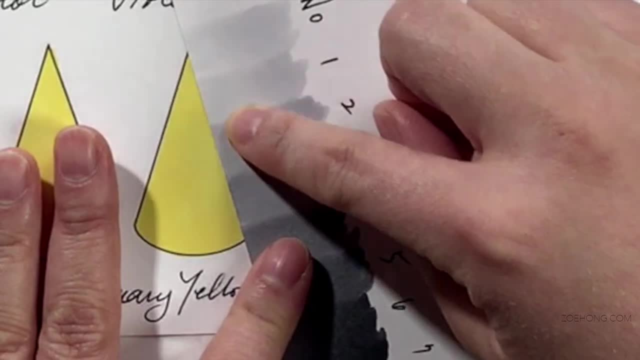 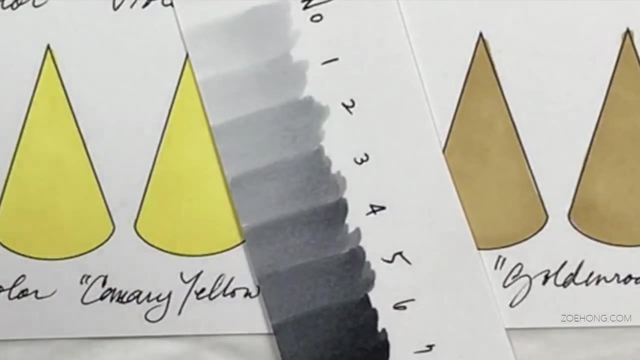 and put your value scale right on top of the color, squint your eyes So everything becomes real blurry And there's going to be a point on this scale where you don't really see a line of difference because the value is similar enough If they start blurring together. 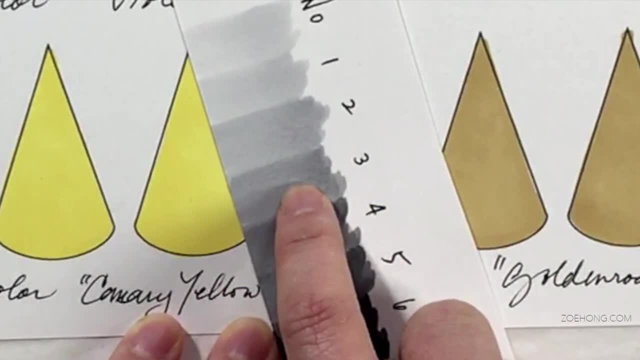 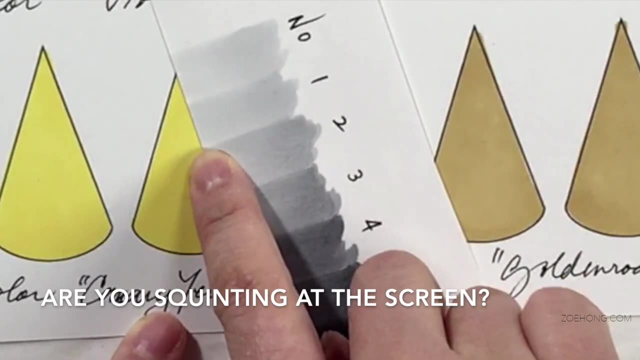 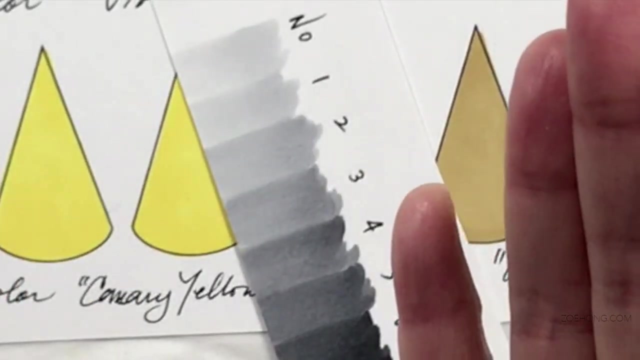 these two are never going to blur. Because this is too dark, Okay. The difference is always going to be distinct by here. Okay, Do you see how it starts blurring? Because it's a similar color, because it's a similar value. Okay, And so? 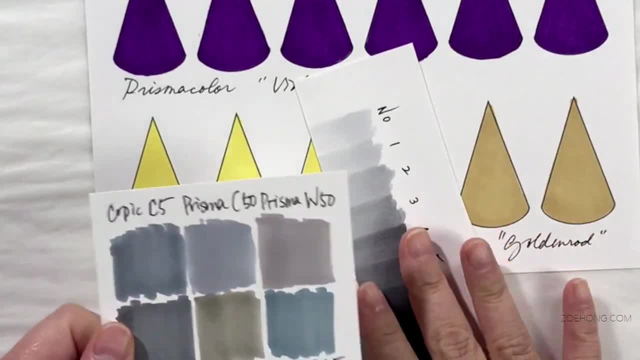 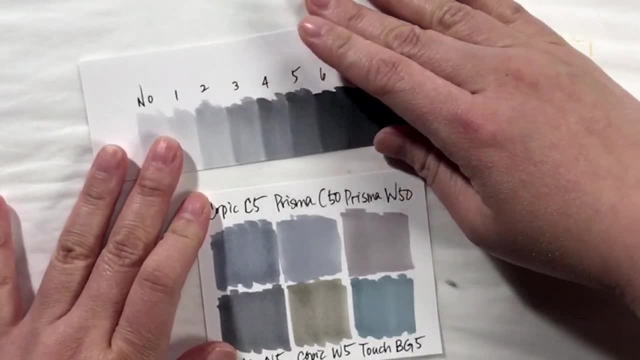 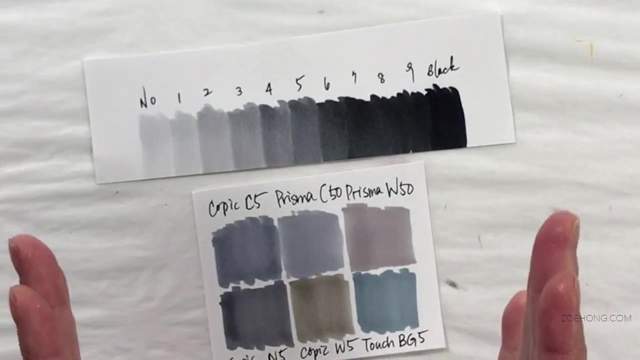 your value match is in here. The next thing you want to think about is the color of the gray. There's a lot of gray scales out there. Some brands have several gray scales. This, I swatched the middle gray, either the five or the 50%. 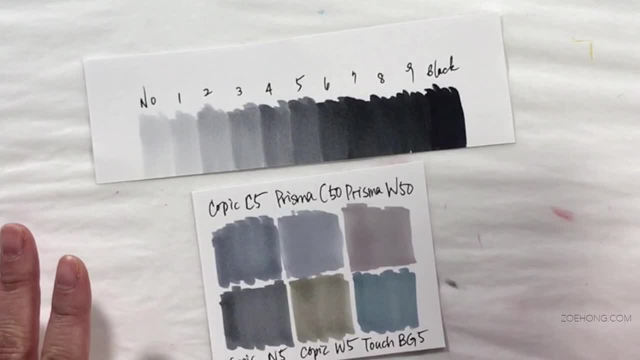 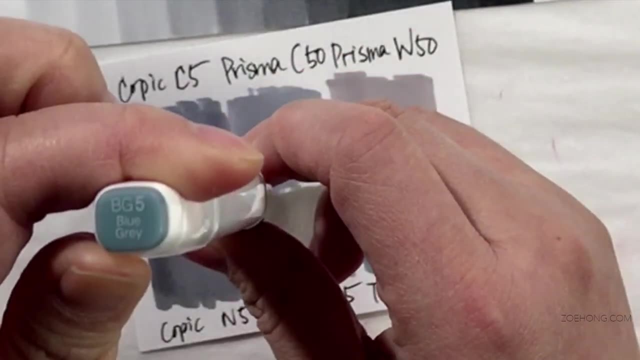 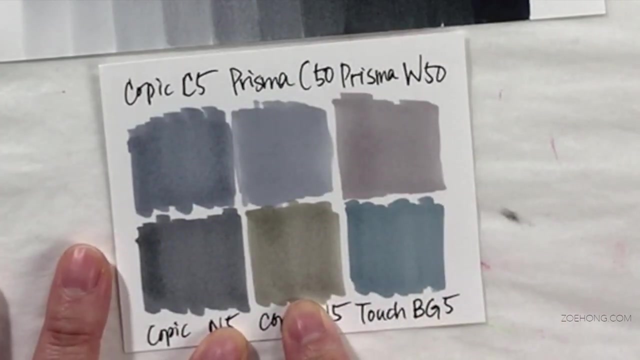 in six different gray stories. Okay, This is currently my favorite series right now. This is a touch blue gray BG. This is BG5, this one. Look at the shade differences. This warm gray is really green. Some people will call it a French gray, And it's this. 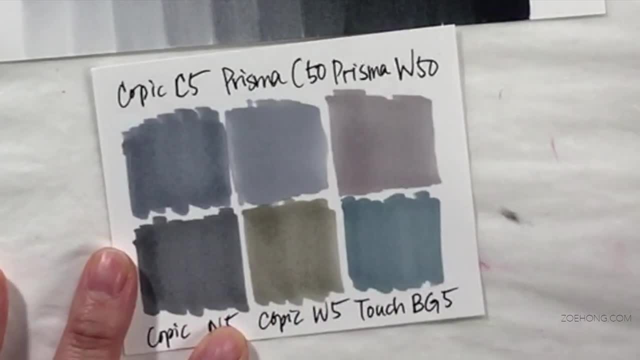 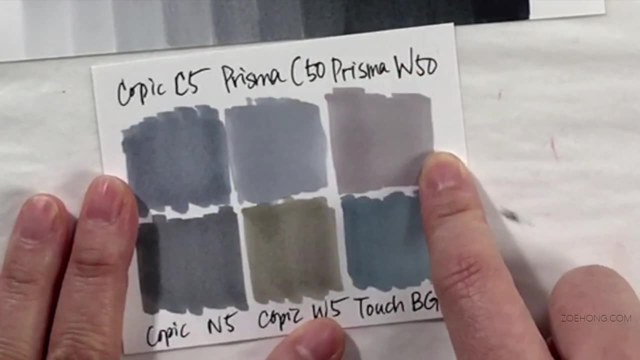 this gray family that I would more often pair with yellows and greens, because they share an undertone: This warm, this Prismacolor warm series. it has a purplish undertone, So this would pair great with purples: red violets, pinks, reds, even oranges. Yeah, I would put that because 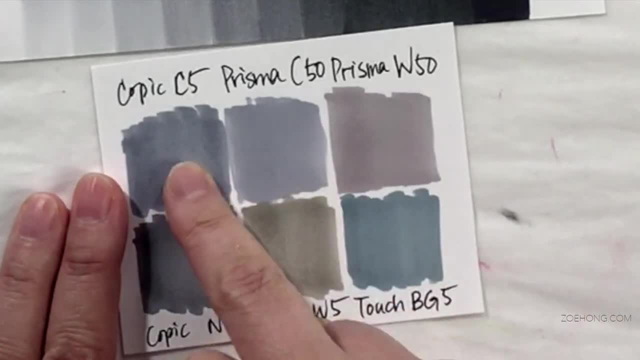 I think this is too green to go with orange. And then these are very cool. Okay, Now do you see the value difference between these two? brand to brands, The values are going to be a little bit different, So you need to make your own value scales for the grays that you use. 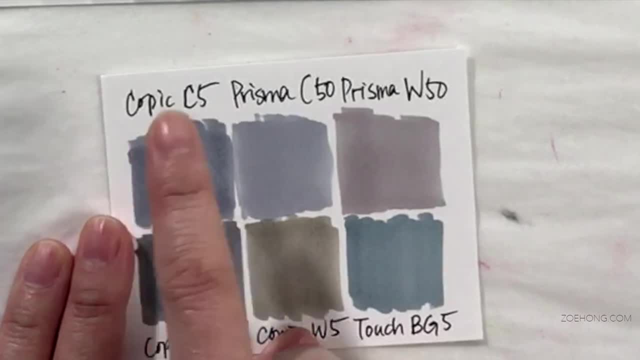 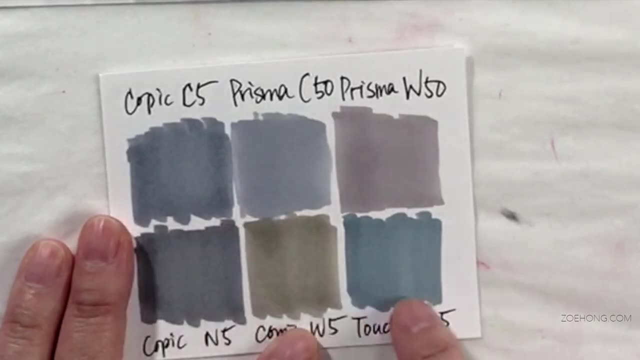 So this is a Copic C5, cool gray five. This is a Prisma cool gray 50%, And these definitely run cool, Obviously not as blue as the touch. And then this is the Copic neutral grays, And it is the most. 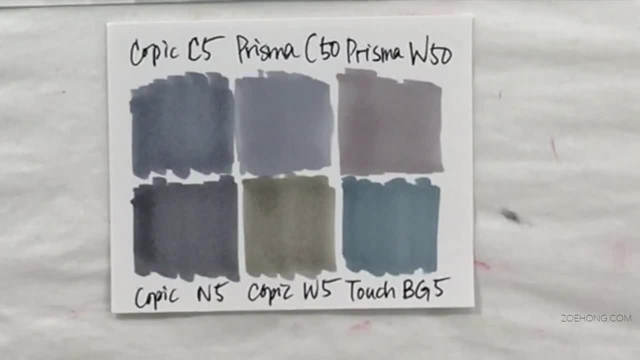 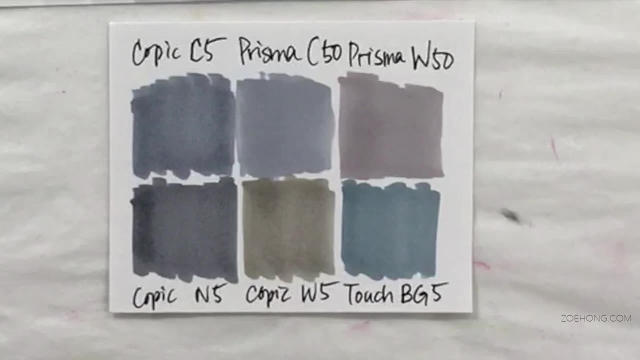 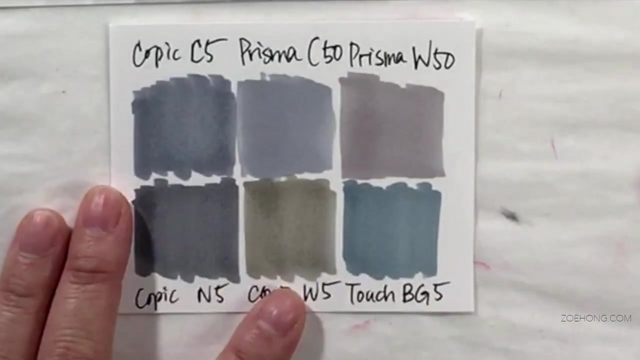 neutral. out of the grays that I currently own, The one that has the least, you know, distinguishing undertone, And these are great for all kinds of blues. Also, some of the cooler purples, blue greens- Okay, That's what these are for. So when you are thinking to put a gray, 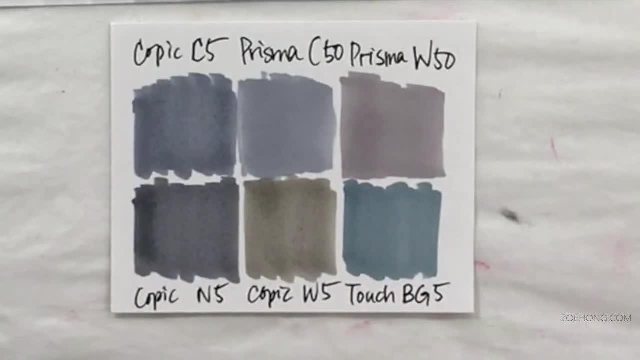 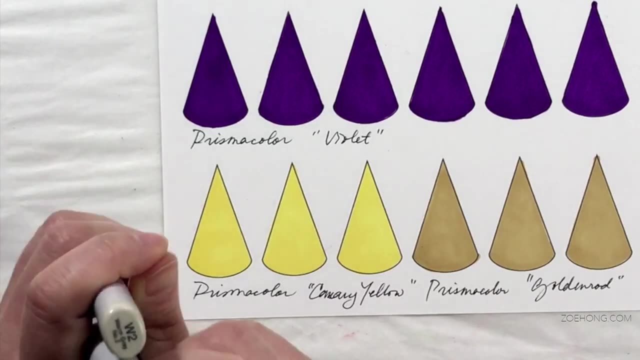 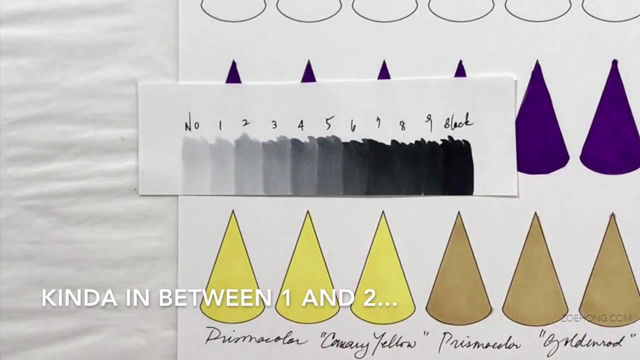 on top of a color. think about the value you want and think about the undertone you want. If I want to create a tone of a yellow, I have a warm zero, one, two here. Okay, Remember, the two was pretty close, So I'm going to start. 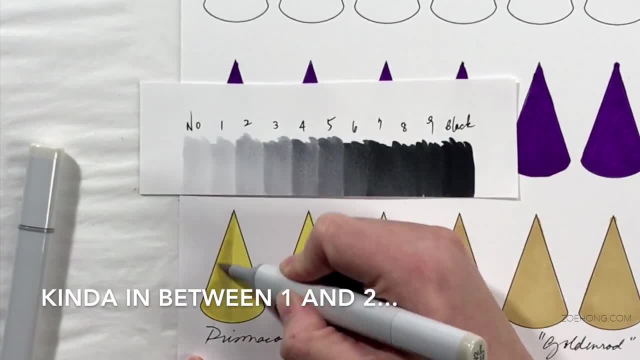 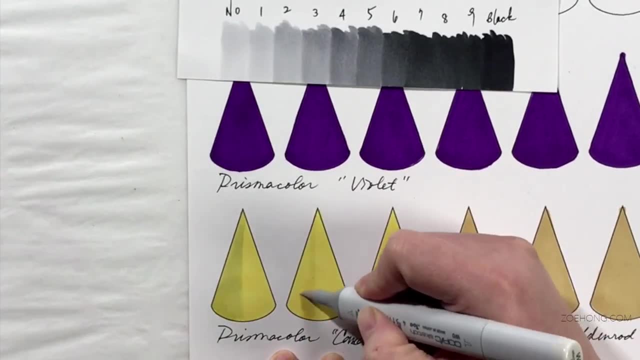 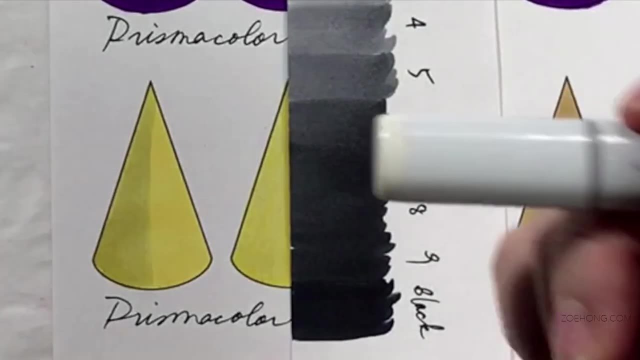 there. So yeah, layering them together will produce a darker color, but it's still light enough that you really see the yellow. still, This is a W zero. You can tell the difference between these two. This one is a little bit toned down, but because this color is so light, 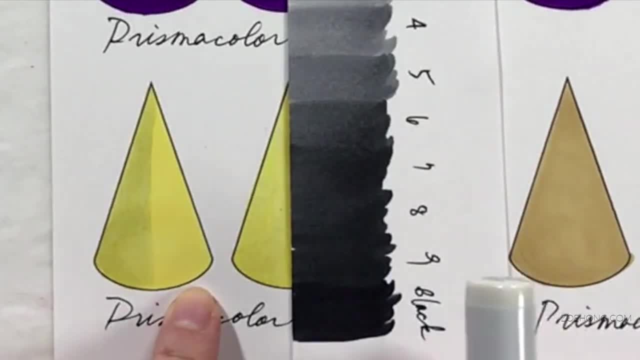 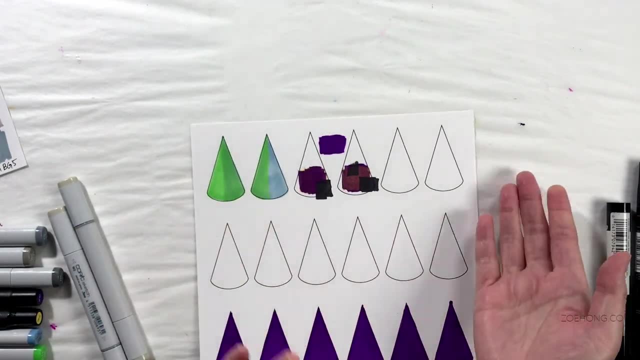 it's not creating as much of an impact on the yellow. Okay, The last is mutes, And we went over that with this here, layering the yellows and the purples together. We could try it with some other colors too. I pulled. 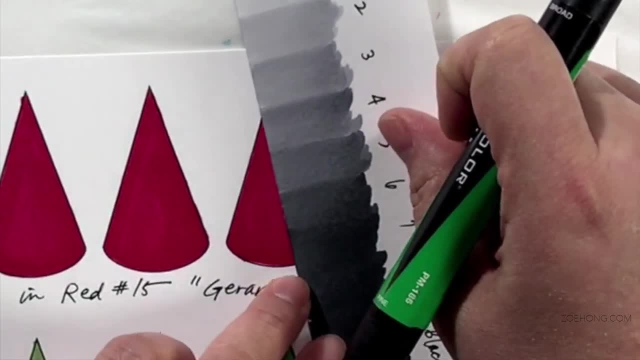 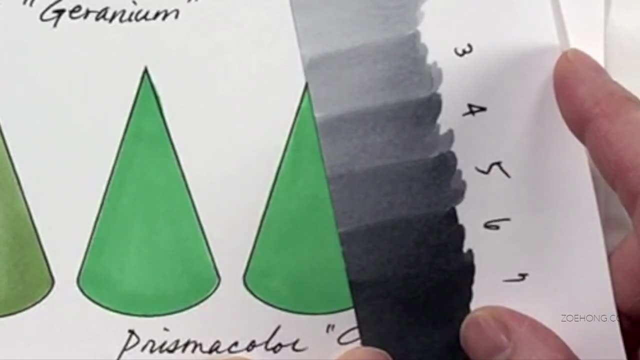 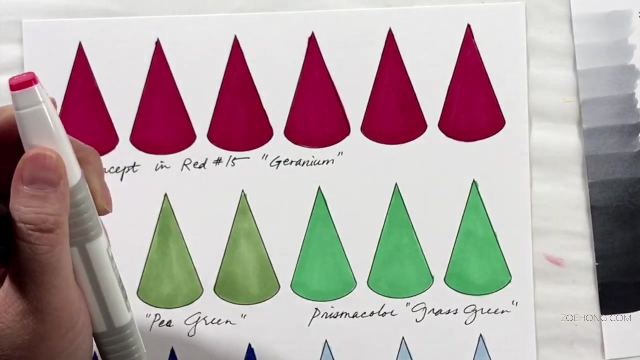 a few different greens to test out. Red typically will run like a five- six. It actually wants to be in between there. right, The grass green is closer to the five than the six. This one, which is this concept in geranium, is a touch darker value. Let's try putting this green on and seeing what. 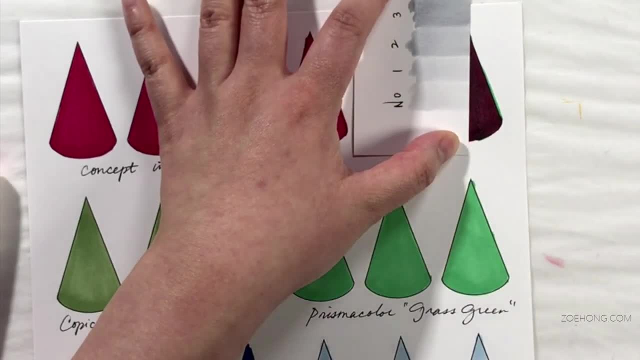 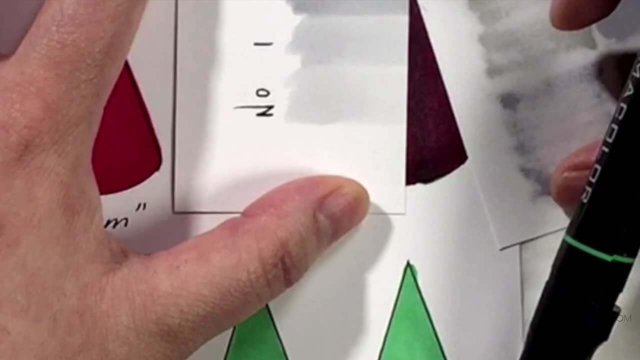 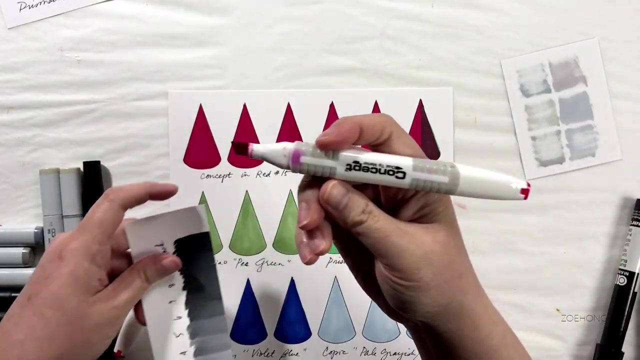 happens. So you're getting this really awesome burgundy color. actually, I like that, but that is a really great burgundy color And now, if you're mixing paints, you know how to make burgundy red and green. By the way, this concept brand- okay, this is a nice cheap brand that I bought. 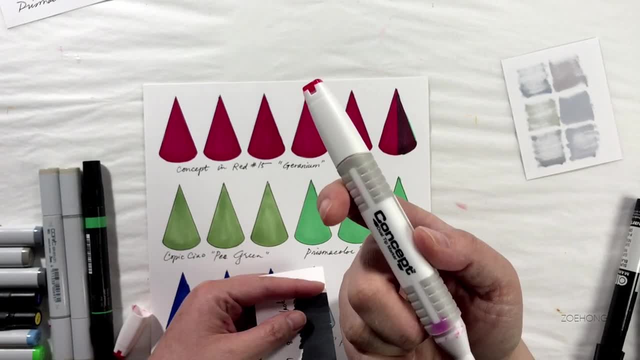 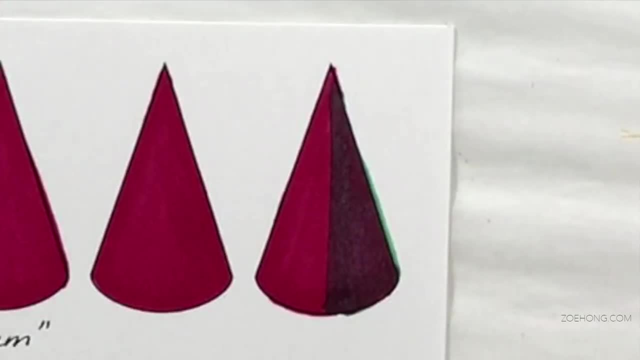 It's called Apcotax. A prendre white is definitely up to buy. I bought two of these at Jerry's art oraama in New York last time I was there And I'm actually enjoying these quite a bit. Sometimes I find that they start kind of like getting a tiny bit grainy And I just like to 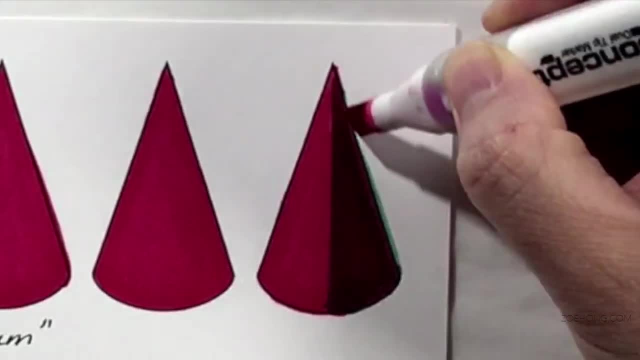 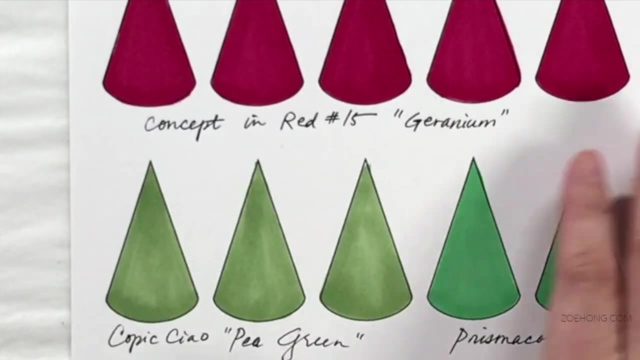 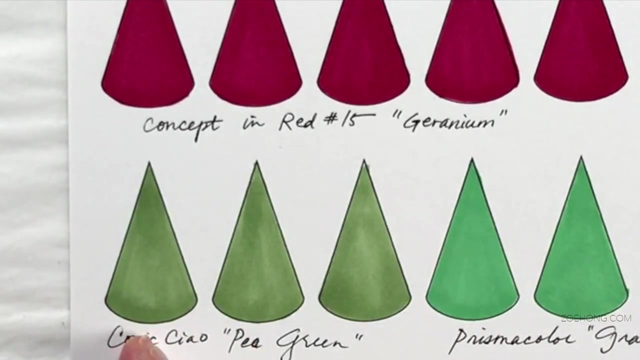 go back in and put in another layer, and it kind of tends to blend things out When you're muting a color that's not like pure saturated color, but something that's already toned down a little bit into consideration. because think about if you put this dark, bright red on this dull green that's. 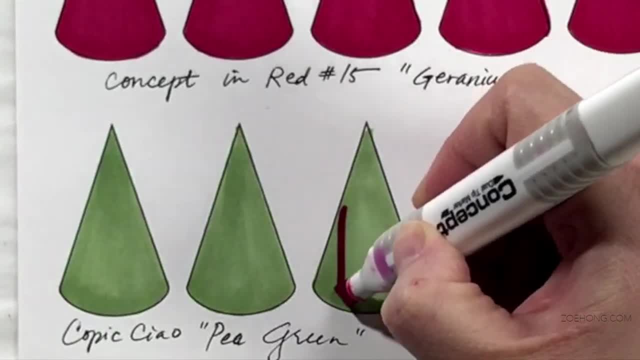 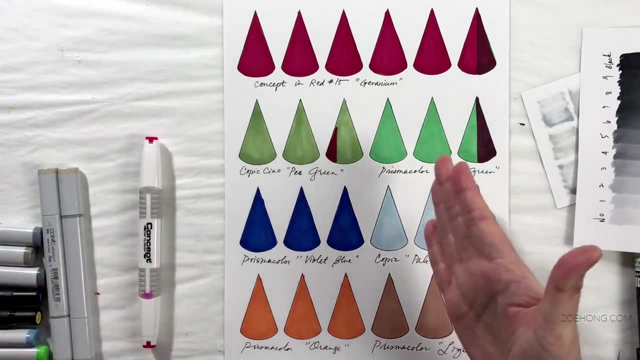 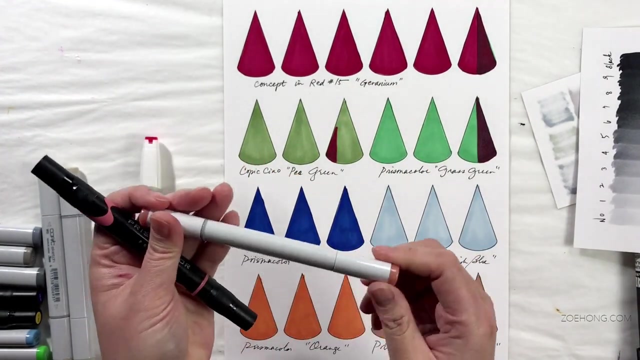 gonna pat like a huge punch. you're like almost obliterating that green right. so if you want to mute a pea green like this, this is the copic chow. and pew green, pea green, not pew green, puke green. no pea green i would use. i would go for a toned down red like this is the. 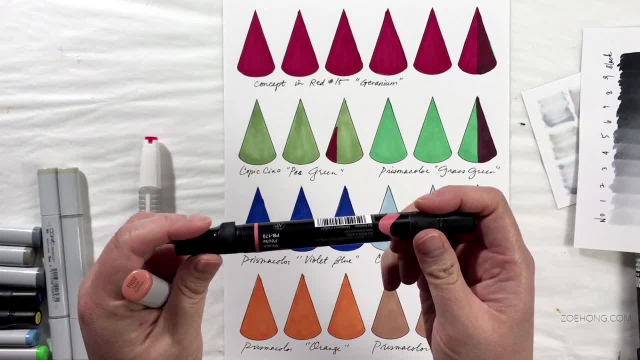 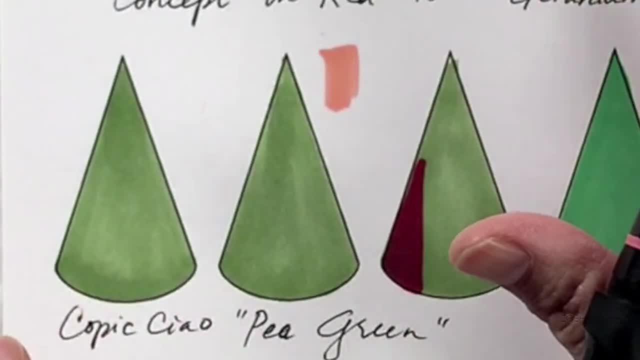 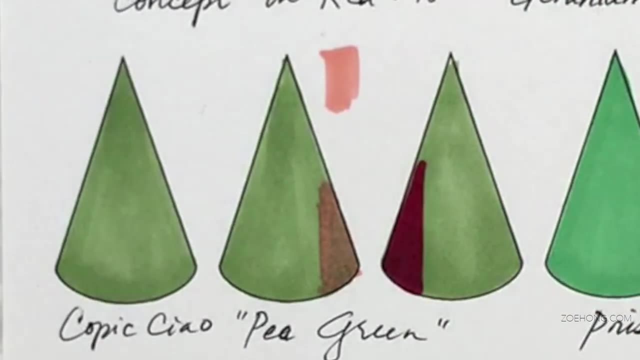 copic rose salmon. this is the prismacolor peach. this is what it looks like by itself. it's a tint of a red. basically is what it is. that's what peaches are. they're red plus white, like a warm red plus white. so you're still seeing more of that green in there, but you're still seeing more. 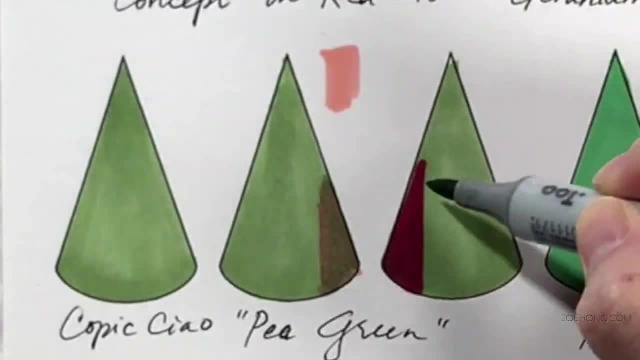 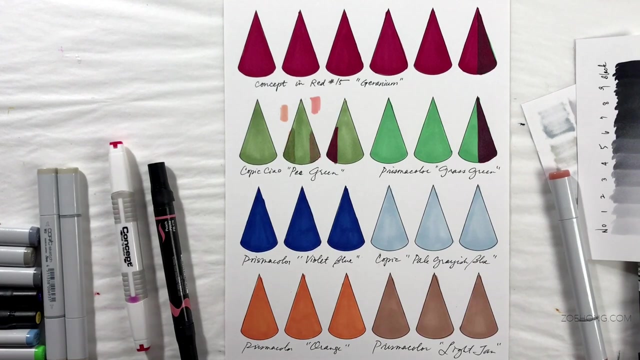 there that that peach is really powerful, though bring that in again. see, it doesn't touch the red so much, but it does blend in with that peach better. see, this one is a softer color to begin with. so what's the practical application to learning all this layering? for me, the big practical 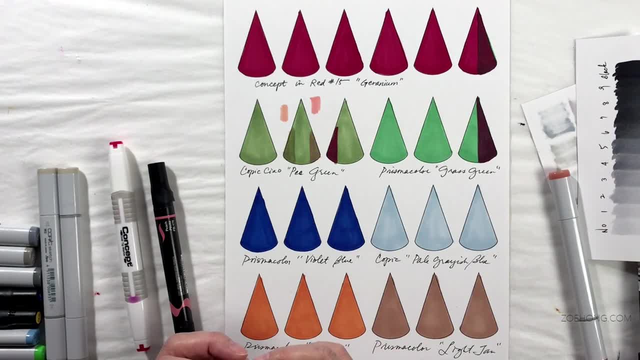 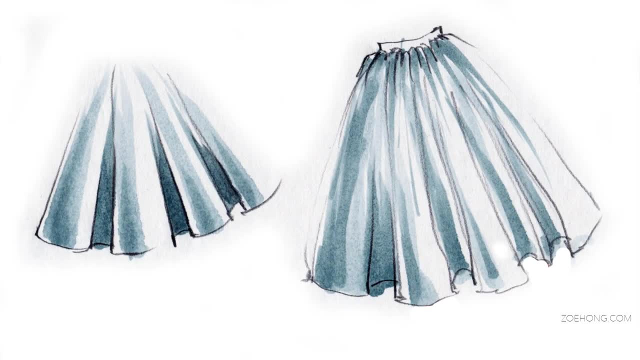 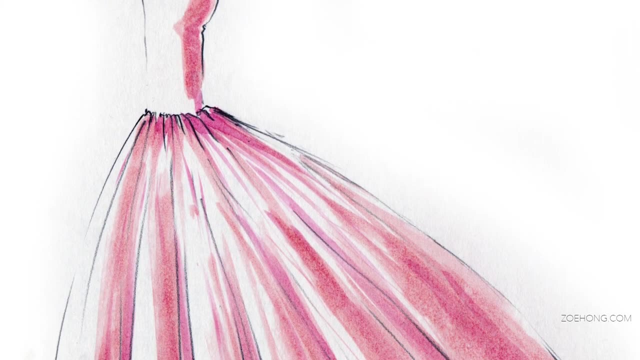 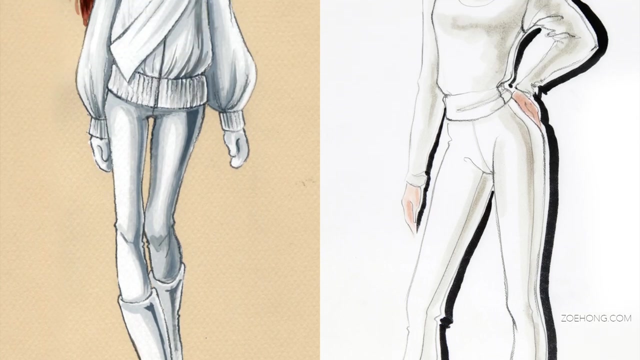 application is choosing shading colors for my illustrations. you we have three main options for choosing shadow colors. a few weeks ago, i posted a video on shadow placement- where to put your shadow so that your garments look 3d- and now we're going to talk about what colors to use so that your garments look 3d, look interesting, etc. number one: you can shadow. 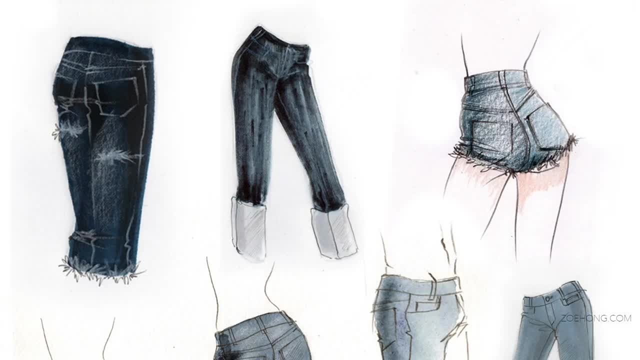 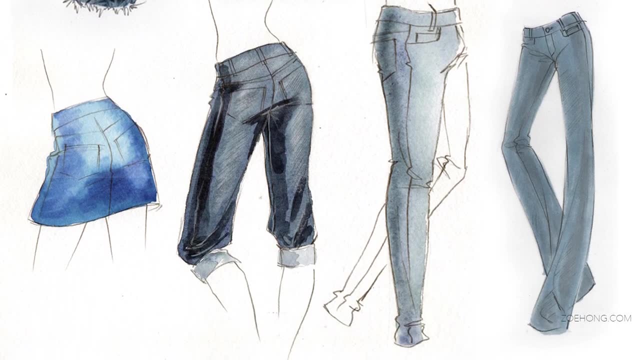 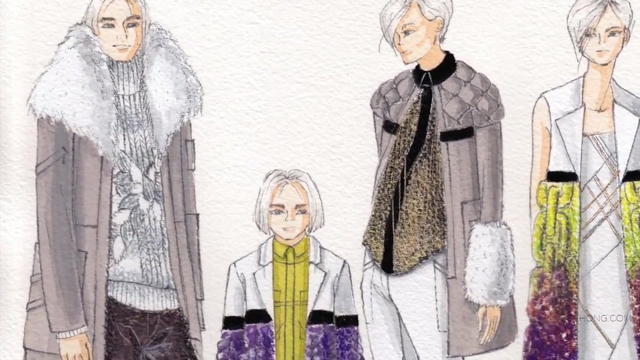 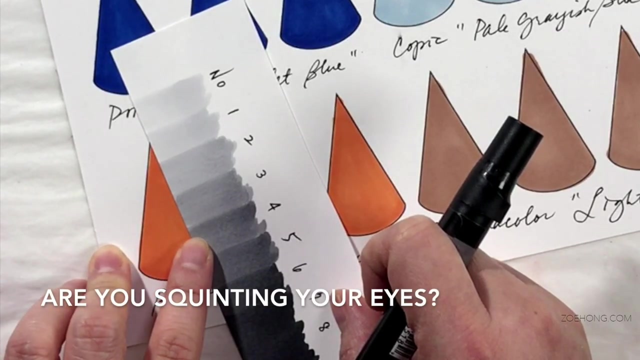 your garments with gray. in my own work, i choose to shadow with gray when i want to tone down the color, or i'm using a neutral okay where i want it to look more toned down, more chilled out. this prismacolor orange, what value is it? i would say it's like hovering between a three and a four. 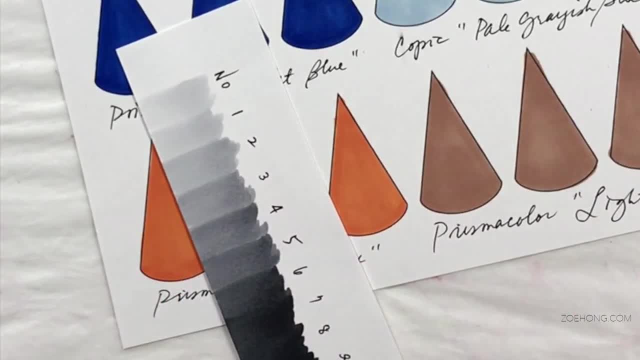 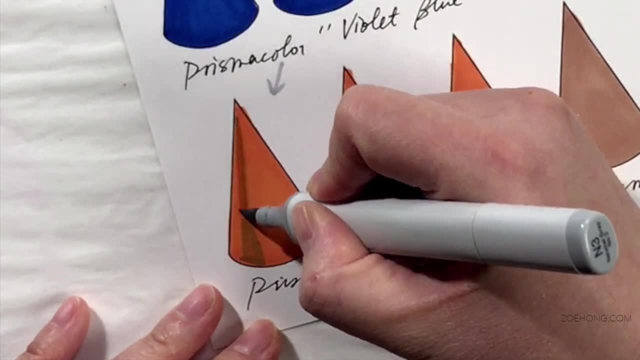 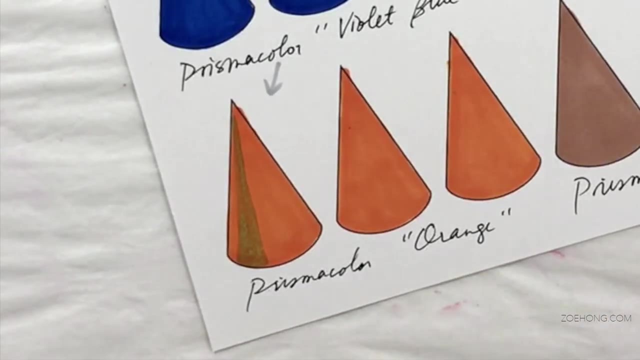 and so that's the color i want. this is a natural three. so if i want to shadow it- and that's my light source- i will put my shadow over here, and i'm going to go ahead and do that. and i'm going to put my shadow over here, and if i want to blend it out more, i would take that same color again and i 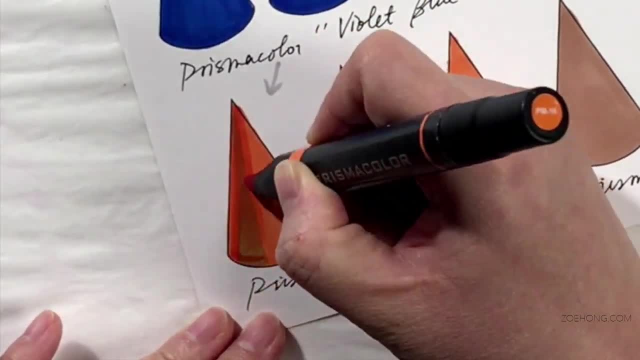 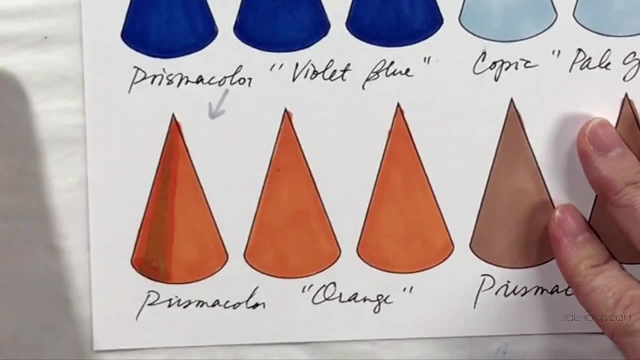 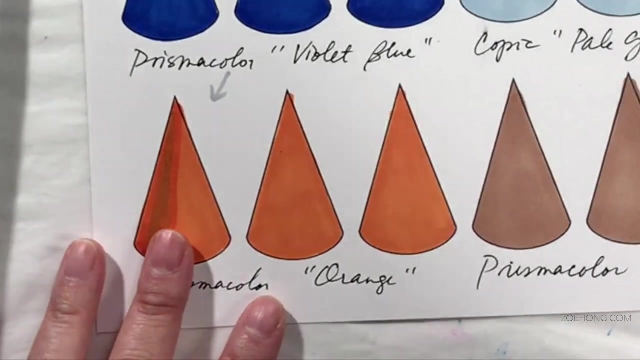 would layer it up and i would let the edges bleed some of that orange to kind of blend things out, and then i get the shadow. i personally think that when you have a color as vibrant as orange, the gray really dulls things out and shading with gray is a better option. 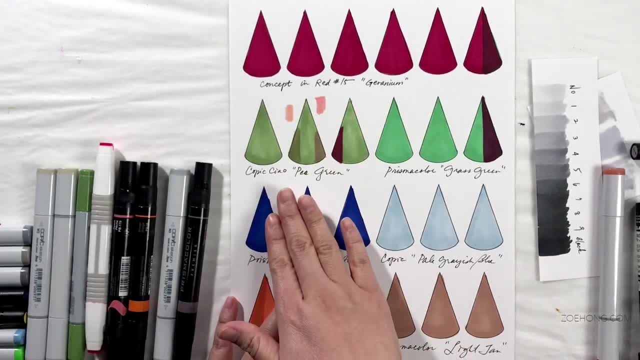 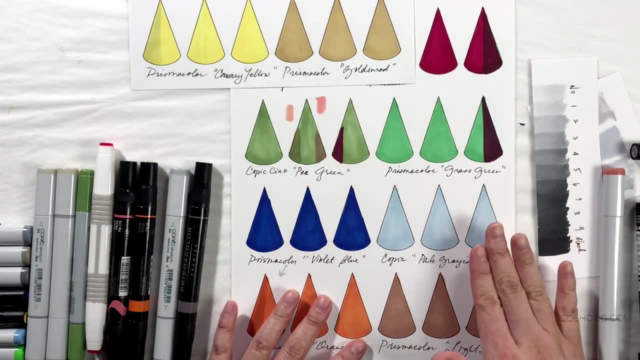 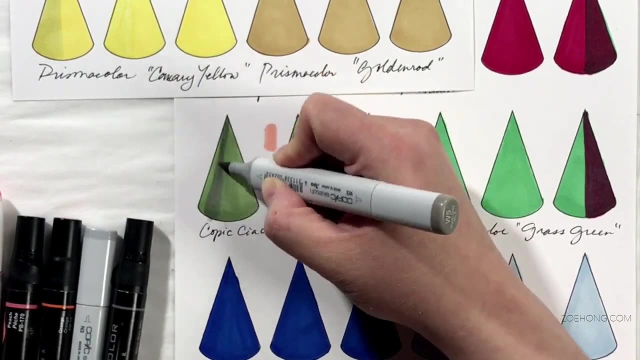 for things like that are duller, like this green is kind of dull, this golden rod is kind of dull. even this blue would take a cool gray quite nicely, something like this: here's a warm gray five, and then again i would take that original green and blend it out. 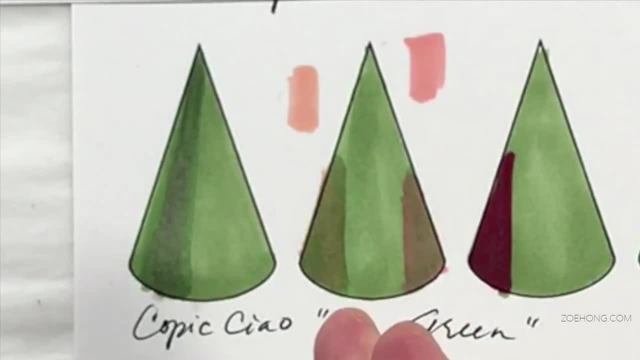 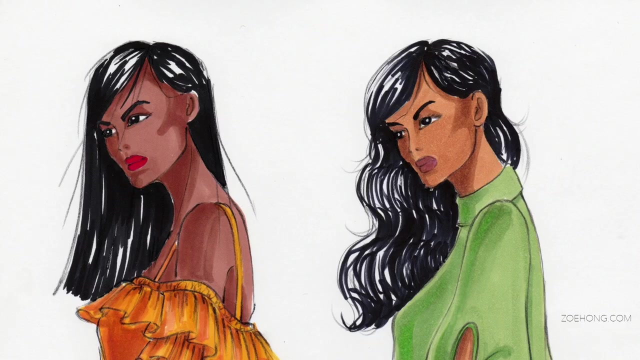 and you get that nice shadow. and the gray shadow works much better on a dull green than it does on the orange, in my opinion. when you have bright colors like the yellow and the orange, i personally like to go with option number two, which is a darker, more intense version of the base color. so when you have 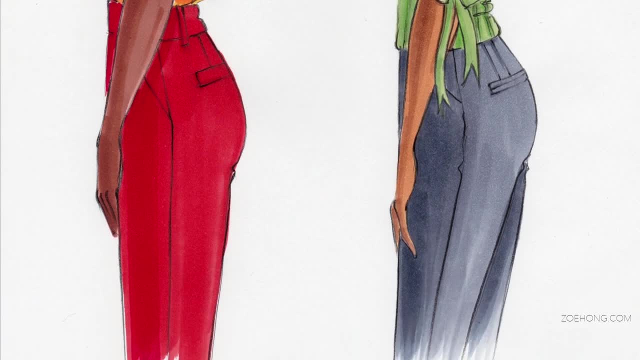 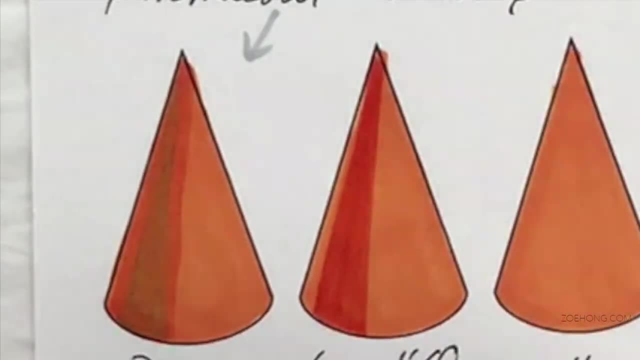 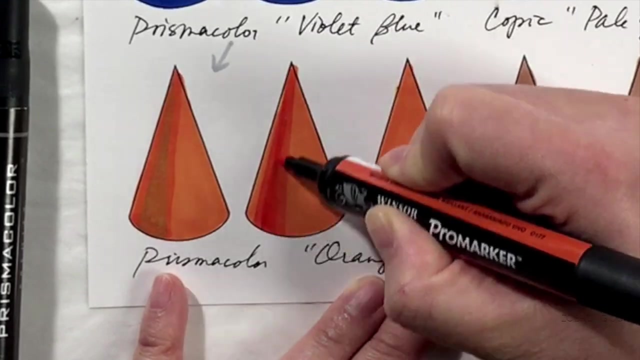 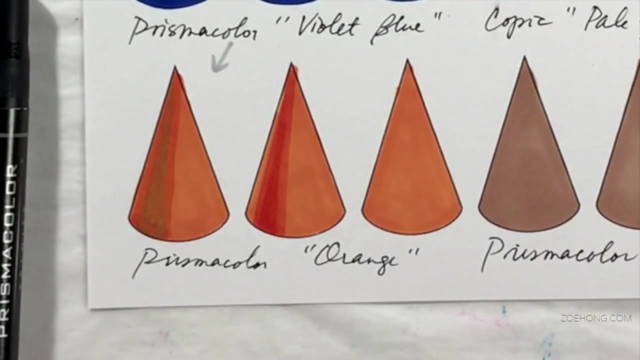 prismacolor orange, i would shadow with a darker orange. this is windsor newton pro marker in bright orange and that works as a shadow color better for me than that. sometimes i'll go in again and put in a darker shadow in between and you can use yet an even darker color or another layer and it kind of gives it. 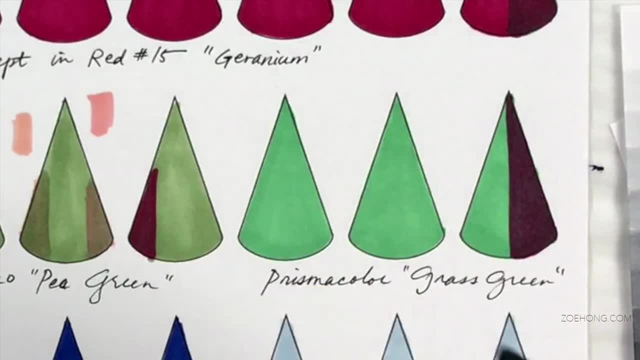 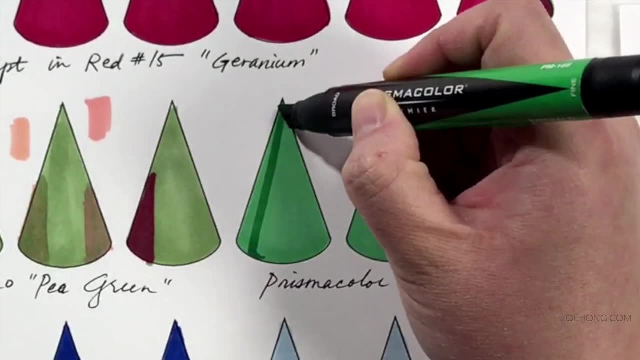 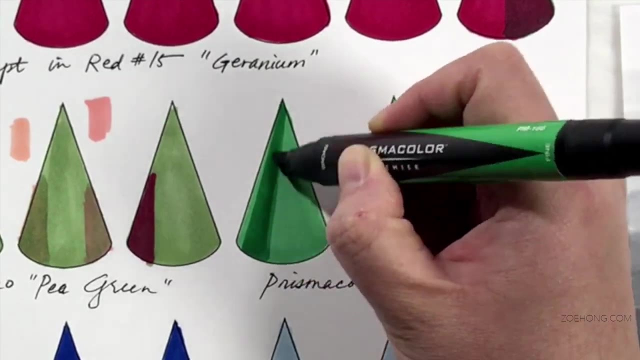 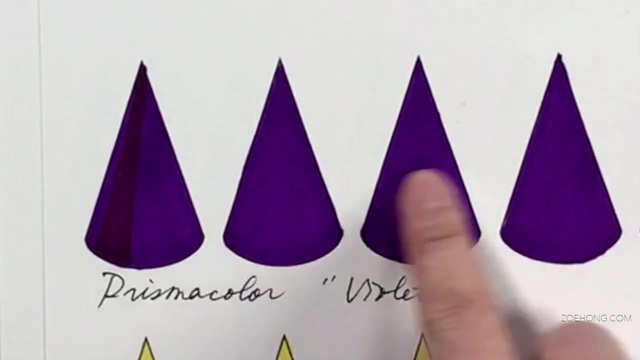 another dimension, all those good things, this beautiful, bright green, that's prismacolor grass green, this is prismacolor and emerald, and again this one has a really beautiful, vibrant kind of thing going on. so here's the thing I want to show you. so this is Prismacolor violet and this is Prismacolor. 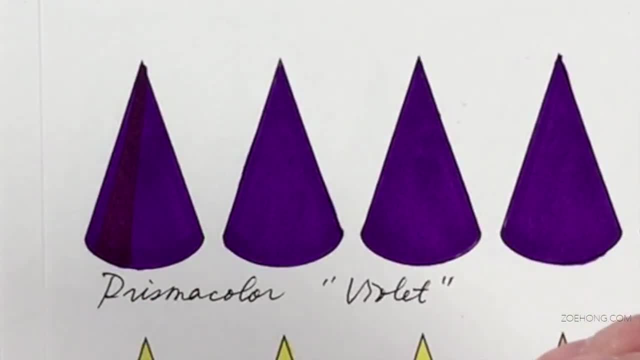 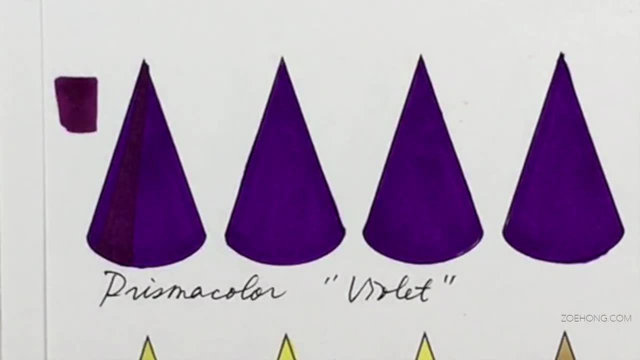 dark purple and this color. it is a redder purple. on the come on the same conversation track as choosing the shadow colors to change their overall mood. if you wanted to warm up an illustration, you could choose a warmer shadow color to help that look like this dark purple. on the other hand, you 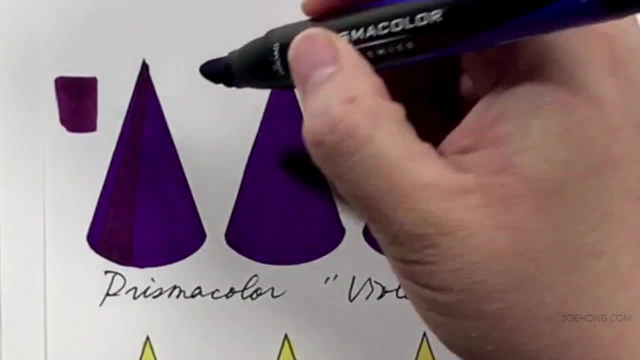 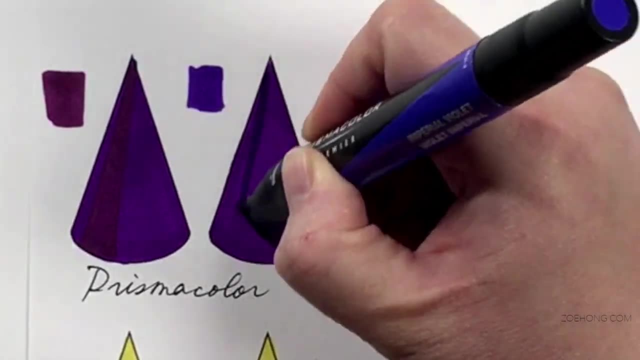 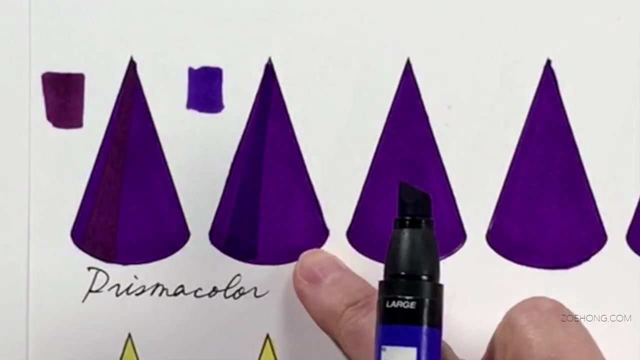 can choose another purple. this is Imperial violet, which is a much cooler purple, bluer, and you can shadow with that and that gives a different vibe. so even if your fabric base color, if this is your swatch color and you've got that color going on, you can still kind of alter the mood and the general feel for the color by changing your 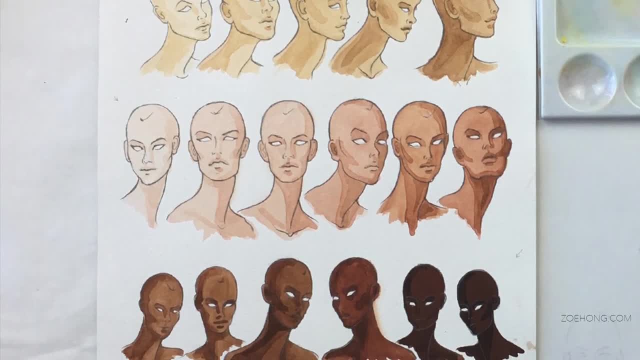 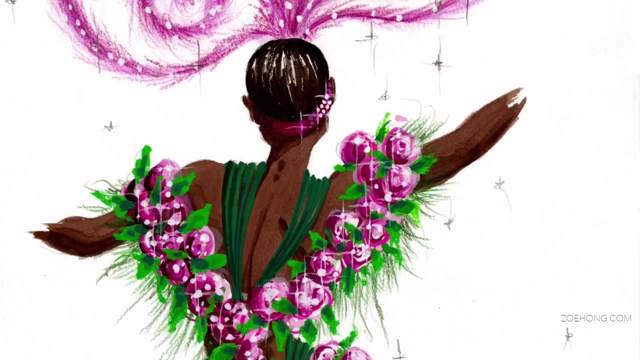 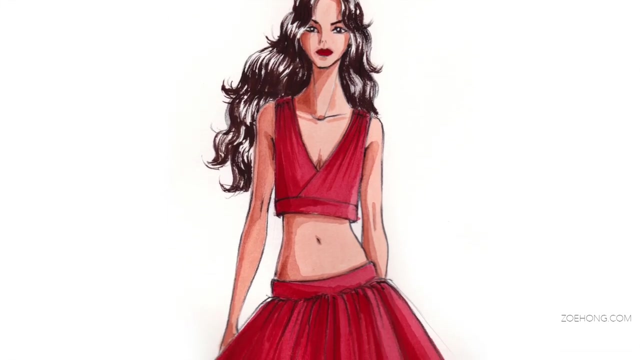 shadow color. this is how I like to shadow skin tones with the darker, more intense color. I absolutely never shadow skin tones with gray. it always looks terrible, unless I'm doing like a super stylized thing where I have a really weird skin color. if I'm going for a natural skin color, 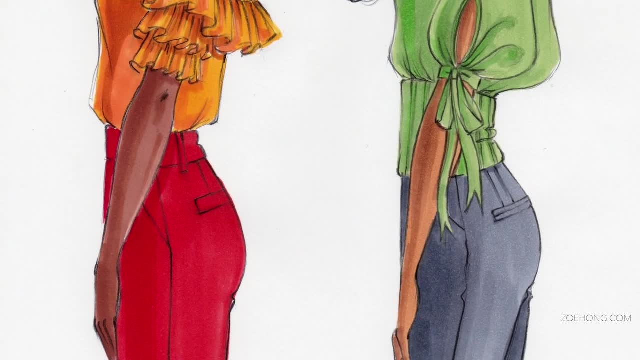 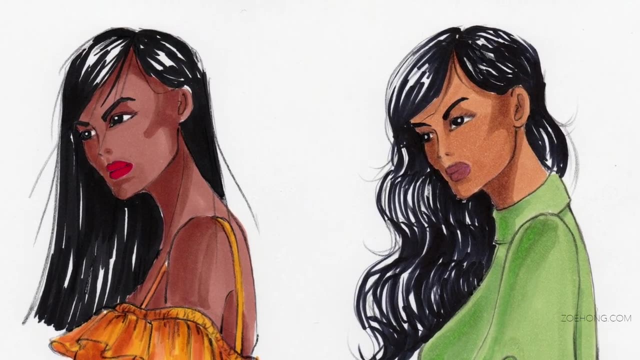 then I'm not going for the eye the range of a good kind of кол-white. but if I'm not, you can imagine never shading with gray, I'm always shading with a darker version of the base skin color. This base color is the Prismacolor light tan. 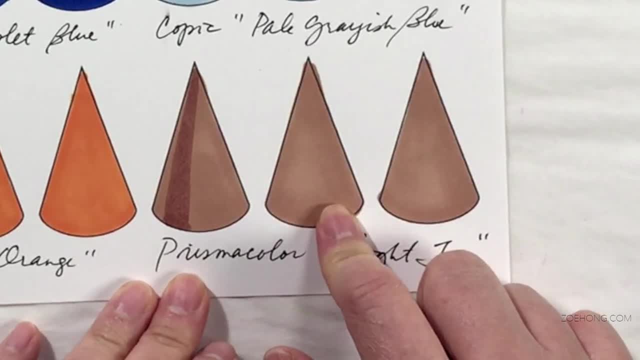 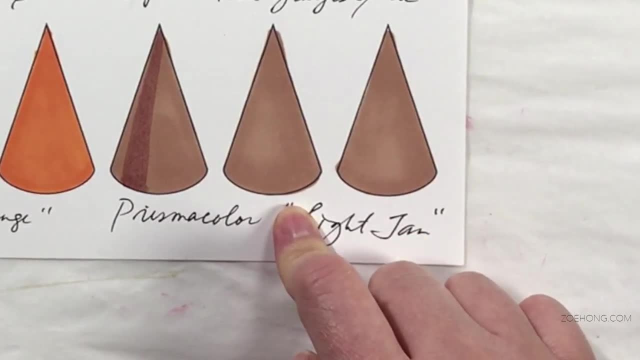 If you're using this as just a you know a coat color, just like a you know rosy camel cashmere coat, sure you can shadow that with gray if that's the look you're going for, Here's a warm gray five. I would not want that shadow color on skin. This is not the kind of thing where you know. 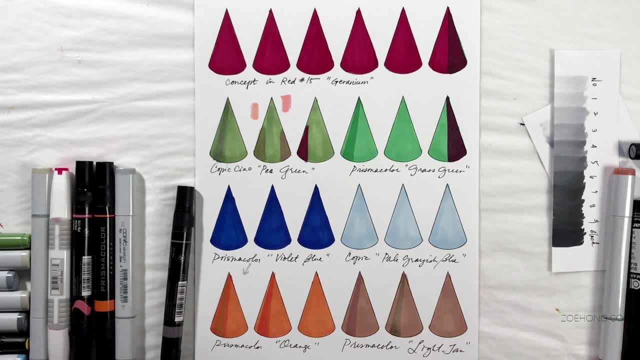 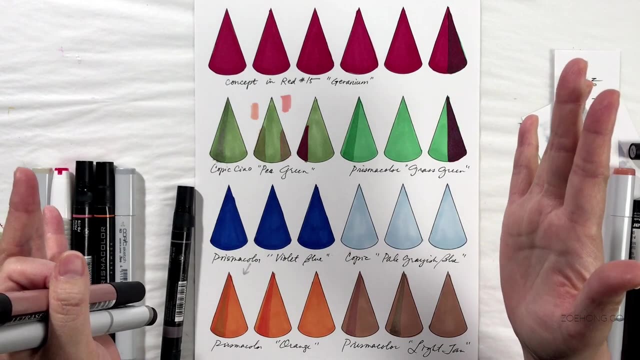 watercolorists who do these portraits. they do these really stunning skin tones with like blue shadows and you know like they can really manipulate skin in beautiful ways. but when I'm talking about like fast marker design sketches, I'm not trying to go for like multi fast marker design sketches. I'm trying to go for like multi fast marker design sketches. 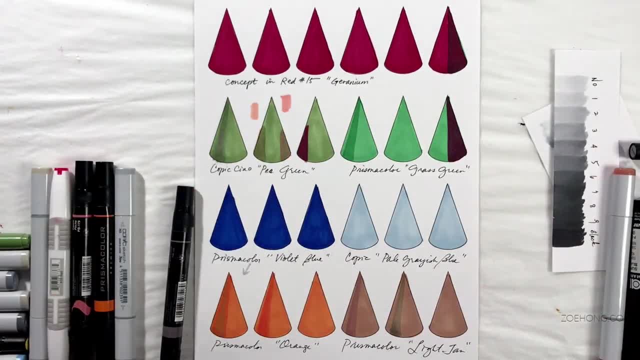 I'm not trying to go for like multi fast marker design sketches. I'm not trying to go for like multi faceted, you know, beautiful, catching the light skin. I, you know I can, I can have fun with that in watercolor. but for design sketches I just want enough marker work so that things look 3D. 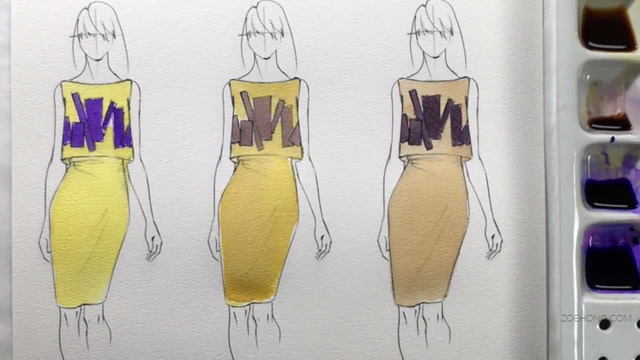 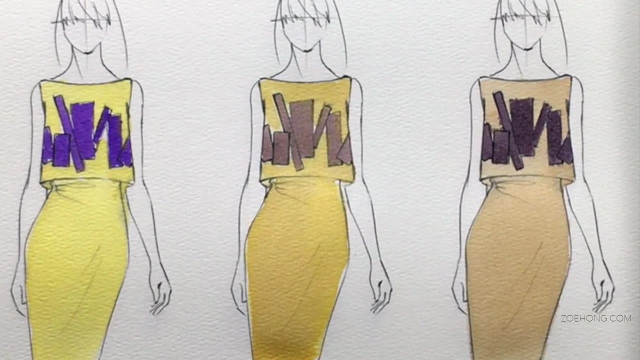 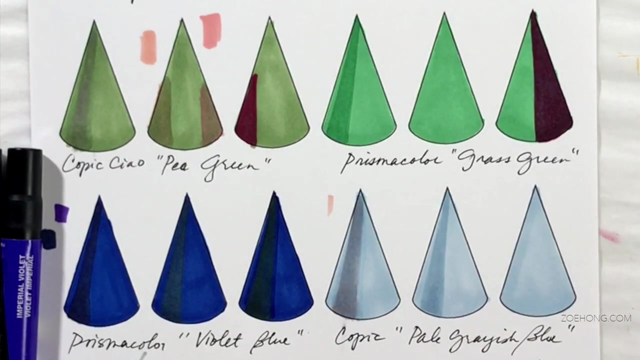 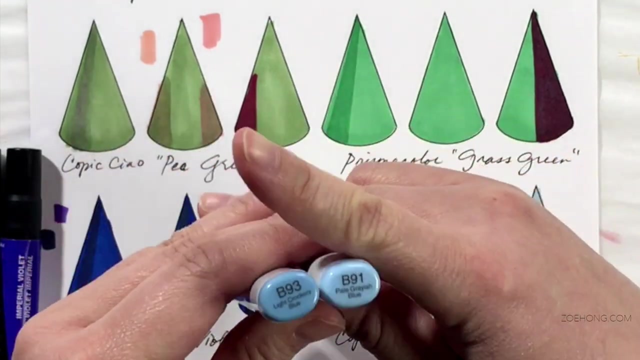 The third option is to use your compliment to create a muted shadow, And you can do that if you want a more dimensional look to your garments, to your shadows. So this is the Copic pale grayish blue with the shadow of the Copic light, crockery blue. Okay, B91 and B93.. And so, again, when I want, 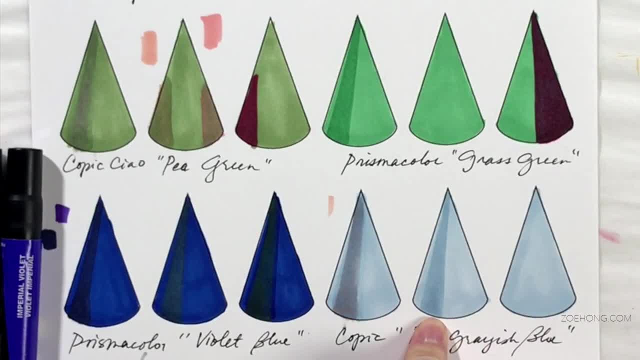 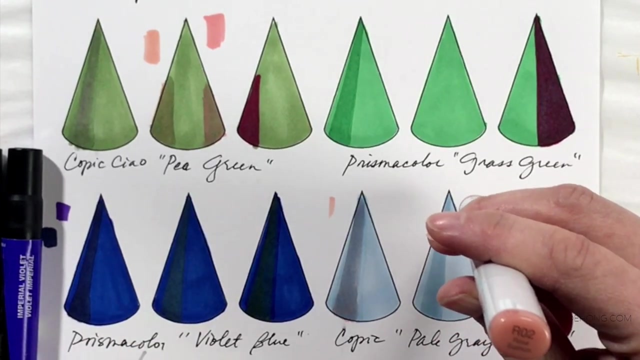 to really punch out the color and make the blue prominent, just using a darker, more intense shade for the shadow. Now, here in this, if you want a little bit more depth and create muted shadows which, in all honesty, is a little bit more realistic, Then I layered the RO2 rose salmon, which is a tint of orange. Okay, It's. 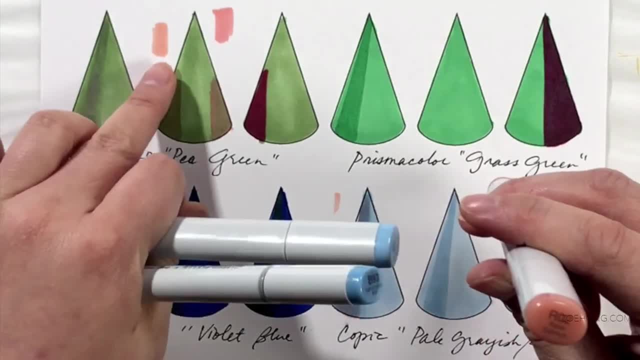 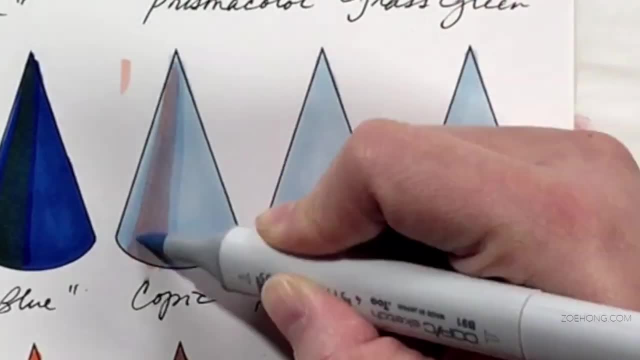 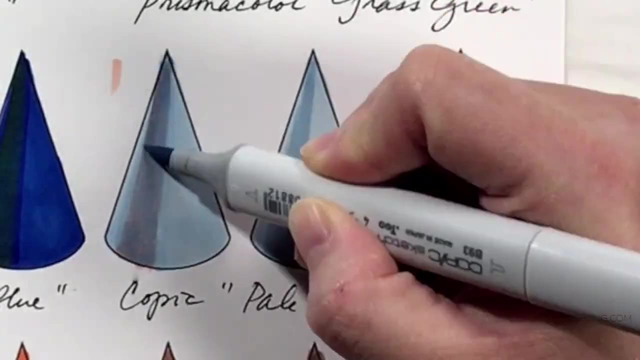 like a reddish orange and it's a tint. That's the color by itself right there. So I layered some on top of the pale grayish blue And then I went in with the layer of the, the light crockery blue. So it's still blue, but it's a little bit duller. The bright it's less. 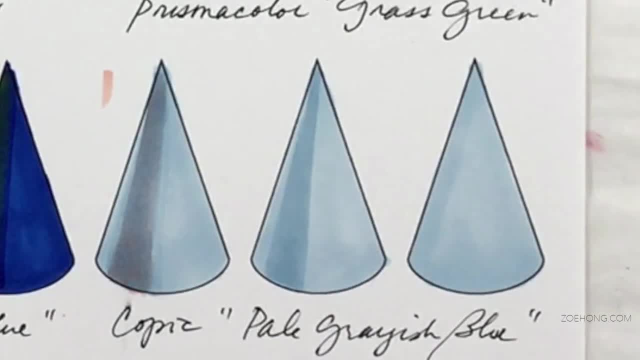 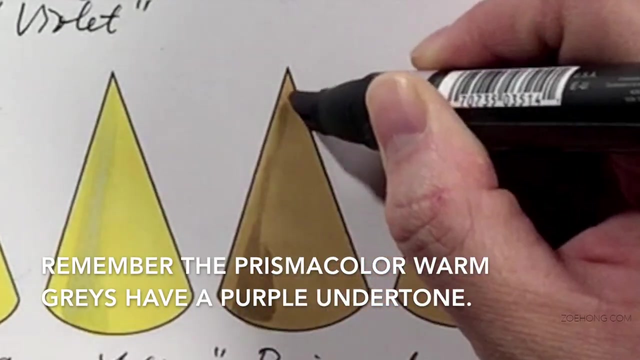 bright, but I think that it looks more interesting and it has more depth to have those mute undertones in the shadow. This is Prismacolor golden rod and this is a warm gray 40. And again you're bringing some of that soft. 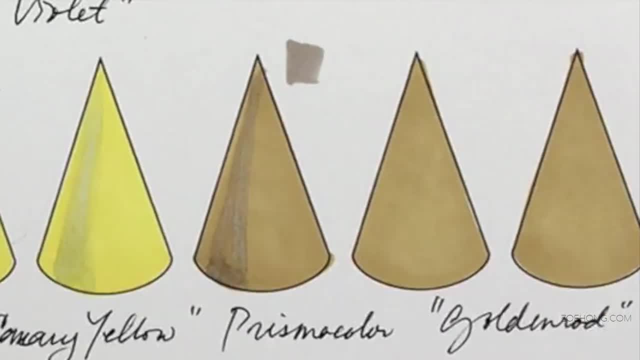 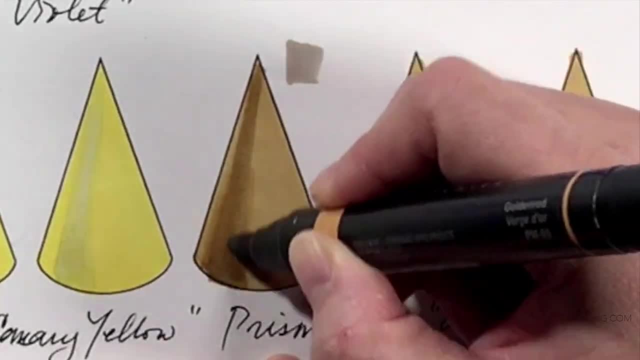 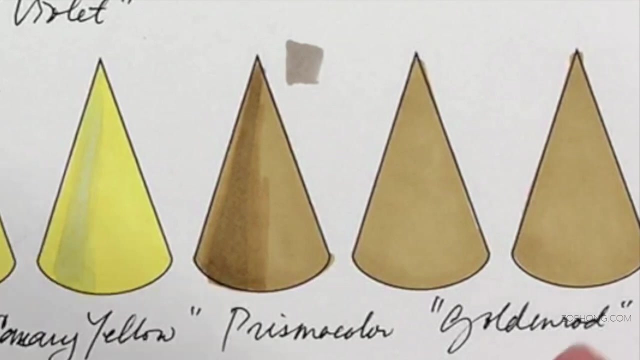 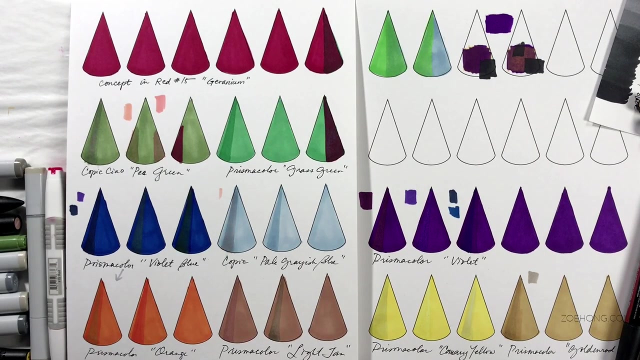 muting into the shadow And then, if I take the golden rod again and layer it some more, I'm like warming it up and kind of blending it back in with the rest. So, using the compliment, finding the right color can really add some depth and dimension to your shadow work. All right, I hope this video 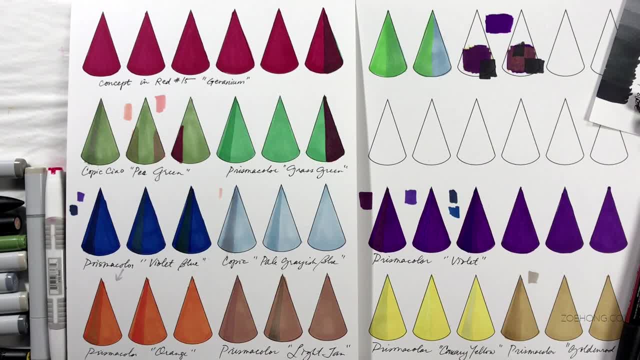 was helpful. Please do give this video a thumbs up If you learned something new today. leave your questions in the comment section below. share, subscribe. you know all those ways you show me love and I will see you in the next video. 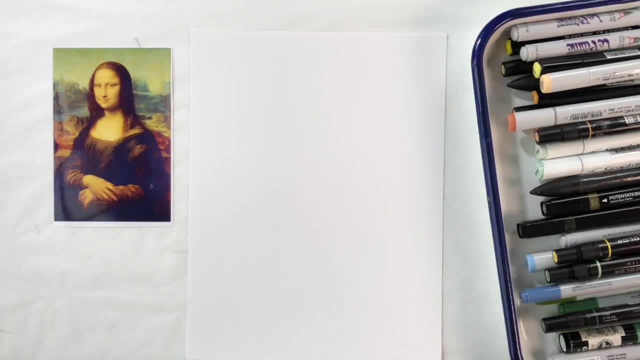 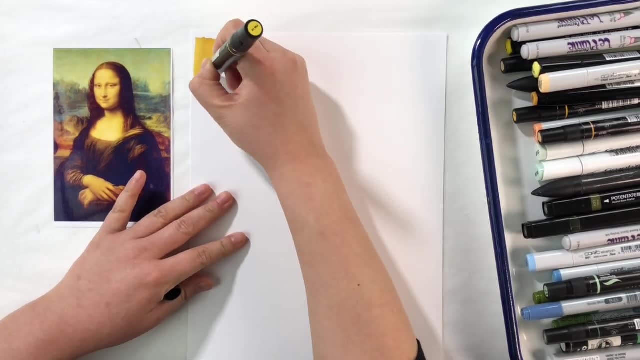 Hey party people. in this video I'm going to discuss choosing a color story for your fashion collection. Specifically, I'm going to one go over several methods to develop your color story, to list factors you have to consider when developing your color story and three answer. 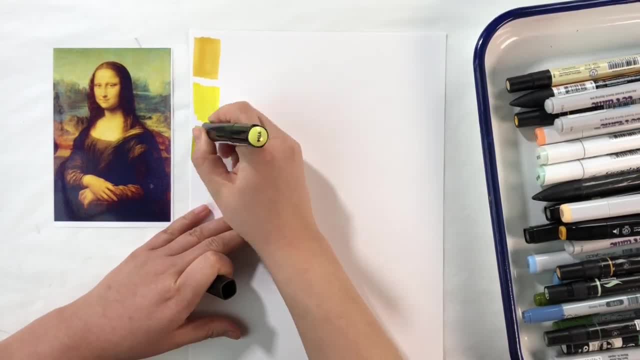 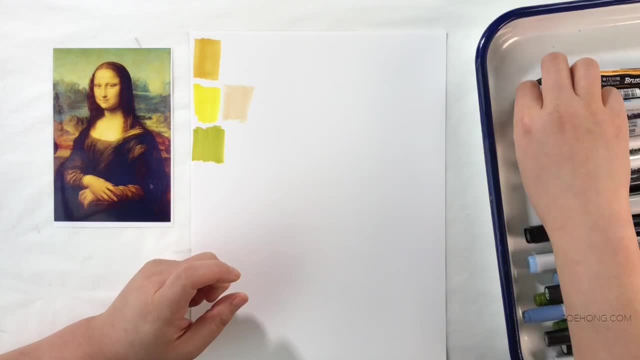 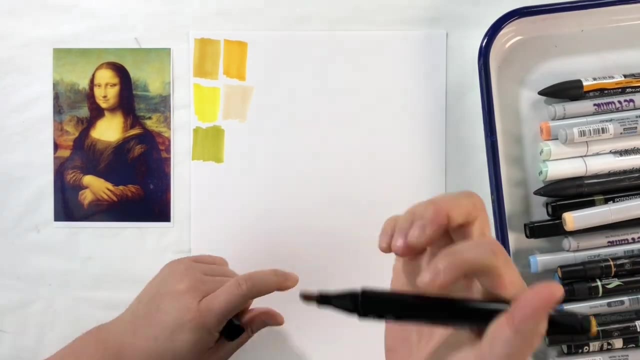 the number one question. Well, ask me about color stories. First up methods to develop color stories in the industry. large to medium sized companies often use trend forecasting, color forecasting services to help them. Most smaller businesses can't afford or don't want to use these services. One method is: 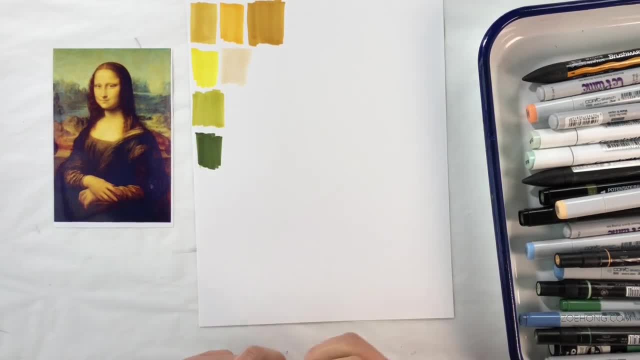 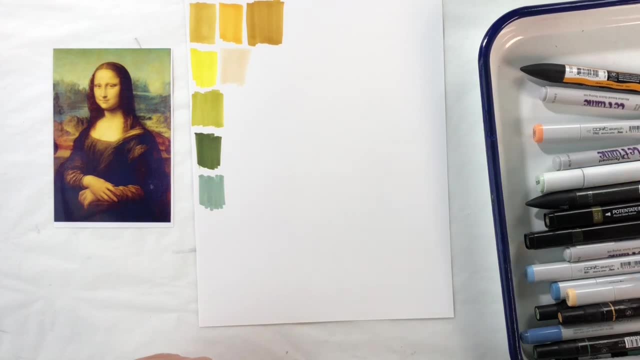 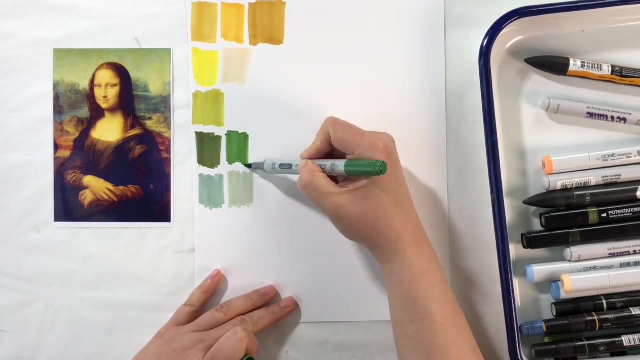 to pull colors from an image or a couple of images. These images can be from your sketchbook development or your mood board. You know I would only pick like a couple of images at most. Otherwise you just get too many colors a lot of the time. One method I like is to choose a work of art. 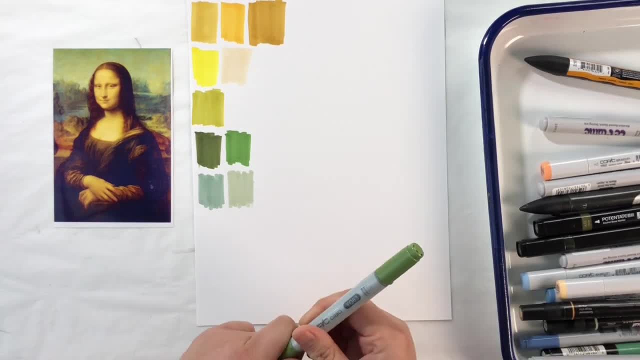 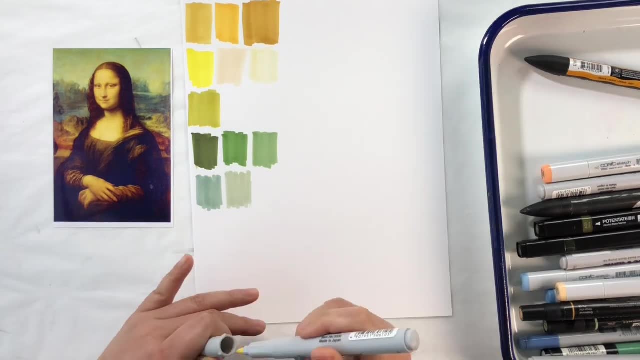 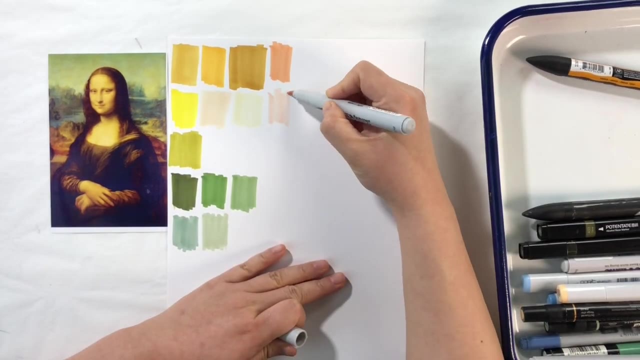 that your customer would enjoy. Remember all design decisions. go back to your customer, your muse and your brand. Listen, if Raph Simon can get fire from Calvin Klein for not designing for the customer, so can you. Anyway, this work of art can be. 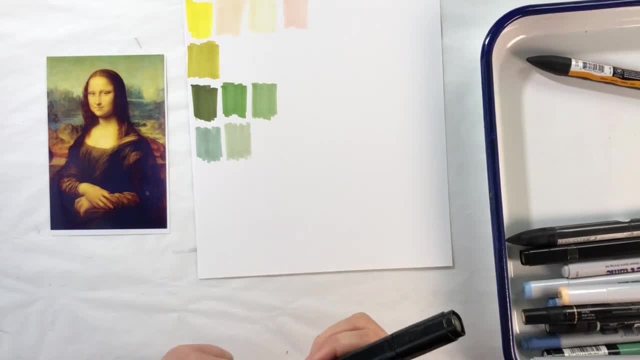 a painting, a photograph, a sculpture or even a building. Pull colors from this painting to create your color story. If you watch the colors and textures video from my fashion design process series, then you know that I was inspired by extraordinary chickens And that whole thing. 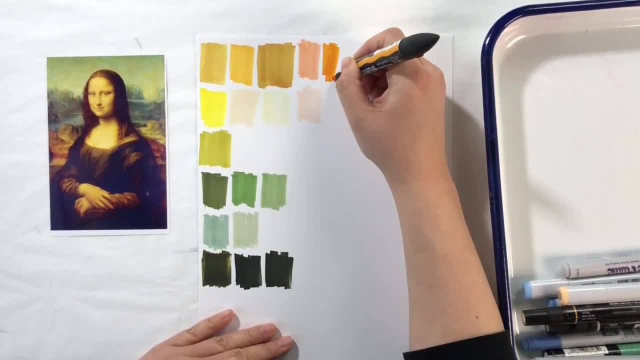 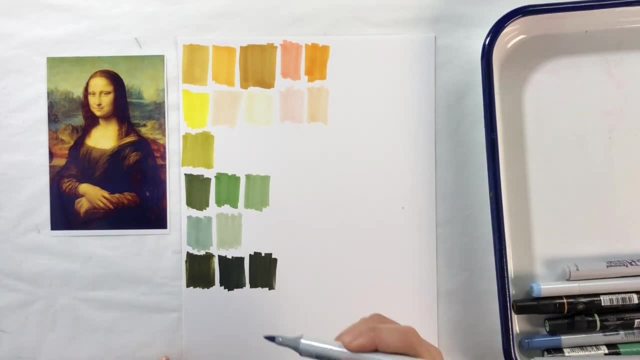 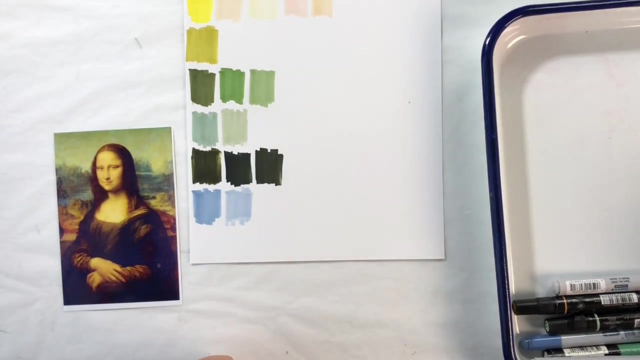 has become this long running inside joke between me and long time viewers of my channel. And yeah, there was this amazing photo of different color chicken eggs in the extraordinary chickens book And that was the inspiration for my color story. And then, yeah, sometimes you'll have to take an image and round things out by adding an extra. 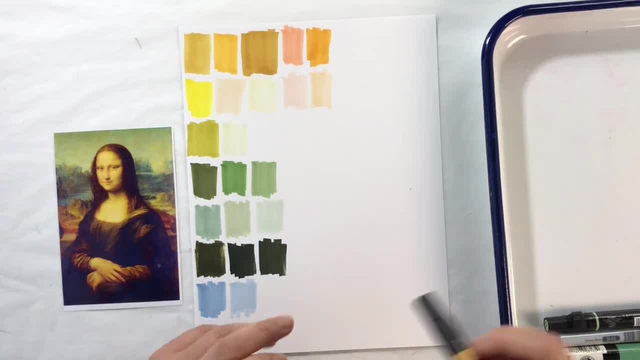 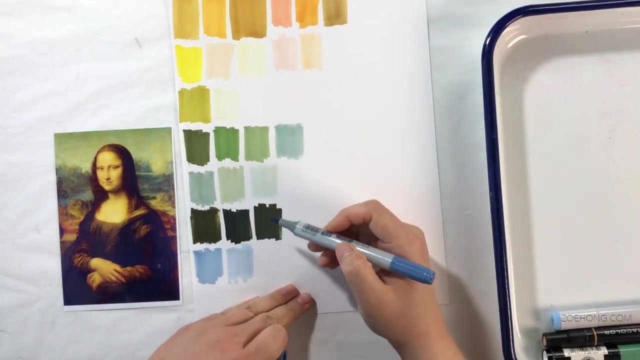 neutral or adding an extra pop color. But you can start from that work of art. The piece of art has to relate to your customer. It should be something that your customer would enjoy looking at, would enjoy having a print of in their home, or maybe even the original. 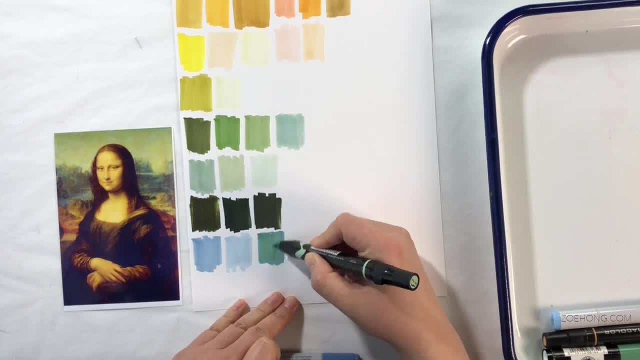 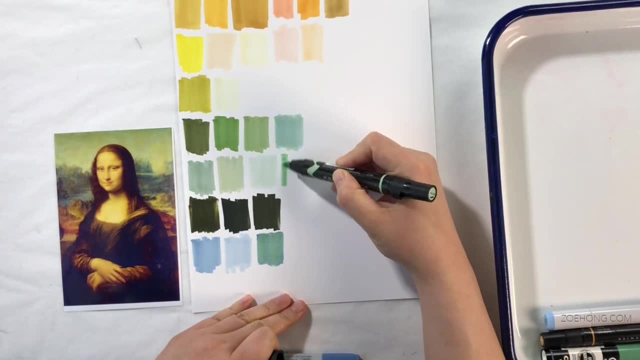 Something like that. Okay, it all has to relate In this example. let's pretend my customer is in her 30s and 40s. She lives in a big city. She wants an urban uniform without relying on too much black. She likes to look polished without thinking too hard about it every morning. 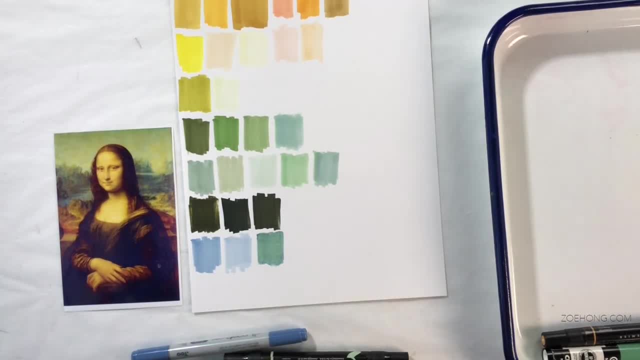 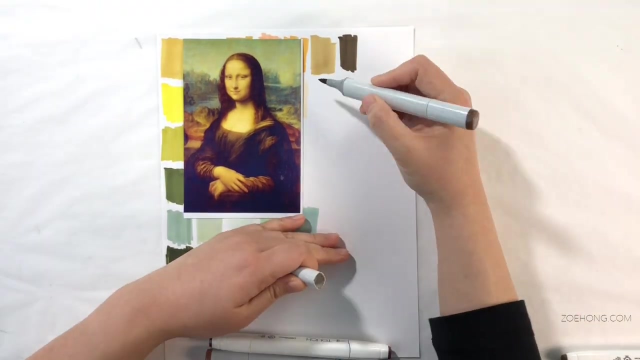 You know everything should go with everything else And she travels a lot for work, So she likes the core of her wardrobe to all coordinate with each other for fast and easy packing. I chose the Mona Lisa as my color inspiration. It's dark, it's moody, it's subtle, it's a little mysterious And it looks like there can be a lot. 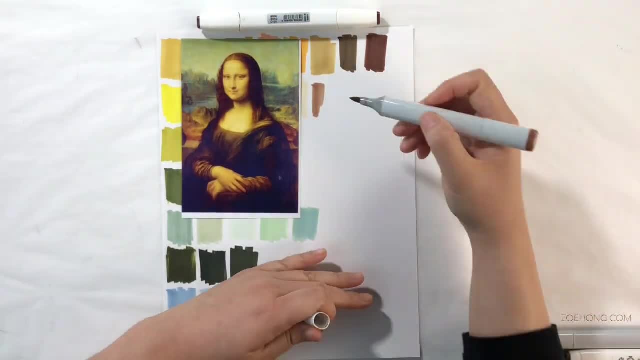 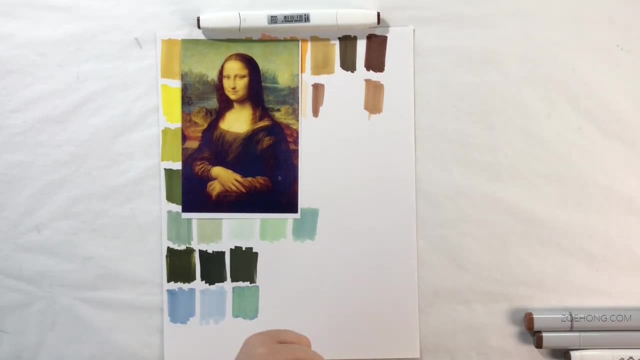 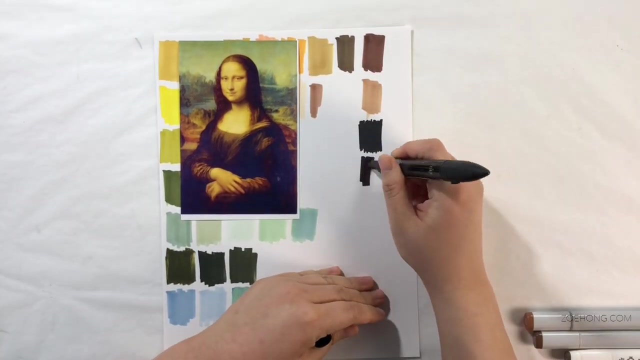 of different but cohesive, harmonious color stories. There's a lot of greens, a lot of browns and oranges, golds and some lighter blues in the background. Color stories should have a balance of colors and neutrals Should tell the story of the mood of the collection And then the neutrals sell. I mean. 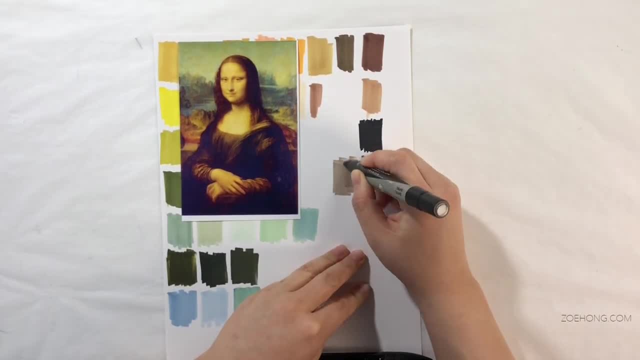 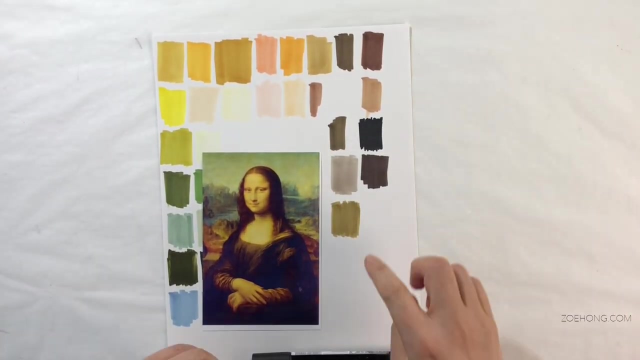 let's be real, the neutrals will most often sell the higher quantities. Color stories should have a balance of light, medium and dark colors. I say the word balance because creating a color story is not math. There's no one formula that suits everyone. You have to think about whether or not 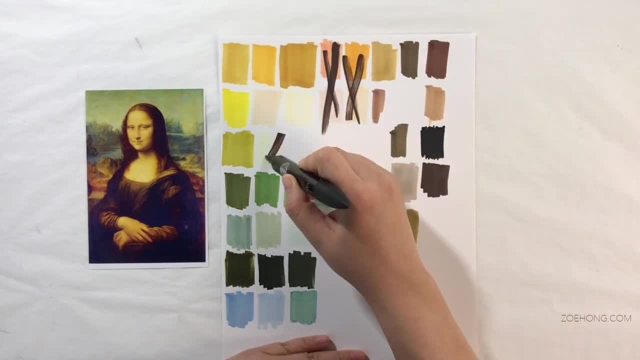 your customer wears a color story. You have to think about whether or not your customer wears a lot of color, whether they wear a lot of dark colors, or maybe your customer loves pastel colors, Maybe they love acidic tones. Again, back to what your customer wants. 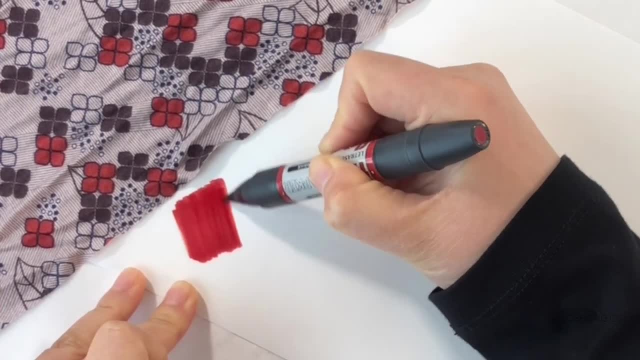 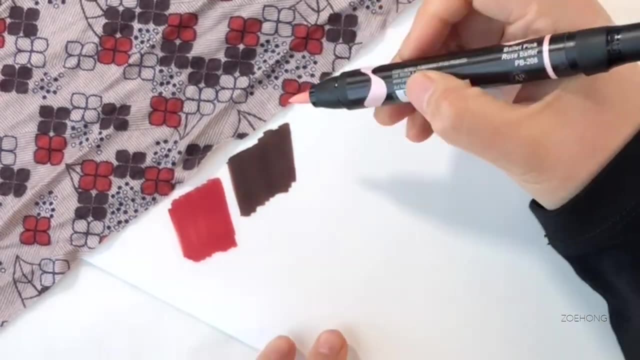 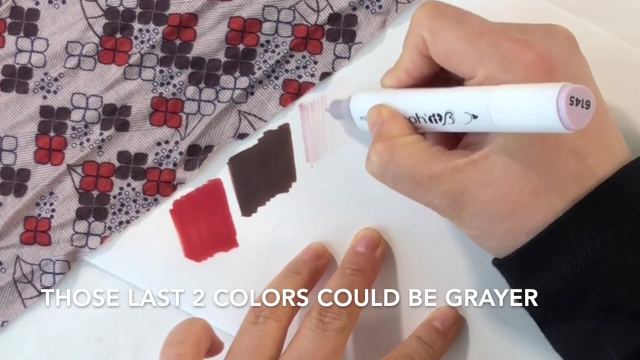 Another method is to visit your fabric sources and look through their prints And you may come across a print that is perfect for your collection's direction that season, And you can pull colors from the prints to create your color story. Design companies do this all the time: Pull colors from a print or recolor a print to match. 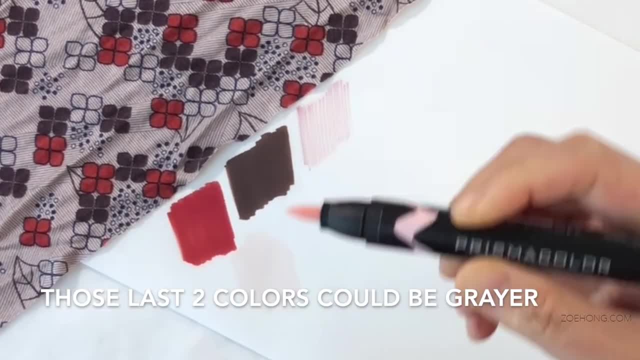 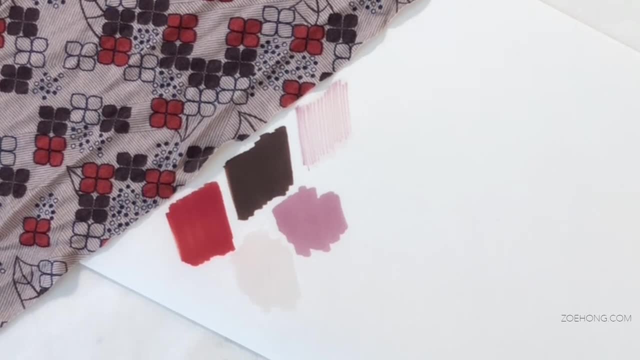 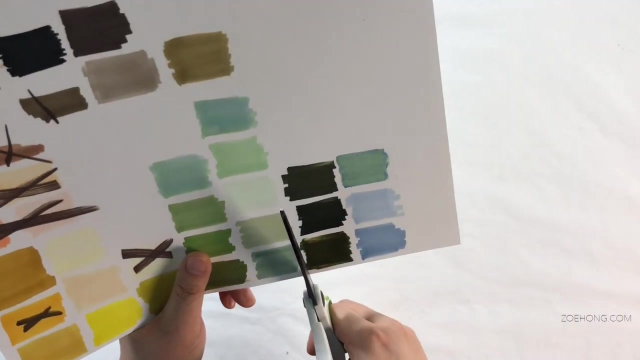 their color story, so that everything works together. And, honestly, you don't even have to use the print. You can just use it solely as color inspiration, because I like the colors of this print, but I don't love the print. Another method is to start with a color that you're really. 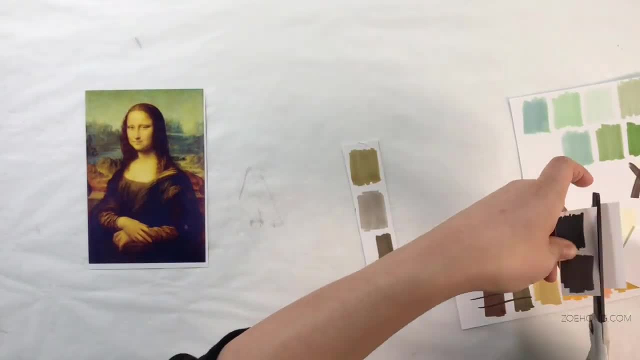 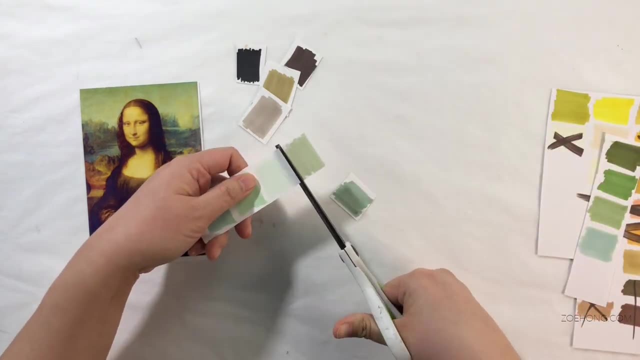 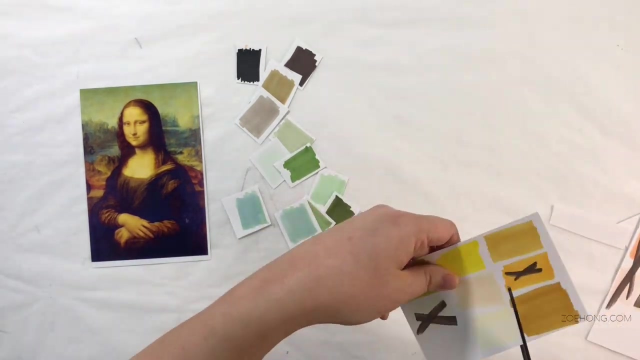 feeling and you think will be hot in the near future, And start playing with color schemes. I have a whole color lessons playlist where I go over what complementary, split, complementary, monochromatic, analogous and triad color schemes are. And remember these color schemes are not limited to bright red and bright green. 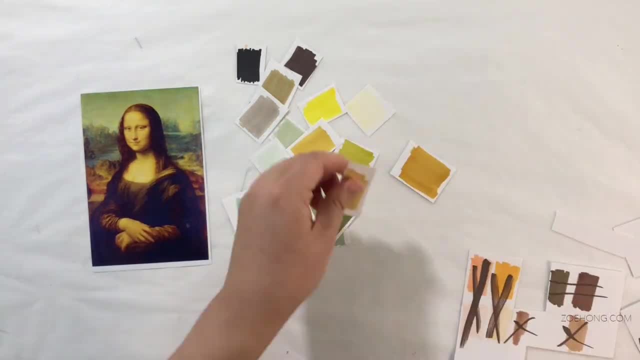 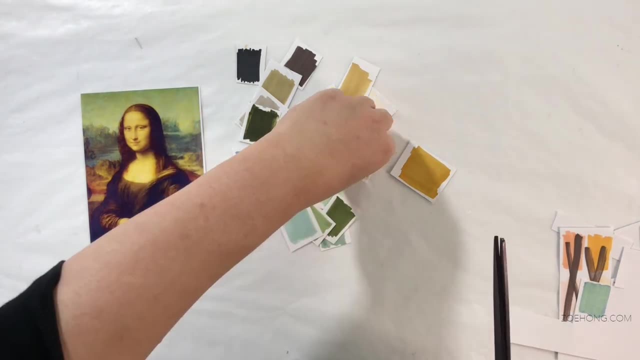 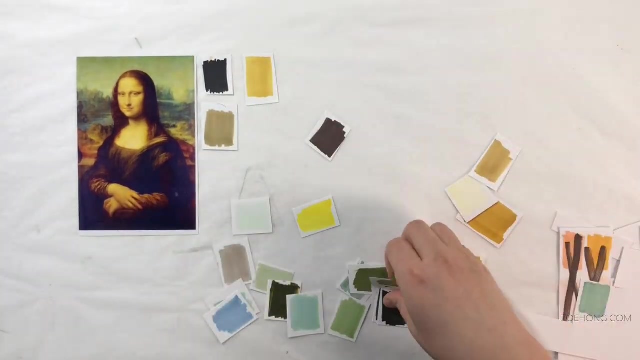 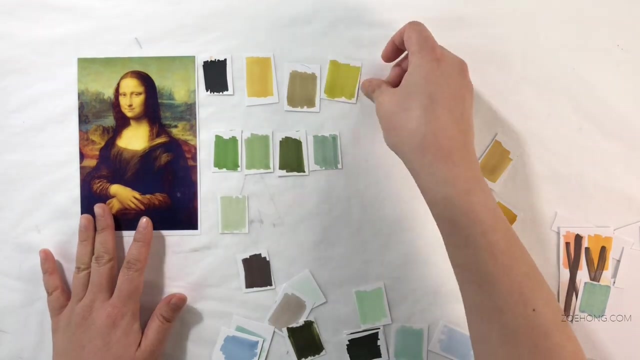 as the complement And the red and the green complementary color scheme can actually be a rich, deep burgundy, Soft, grayish green, rounded out with a winter white and a charcoal gray. Okay, And it's not about the bright, the raw color on the color wheel, And some students think that 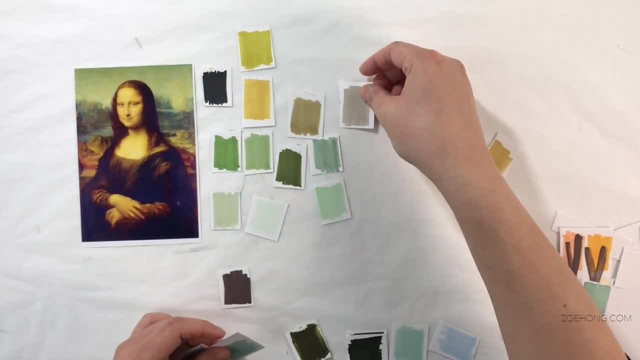 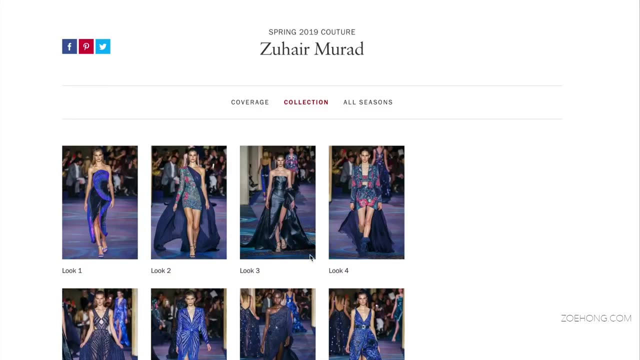 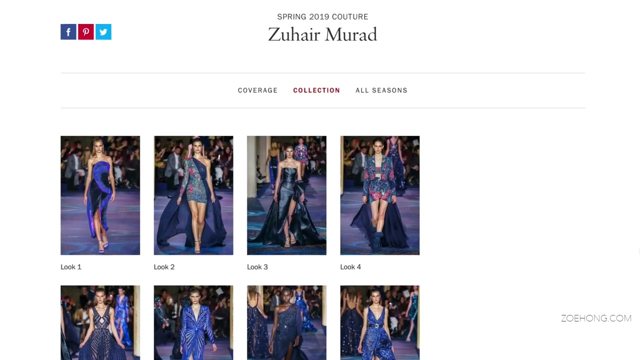 these kind of standard color schemes are too basic to be used in high fashion, but they could not be more wrong. I screen grabbed these from Voguecom. This is the spring 2019 couture collection from Zuhair Murad. Apologies if I pronounce 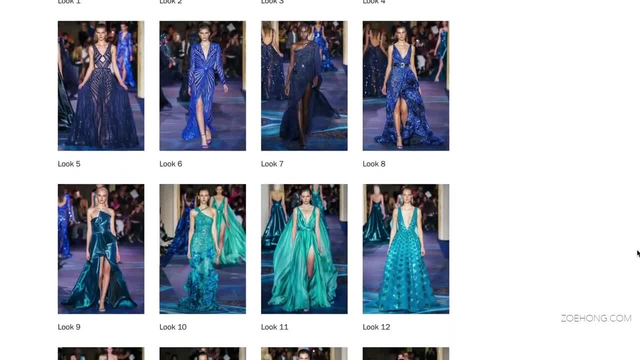 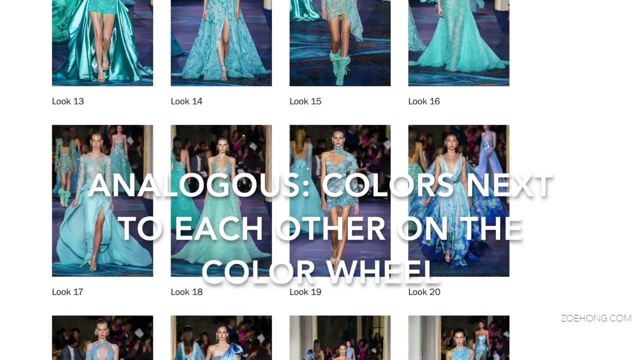 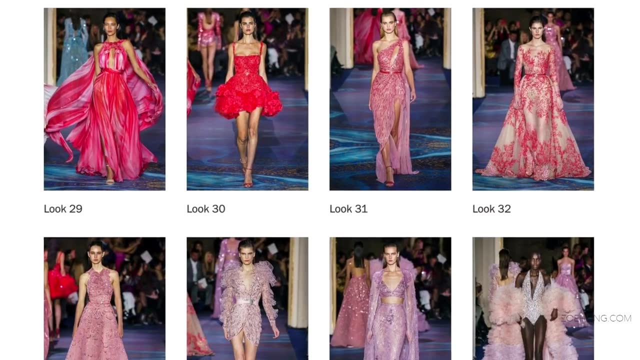 that terribly, And this collection uses a beautiful analogous color scheme, which analogous means neighboring colors on the color wheel, And we have a blue, green, blue, blue, violet, violet, red, violet color scheme And some of the colors are the pastel version. Some of them are the really 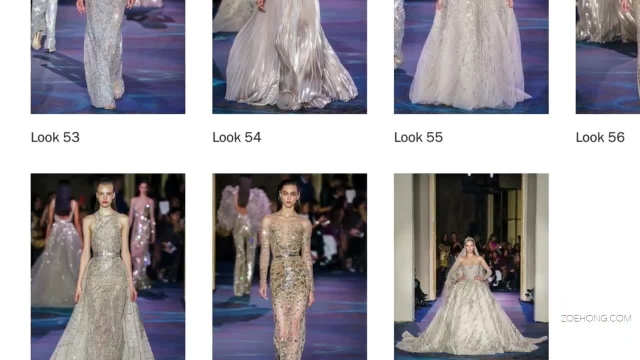 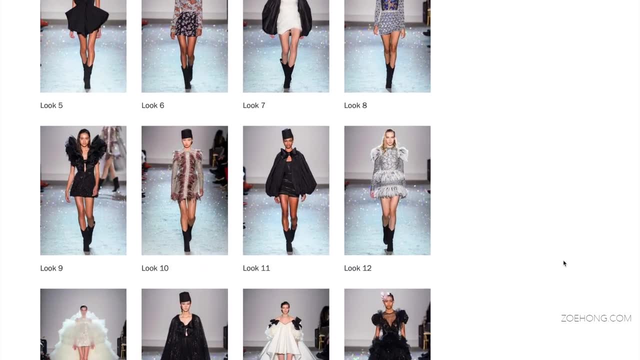 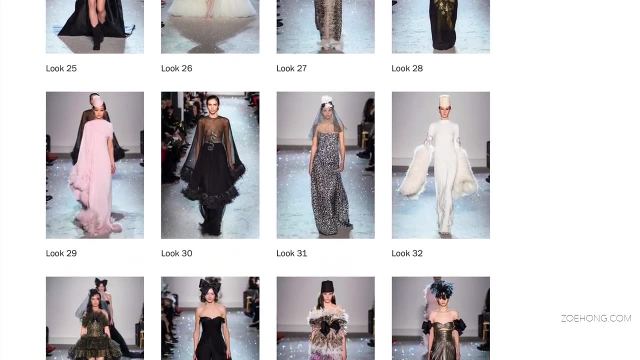 bright versions of the color, but it is an analogous color scheme. Here's Giambattista Vali, and Vali uses another analogous color scheme: a lot of black, a lot of white, for sure, but then also a lot of red and a lot of red violet, which 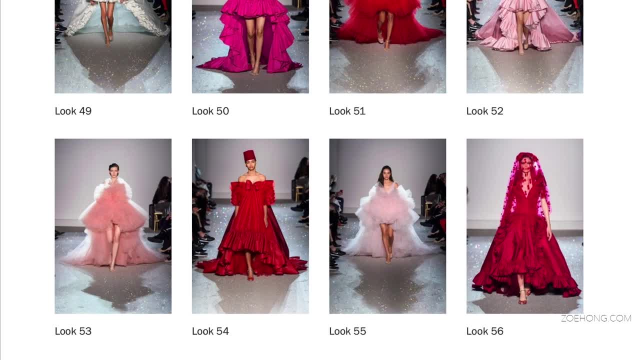 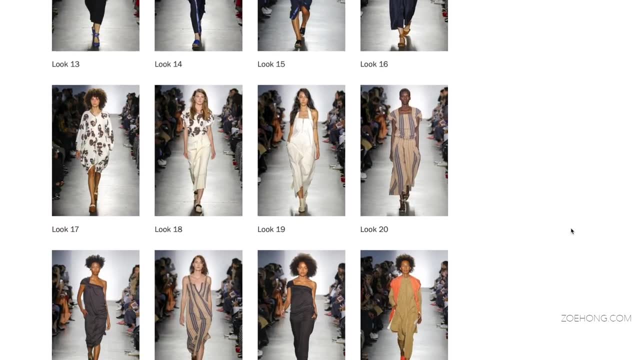 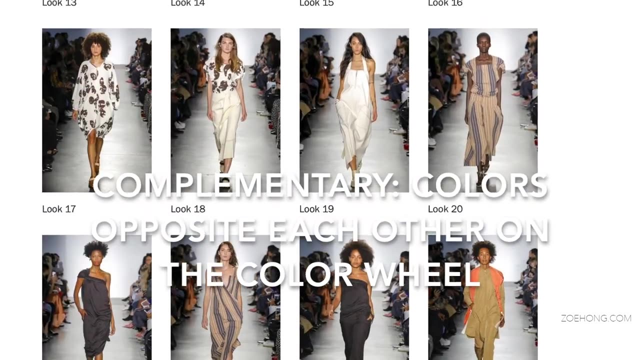 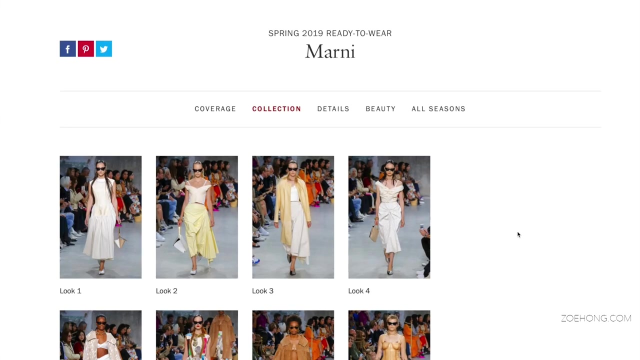 translates to these beautiful bright pinks. Here's Zero Plus Maria Corneal, and this collection showcases a complementary color scheme with a soft blue and some bright oranges and some neutral tones like white and camel. This is Marnie and Marnie. I mean this collection has a lot of colors but the 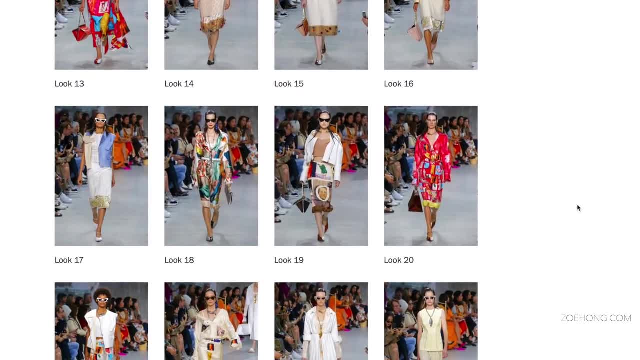 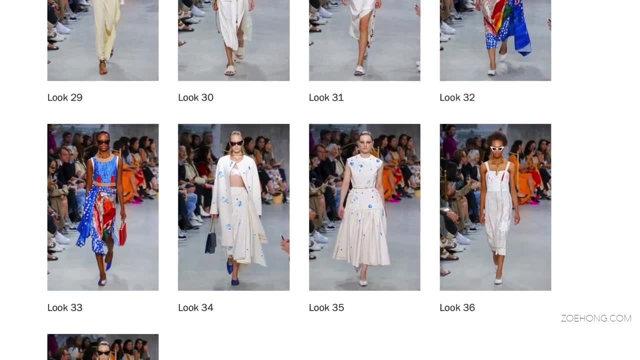 main color scheme of this collection is a little bit different. This is the main color scheme of this collection is a little bit different, but the main colors are your primary triad- red, yellow and blue- and you know they're in the prints. there are little bits of other colors but the 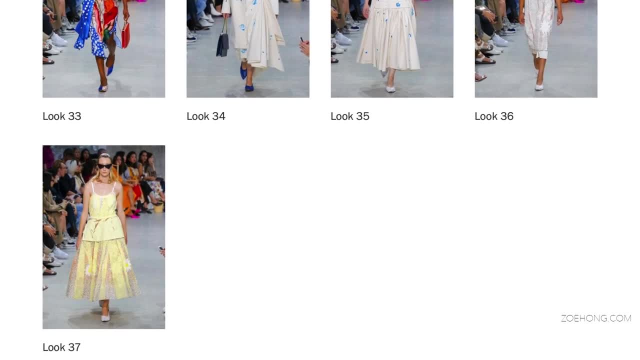 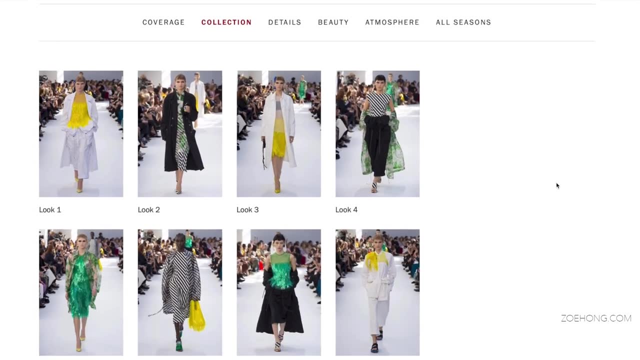 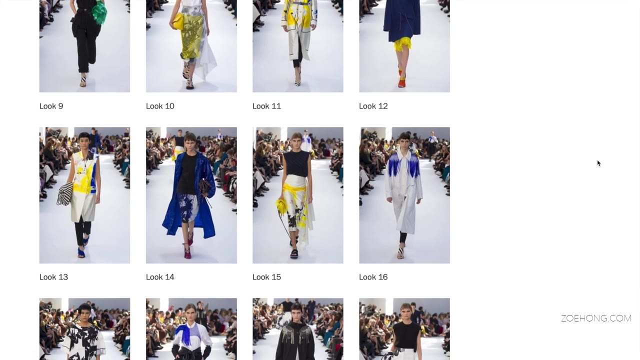 dominant colors are red, yellow, blue and tons of white. Here's Dries Van Noten spring 2019, ready to wear, and this beautiful analogous color scheme is yellow, green, blue, orange, and then rounded out with a little bit of yellow, and then rounded out with a lot of white and a lot of black, and in this case, 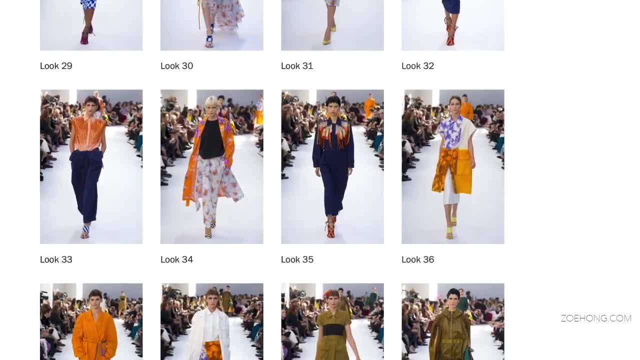 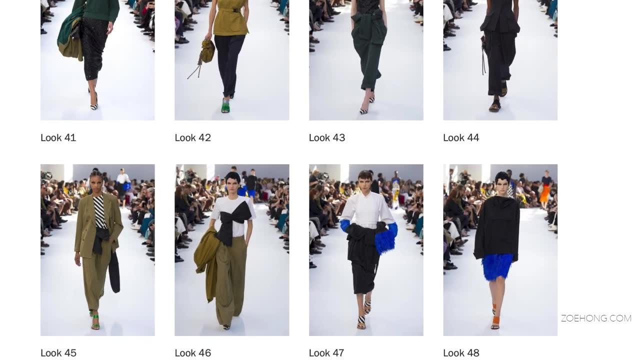 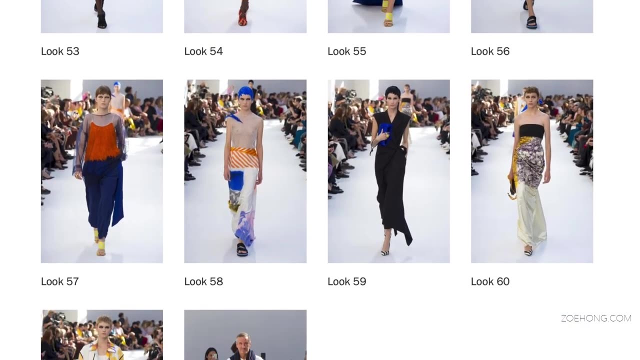 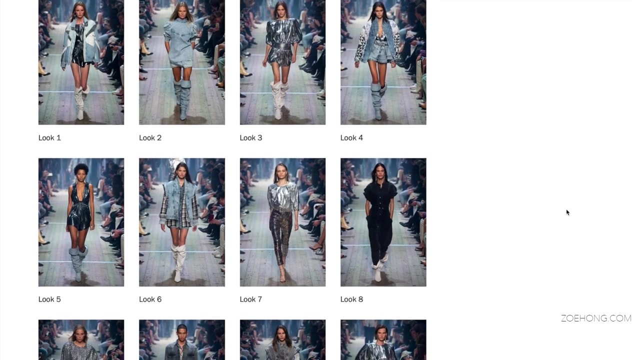 he's using the really rich, raw, saturated versions of these colors, but also with some bits of navy, a, an extra-neutral, some olive green, gay. but it's a very bright, colorful spring collection. And here's Isabel Marant, who is using a complementary color scheme in a very muted, soft, subtle way. you've got red, orange and blue green. 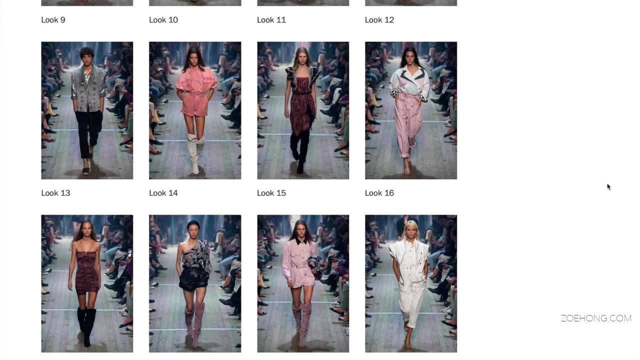 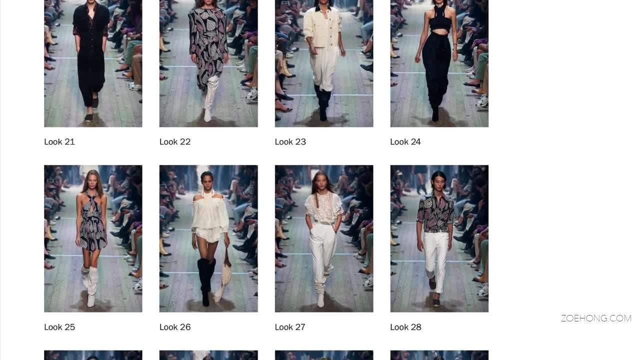 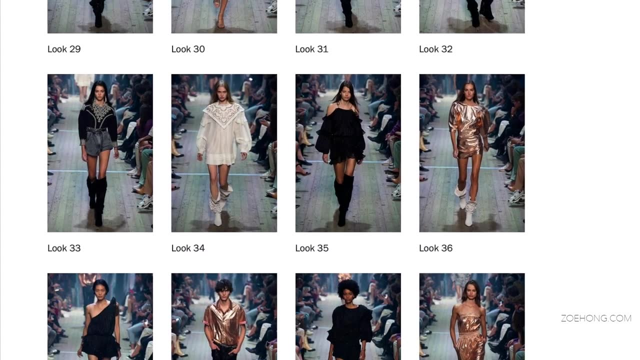 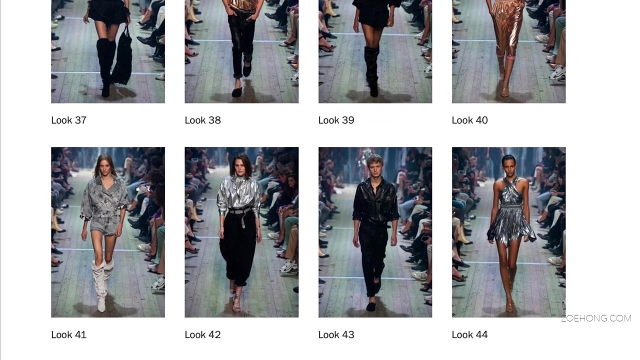 and the blue green has been muted a lot, and it has a lot. it's bait is barely a tinted blue and then a lot of muted red orange, melany tones with white and black and the metallic version of red orange to round it out. so yeah, a lot of big time designers showing at the main fashion weeks. 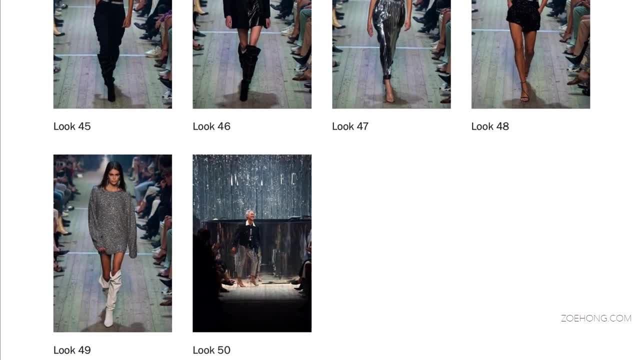 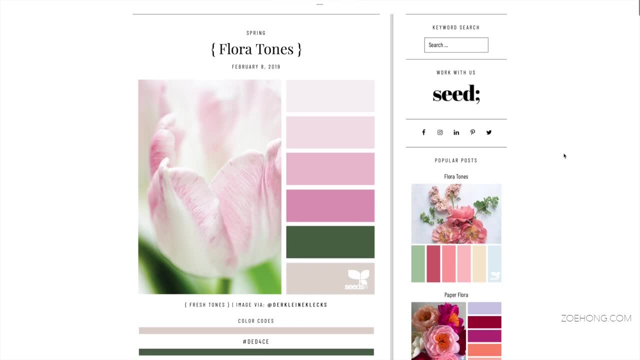 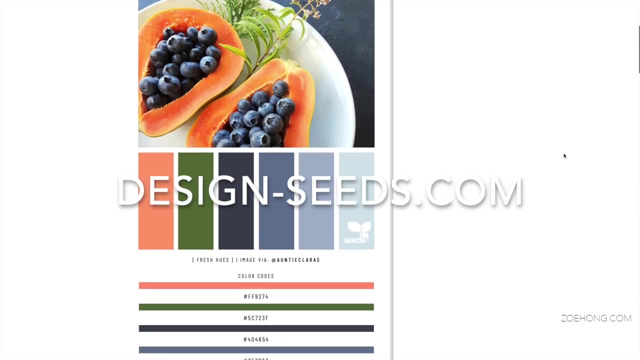 are using these academic color schemes as a jump point for them, and so, hey, if it's good enough for them, should be good enough for you too. another method is to check out websites that put together color stories, like designseedscom, and there are actually a lot of websites that do. 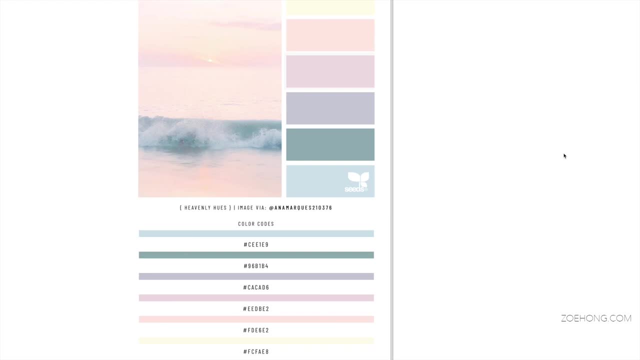 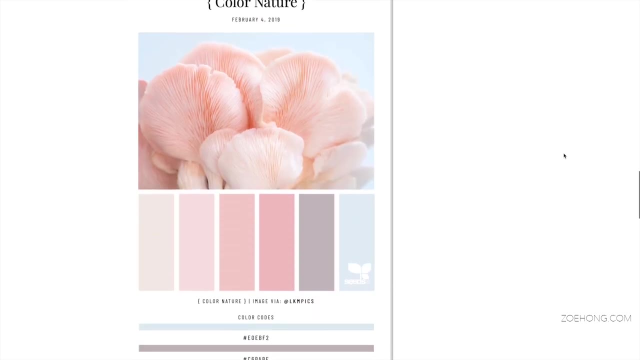 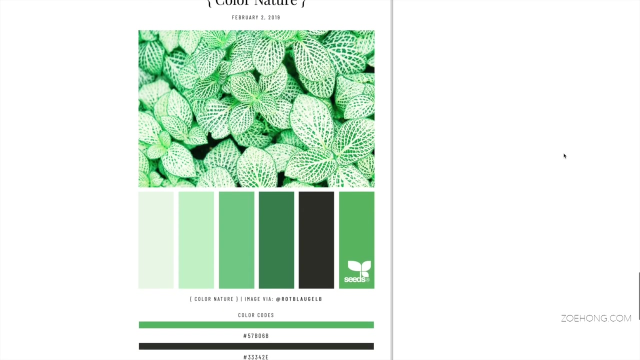 similar things and these websites. they're not built for one particular industry. you could take these color stories and apply them to home decor, apply them to an illustration, apply them to a fashion collection, and a lot of these also follow many of the kind of standard you know: complementary, analogous, split. 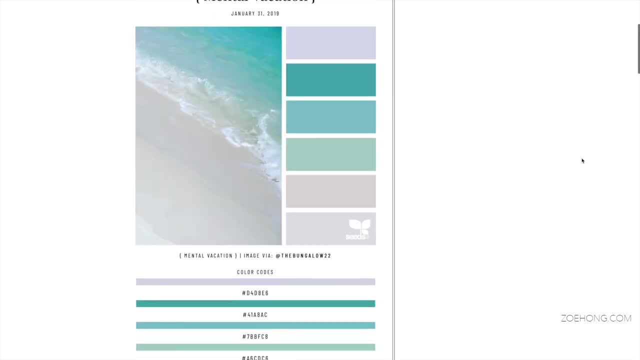 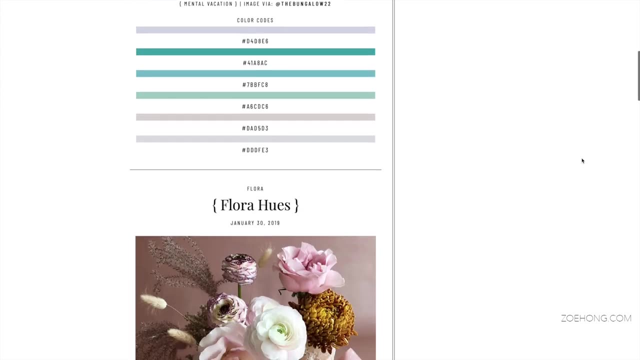 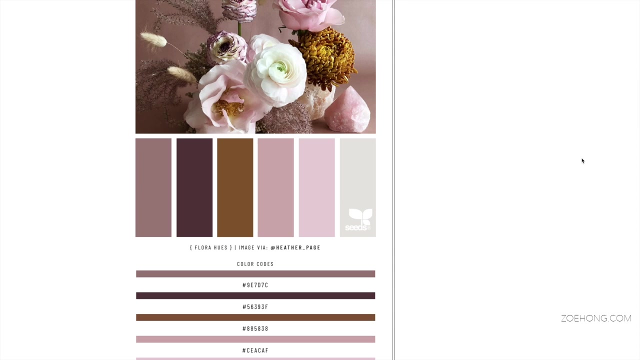 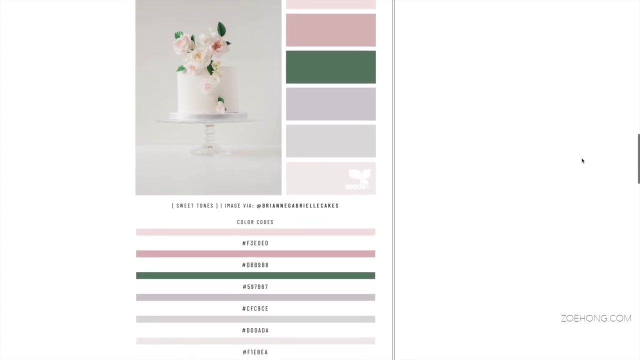 com triad kind of color stories. here's an analogous color story with blue, greens and blues and violets. here is a complementary color scheme using very muted gold and violet, yellow and purple, but muted. here's another complementary story: red and green, but now it's pink and like duller sager greens. 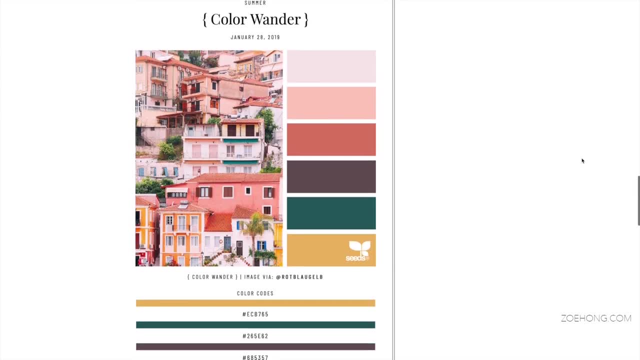 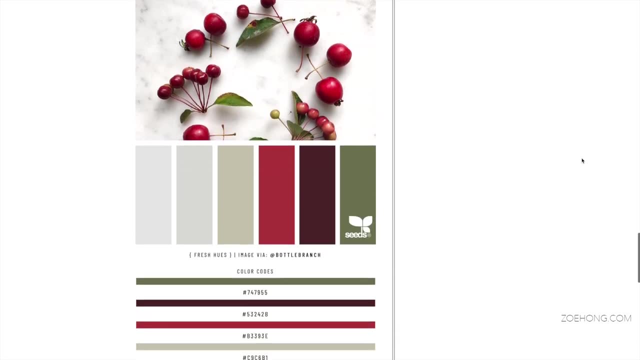 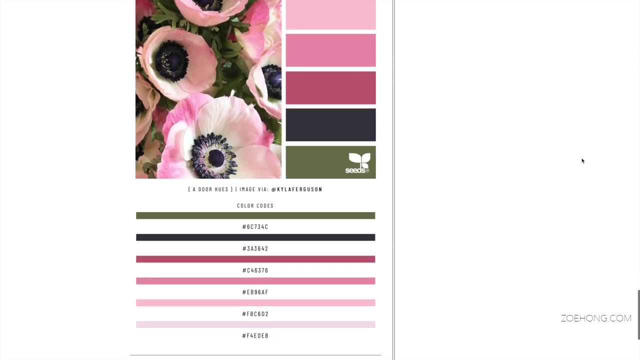 and some neutrals, okay, and so forth and so forth. now let's talk about some of the factors to consider when putting together your color story. number one: add a little bit of color to your design, as always, what your customer wears, this is always the number one factor. what's daring and 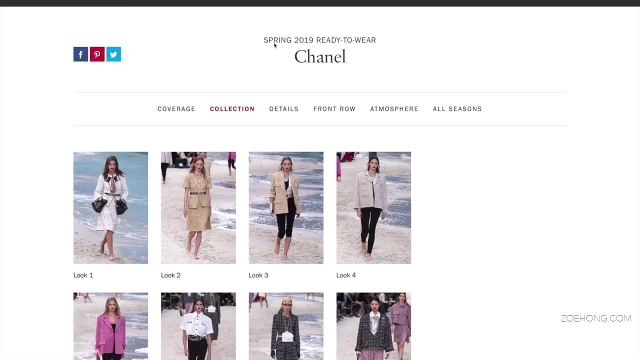 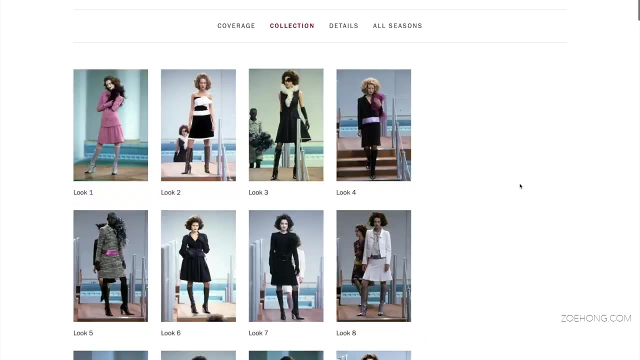 bold for one kind of customer can be quite boring for another. uncle carl would never do a chanel collection without some black and white, without a little black dress, without some tweed. valentino has long been known for valentino red, and so even now, when valentino is no longer there, it's so part. 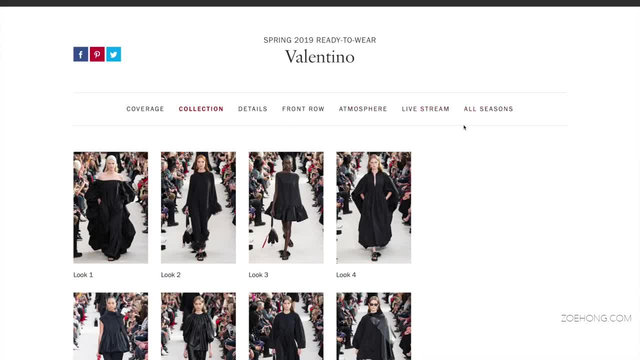 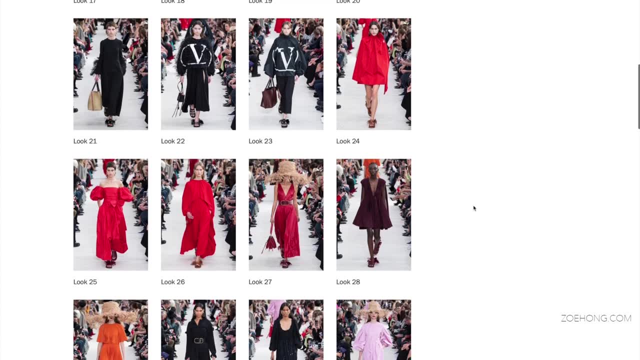 of the heritage, that every designer who works at valentino red has a lot of experience with it, and so it's important to remember that valentino remembers to include the valentino red. even if your company doesn't have a specific signature color, always think about what your customer. 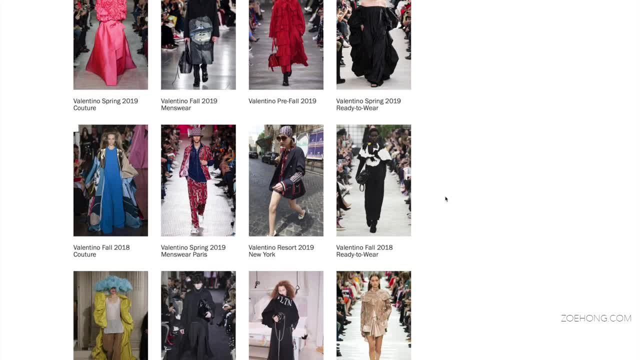 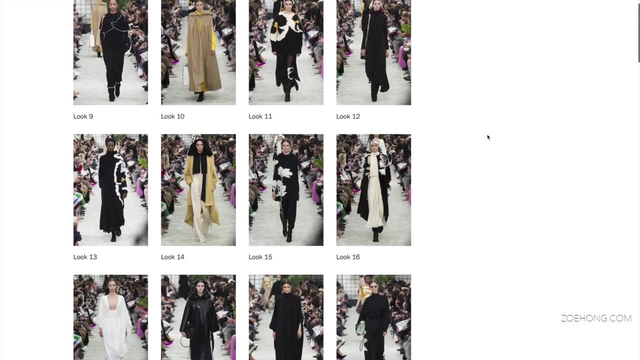 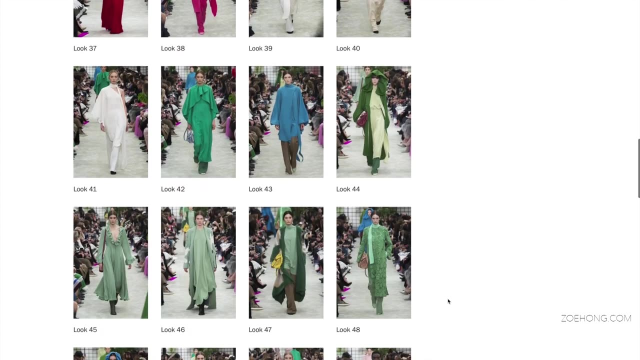 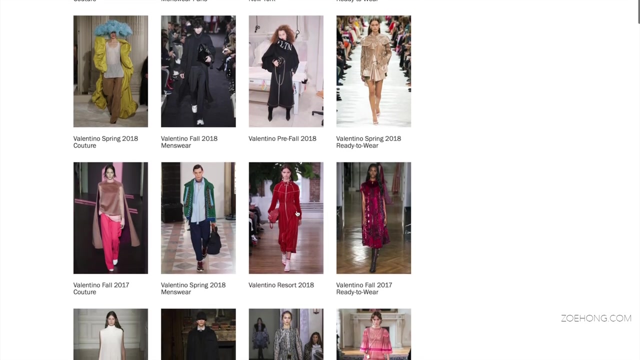 expects from you, your brand number two: what season are you designing for? you want something fresh for spring, something rich and warm looking for fall, something chic and nautical for resort, things like that. and, yeah, i highly encourage you to look at the collections of designers you admire. 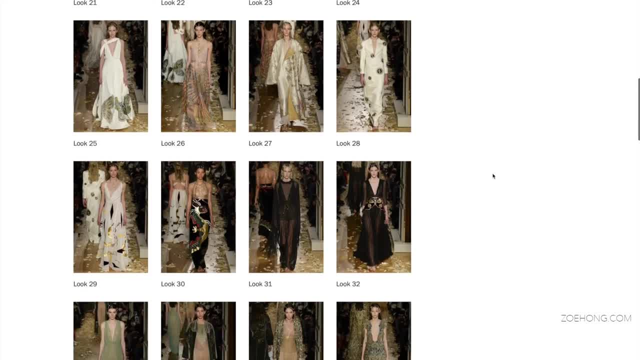 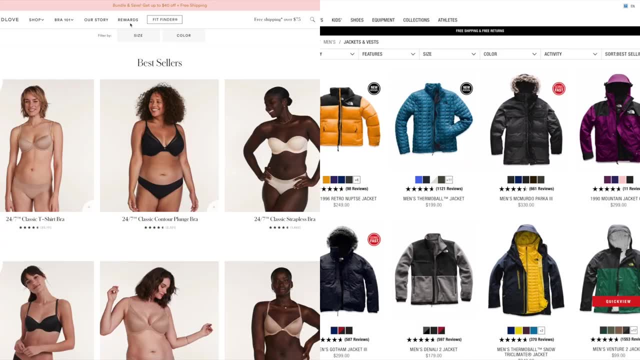 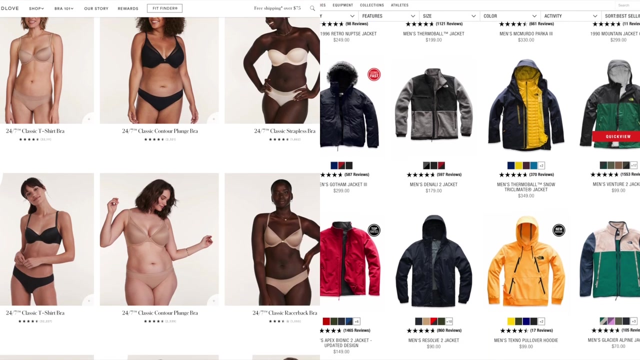 designers who kind of have a similar style as you and see how they approach color stories. three: another factor you have to consider is what item category you're designing, especially now where a lot of these single item category companies are really flourishing. okay, and you know, do you wear the same colors, lingerie, as you do, parkas? okay, obviously, there's going to. 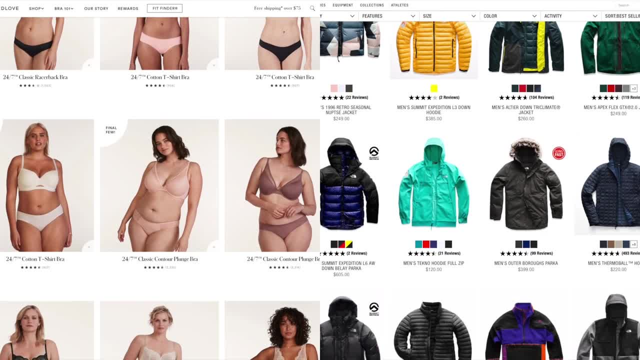 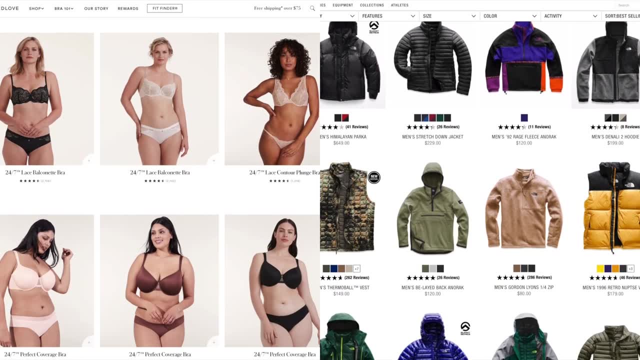 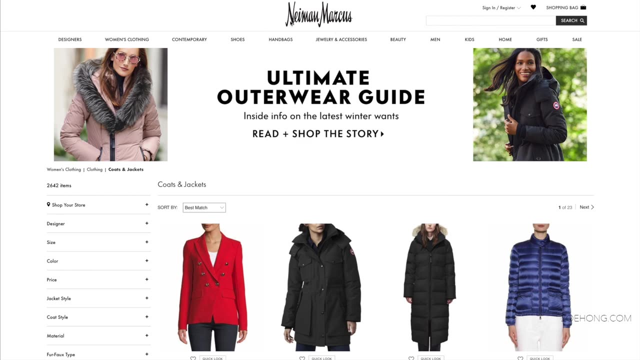 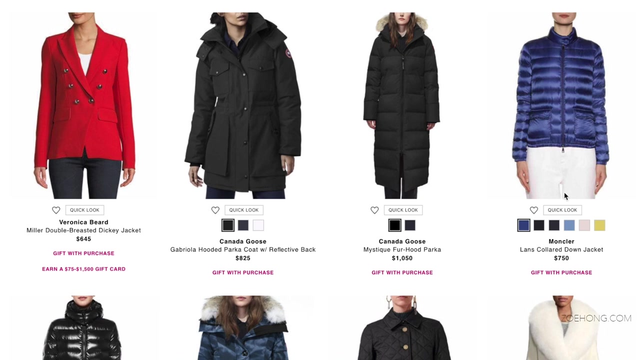 be some overlap, but for the most part they run different color stories. you know, orange is definitely one of those colors where you have to kind of be careful about the placement. number. four: another factor is: in the industry you must offer every style in multiple colors. it is a complete waste of money spent on developing the sample and perfecting the 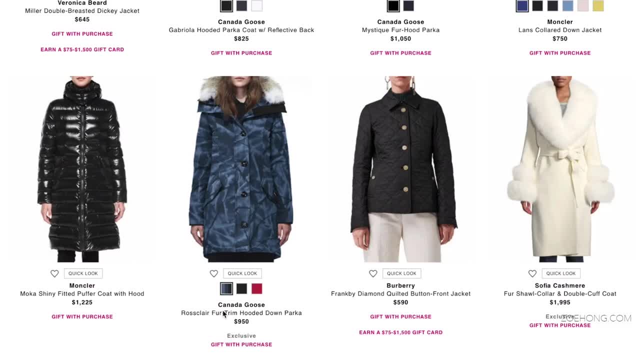 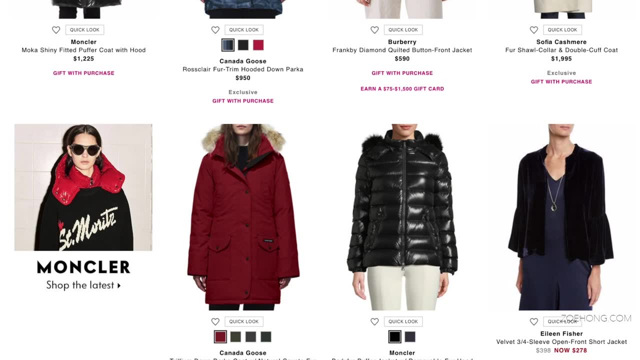 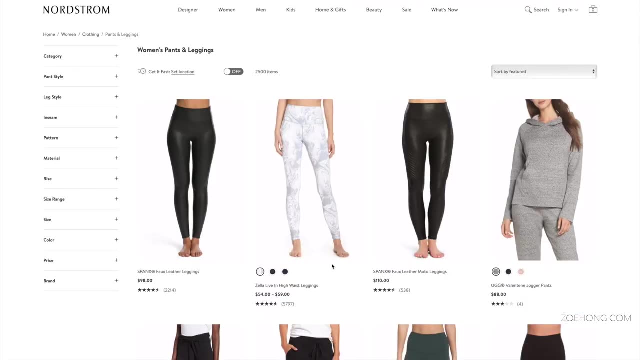 fit to offer something in one color and lose out on all the potential sales from people who might just not love that specific color that you offer it in. okay, even wedding gowns come in different shades of white. okay, the only exception, i think, is black. like black is so, uh, such a big seller. 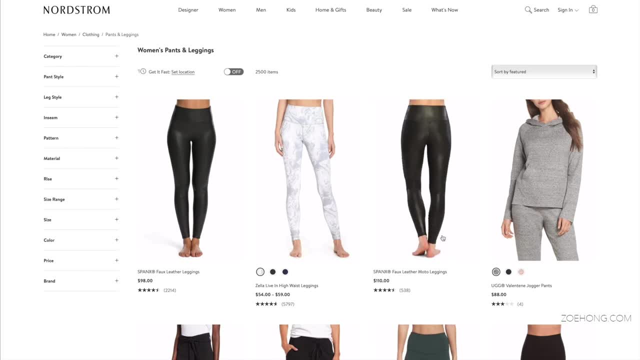 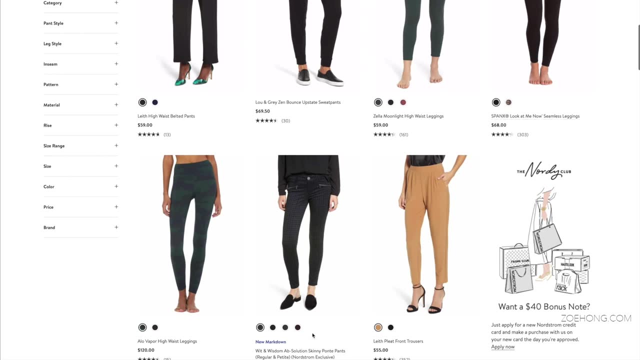 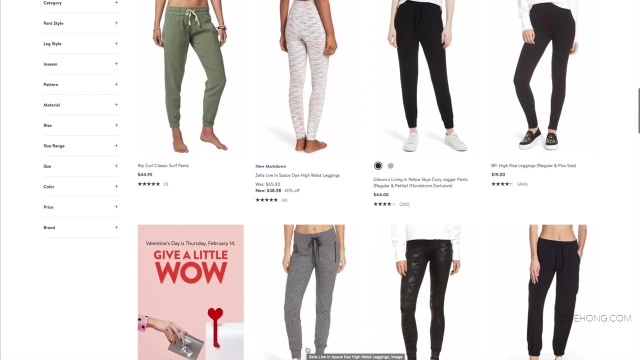 you can get away with offering just black in a style- and you may think you know, zoe, i go to nordstrom and i see lots of stuff selling in one color. yeah, just because a designer offers three colors doesn't mean that the store is going to order all the colors like. 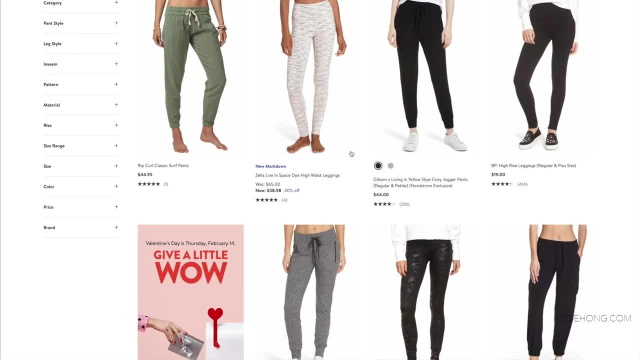 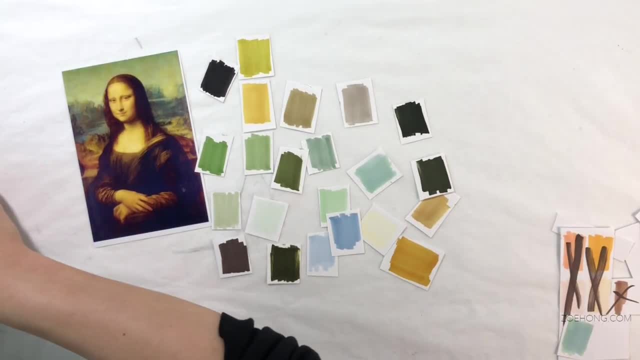 nordstrom may order the pink one that you sell, and then a different boutique might order the blue version of that style. number four: use a bit of color psychology to convey your mood and message. you do not have to be a designer to be a designer. you have to be a designer and you have to be a 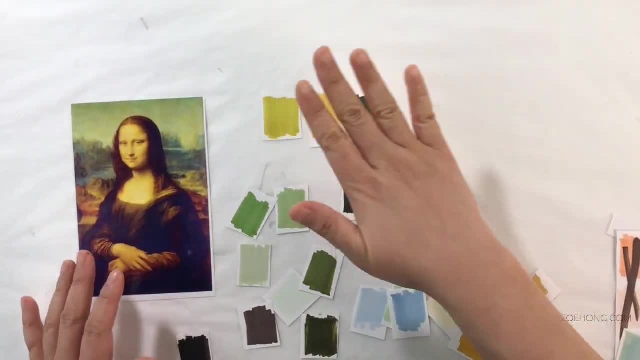 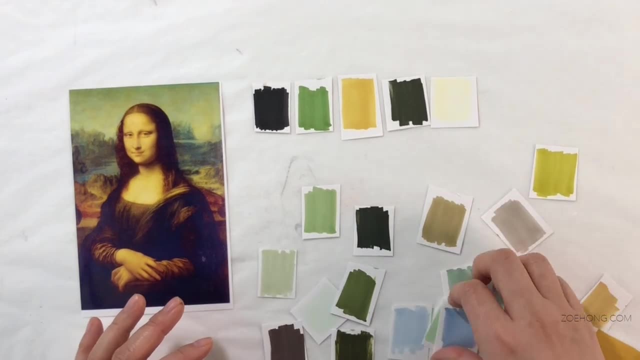 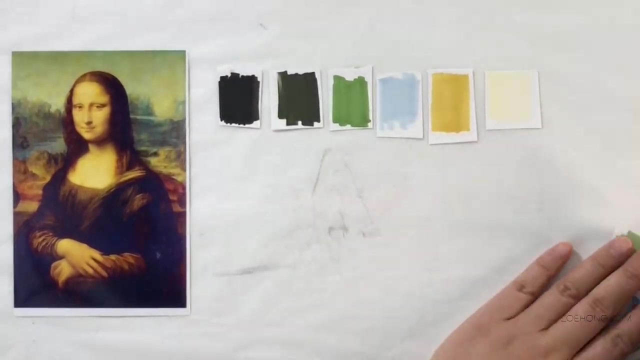 designer, you do not need to overthink this. okay, bright yellows convey sunshine and happiness, and pale lilac is pretty and light and soft, and using a lot of dull grays and browns can showcase a rather somber mood. so when you're putting your color stories together, think about the mood you're. 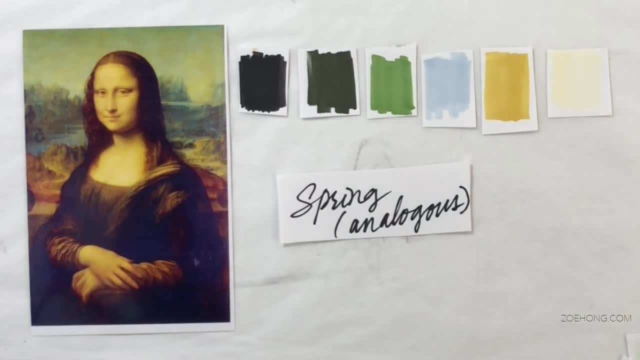 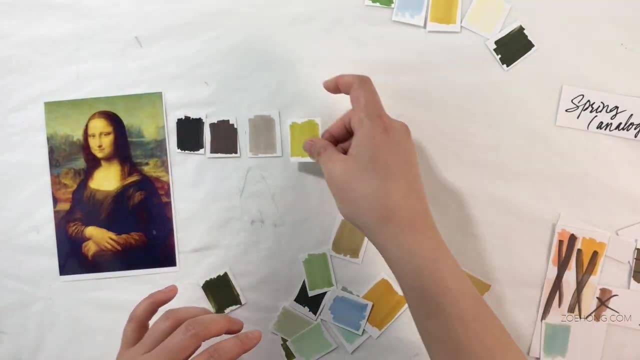 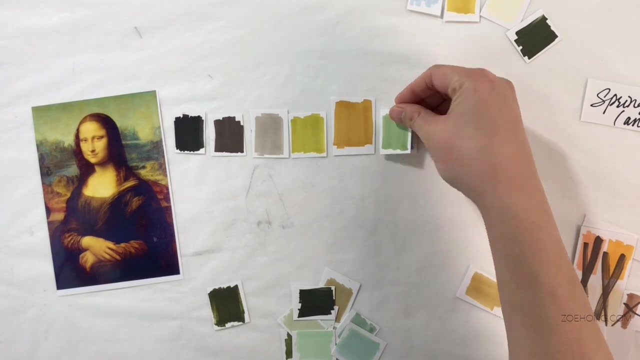 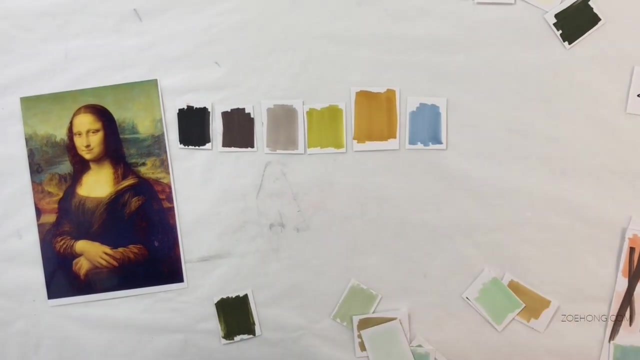 trying to convey and what colors help illustrate that mood. number six, and this is going to be the most important one in terms of fashion business, is: you will often choose colors and fabrics at the same time, simply because of sourcing logistics. you will sometimes be limited by what's available at your price point and whether or not you can hit the minimums. 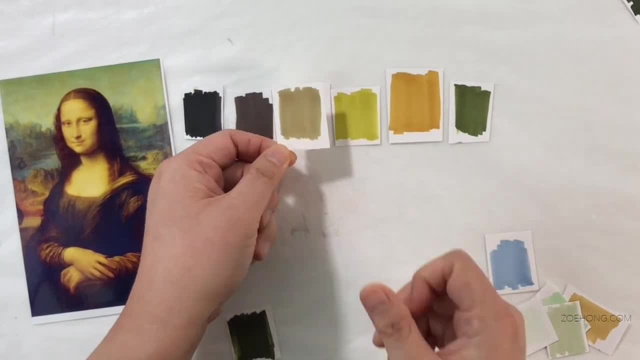 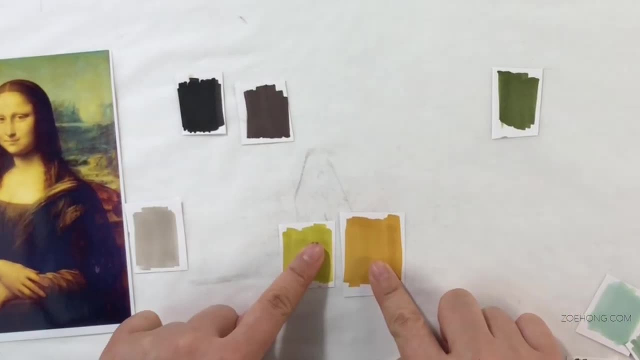 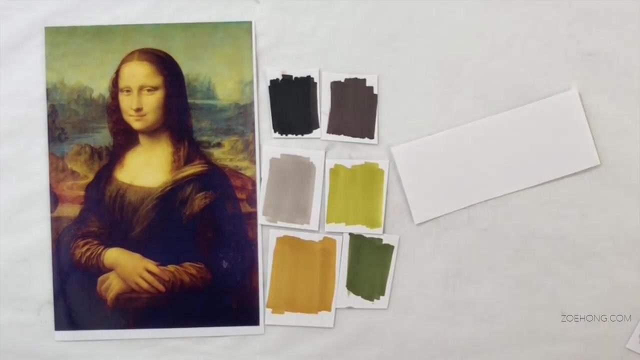 of the fabric wholesaler. if you can meet the minimums and you have the time to do it, you can get a fabric custom dyed. okay. anyways, always keep in mind that colors will look a little bit different depending on the texture as well. okay, so merging all these factors together, using 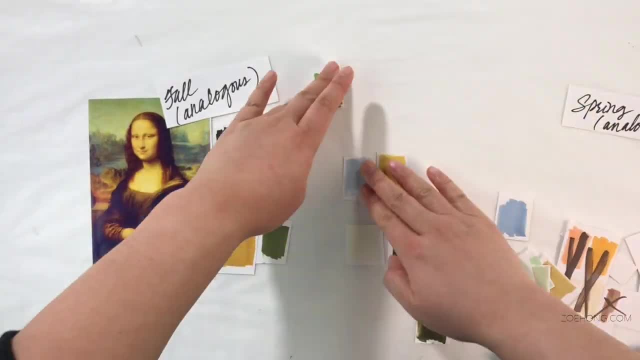 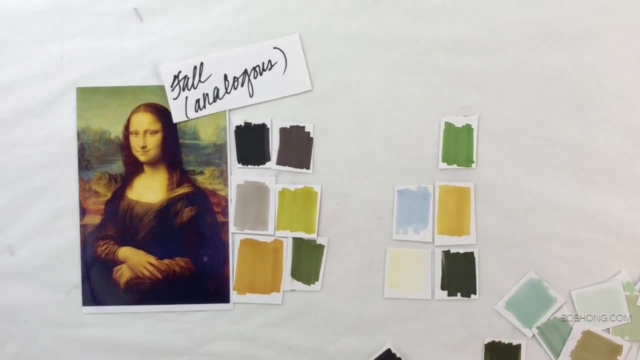 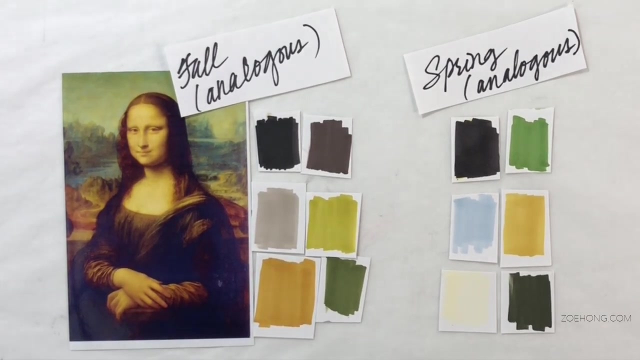 the Mona Lisa sample from earlier. we've got our customer, we've got our season, which is fall. we're doing blouses and pants and coats. okay, I want to pick a couple of blouse fabrics, a couple of pant fabrics and maybe coating or maybe two. I have my approximate color story that I want here and you can, you know, tape. 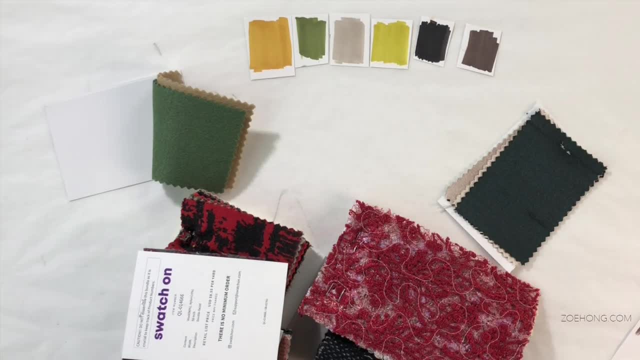 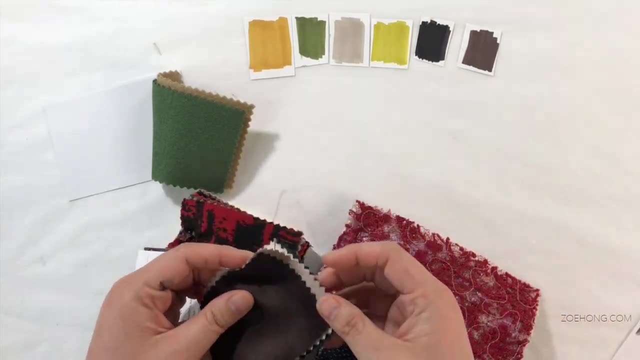 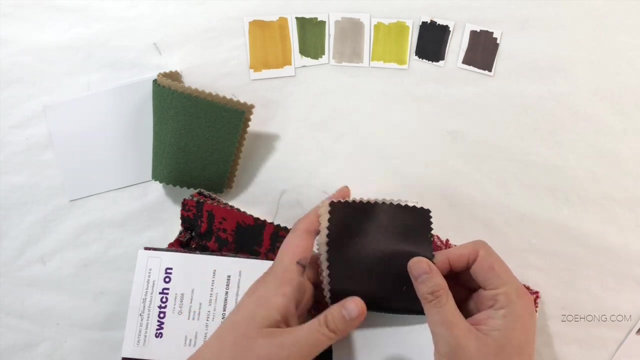 these chips onto a piece of paper and take them to your fabric person and you start looking for your fabrics and you see what's available, because I don't know about you, but it's so much easier and cheaper to go with what's available in stock before you start asking for dye to match things. 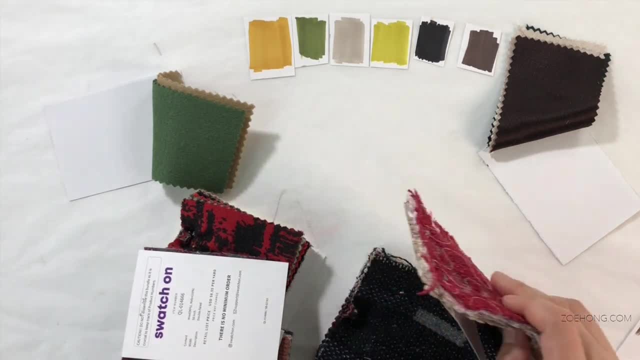 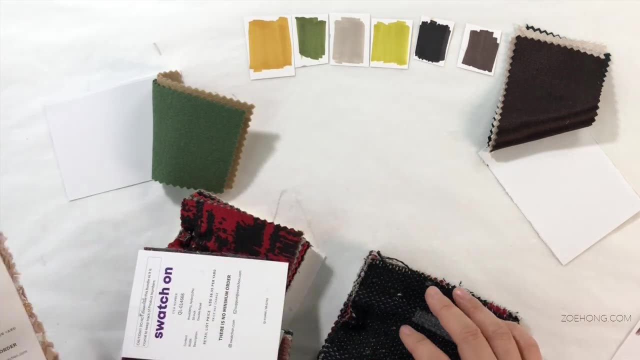 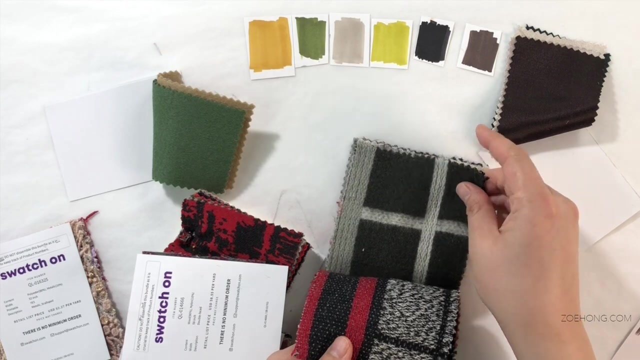 So you start looking at what's available, what's cool, what basically follows the color story you have laid out, and you just start building your fabric stories with your color story and some of the colors might change a little bit and you might find out that you like the new color story. 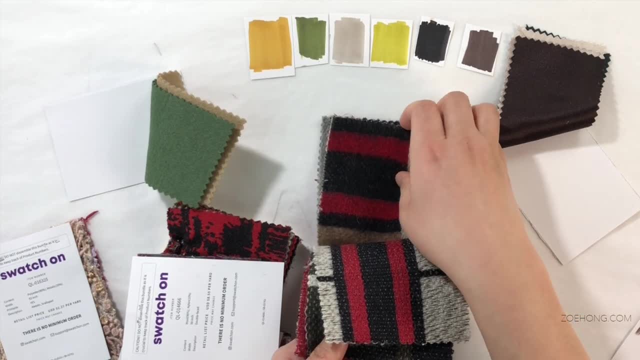 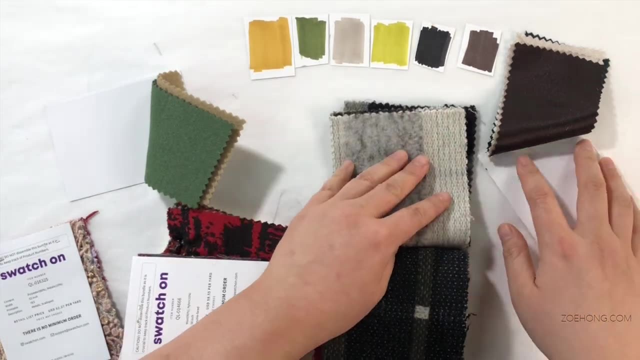 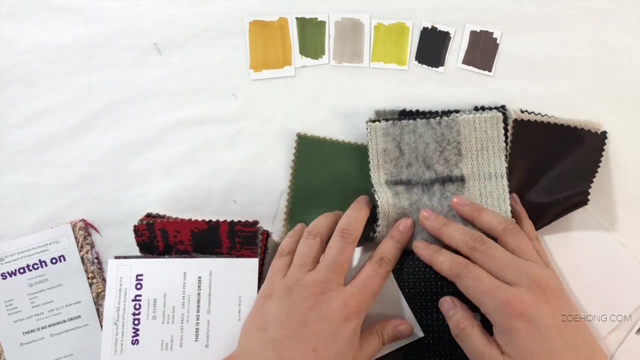 better. Now let's answer the most frequently asked question about color: How many colors should be in one color, How many colors should be in one collection? In the industry, in business- and this is important because fashion is the intersection of creativity and commerce- The number of colors you have in a collection is all about the 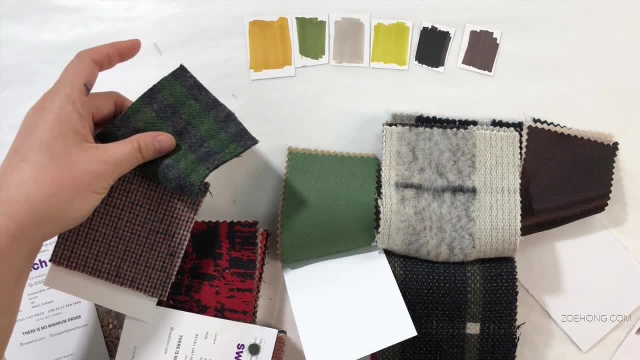 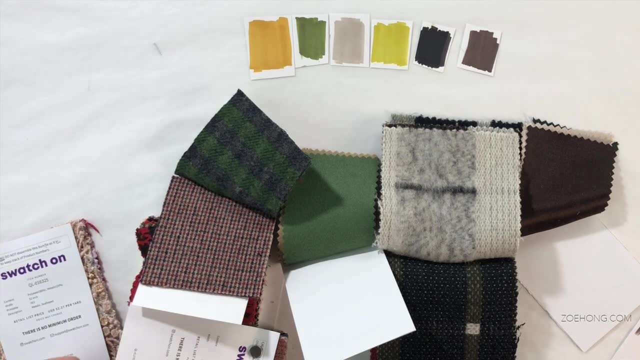 fabrics you have in a collection, which is dictated by the size of your company, the size of your collection and what order minimums you can fulfill. You can learn more about fabrics in the fabrics playlist, which I'll link in the description box, And I already know that there's so many of you. 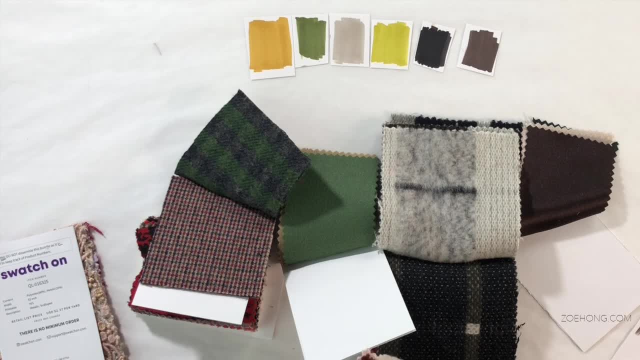 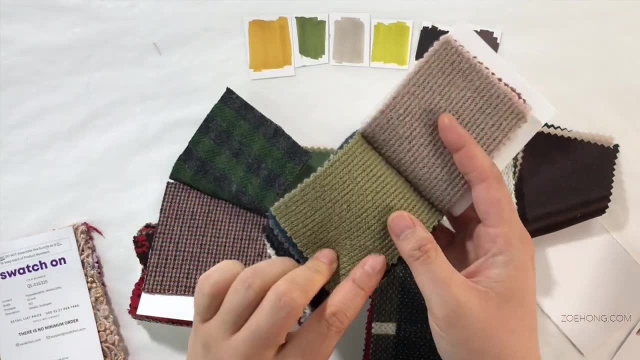 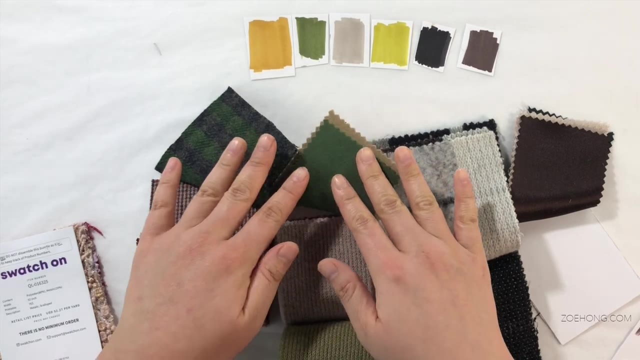 watching right now. who hate this answer? You want me to tell you a number. Only have six colors for every collection, everybody. Yeah, that's not how things work. There's so many different kinds of fashion companies out there and even for all- let's pretend, 100%- of you watching this video. 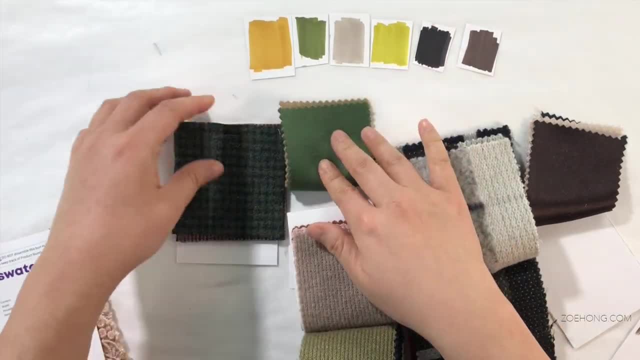 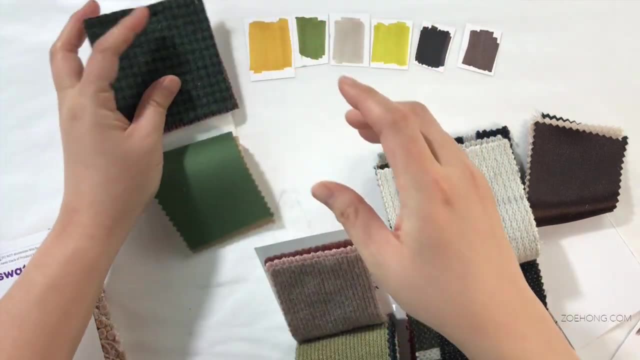 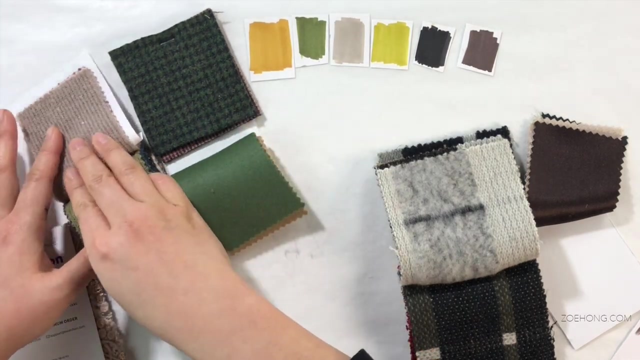 are doing startups. There's so many different kinds of startups So you do have to consider. you know what are the minimums of the places that I'm sourcing. you know how many items categories like: am I doing just bras or am I doing hoodies and jackets? 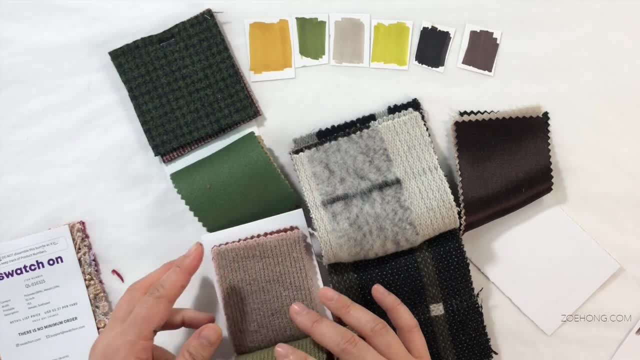 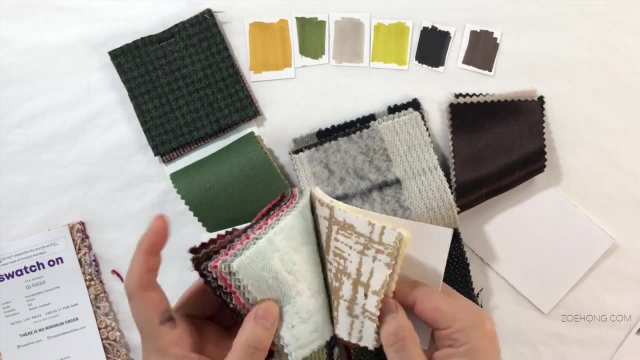 and parkas, or am I? do you know? you have to think about all these factors that I just listed. Sourcing is a headache. It's a big deal, and minimums, especially for startups, is a huge deal. Why do you think I was so excited to introduce you to this? 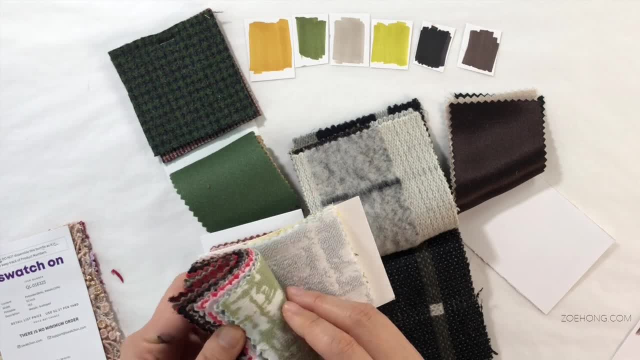 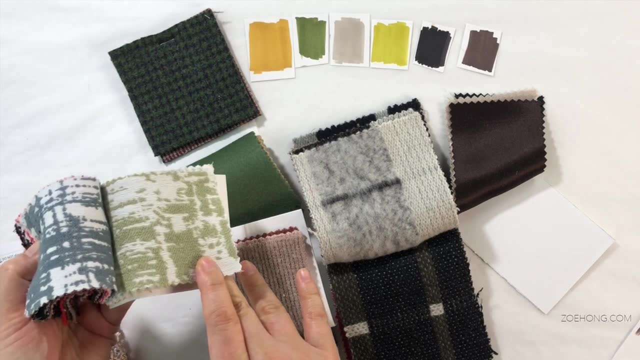 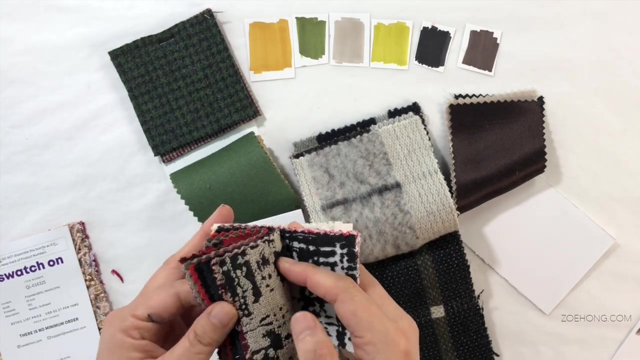 I was so excited to introduce y'all to swatch on and you know I kept talking up really excitedly about how swatch on has no minimums and it's. it's rare. you know there are a ton of companies out there that will do 100 yard minimum, a thousand yard minimum. You know some people. they'll say 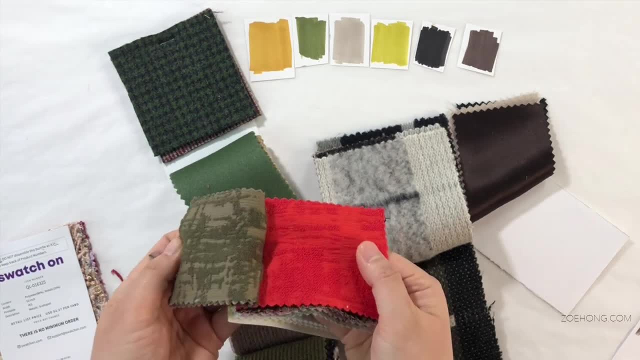 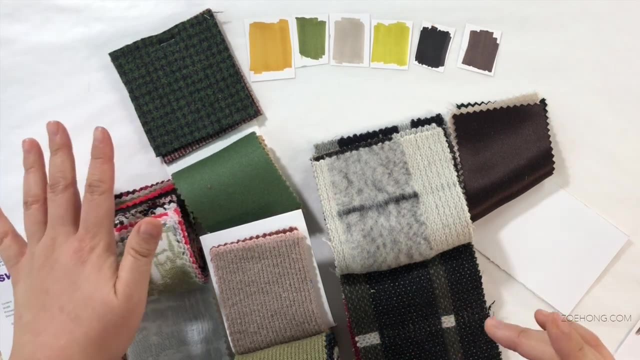 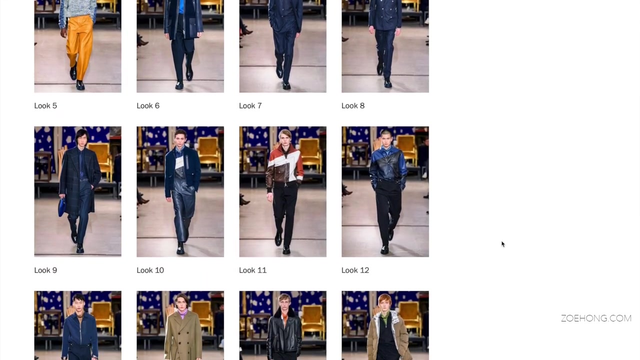 your minimum is one piece, And by one piece they don't mean one yard, they mean one roll And it can be anywhere from 50 to 100 yards in that role. So you have to ask them how many yards are in a piece? And you might think, Zoe, am I going to look amateur and 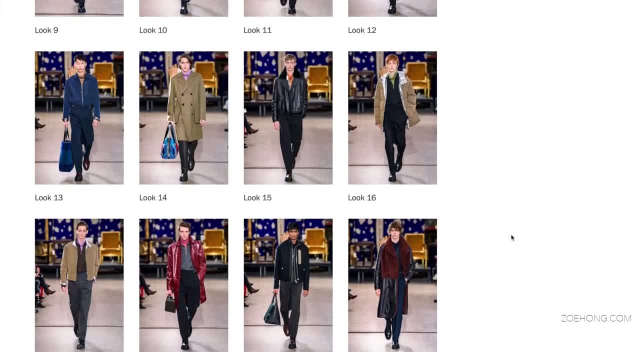 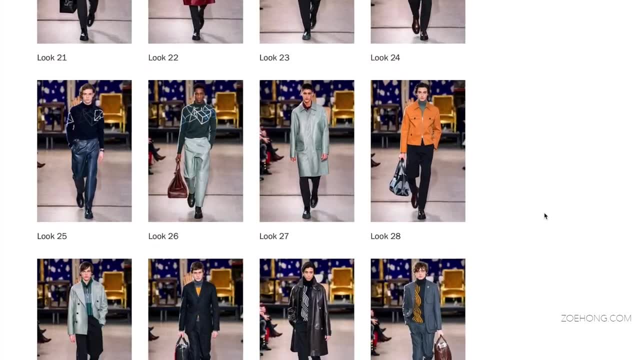 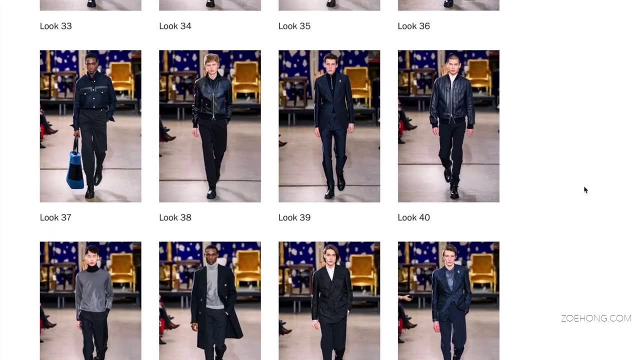 small if I have a narrow color story. No, okay, Even well-known big labels will showcase a narrow color story because it looks good, it looks cohesive and it really communicates their aesthetic message that season This Hermes collection has a great complementary color scheme. 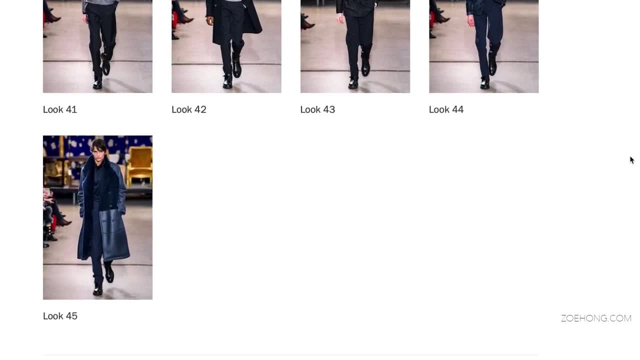 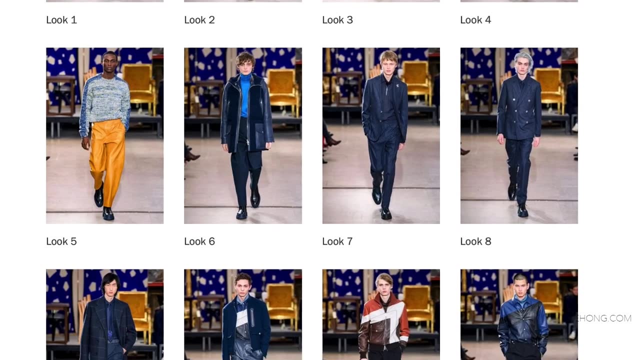 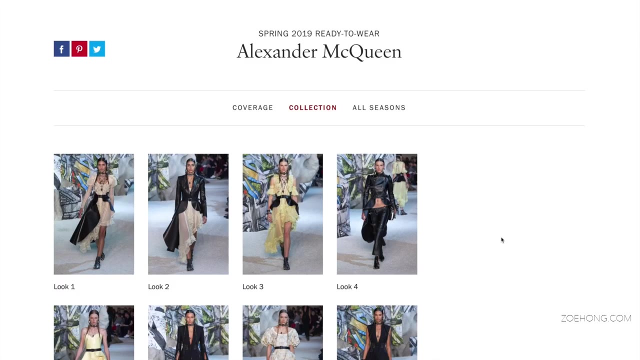 using orange and blue, but not raw orange and blue, but definitely more subtle and sophisticated versions of those colors, which is very much their brand. okay, And they've got these little hits of red and green, which is another complementary pair, And this McQueen collection using a primary 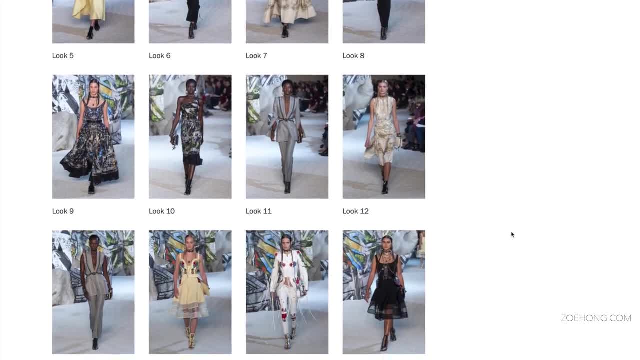 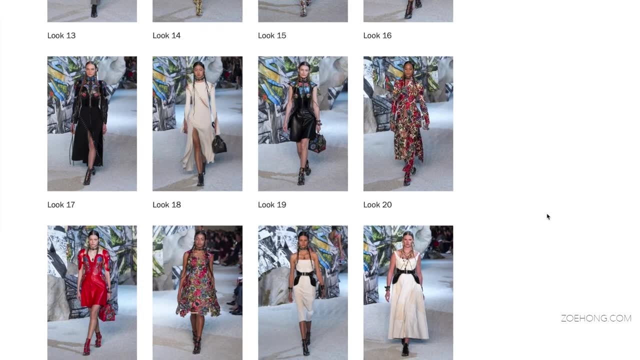 triad with red, yellow and blue. And you know you see some bits of other collections in the prints and embroideries. but red, yellow, blue with black, white and gray, that's their color story. And let's be real, McQueen and Hermes are huge brands, But you know. 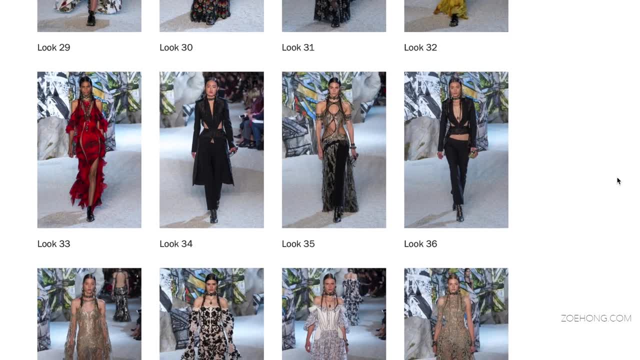 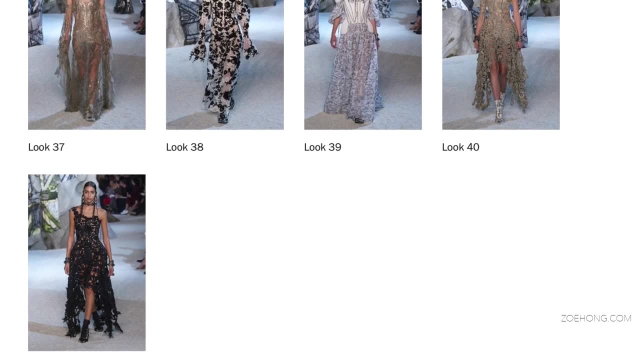 they chose these focused color stories, so if they can make it look good, so can you. And that's it for today on color stories and how to put them together. Please give this video a thumbs up if you learned something new today. Share, subscribe. drop your questions in the. 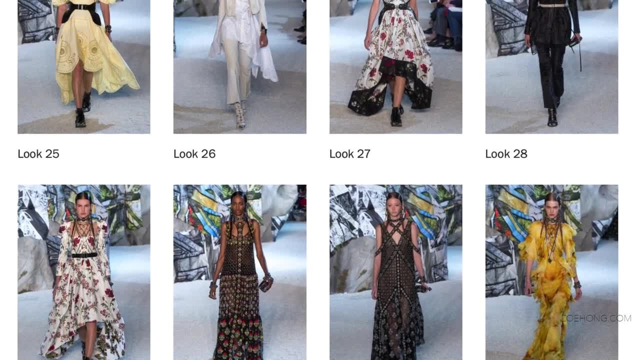 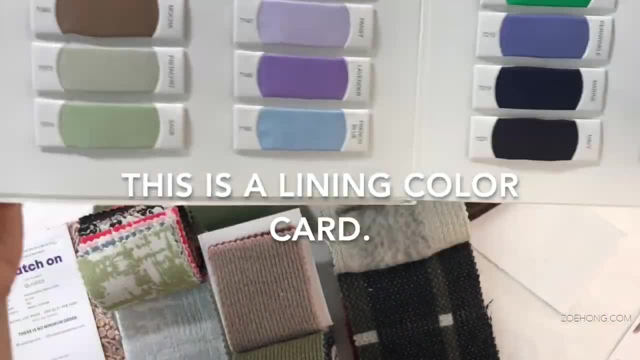 comments section. Check the description box to links to all my shenanigans, links to videos related to this one And I'll see you in the next one. Bye, And you know you may think that putting together color stories is difficult with all the factors. 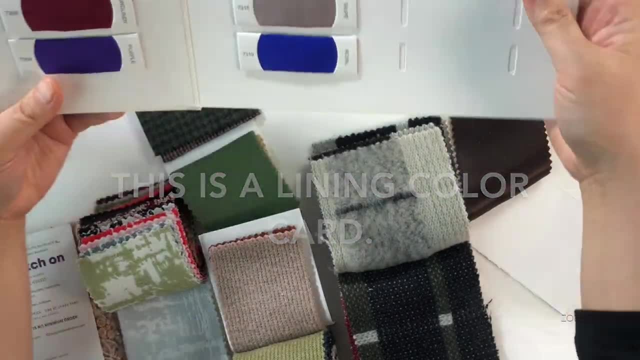 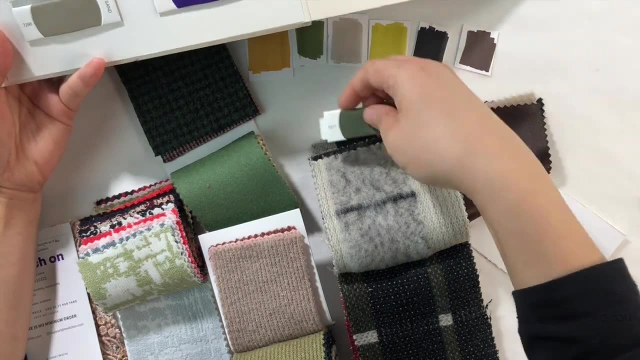 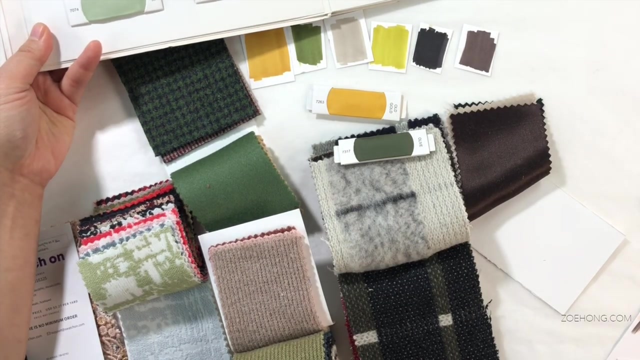 involved, but unless you're new to my channel, you know what I'm going to say: Hashtag, always be practicing. Hashtag, practice, not magic, because we are made of practice, not magic. And hashtag- if your first one sucks, you're right on track. What does that hashtag mean? It means a. 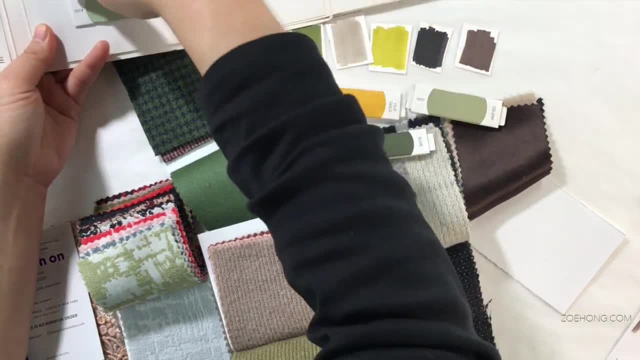 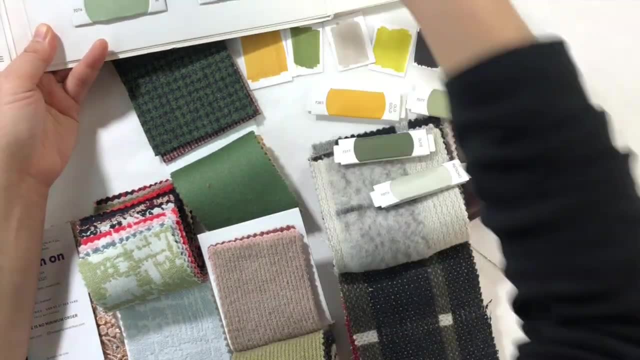 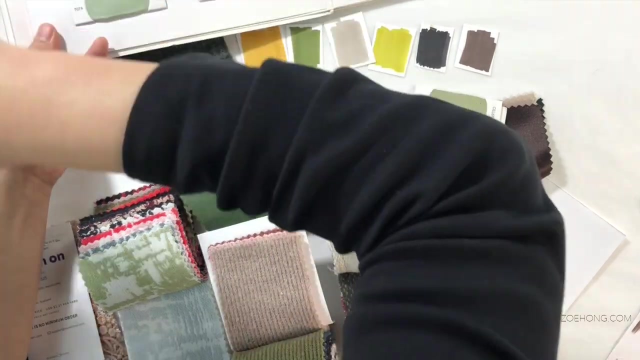 lot of people are so afraid to do something that they never get around to doing even the first one. So if you try it, if you do the first one, you're on track. You've gotten started. Have fun practicing putting together color stories. Go look up some runway shows and lookbooks of your favorite designers. 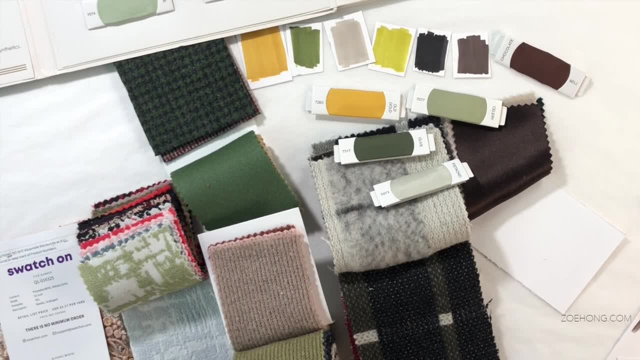 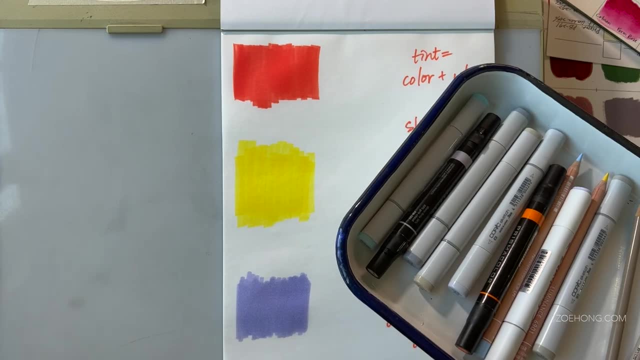 and analyze their color stories And I'll see you in the next video. If you're playing a drinking game or you drink every time, I say undertone, don't do that, because you'll end up in the hospital. Hey, hey, party people. Today we are talking. 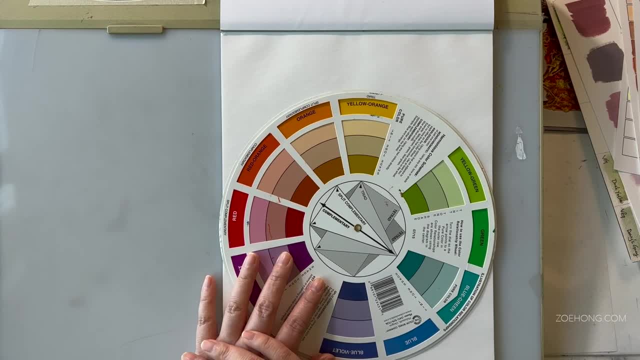 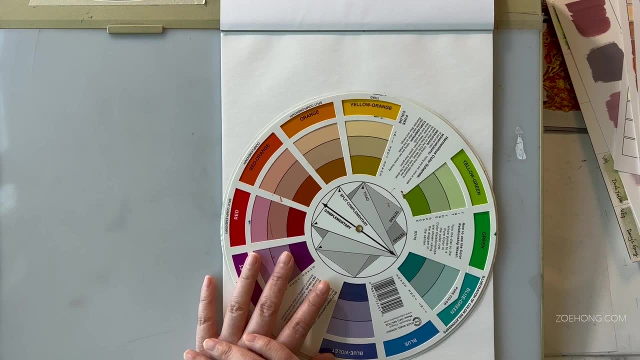 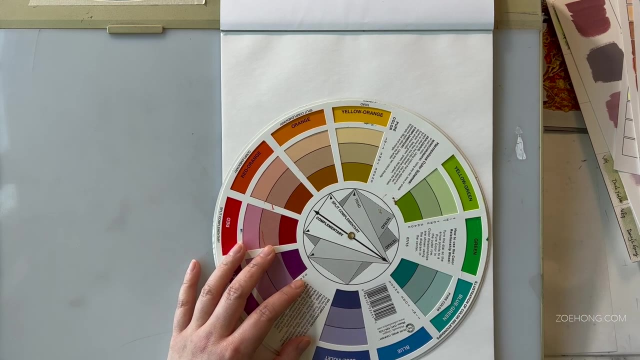 a little bit more color theory. What are undertones and how can we use them? Why do we care? All those good things, All right, This is another color theory for fashion application video, And if you have any more questions about color, drop them in the comments below. Okay, 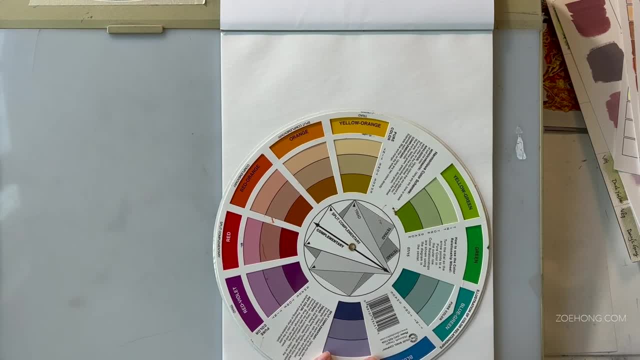 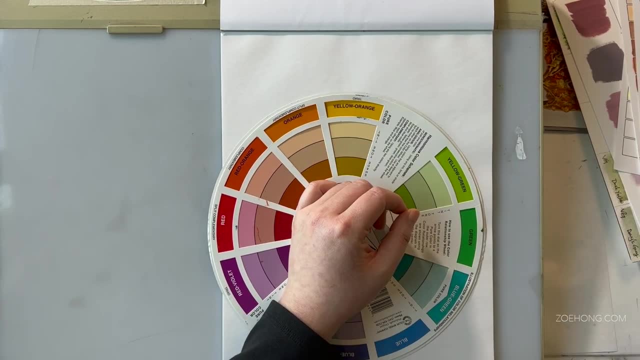 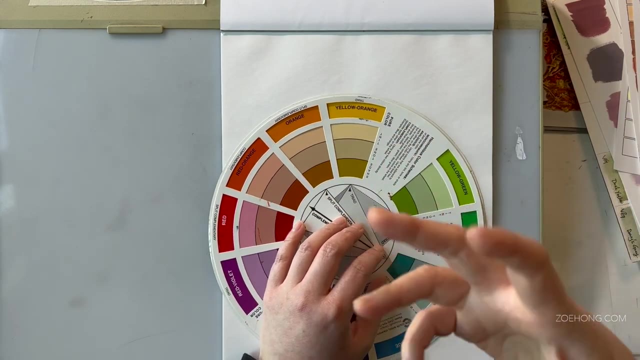 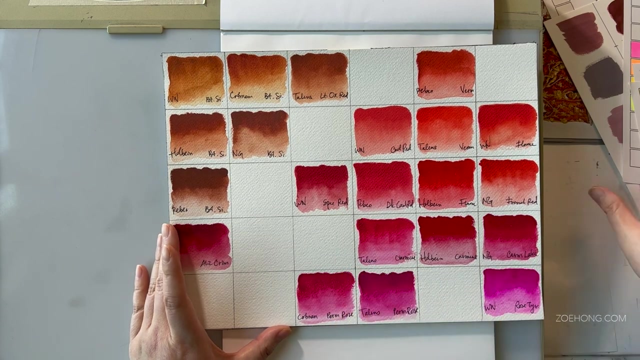 First of all, what is undertone? Undertone is basically when you look at a color and you can tell if a color is Brown or red or orange. Undertone is what kind of orange, What kind of brown, What kind of red. These are color swatches that I keep on me at all times And these are just straight. 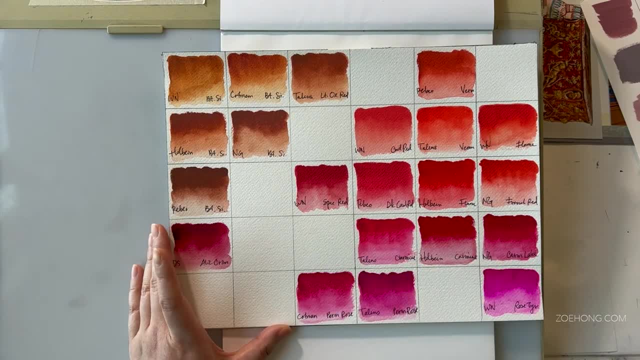 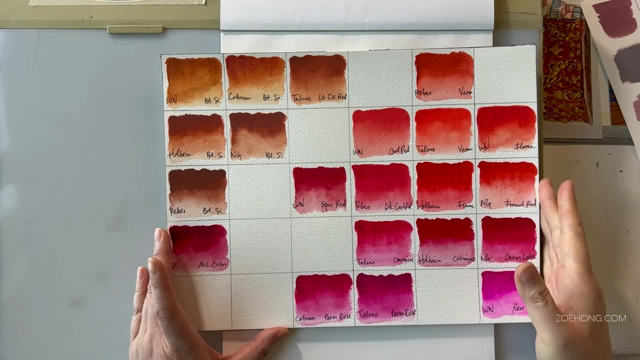 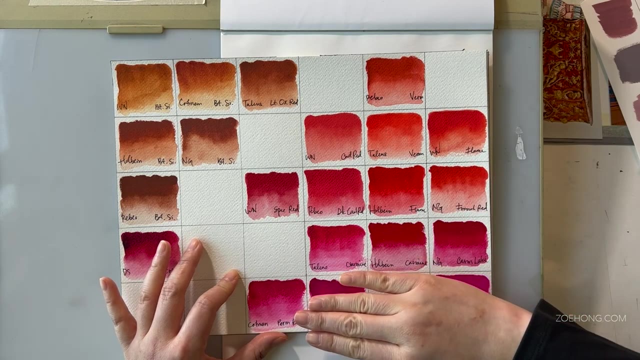 out of the tube colors that I have And you're like, wow, you have a lot of reds and browns. And it's like, yeah, because I just do a lot of product testing, But yeah. So when you look at a red, for example, okay, Maybe not this one, but these can all. 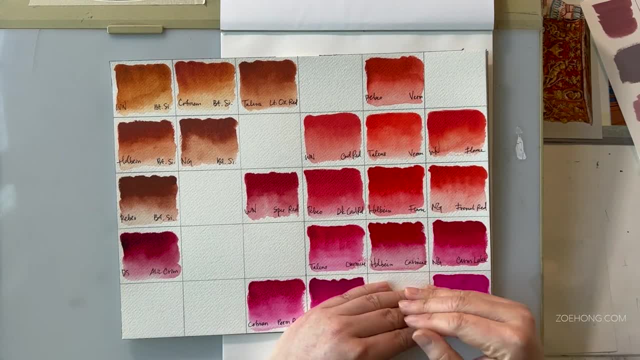 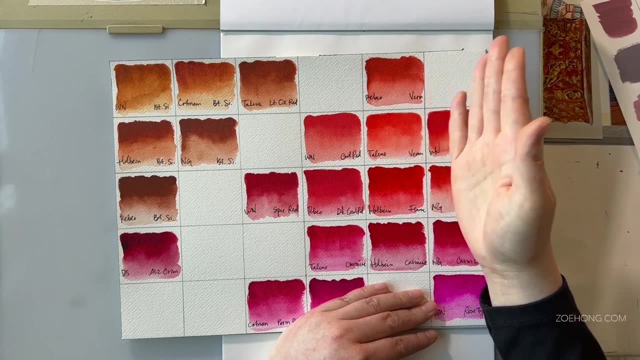 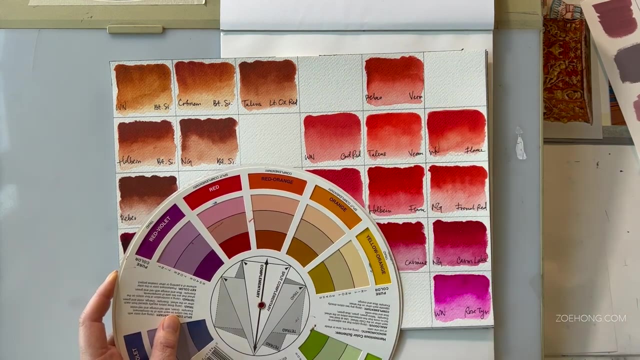 be classified as red. You're looking at a bunch of colors. These are reds, But you also have these warm toned reds up here. They lean a little bit more on the orange. Okay, Where's my color wheel? When you look at the color wheel, these orangier, warmer colors, veer. 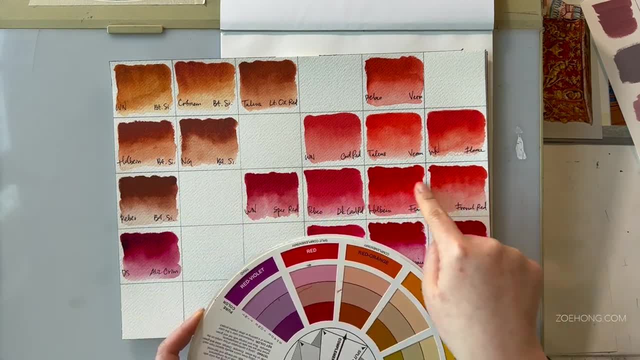 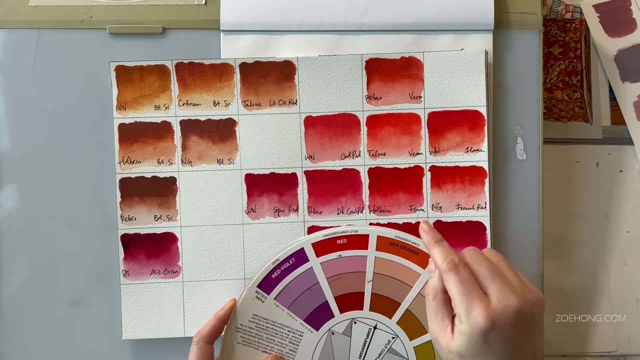 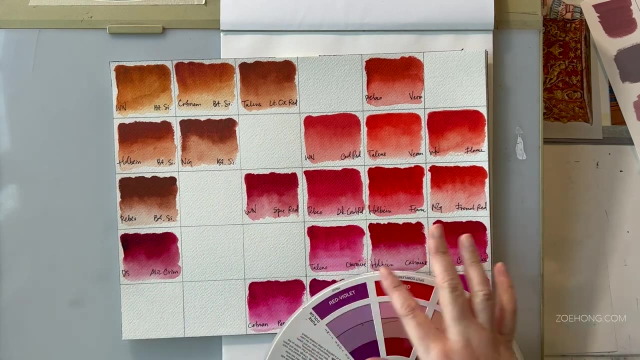 red orange, These middle, this middle row is closest to true red, neutral true red, in particular in here, Not so much here. This is starting to get a little bit dark And then in here we have cooler toned reds that are not quite red violet but tipping red violet. These 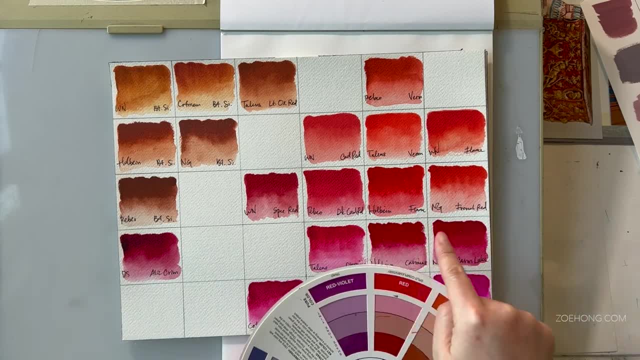 two are in red violet territory. These are more cool toned reds And anyone who has shopped for a red lipstick, you're going to find a lot of cool toned reds And you're going to find a lot of cool one. Those are more like the 2021 colors. These are more like the 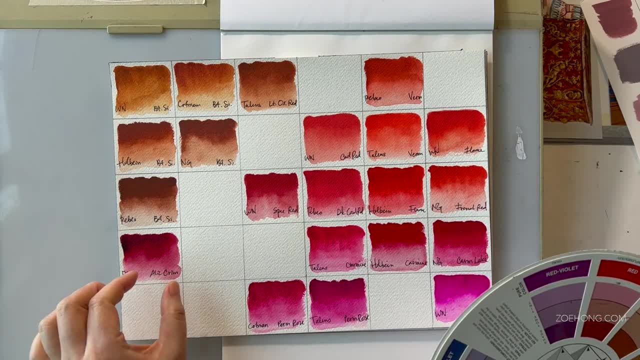 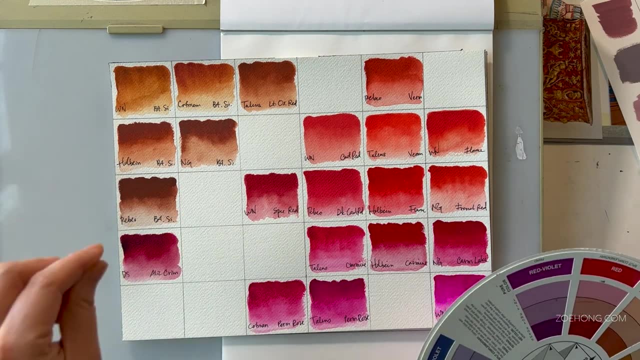 same colors that you're looking for, but with a more lighter tone. And this one I put kind of separately because it's so dark. It's more burgundy territory. This is a alizarin crimson, but it's not quite red red, It's a shade of red, Okay. So these are all undertones. 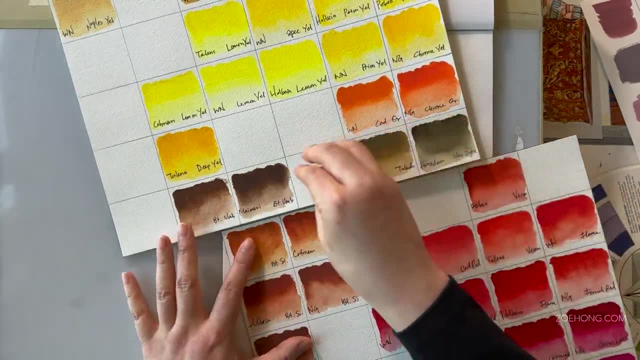 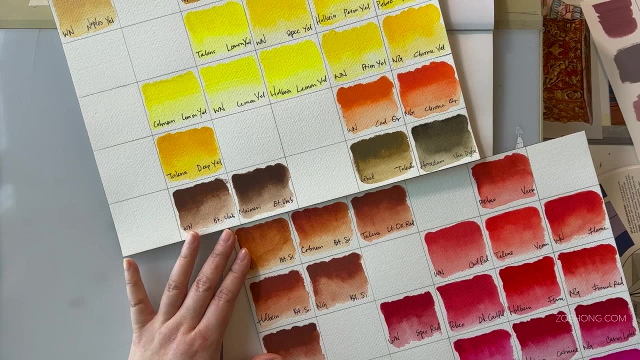 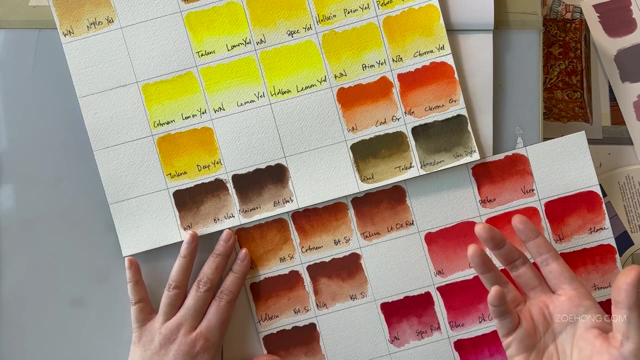 Now again, if you look at these colors, you can all be like, yeah, those are browns. Okay, Individually you could say, yeah, those are browns. these over here tip orange, they're orangey browns. they're called burnt siennas and burnt siennas. 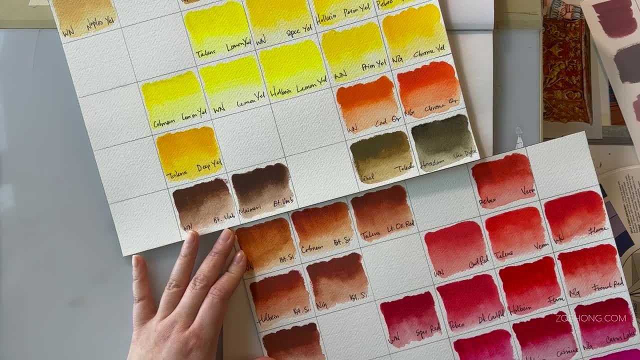 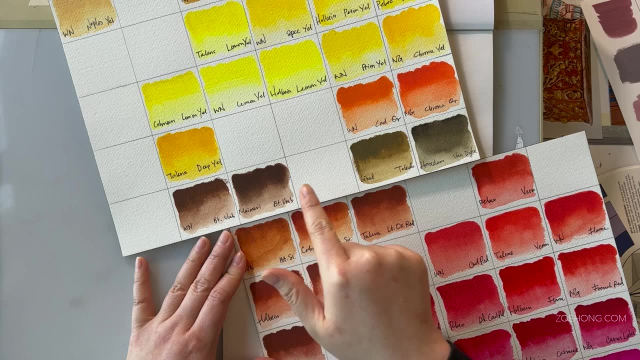 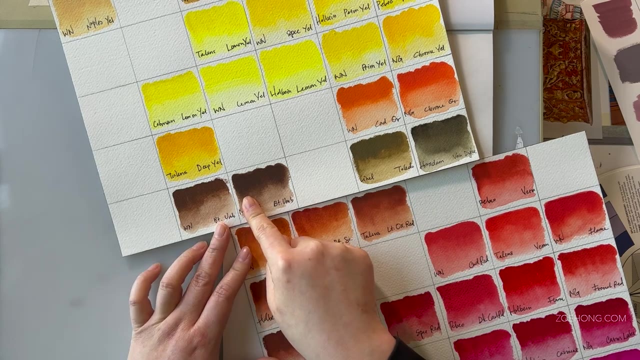 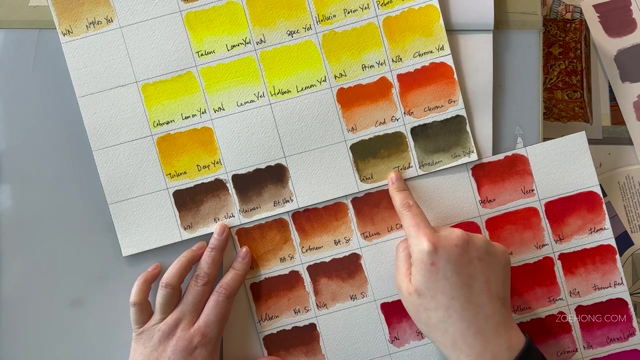 are orangey browns, earthy, kind of rich soil reminiscent clay, red, clay, sort of uh colors. and then we have these colors that tip more red, more rich red browns, and these are probably the closest to what just your average person will call brown. and these in here this one tips yellow and this one tips green. you see the green undertone in here. 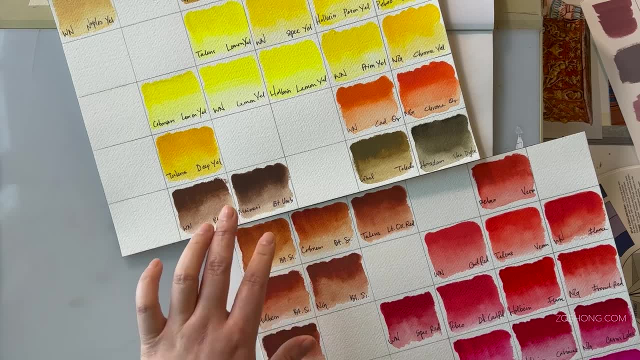 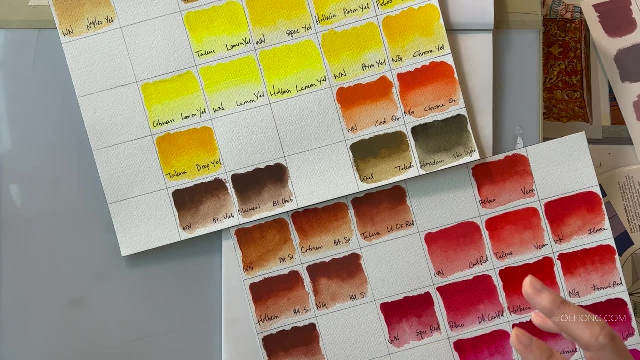 and the yellow undertone in here. okay, quick side note: i have all my lights on and i have the shades to uh the window open, and this is how you should also be doing your color work. if you're doing anything involving colors that requires accuracy. you want to be doing it in the early afternoon. 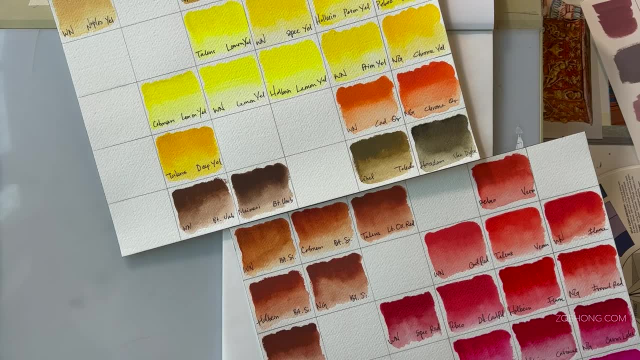 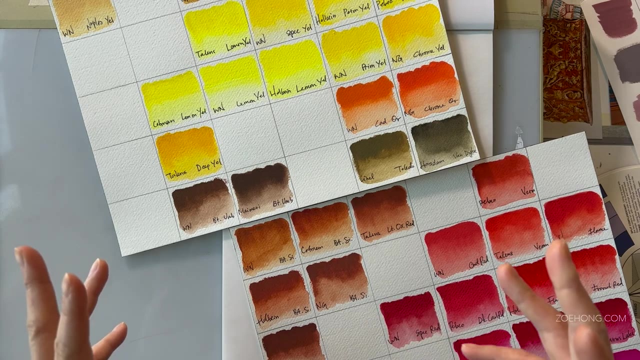 when the sun is high it's super bright. your windows are open, so you're letting all that light in. or all your light bulbs are clean and white. okay, most of us like a moody golden light bulb with a you know uh on our table side lamp in the living room for everyday life, but for color work. 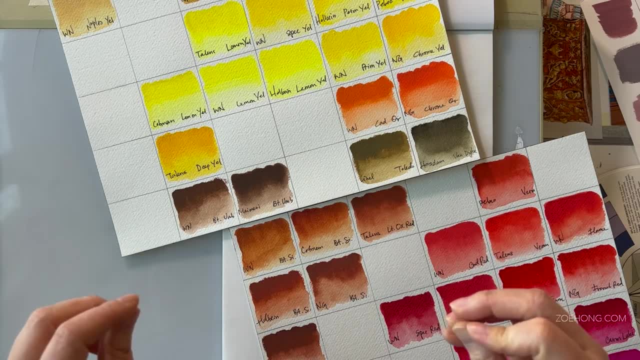 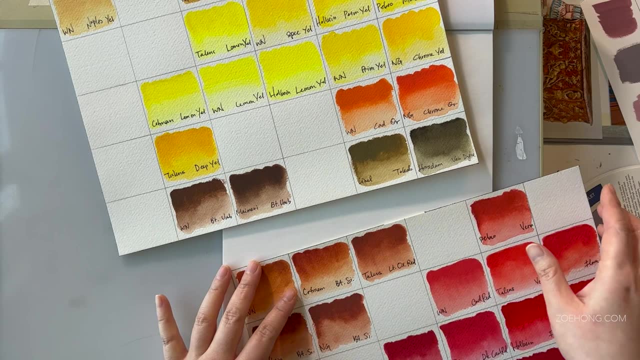 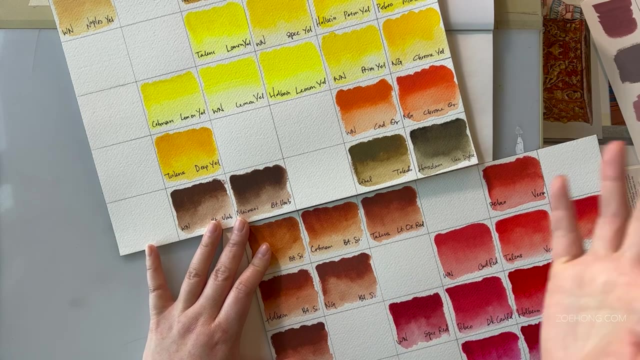 you want white light bulbs, daylight light bulbs, actual daylight outside, like that. so, anyway, all these browns have different undertones, they're all different colors. they're all different colors and that's how you know. oh, this would go well with a brown- what kind of brown? and we're going. 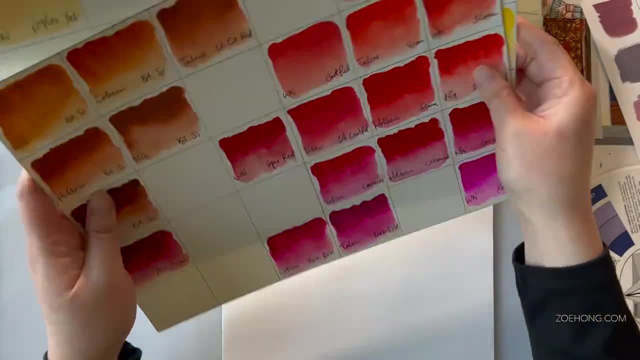 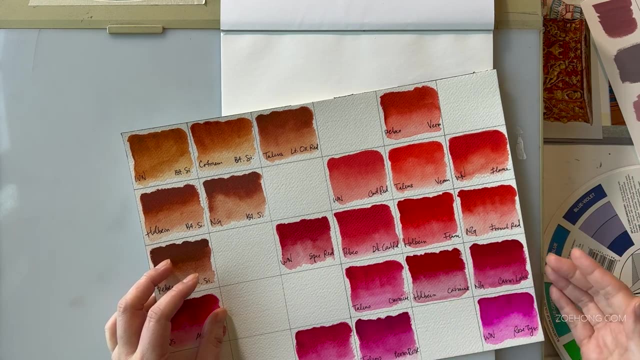 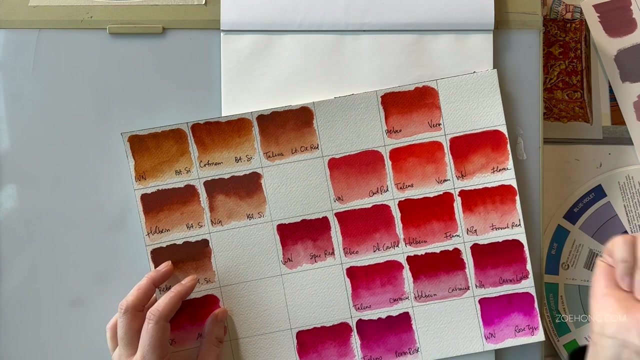 to talk about that more in depth today. so that's undertone. that's kind of the undertone is like: what is the under current of the color? what is the family it belongs to? this is a brown that belongs in the orange family. okay, orange undertone. so what is the difference between a tone? 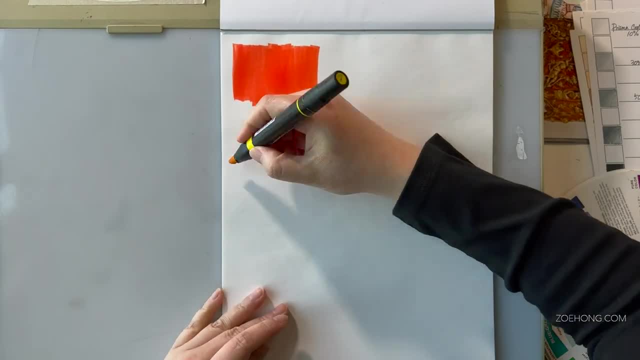 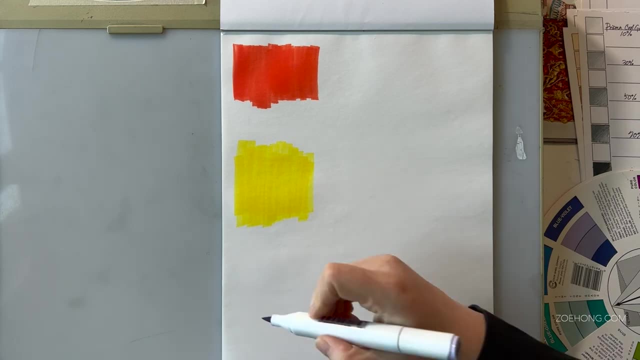 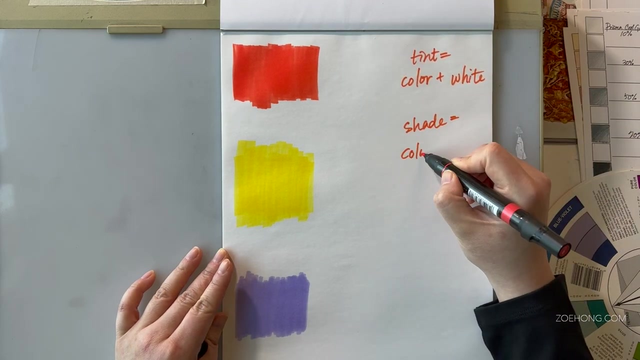 and a undertone. okay, so rewind a tiny bit. there are four different ways to desaturate a color, and when you say the word desaturate, i mean make it less punchy and vibrant and bright. so if you want to take a bright red and you want to soften it, darken it, lighten it, these are all desaturation methods to get a. 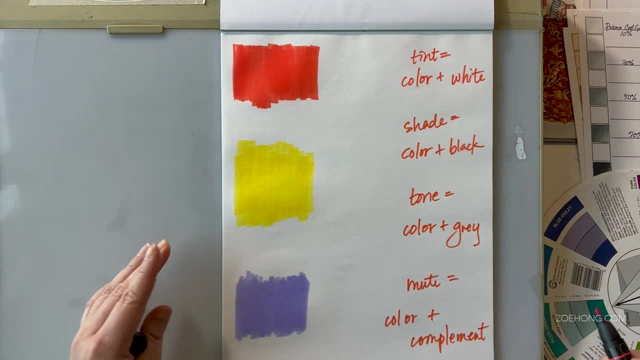 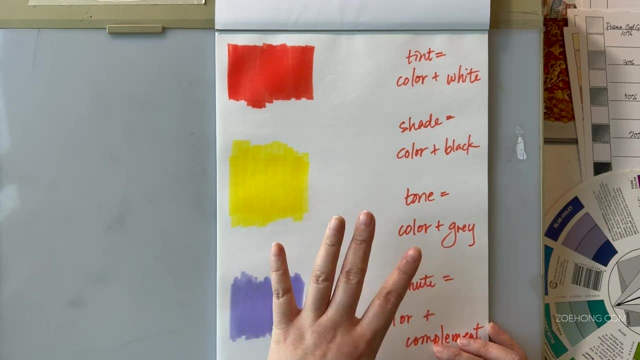 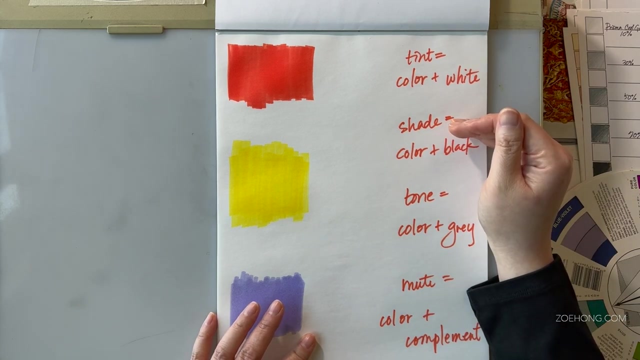 slightly- not quite so- bright red. people use these terms like loosey goosey in the real world, but in terms of color theory these four words have very specific meanings. a tint of a color is color plus white, shade is color plus black, tone is color plus gray, and mute is color plus complement. okay, 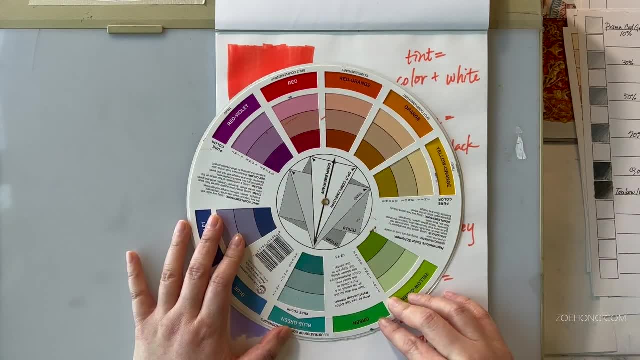 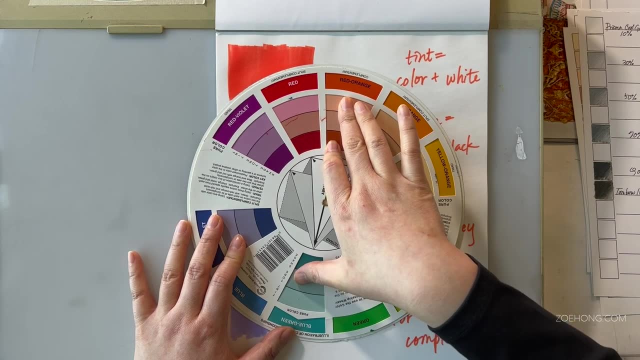 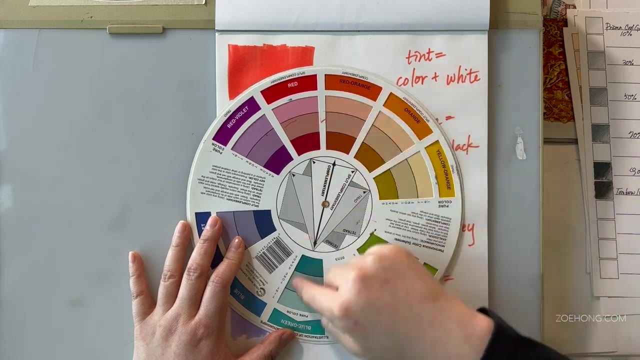 so when you have any color on the color wheel, the direct opposite on the color wheel is its complement, and when you mix two complements together you get a very different sort of desaturation that is really beautiful and can harmonize back and forth with each other Here. 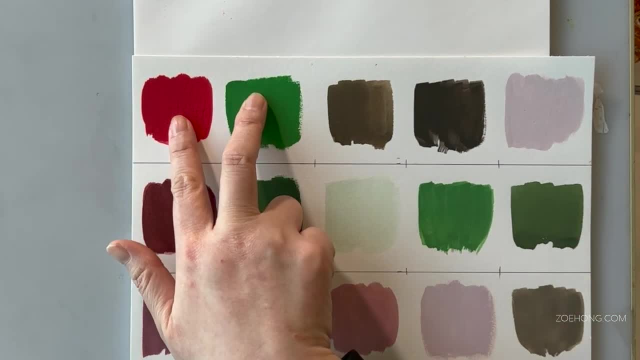 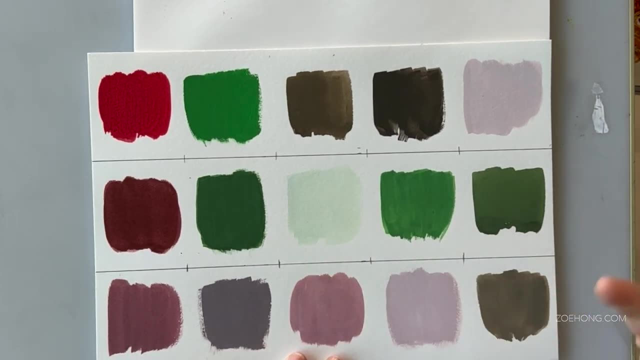 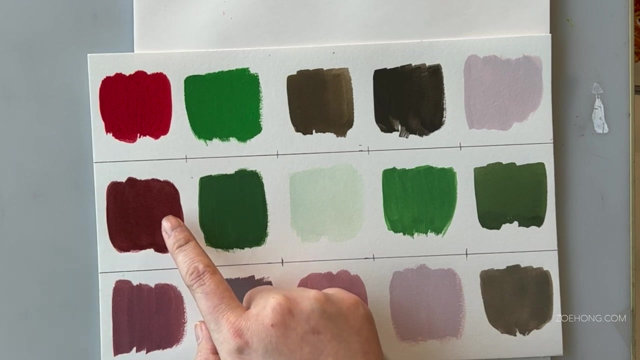 are some color swatches I created with gouache out of red and green. Okay, first you'll see this: this is green plus white. just a pure tint gets a really cute mint color. and then here is red plus black. you get this really nice burgundy color and you can actually get like really nice burgundies. 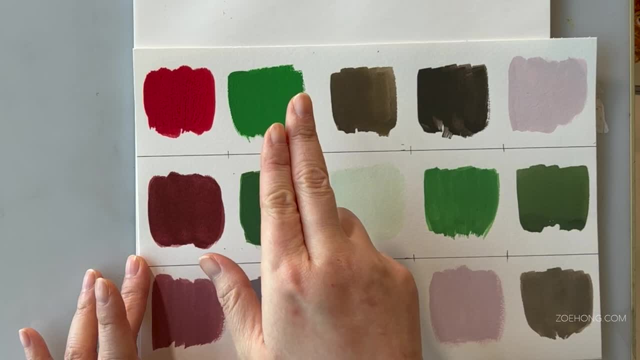 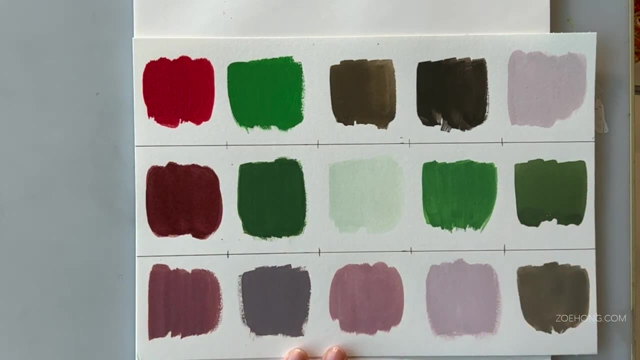 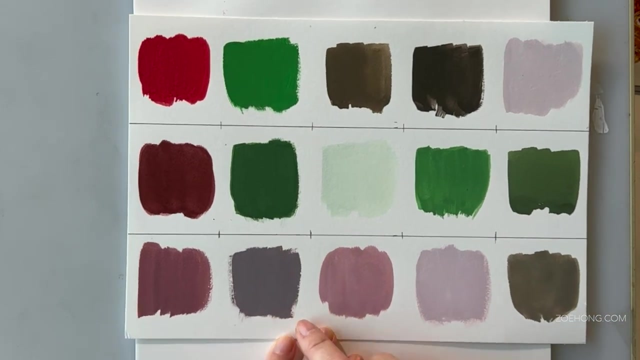 by adding red and black or red and green. Okay, they provide different results. you should try it out yourself. Okay, red plus gray. okay, here's one where it's red plus gray. it reads really gray, but it definitely has these very pink undertones, right red undertones. 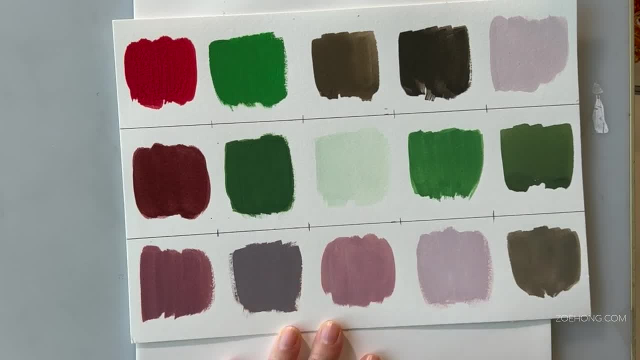 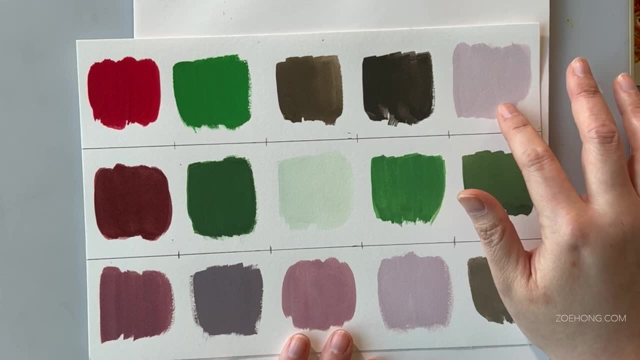 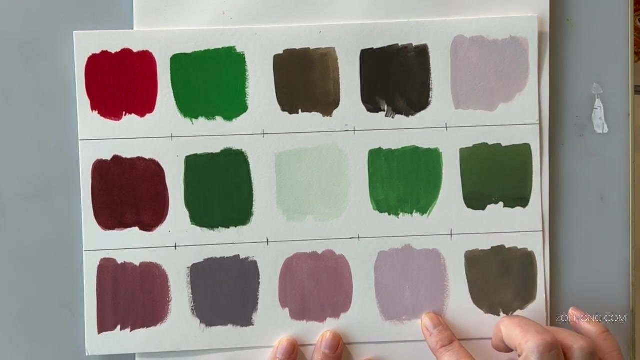 And it starts looking a tiny bit purpley because of the pinkness in there. Okay, same as this. this is a lot of white, a little bit of red and a tiny bit of black, but you see how red, white and black all go in there. Also, here this is a lot less gray than the others. these are very neutral. 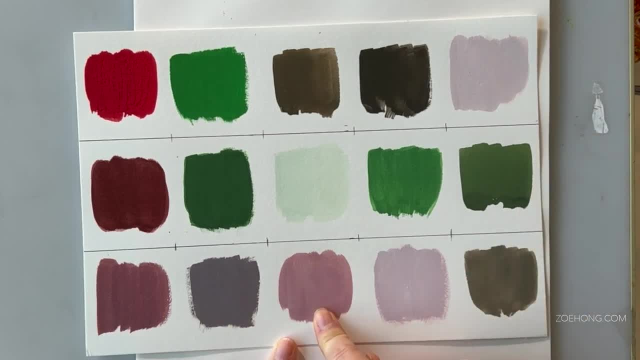 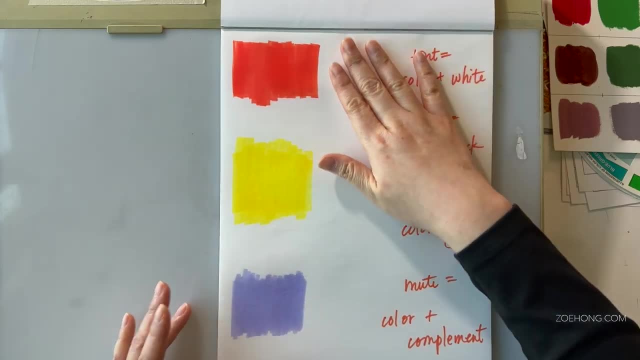 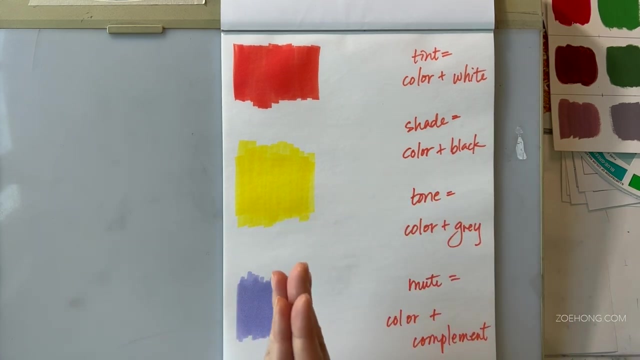 this one is more pink, but this is also toned red somewhat. This is a lot more red than these three. When you are choosing a gray to mix with your colors, it's important that you stick to the correct gray in order to not change its undertone. So when you 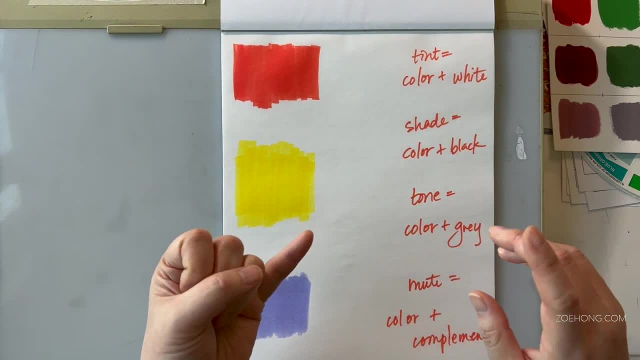 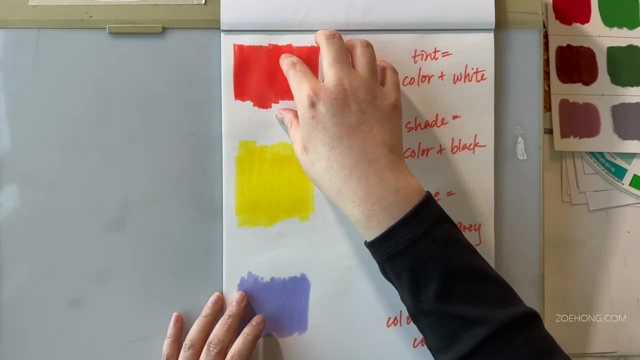 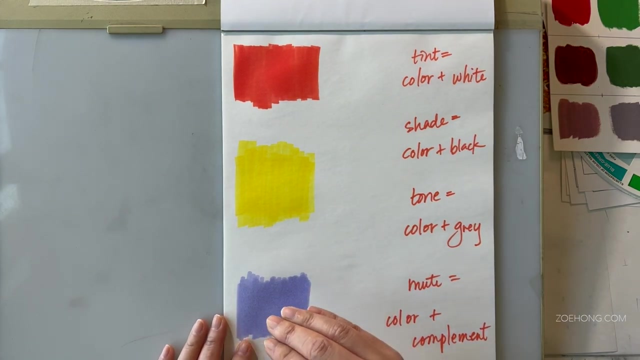 have. you have three kinds of grays, generally speaking. we have cool grays, we have warm grays and we have French grays. Now, when you are choosing a gray to mix with your colors, it's important to red and orange colors, get a warm gray, and blue, blues and purples get a cool gray And yellows. and 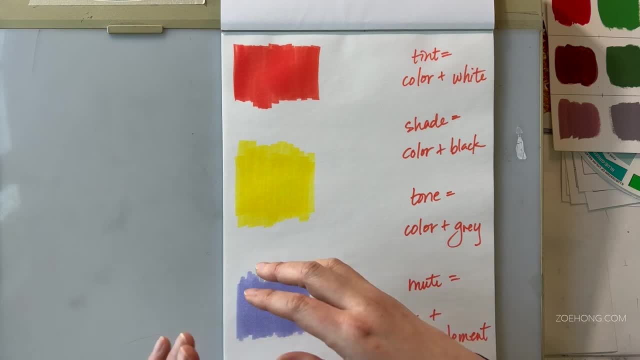 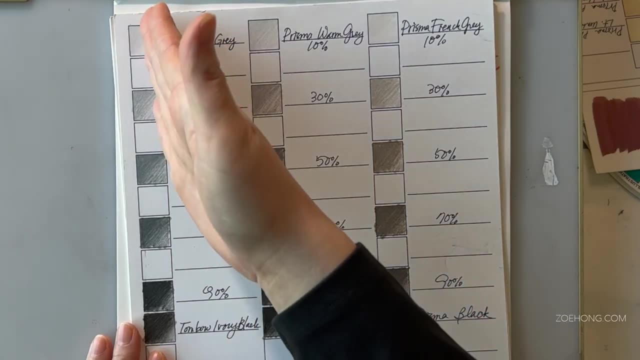 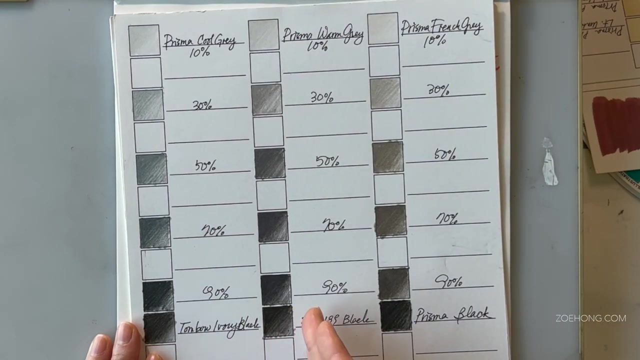 greens get a French gray, because French grays have kind of a yellowy, greeny undertone. These are color pencils, just but to demonstrate, do you see how cool these are and how these tip more warm, like there's a little bit of red in there. 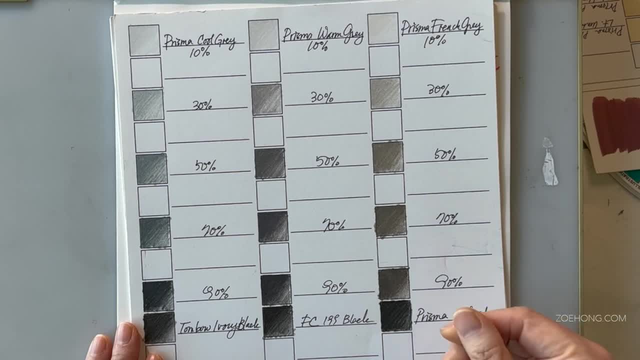 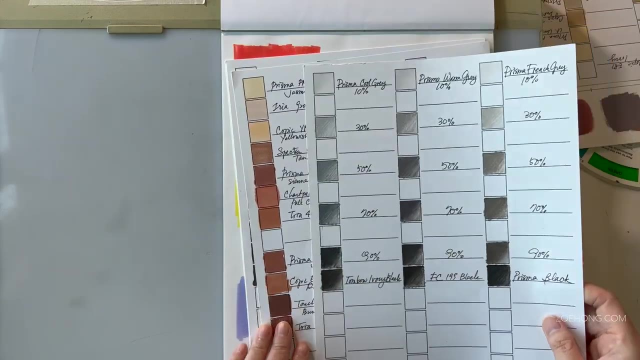 And these have a more yellowy greenish undertone. These are French grays. Okay, can you see the difference between the three? Now, I want you to keep this in mind, because labels mean nothing. Art Supply companies label things ridiculously, Okay. so these are Prisma Neopiko. 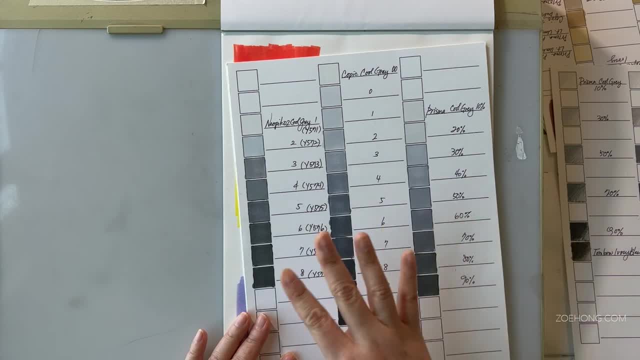 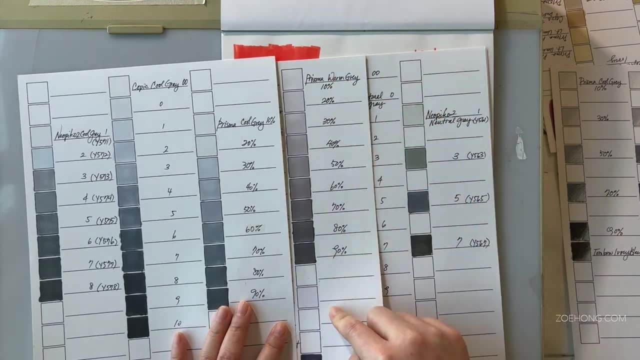 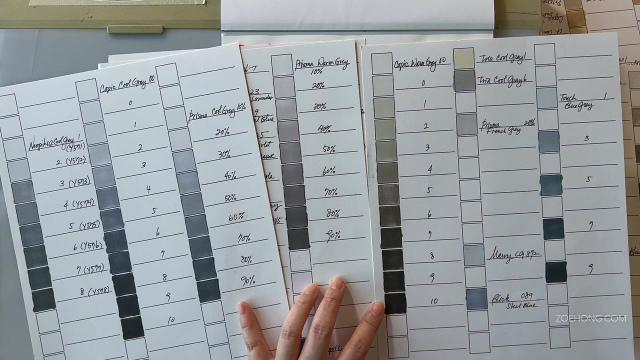 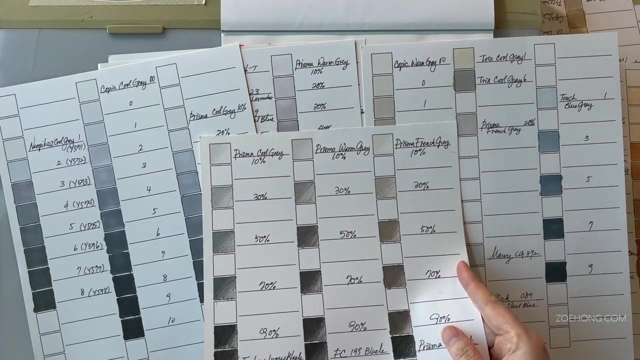 and Copic cool grays And they're all fairly similar to each other. so the cool gray is fairly standard. However, this is the Prismacolor warm gray which tips a little bit purpley, a little bit red. Here is the Copic warm gray which tips yellow green, which is like the Prismacolor French gray. 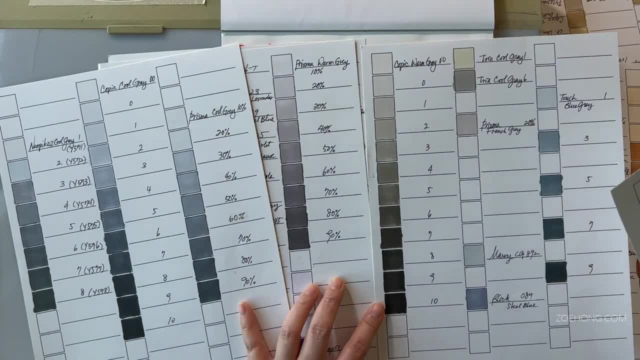 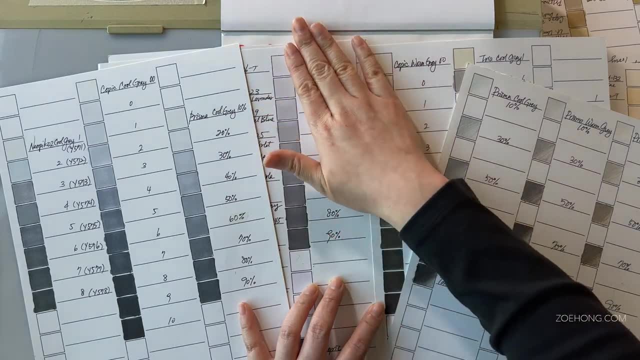 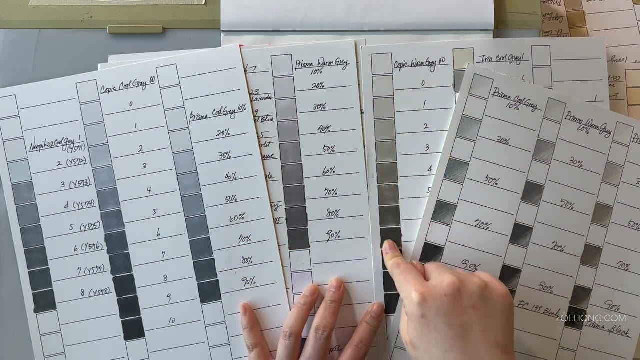 color pencil. So listen, learn your colors, but don't get too wrapped up in these labels. This just regardless of label: this is a warm gray, This is a cool gray, This is a green toned gray, This is a red toned gray, et cetera, et cetera. So always think of it in those terms and 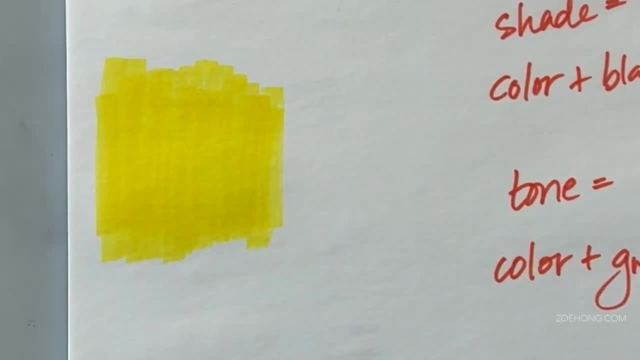 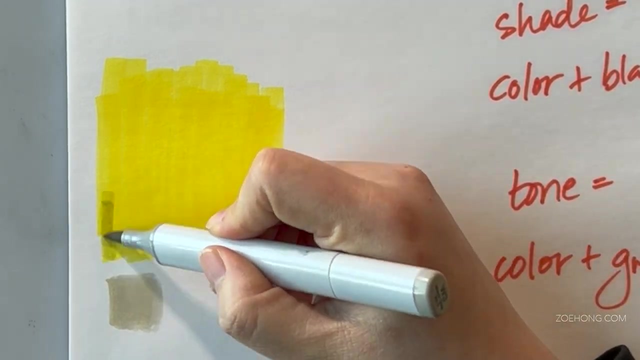 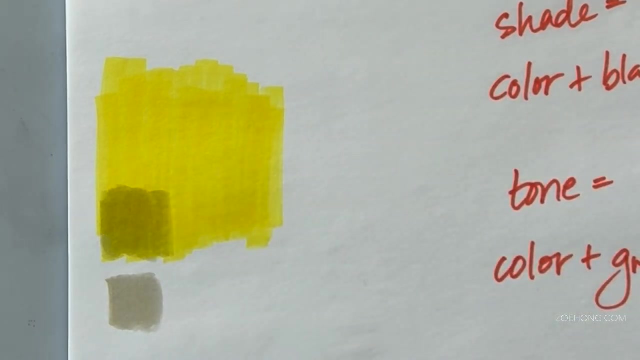 not necessarily what's on the label, But with yellow you definitely want that yellow toned green, greeny gray. This is Copic's warm gray three, and here's it by itself. And do you see how yellow That tips? And so when you layer the yellow, that's really dark. Let's try a lighter one. 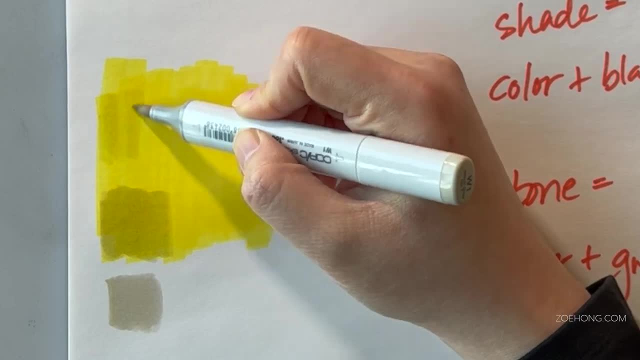 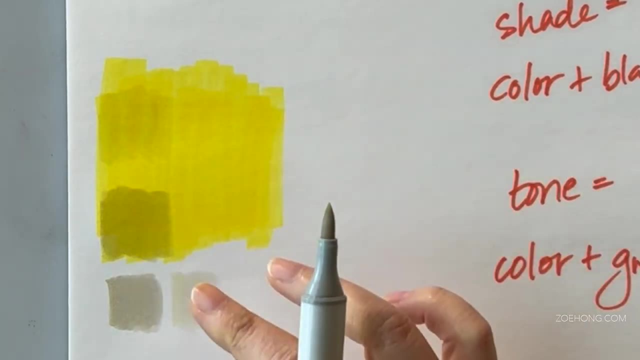 The yellow is already a light color. This is that yellow toned yellow gray. Do you see how these work together? It doesn't fight the base of the yellow, It just makes it a little bit darker, but not black, Whereas if you added a cool gray- whoa, that's way too dark, That'll overpower the yellow. 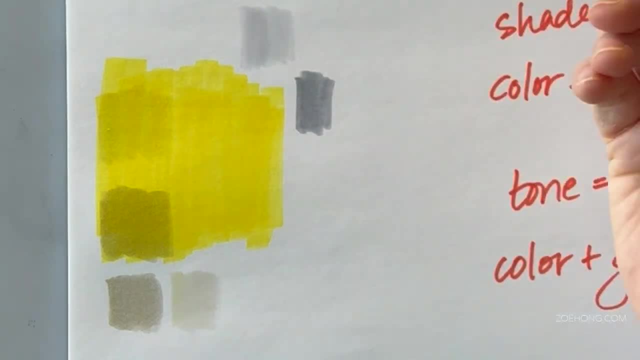 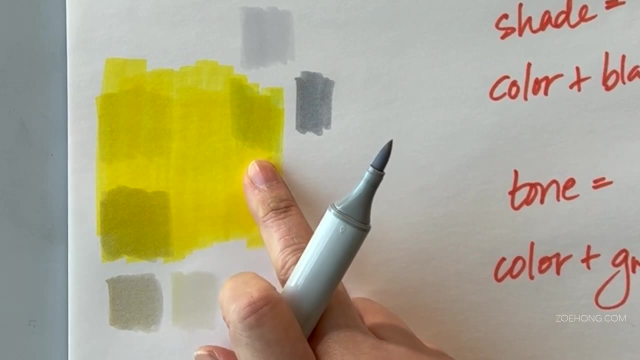 So even if you have this really light cool gray in here, you see how different those colors are. If you put this in here, you will start changing the undertone. You see how it's now starting to look a little bit green because you're making the yellow cooler. So 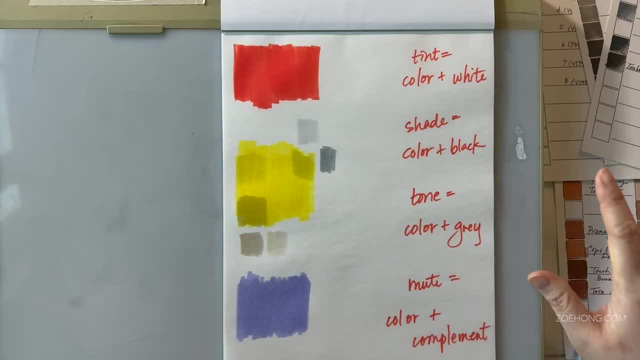 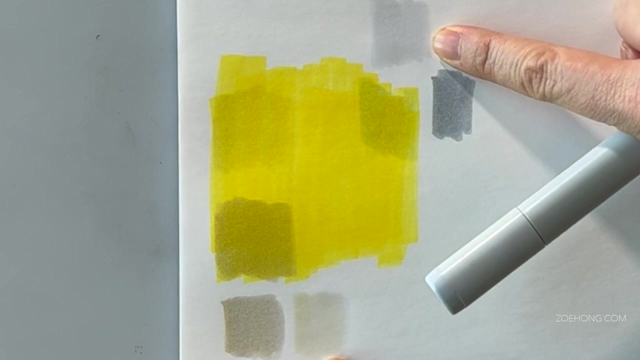 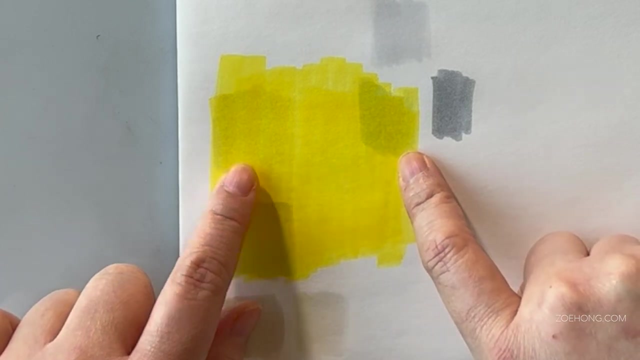 it's tipping towards blue. Orange is the warmest color and blue is the coolest color, And so anytime you're like tipping blue towards blue, you're getting cooler and then the reverse. So you see how these grays. they're so similar to each other in value, but this is changing it to a gray undertone. 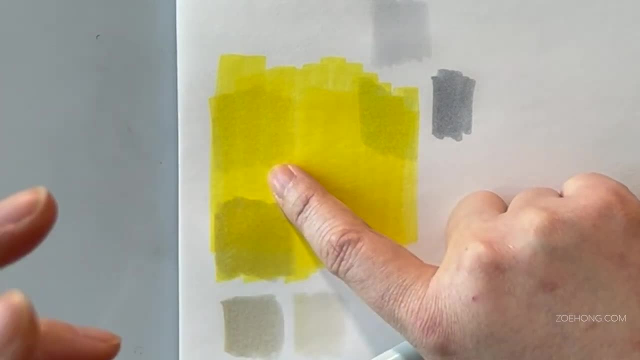 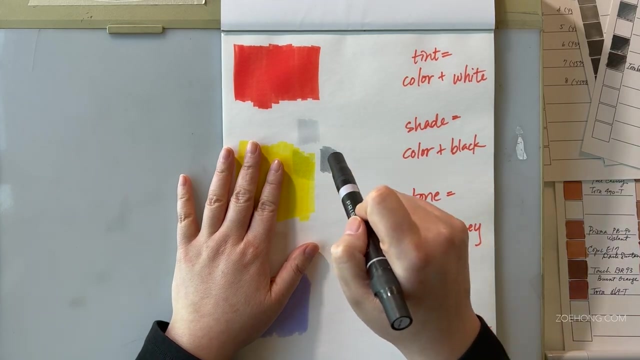 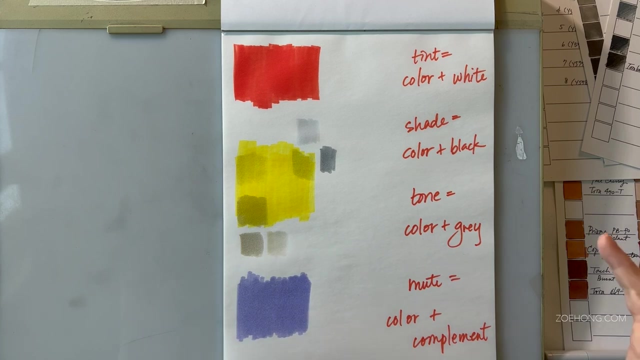 where this is: keeping the yellow and then just adding the gray, And you see how that harmonizes better. I mean, ultimately, if you want a green or yellow, then yeah, you can mix these colors together. That's the whole point of color theory. is, you know, not like a restrictive? 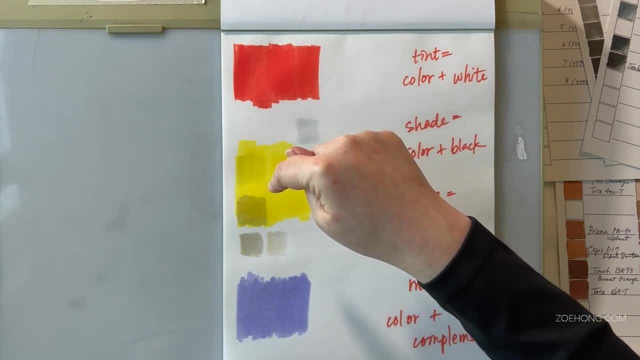 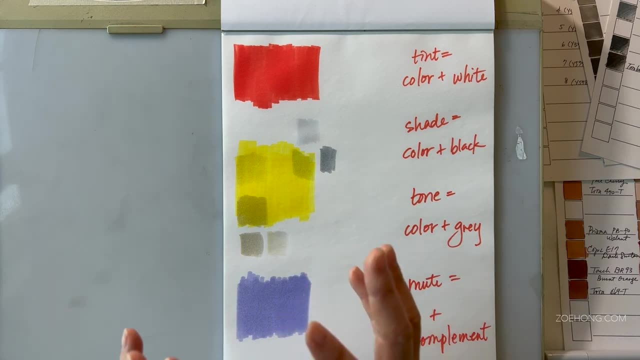 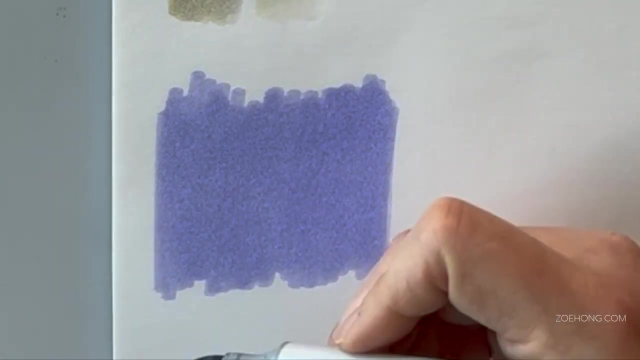 set of rules that force you to do things in a certain way, but to give you, like, information on how color works so that you can make decisions and not just trial and error. This is violet, And so let's add this cool four And you see how that harmonizes really well. This one is pretty warm, And when we look 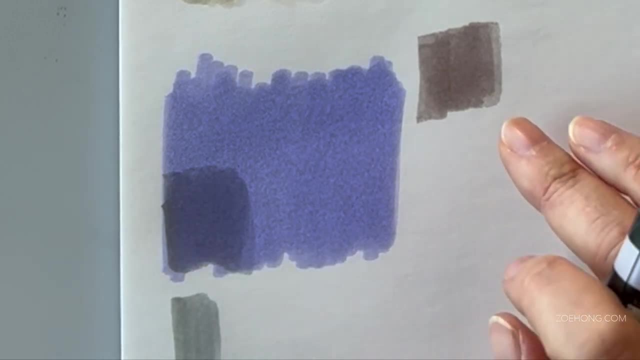 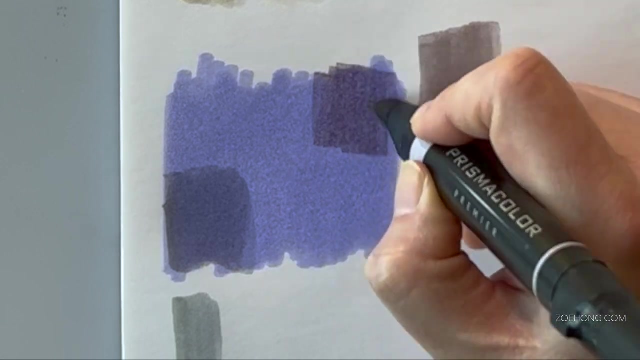 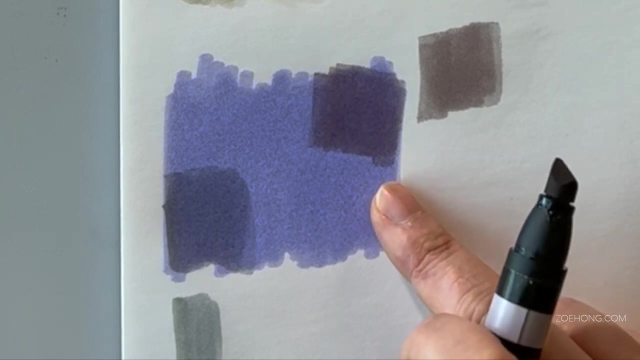 at it. it does tip purple, but it really tips red, Okay, and it's very obvious when we put it next to something that is truly purple. So when you layer it together, you see how you're warming up that violet significantly, right. So that shares an undertone And you're 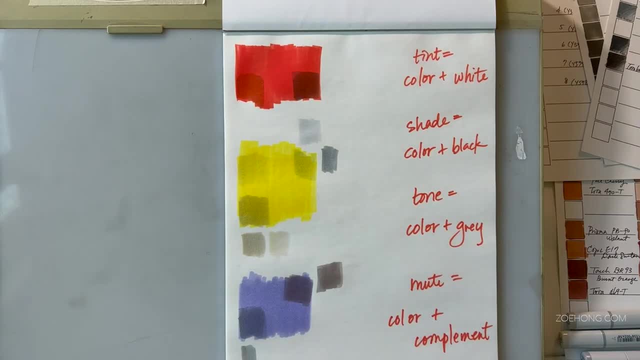 and that tips it very red. So learn how these grays work. so when you're making your tones, you can decide: I want to keep my original undertone of my color and just tone it down, or I want to change it radically. But honestly, if you're trying to stick to a specific color story, 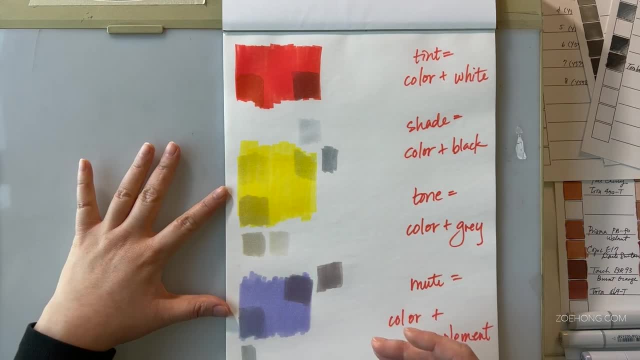 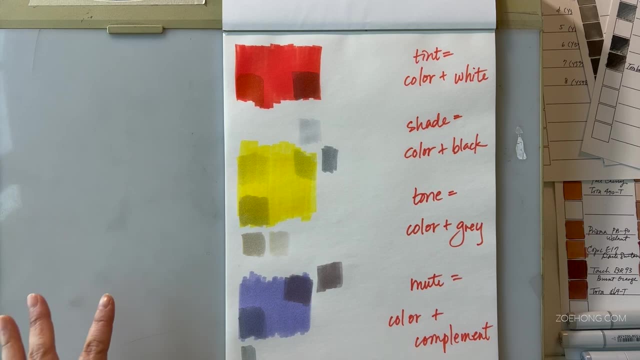 like if you are trying to stick to yellow and purple as a complementary color story, you don't want to start adding greens and reds to that. That's, you're starting to go in too many different directions and so you want to stick to the grays that work for the yellow and work for 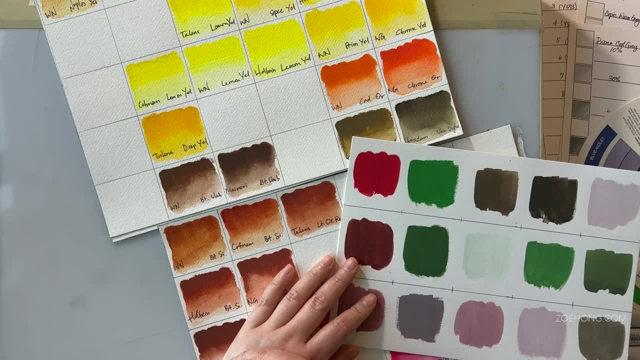 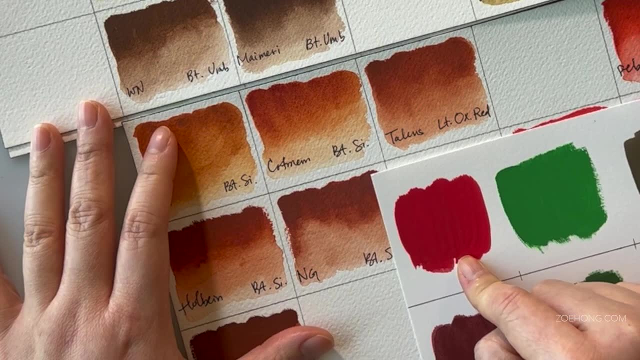 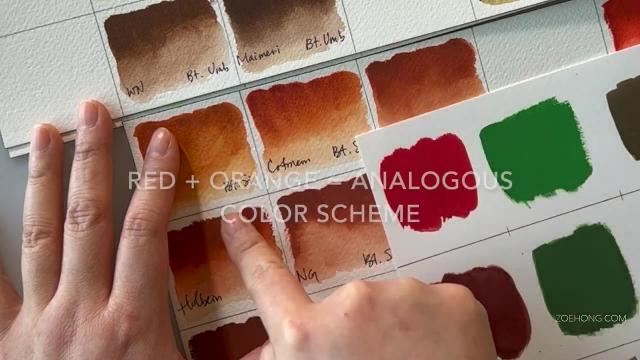 the purple. So how are we applying this knowledge to fashion? Okay, number one. let's say you're putting together an outfit. let's say you have this red and you want to work in some warm neutrals. okay, so you can go in here, because these are more orange, but they have enough red in them. 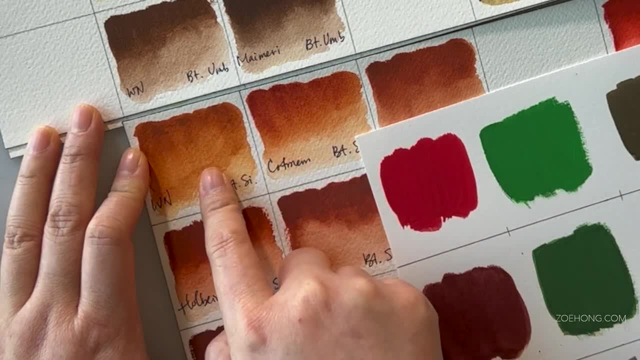 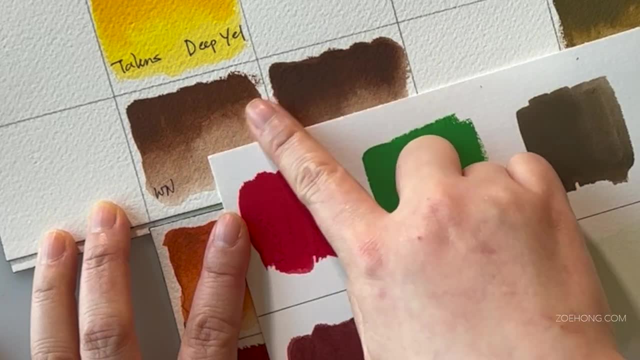 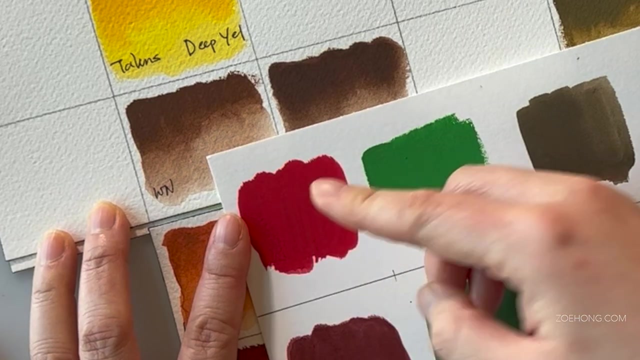 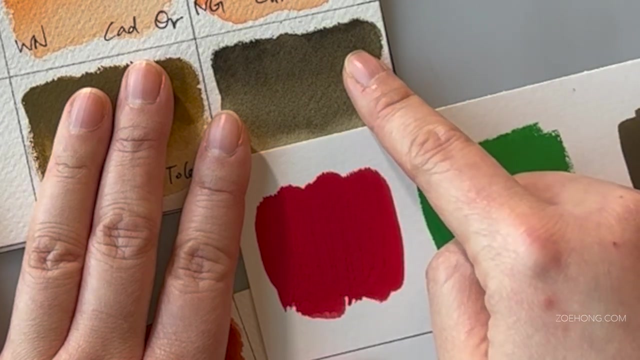 but can you imagine throwing a beautiful leather blazer in this color on top of a red sweater? these browns also work because their base is this red, and so these all work together because they share an undertone. this works because this is green. okay, this is like ordering deep olive. 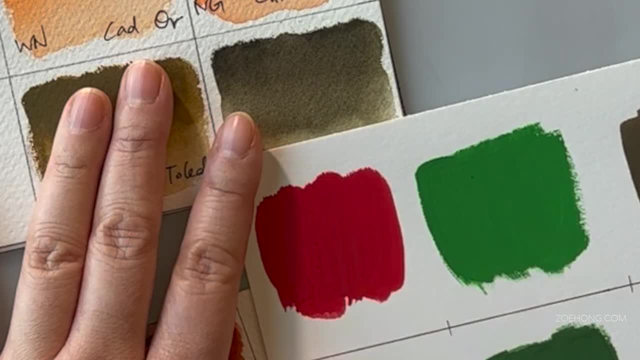 and since green is its red, compliment it's. they don't share an undertone, but they're compliments and they complement each other. that's where that work comes from. and yes, it's spelled with an e and not an i. compliment with an i is when you say nice things about someone. compliment with an e. 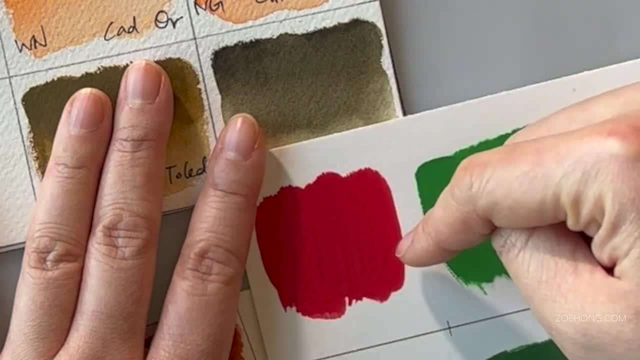 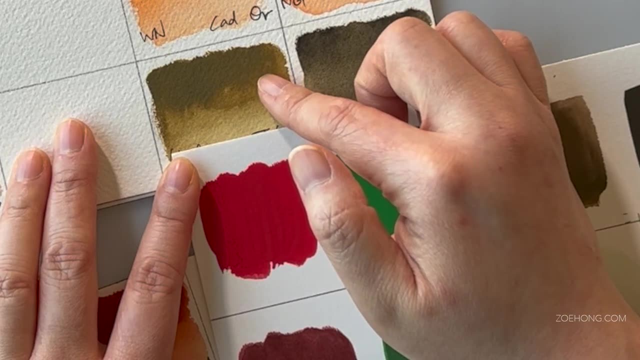 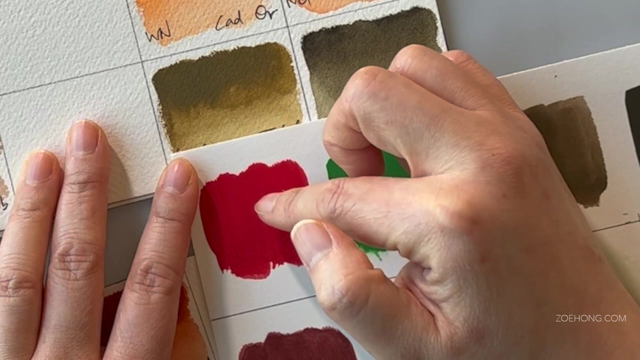 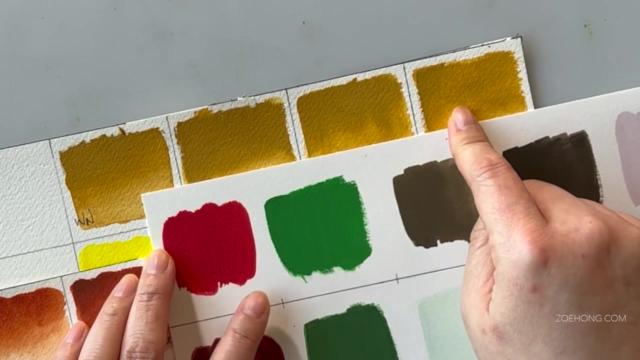 is when things go well together. okay, compliment these. this is the least pleasing pair because this has a yellow, yellow, green undertone, which is not a great compliment for red, nor does it share an undertone with red, and so these fight each other. they do not work. these can work kind of depending on the texture. 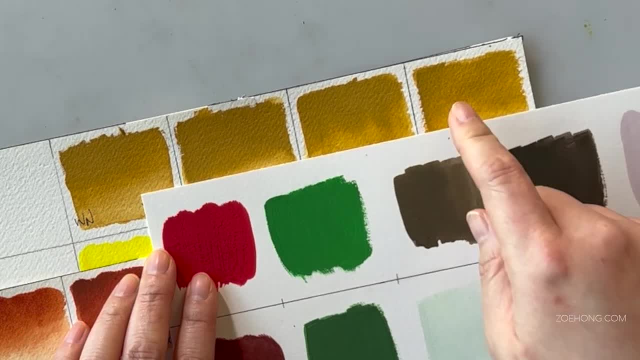 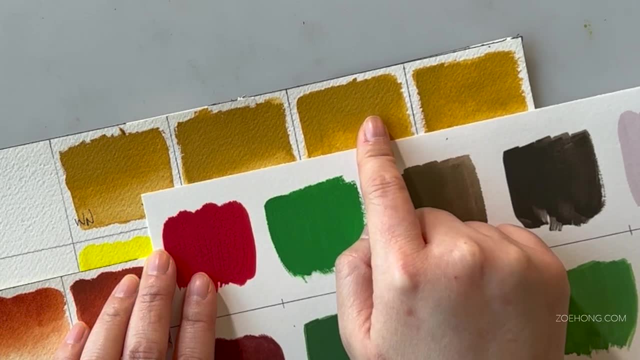 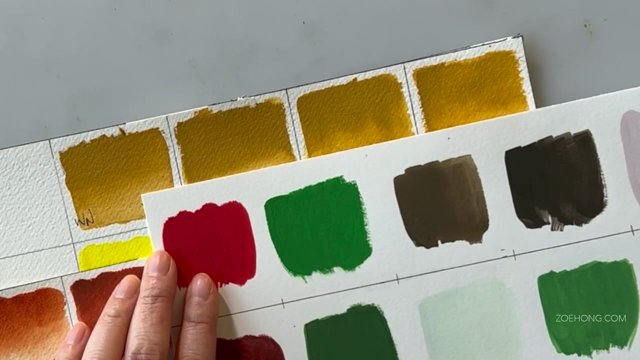 it will really depend on the texture, okay, but these will definitely give like a more 70s vibe. can you see these like golden corduroy flared trousers with a red turtleneck, merry 70s. it works, but it definitely gives a retro vibe, for sure. you know. compliments in an outfit. 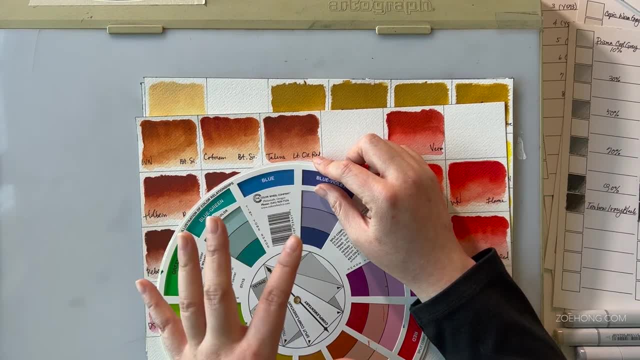 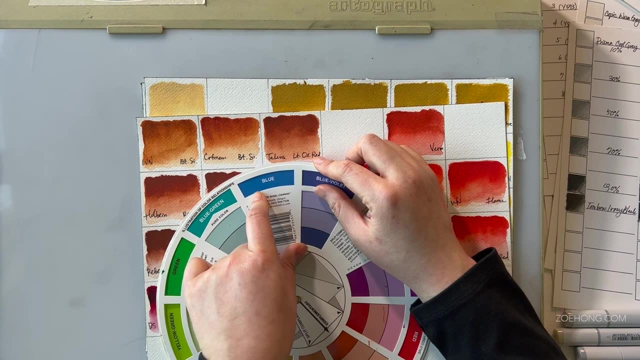 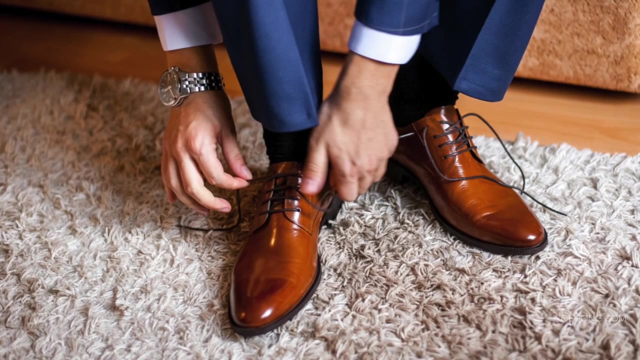 are really noticeable in menswear. menswear uses this a lot. when you see a man in a blue suit- and not it doesn't even have to be this bright, it could be slightly darker- often is- you will see them in a brown belt and shoes, and you're going to see them in these beautiful burnt sienna colors. 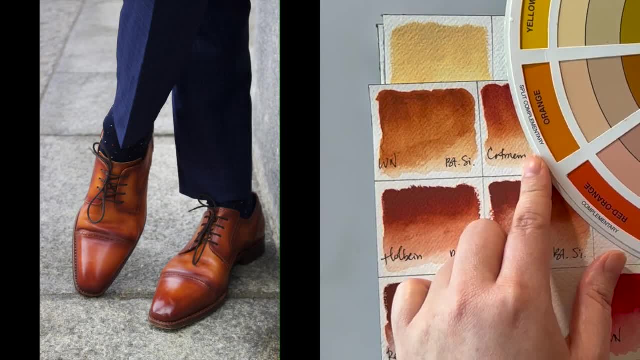 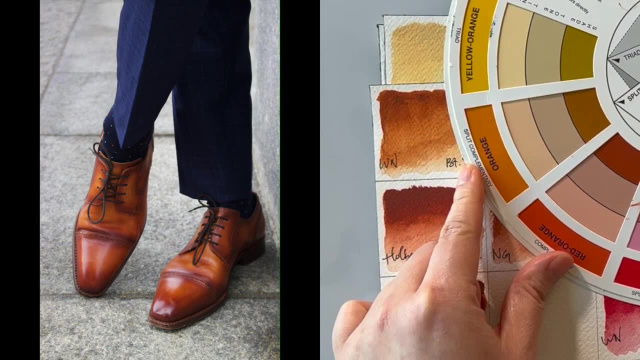 i'll give you a quick look at my blouse and just a little shock on my bra, but i will tell you i have changed a little bit of my shirt color because i think you can see that the edge is not as white as my thong, and so i fall in love with my blue shirt color, and i hope it doesn't. 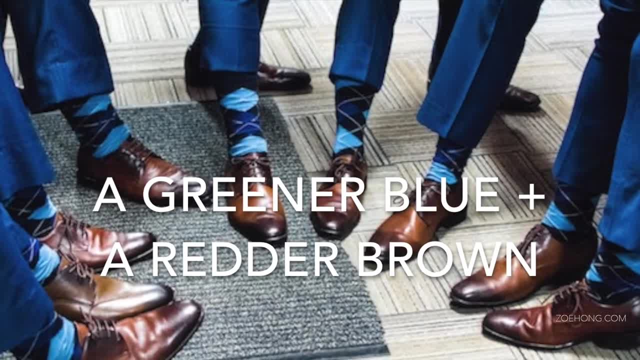 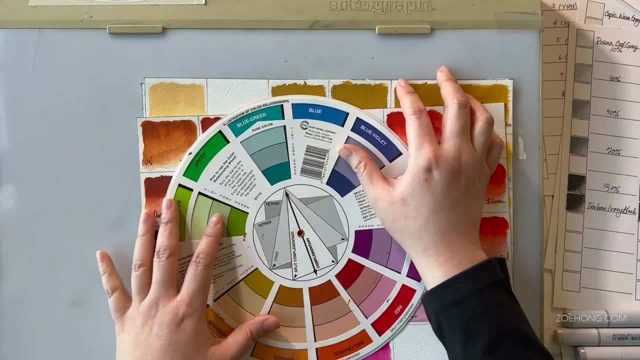 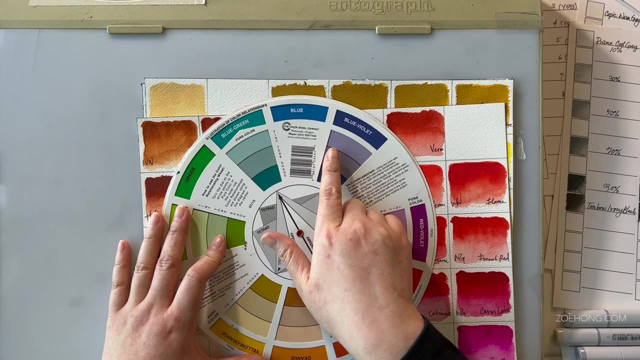 look like a mess to me. when i'm wearing a blue shirt, i often wear it like a top top, top temperature to be more poky pink, so i always wear a navy and navy shirt. look like i'm wearing a navy blouse. Now, when you have a blue, that's tipping more violet. you know, you get a little bit darker, you get a little slightly more violet- maybe not this purple. 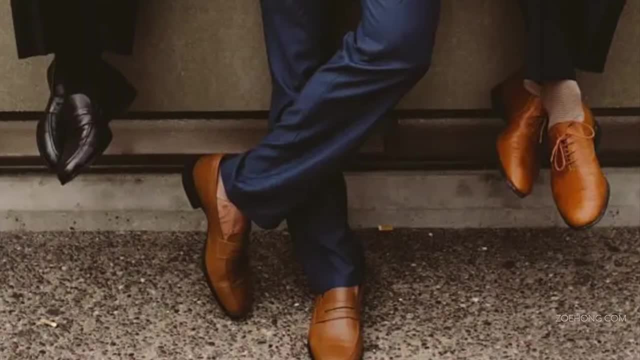 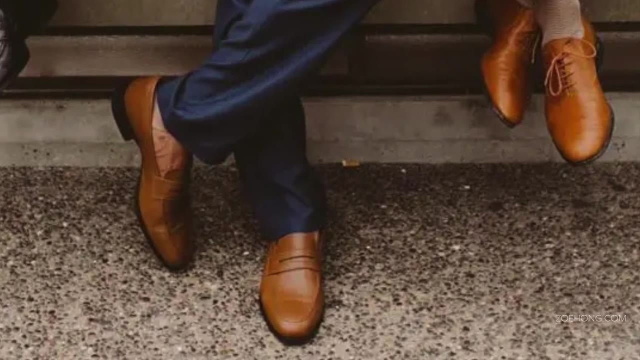 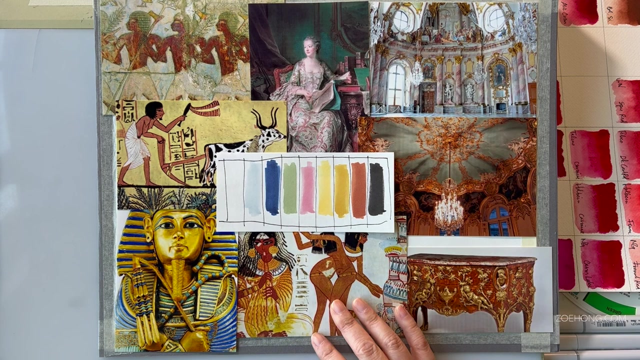 The complement is more yellow, more golden. So when you're in this territory, you're going to veer cooler, more yellow toned browns. This is a mood board that I did. This is a fashion project I did And it was only a teaching demo. 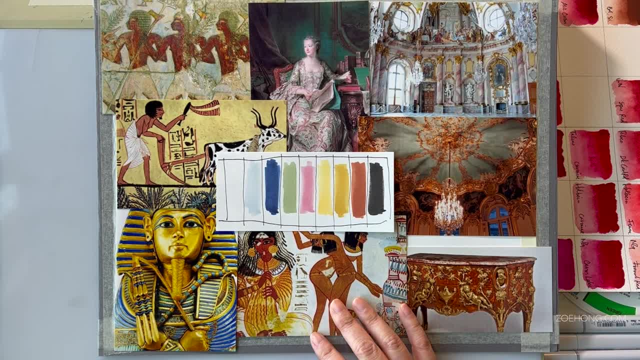 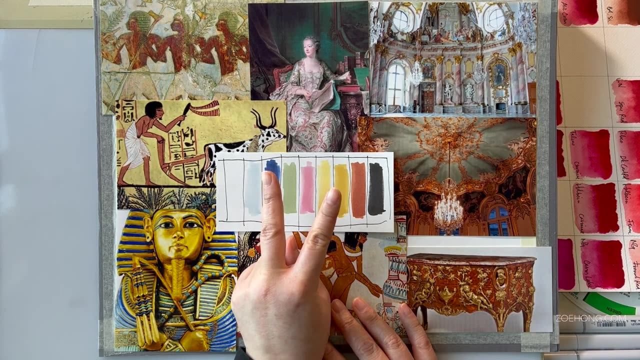 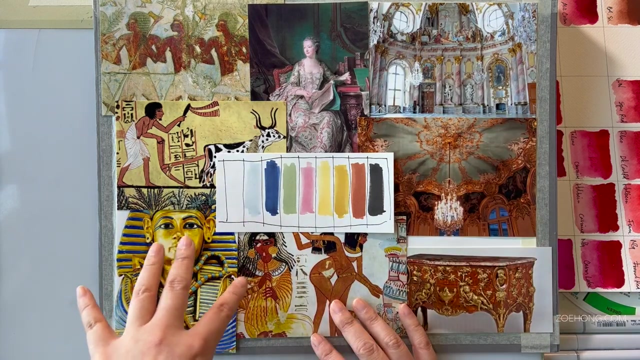 I did it really fast for a teaching demo, And I cannot even begin to tell you when and why I did it- Maybe for Patreon, maybe for a different YouTube video, But the brief that I gave myself and gave to my students was: pick two time periods in two different countries, parts of the world, and use references from those time periods and countries to put together your inspiration for a fashion collection. 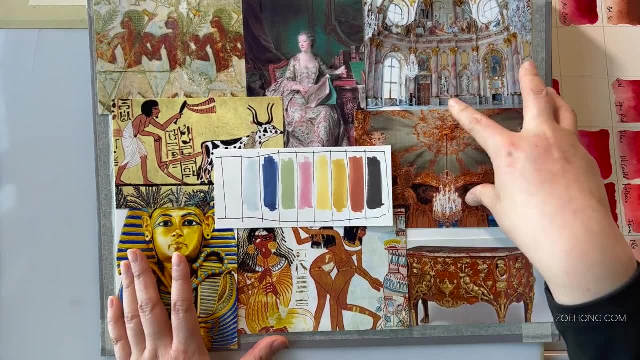 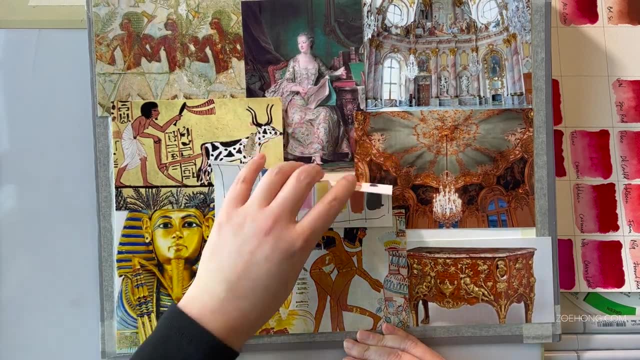 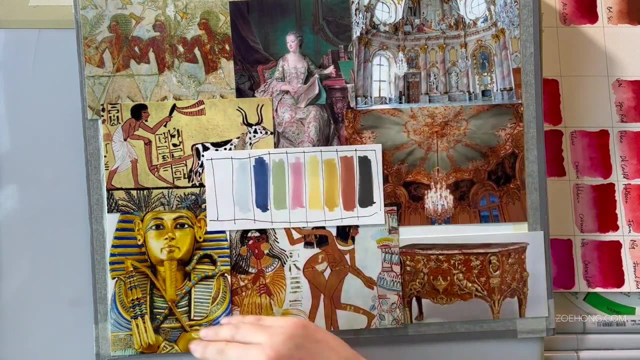 And I chose France, Rococo, France Baroque And ancient Egypt. And I didn't have my color story at the time, Don't look at this yet- And I just wanted to. you know, I brought all these in together. 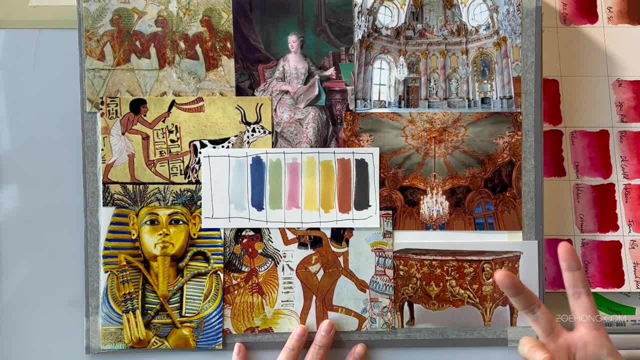 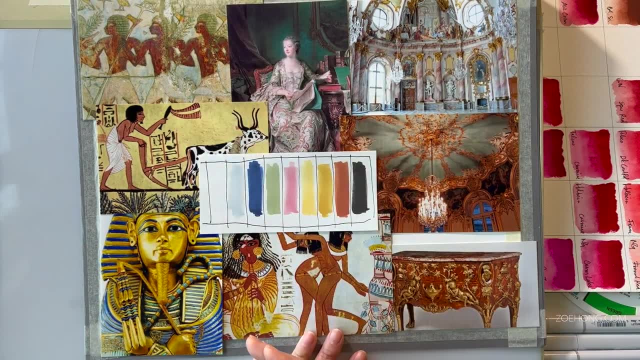 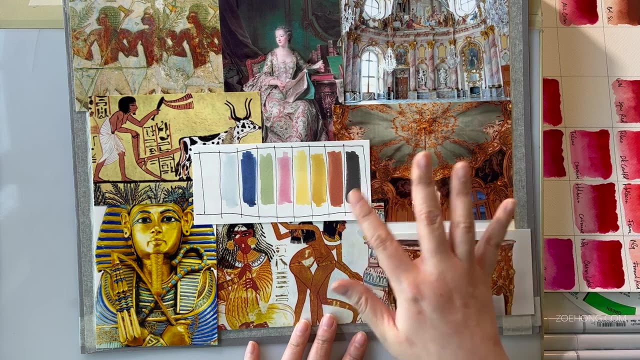 And what do you notice? first, The rich browns, right, They're very warm orange toned. in all this Egyptian art, all this ornate wood, you know, warm wood, gold, And in this picture I really like how the lighting makes all the gold look copper, really more warm tone. 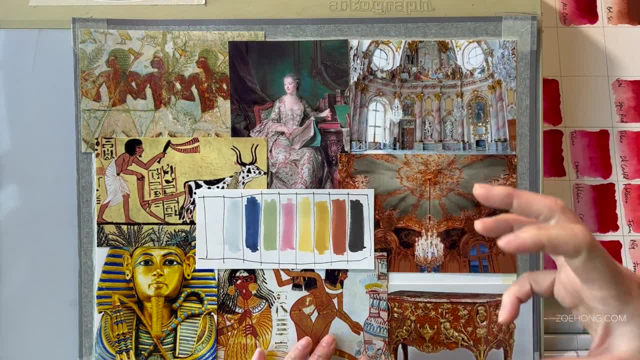 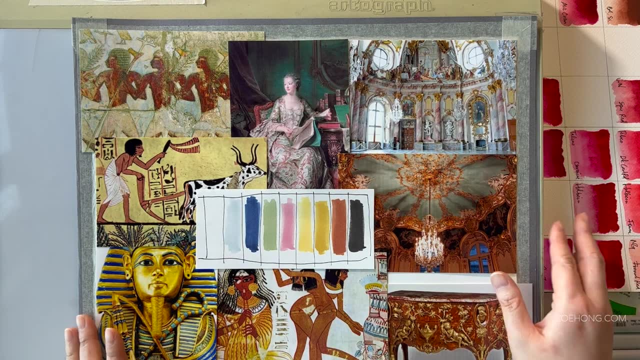 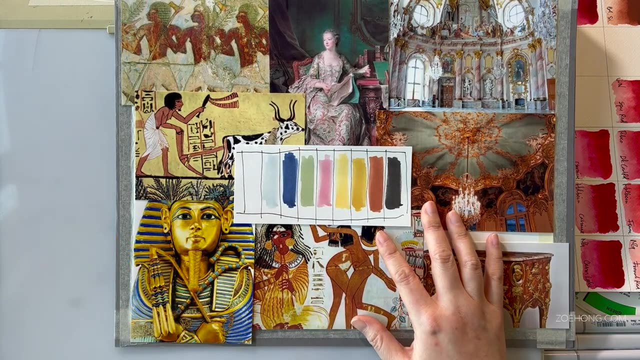 But even in this, where it's broad daylight, the gold is so warm, it's veering orange, So I like that And that was very prominent, Okay. And the second most prominent color was the blue. Okay, These deep cobalt, super saturated blues. 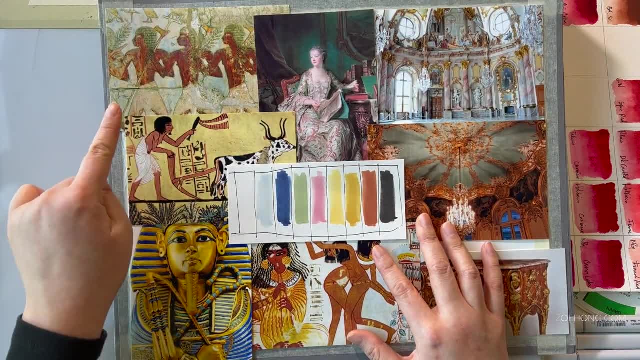 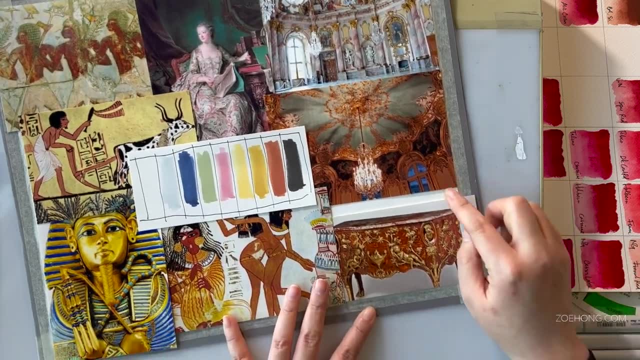 And some of these pastels peeking out in here, Bits of pastel in here, All these pastel blues in here. And then, for some reason- I know this is just lighting, but it just it was such a punch And there's blues in here. 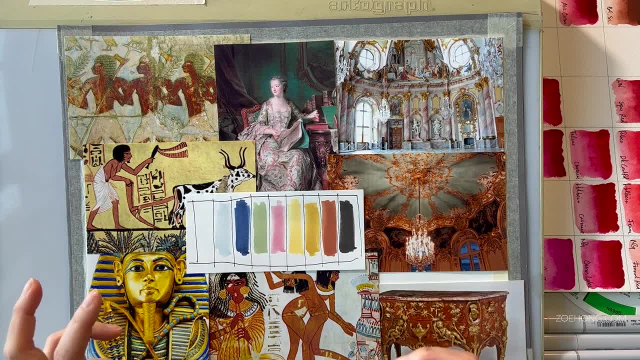 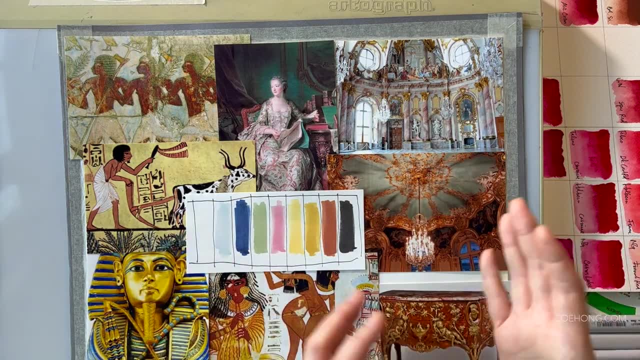 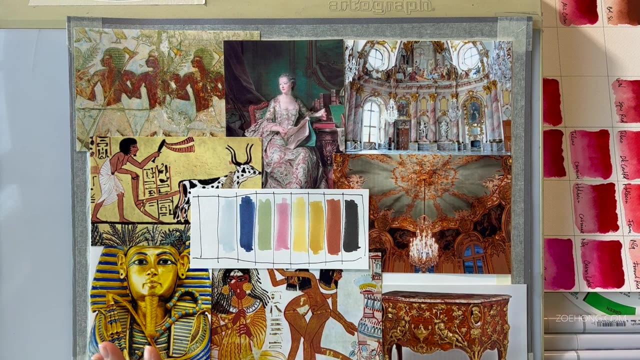 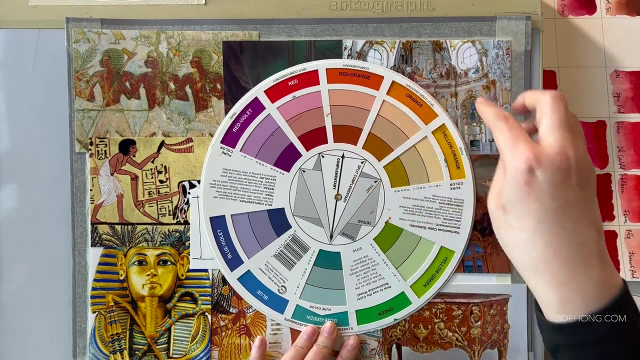 So I wanted this warm sort of but like, really focused on this gold and the brown Because I didn't want one or the other- Okay, Because they are so much the essence of these two time periods and contrasts. And so I played around and was like yellow and gold and these woods. 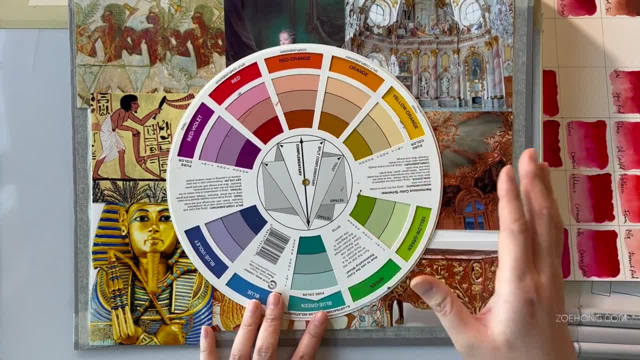 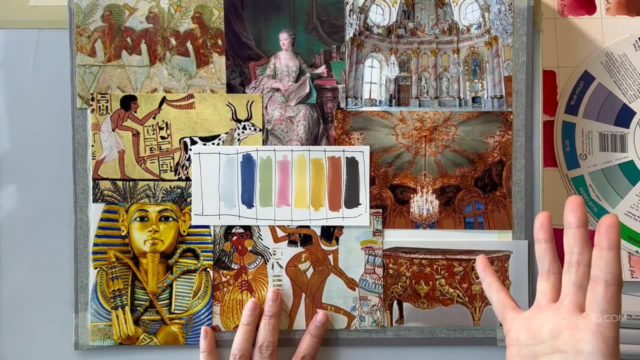 Here's where understanding undertones comes in, Because when you look at all the desaturated and saturated colors on a mood board like this, then you can understand the source of the color, When you understand these warm undertones here, here, here. 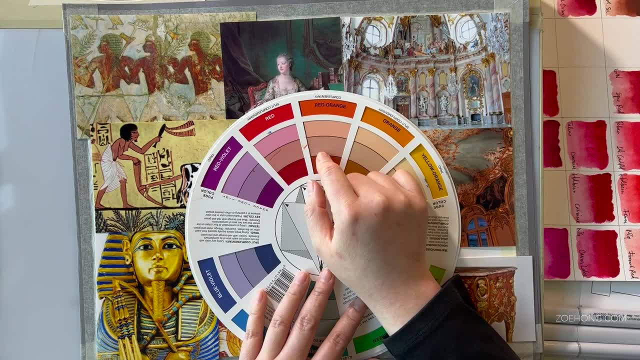 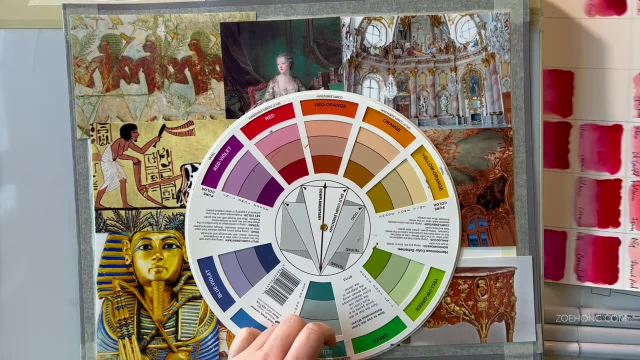 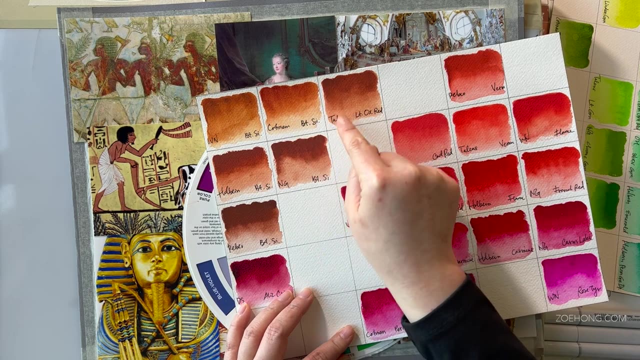 then you know that Red orange is the source color, The mother color. Okay, That's the base, And we're talking like these. Okay, These orangey, but more redder toned. They're redder than this bright orange one. 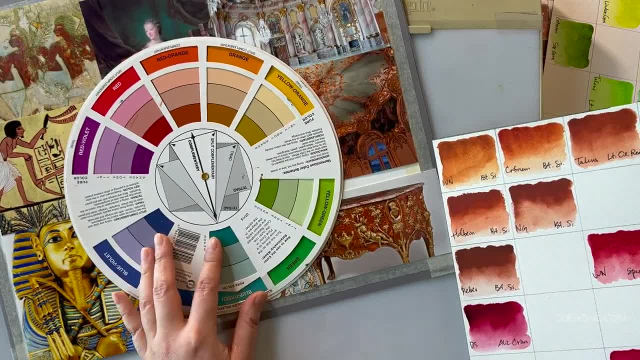 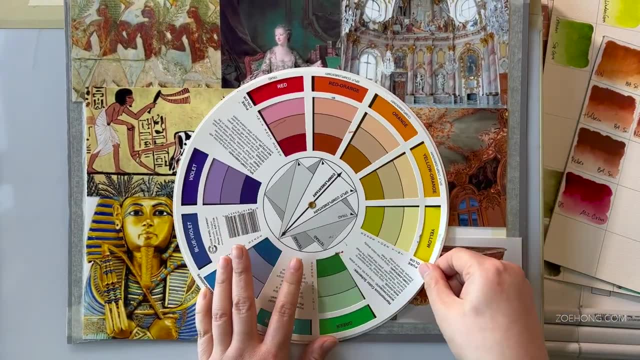 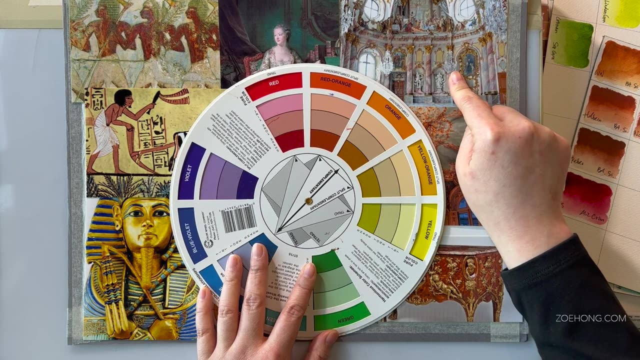 They're in here. You see how similar they are, These colors in here And this gold, while it's not, you know, bright, bright yellow, it's more yellow orange because it's gold, especially in here. And so when I started kind of analyzing the colors that I liked, 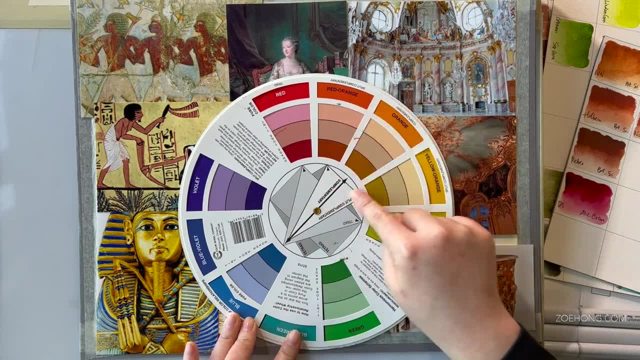 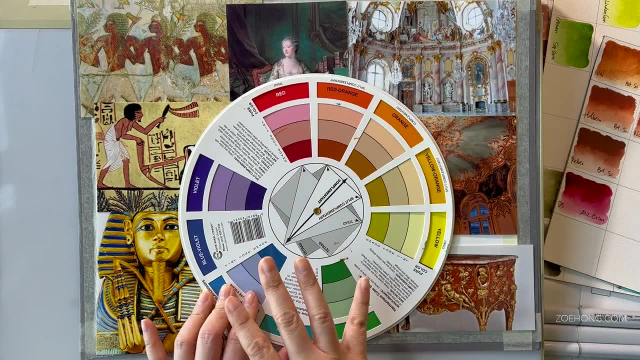 I put together this split complimentary color story. It's blue, so much blue. yellow orange, all the gold, and red orange all the browns, And that became the basis of my color story. Okay, All these golds. 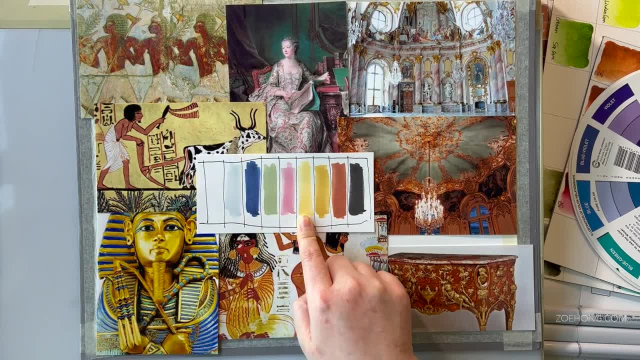 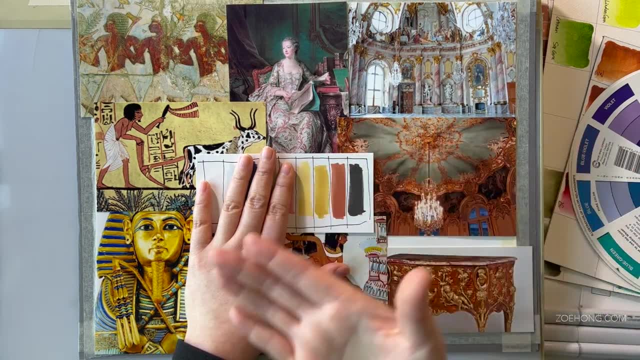 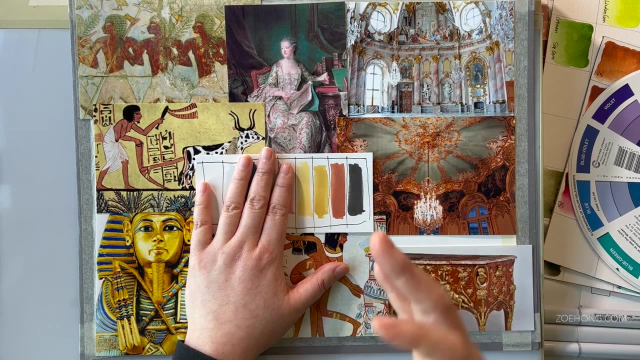 I put in a light base, I put in a baby gold- this in here- but also because I wanted to punctuate all this warmth, I really wanted all this like warm undertone family. I didn't want a lot of white and gray, like none of these, like light, chalky things. 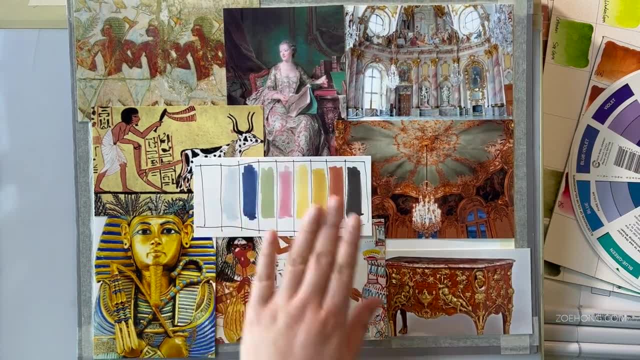 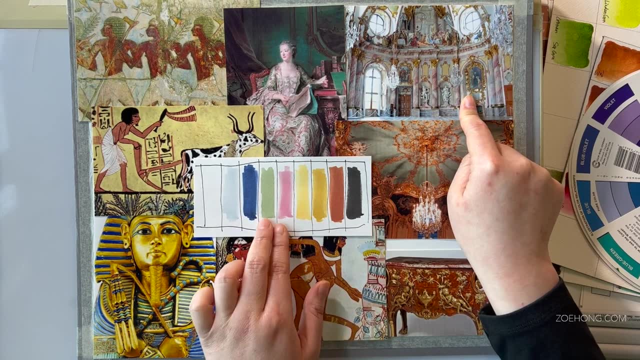 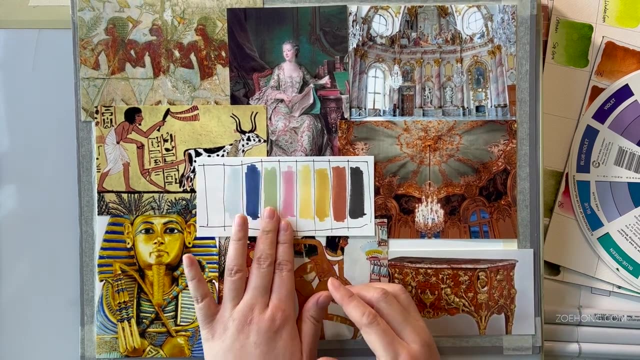 Although that is kind of also reminiscent in Baroque, And I definitely wanted the blues, this blue and the Rococo blue And these are just Pop colors. you know, I think pink is very popular in Rococo, It's like, but it's definitely. these are pop colors and this I was always on the fence about it. 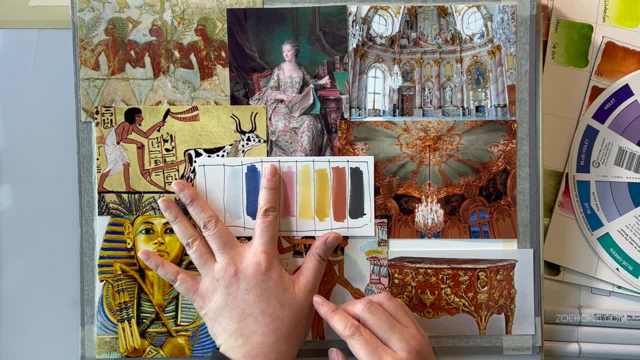 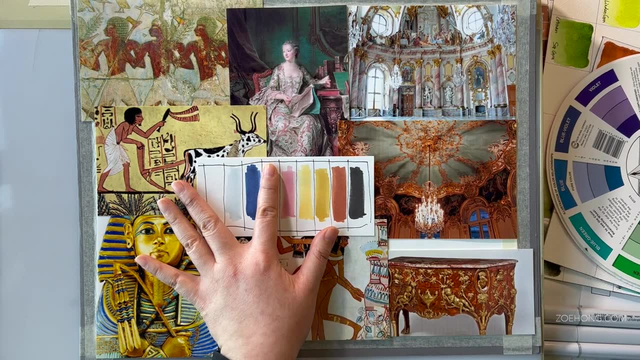 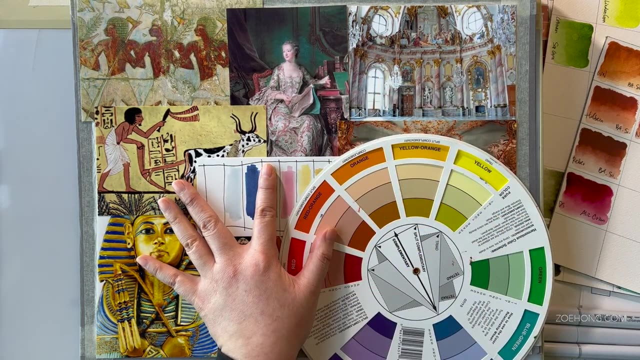 And now that I look at it again, I really want to take that green out. I think the pink is really important in there, though, But see, I could almost see myself tipping a little bit warmer so that it stays red orange. 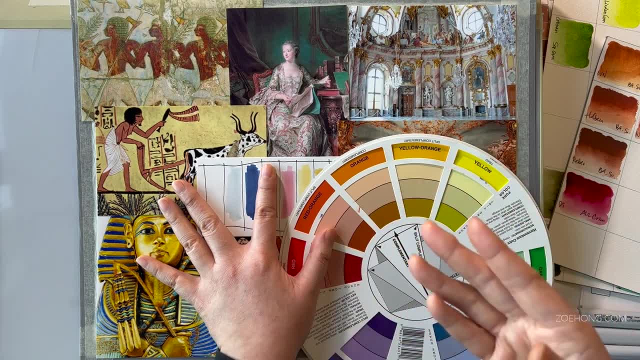 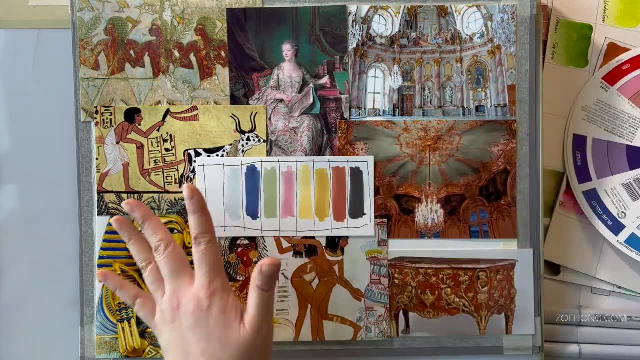 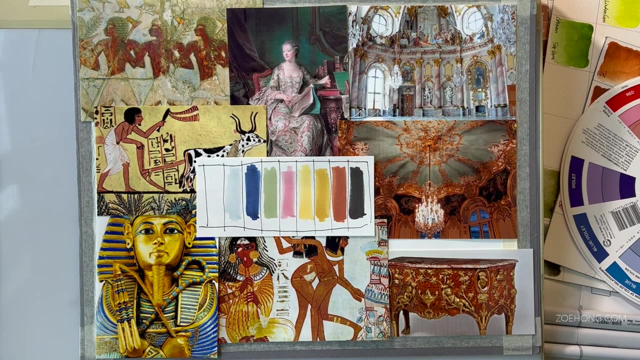 And it really is to say sort of like varying levels of warm With the complement of the blue, and that's how I started developing a color story based off the inspiration images that I put together. so it's the knowledge of all the other color lessons that I've already posted. I'll put the link to the playlist. 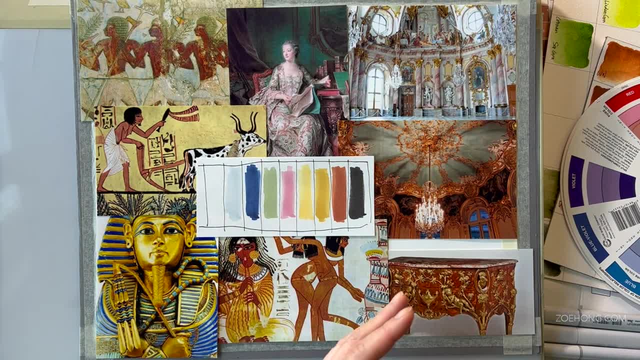 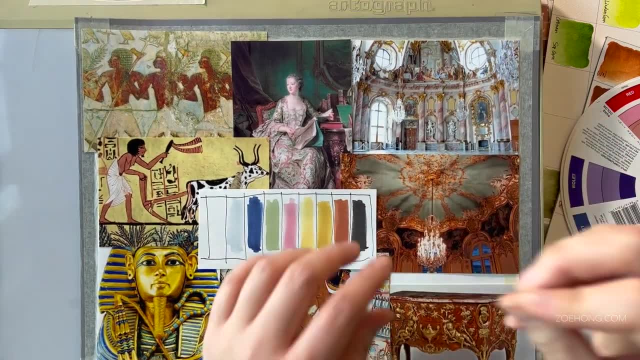 in the description box below. Also, understanding undertones helps you figure out what the base Colors are for all of these neutrals. OK, these are all. these color lessons are building blocks to a foundation of color knowledge to reduce your trial and error. 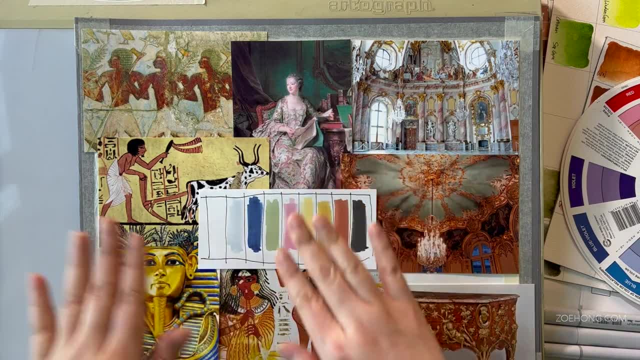 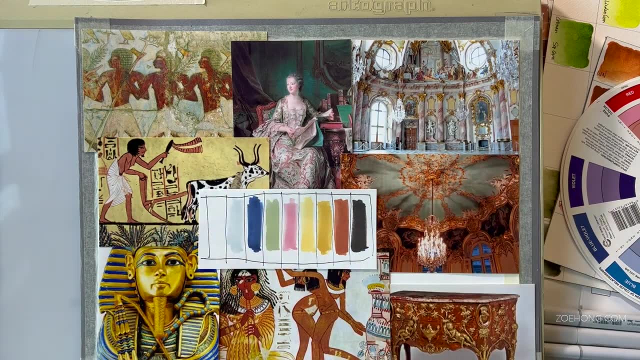 you know, to reduce the time you spend making one hundred color chips- And you know, a thing you could have done is to make color chips of all your favorite colors and kind of put them together and play around. But that takes a lot of time and effort and we move fast in fashion. 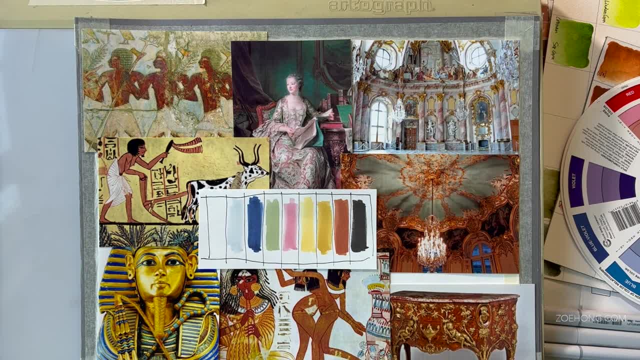 All right, That's all I can think of to say about undertones. Please heart this video if you learn something new today, Share, subscribe. drop me all your color questions in the comments below And I will see you in the next video. 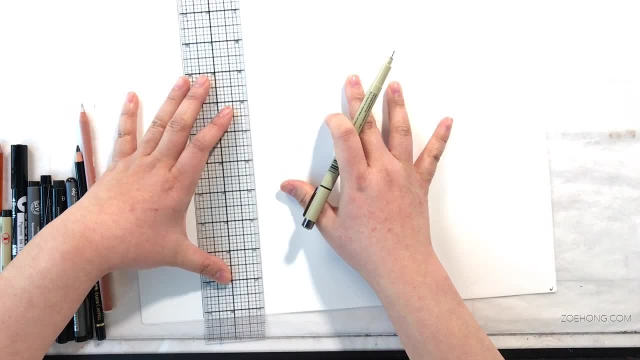 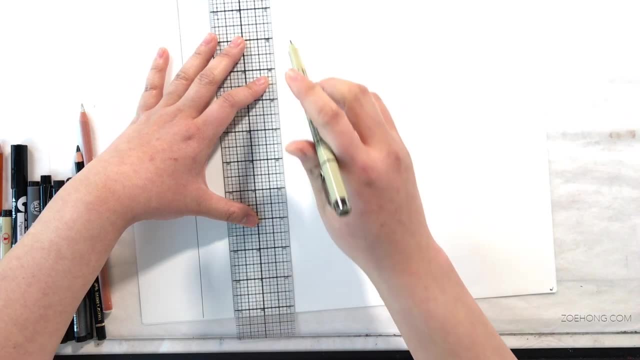 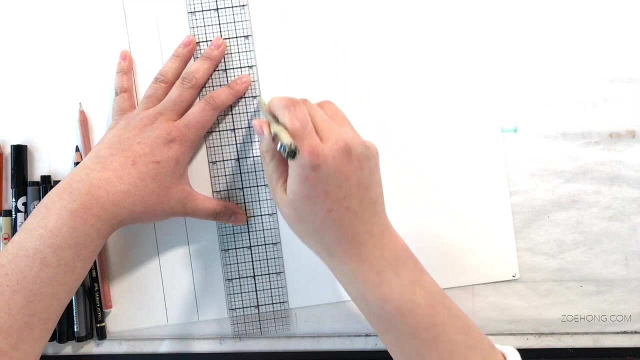 Hey everyone, welcome to a brand new series on Fundamental Fridays. This series, we're going to go over how to illustrate black textures. It's really a matter of Figuring out shades of black, just like you would figure out shades of red for illustrating a red texture. shades of blue for illustrating a blue texture. 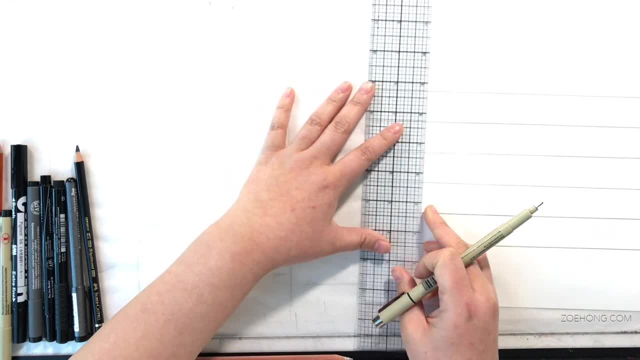 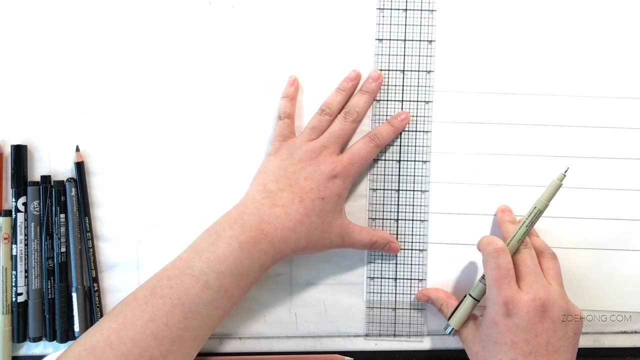 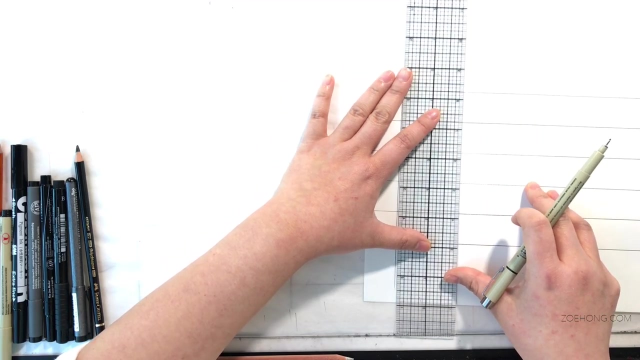 The only thing that makes it more difficult is the differences in the shades of black are so much more subtle than differences in shades of yellow or green. Right And yes, you can, And I do, use dark grays as part of the shades of black. 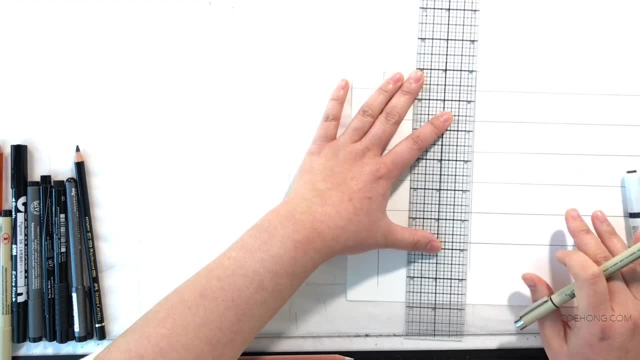 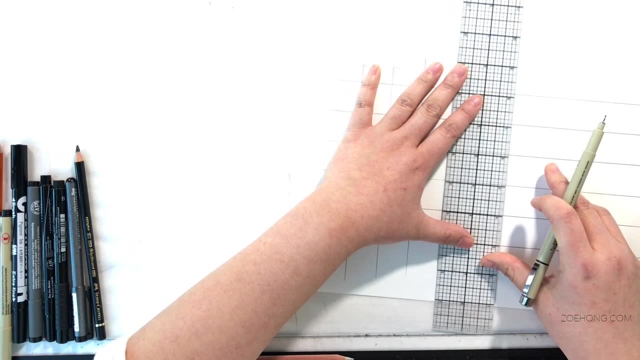 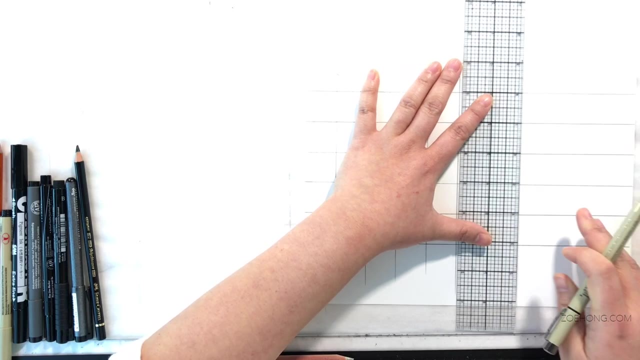 But you have to get really choosy about which dark grays you use, because there's a line Between charcoal gray and your darkest grays and light black and you never want to cross that line. you want to stay firmly in the light black camp. 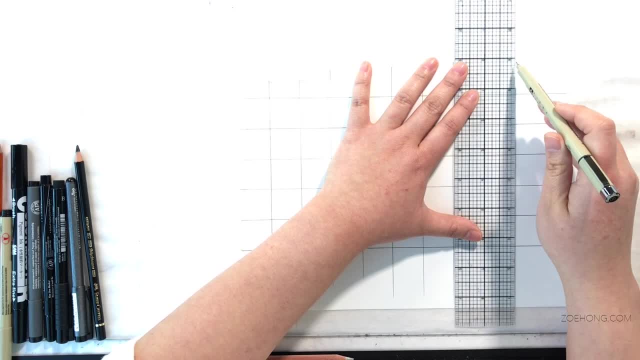 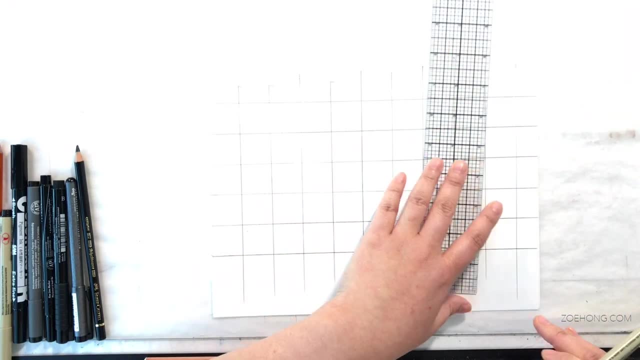 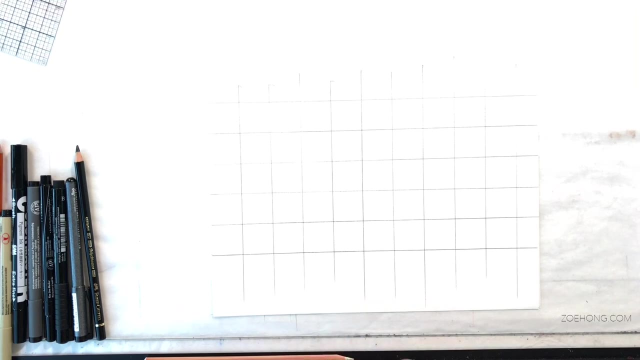 And I'm going to show you more about that as I start pulling out my markers and showing you what these colors look like. But I want to preface all of that by saying I have deliberately over lit this video, like you can tell, like there's so much light pouring all over my studio table right now. 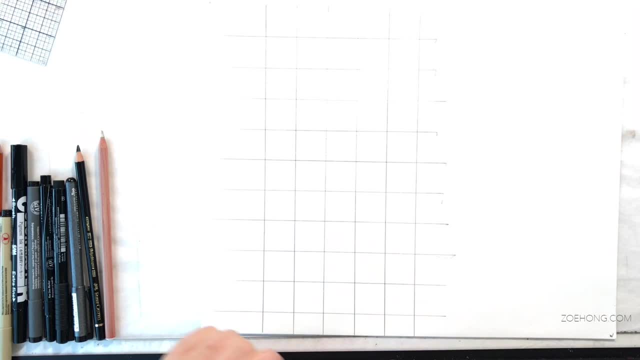 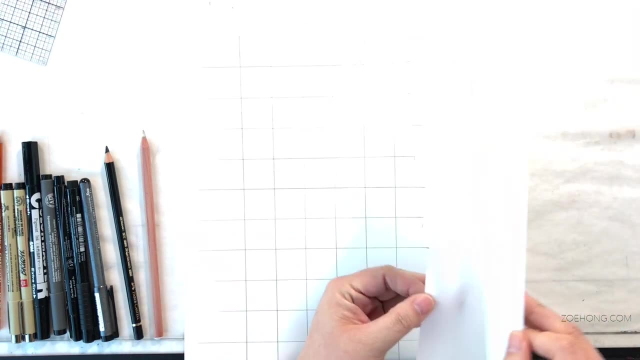 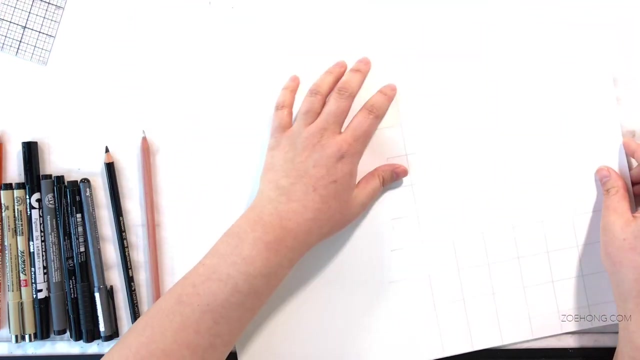 And I did that on purpose, so that you can really see the differences in all the shades of black that I'm about to show you. Now, when you see these blacks in person, the differences are going to be going to be more subtle and everything is going to be darker, because this whole 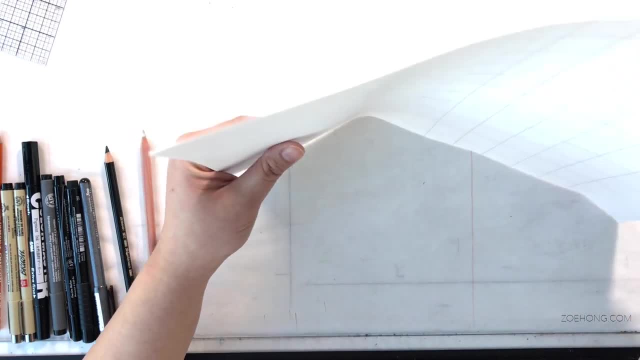 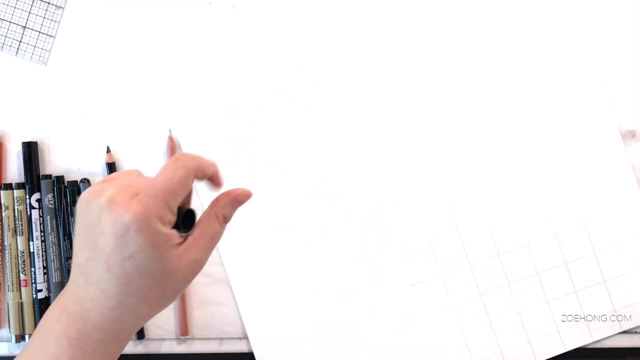 video is purposefully overexposed. OK, so keep that in mind when you're shopping. It's like, oh, it didn't look like this in Zoe's video. It's like, no, everything is going to be darker, The differences are going to be more subtle. 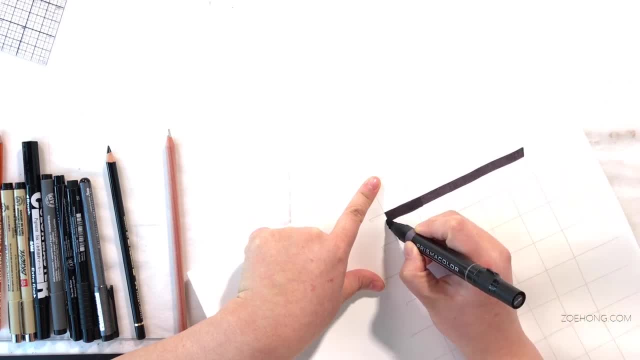 But you know I was trying to accommodate all the different computer and phone and tablet screens out there that you guys are going to be watching This video on and really make sure that you guys can see the value and tone differences that I'm talking about. 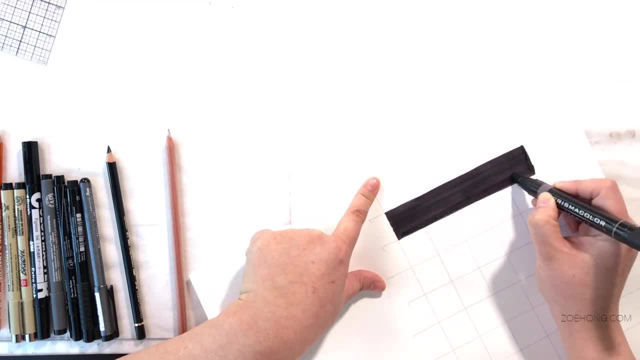 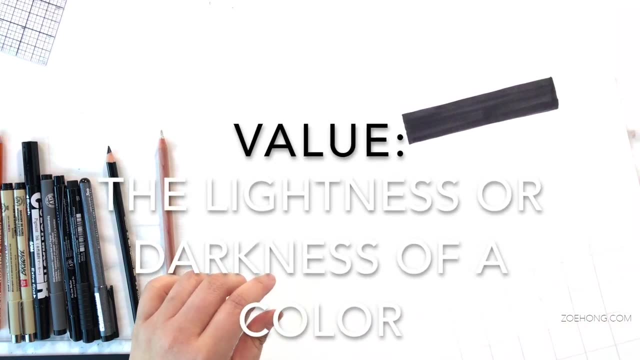 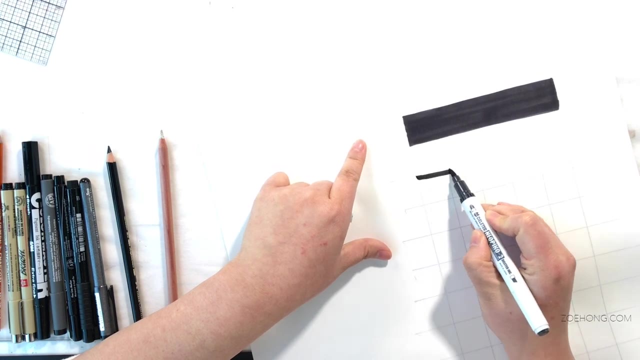 Now I'm going to use these words a lot in this video series- value and tone. So value means the lightness or the darkness of a color. So when I say look at all these values, it means look at how all these different. 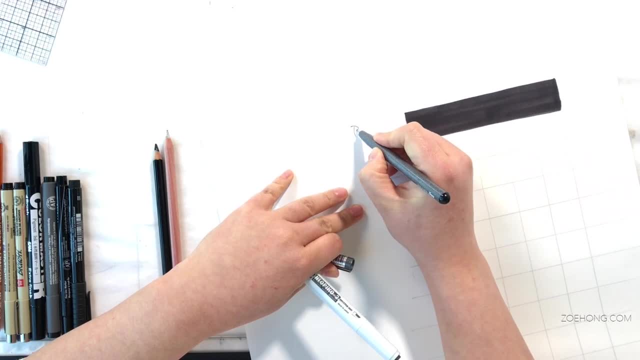 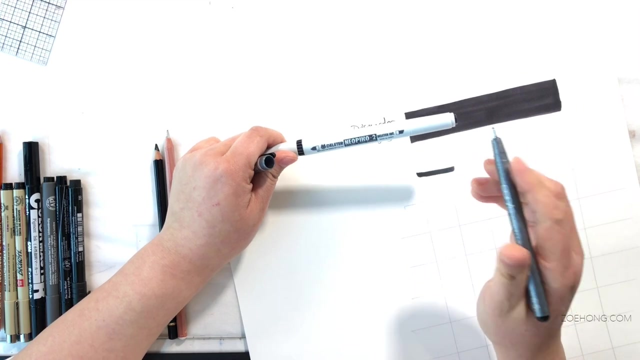 colors. some are light and some are dark. You have all these lightnesses and darknesses of shades of black, And when I talk about tones I mean undertones, Just like any other color. I mean you can have a green and you can. 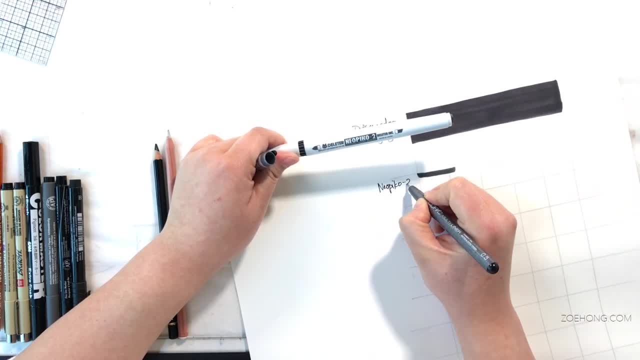 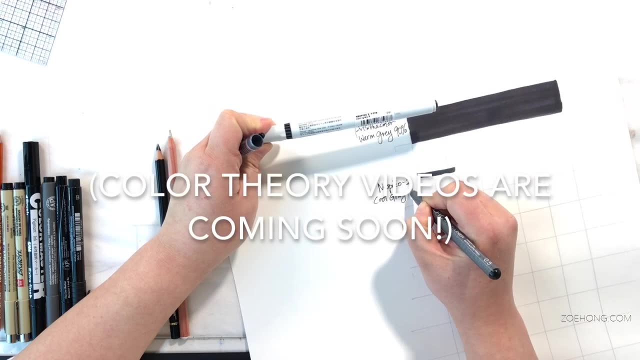 have greens that have blue undertones, more bluish greens, not so blue, So they look turquoise, but you've seen them right: Cool greens, Bluish greens. And then you have greens that have yellow undertones, you know, warm greens. 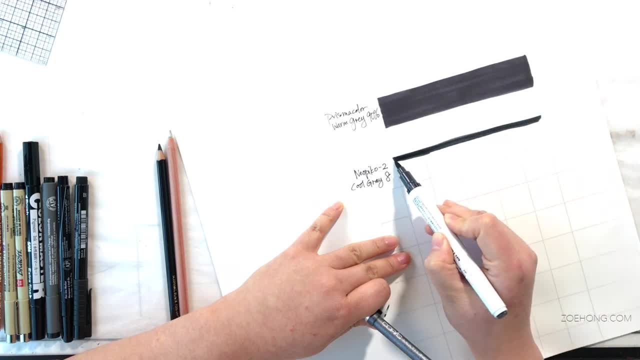 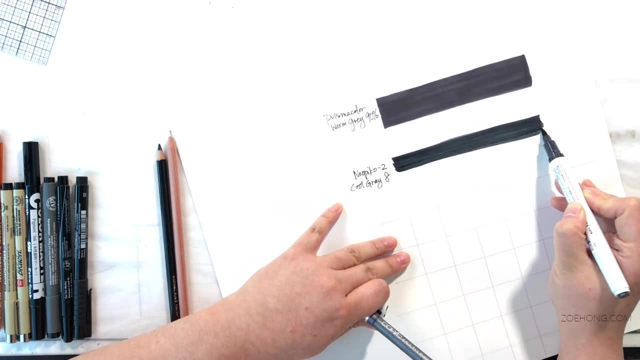 you know, not quite full chartreuse, but the warmer greens And, just like that, blacks also have different undertones that I'm going to talk about. You ever go marker shopping and you see how Copic has a warm gray, a natural gray, a cool gray. 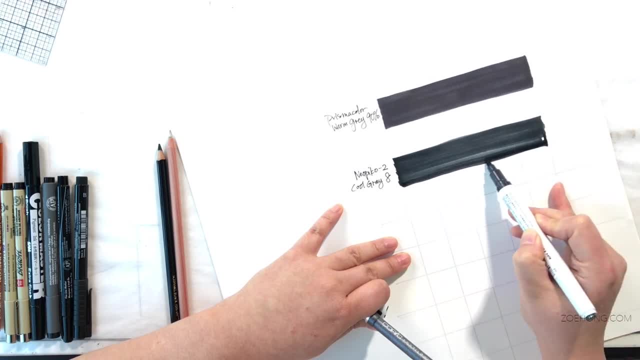 I think they have another one too, like they have a bunch of different kinds of grays. Prismacolor has a warm gray, French gray, neutral gray and cool gray that I can recall. So these all have these different gray undertones. 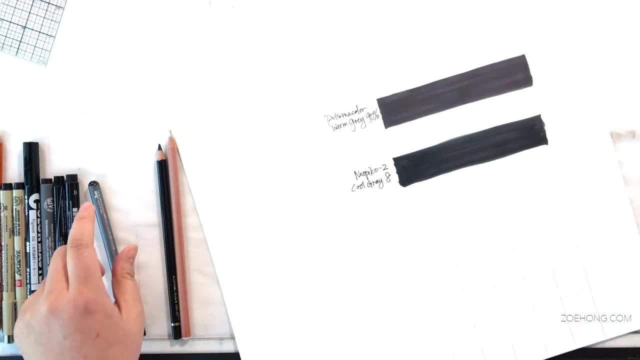 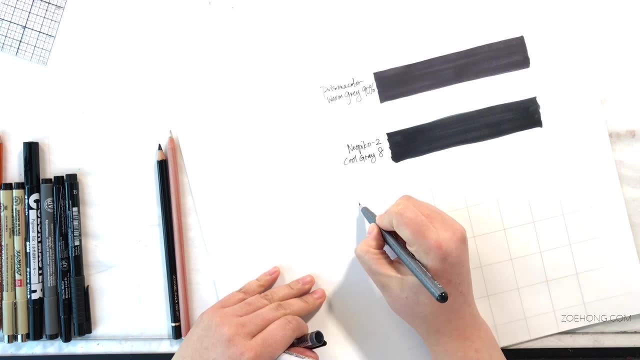 And when we start hitting the black markers, the same is going to be true. You're going to the lighter the black is, the more of an undertone you're going to see. And then I'm going to show you some super black markers where there's not a tone, it's just black, black, black, black. 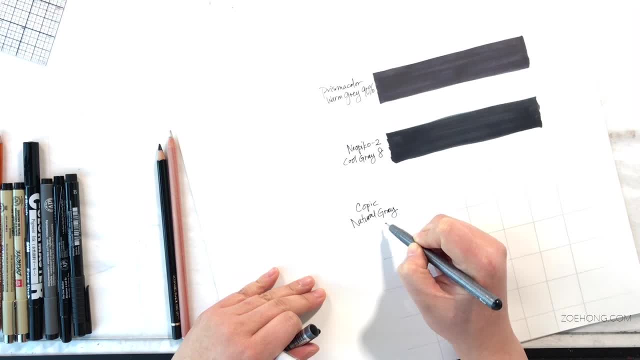 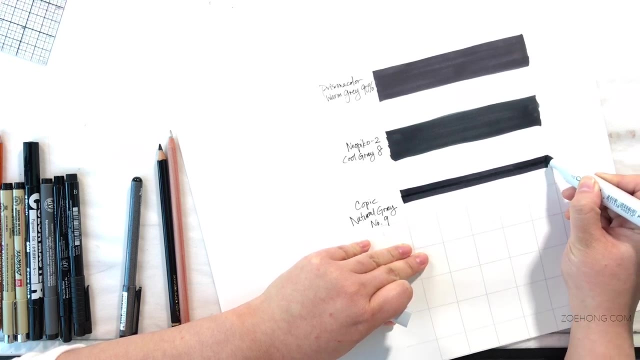 black. So much black, serious black. Like serious black. Isn't that a Harry Potter character, Anyway? So what I'm doing now is I'm laying down bars, test bars, of the darkest grays I have in my marker kit, I have in the Prismacolor sets. 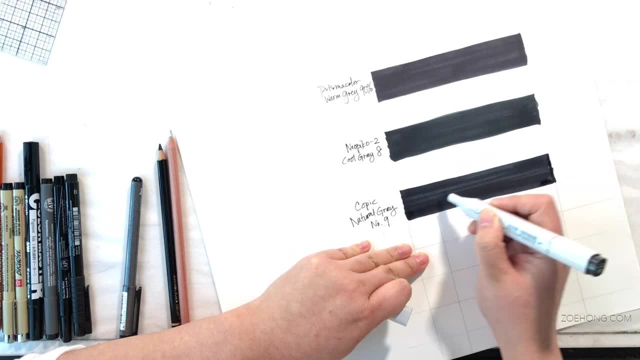 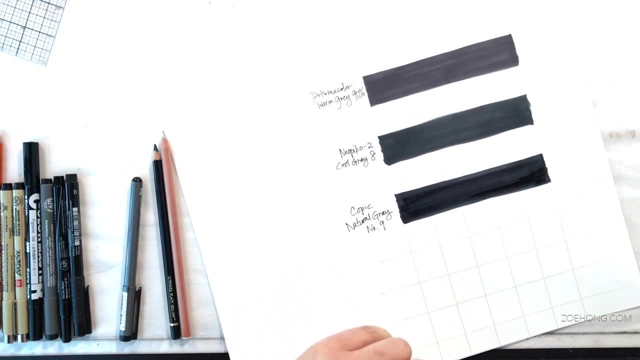 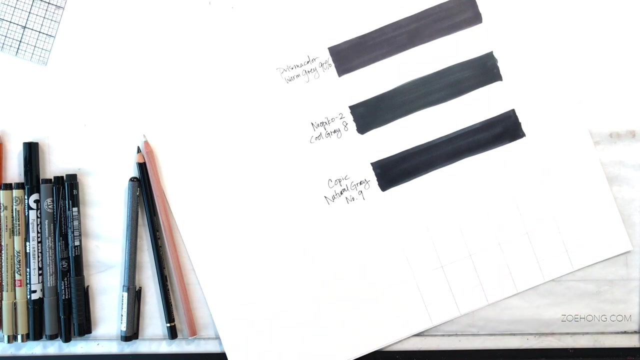 I have a full set of warm grays and a full set of cool grays, So I made a bar for the warm gray And in the Copics I have natural gray nine And I have a full cool gray series. And the Neo Pico 2s is a marker set that I bought in Japan that I still haven't. 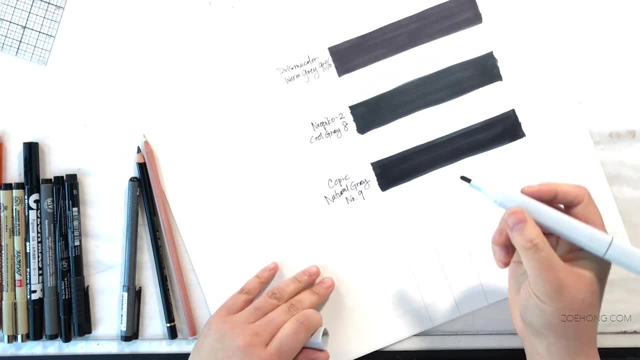 gone around to testing. Yeah, I'm always testing stuff And you know, nobody is telling me what order I need to test things in, So I just test them. I just test whatever looks exciting to me at that point in time. 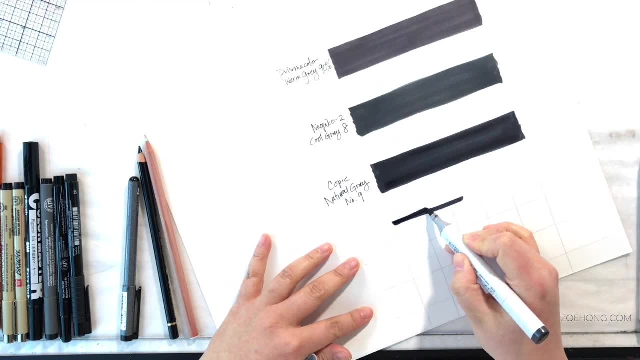 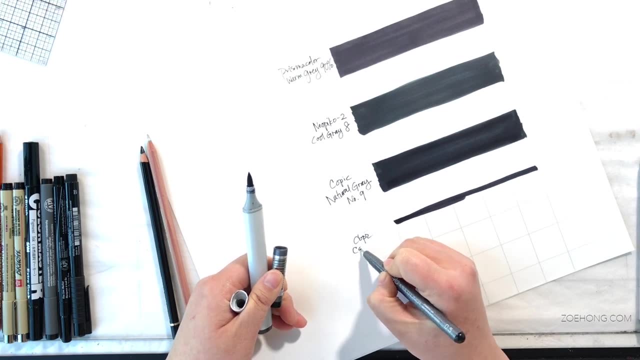 And these, unfortunately, have been kind of pushed to the side, But I pulled them out for this demo and I pulled the darkest gray that was in the set. So that's their cool gray eight, And I don't know if they have, you know, a gray nine, ten, eleven, whatever. 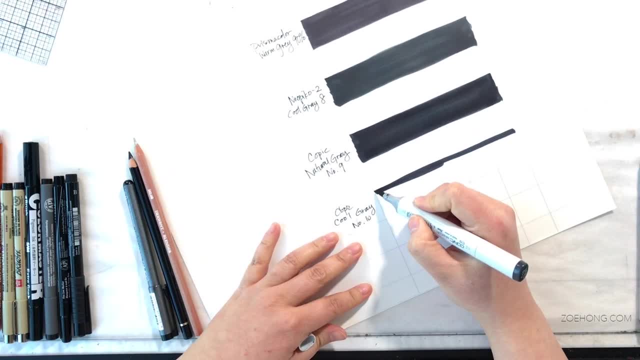 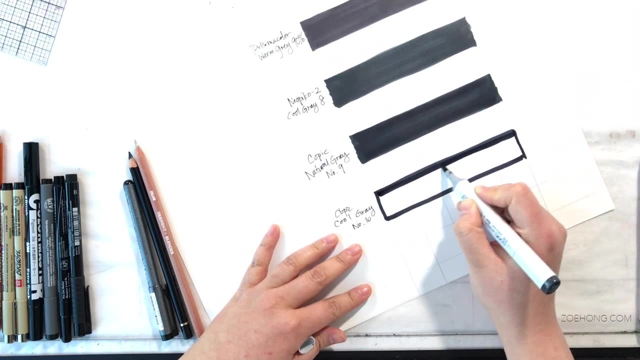 But this is the darkest that was there And when I look at it, the value of it is comparable to the warm gray ninety. So I'm rolling with it With the Copics. their darkest gray is the ten, But I don't have a natural gray ten. 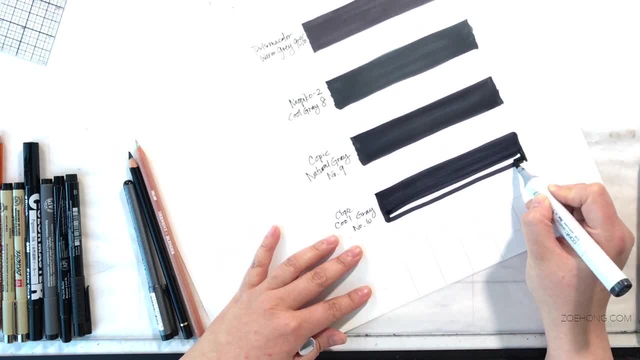 I have a cool gray ten, But look here you can see, as I'm laying down the color, that the values of the natural gray nine and the cool gray ten are very similar, So I'm just rolling with it. I'm going to assume that if I had a natural 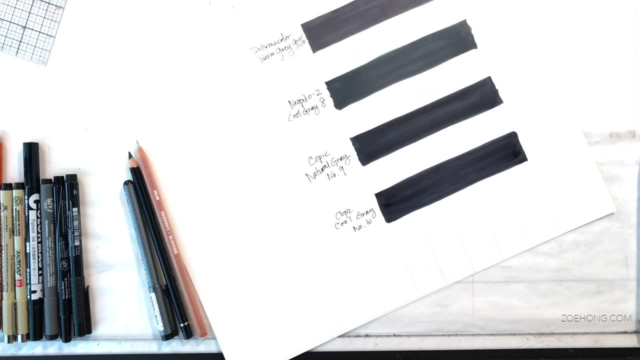 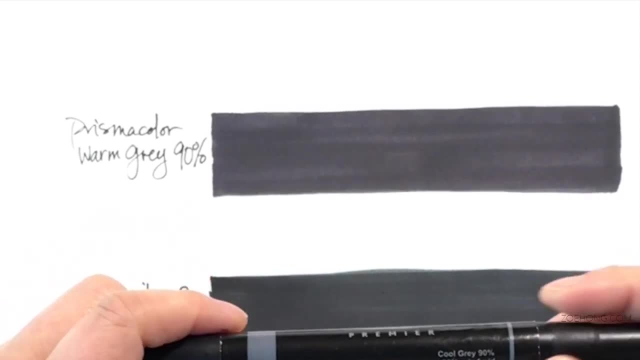 gray ten. it would be slightly darker and that might be even a little bit better. So I'm going to test out my blacks and grays on these main four bars, But I want to show you just a couple other really dark grays I have in my kit. 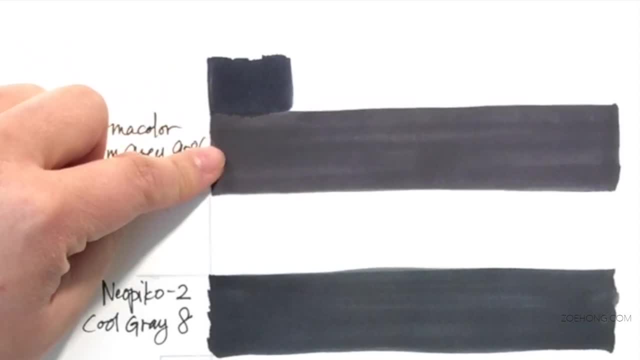 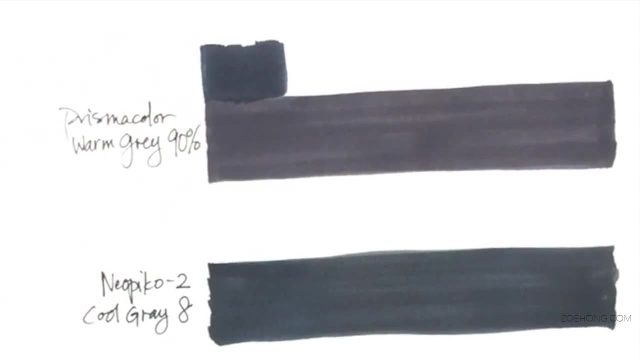 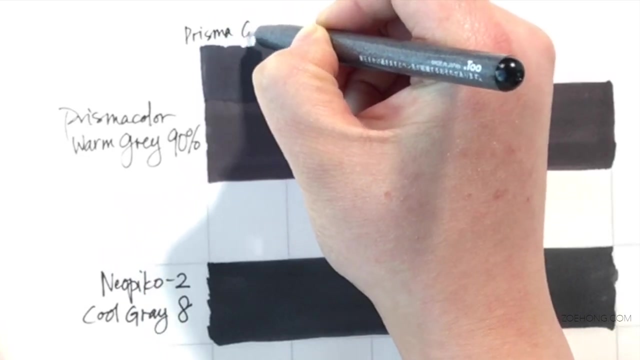 This is the Prismacolor cool gray in ninety And I don't love this as a light black. It has such a cool undertone that it very much looks like charcoal gray to me, And so I'm not going to use it. The warm gray- because it's got. 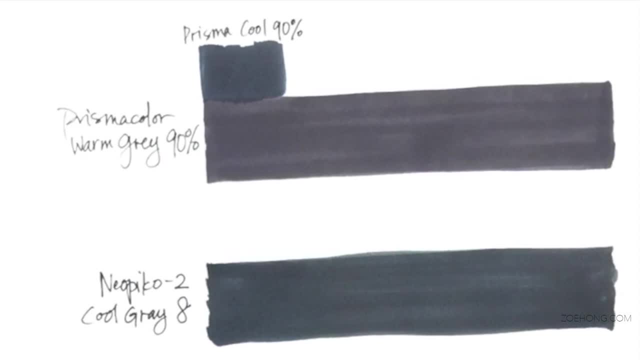 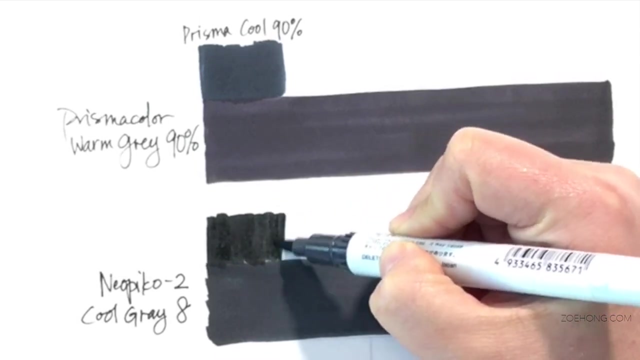 that brownish, purplish undertone. it suits for warm, light blacks. This is the Neopiko two neutral gray seven And you know the value is a little bit lighter, but kind of like the Copic natural nine and the cool ten. 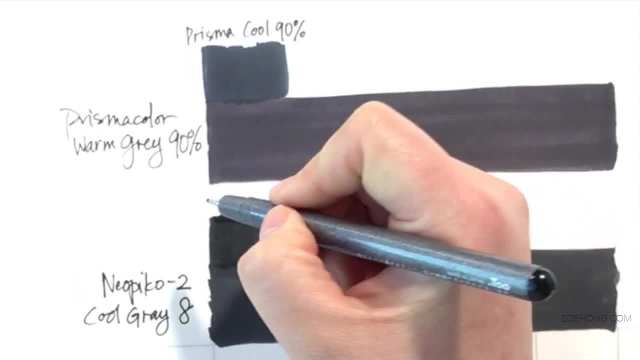 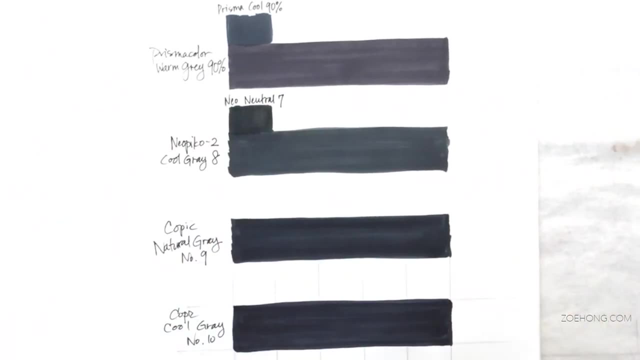 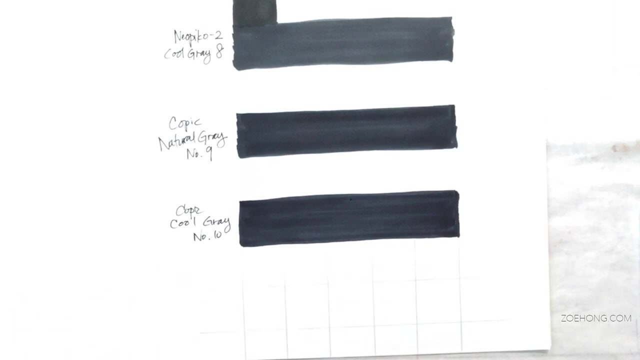 The difference is minimal And you can see the undertone is definitely much more neutral. What I want you to pay attention to right now is how you know not all 90 percent grays from one brand are the same in value and not all the 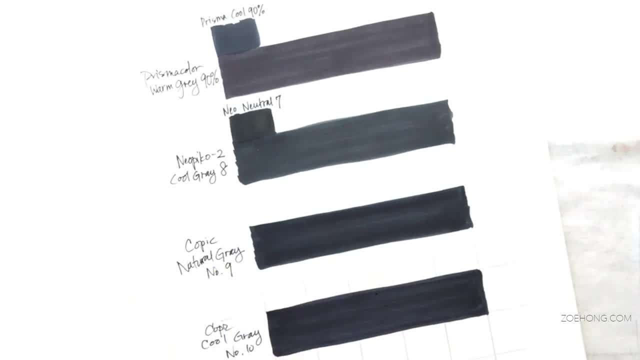 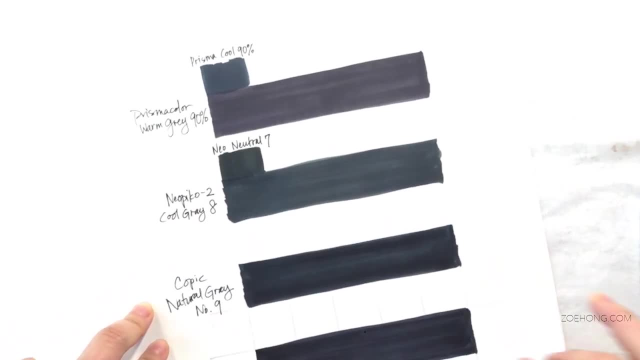 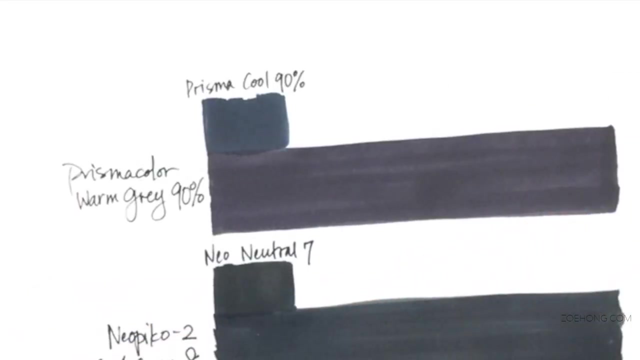 gray nines and the gray tens from another brand are the same value. You have to really look at each individual marker and test it out on its own. Now let's get started with our black markers. First up is the Prismacolor Black PB98.. 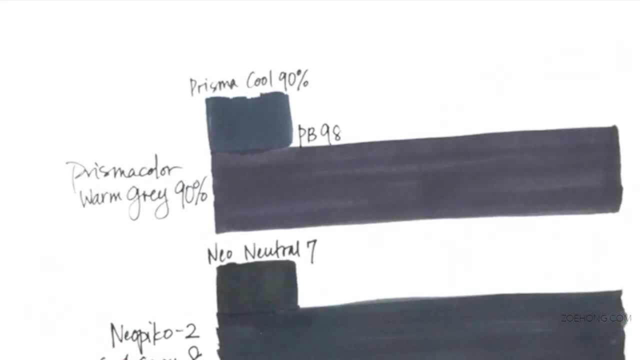 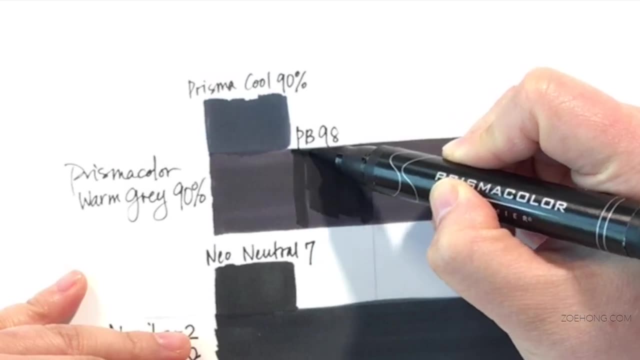 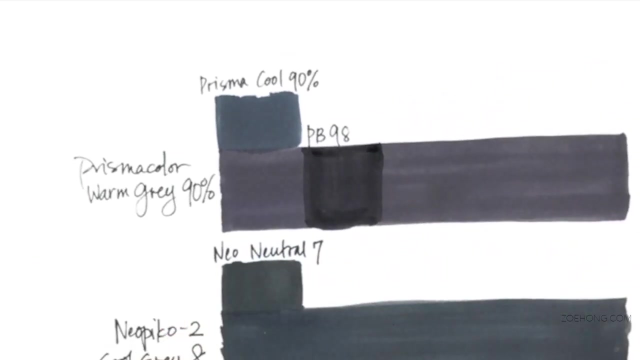 And I'm going to layer it on top of the Prismacolor Warm Gray 90 because that's how I'm going to use it. any time I'm testing media, I try to test it as closely to how I'm going to use it in my final illustrations as much as possible. 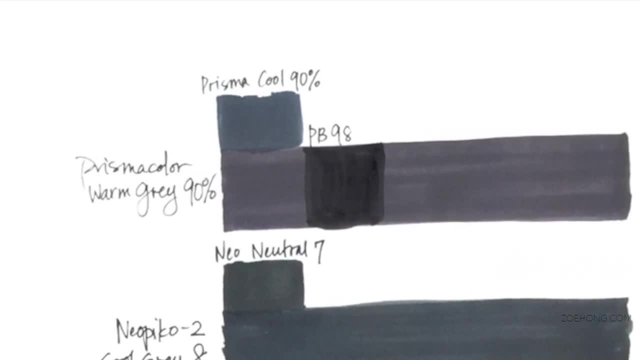 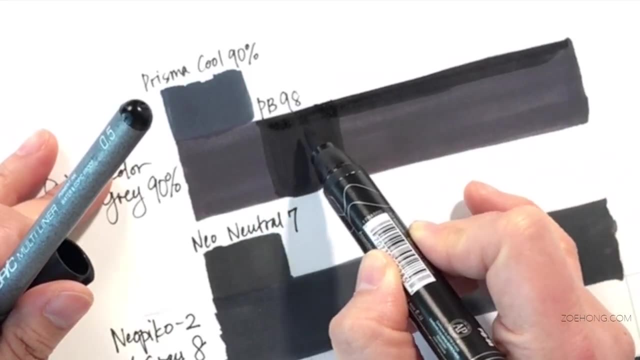 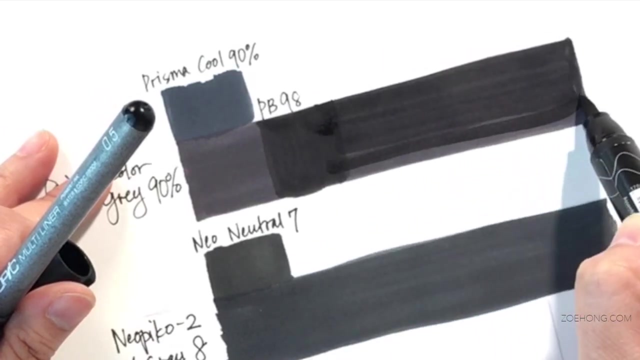 And when I illustrate, let's say, a black blouse, I will have a light black base fabric color and I will use a dark black to do my shadows. And so let's pretend I use the Prismacolor Warm Gray 90 as my light black. 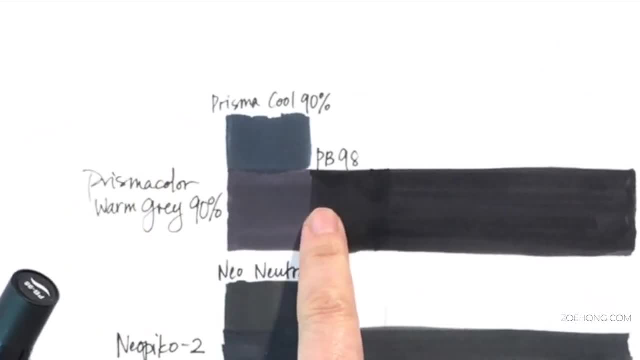 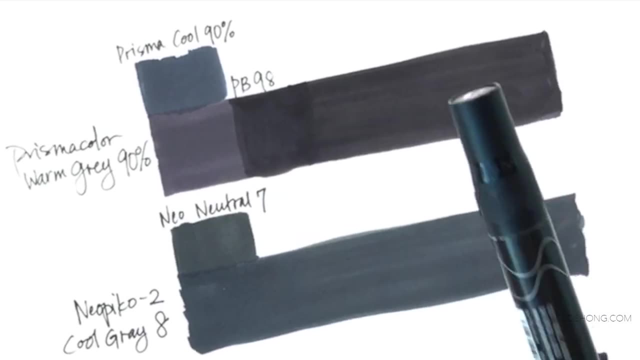 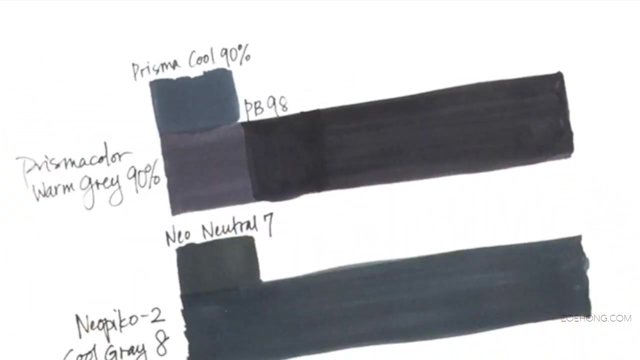 And then I would use my Prismacolor Black PB98 as my dark black, my shadow color, And I would layer the shadows on top of the base color. And so I'm going to test it by layering it on top. Prismacolor has a second black called Jet Black. 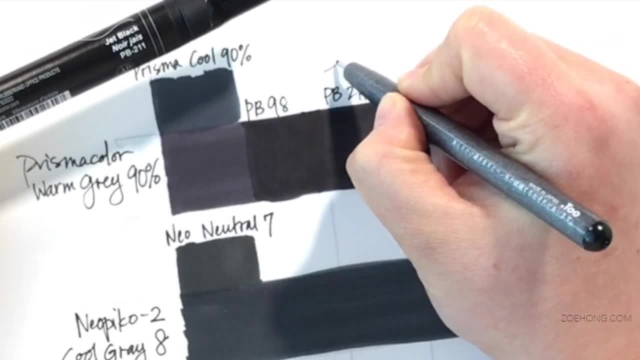 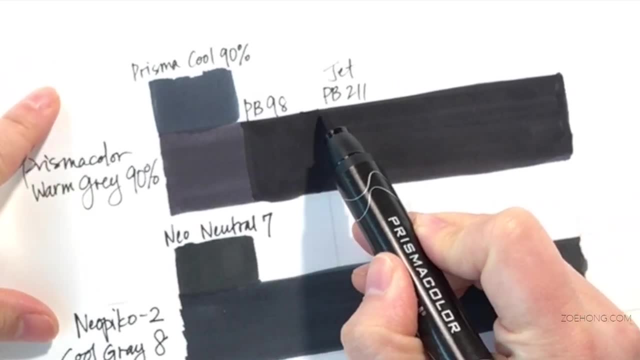 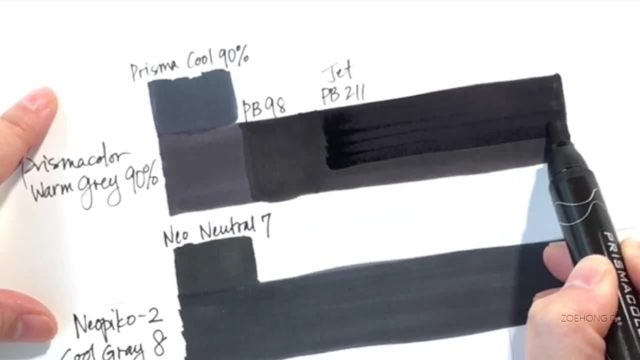 which is their PB211. And it is darker and a slightly warmer tone than the PB98. And I'm going to layer it on top. You have a few options here Because you have the two blacks. you could actually use the Jet Black as a second. 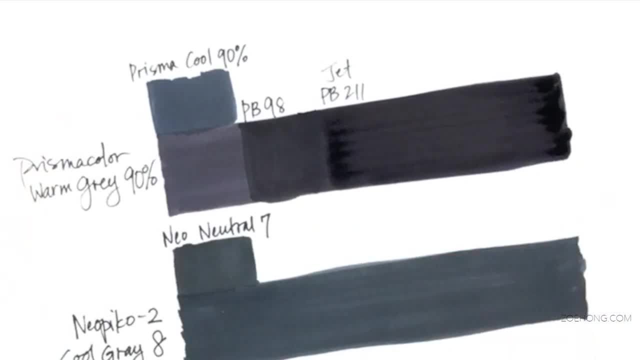 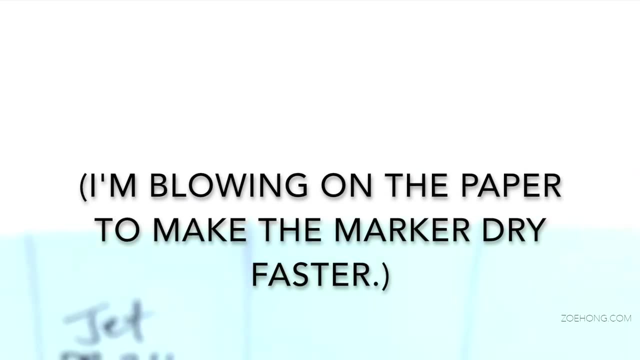 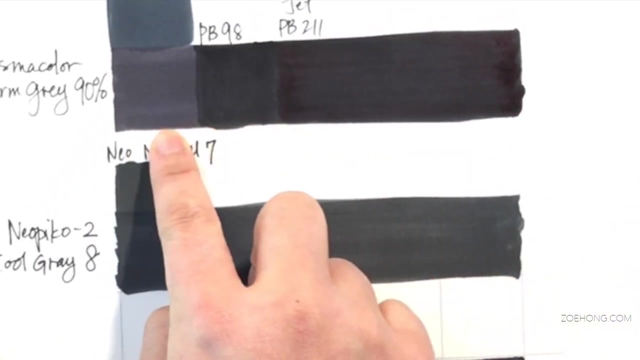 shadow. You know, if you watch my shading series, then you know that I like to have multiple values of shadow so that it looks more 3D, It looks more, it has more depth, interest. So you could do that. You can use all three of these colors. 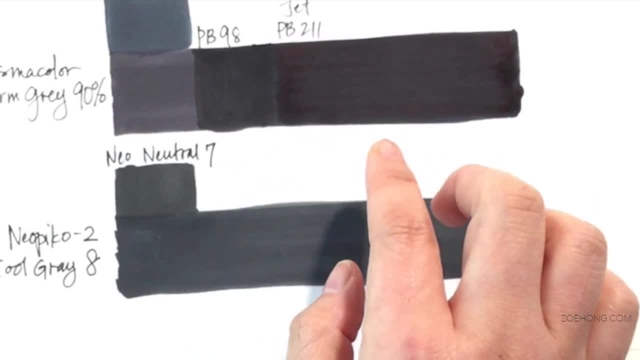 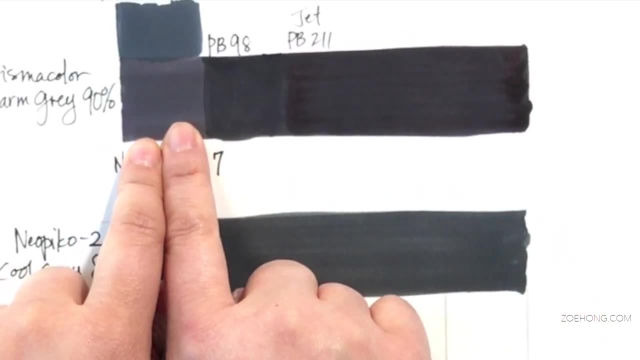 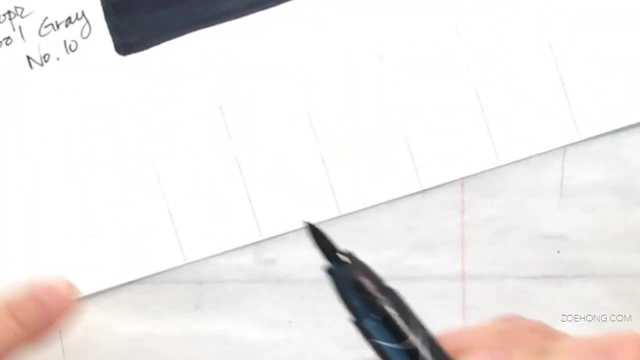 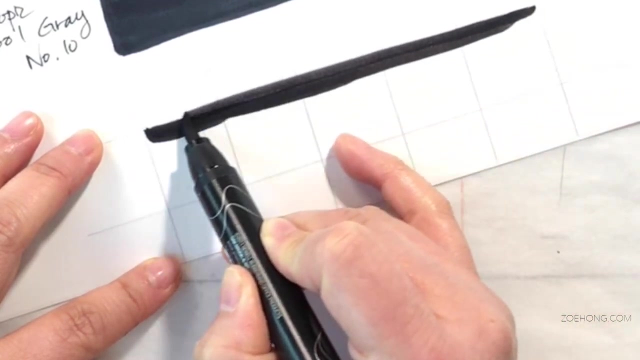 these blacks grays to create different shadows. or you could just use the Prismacolor Black PB98 as your light black, Because out of all the markers labeled black in my marker kit, the Prismacolor PB98 is the lightest black. 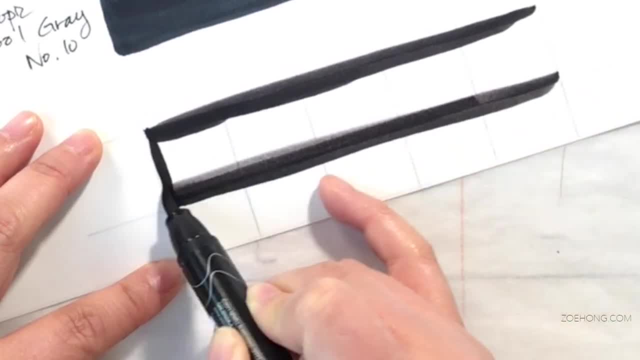 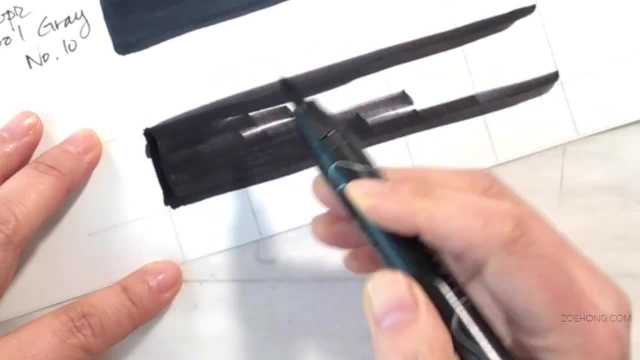 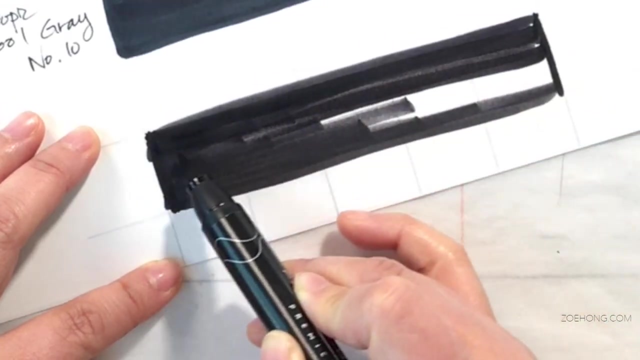 And so I often do use this as my light black. It again depends on the fabric that I want to render, or whatever it is you want to render. You've been to the fabric store, you've seen black fabrics and you know. 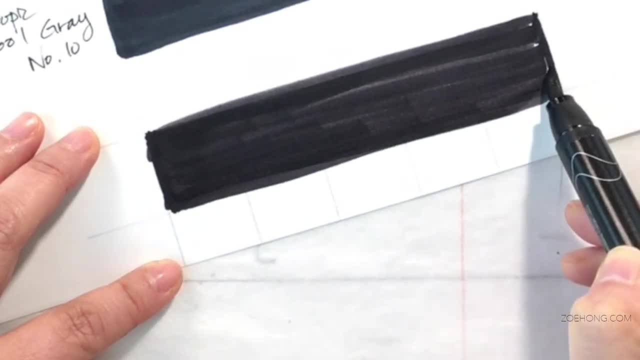 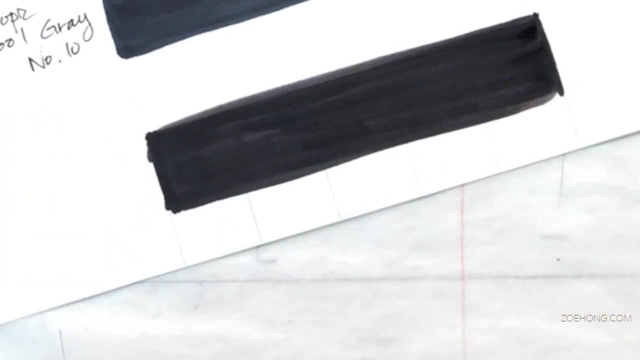 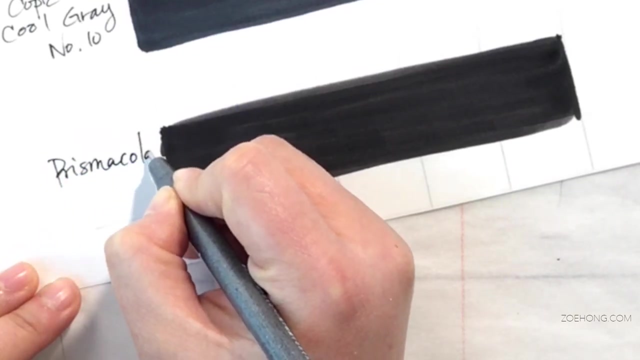 there are so many different values and tones of black fabrics. You know, when you look at black denim it's much more faded looking because you see a bit of those white weft threads poking through. And you know black silks that have kind of a soft shine. 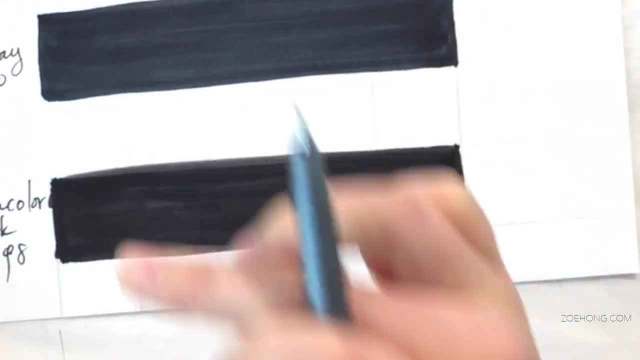 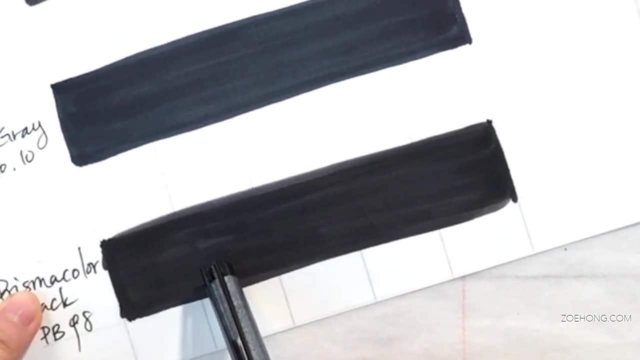 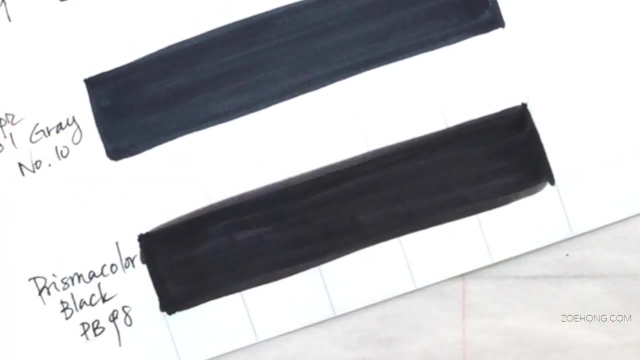 surface. those blacks tend to look much darker than black silks that have a matte surface like crepe. Crepe is not shiny And so it's. it looks more intense and dark and black, whereas charmeuse and satin. they have that glossy sheen on the surface and it looks lighter. 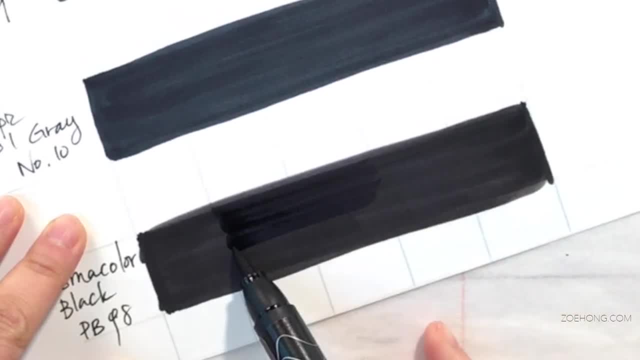 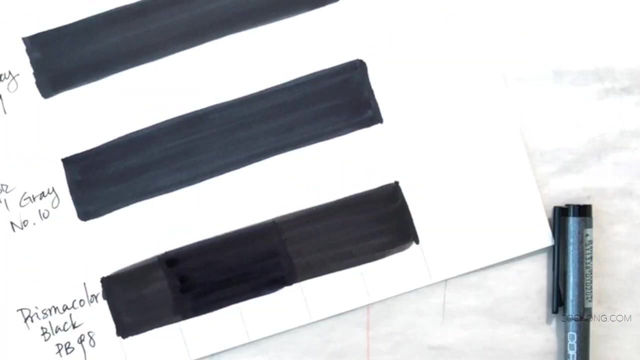 So I'm showing you guys all these options so that you can match your fabric, because sometimes it'll be black but it'll look really close to the darkest gray you have in your kit, And sometimes it's so black that you have to use this light black as your base color instead. 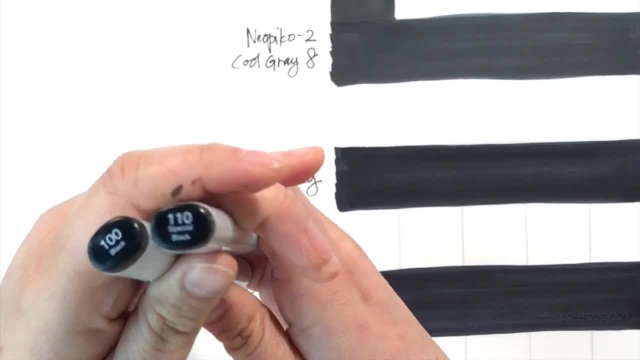 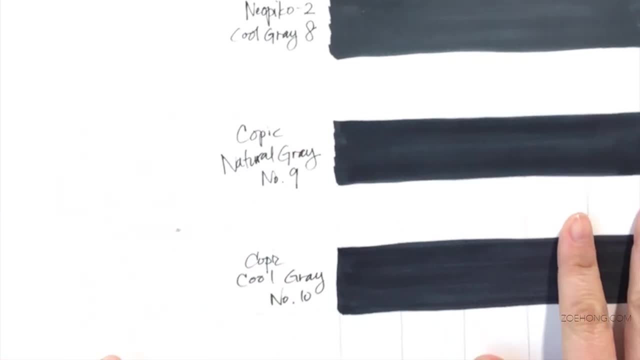 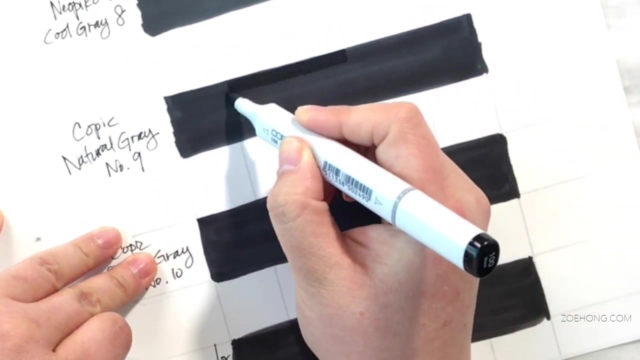 So here I have two Copic blacks. I have their black 100 and I have their special black 110.. And their special black. I don't know why that's so funny to me. Special black- it's special Black is a little bit darker than their regular black. 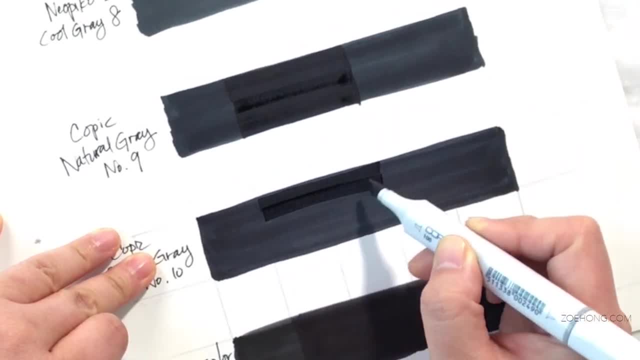 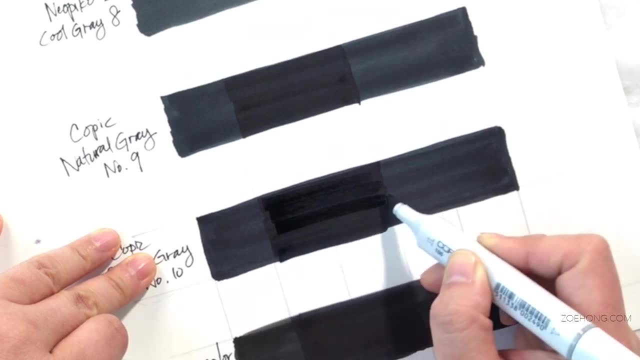 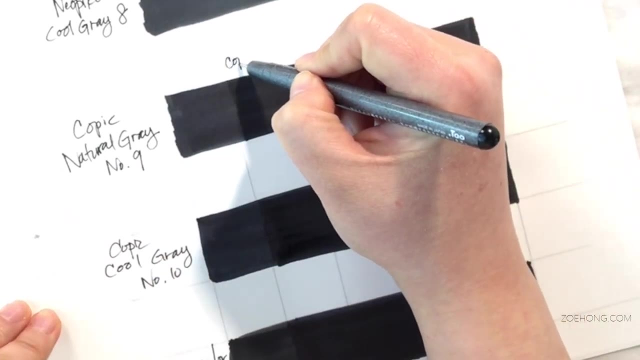 Although I have found that the value difference is not as intense as the value difference between the two Prismacolor blacks, but there's still a distinct difference. So here I am, layering the black 100 on top of the Copics that I have out here. 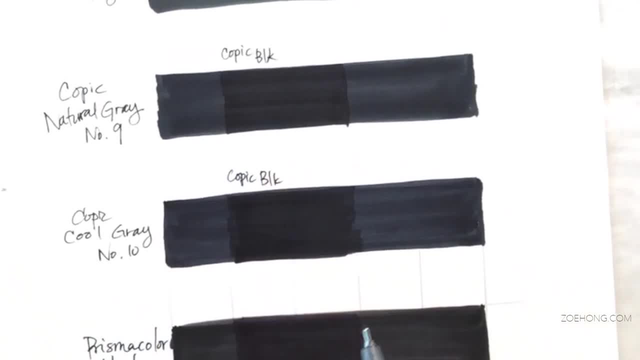 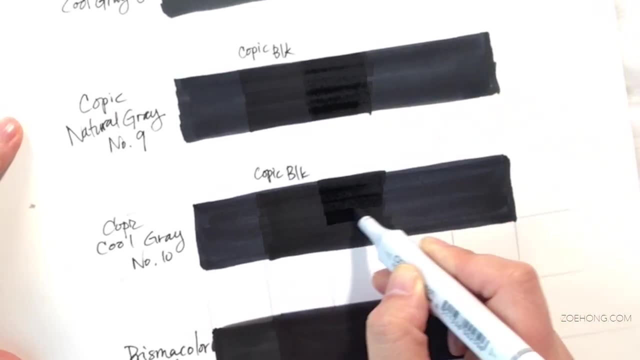 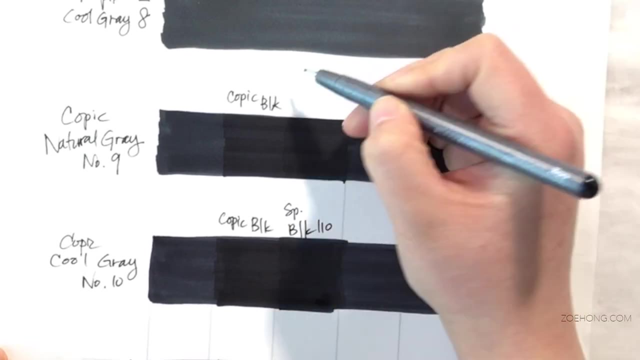 And you can see the value difference between the grays and the blacks: light black, dark black. And here I am layering the special black 110 on top, And now you are seeing this family of black colors. Now I'm layering the brands together right now, just for organization's sake. 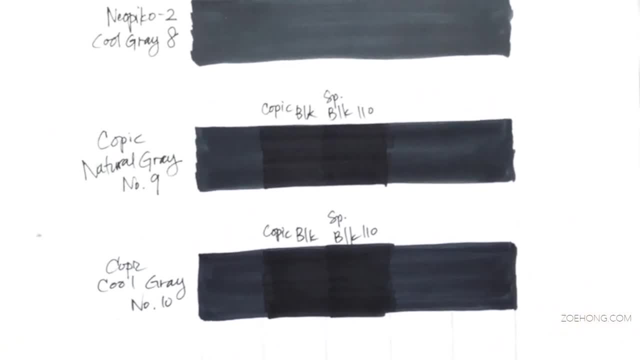 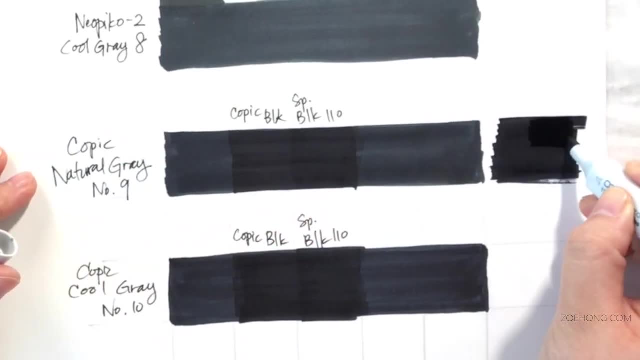 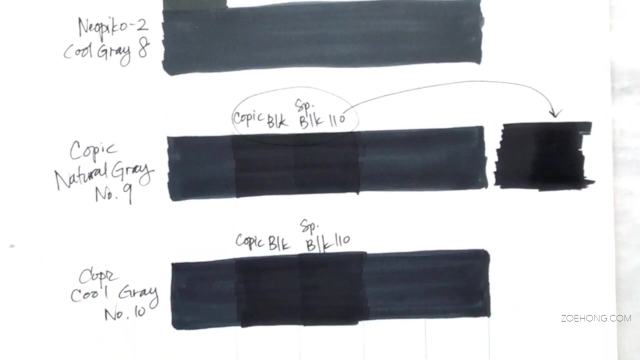 But people who watch my channel know that I mix and combine and overlap the colors in the same illustration constantly. Or you can just use the two Copic blacks as your light black and your dark black, without the grays. Here's how it looks, just the two of them. 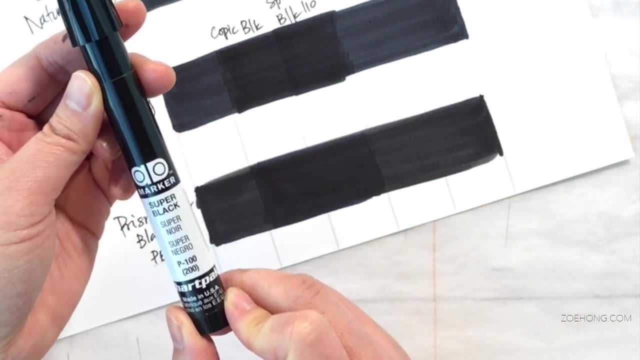 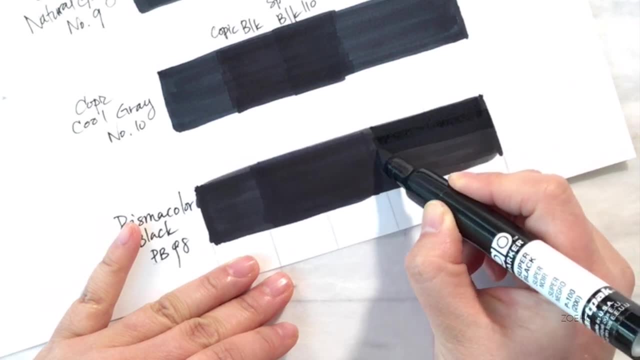 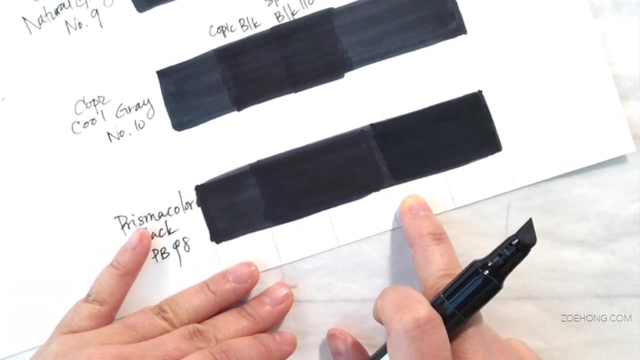 Now I'm going to bring out the big guns. This is ChartPak Super Black, and it is super black. Look at that. Look at that Prismacolor Jet Black. no contest, I mean look at that Whoo. 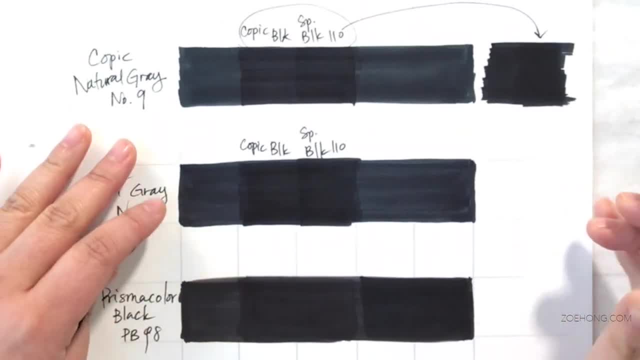 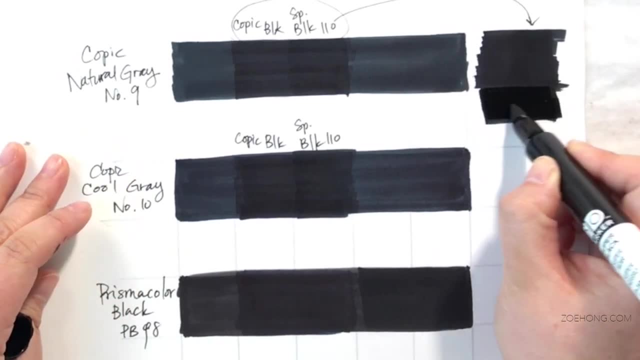 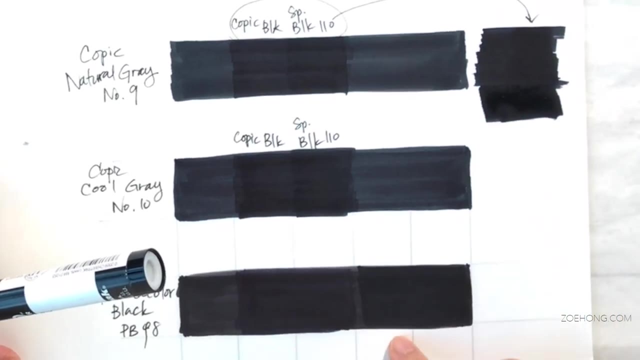 Hi, Super black is super. Always make sure that you're looking at the color after your marker has dried. I love ChartPak brand because they smell. They've got that awesome like marker stink, you know, but I'm kind of weird. 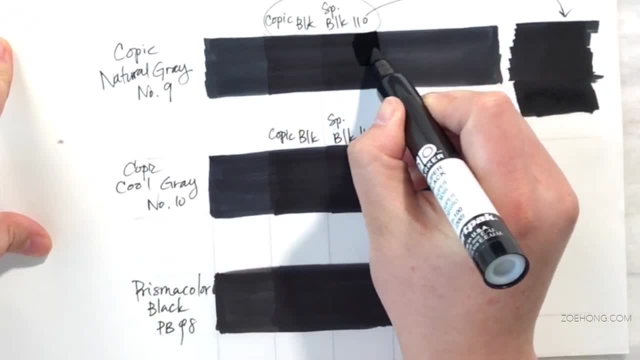 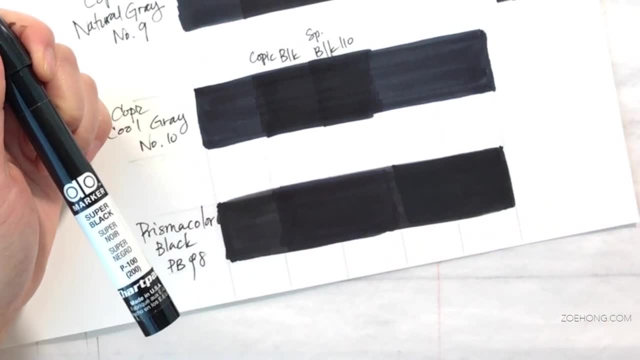 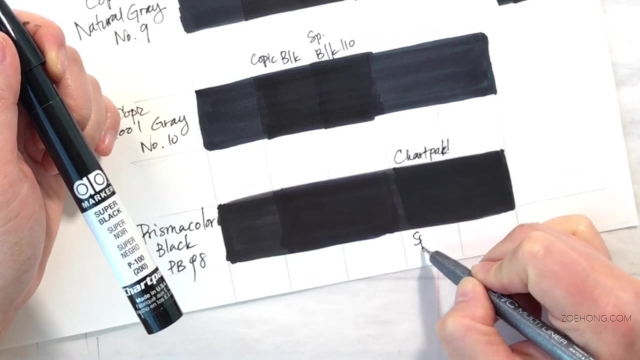 I also love the smell of gas stations and cigars, Anyway. So this is ChartPak Super Black And you know I really love ChartPaks. They they perform super well and they're not really on the expensive end for markers. 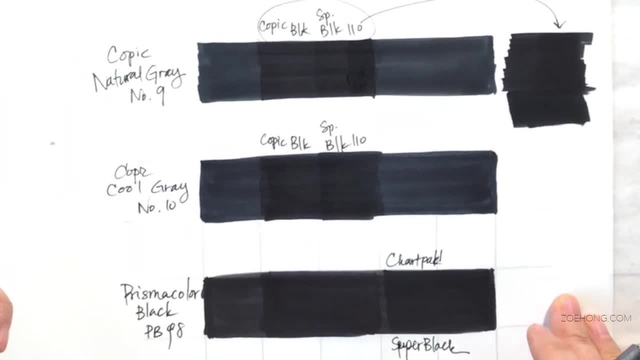 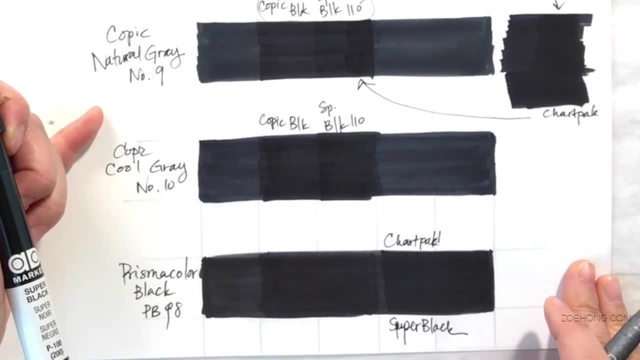 I am going to be doing a marker roundup video as my next visual playlist on Whatever I Want Wednesday coming up in the next few weeks. So stay tuned for that. But in the meanwhile, yeah, go check out ChartPaks, They are. 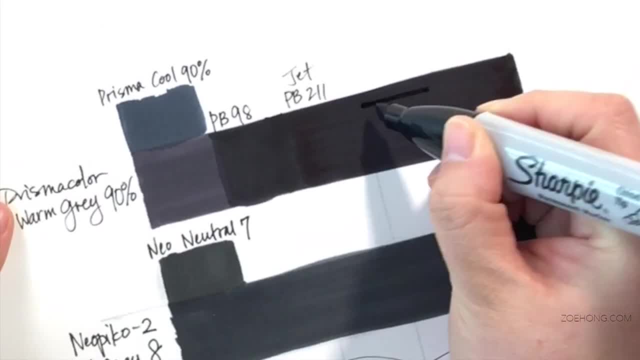 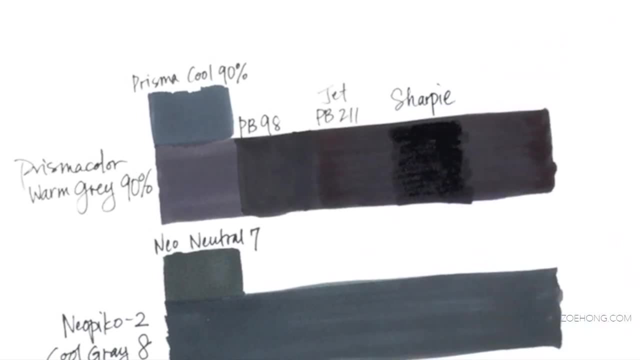 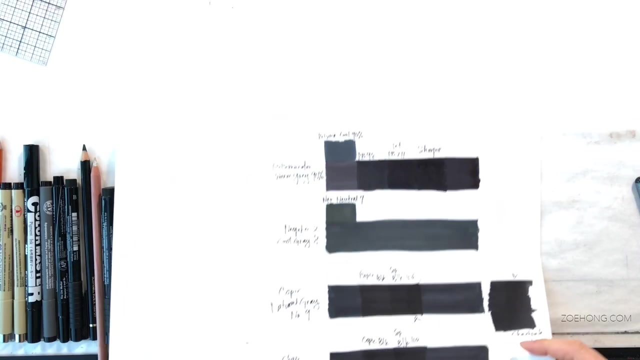 Underrated, I think. So now I'm testing out a Sharpie. sometimes I use a Sharpie because it's black and it's very black, as you can see again, just kind of making that jet black look not very jet at all. 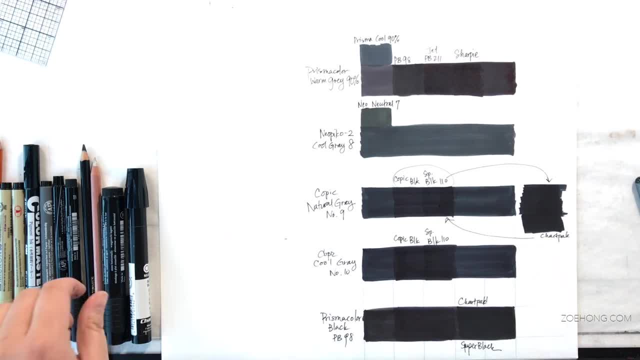 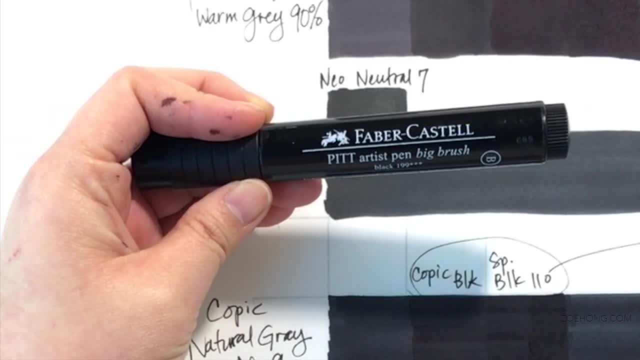 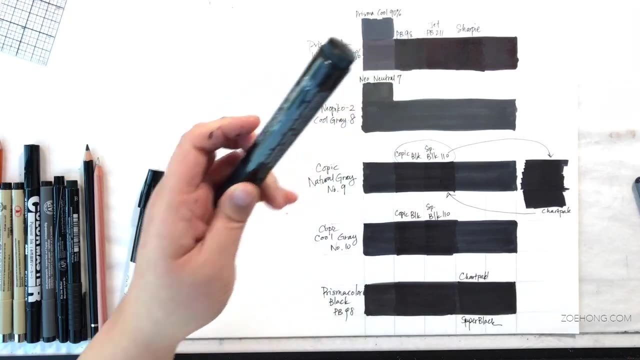 Now I have quite a few markers. Of course I don't have every marker under the sun, not every black marker, But this is the blackest marker I have ever seen. This is the Faber-Cassel Pitt Artist Pen Big Brush Pigment Marker in black. one ninety nine. 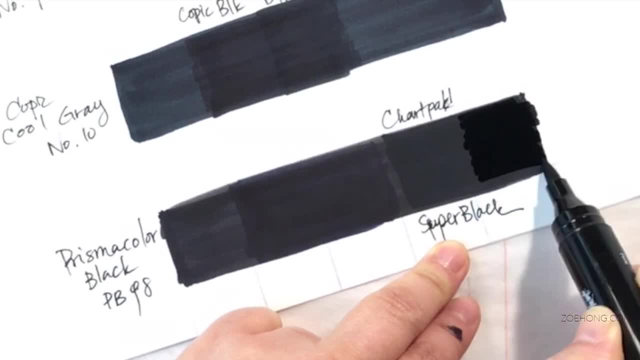 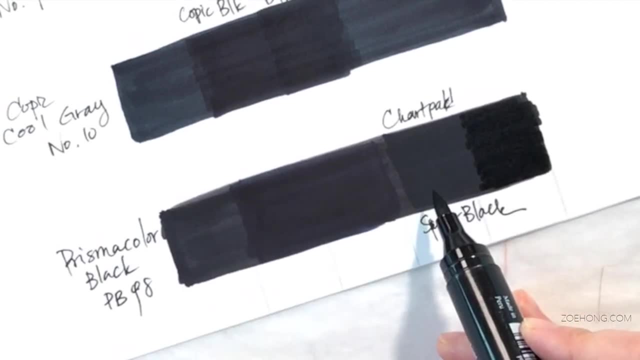 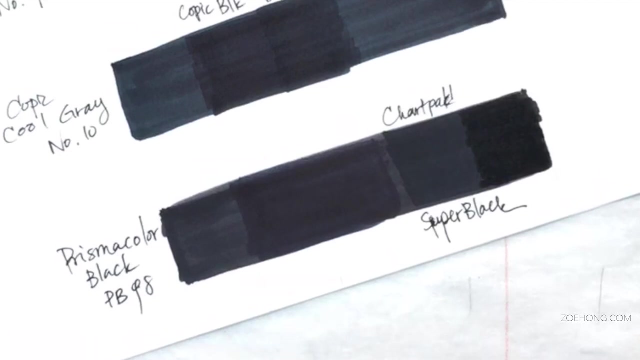 And it is black y'all, Seriously black. Look at that. I mean, hold on a second. We have to let it dry first before we really see the color. But do you see how, like all like the other blacks, Like this whole row is? they're all labeled black, but they just look like. 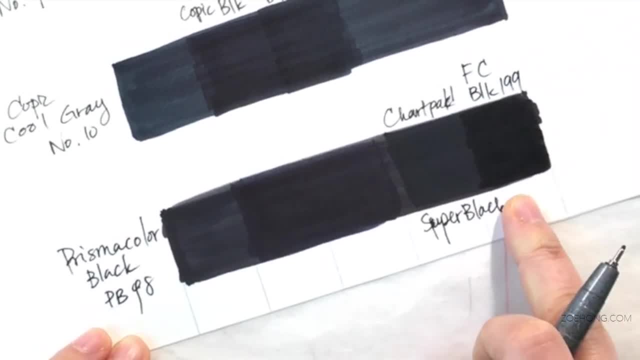 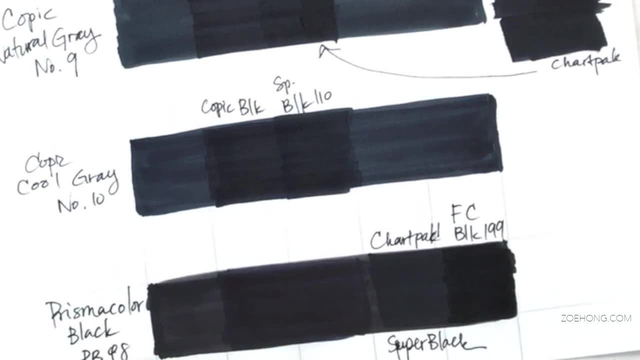 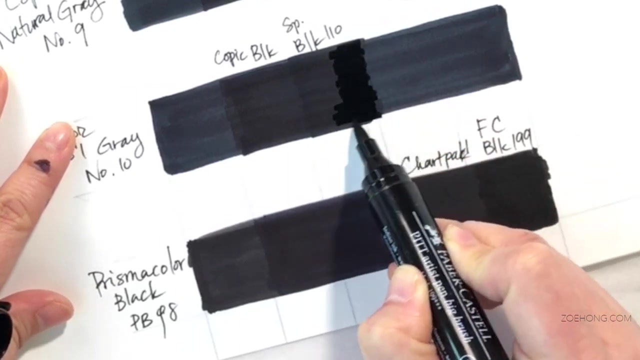 wimpy little 50 percent grays in comparison to the Faber-Cassel black. Look at that. OK, see, now it's dry and you can really see how black it is. And that's the most intense black. Look at that. This is layered on top of the Copic Special Black. 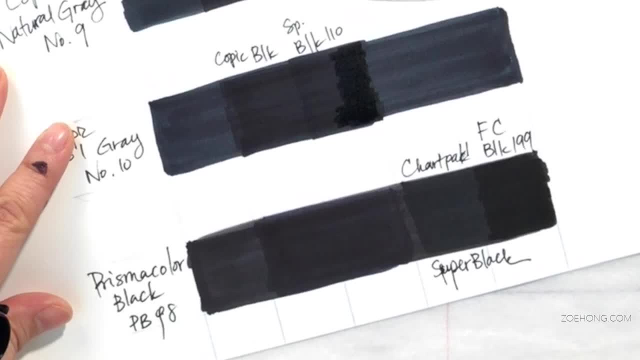 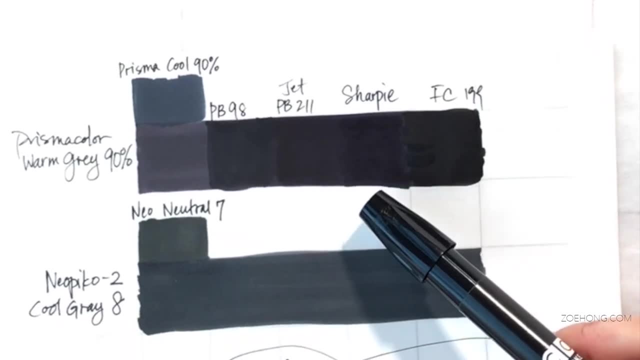 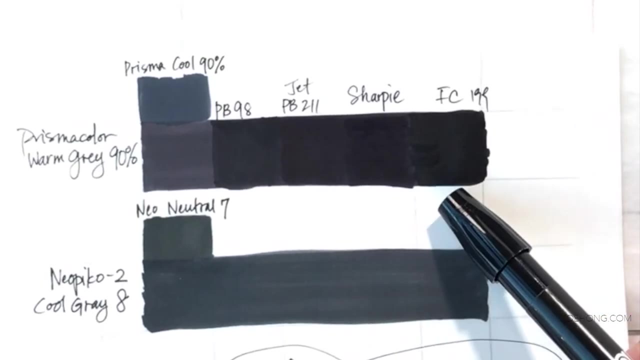 Sorry, Copic, your black is not all that special. And here's the Faber-Cassel black compared to the Sharpie and Yeah, look at that. I mean there you can see a bit of a tone difference. But yeah, that Faber-Cassel it's so black it has no tone. 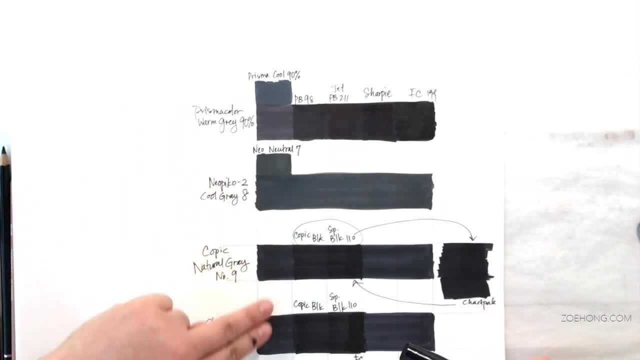 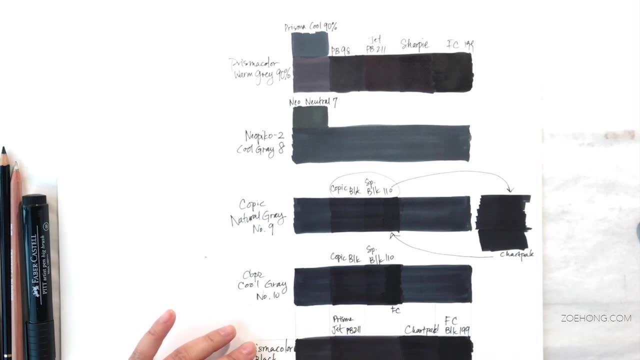 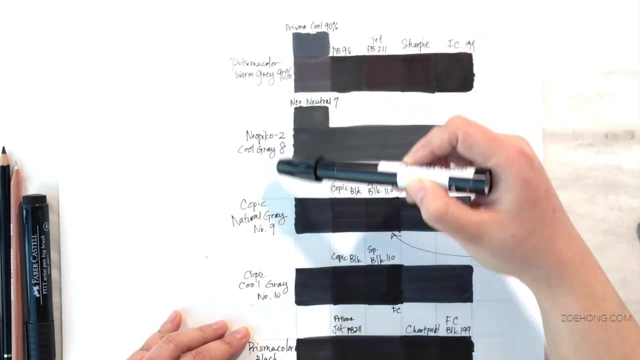 It's just black. Now, at this point, you may be thinking, Zoe, I'm not going to be using any of those dark grays, I'm just going to go with the blacks that you showed me, since you showed me several shades of black. 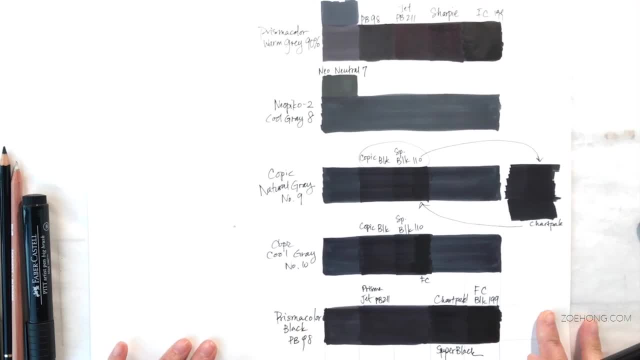 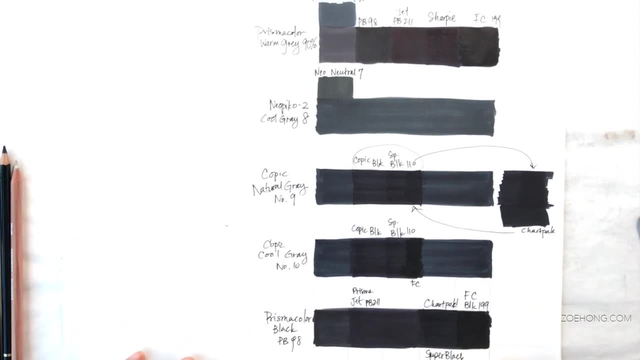 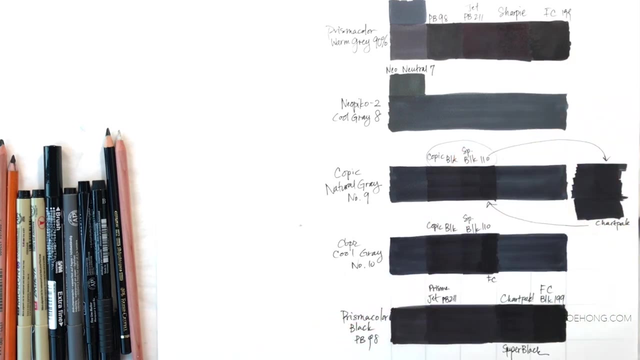 All right, Let me talk about the flip side of that for a second Number one. remember this video is overexposed to show you more clearly the differences. So remember: these grays are going to look darker in person without crazy blasting studio lights. 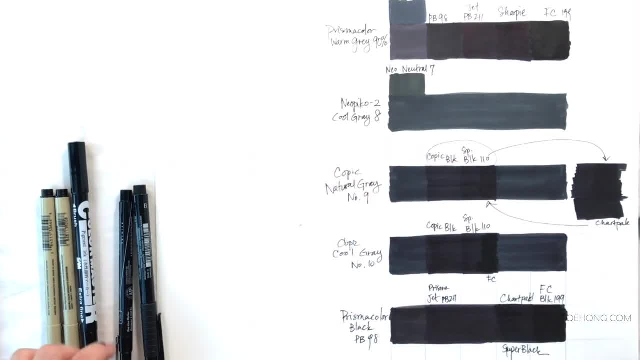 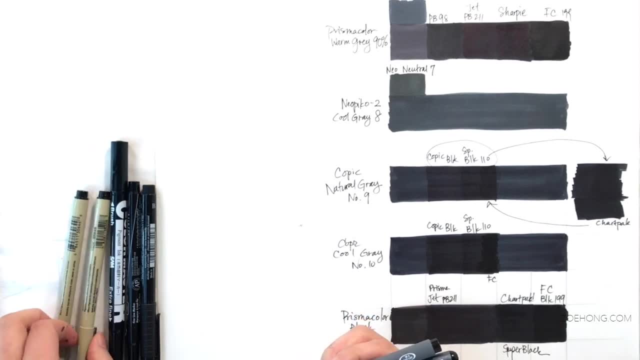 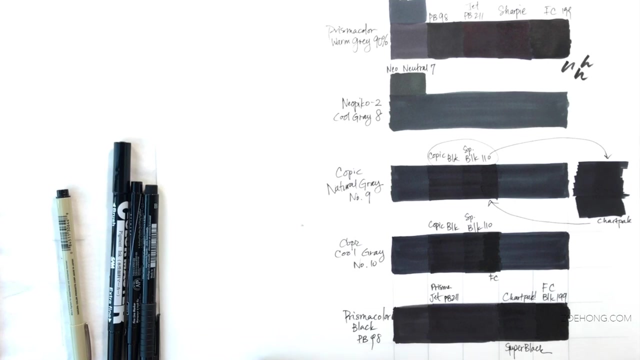 OK, number two: Using dark blacks or light blacks and the blacks and whatnot are fine if you don't need to put down a lot of design details and textures on top, But if you want to do that, you are going to want to use another black medium to draw. 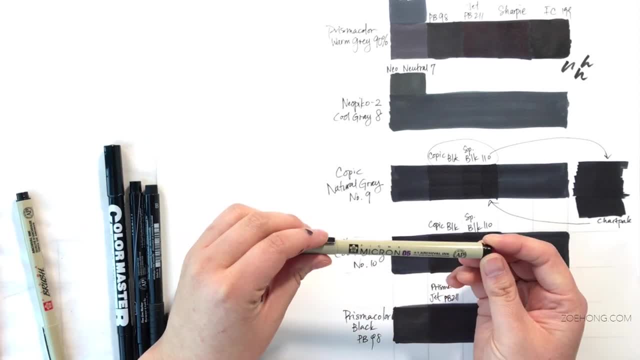 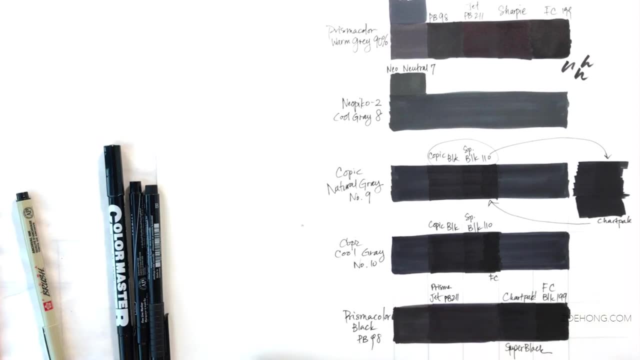 and illustrate textures and design details on top, And so it's better to use these darkest grays so that when you use a black fine liner, a black color pencil, to put in these details, those details show up, you know, depending on the look. 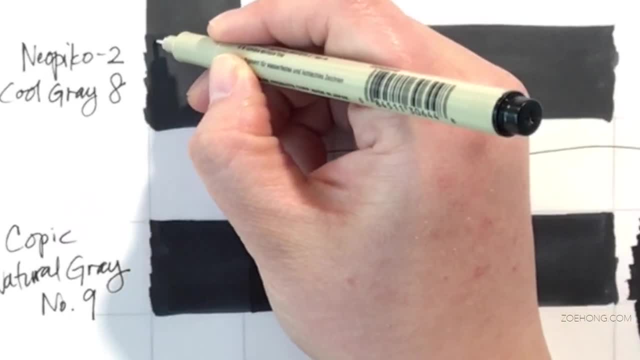 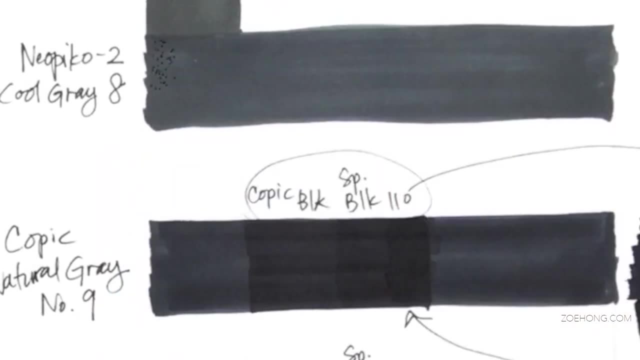 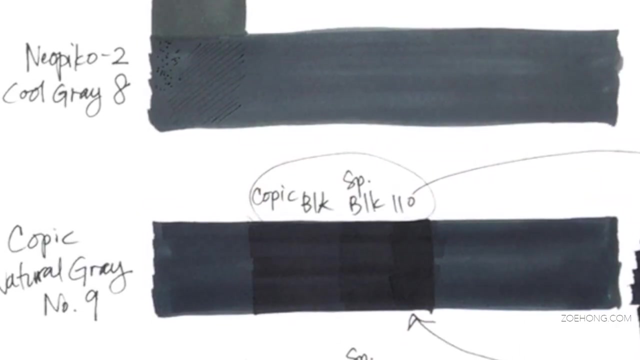 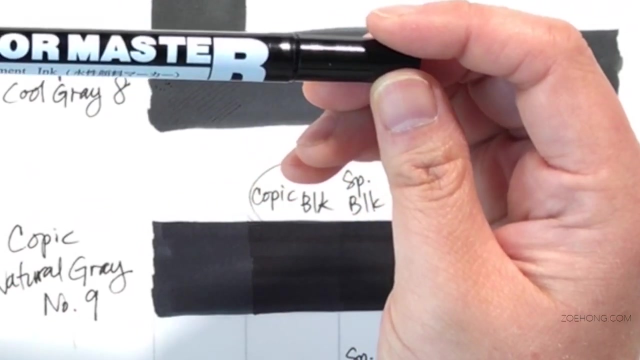 that I'm going for. if I want to really blast out some design details, I will outline things in white. If I want a more subtle look Or for textures, I will use black on top of a super dark gray. I use fine liners from Copic Staedtler, Prismacolor and the Sakura Microns. 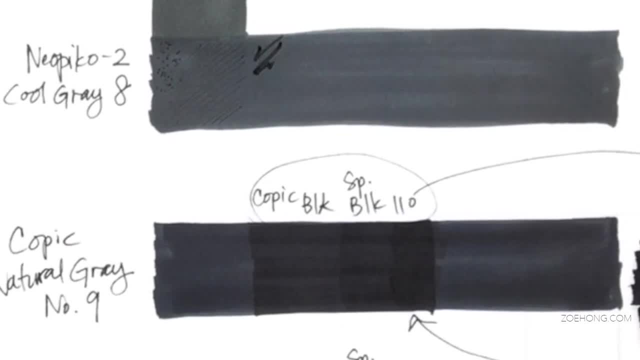 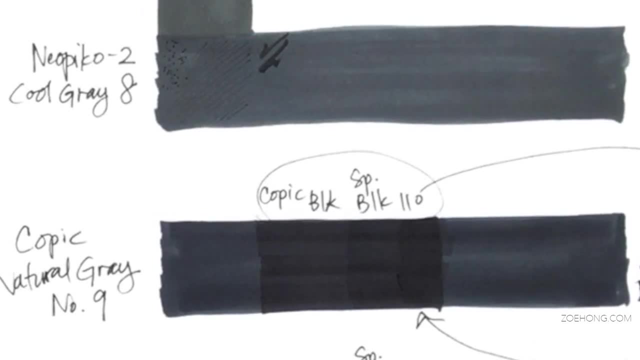 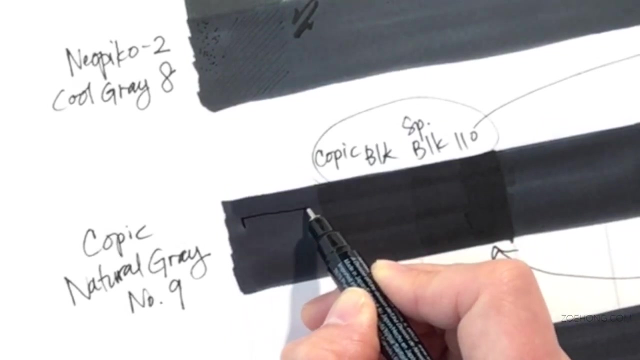 which seem to be the industry standard, although I don't find them any better or worse than the other brands I mentioned. And then, if you watch my first visual playlist, then you know that these color masters, I use them as fine liners And you can use brush pens to put in textures and details. 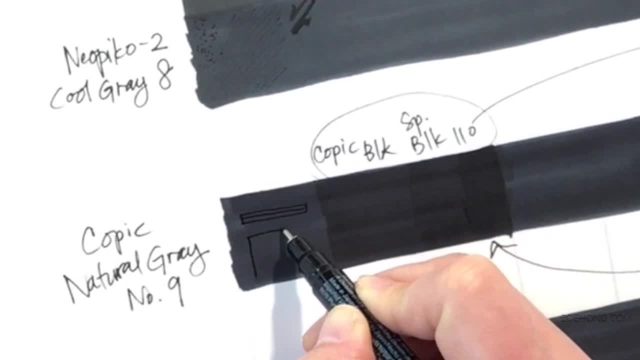 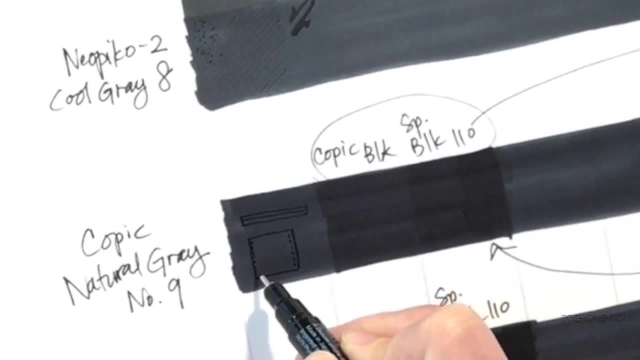 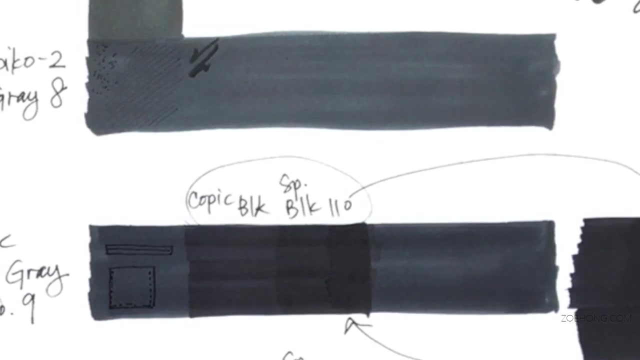 or draw patterns or prints on top of the dark grays. I use black fine liners to draw in design details, like these pockets that I'm doing right now, and top stitching Again if I want the more subtle look. sometimes I want everything to pop. 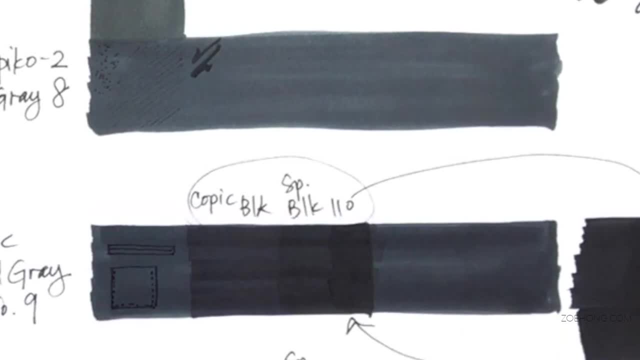 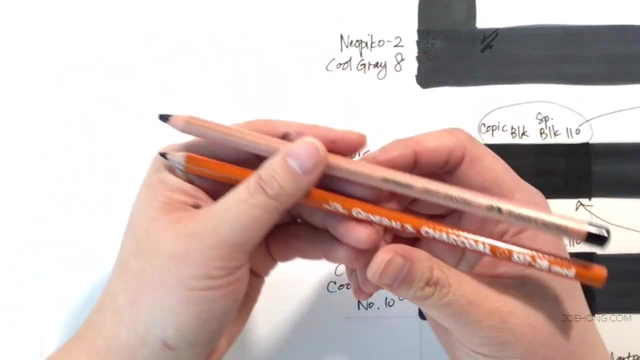 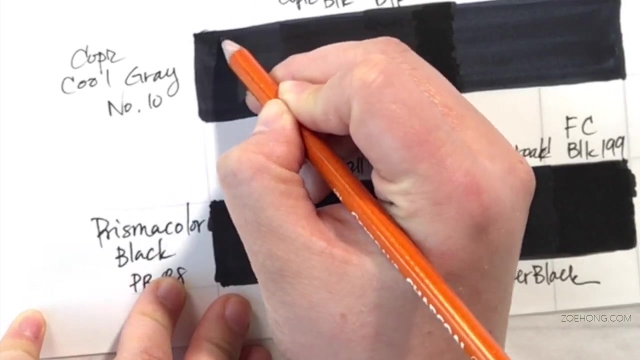 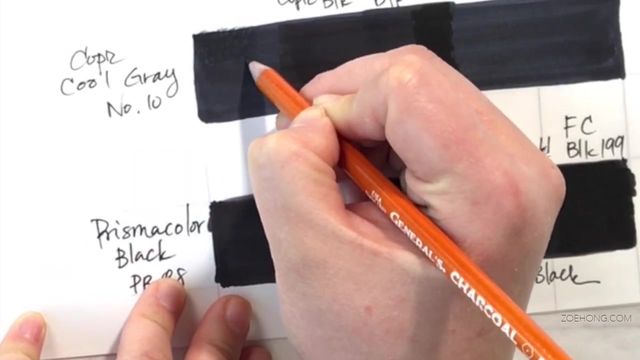 and be super clear. so I'll use a white instead And I will demo that in a future video in this series. I'm going to go over a few of the black pencils that I use. If I want a fuzzy texture, I will take a black color pencil or charcoal pencil and illustrate those. 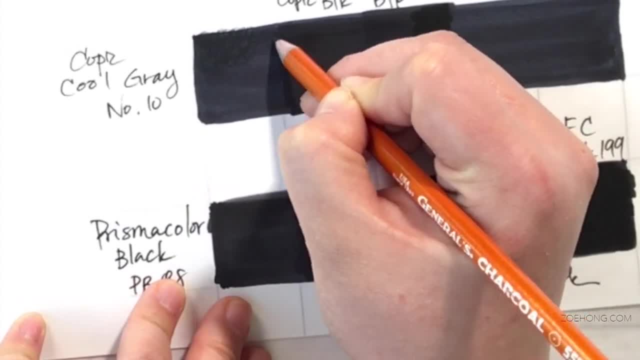 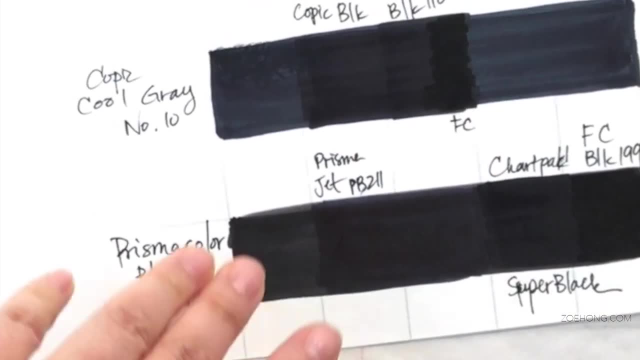 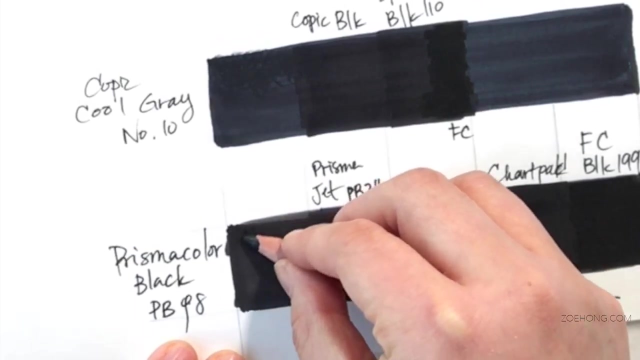 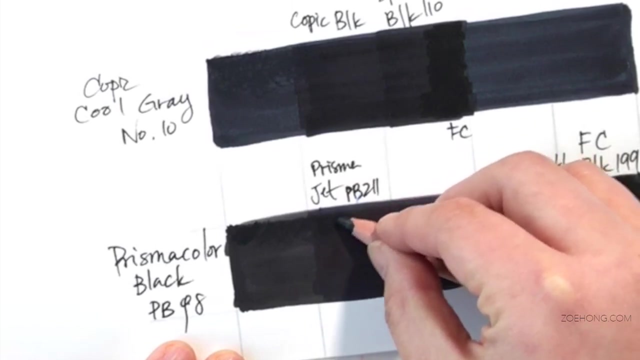 textures on a lighter black. This one is almost too dark for the fuzziness to show up Again. it's really about matching your fabric and the look you're going for. Maybe you want something lighter, like the Prismacolor Warm Gray 90 as your background to put soft mohair boot clay cashmere. 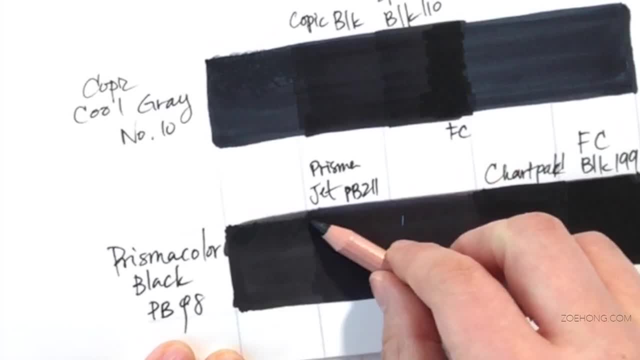 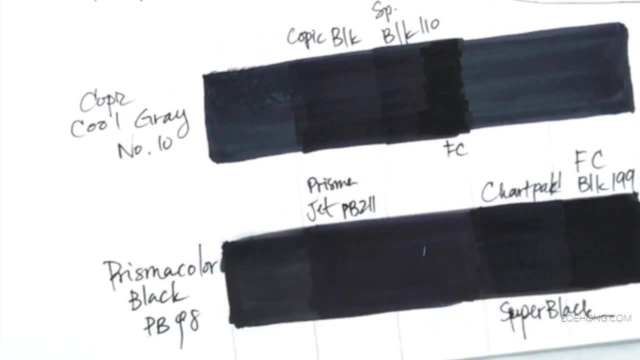 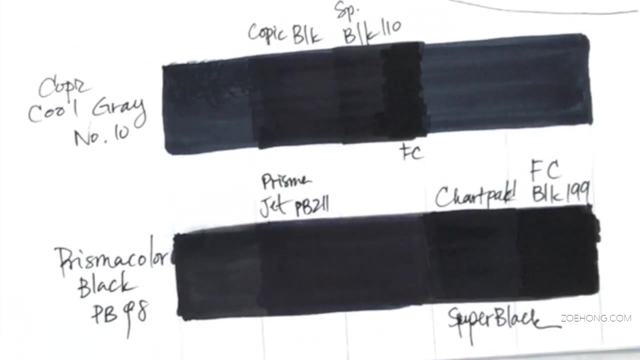 textures on top with the charcoal pencil, like I'm showing you right now. Now, when you put the black charcoal pencil on top of the shadow color blacks, the darker blacks. yeah, they're not going to show up that much, but it's fine. 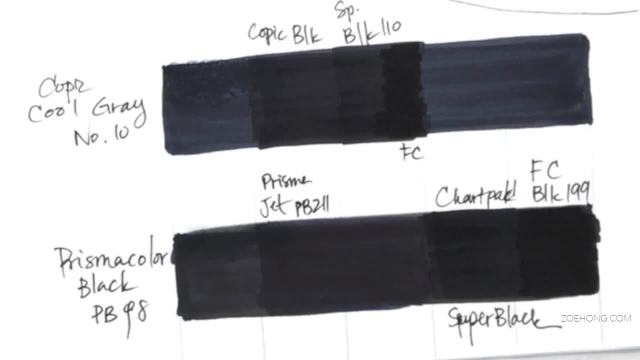 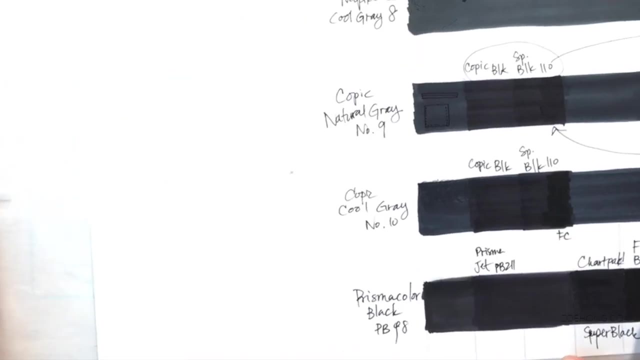 Most details and textures show up less in shadow garments In general anyway. I mean, unless you have really light color garments, you know, even in a blue garment you're going to see less detail, less texture. you know, in the armpits, under shadow areas, things like that. 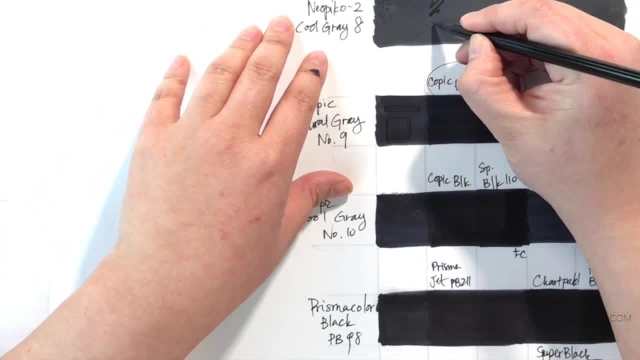 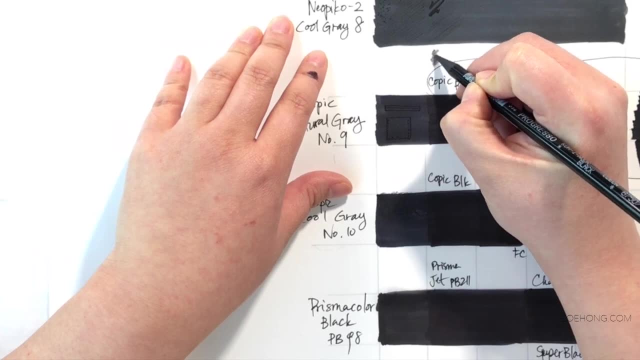 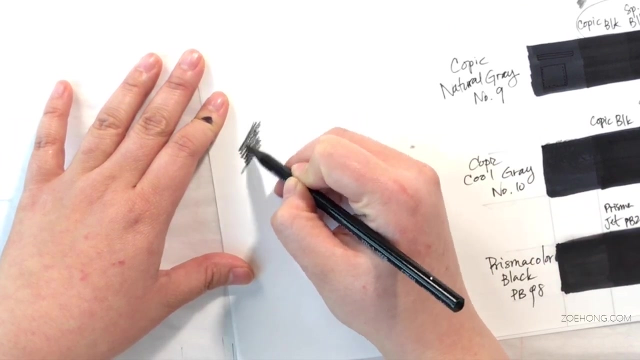 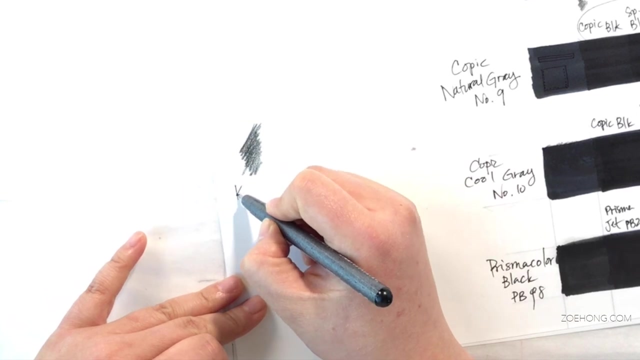 There are some varieties of values and tones in color pencils as well. But you know, with color pencils values can be determined more by how hard you press and if you use blenders like blender pencils or the alcohol, rubbing alcohol or baby oil. those tricks I went over in the shading with color pencils. 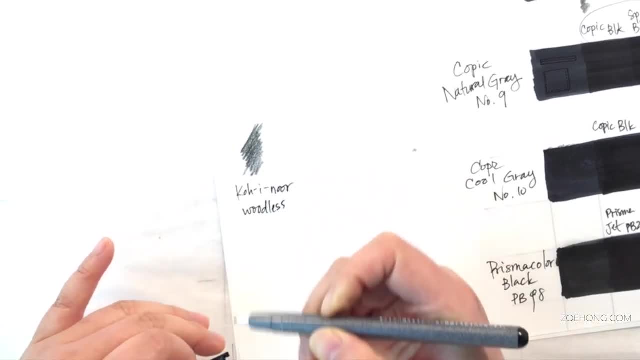 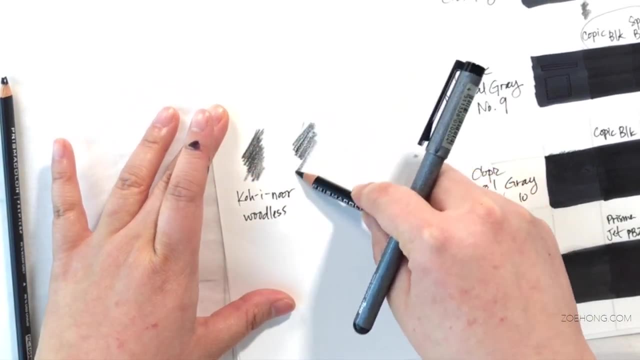 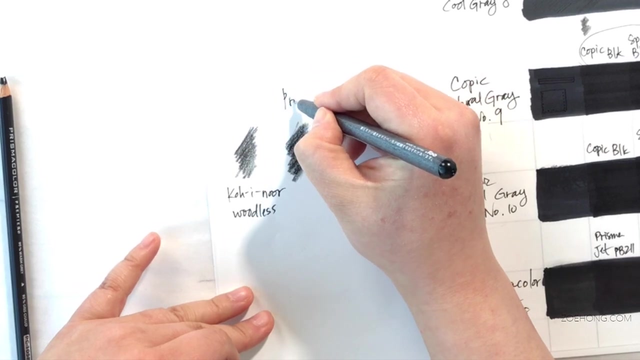 video. this is the Koh-I-Noor Woodless pencil. I really like it. It's a very firm pencil and it makes for doing delicate details pretty nice. This is Prismacolor Black, and long time viewers know how I feel about Prismacolor already. 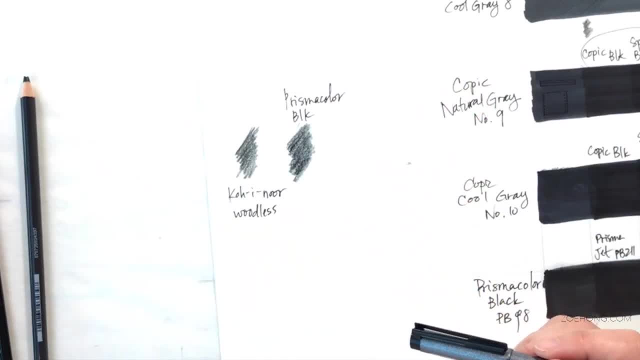 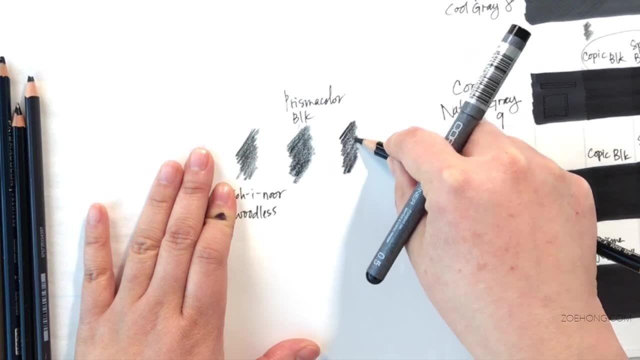 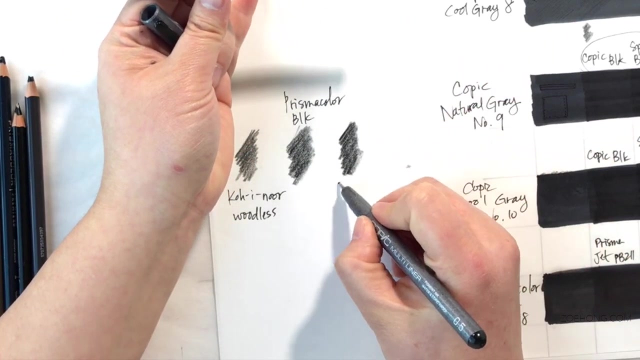 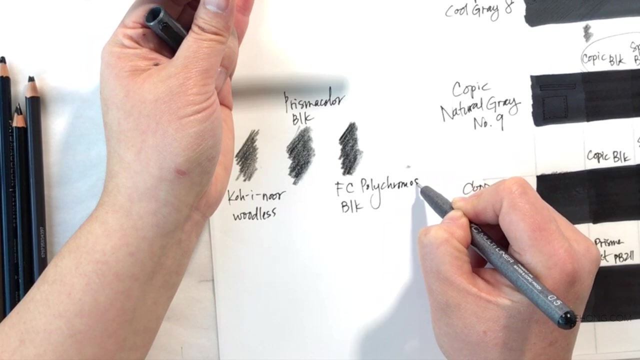 The colors are nice, They blend beautifully. Their leads are soft and snap, Even if you think about sharpening them. I have a few of You have been recommending the same color pencil sharpener to me and they say it works like a dream on Prismacolor. so I'm about to get that, because those 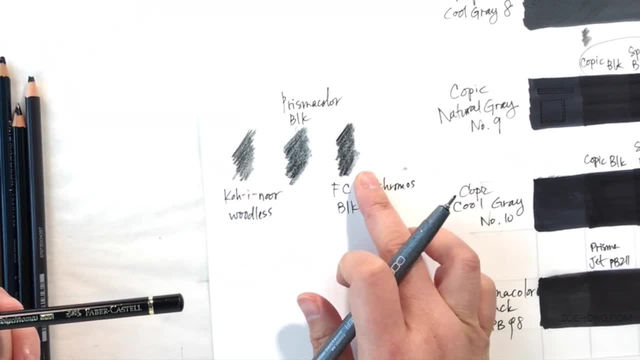 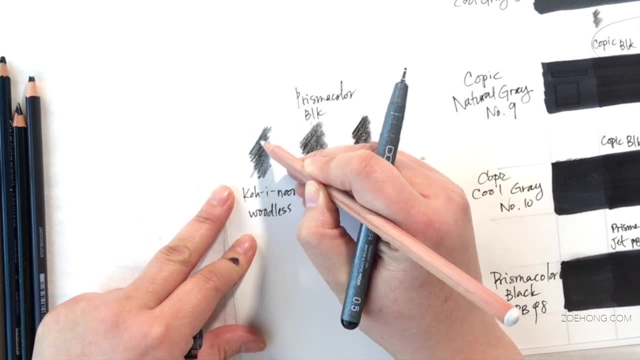 Prismacolors are no joke. And then this is the Faber-Cassell Polychromos in black, And you know they are just a high quality color pencil in general. Now I'm just putting the little blender on these so you guys can see how. 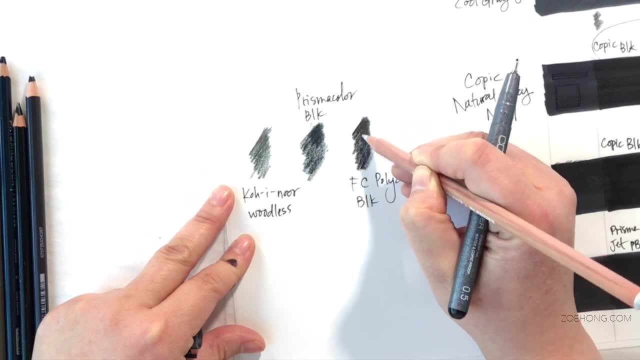 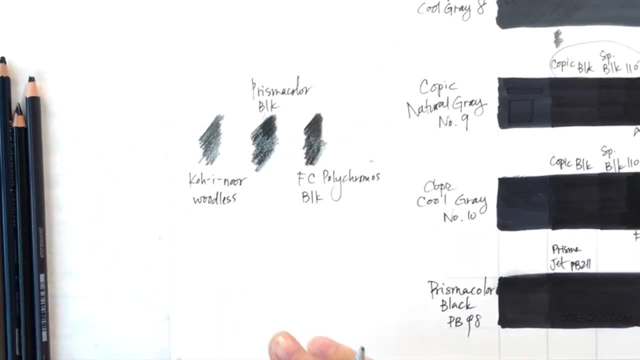 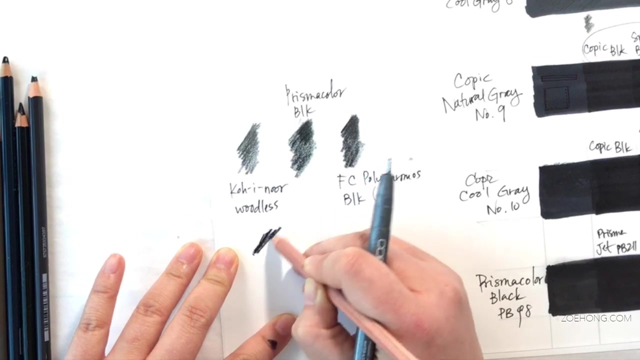 that effect looks. The Koh-I-Noor is a lighter black. Again really great for the detail work because it really keeps a point. The Prismacolor Black is quite black with a bluish undertone And because it's so creamy it reacts to that blender really quickly. 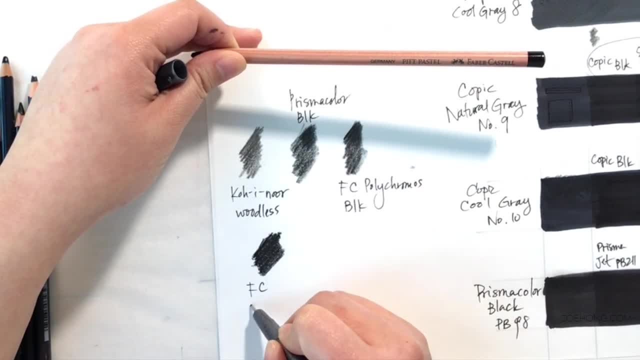 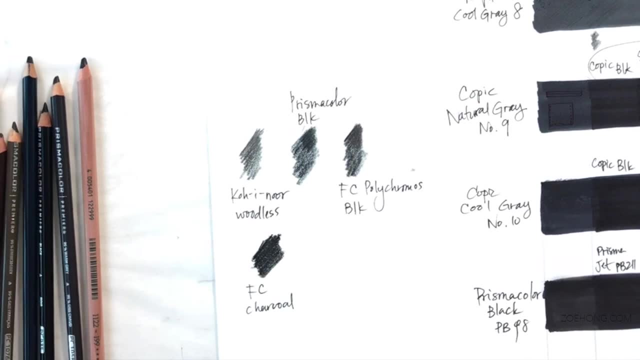 And then the Polychromos has a more neutral tone to it. So, depending on what you're going for, I also like to use charcoal pencils for some detail works. I don't use full on charcoal because- oh the powder, it flies everywhere. 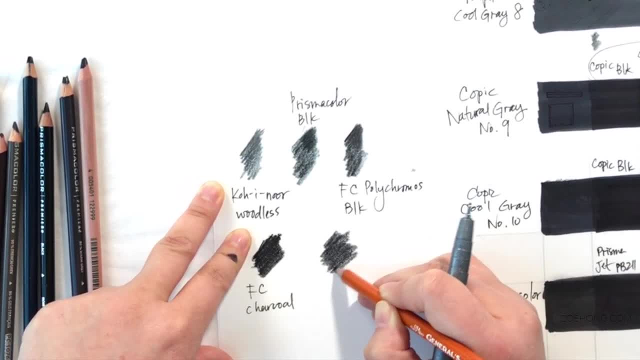 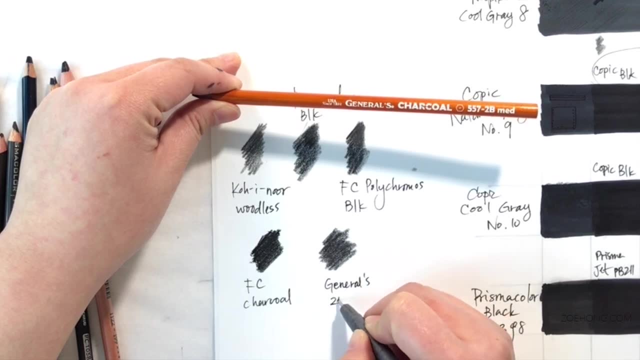 Charcoal pencils are much cleaner and neater and not as much kick up. The Faber-Cassell charcoal is the cleanest. The Generals I like I have in several lead weights- See the difference between the 2B and the 6B. 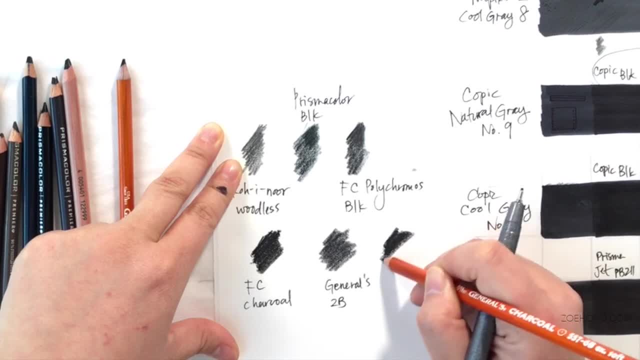 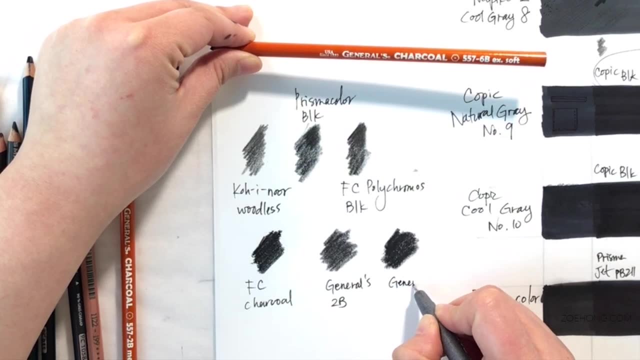 The 6B, of course, is softer and darker, just like with pencil lids, you know, the 6B is really soft and dark and the 2B is still soft, but not as soft and dark as the 6B. 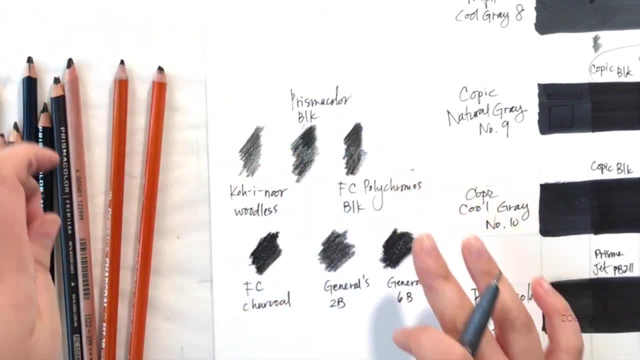 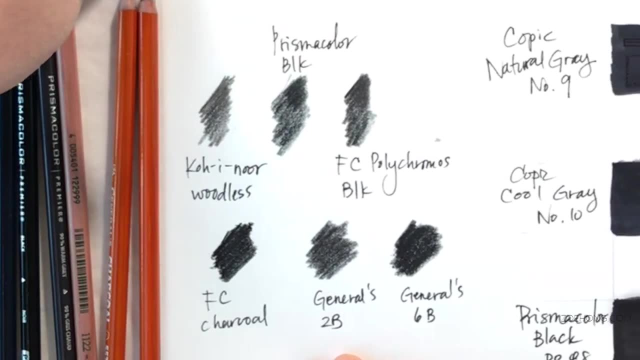 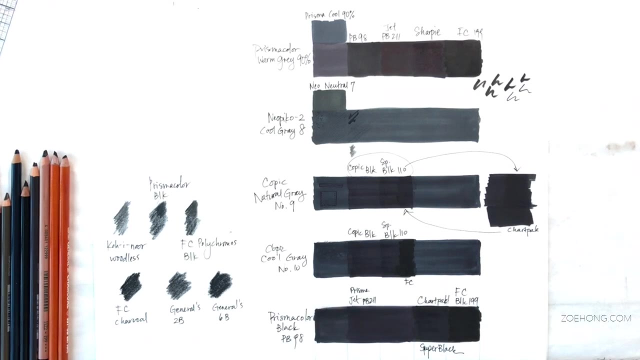 So there you have it. Look at all of these markers and color pencils and charcoal pencil options for you to get started on illustrating your black textures. Look at this chart, Isn't it hilarious? Like that, those Prismacolor warm grays- 90 percent. 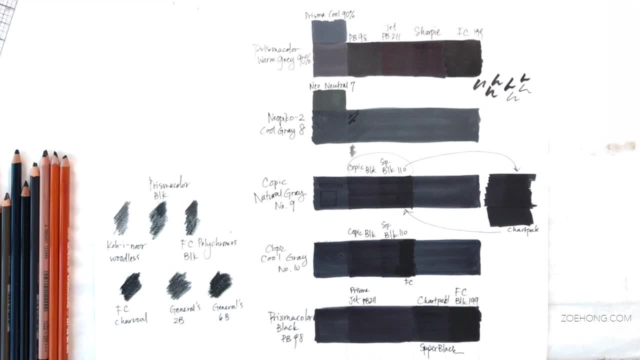 They look so light in comparison to all the blacks that I showed you. And now that everything is dry, look at that bottom bar- You can really see how dark that Faber-Cassell black is. Look at all those shades of black, right. 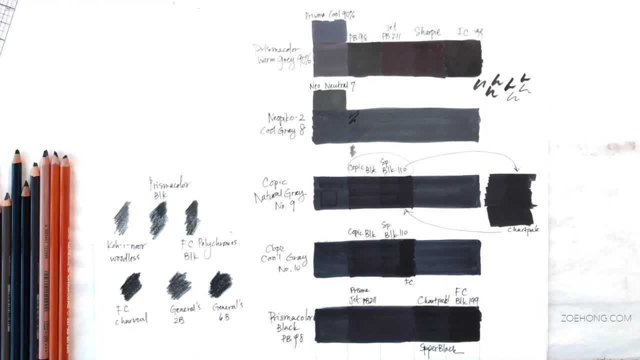 As this series continues, I'm going to go over other media and then start doing some small sample illustrations of different textures you can create using the media I introduced in this series. But as a starter video, I hope this was helpful to help you figure out what 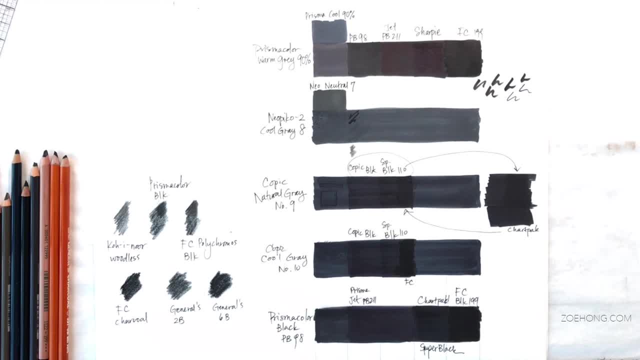 markers and color pencils you should buy to get started on your black illustrations. If you found this video helpful, please hit the thumbs up button. Subscribe, if you haven't already, so that you can get a notification for when I continue this series. Share this video. 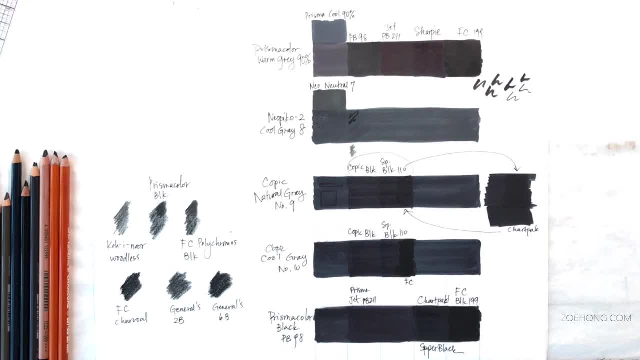 With anyone who loves designing with and wearing as much black as I do. my students in class really freak out when I wear something that's not black. They're like: what are you doing, Zoe? What's going on? I don't understand.